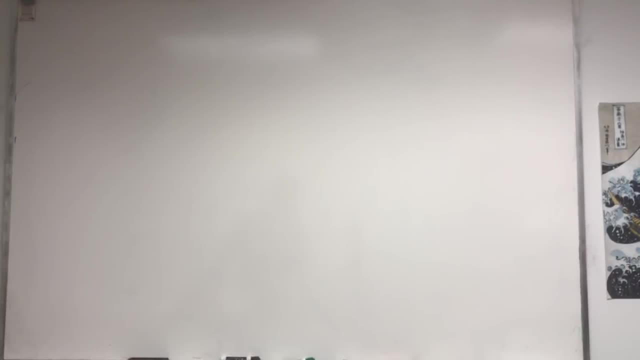 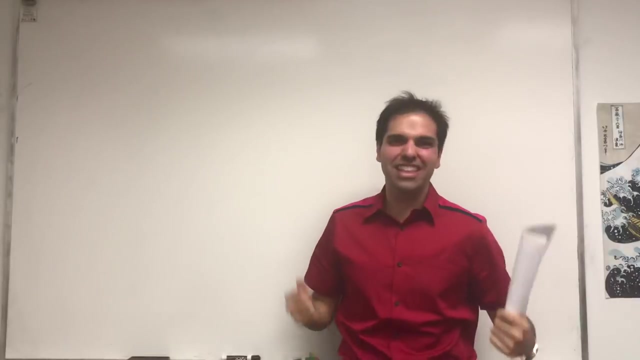 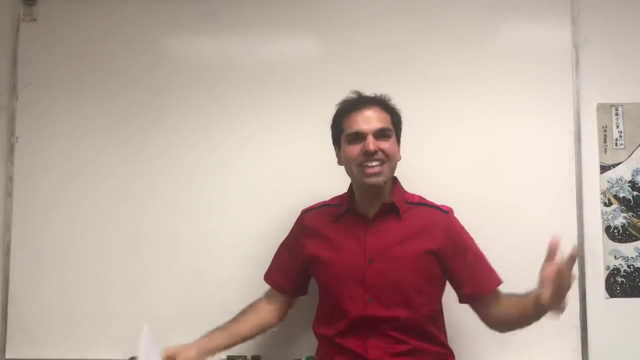 3, 2, 1, Dr Payam, Hello And welcome to our 111 true-false linear algebra questions extravaganza. Because Black Pen told me I should do a crazy marathon and I was like: well, he's done integrals. and I was like, well, why not just do linear algebra? So let's. 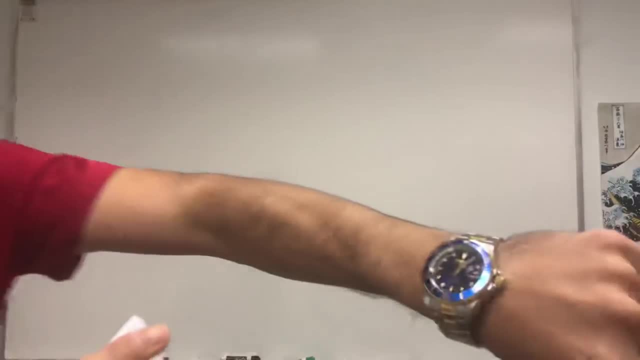 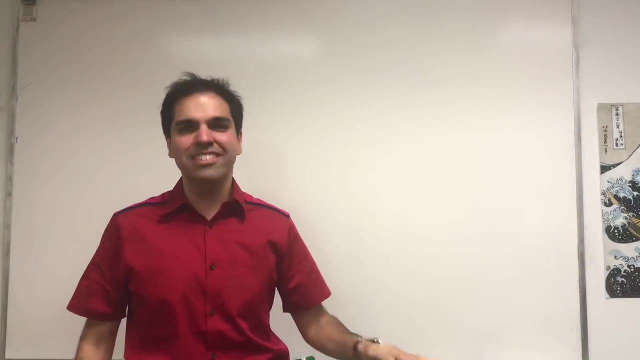 see how long it'll take. So just that you have proof, it is 1 over 7, and let's see, maybe I bet with him it'll only take 2 hours. but he was like, ah, you think it's gonna? 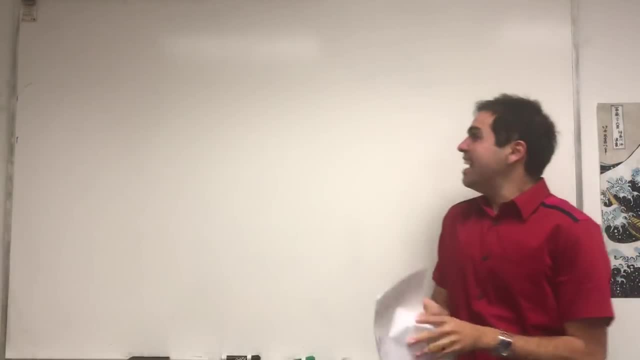 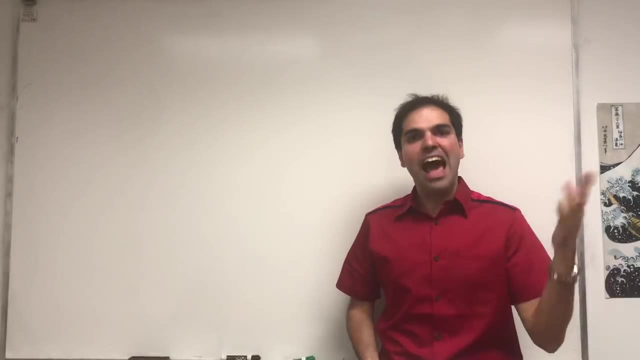 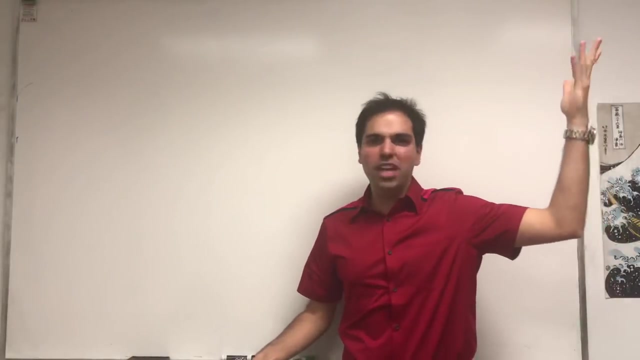 take 2 hours, but it'll take longer, We'll see. And also to make this even more fun, because there are 111 questions, I actually googled what the 111 most popular languages in the world are. Google gave me some lists from 1997.. I don't know how accurate this is, but let's see. 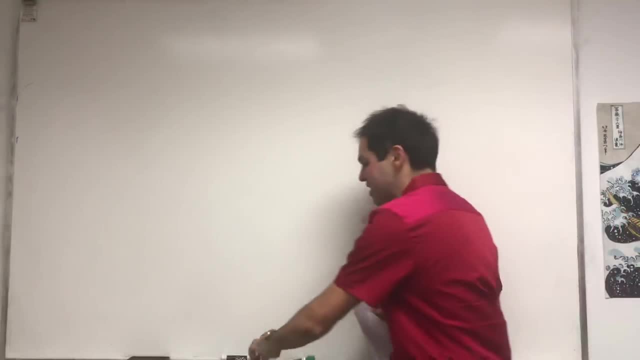 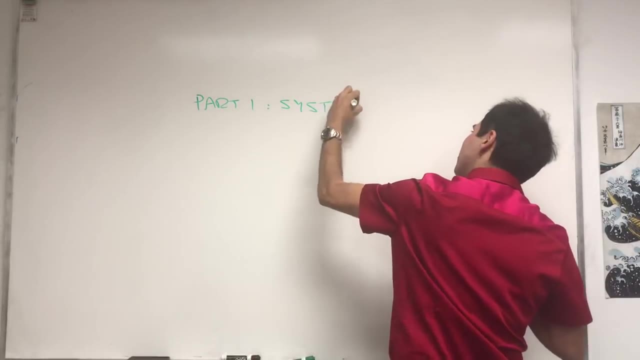 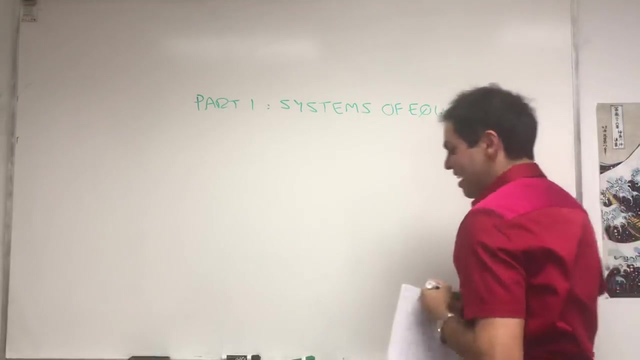 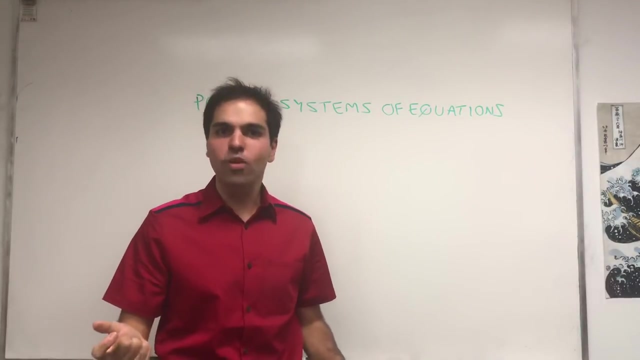 So the first part deals with systems of equations, So part 1.. So let's do a couple of true-false questions with systems of equations. And so, first question, and the most popular, The most popular language in the world is Mandarin, and 1 in Mandarin is eeeeee. 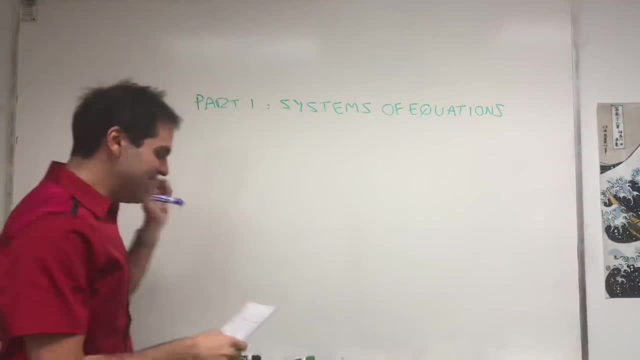 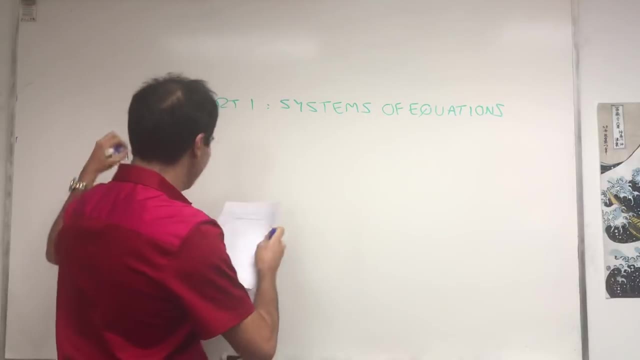 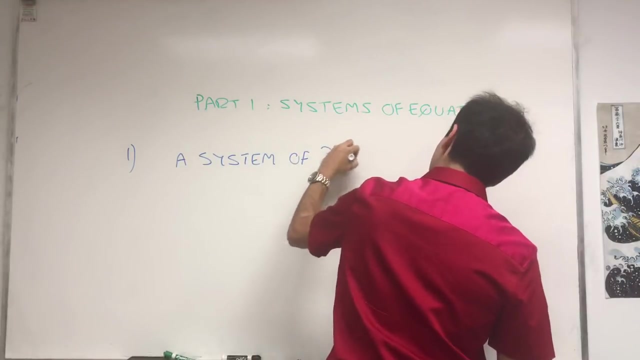 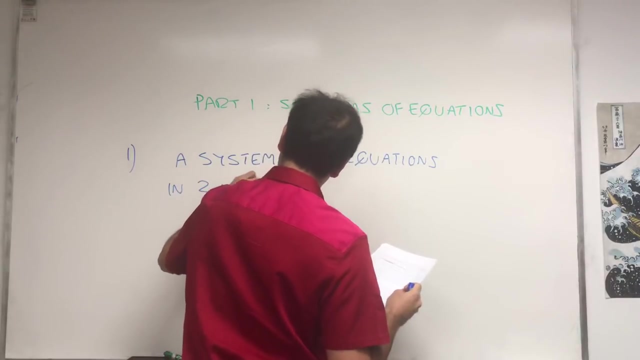 It's so cool, It's like: eeeeee, I'm so excited. So question 1.. Well, that's off to a good start already. So question 1. A system of three equations in two unknowns must have no solutions. 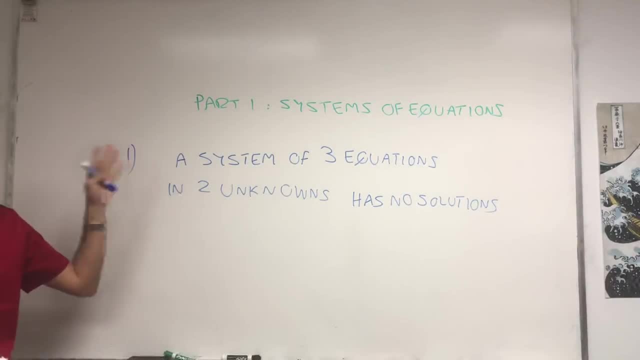 In other words, if you have more equations than unknowns, is it true or not that this must be inconsistent? So think about this and while you're doing it, let me check if the video is actually recording, Because otherwise I'll do this for five hours and no one will ever know. So let's see. 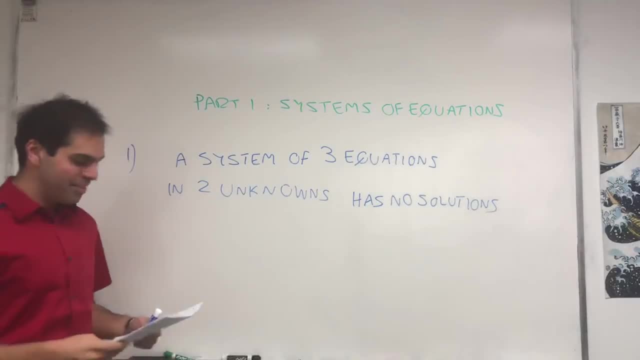 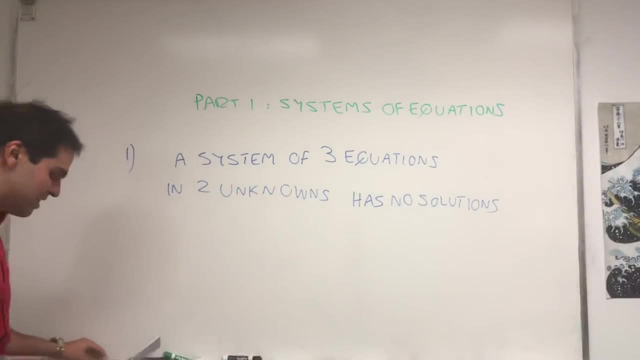 Yes, indeed, it is recording. so that's good, All right, True or false? Well, it turns out this is false. Just because you have more equations than unknowns, it doesn't mean that you have more than that. you have no solutions. 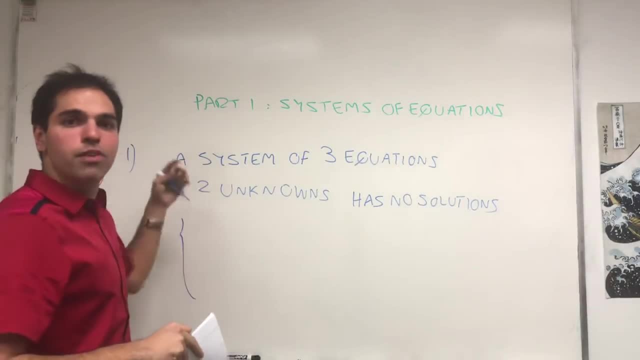 And, in fact, let me give you a system with a lot of equations, Not that there are no equations, Not that there are no equations, Not that there are no equations. It's a system- we have many unknowns- that has a solution. 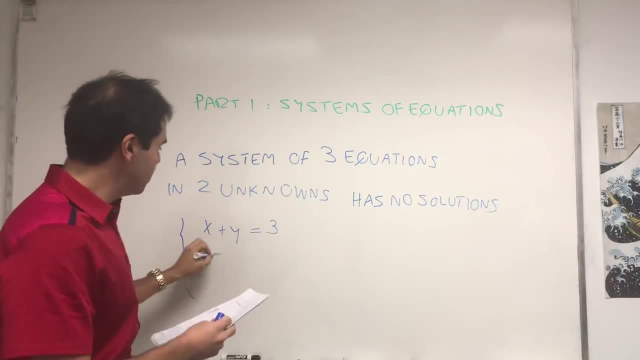 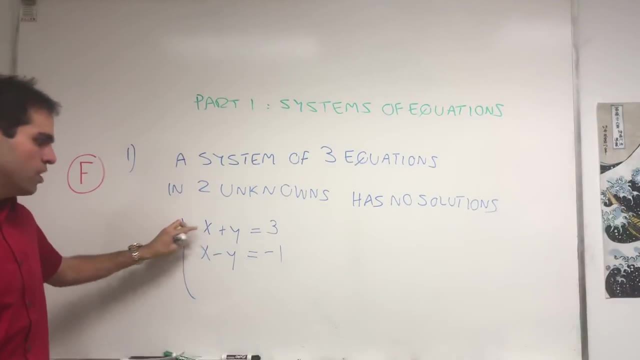 So x plus y equals 3.. x minus y equals minus 1.. So you can actually check. this has a solution already. And for the last equation let's just do 2 times the first equation. So 2x plus 2y equals 6.. 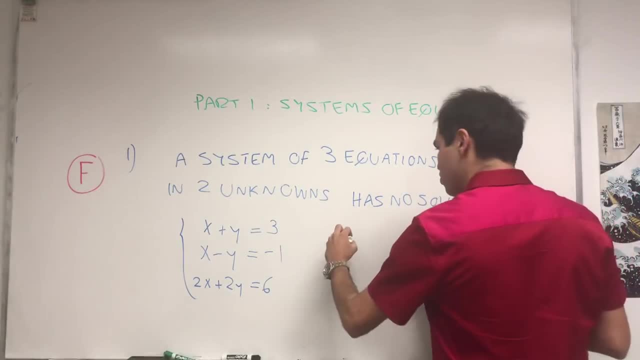 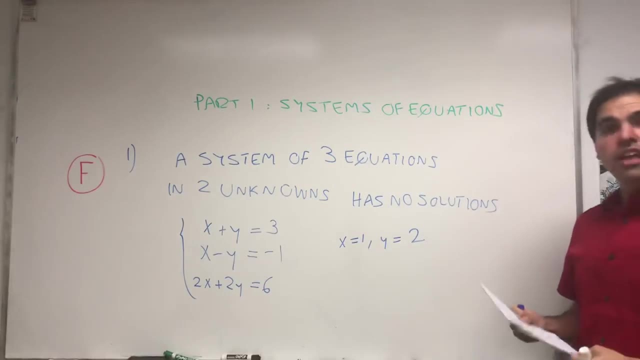 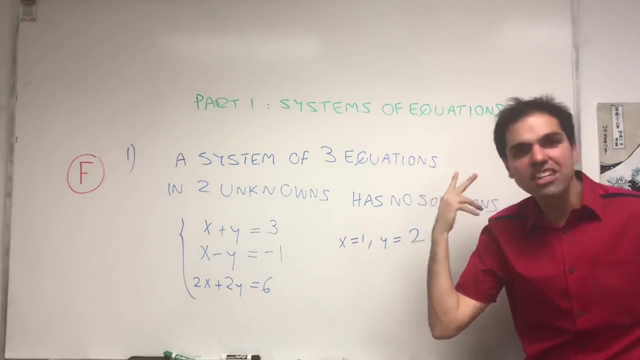 And it turns out, I think, x equals 1 and y equals 2.. If you do that, then you get that this has a solution. So in general, the number of equations and the number of variables doesn't really matter if it has a solution or not. 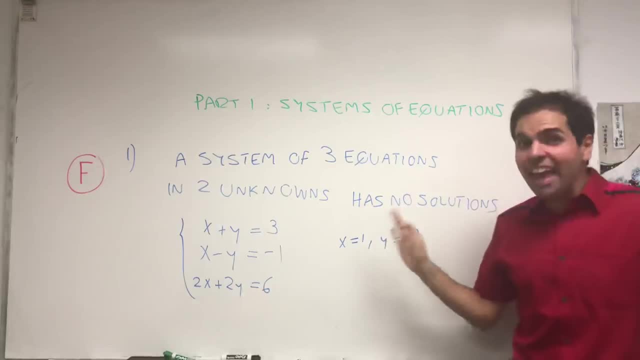 And you may say: what can we say about those equations? All we can say is there is some choice of the right-hand side. So here is 3 minus 1, 6. It could be 2,, 4, 7 or something. 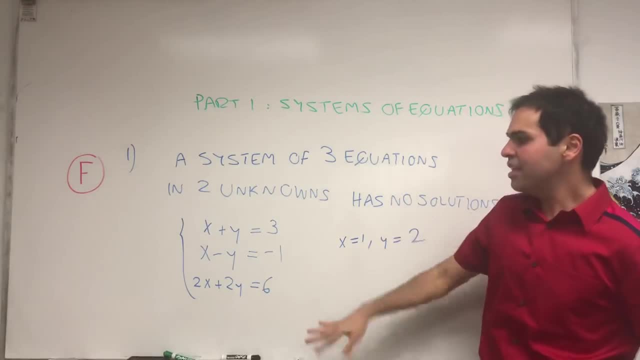 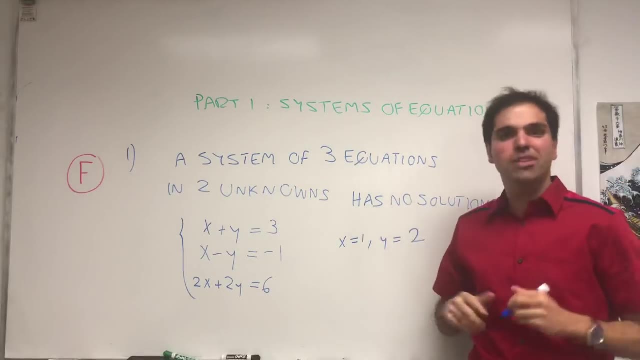 There is some choice of the right-hand side that gives you no solutions, because it turns out this equation has two pivots and the pivots are really what tells us if it has a solution or not. So the right-hand side, for some value, has no solution. 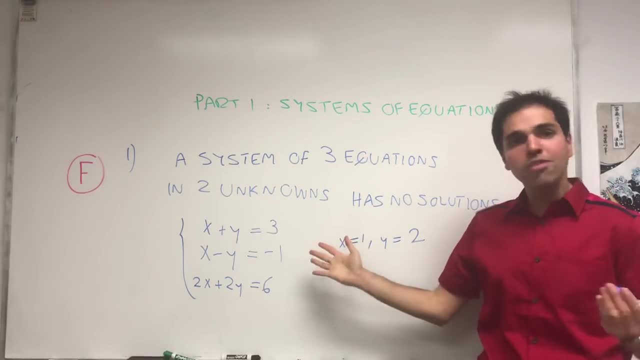 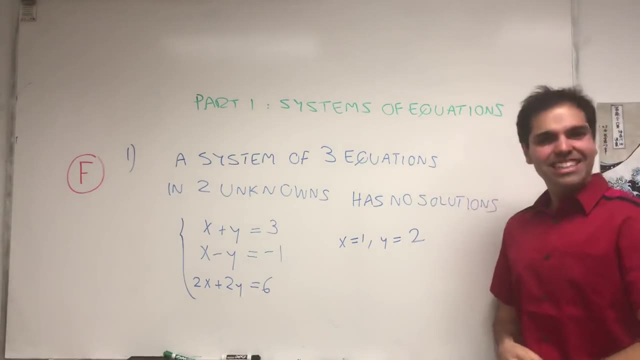 And that's all we can say In general. that's it In general. if I give you a value, it may or may not have a solution and we can't really say more about this. Good Question 1, and then 110 questions to go. 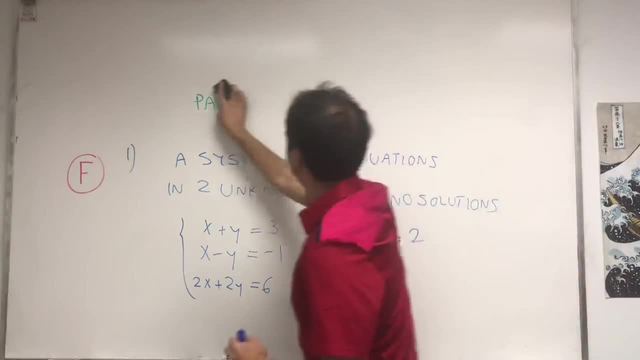 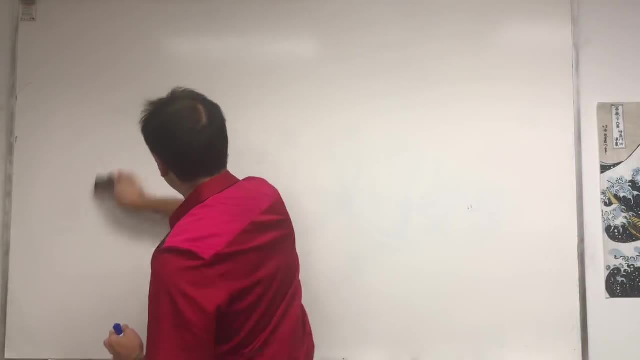 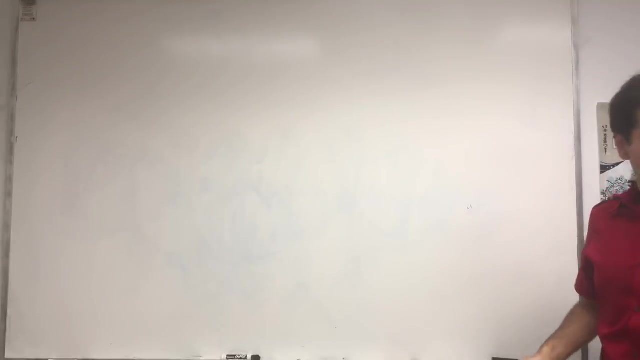 So let me erase that. Let's see Question 2.. And let's also see how messy this whiteboard will get. So now let's do a question, Question 2.. So what if I put two equations in the opposite direction? 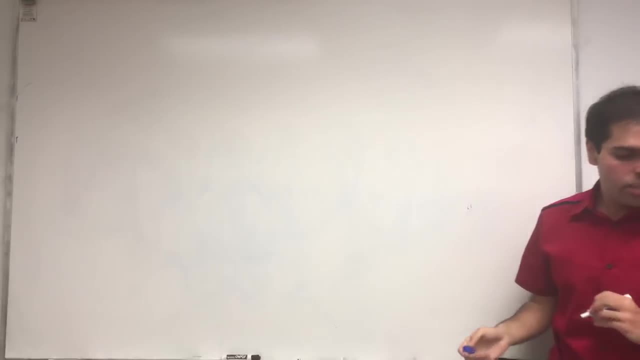 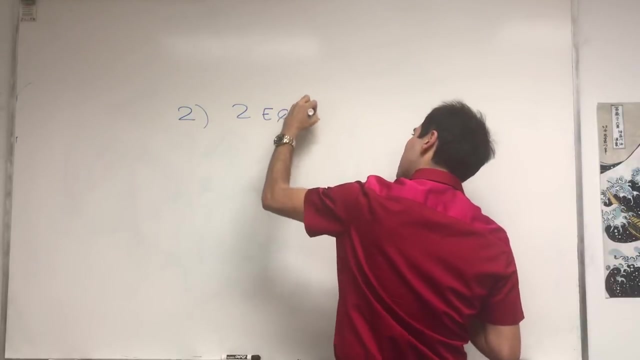 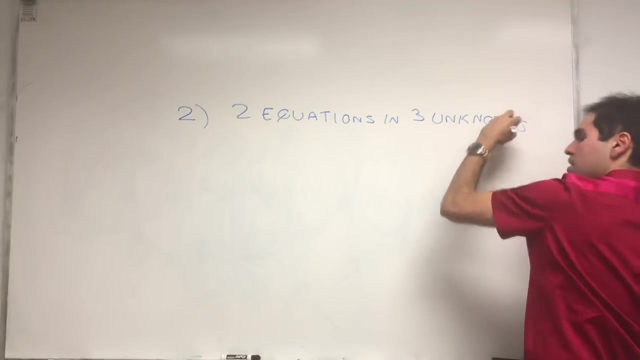 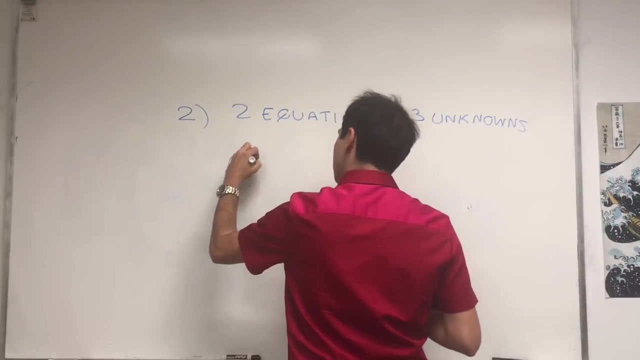 So before we had three equations and two unknowns. what if we have two equations and three unknowns? Two equations and three unknowns cannot have exactly one solution. Question 3.. Question 4.. Question 5.. Question 6.. Question 7.. 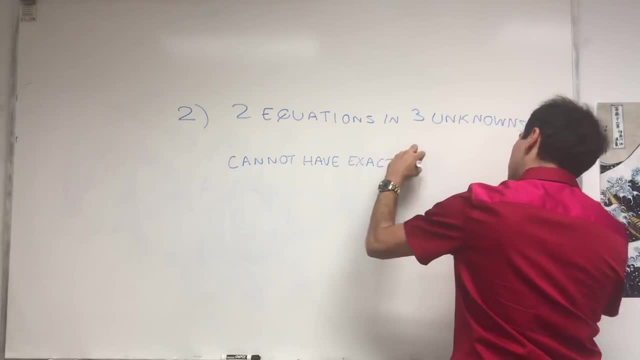 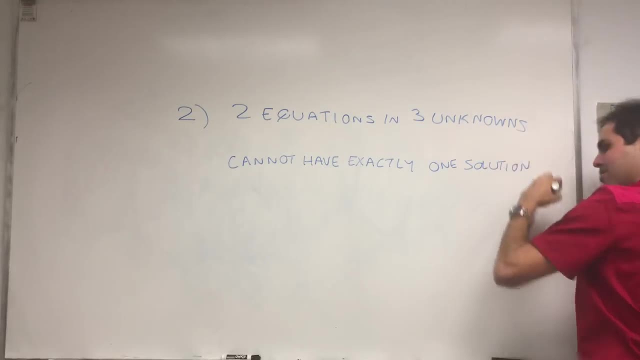 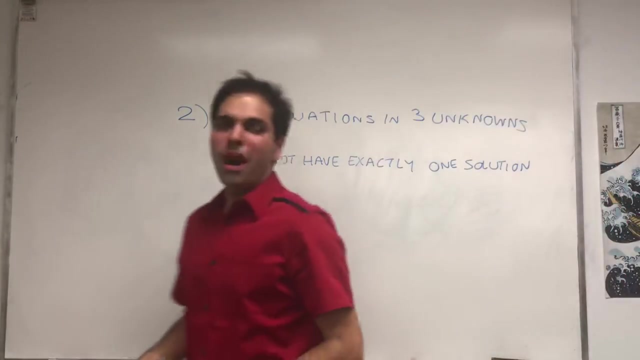 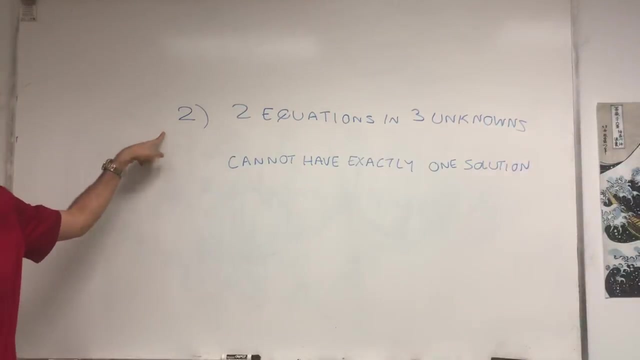 So could it, or could it not, have a unique solution? Think about this and, while we're at it, the second most popular language in the world- sorry, it's not English, but Spanish- and two as in dos, like dos equis. 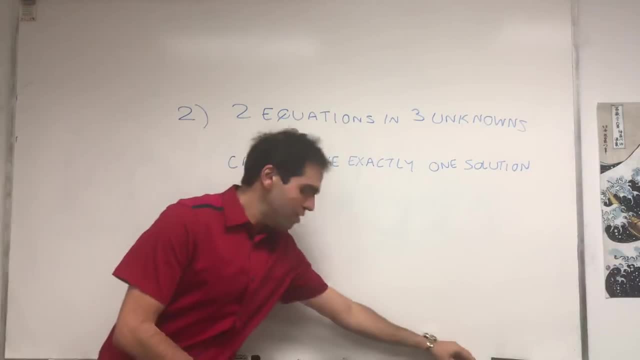 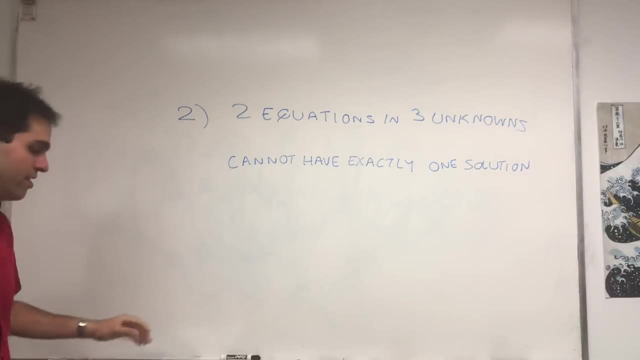 Okay, so very good. alright, let's think about this, and it turns out, drum roll. the answer is true. It turns out such a system can never have exactly one solution, and here is why. So an equi-system of two equations and three unknowns. you can write it as a two by three. 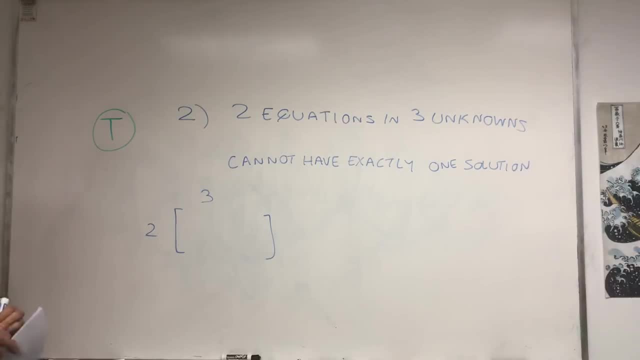 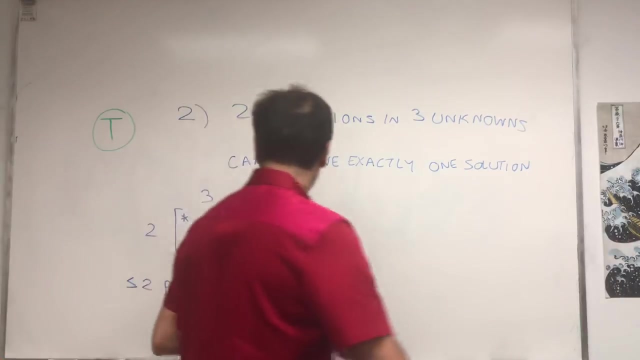 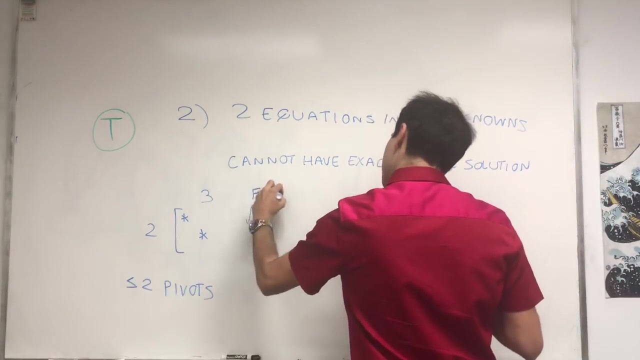 matrix. Okay, And now think about this. so two by three matrix, how many pivots could it have at most? It has at most two pivots, so less than or equal to two pivots, which means the third column will always be a free variable. 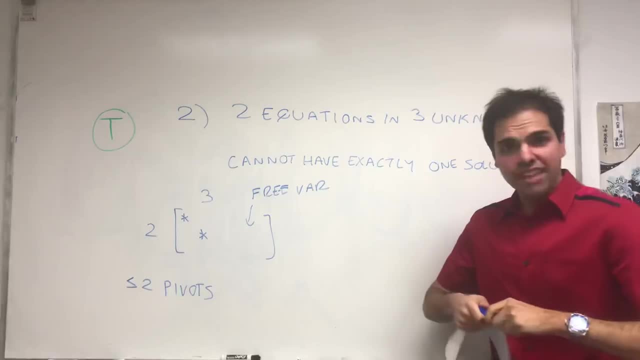 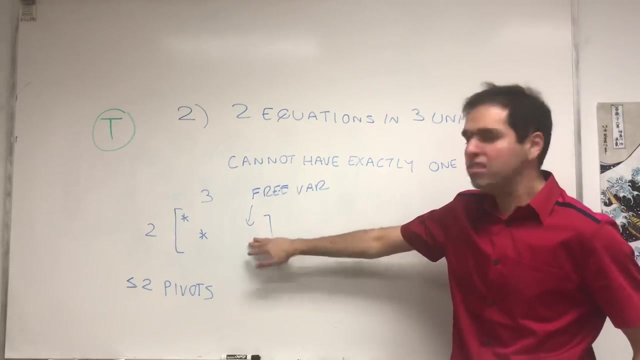 And what does that mean? Well, a system. well, in this case, either it has no solution and then we're done, we cannot conclude anything. but if it has a solution, it's impossible that it has exactly one solution, because because of that free variable you get sort of a parameter of solutions. 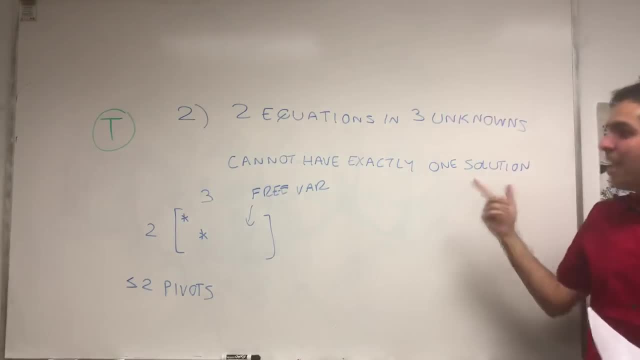 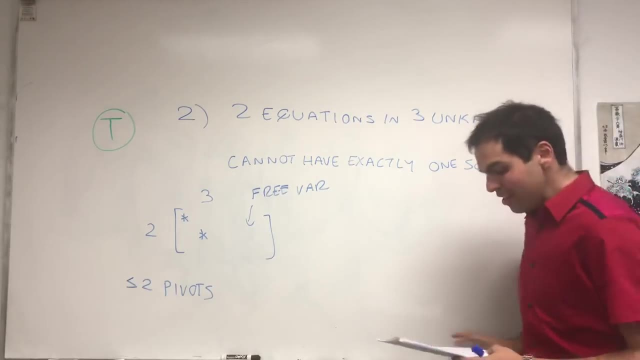 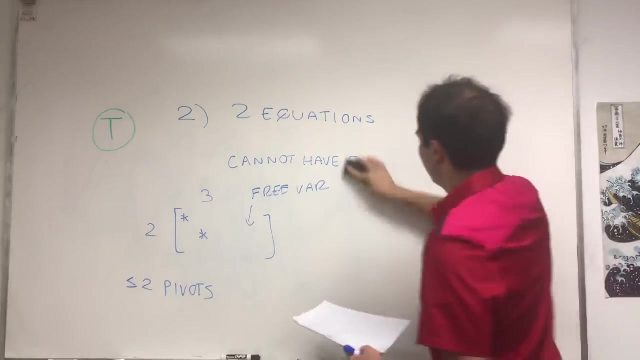 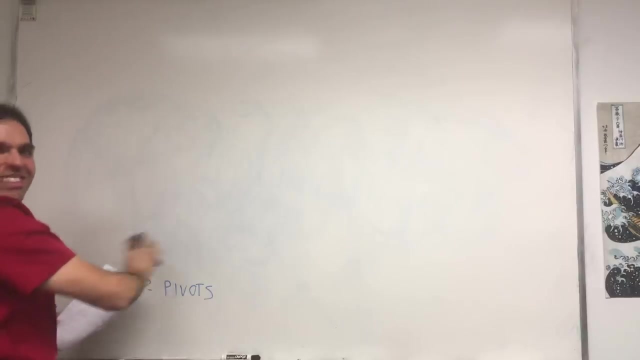 and that's why there are infinitely many solutions. So in that case, either no solutions or infinitely many solutions. there's not much you can say about this. Okay, now let's move on. let's talk more about equations, and now look at the muscles. 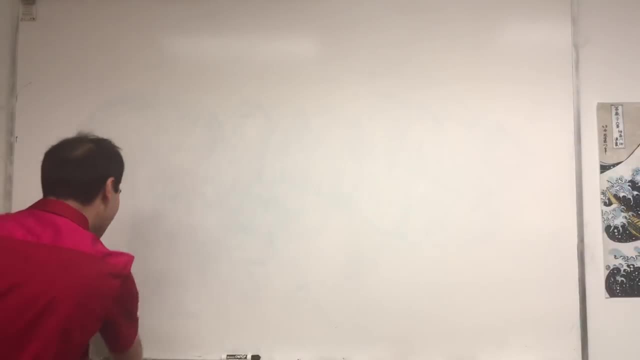 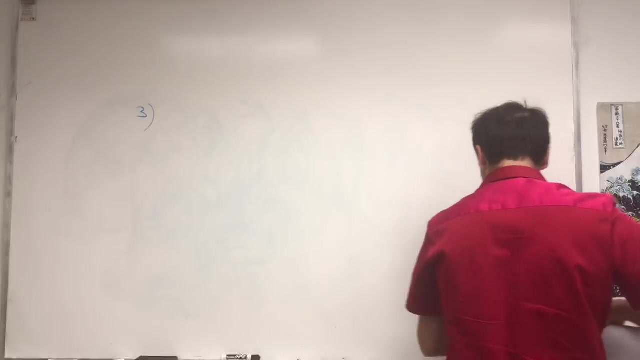 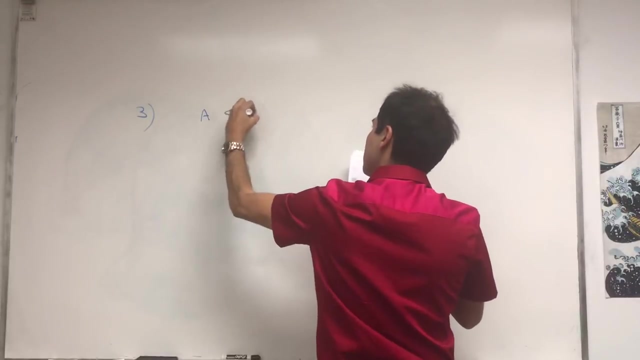 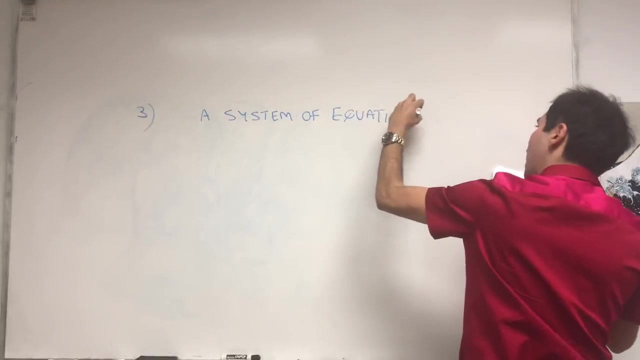 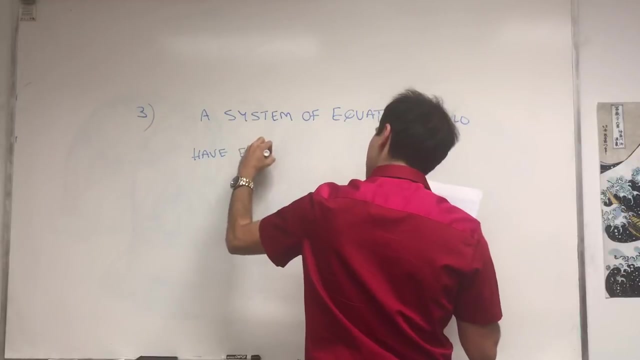 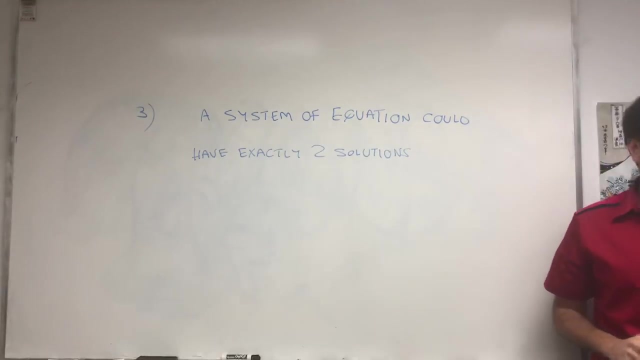 I get by doing this 110 or 111 times, okay. Question three, again talking about systems of equations. so let's see, In a system of equations, of equations, it could have have exactly two solutions, because we've seen a case where it has no solutions. we've seen a case where there's actually one. 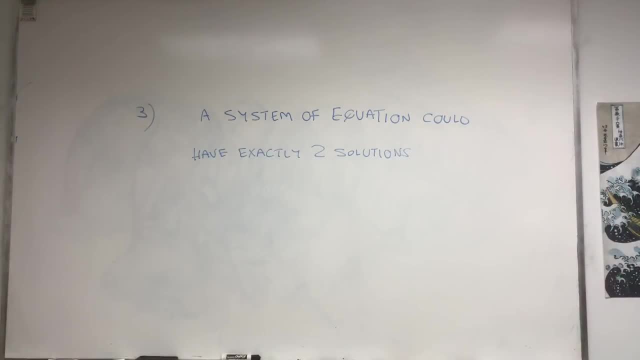 solution. Question is: could it have infinitely many solutions? Well, it could have infinitely many solutions. It could have infinitely many solutions, And I'll be back in a second because I need a better marker. And, by the way, third most popular language in the world: English, and America and UK. 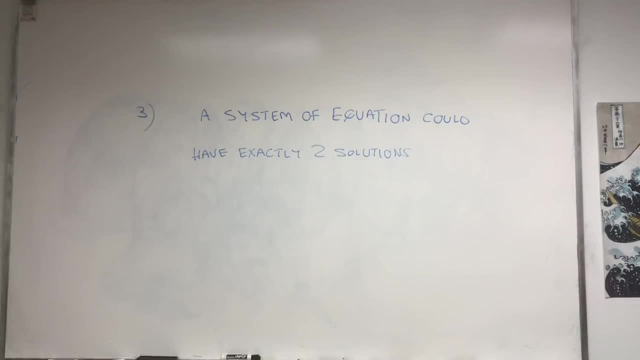 and other countries. And, by the way, three in English is three, you know, long-lived fixed points. Okay, and the answer is drum roll, it's five. Okay, All right, it's false. or, as in English, we say false because it turns out- remember this is. 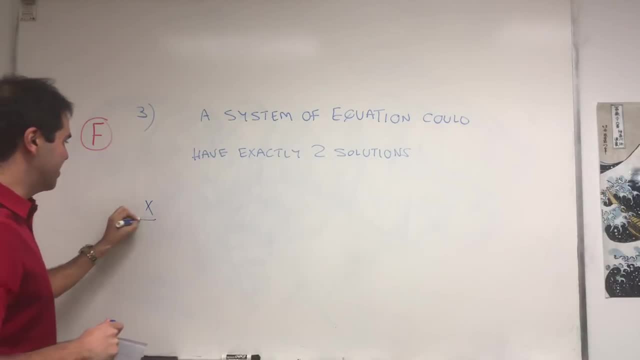 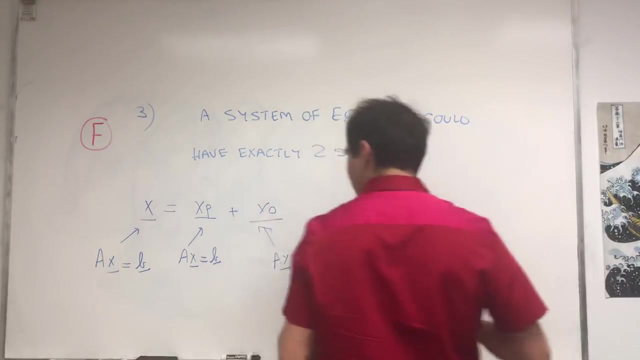 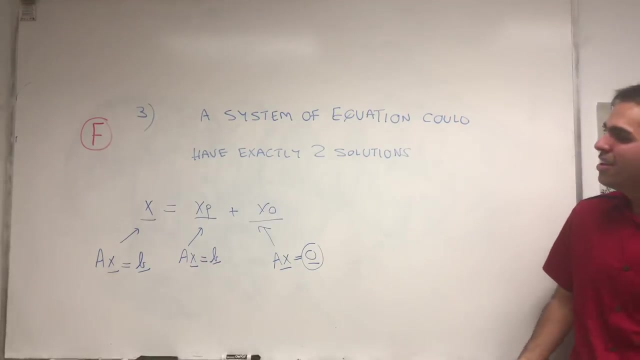 beautiful theorem that says: ah, if you have the general solution of ax equals to B, it's equal to a particular solution of ax equals B plus the general solution of the homogeneous equation ax equals zero. it's very similar and not a coincidence that for differential equations you have something similar: the. 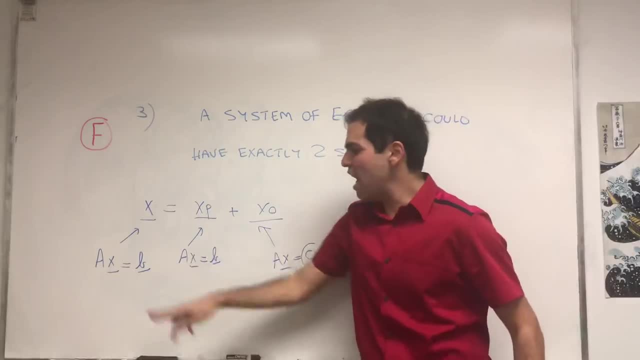 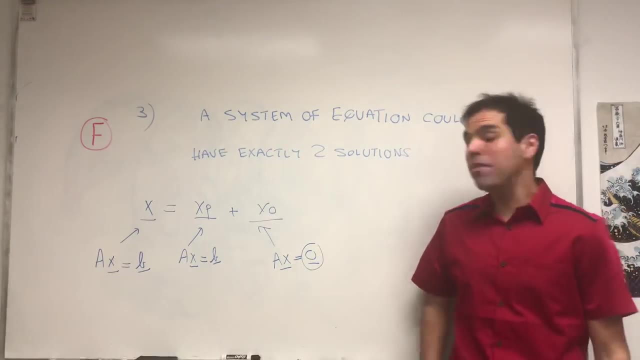 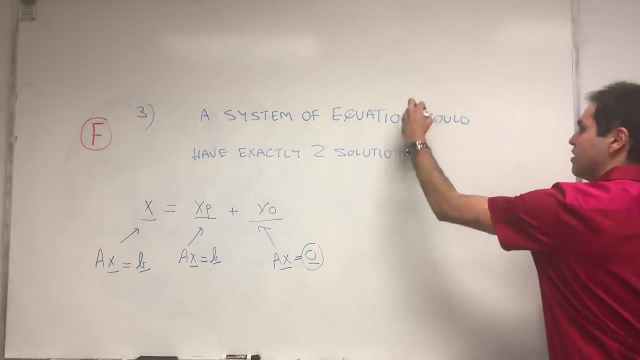 general solution of a differential equation with F on the right hand side equals to a particular solution of the equation which you get with variation of parameters, for example, and a general solution of the homogeneous equation. and I forgot that. eh, here, and so what does it tell us about solutions? suppose you want to solve ax. 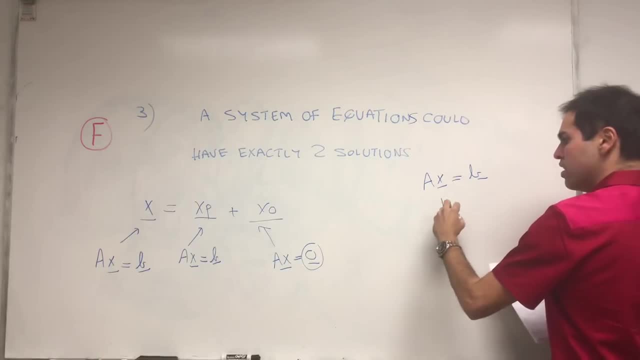 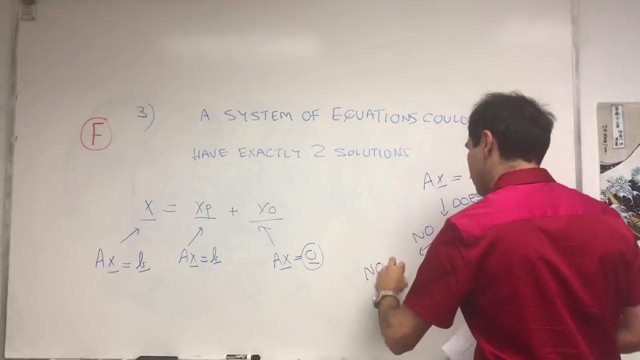 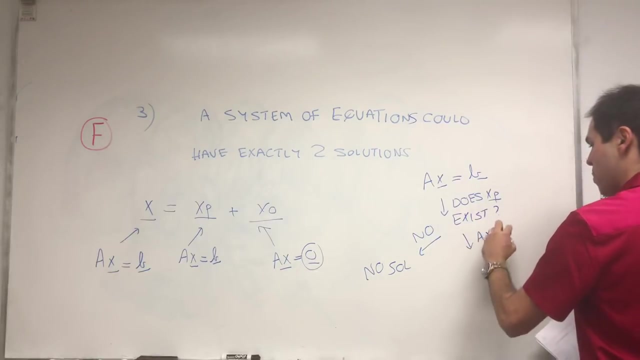 equals B. the question is first, does a particular solution exist? well, if no, then there is. there isn't even one particular solution, so we have no solution. and the other question is: then we have to talk about ax equals zero. okay, if a solution here وأ presenter. 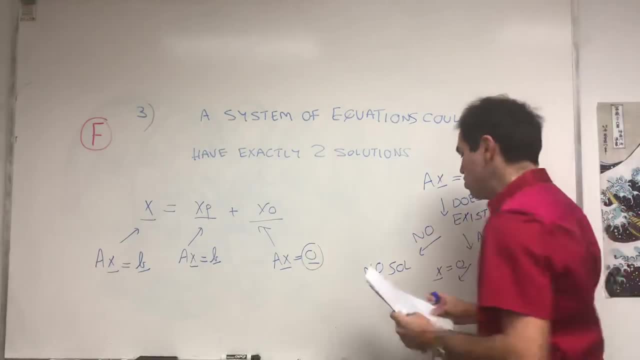 and and, and you know, ax equals one solution. sorry, ax is the solution where ax is equal to derivative of x. how's that? and he's ava il Im a here, you'll see Après it has. actually there's a distinction, maybe even between a and b, but actually in our thinking A x equals B plus X P, which is xp one time. so in that case it just means the equation: x equals b plus zero, which is X P. windows, x p, long time, many're the thing, uh…. in that case it just means the equation has only one solution, and in that case it just means the equation has only: and in that case, 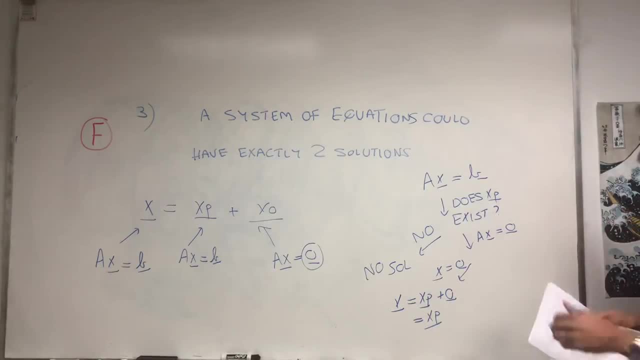 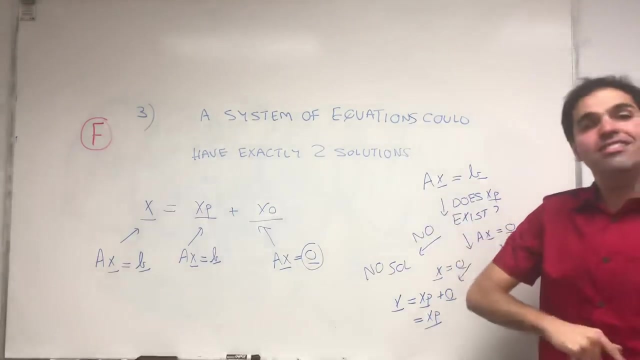 the equation has only one solution. just that particular solution, Or Ax equals 0, has a non-zero solution. And here's the thing you have to understand about Ax equals 0. If Ax equals 0, then A of 2x is also 0. And A of 3x is also 0. And actually you get at least a whole line of. 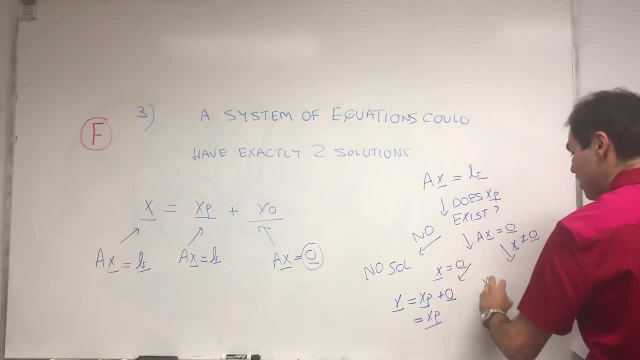 solutions, in which case there are infinitely many solutions. X equals to the particular solution, plus infinitely many of those homogeneous solutions. So in that case we get infinitely many solutions. In that case we get one solution. So what does that tell us? A linear equation. 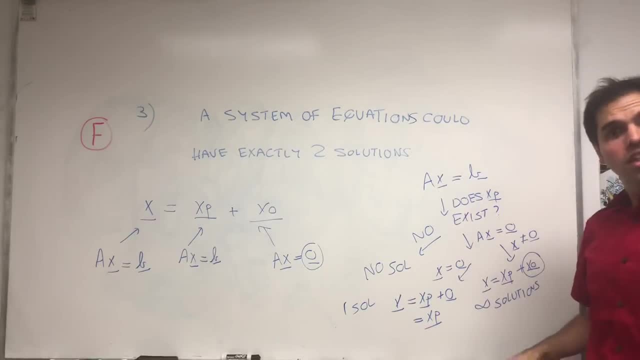 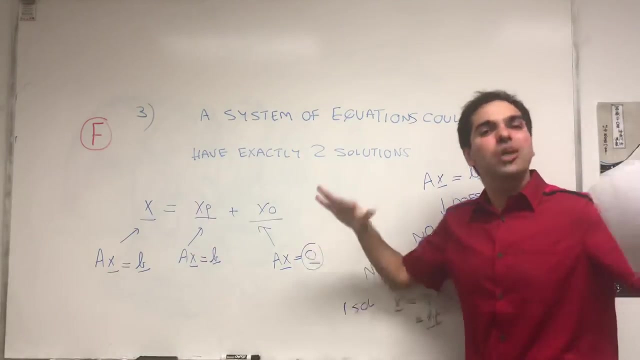 either it has no solutions, one solution or infinitely many solutions. It could never happen that you have exactly two solutions. Because of this, Ax equals 0,, which is sort of the kernel. it's literally the kernel of A. it's where all the solutions lie. 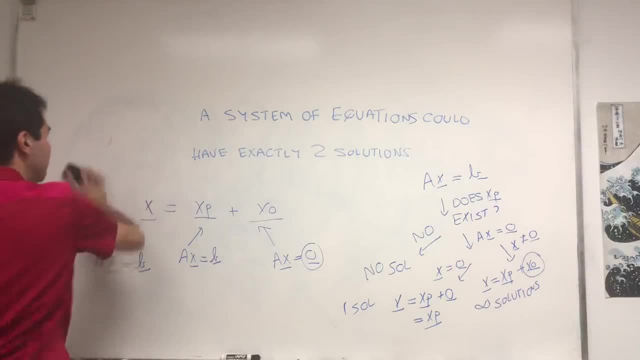 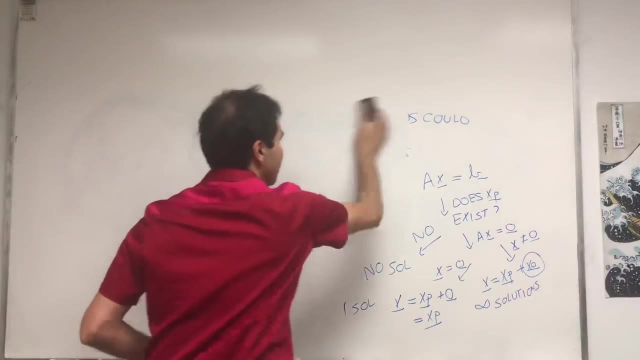 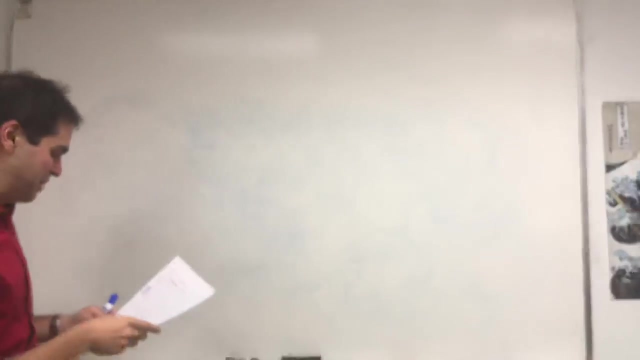 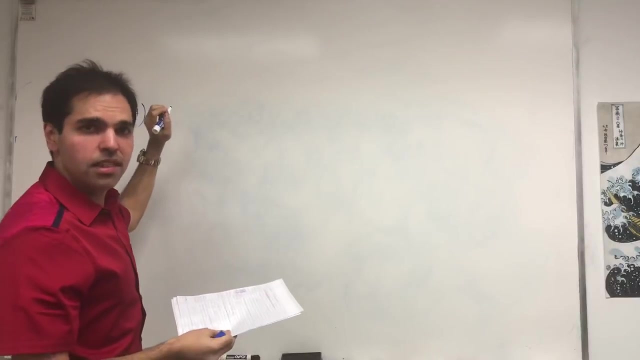 Okay, wonderful. So that's one thing that always confused me. But it is indeed true that at least linear equations can never have two solutions. All right, question four. Now let's talk pivot to me, okay. So if, when you want to solve, Ax equals b, if there's a pivot, 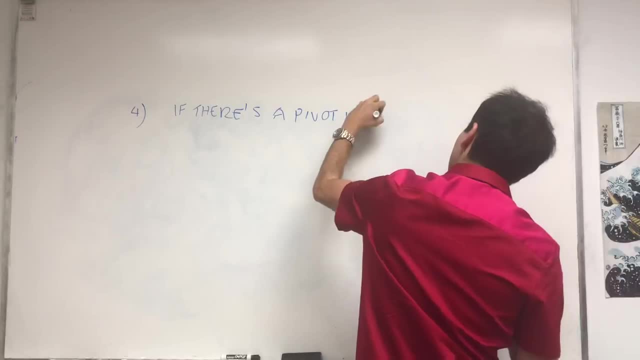 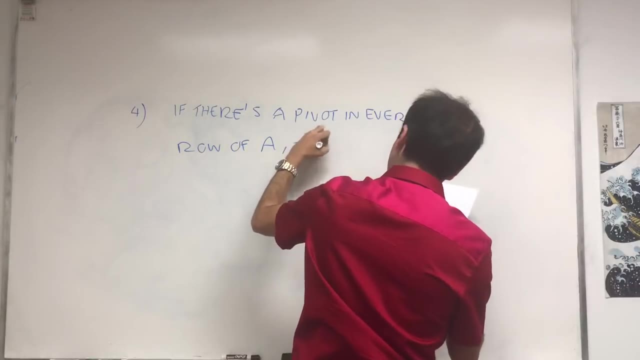 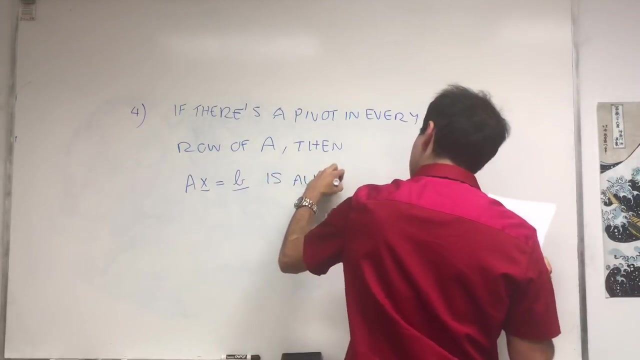 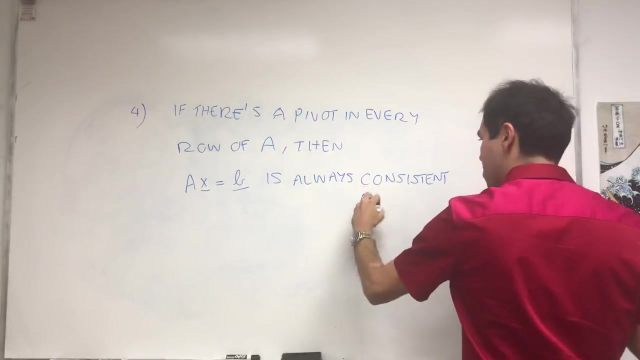 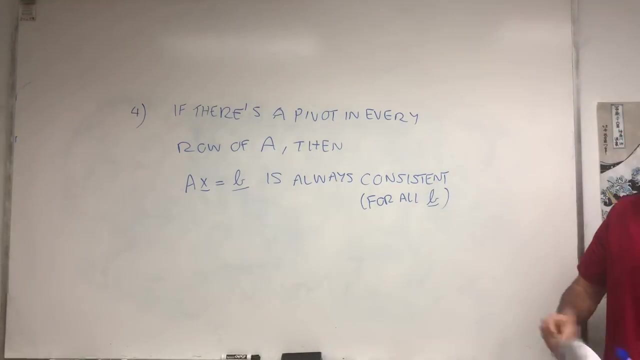 a pivot in every row of A of A, then Ax equals b, is always consistent, Again, for all b, Which is a pretty strong statement. So if, no matter what b is, if you find a pivot in every row of A, then the system is always consistent, Which I find hard. 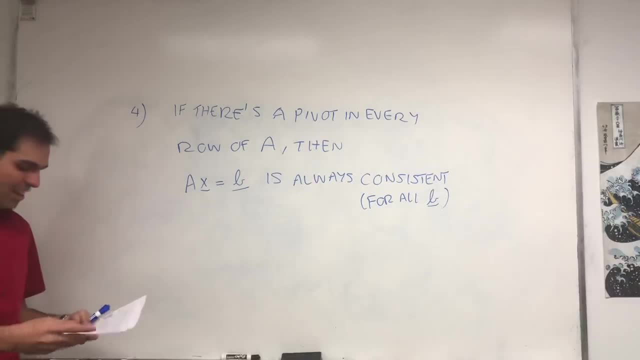 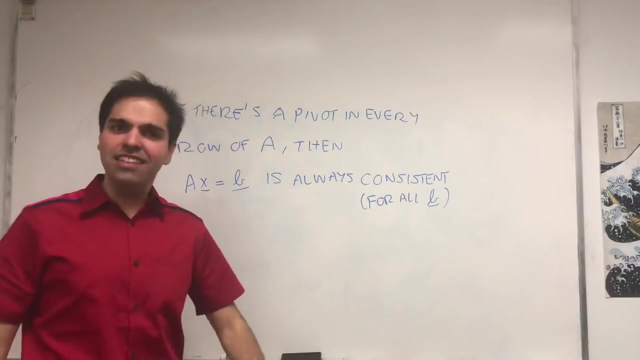 Hard to believe, But let's see. And while we're at it, the fourth most popular language in the world, believe it or not, is Bengali. Who would have known, By the way, Bengali as in in Life of Pi? 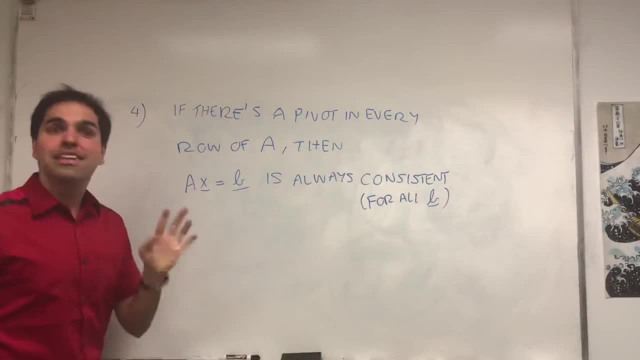 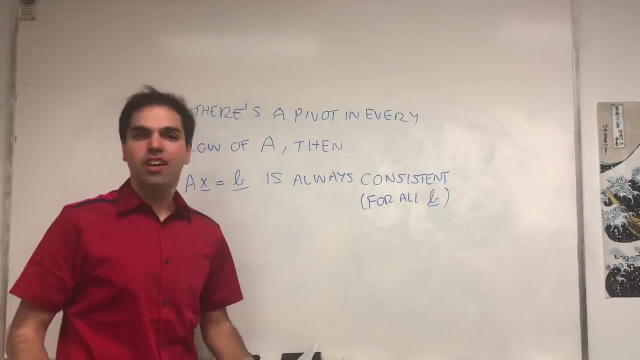 And four: in Bengali is thar, almost like thar, like a tiger, Or also I like to think of it as thor. So it's thor, but with an A, Which is, by the way, interesting. I know it has nothing to do with math. 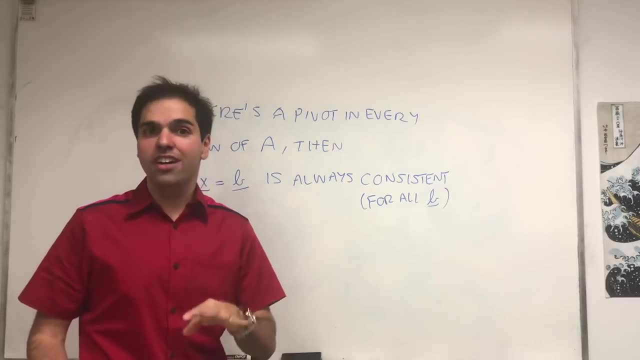 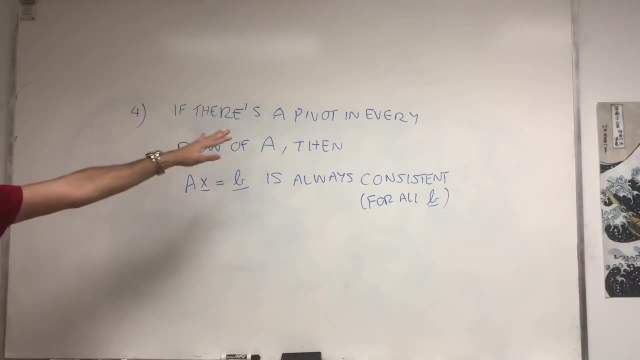 but in Farsi four is chahar. in Bengali, thar Sounds very similar. Okay, Now question: if there's a pivot in every overbite of row of A, is the system always consistent? Surprisingly, it's true. 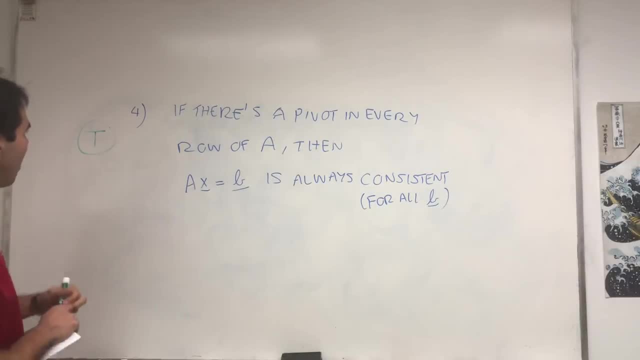 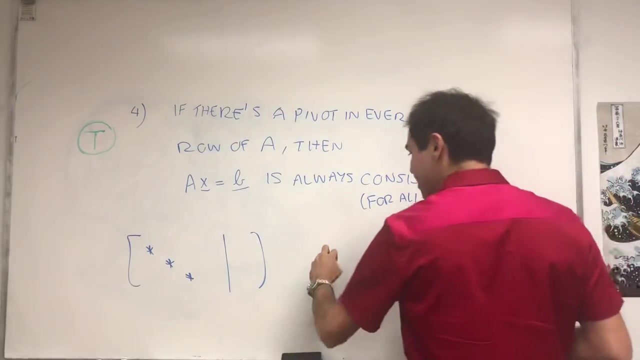 And this is really why this sucks, and this is why pivots are so important, Because, look, suppose there's a pivot in every row of A like this, and suppose this is B. There's this really nice fact about systems, namely the only way a system can be inconsistent. 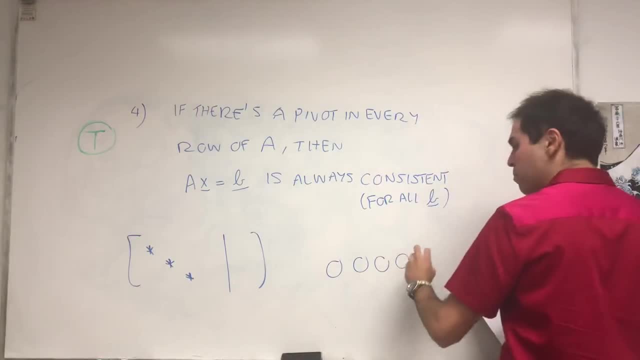 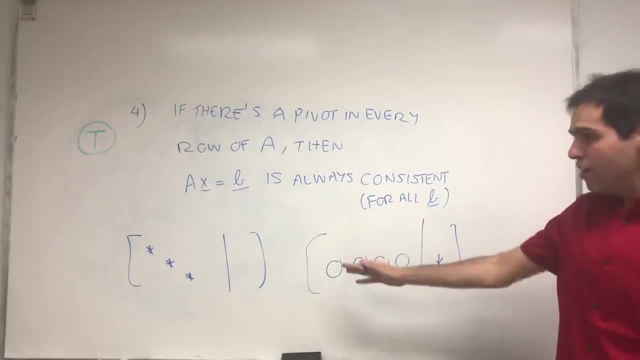 has no solutions if there's a row of the form bunch of zeros in A and something non-zero. But look, if there's a pivot in every row, there's no way that you can get bunch of zeros and then something non-zero, because pivots are non-zero. 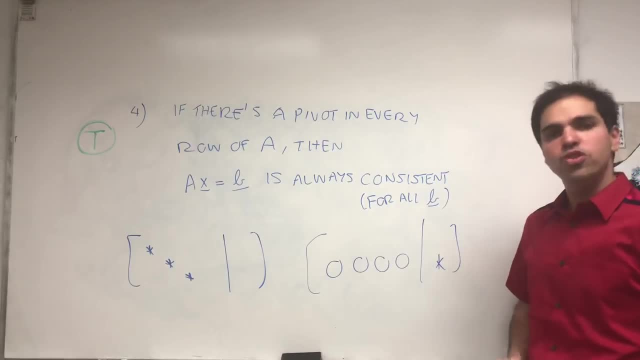 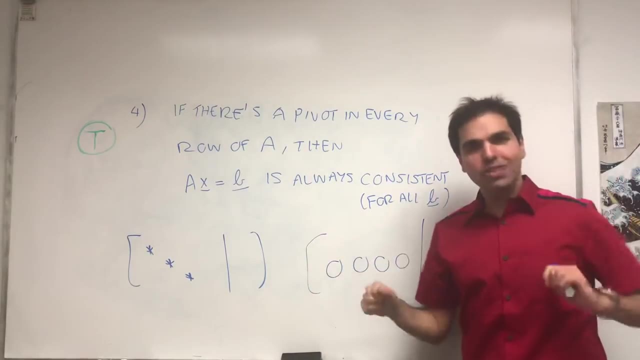 And that's why it is true that, no matter which B you choose, you always get that it's consistent. And this is why, coming back to questions one and two, the number of equations don't really matter, The number of variables doesn't really matter. 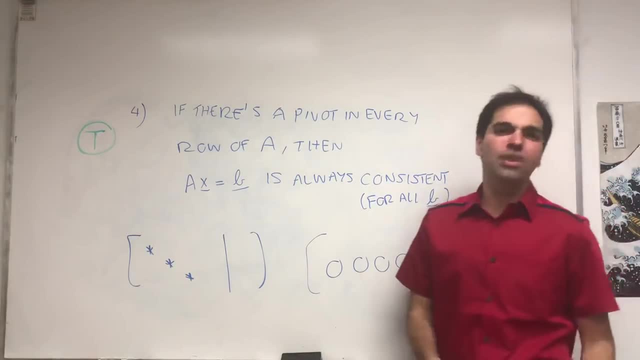 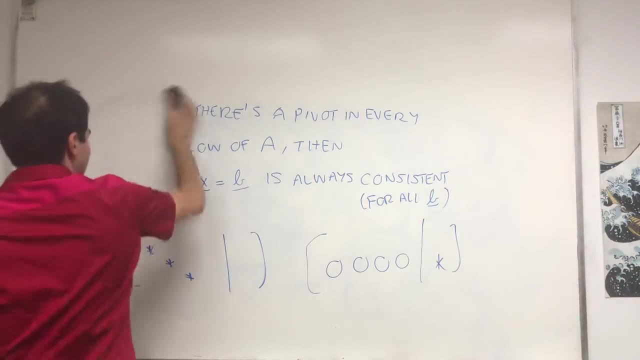 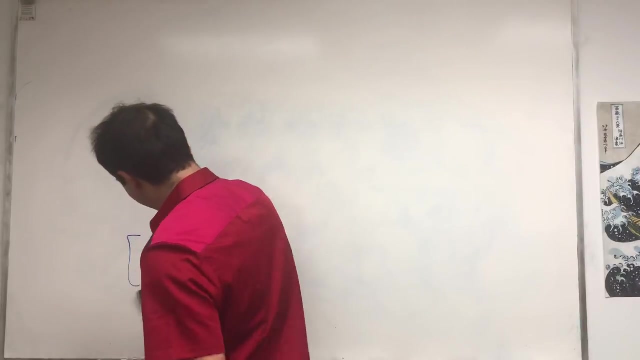 What does matter is the number of pivots. Those are the ones that tell us if we have solutions or not. Okay, next question, so question five. I don't know, black pen, red pen? I think you might be right, It might take more than two hours. 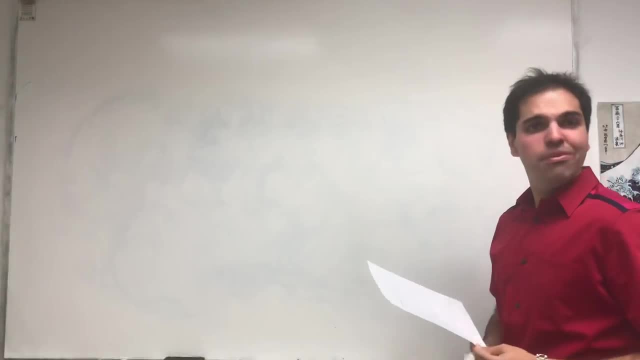 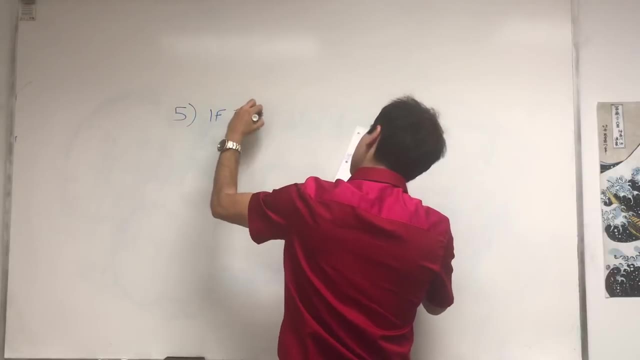 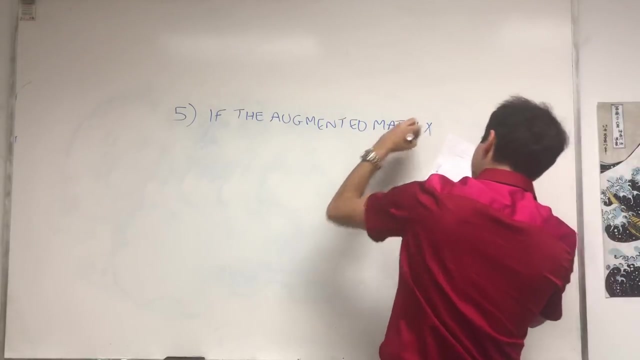 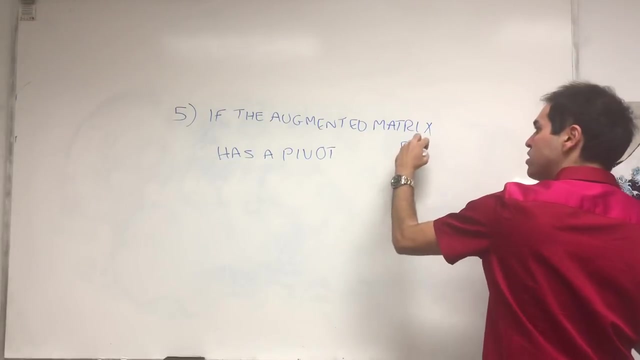 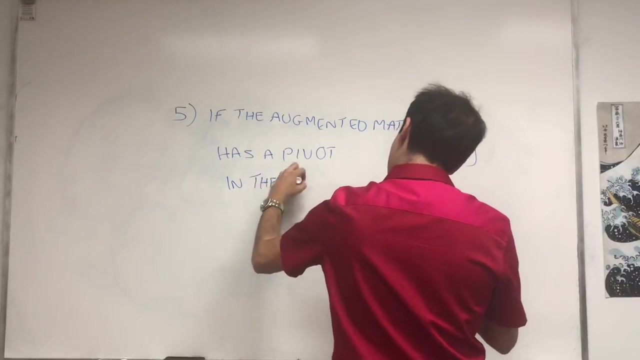 Okay, next question, so again with having to do with pivots. So if the augmented matrix matrix has a pivot- and again augmented matrix really means the matrix of A and B, so has a pivot in the last column, then AX equals to B is inconsistent. 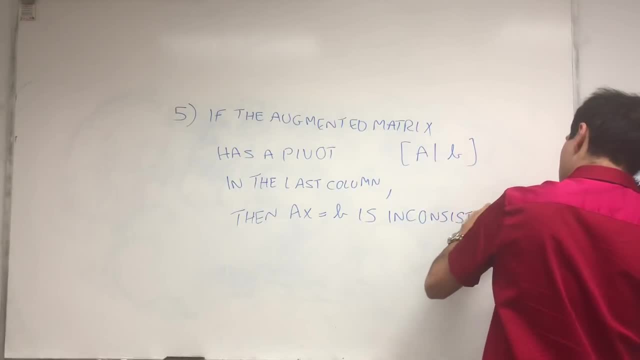 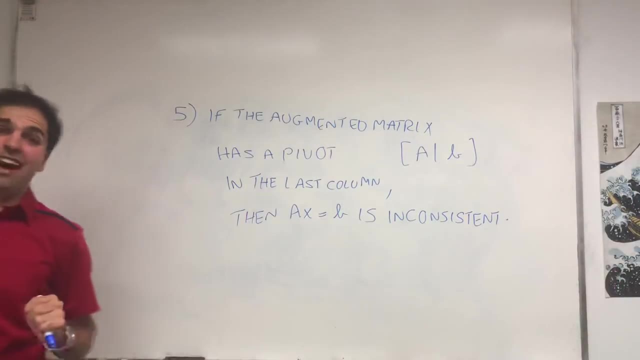 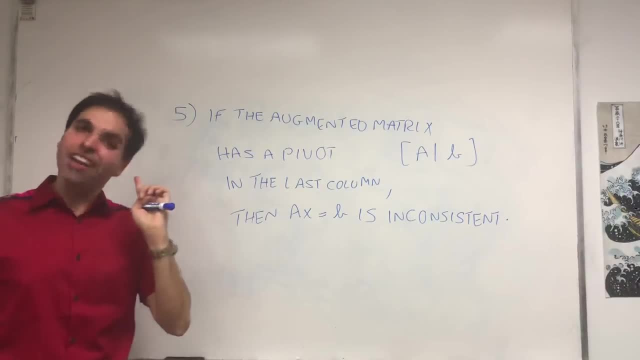 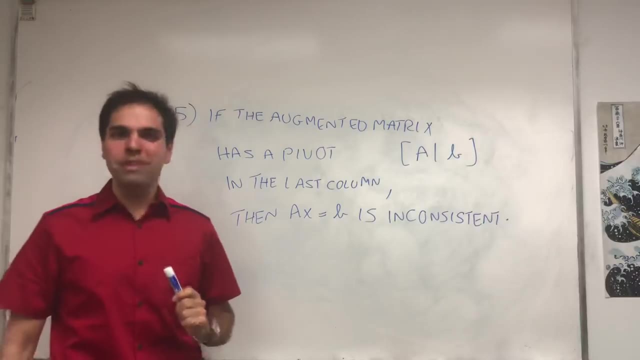 and five in Hindi is, which is also very interesting because in Farsi it's That's what Farsi they sometimes call it Indo-European language, But because it's a similarity between you know, I guess Hindi and also it actually has the same structure as European language. 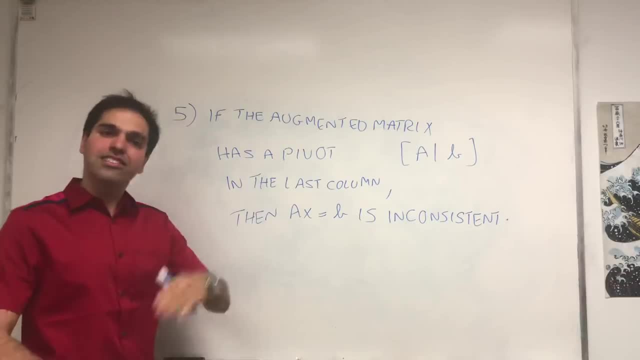 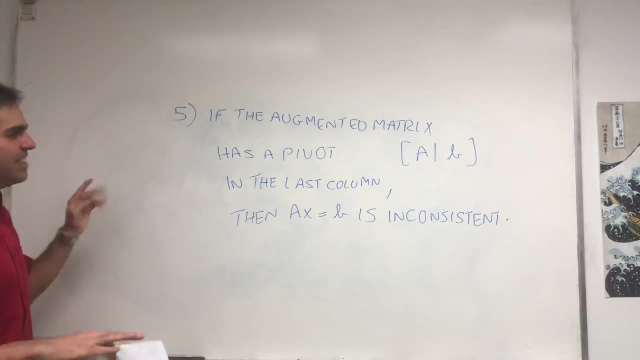 For example, the verb comes last, and then there's a subject and an object, et cetera, et cetera. So this is cool And let's see, is it true or is it false? It turns out it's true by the same argument as before. 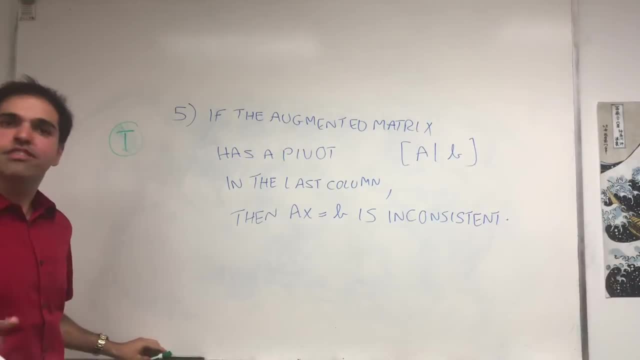 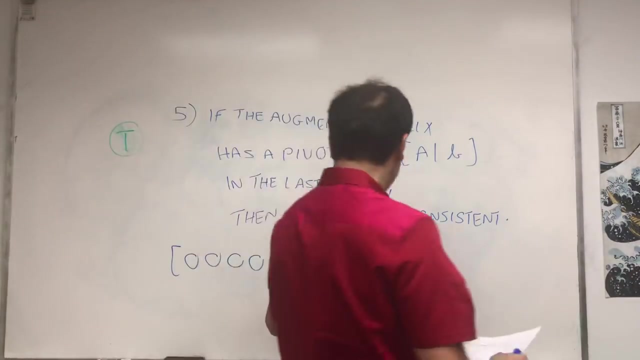 Remember the quintessential way for testing if something has a solution or not, it's simply look. if there's a row of the form 0, 0, 0, something, Okay, well, in that case, is there a row of form 0, 0, 0, something? 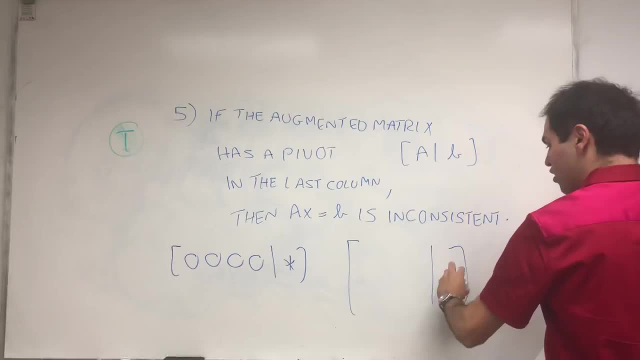 Well, yes, because look, there's a pivot in the last column. let's say here, and one important thing you need to know about pivots: everything to the left of the pivot is 0, just by this triangular structure of the row, echelon form. 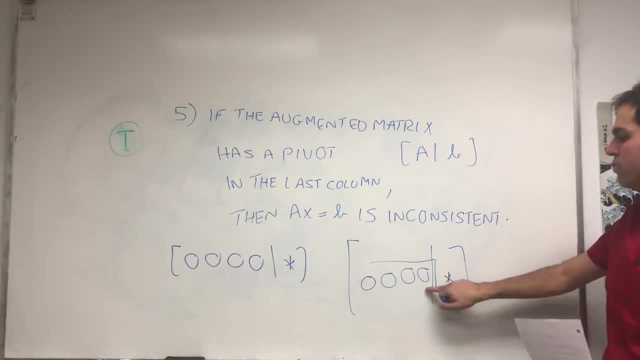 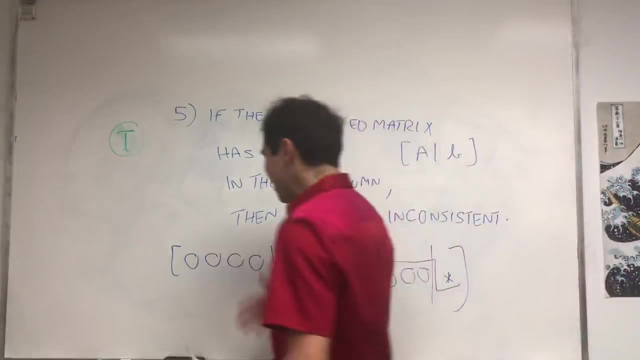 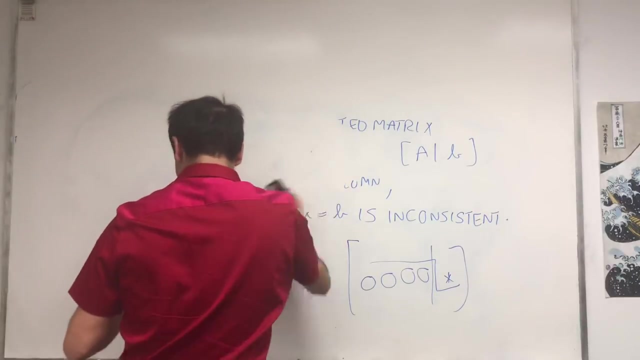 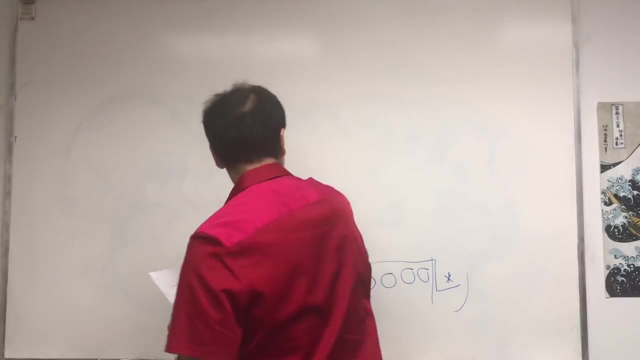 And that's why we do have a row of the form 0,, 0,, 0, something, And that's why the equation is inconsistent and bam, that's it. So this is why this test is so useful. Okay, And our next question has to do with something similar. 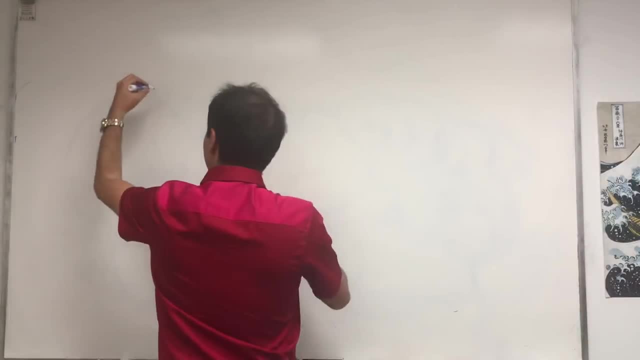 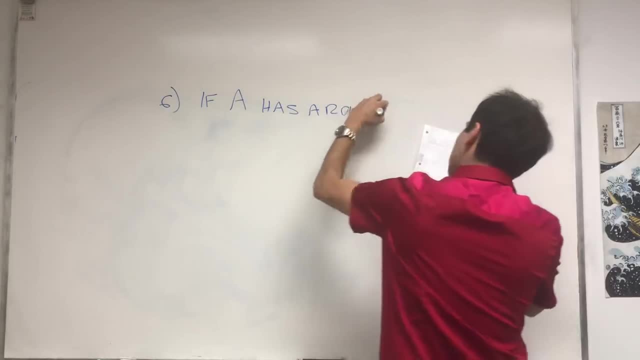 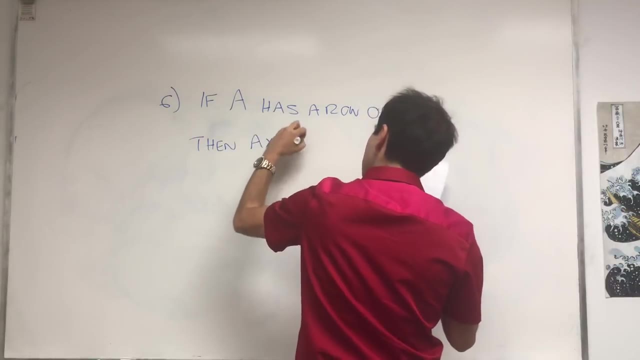 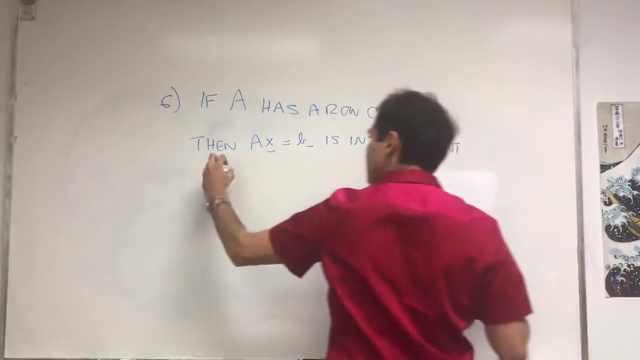 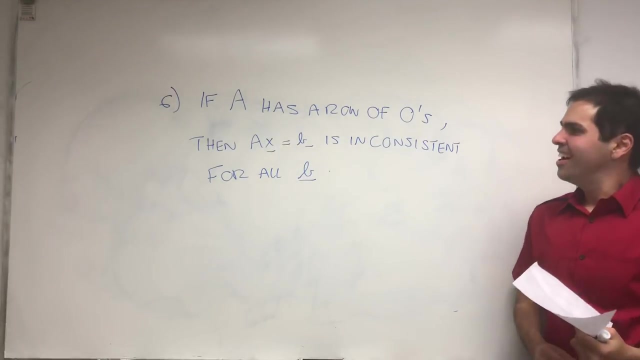 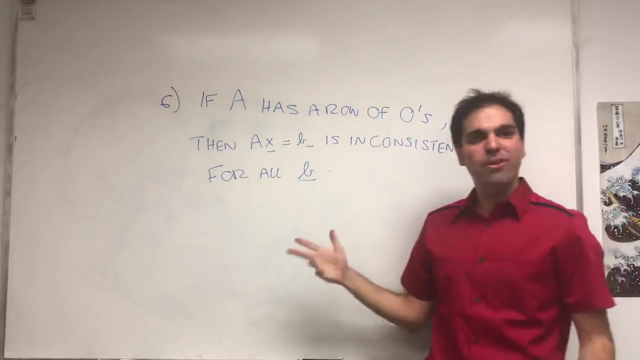 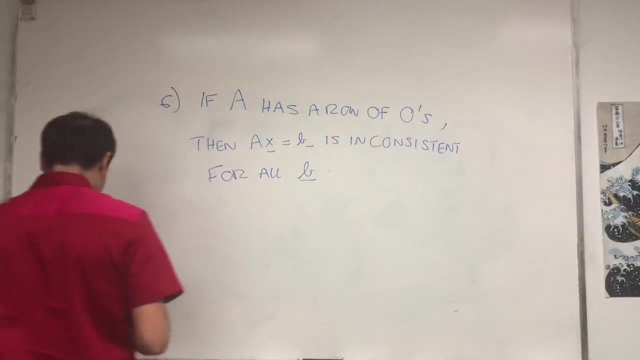 Then AX equals B is inconsistent for all B. And sixth most popular language in the world, Portuguese. And sixth in Portuguese is seis, Just like in Spanish, seis. Think about this. And it's false, Because let me give you an example of such a system, a very trivial one. 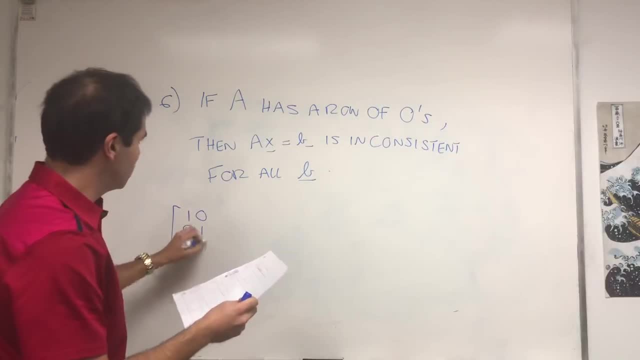 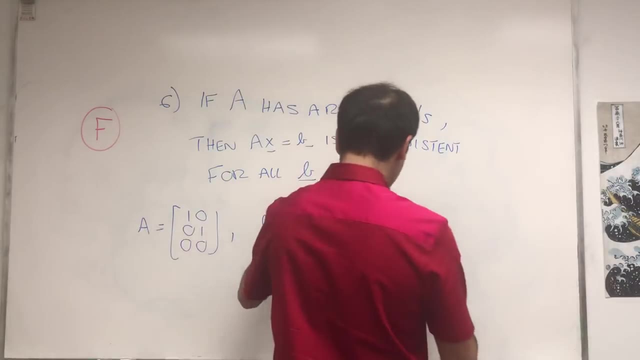 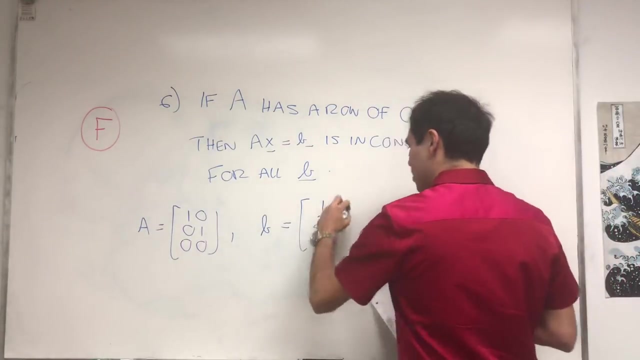 A is 1, 0, 0, 1, 0, 0.. 0.. So it has a row of 0s, And then B, it's simply 1, 2.. So X is 1,, Y is 2, and then just 0.. 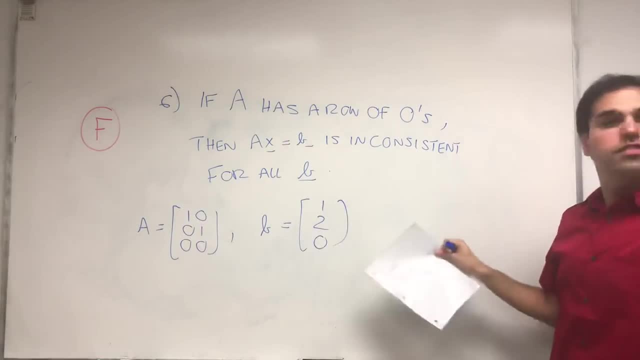 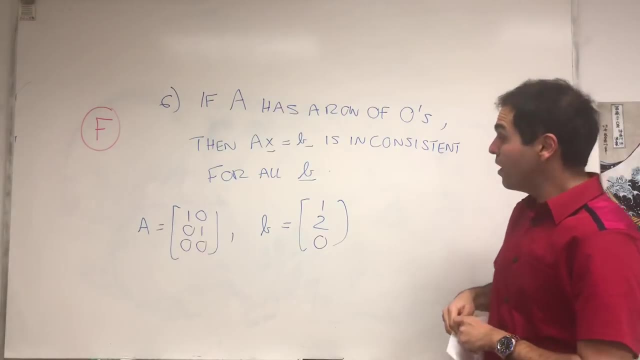 So the system becomes: X is 1,, Y is 2, and 0 is 0,, which is consistent. I think it's similar to a question from before, But again, what made this work or not work? So what can we say? 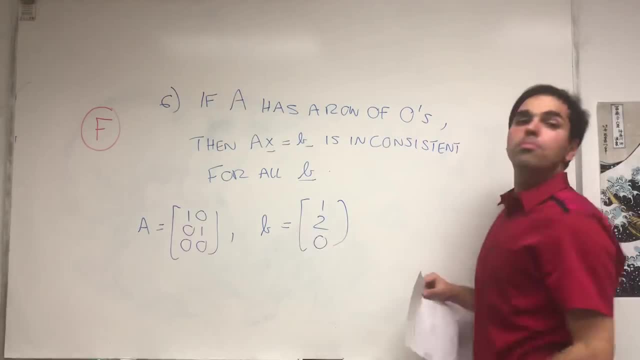 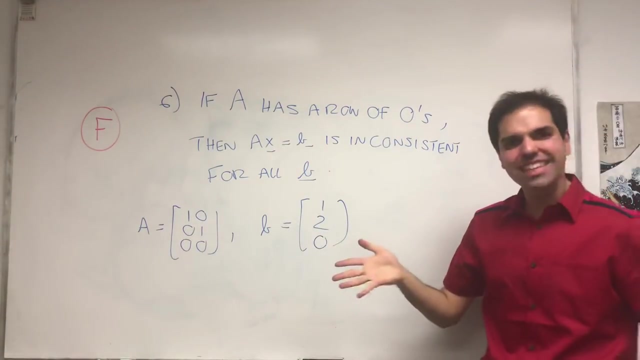 OK, The only thing we can say is there is some B for which this system is inconsistent, Namely just to choose B such that the last entry is non-zero. So again, in terms of pivots, we can't say it's always inconsistent. 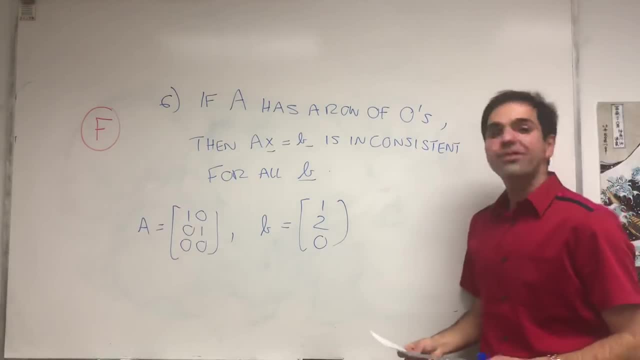 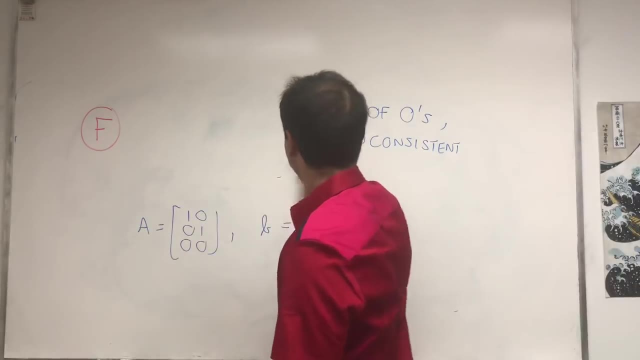 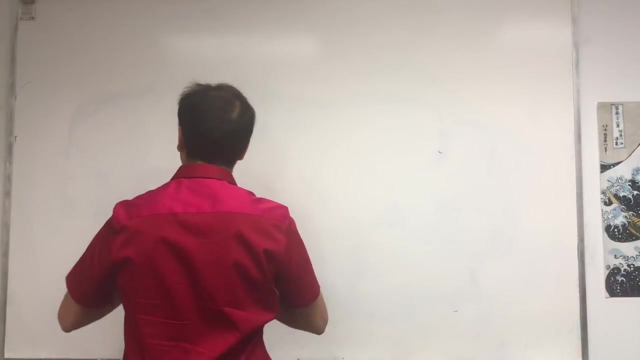 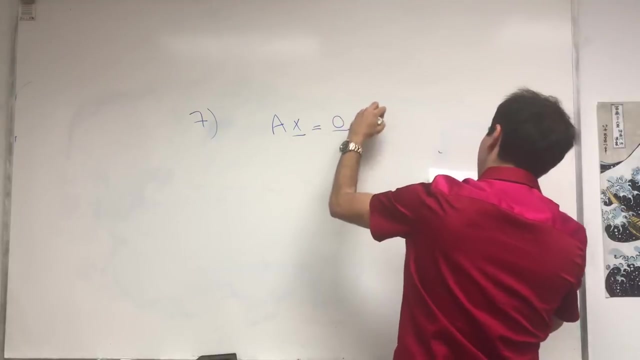 We can just say it's sometimes inconsistent, So you just have to be careful about that. OK, And question seven: Quickie. OK, Ta-da-dum. So we talked about inconsistent systems. What about this system? Ax equals 0 is always consistent. 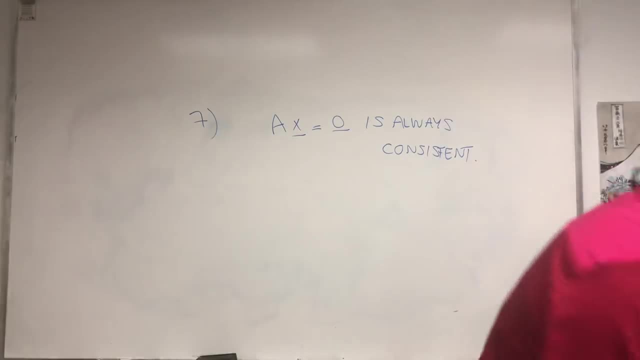 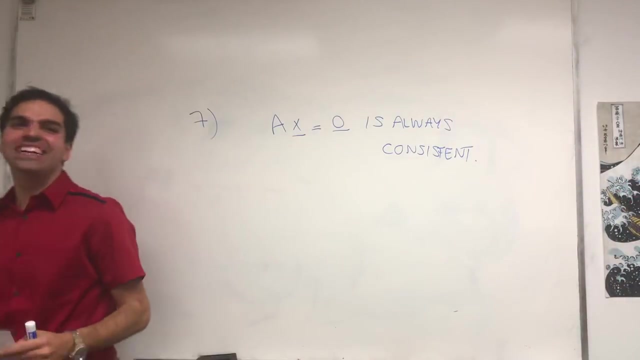 In other words, the homogeneous equation always has a solution. Let me take a sip of my water, Ta-da-dum. And the seventh most popular language, Russian. And 7 in Russian is cm. Really cool, Almost like psi m. 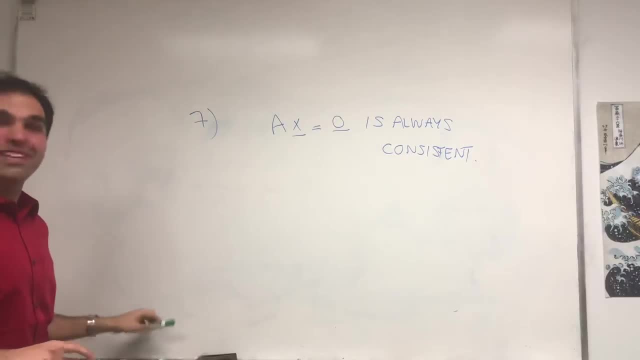 And let's see, I don't know why I put the red one, Because it's actually true, Because there's a very easy solution to this: X equals 0.. X equals 0 is consistent. X equals 0 is consistent. 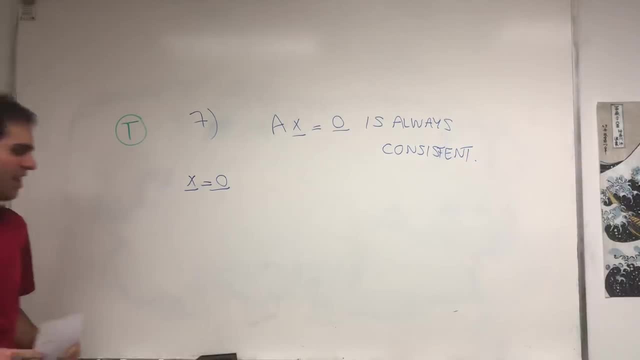 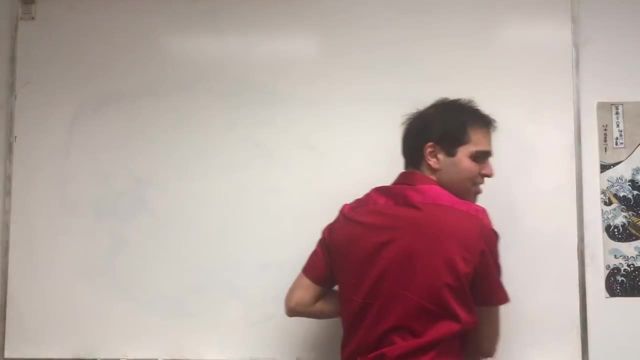 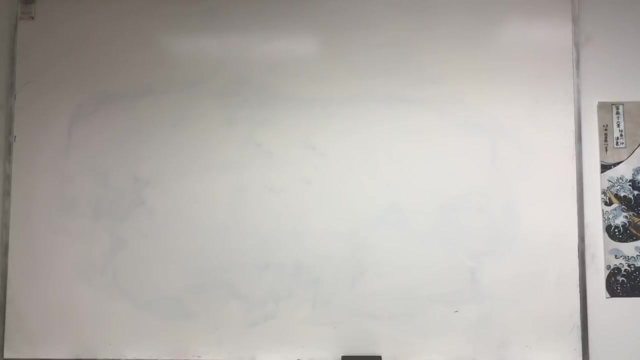 X equals 0 is always a solution of the homogeneous equation. And there you go, OK, So now we talked about equations, And now let's talk more about linear independence and linear dependence. I'm sorry for walking around all the time, But I know I'll be here for a couple of hours. 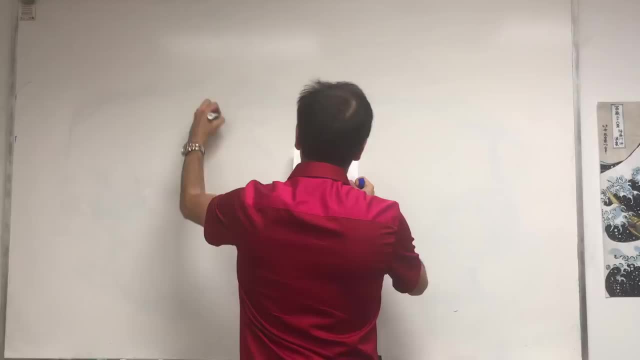 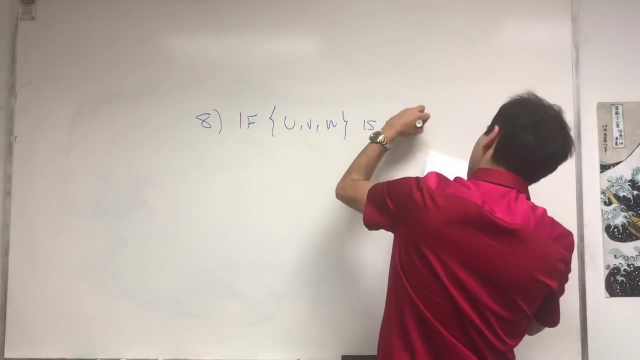 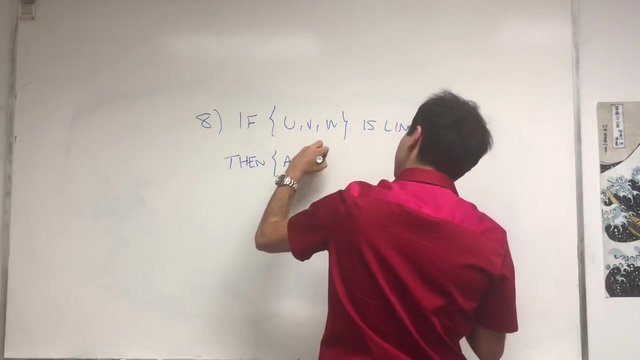 So I can do this Question eight: If uv double is equal to 0.. If uv double is equal to 0.. If uv double is equal to 0.. If uv is linearly dependent, then for any matrix, aau, av, aw is linearly dependent. 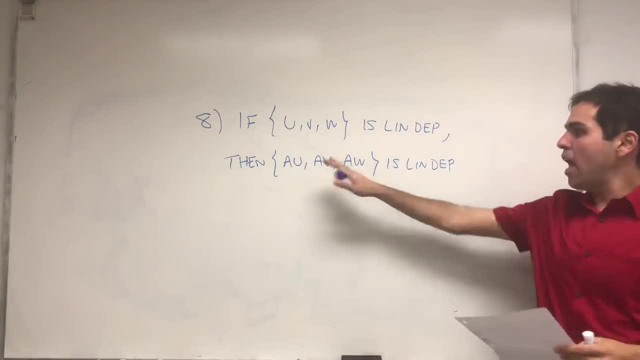 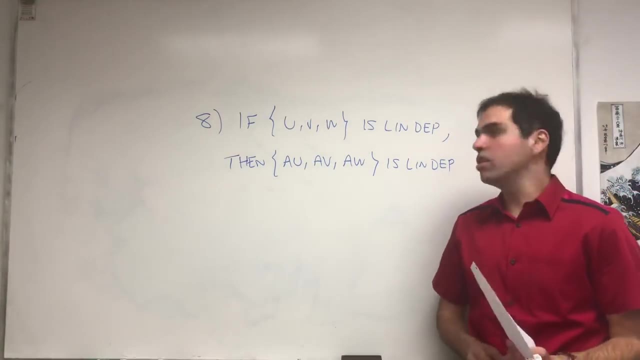 Which is surprising. So, by the way, I'm not giving any assumptions on a. I don't say the columns are linearly independent. I'm not claiming anything is one to one, Just in general. Just in general, If the input is linearly dependent, then the output is also linearly dependent. 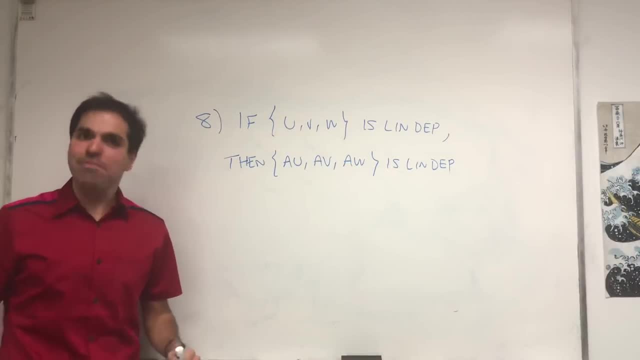 And eighth most popular language in the world, Japanese, And eighth in Japanese. this is so cool. is hajji Literally hajji Yep? It's cool And, as I said, this is quite surprising. It turns out this is true. 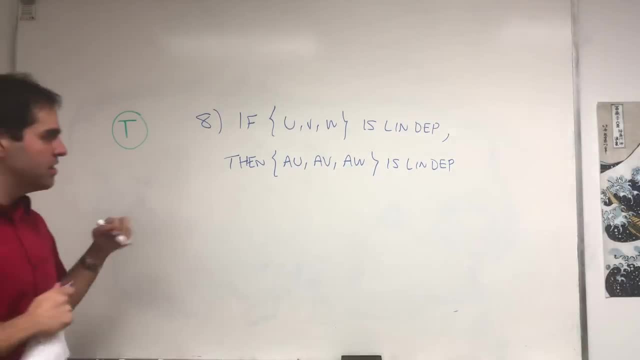 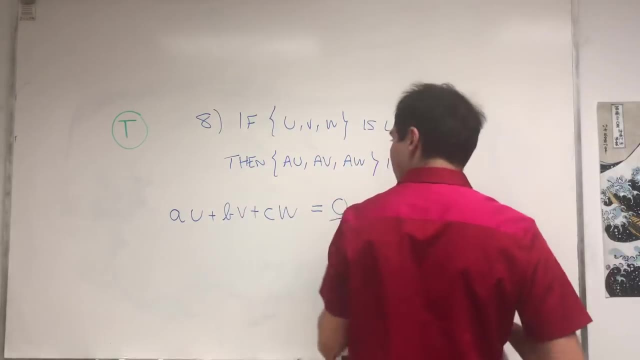 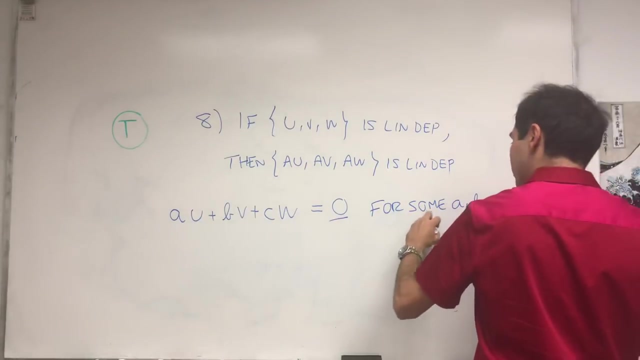 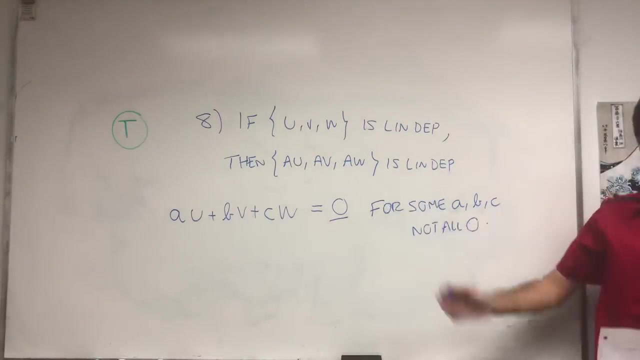 And let me quickly show it to you. What does linear dependence mean? It means that Au plus Bv plus Cw equals to the zero vector for some Abc, not all zero, Because if Ab and C are zero, this is trivially satisfied. 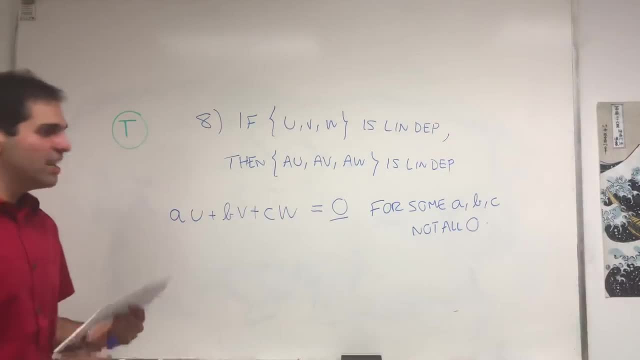 And I like the French way, Like, And that's not the same as: So all not zero means like all three are not zero, But not all zero means one of them at least is not zero. OK, So we have this equation. 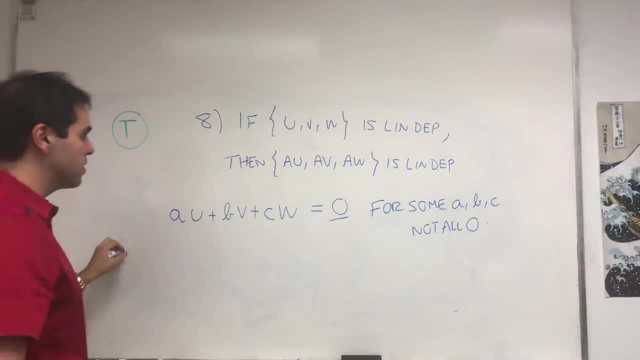 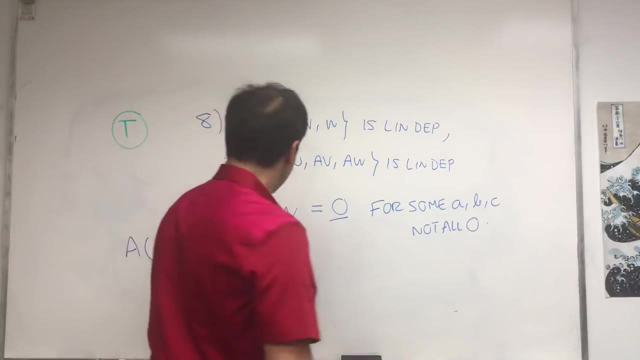 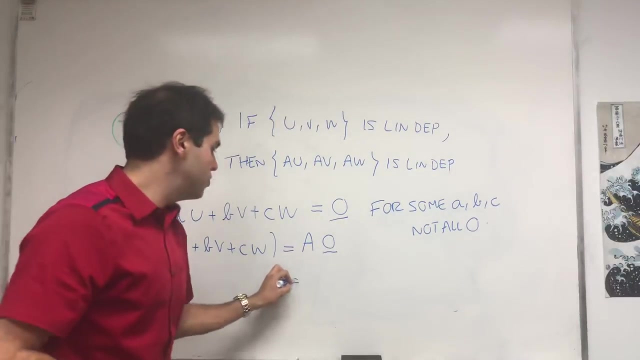 Let's just apply A to it Because we want: Au plus Av plus Aw is zero. So Aau plus Bv plus Cw equals A0. And A applied to zero is just zero. Has to do with the previous question where x equals zero always satisfies Ax equals zero. 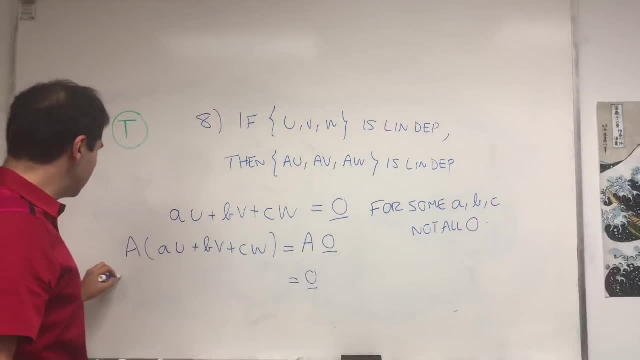 And here we can just use FOIL it out like distributivity. So Aau plus Bav plus Caw equals zero. And notice, it's precisely what we wanted. We wanted some constants, Not all zero, which they are by assumption. 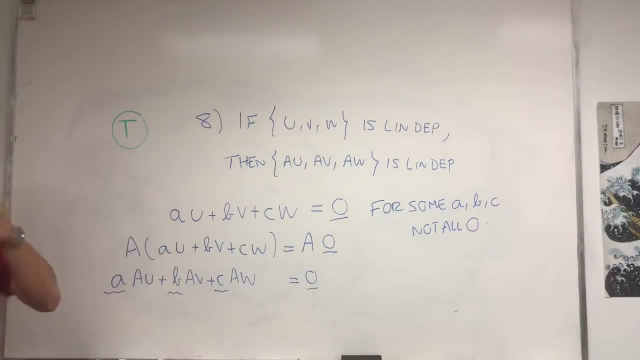 Such that Au plus Av plus Aw satisfies some linear combination in zero. So those ones don't necessarily have to be the same as the first ones, But it turns out here. they are just by luck, And that's why we're done. That's why Au plus Avu, Av and Aw, they're linearly dependent. 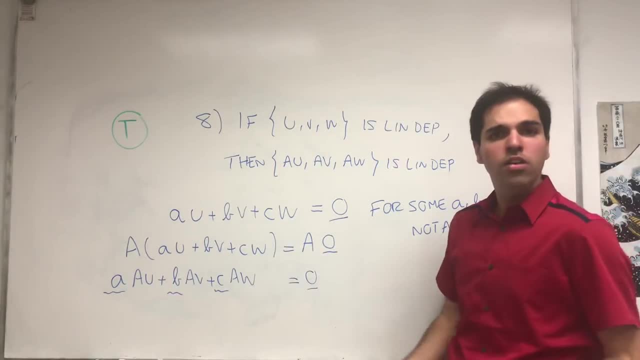 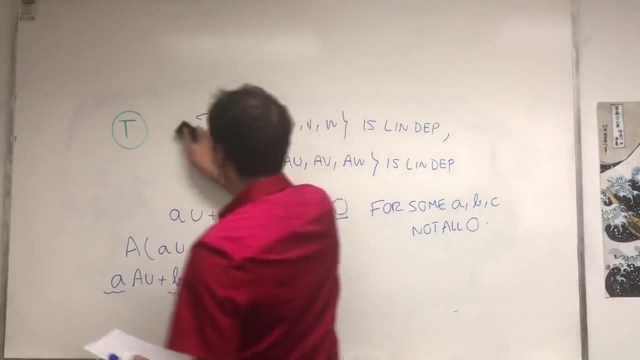 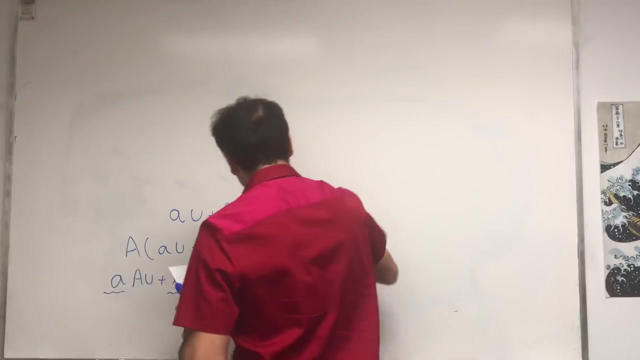 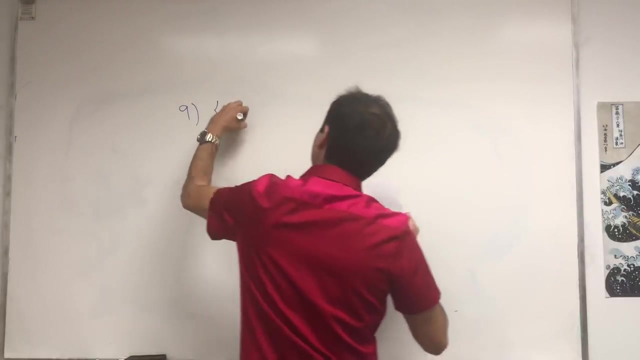 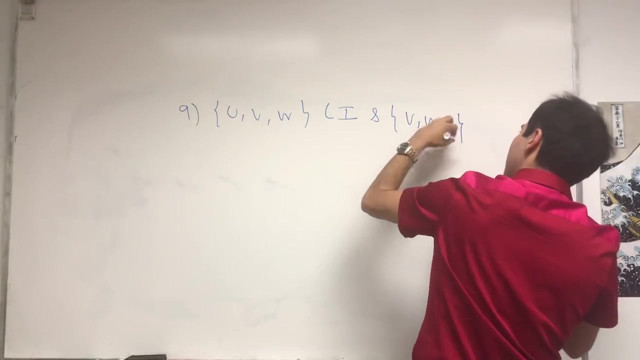 And again we have knows use any assumptions on one-to-one or linearly independent columns. That works for any matrix for which this makes sense. Good, That was question 8.. Now question 9.. uvw linearly independent and vwp. linearly independent implies that the whole set is. 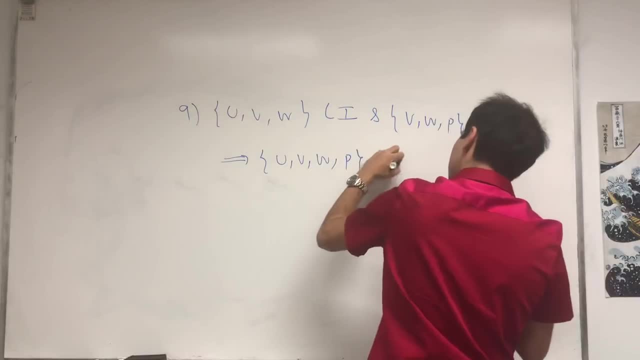 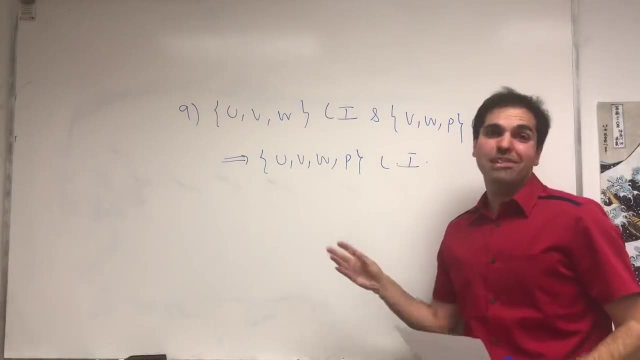 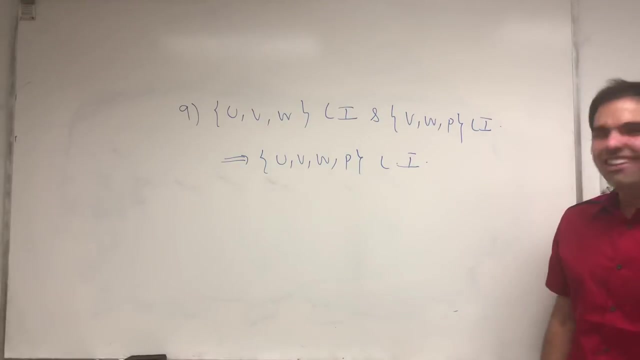 linearly independent. uvwp: linearly independent. I have to say I don't know why the question got myself into, because this is question nine and we still have a hundred and two questions to go. What did black pen and red pen do to me? Why do I always get into this peer pressure? 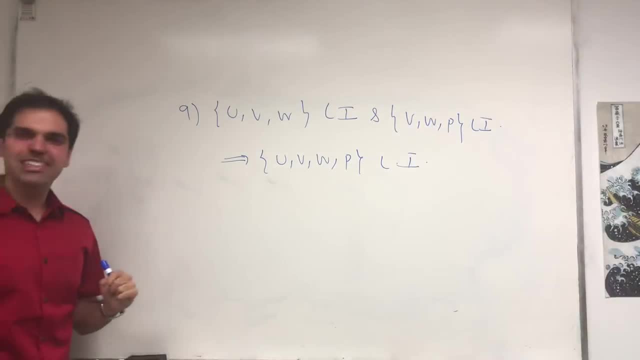 And also ninth most popular language in the world, German, and nine in German is nine. it's also interesting because nine in German means no, so it's confusing language. but so if you put sort of two linearly independent sets together, is the results still linearly independent? and the answer is false, because notice. 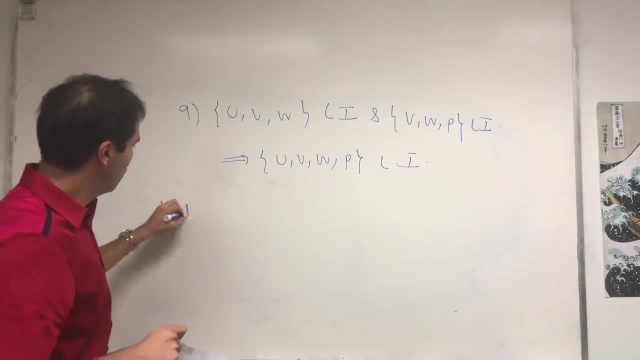 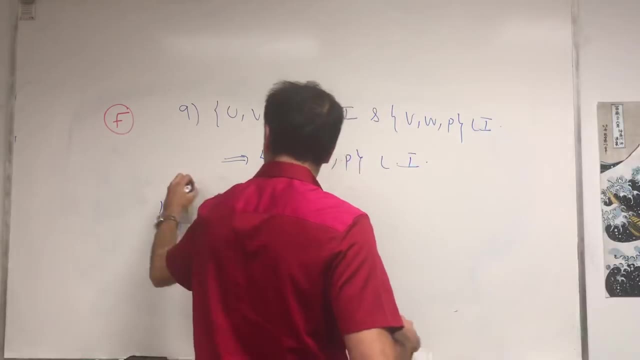 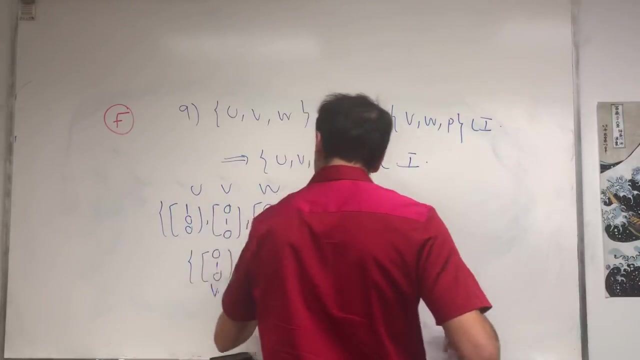 if you take, let's say one zero, zero, zero, one zero and zero zero one, u v, w, that is linearly independent and also so vwp: zero, one, zero and zero zero one. and let's just say two zero, zero, vwp, that's also linearly independent. but if you put them, both of them together, so one zero. 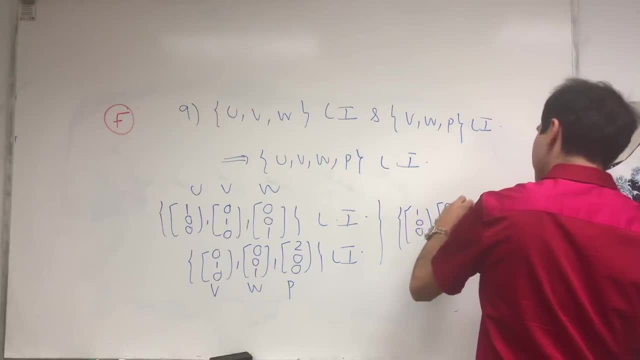 whoop: 0, 0, 0, 1, 0, 0, 0, 1, and 2, 0, 0.. Well, that's linearly dependent because this vector it's 2 times this vector. 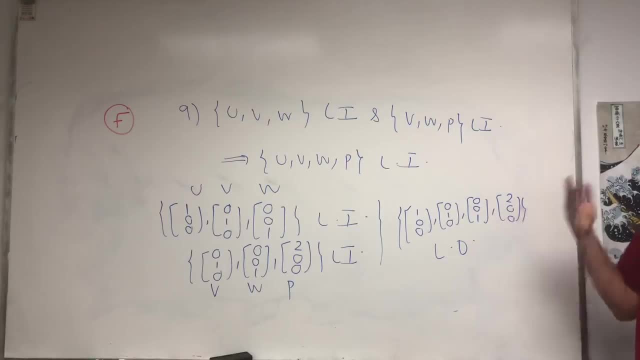 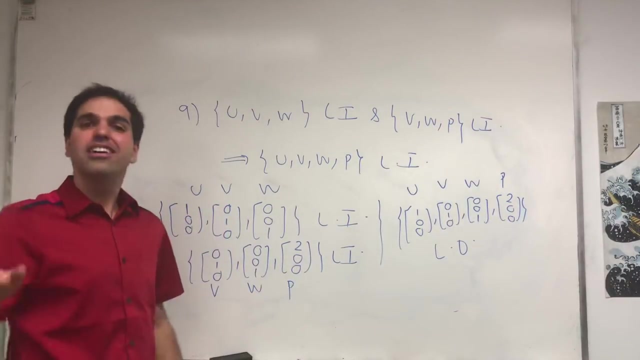 So there is a relation between the two And therefore this is false. You cannot just put two sets together hoping they're linearly independent. Sometimes it works, though. That's a cool thing, especially for some eigenvectors with different eigenvalues. 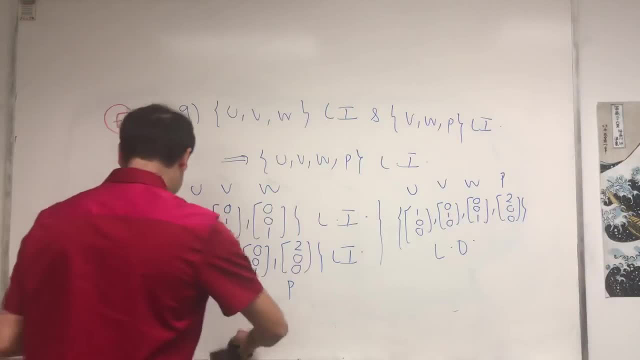 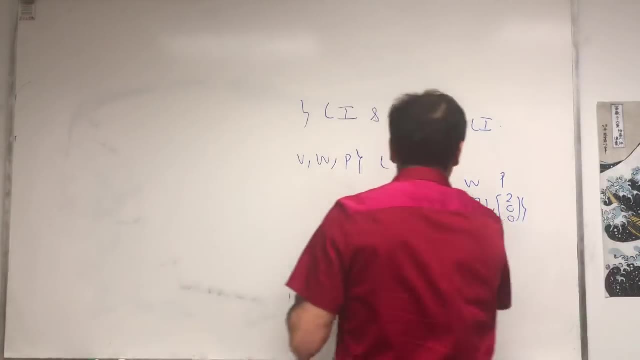 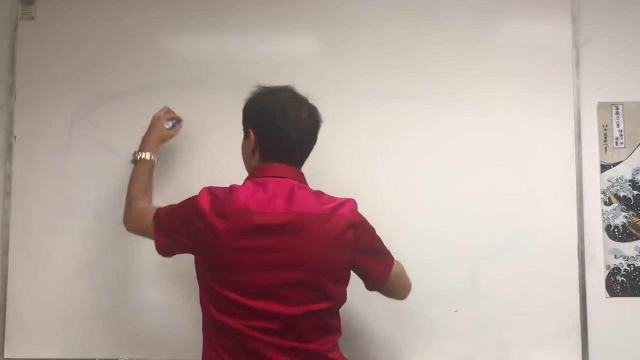 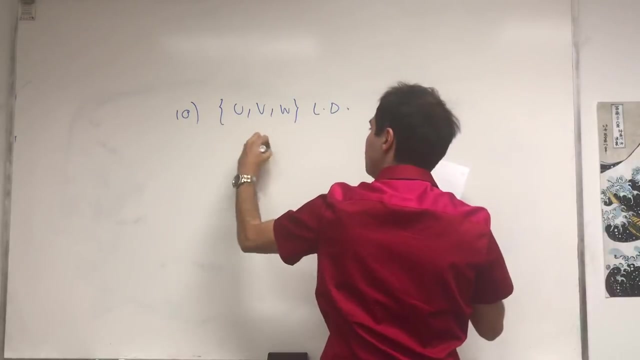 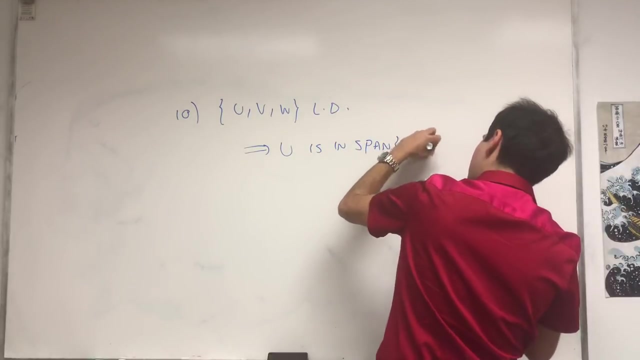 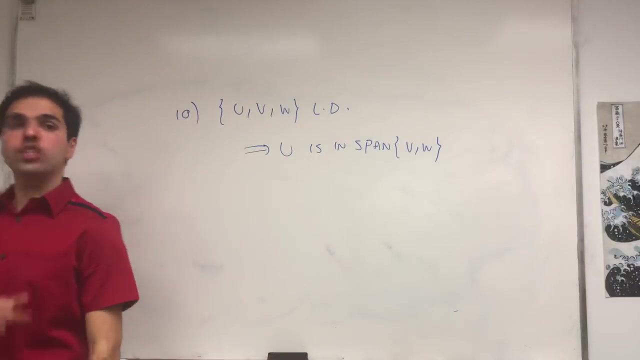 But we'll talk about that in three hours. Next question, Question 10.. uvw linearly dependent implies that u has to be in span of v-double. Now, 10th most popular language, or maybe I should correct this: It's not the most popular language. 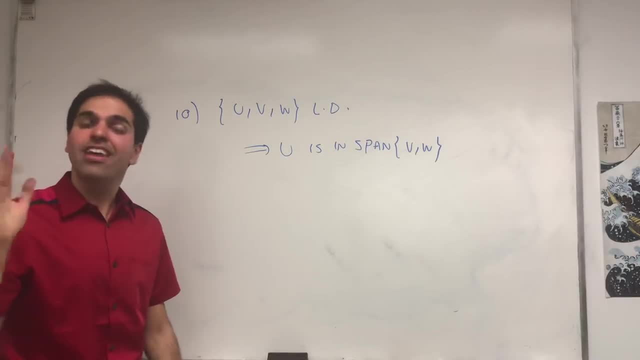 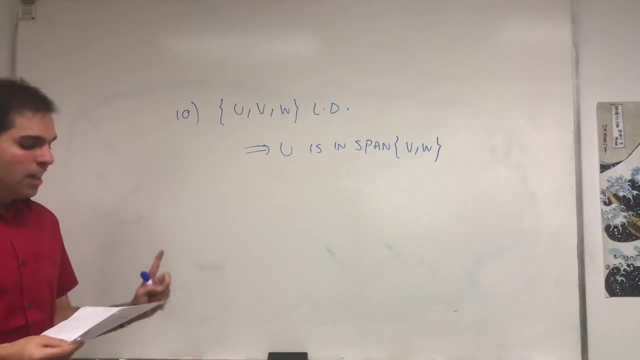 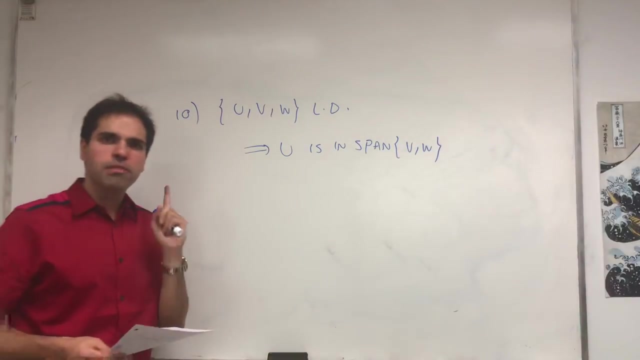 but including dialects, So you'll see a lot of Arabic also, because there are a bunch of different countries that speak Arabic, But this one, the 10th most popular language, is the Wu dialect of Chinese. I think someone told me it's the same as Shanghainese. 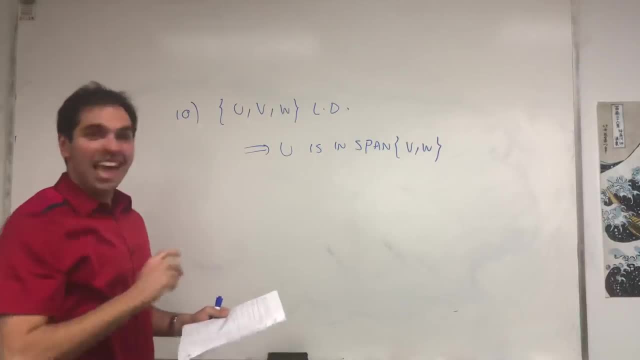 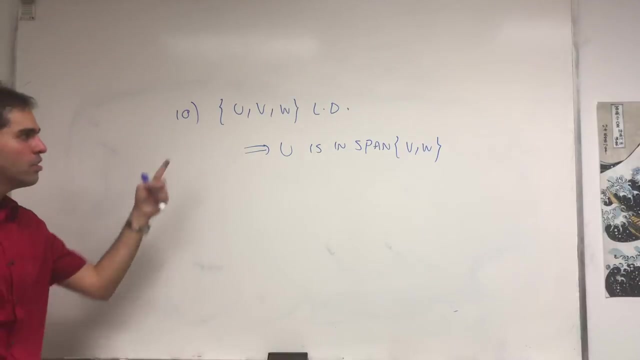 But I'm not 100% sure. And the 10th, most popular- I mean 10 in this Wu dialect- is Cool Anyway. so if a set is linearly dependent, does that imply the first vector is in the span of the other two? 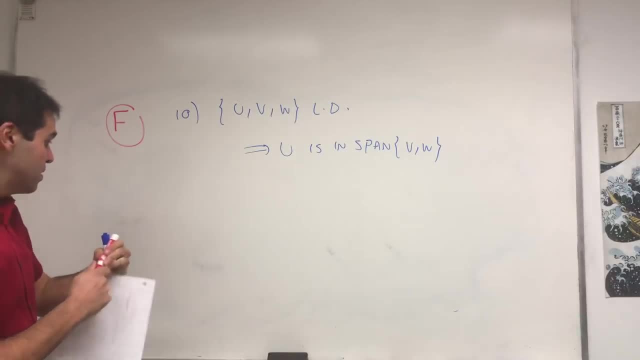 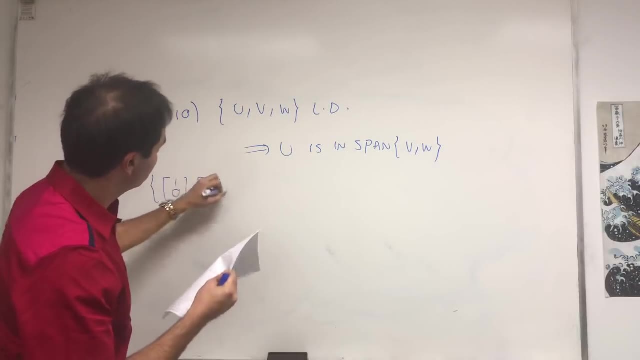 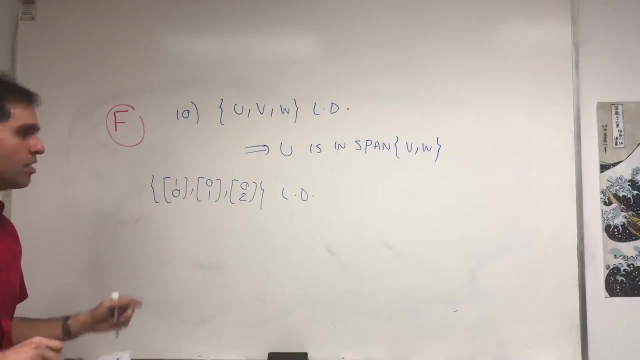 No False Because, for example, let's take the following: set 1, 0,, 0, 1, and 0, 2.. That's linearly dependent because this is 2 times this vector. But, see, 1, 0 is not in the span of those two vectors. 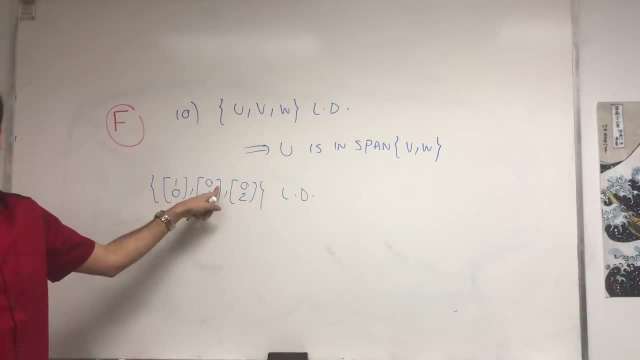 because for the span of those two vectors the first entry is 0. But 1, 0 is not, in that The first entry of 1, 0 is not And 0. So that's why it doesn't work. 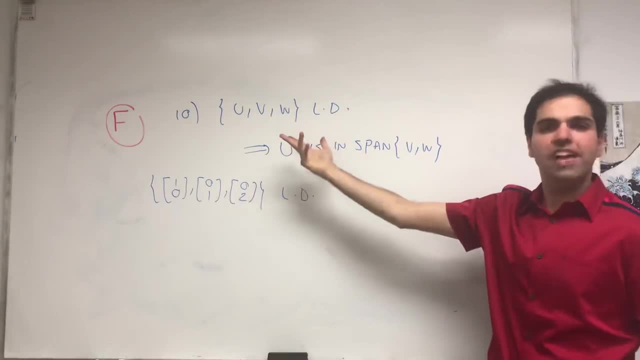 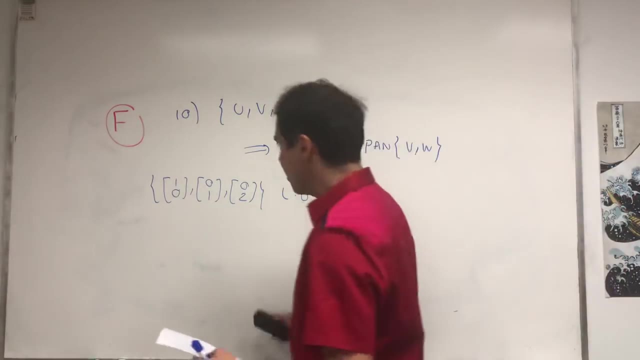 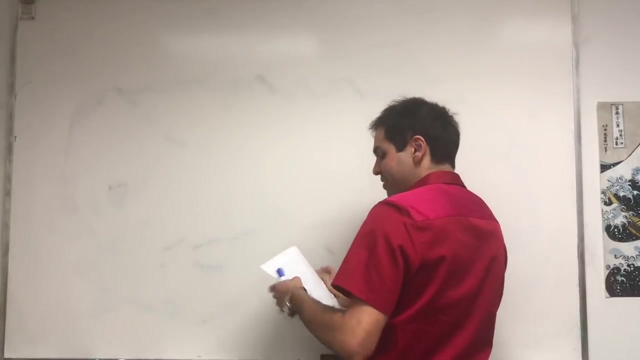 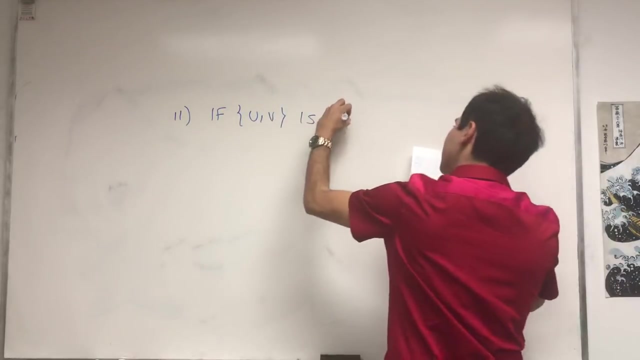 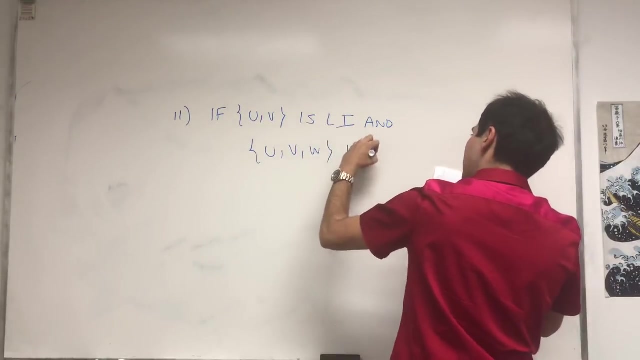 What is true, though, is that one of the vectors is in the span of the other two, but not necessarily the first one. Now let's do a related question, Question 11. If uv is linearly independent, But the whole set uvw is linearly dependent, 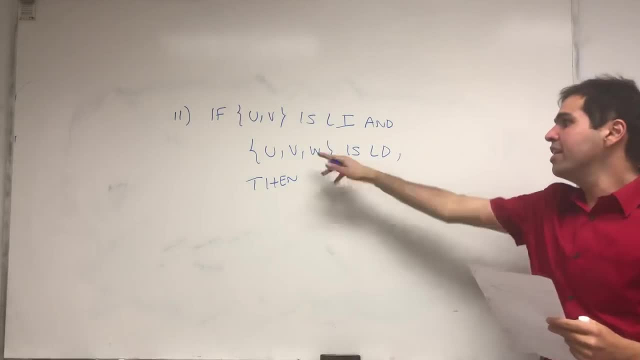 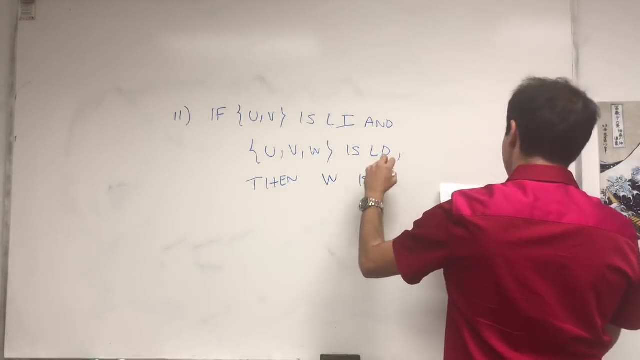 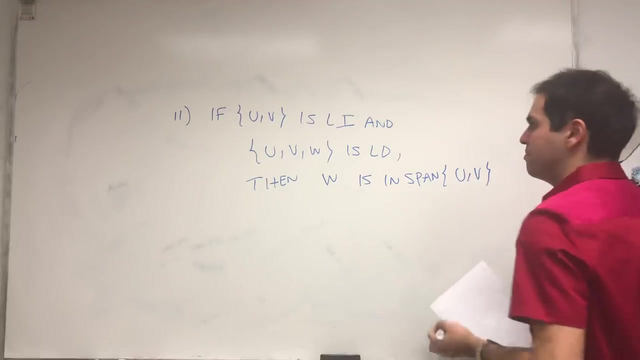 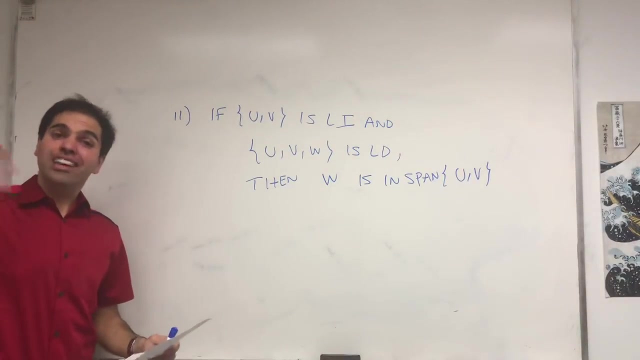 So suppose you start with a linearly independent set And you add a vector, it becomes linearly dependent. Is it true that w is in the span of the first two vectors, 11. Language Language: Javanese. So not Japanese but Javanese. 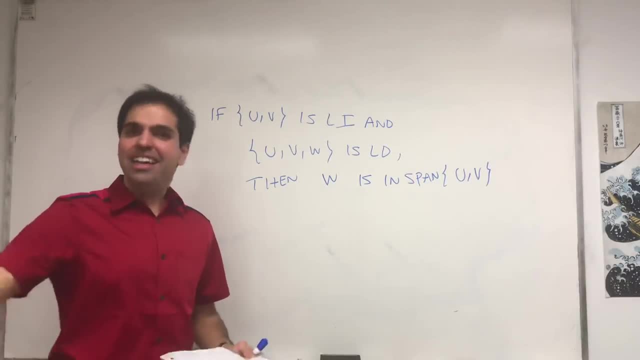 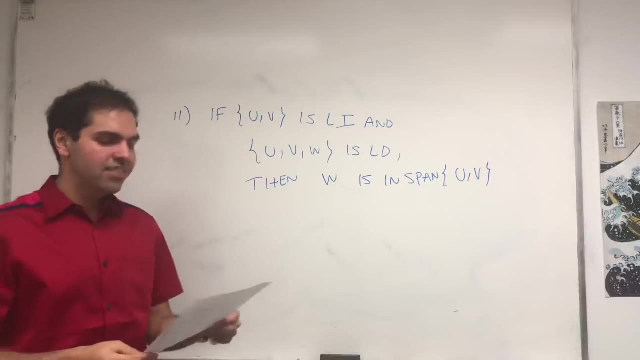 So the languages speak, I think, in the island of Java, And also not the computer science language. so a different language And 11 in Javanese is Ah, alas, And this is true. OK, why is that true? 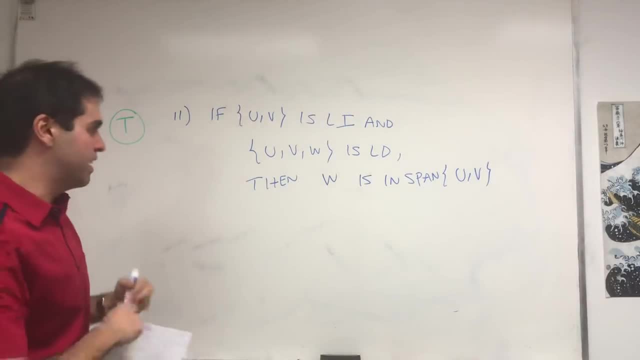 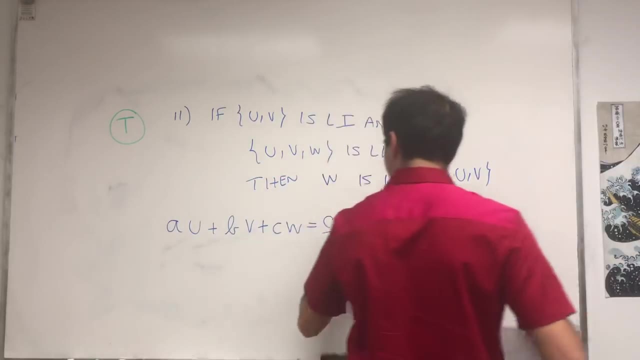 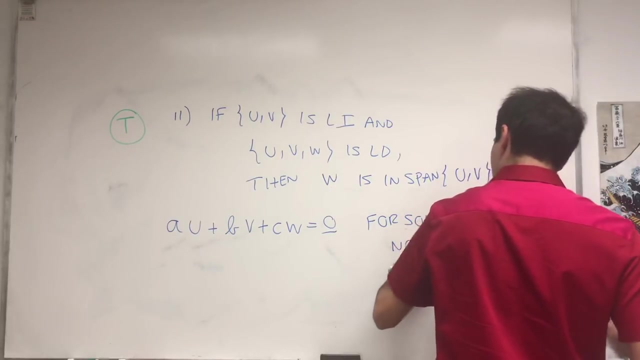 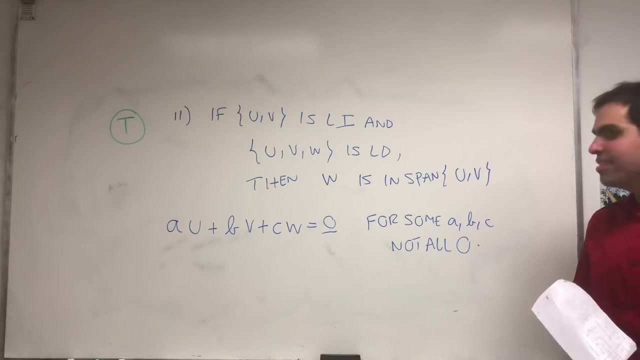 So, because this is linearly dependent, we know that au plus bv plus cw equals to the 0 vector for some abc, Not all 0.. I'm claiming that c is non-zero. I'm claiming that this sucker is non-zero. 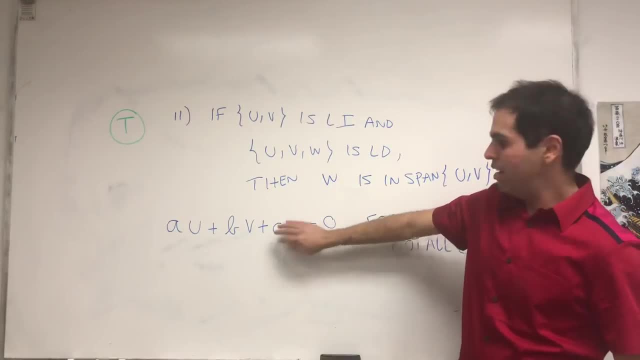 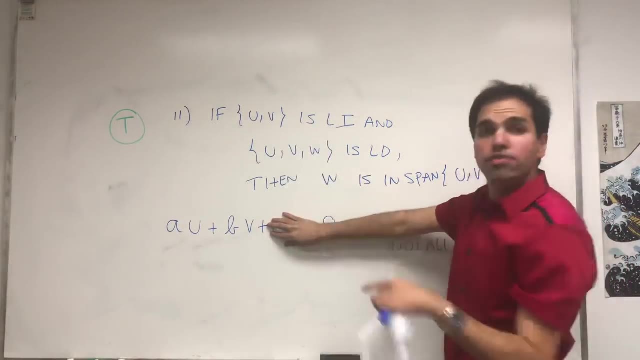 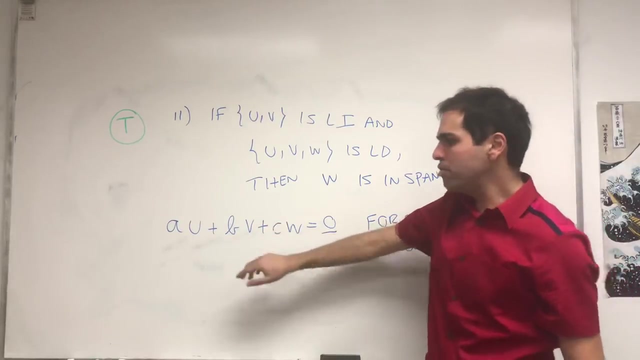 Why If c were 0, then this would be 0. And we get: au plus bv is 0. But look, uv is linearly independent And if we had au plus bv is a 0 vector, we would get a and b are also 0, which is a problem. 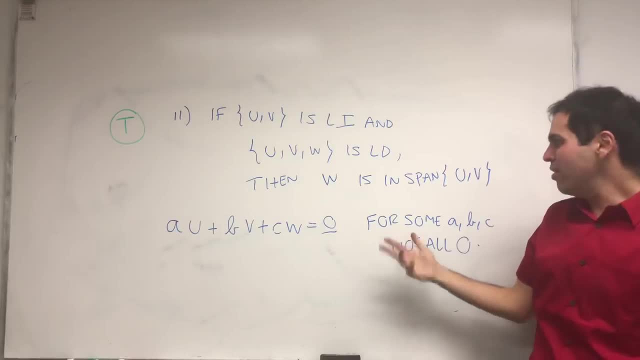 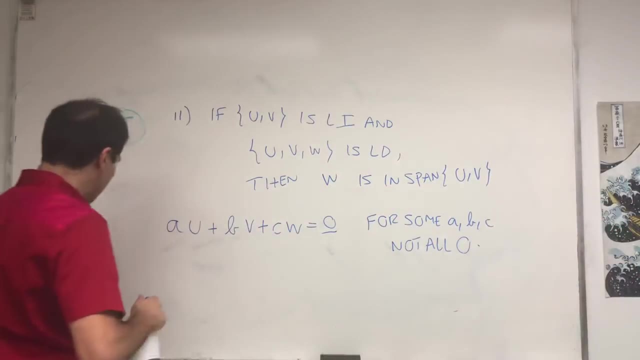 because then ab and c would all be 0, which is a contradiction with the fact that ab and c are not And c are not all 0. So, in other words, I've just shown that c is non-zero, which means we can actually solve for w. 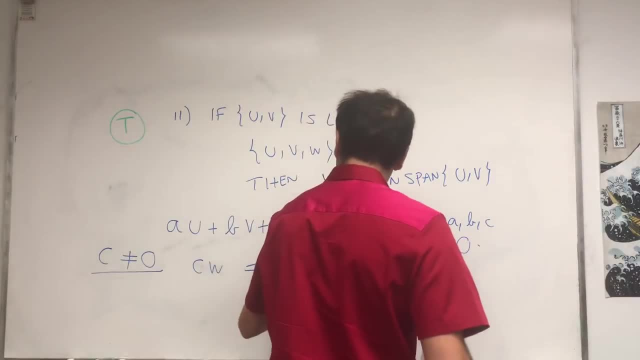 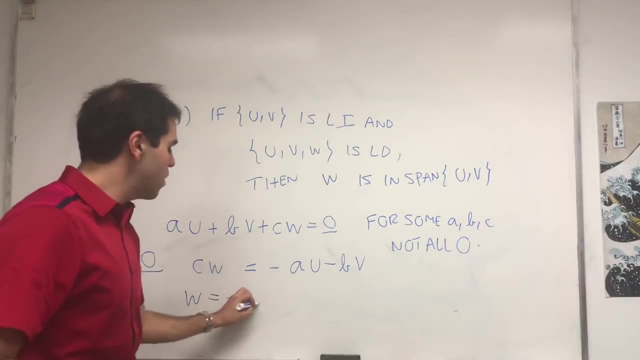 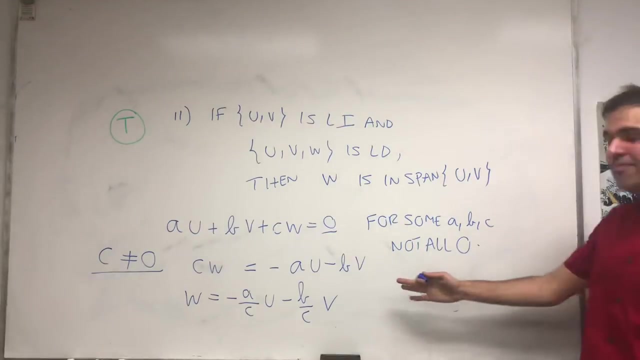 So cw Bay Area is minus au, minus bv. Now, because c is non-zero, we get w. It's minus a over cu, minus b over cv And this precisely means w is in the same order, So we get w. 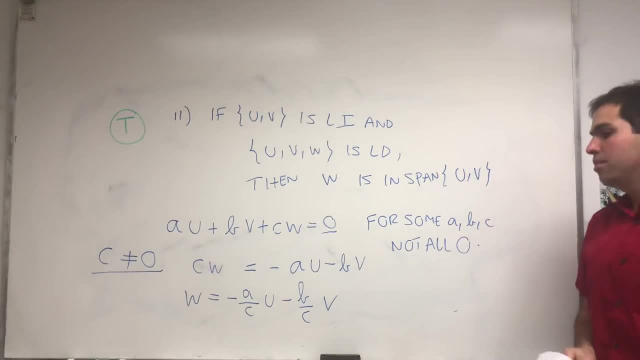 Because w is a linear combo of u and v: Great. 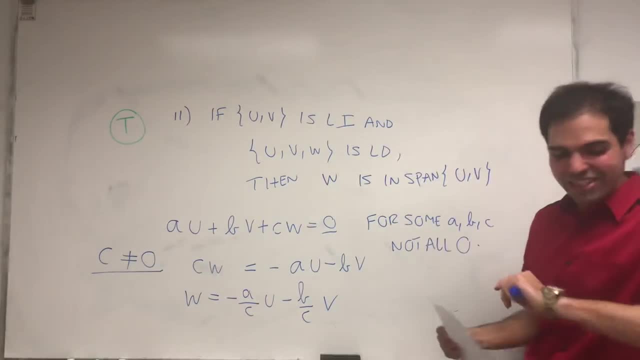 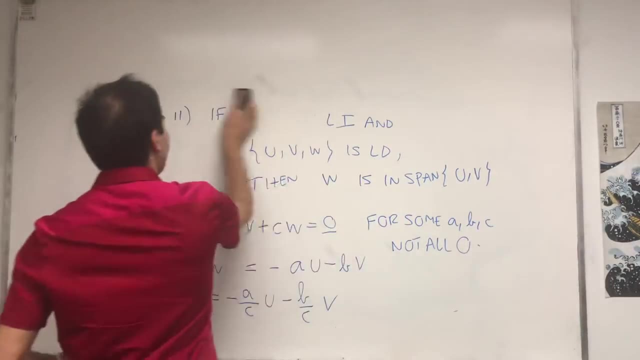 10%, almost 10% done, so we need one more question. And whoa already, what's it called? Yeah, 35 minutes, so we'll see. Damn 300,. hopefully it's not 6 hours, but let's see. 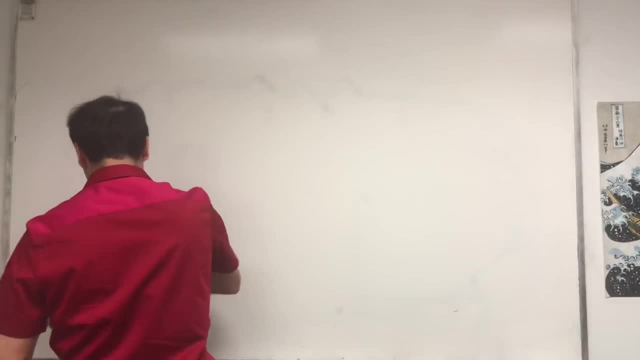 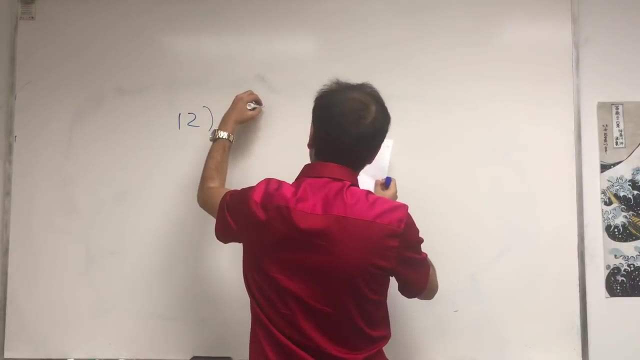 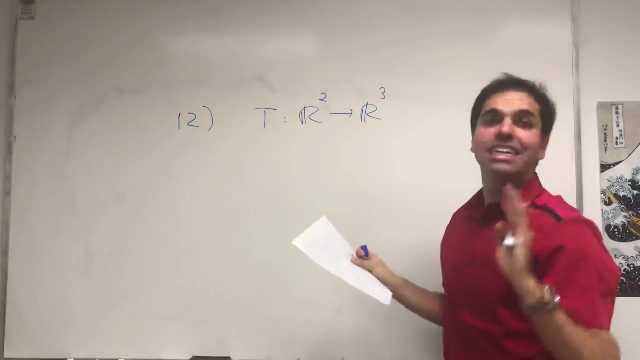 The other ones are kind of long too. OK, let's talk a bit linear transfer transformations now. So if t goes from R2 to R3, and if I write t in this course, it just means that it's a linear transformation. 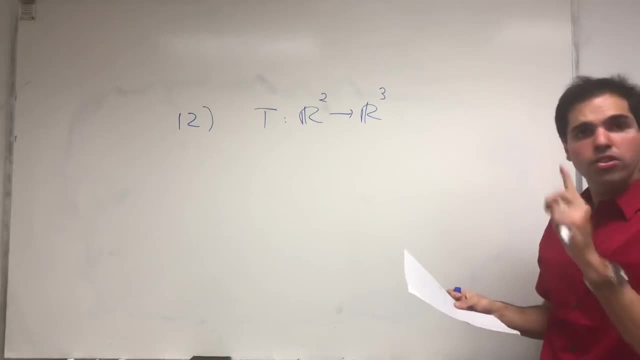 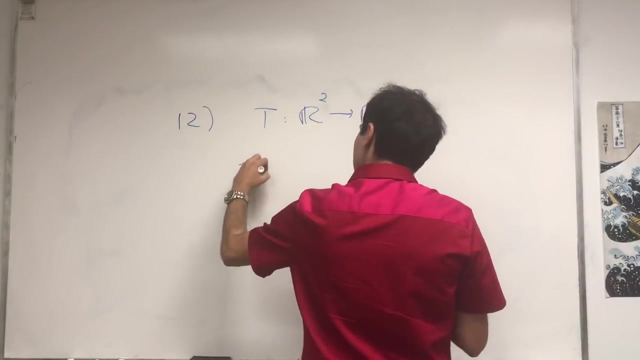 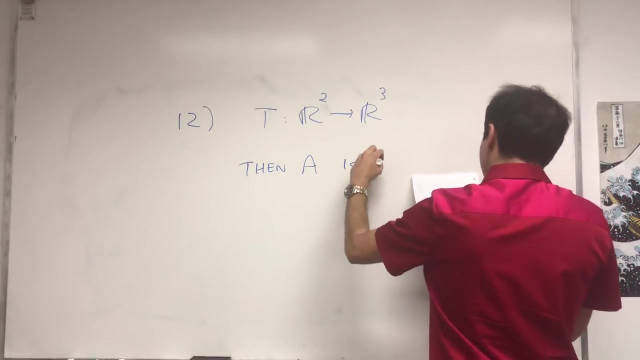 unless otherwise specified. So if t maps R2 into R3, then the matrix of t with respect to the standard basis, so that A, again the matrix of t really with respect to any basis, is a 2 by 3 matrix. 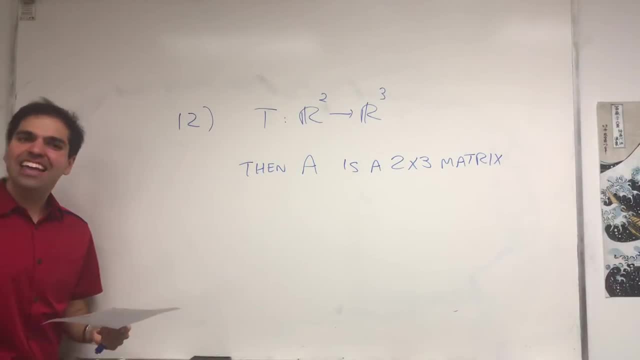 And 12th language, Korean, And 12 in Korean is, I think the L is kind of silent, Nice language, OK, And it turns out this is false. And let's think why it's false. Look, Suppose we have this matrix. 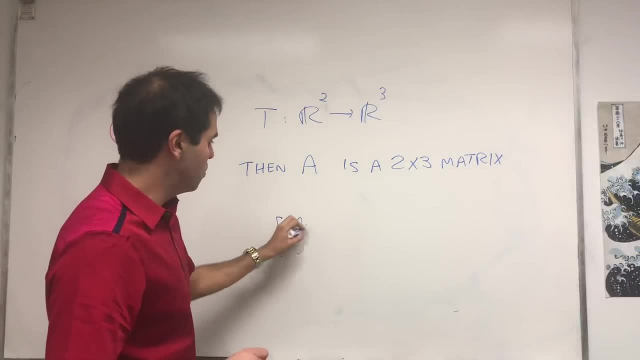 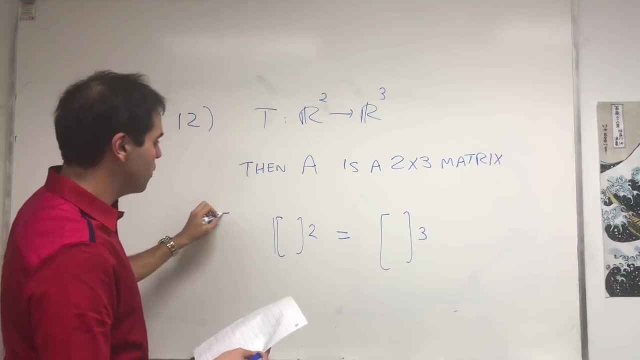 We know the input is a vector of size 2. And the output is a vector of size 3.. Then the only way this matrix multiplication works is if the number of columns of A is 2. And the number of rows of A is 3.. 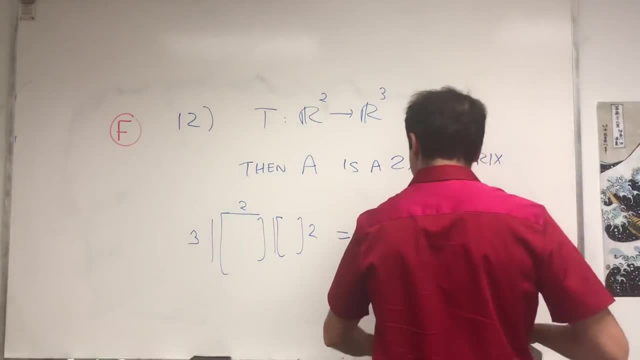 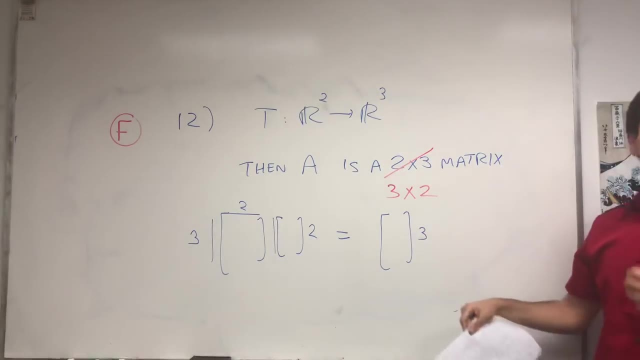 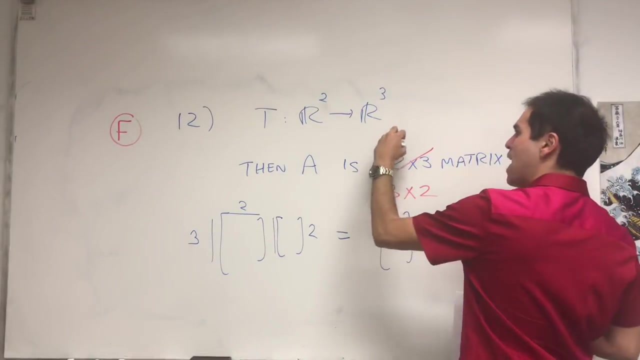 So in fact A is a 3 by 2 matrix. If it were a 2 by 3 matrix, the dimensions wouldn't really match up, And here's a nice way to remember this. So if A is M by N, so here 3 by 2, then N is the input. 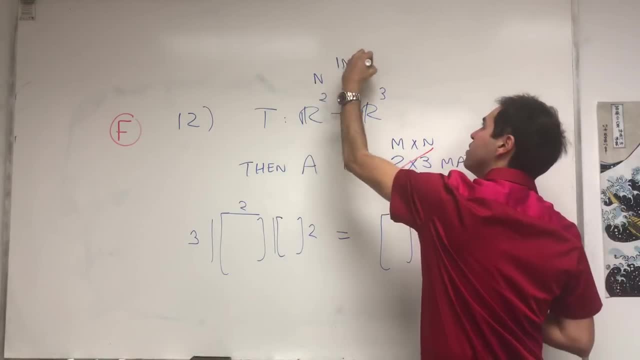 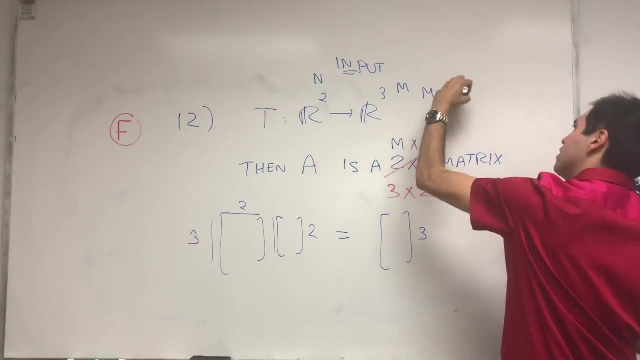 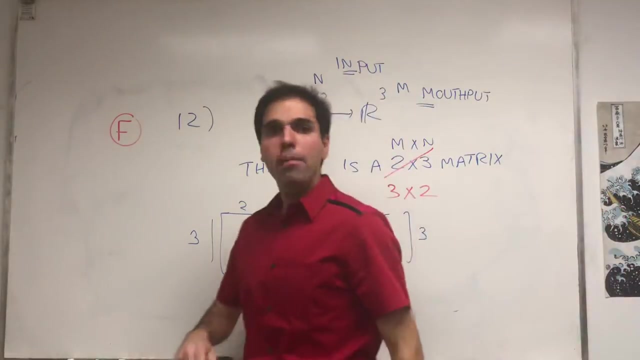 So 3 by 2.. N is the input, So input. so t goes from Rn to the mouthput M, as in mouthput, Like output, but with your mouth. And that's why, if A is a M by N matrix, t goes from Rn to Rm. 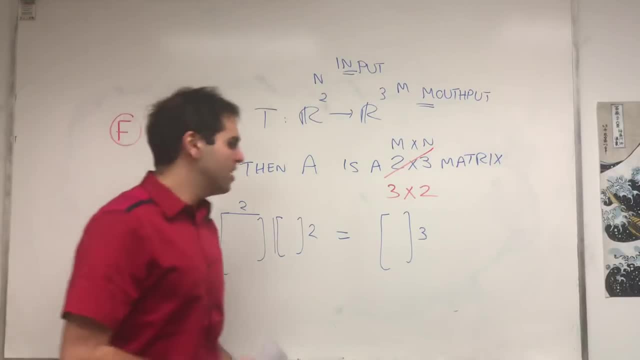 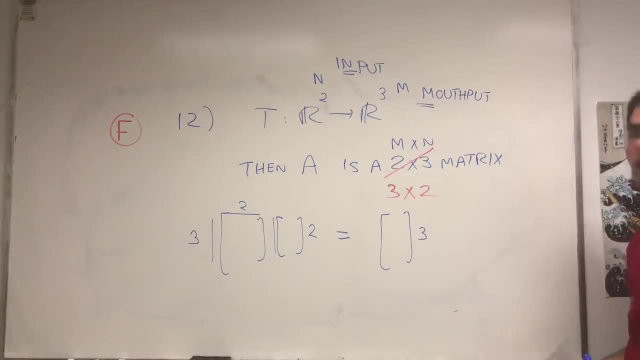 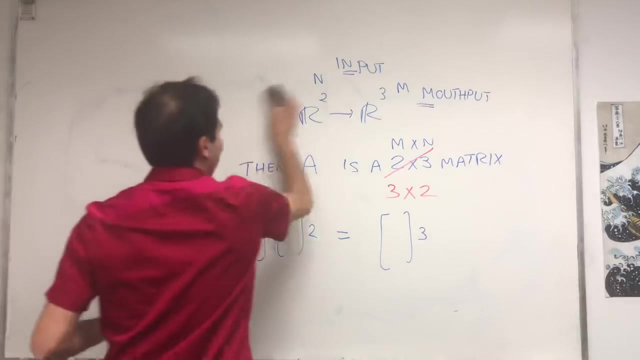 So just remember that you have to switch the two, And I know some other linear algebra books. just say: A is N by M, and then t goes from Rm to Rn, whichever you prefer. All right, that's one thing, And let's talk more linear stuff. 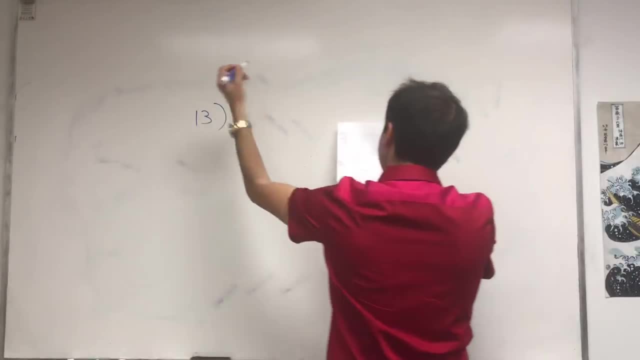 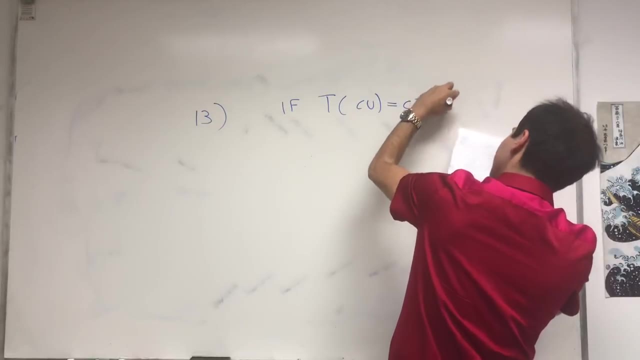 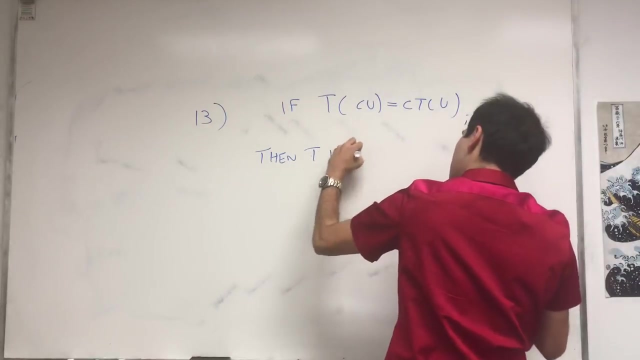 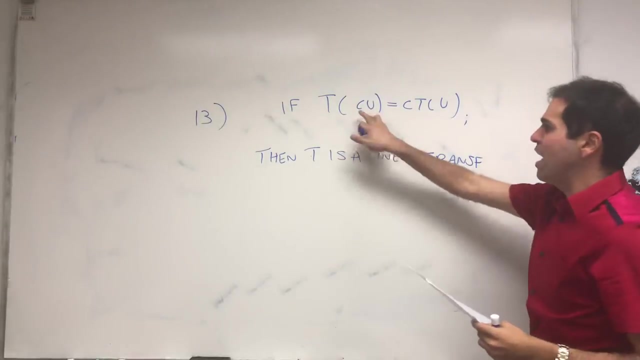 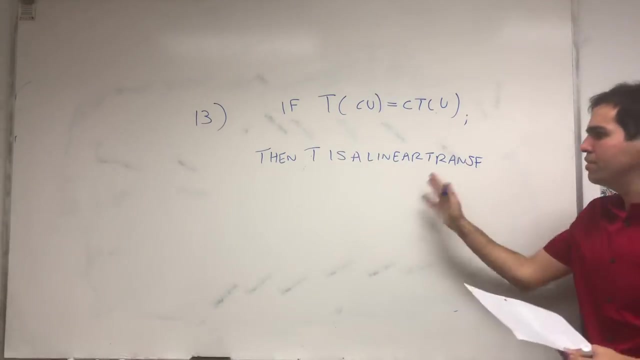 So 30. If t satisfies that t of cu is ct of u, then t is a linear transformation. And here really what I mean: if for every constant c and every vector u, t of cu is ct of u, then t is a linear transformation. 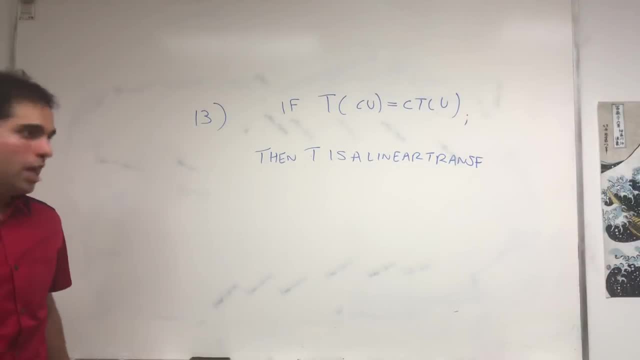 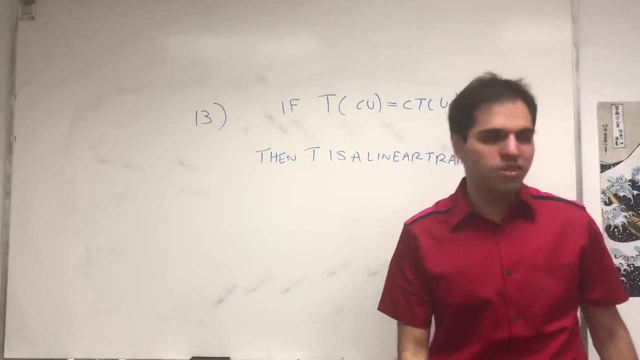 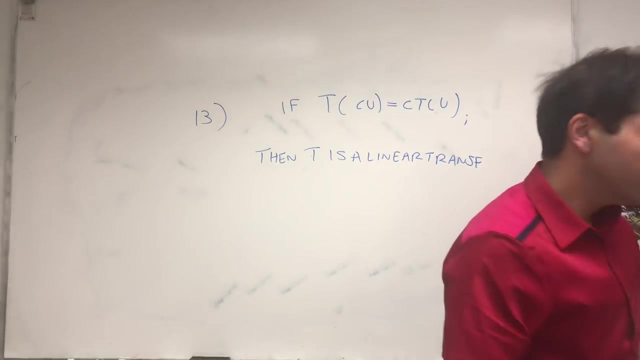 And here I really mean one. let's say from Rm to Rm. in other words, do we need the other property that t of u plus v is t of u plus t of v? Well, think about this. And 13,: the 13th most popular language is French. finally, 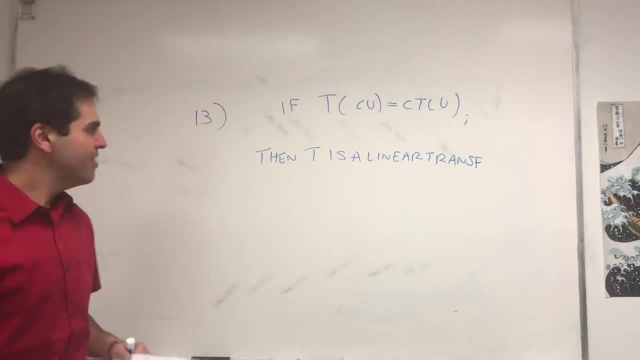 And 13 in French is treize. I went to a French school. that's why this is exciting. And well, I don't know. And well, there's got to be a reason we need the other property. So it turns out it's false. 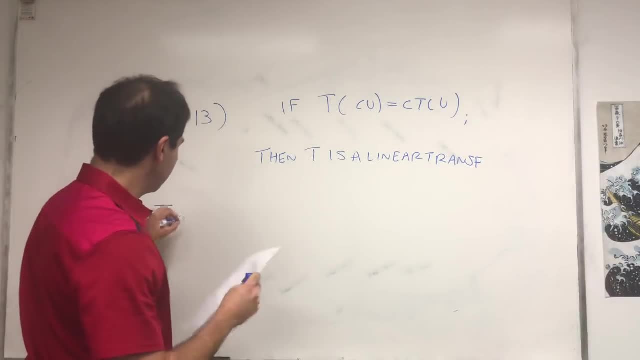 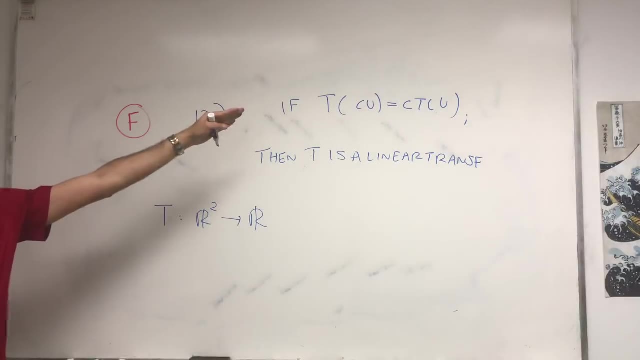 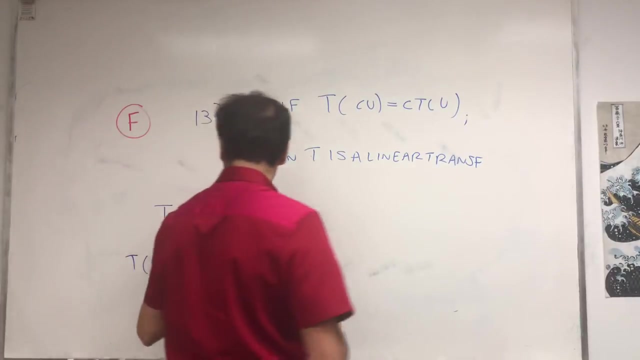 And here let me give you an example: t in this case, from R2 to R. So let's just think of a function that satisfies this, but which is not linear. Okay, so t has two values as an input and spits out another value. 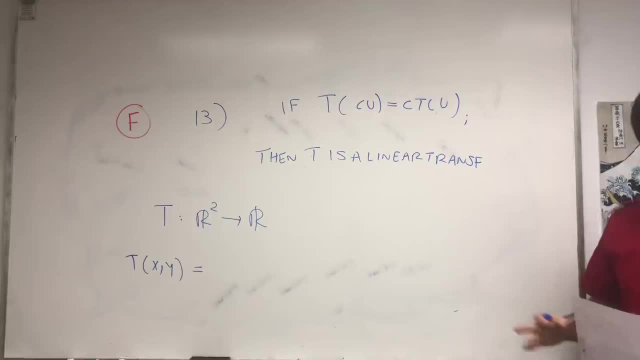 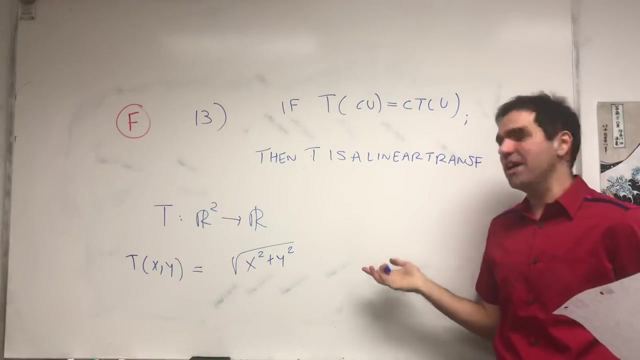 Here's the thing. One idea would be: square root of x squared plus y squared. The distance function which you usually think of multiplicative, like the norm of cx, is c times the norm of x. but not quite true. So what I just said was false. 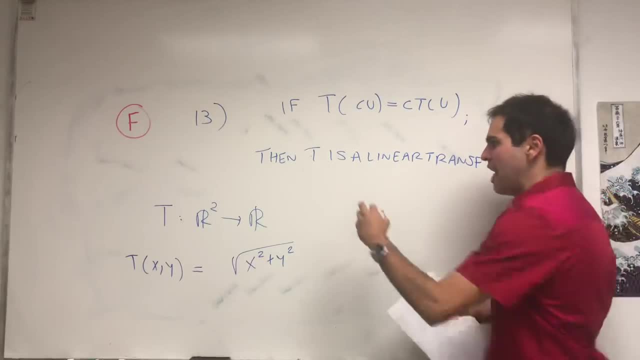 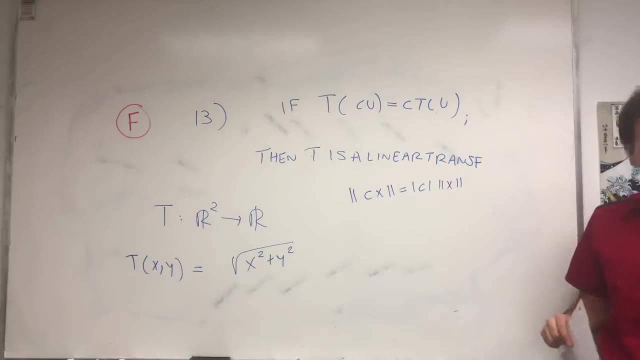 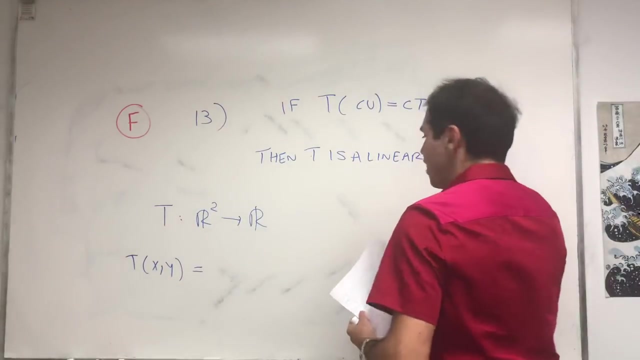 because we have the absolute value business. You know, the length of cx is absolute value of c times the length of x. So we just need to modify this function a little bit to make this work And, in fact, instead of using squares, 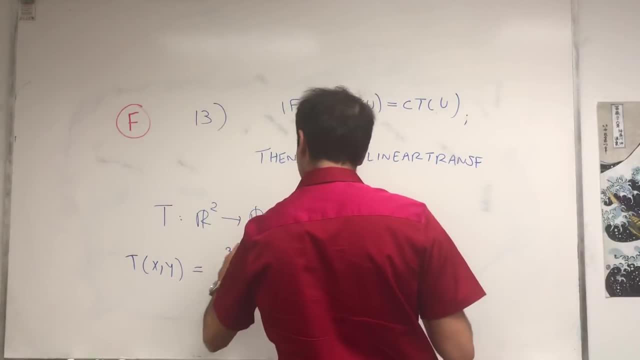 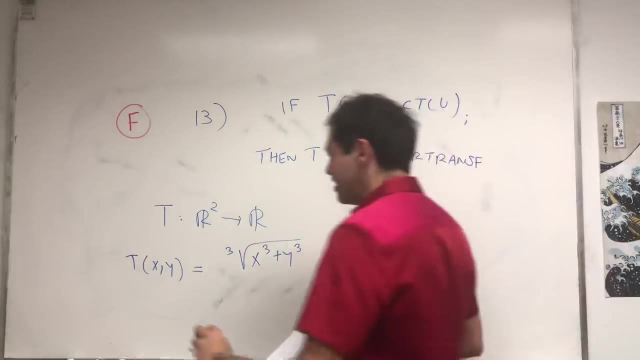 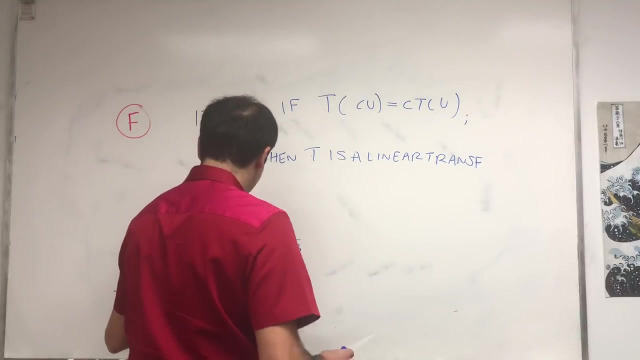 let's use cubes. So in fact the correct answer is cube, root of x cubed plus y cubed, And you can indeed check that. t of you know c times this, so cx- cy, it's cube root of cx, y and y. 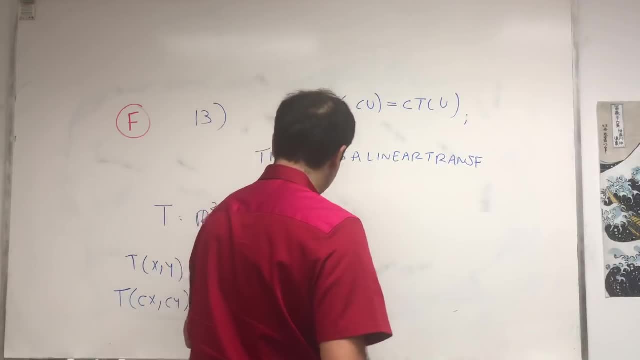 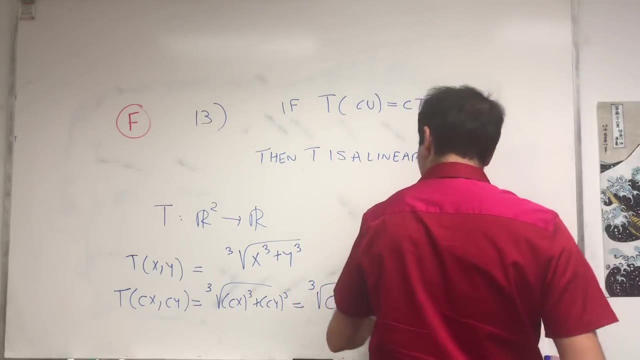 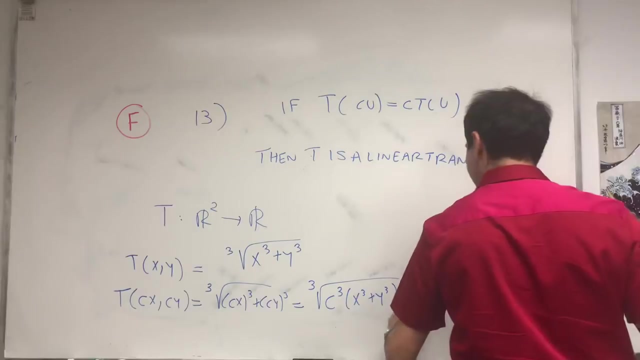 So that's x cubed plus cy cubed And if you want that's cube root of c cubed times x cubed plus y cubed And then that just becomes c times cube root of x cubed plus y cubed. 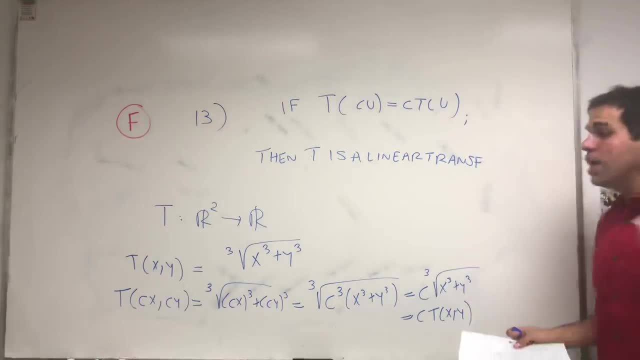 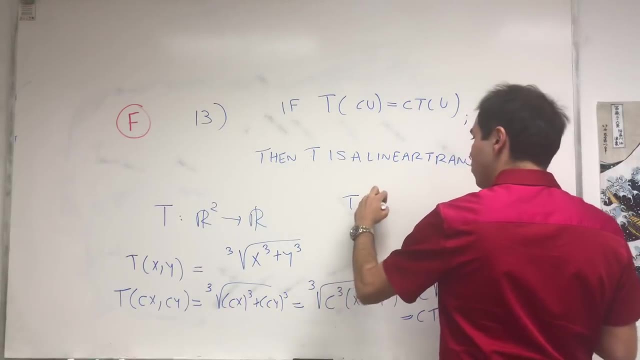 And that's in fact c times t of x, y, So it is multiplicative. but it turns out it's not additive because, for example, t of 0, it's 1.. t of 0, 1, it's 1.. 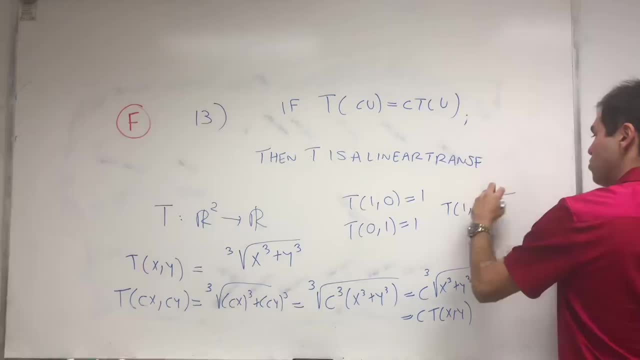 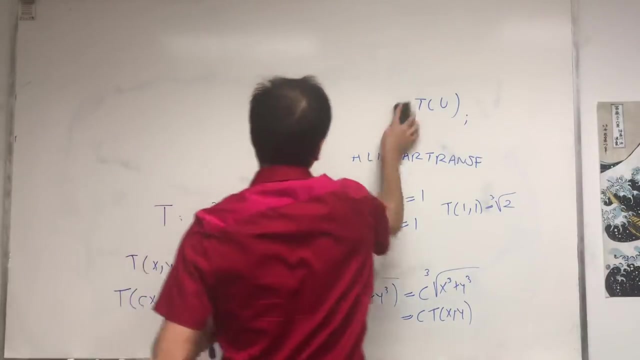 But if you add them, t of 1, 1 becomes cube root of 2, which is not 1 plus 1.. So indeed we need that. you know the other property that is additive. All right, what about the other one? 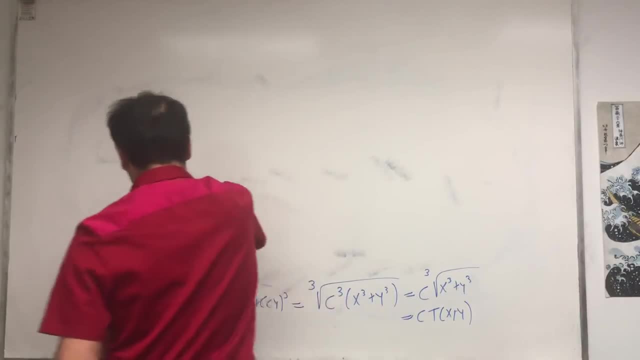 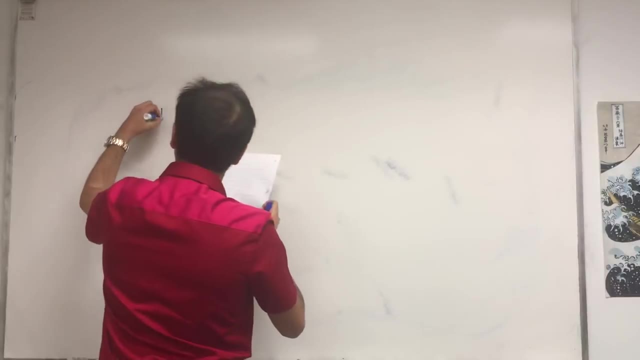 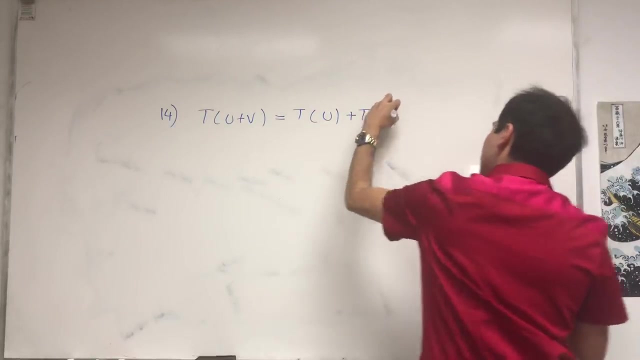 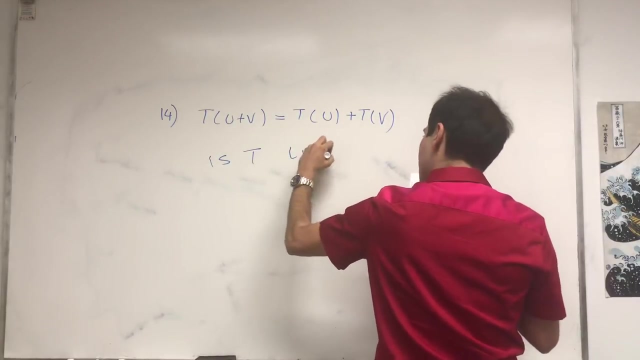 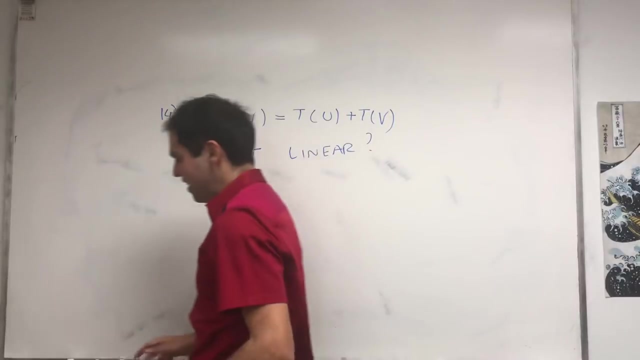 Suppose it's just additive but not multiplicative, So question 14.. So suppose t of u plus v is t of u plus t of v for any vector u and v. Then the question is: is t linear? Okay, 14th most popular language. 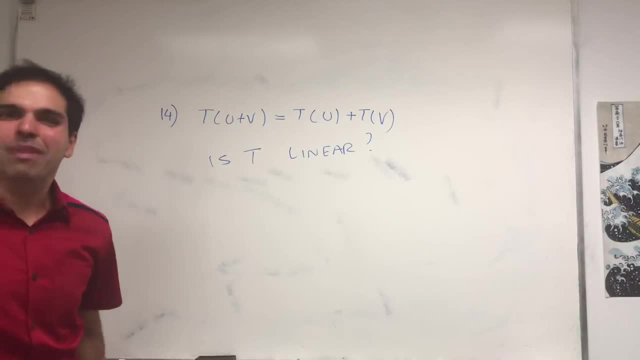 Vietnamese, And I'm super excited, by the way, because I'm going to Vietnam and Thailand for spring break. So that's one. I really like this question, And 14 in Vietnamese. it's muy bon. I love this word because it sounds like muy bien. 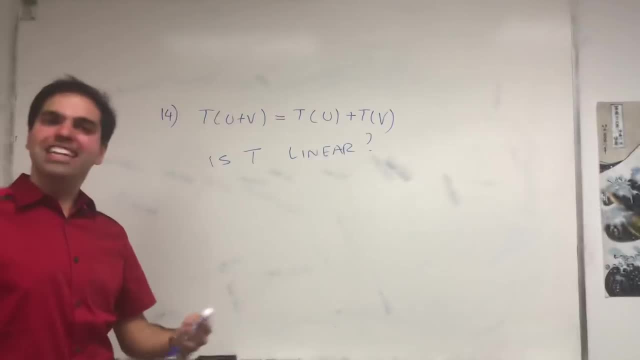 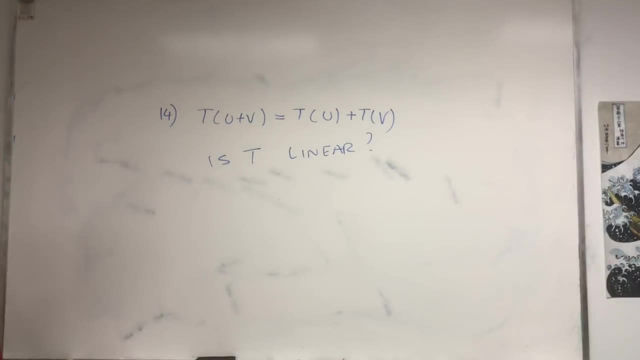 but it's like sort of a mix of Spanish and French, because bon means good, So it's like muy bon, Très bon, And in fact I love that question because this one is interesting And of course, as you might guess, it's false. 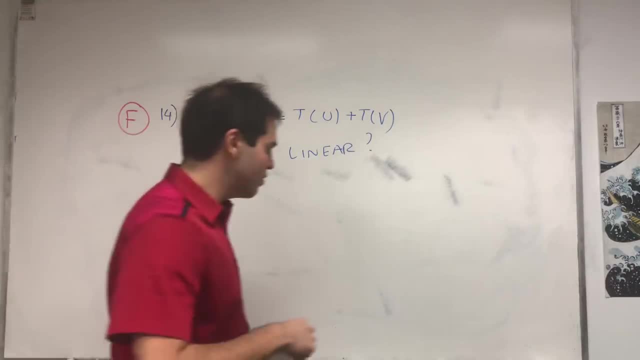 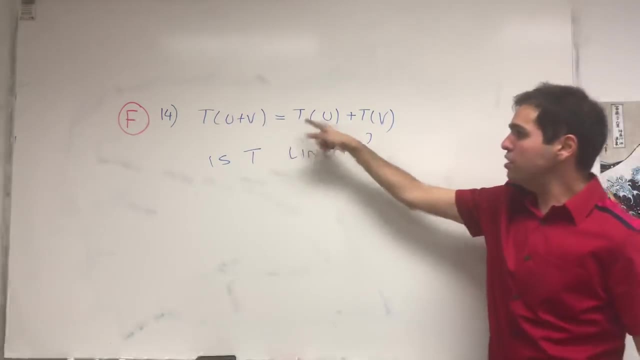 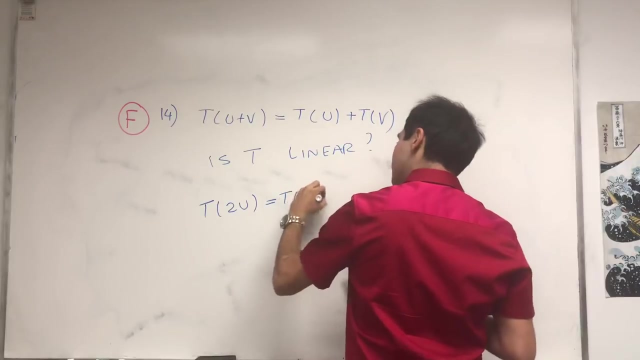 We really need all the properties. But why is it false? And this is super cool, because it's almost true, Because, look, if t of u plus v is t of u plus t of v, then t of 2u is t of u plus t of u. 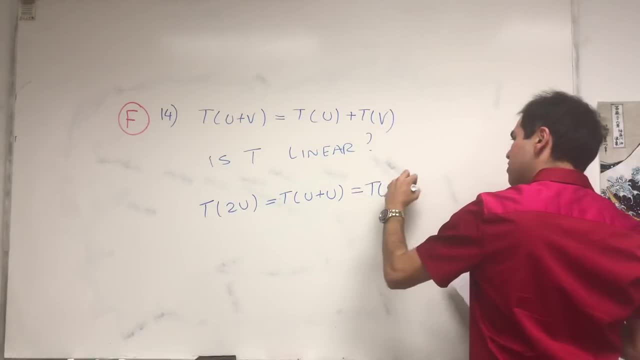 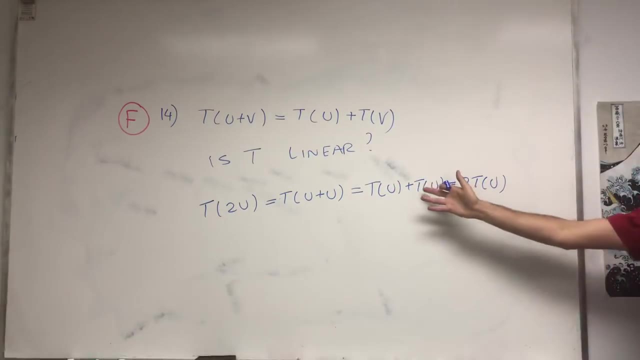 So t of u plus u, which is t of u plus t of u, And that's 2t of u. So at least for positive integers this is true, that t of cu is ct of u And you can actually show for every rational number. 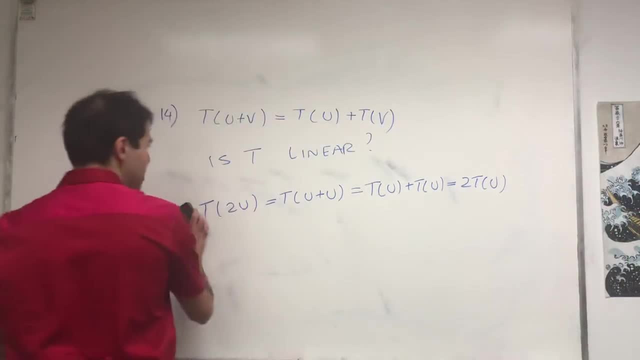 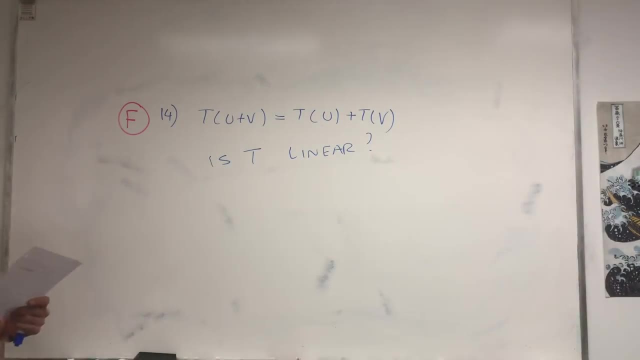 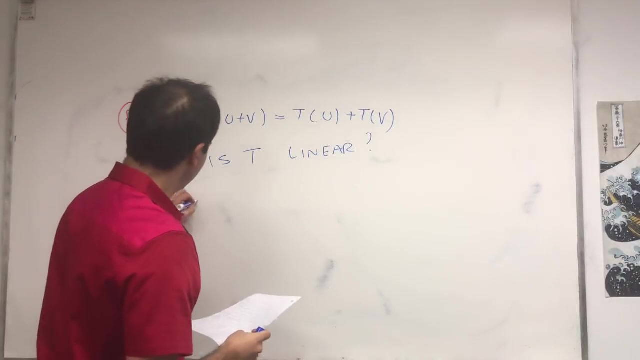 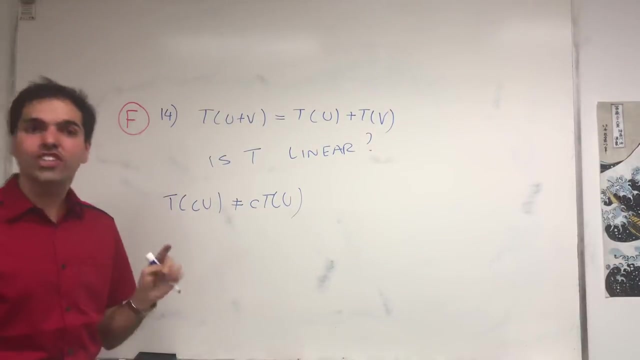 this is also true, just by repeating all those things. But the question is: why is it not true, like for in general, why is it not true that t of cu is not equal to ct of u And, in fact, the construction is so weird? 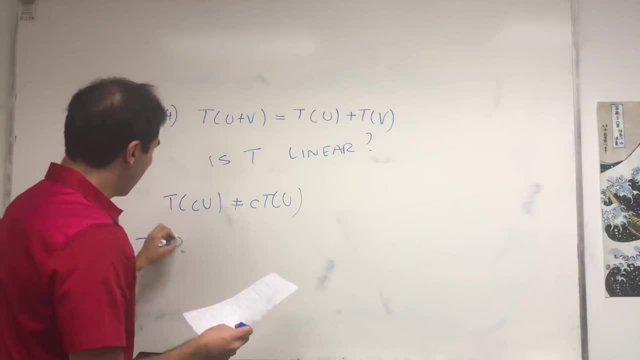 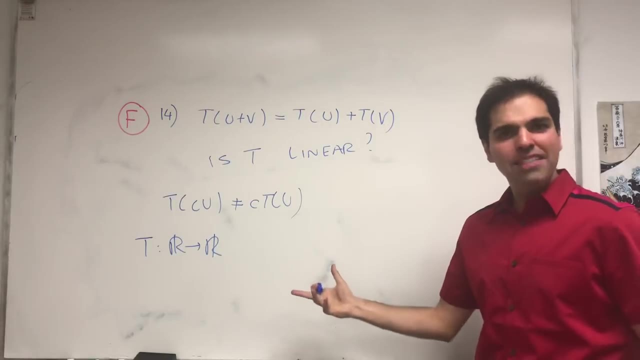 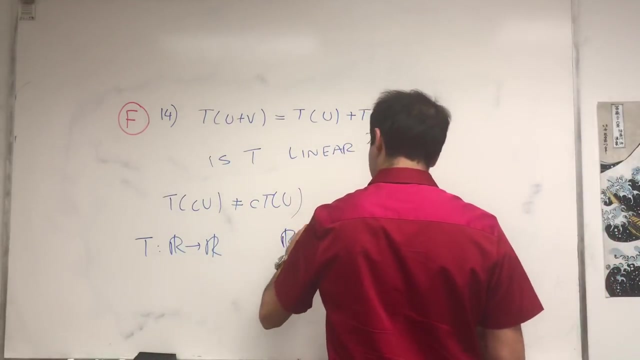 So let me show you what it is. Consider t from r to r, And here r is not a vector space over r, So the field in this case is not r, it's just q, So r over q. So suppose your constants c. 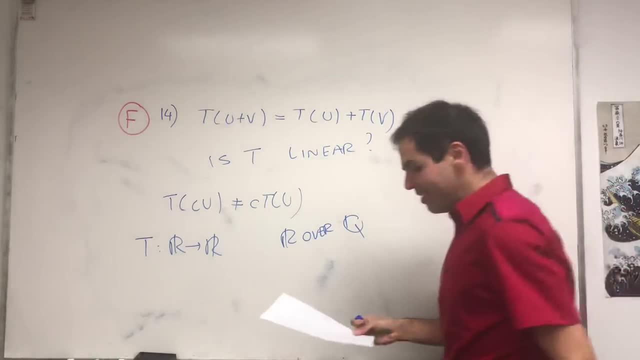 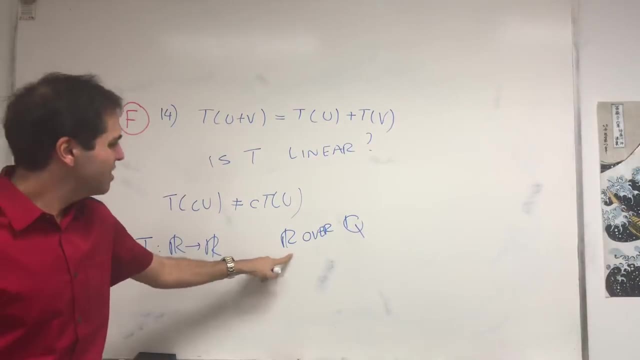 are just rational numbers, Then at least yeah, we'll see. Okay, so possibly my example is not true. So consider a vector space over this and consider the following basis. So in other words, consider this set 1 squared of 2.. 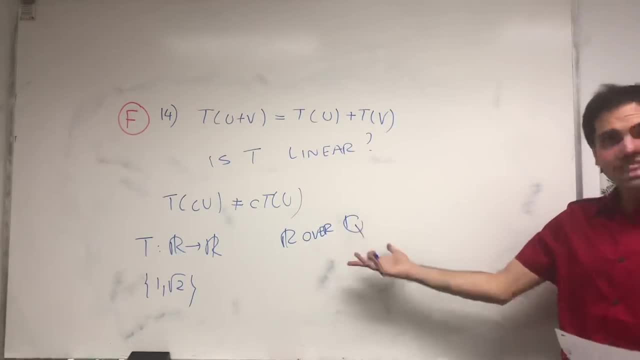 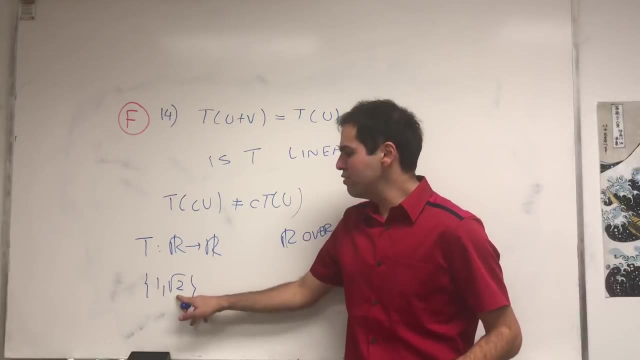 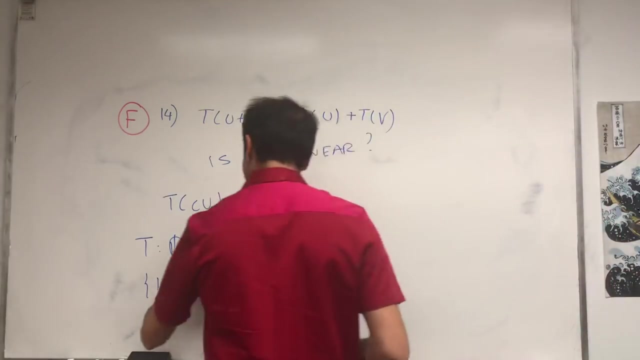 Well, it's linear. it's linearly independent over q, Because there is no way basically to write squared of 2 as a multiple of 1, as a rational multiple of 1.. So this is a linearly independent set. 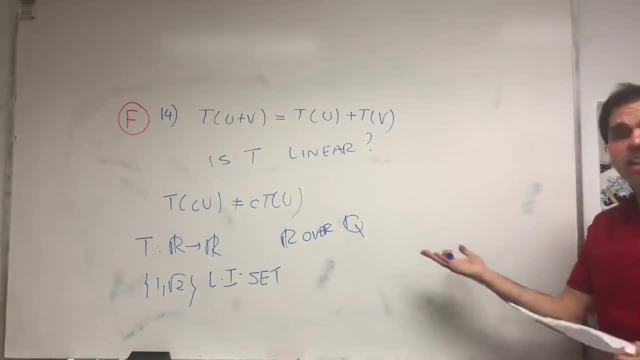 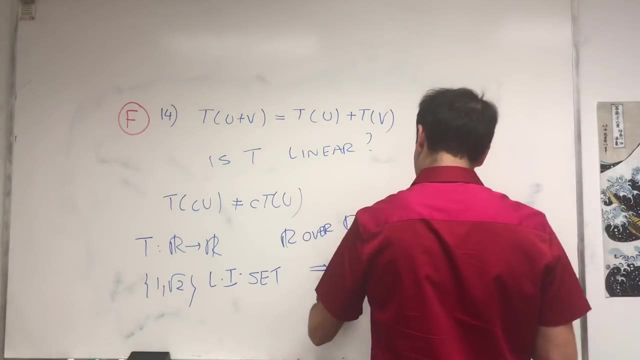 And here's a nice thing on linear algebra: Any linearly independent set, you can extend it to a basis of r, To a basis of r, And I know this is such a weird construction, but it turns out this is the easiest example. 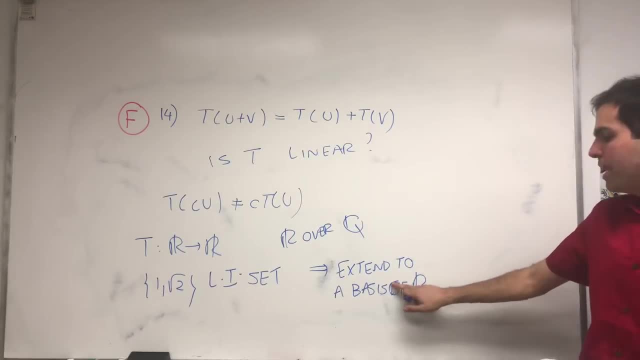 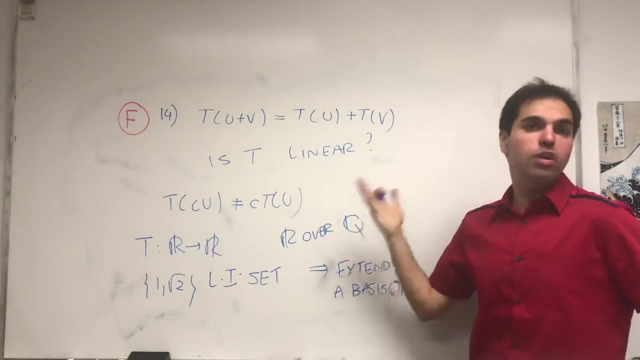 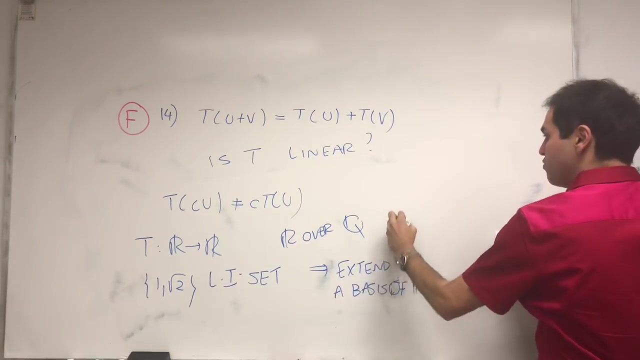 So we have this linearly independent set. We can extend it to a basis And remember to figure out a formula for t. all you need to know is what it does to every element of that basis. So, in other words, define t as follows: 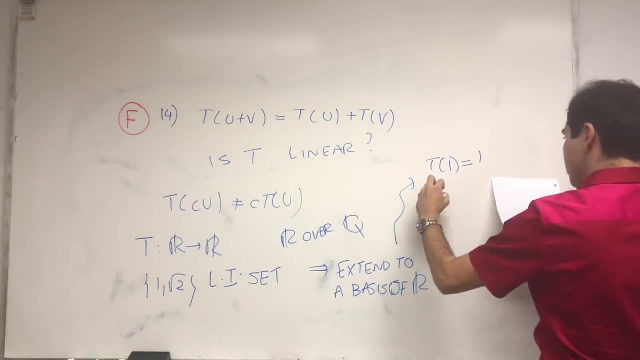 So t of 1 is 1.. t of square root of 2 is 0.. And t of anything else- any other basis vector- is 0.. In other words, graphically t looks like that, So this is 1.. 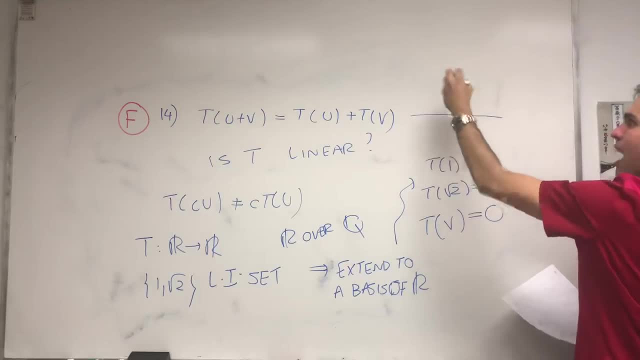 It's 1.. And then you know, for every rational number it's 1., And basically for square root of 2, it's just 0. And everywhere else it's 0.. So that's 0.. 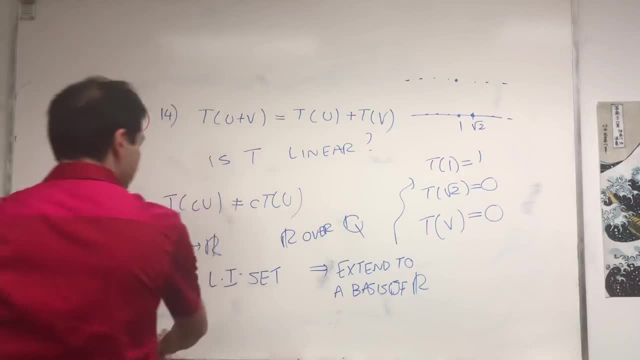 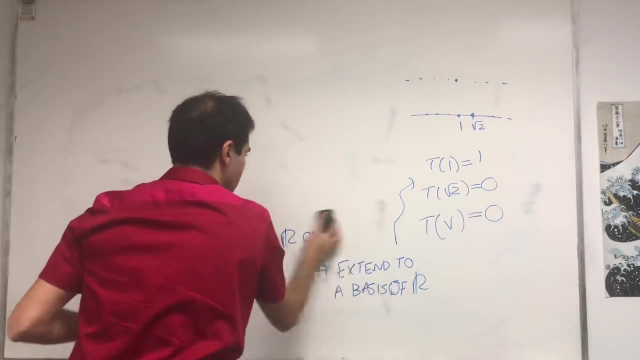 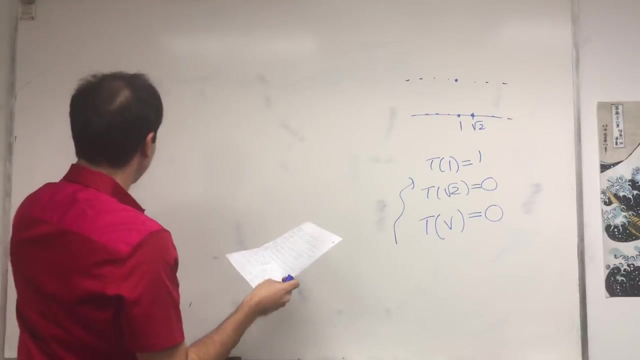 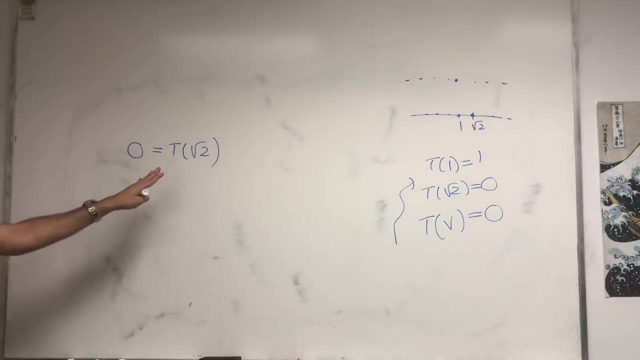 All right, And I'm claiming it's not linear, at least over c, I mean over r, Because then what do we have? Let's see then? Well, t of square root of 2.. That's 0.. But if t were linear, 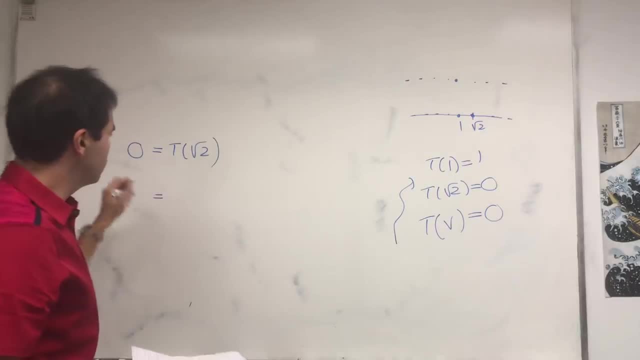 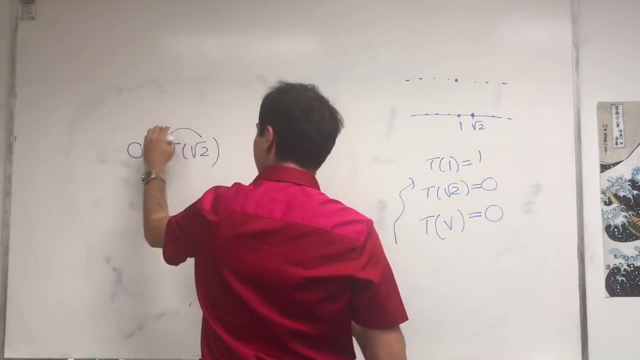 this is what I'm kind of a bit confused about, because we assumed over the rationals, but let's assume over the real. So if it's linear over r, then it means we can pull out the square root of 2, because it's t of square root of 2 times 1.. 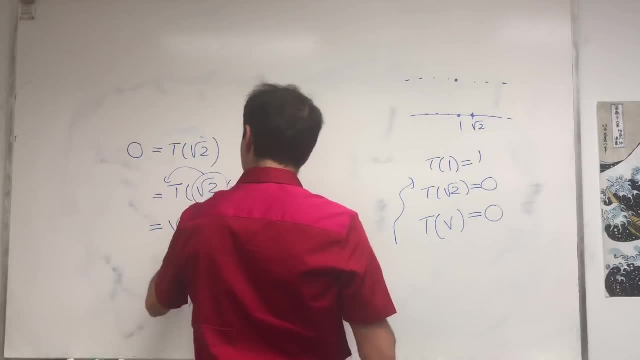 Pull out the square root of 2, and we get square root of 2 times t of 1.. And we get square root of 2 times 0,, sorry, sorry, square root of 2 times 1.. And that's square root of 2.. 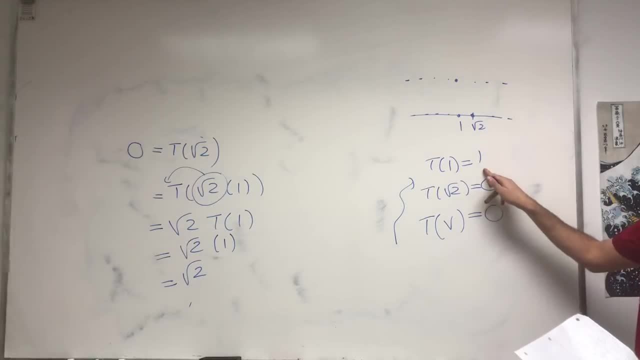 So what I meant to say is this thing: you can actually show that it's additive just because it's linearly independent. But if it were linear, at least over the real number, then you would have this contradiction. So this t is actually not a linear transformation. 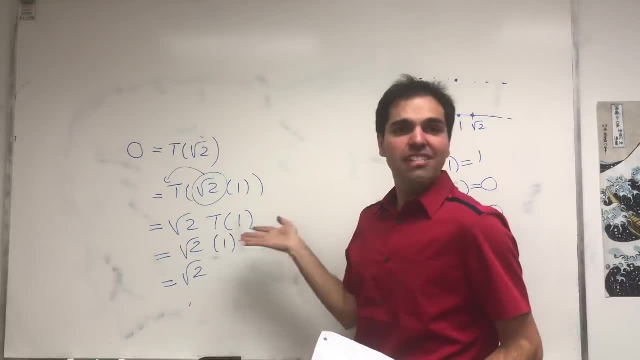 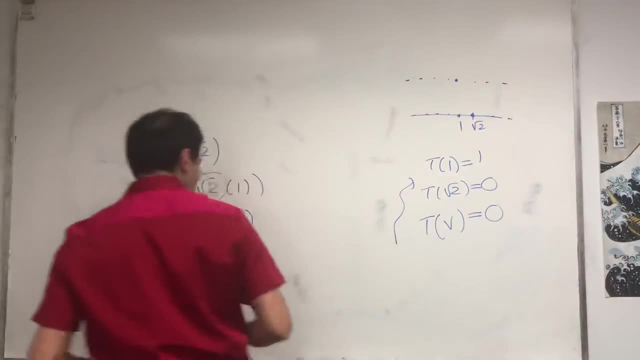 So that's why we get an example, That's why I'm saying the two- what's called the two properties- are very important, So you cannot just go with one of them and not the other. Great, So first sheet is done. 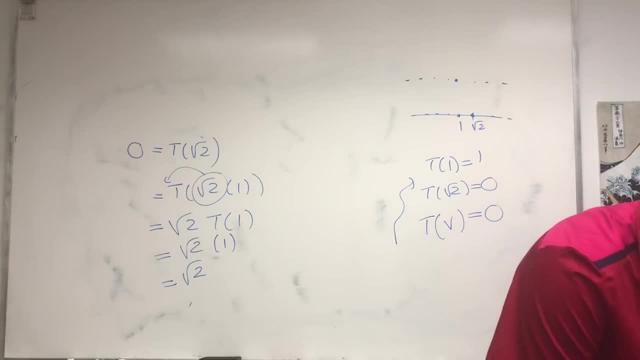 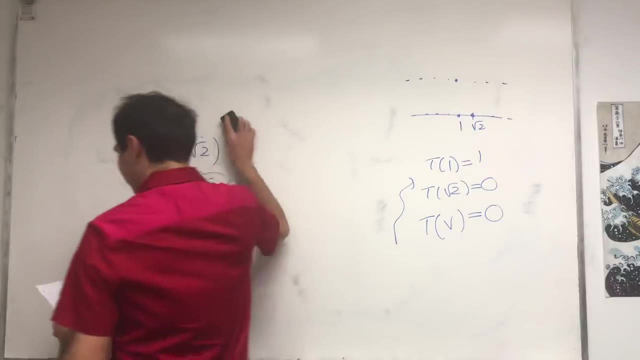 Let's see how many do I have left: 1, 2, 3, 4,, 5, 6,, 7, 8.. Oh, only 8.. So it's not too bad, But I think that was the hardest question. 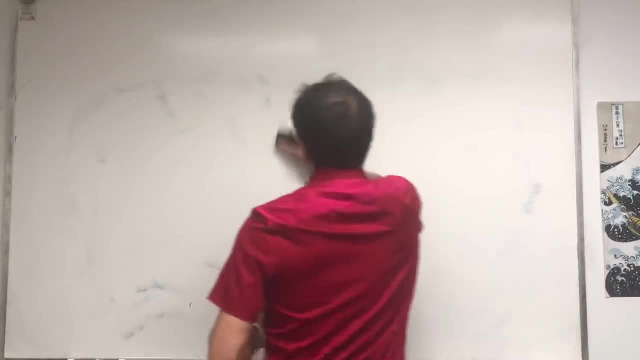 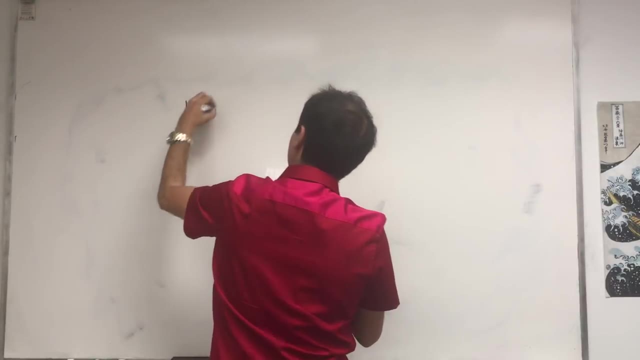 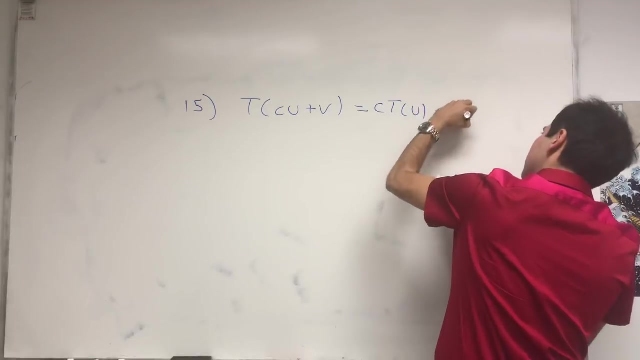 I just don't want to. I have no idea how to solve it, but Okay, question 15.. Again still with linear transformations, Suppose that in this case, t of c? u plus v is c? t of u plus t v. 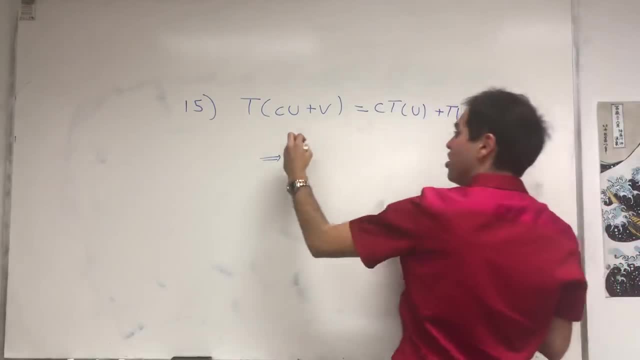 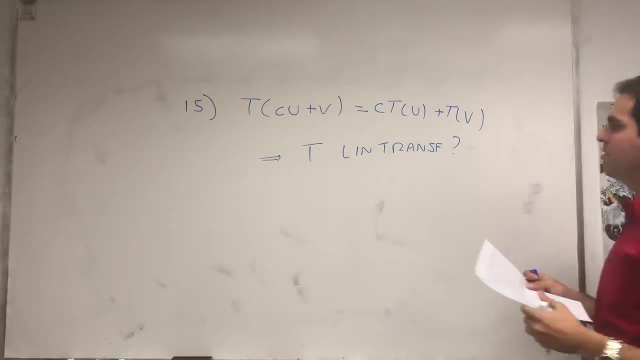 Question is a really strong assumption: is t a linear transformation. Suppose this property holds for every vector u and v and every constant c And 15th most popular language. I've never heard of it. actually that's a weird thing. 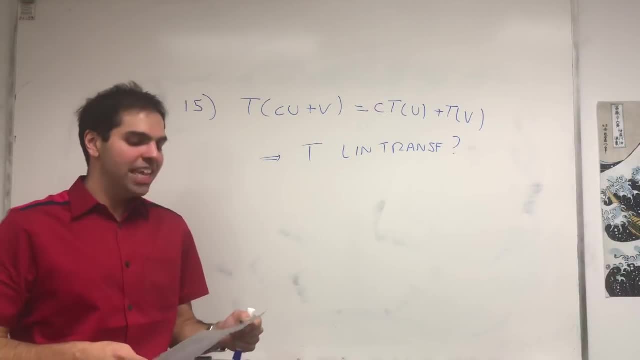 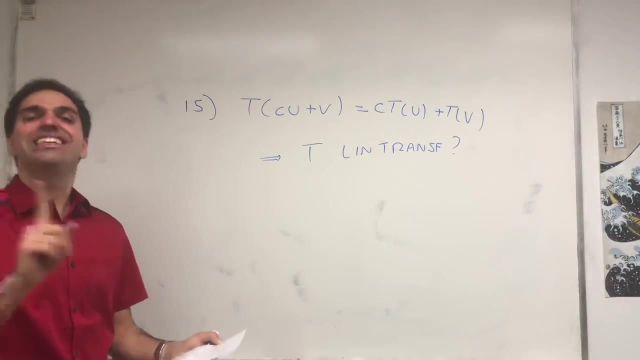 it's telugu And 15 in telugu. it's cute, it's padihenu. Remember this. this will be important for question 18.. So, padihenu And this thing. well, it turns out, it's true. 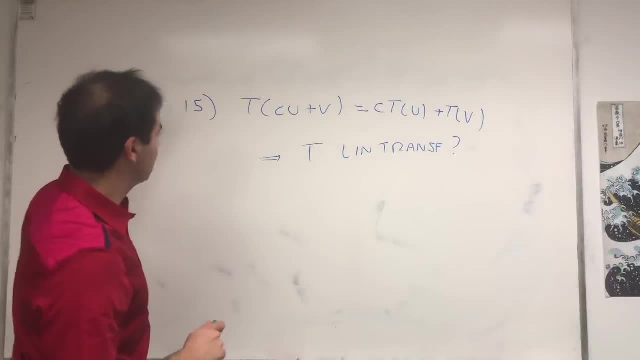 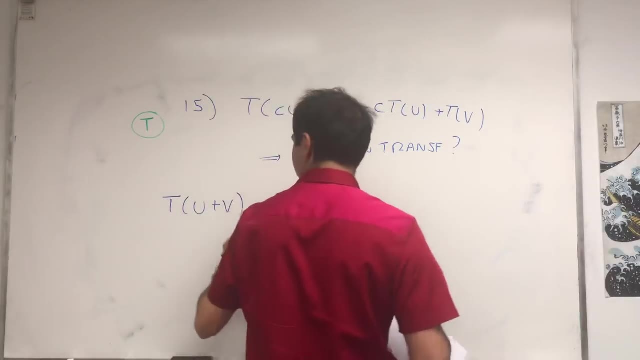 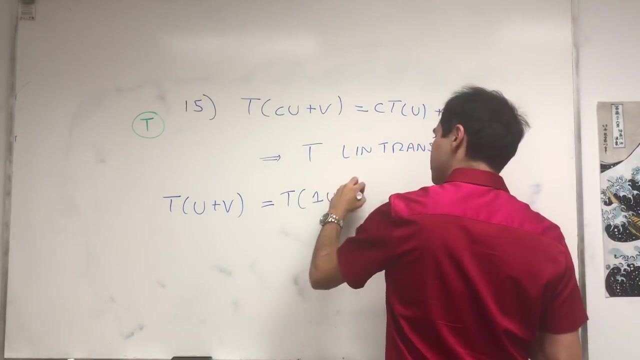 So it's a very neat way of expressing linear transformations with just one formula. Because, look, suppose you want to show t of u plus v, is t of u plus t of v. Well, that's t of one u plus v. So if you let c be one. 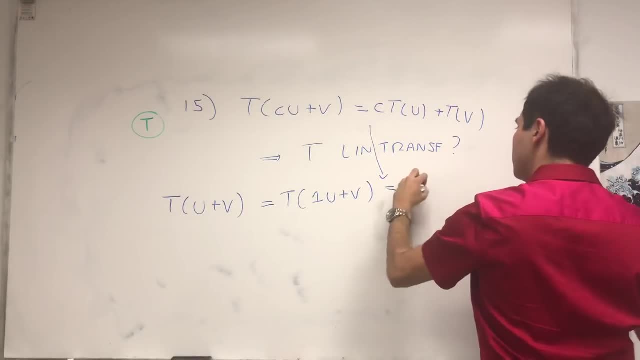 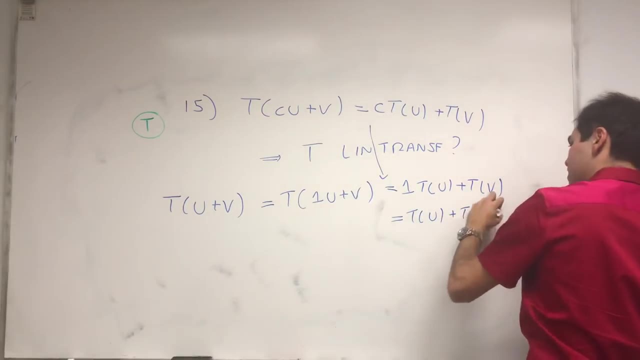 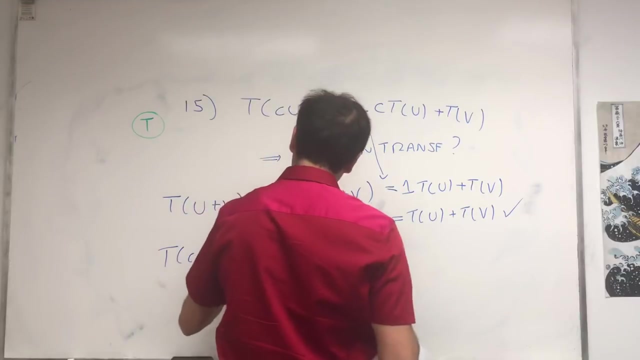 then, by the above formula, we get one t of u plus t of v, and we get t? u plus t v. So that's one thing. And the question is, what about t c? u? Well, that's t c? u plus zero. 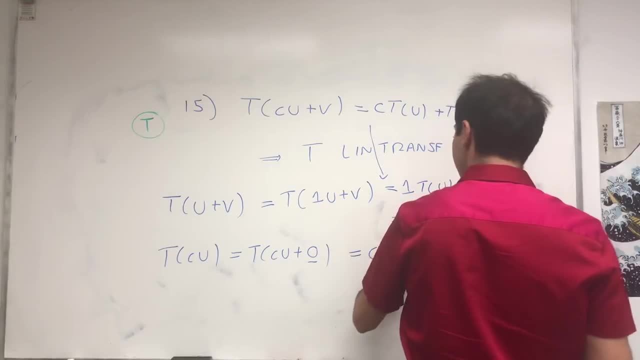 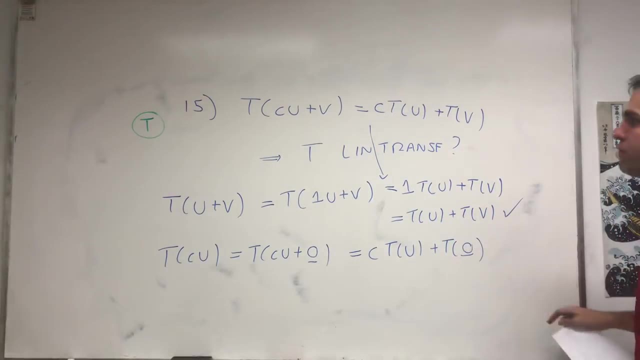 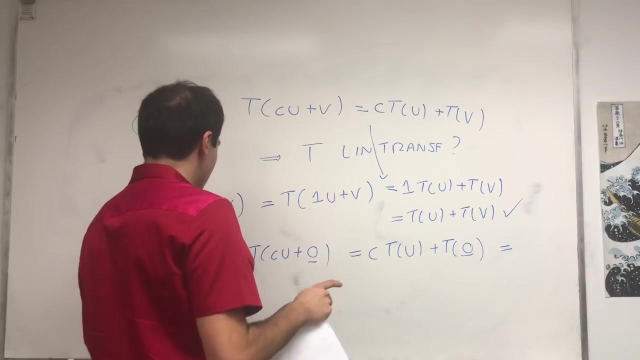 So let v be zero, Then that's c t u plus t of zero. And remember, t of zero is just zero. In fact, let me show this, because t of zero, well, that's t of zero, zero plus zero. 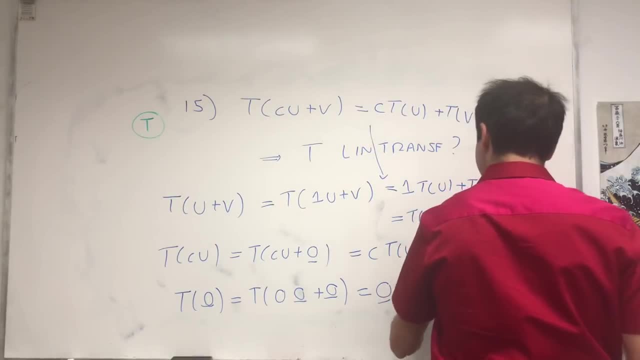 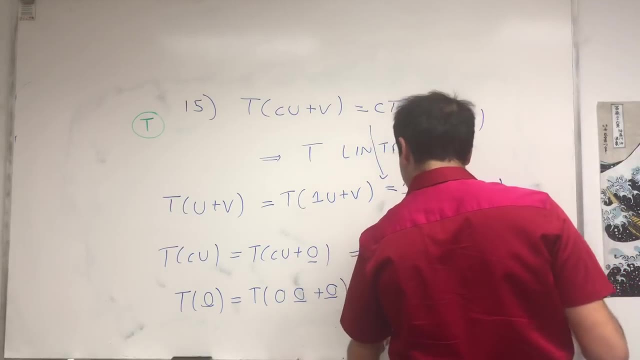 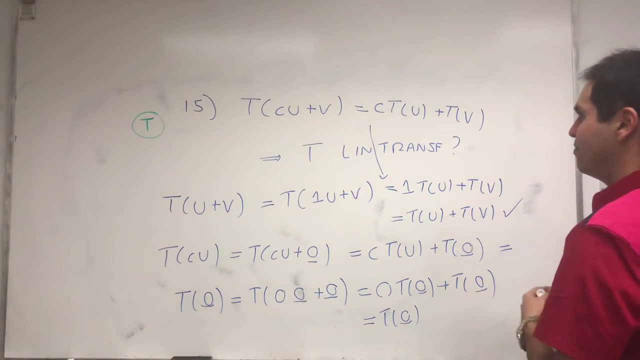 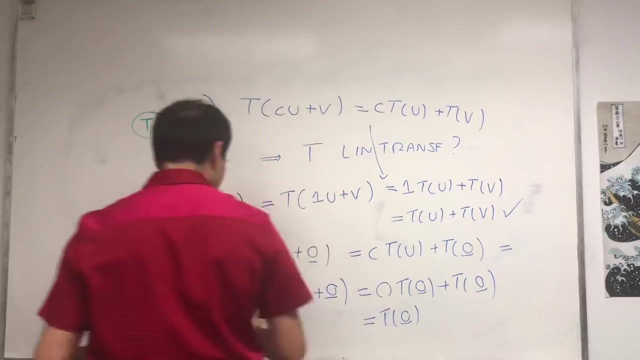 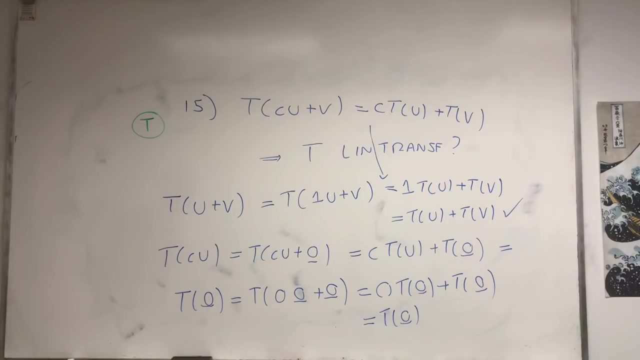 And that's zero t of zero plus zero t of zero, And that's just zero. Well, that's t of zero. One second It's all live. so I have to think about this. So could we get around this? 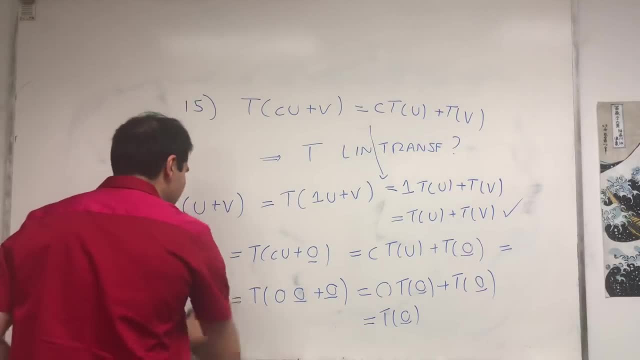 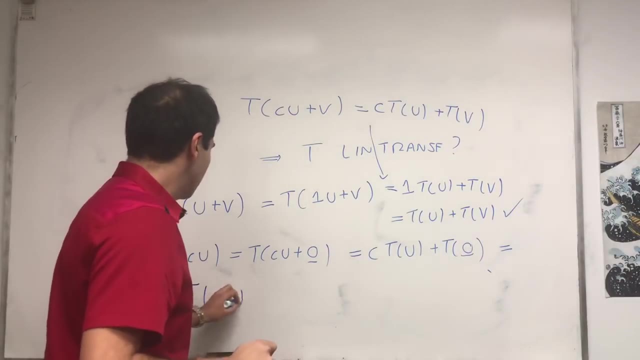 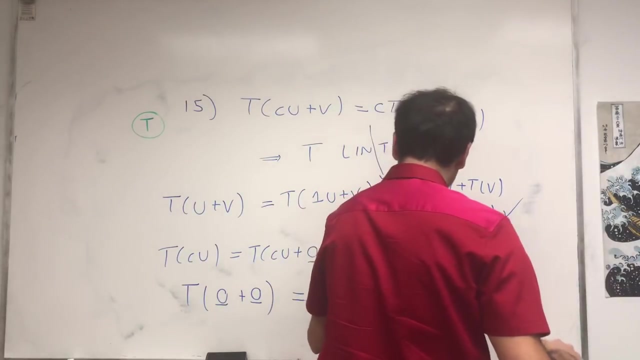 Oh, okay, I'm so sorry. Okay, I figured it out. So why is t of zero zero with this formula? So t of zero plus zero? well, we've just shown it's additive, right. So it's t of zero plus t of zero. 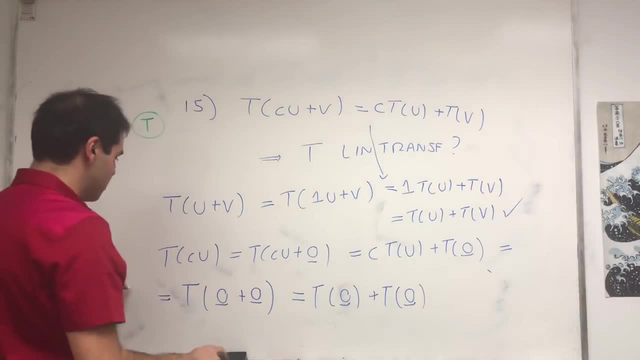 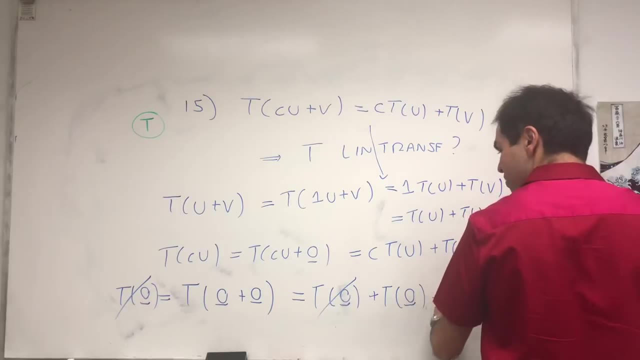 But on the other hand, zero plus zero is zero, so it's t of zero. So t of zero equals t of zero plus t of zero, which means that just the zero vector is t of zero. So in fact, this is then just a zero vector. 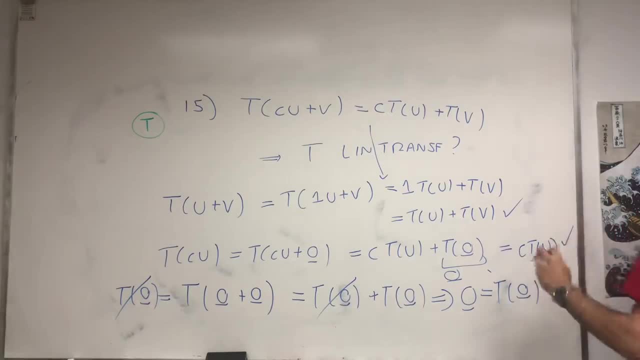 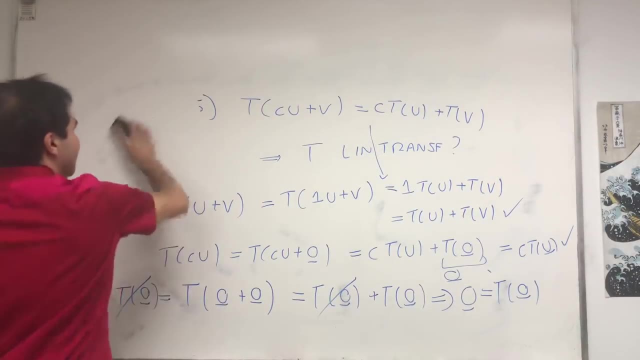 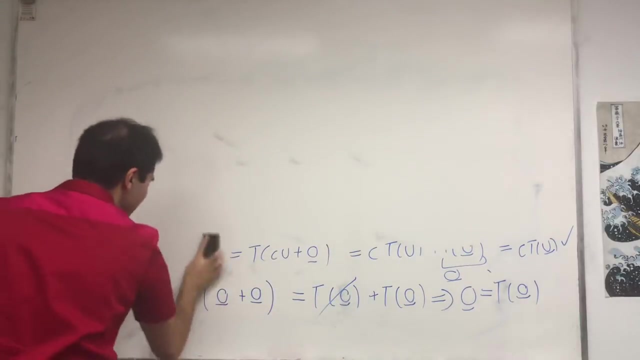 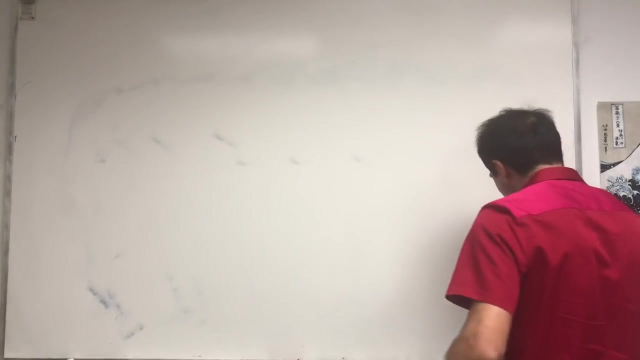 and so we get c t u Good, So that works All right. Moving on, And you'll see the uncut version of this. You now see how much I'll embarrass myself doing the videos, but that's good. I love you guys. 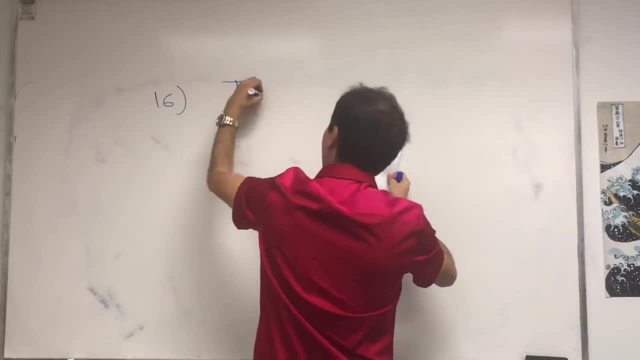 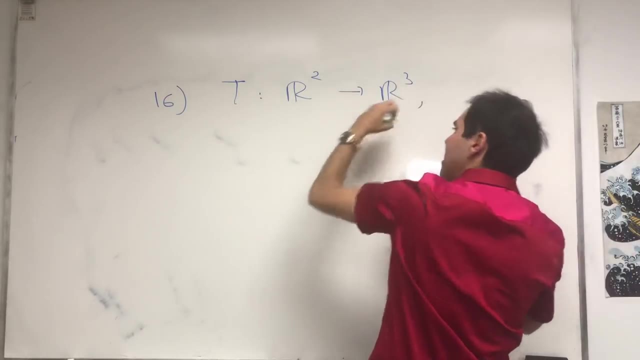 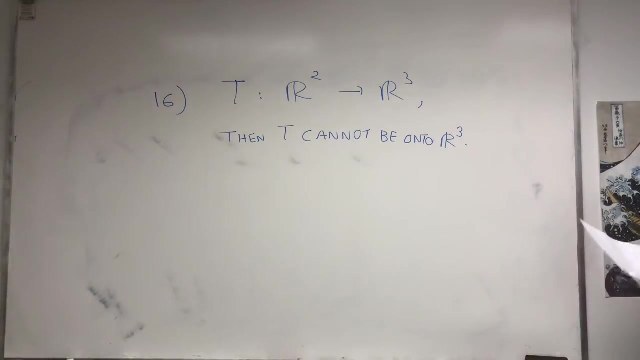 That's why. So this time now we can just assume t is a linear transformation. If t goes from R2 to R3, then t cannot be onto R3.. So it goes some quick question with one to one and onto. 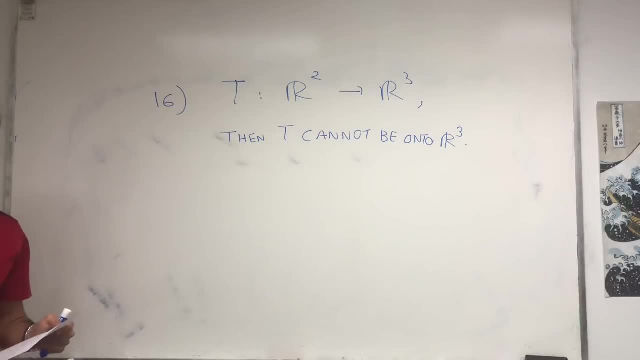 And 16th language. so it's another dialect. It's the Yue dialect of Chinese, So I think just a version of Cantonese from what I read, And 16 in that dialect it's sub-block Okay. So is there any transformation? that maps. 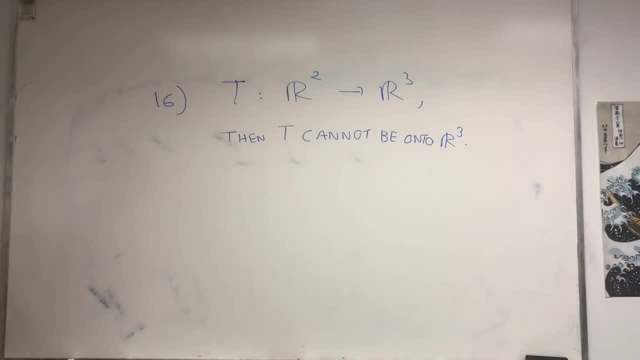 let's say the plane R2, to the whole space R3?? And remember, it's linear, So it just like flips, maybe stretches or shears. And in fact the answer is false. It's not possible And I think usually the best way. 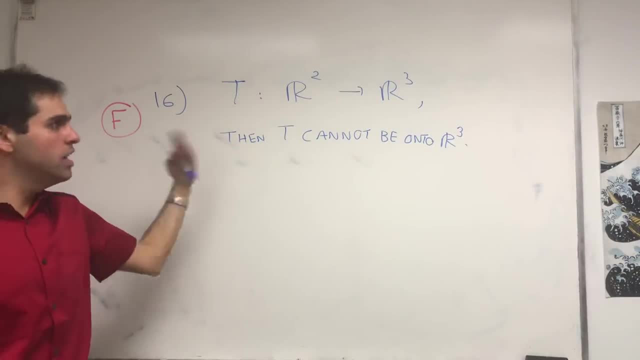 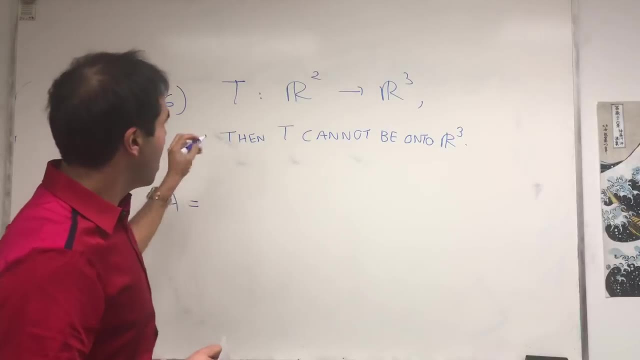 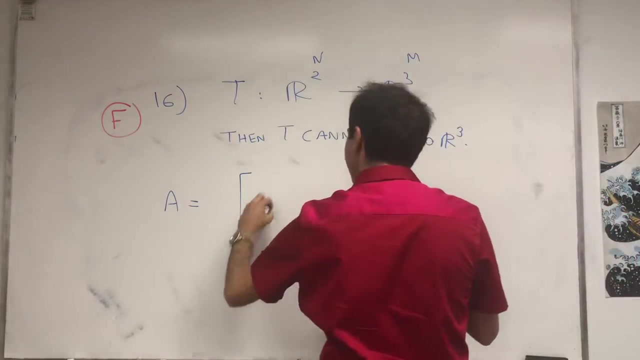 at least in elementary linear algebra. to deal with linear transformations is just consider the matrix. So let A be the matrix of t, Then A- in this case remember input and mouthput. So A would be a 3 by 2 matrix. 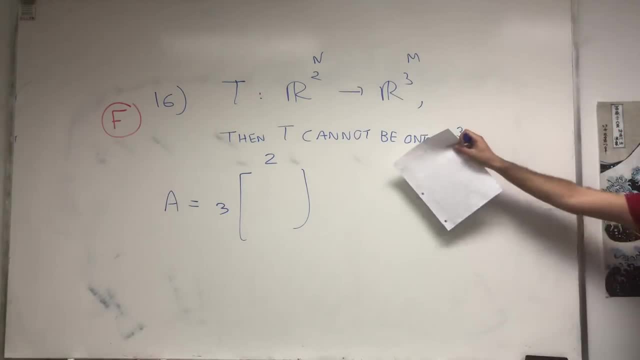 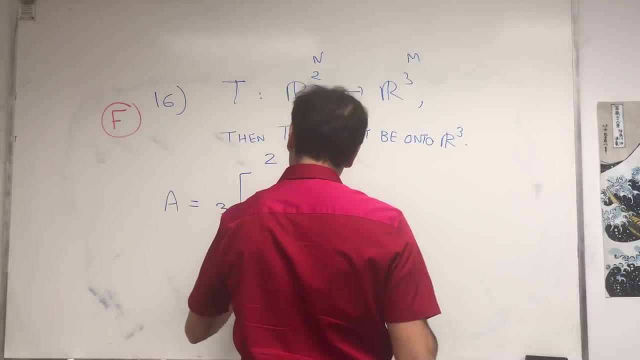 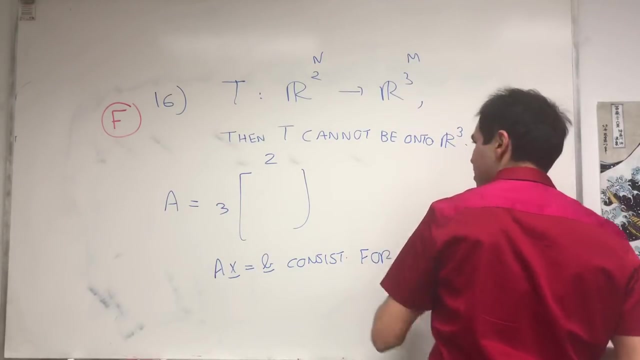 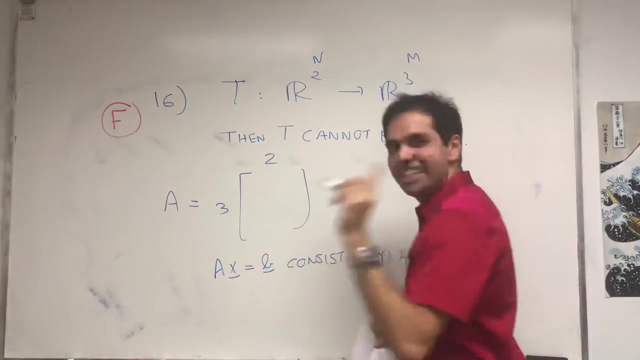 And remember, matrix-wise t is onto if and only if, Ax equals B. Ax equals B is consistent for all B. And the question is: is Ax equals B consistent for all B? No, it cannot be, No pun intended. 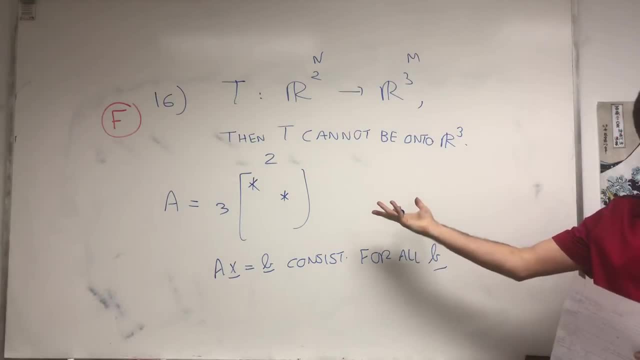 Because, look, such a matrix can only have two pivots at most. That's why the last row has to be a row of zeros, So you can actually choose some B, such that you have a row of the form zero, zero, star. 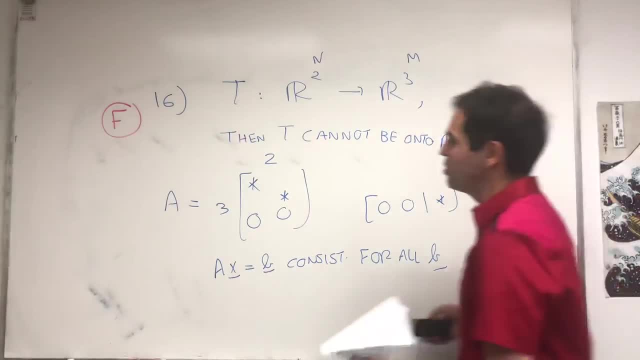 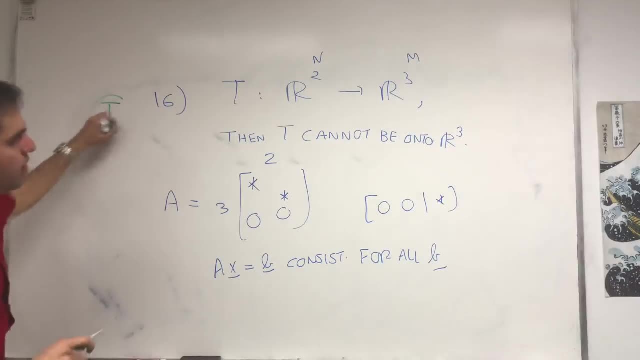 And I realize I don't know why I put false. It is indeed true. My bad, I misread it with. it- can be onto. Yeah, it's true that it cannot be onto. So this linear transformation, therefore. 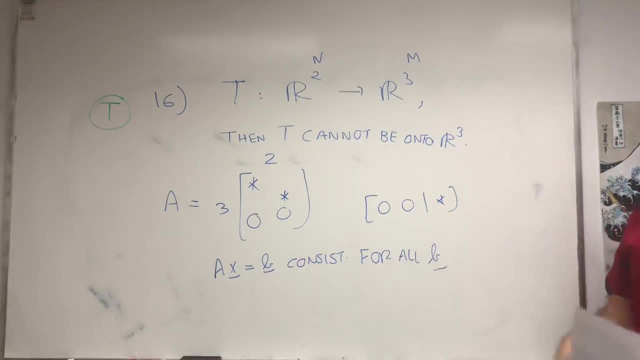 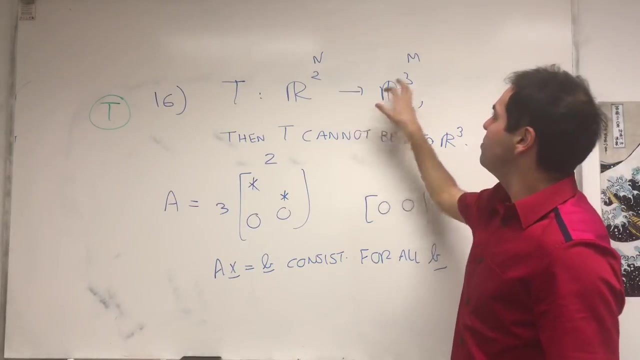 cannot be onto because Ax equals to B isn't consistent for every B, And there are, of course, other ways to deal with this. For example, you see, R3 is a three-dimensional space. If it were onto, it means this dimension is smaller than this one. 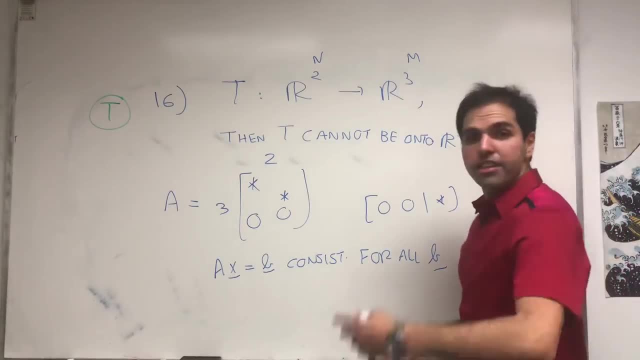 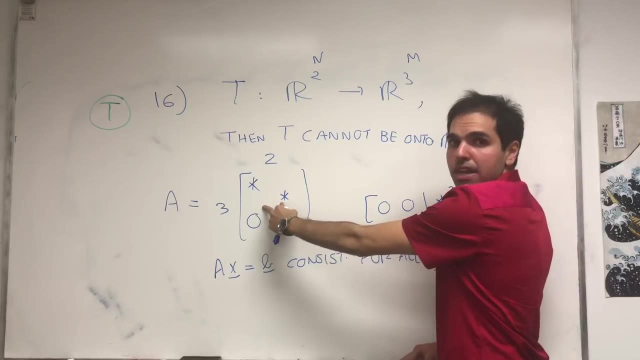 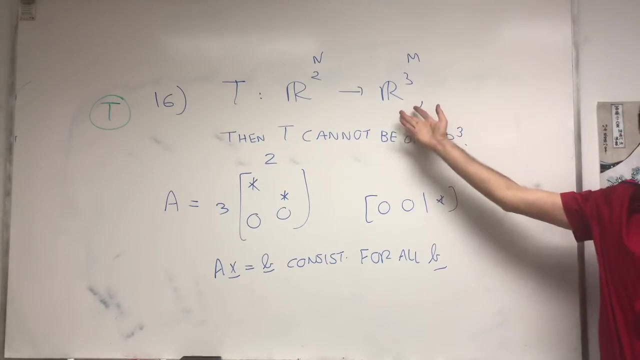 which is bogus, Or you can deal with it with column spaces right Here. the column space has at most two basis vectors, So it's at most two-dimensional. But if it were onto, then the column space would be R3, which is not. 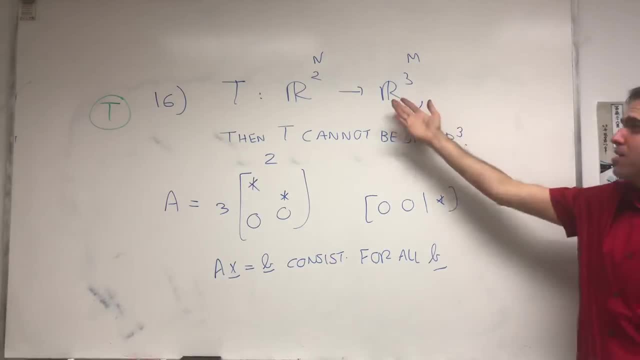 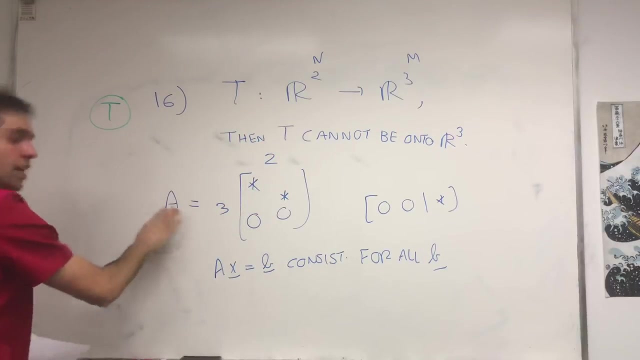 which is three-dimensional, So otherwise it's impossible to express R3 in terms of just two vectors. So different ways of dealing with this, But what I wanted to show is usually those problems with onto one and onto you can deal with by using the matrix. 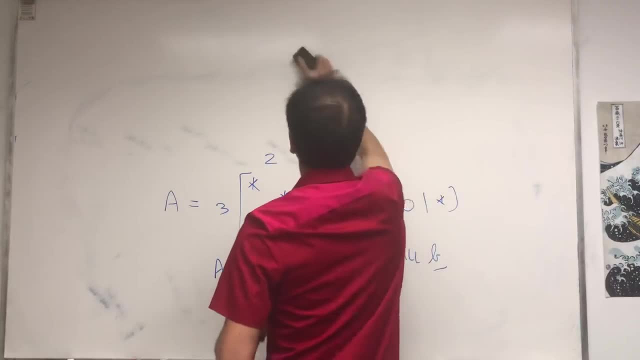 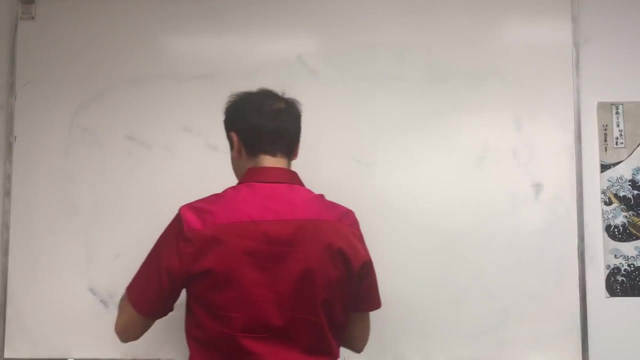 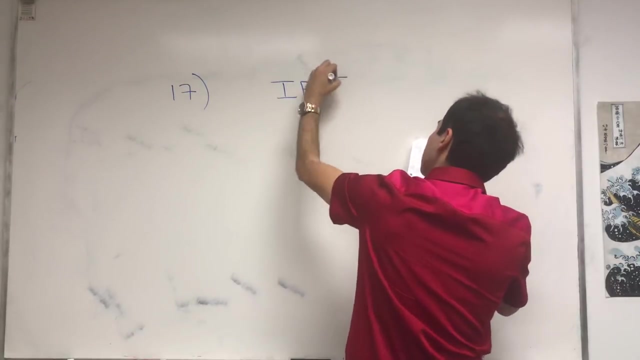 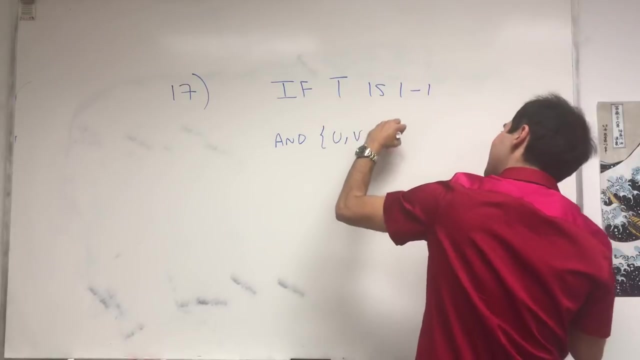 Question 17.. And remember, we're still in part one, But this is the last question of part one. So another one-to-one thing, another linear transformation thing. If T is one-to-one and uvw linearly independent, 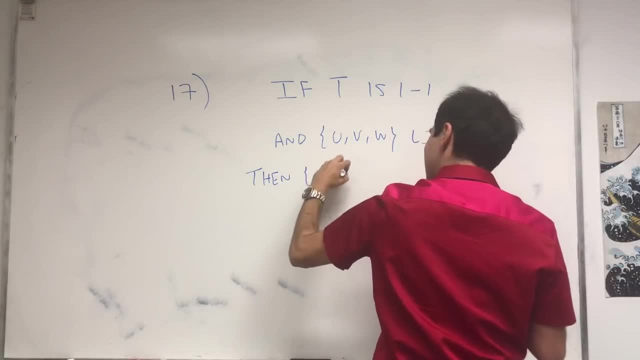 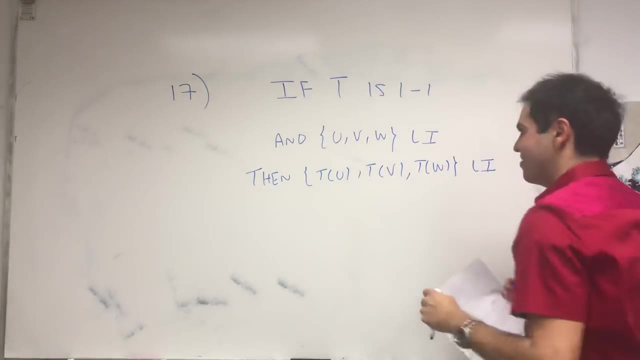 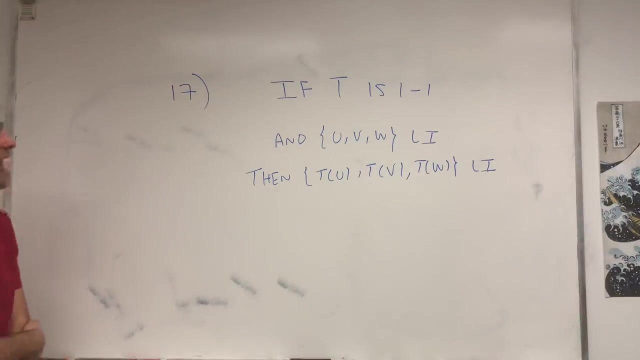 then Tu, Tb, Tw is linearly independent. That's actually one of my favorite math questions, So my students beware, okay. And by the way, that's not quite the same question as before. Basically, the other question with linear dependence. 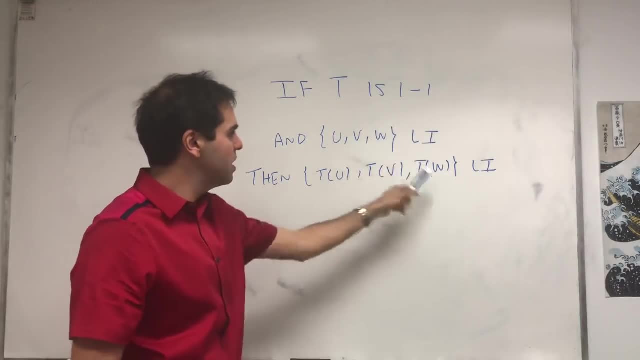 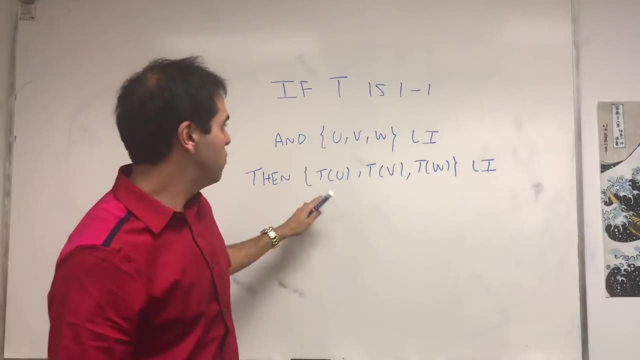 well, it said, if this is linearly dependent, then this is linearly dependent, which is always true. But here we kind of have the opposite. If, basically, this is linearly dependent, is it true that this is linearly dependent? 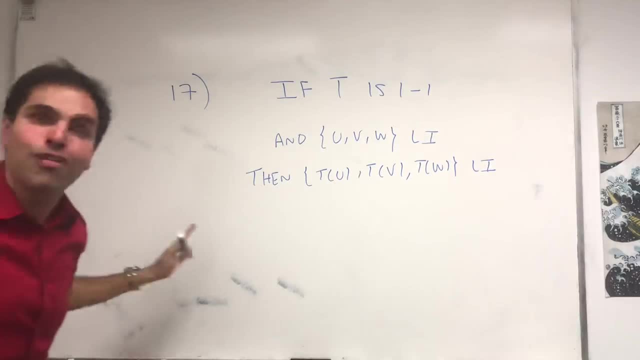 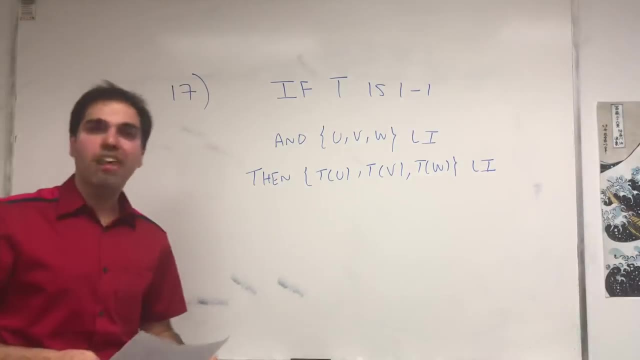 Well, just if it's one-to-one, Or or maybe not, Maybe it's a false question, I don't know, But anyway. so 17th most popular language, Marathi, And 17 in Marathi is: 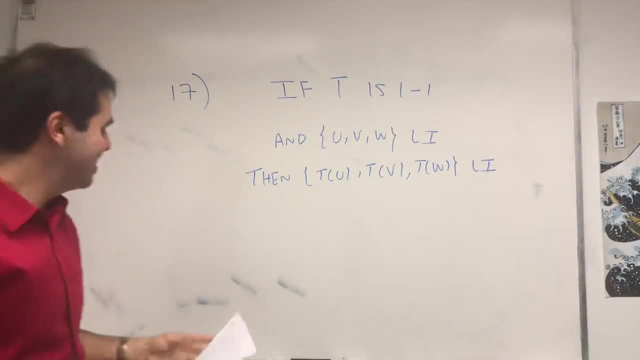 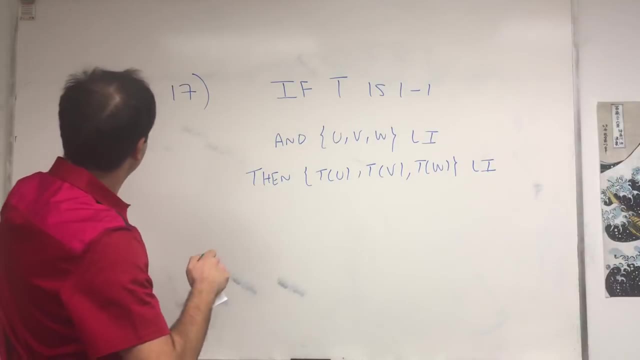 cetera, Like et cetera. Okay, All right, then I'm going to scoot this over. And it is true. Why? Because to show this is linearly independent. we want to show that if 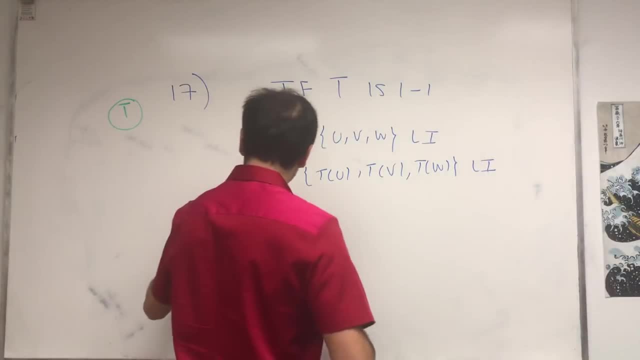 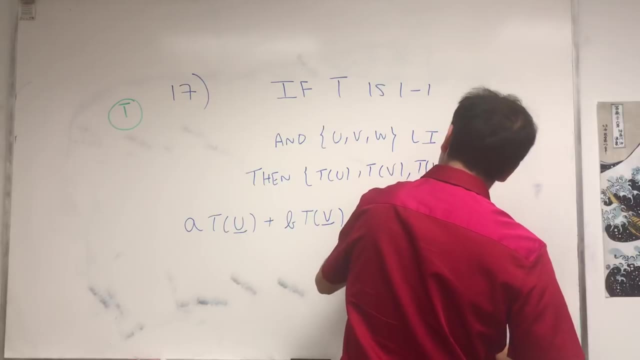 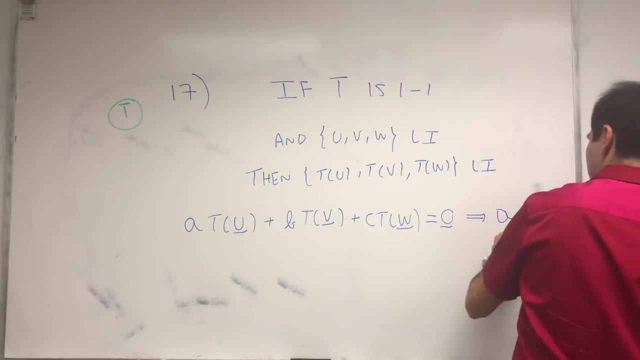 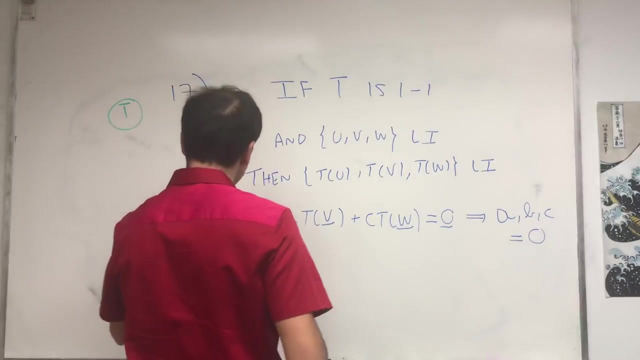 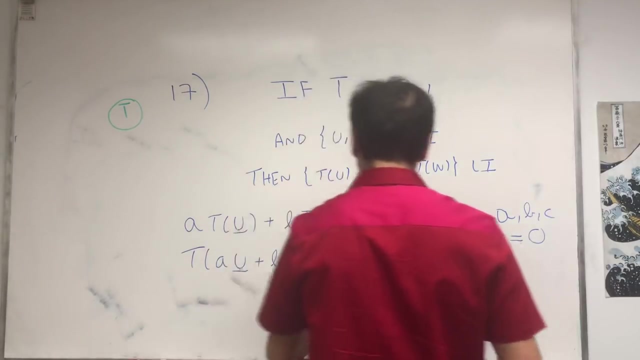 a, t? u plus b, t, v plus c, t w is the zero vector, then a, b and c are zero. Okay, But it's a linear transformation, Because you can write this as a, t, a, u plus b? v. 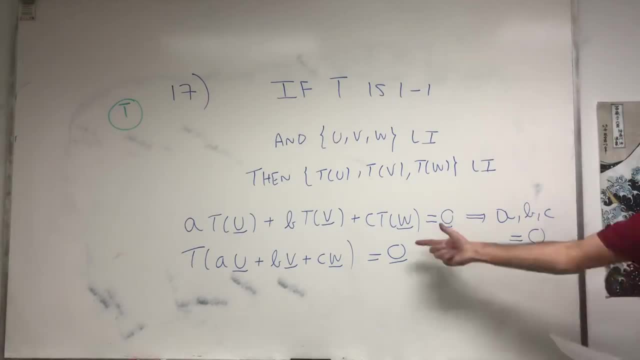 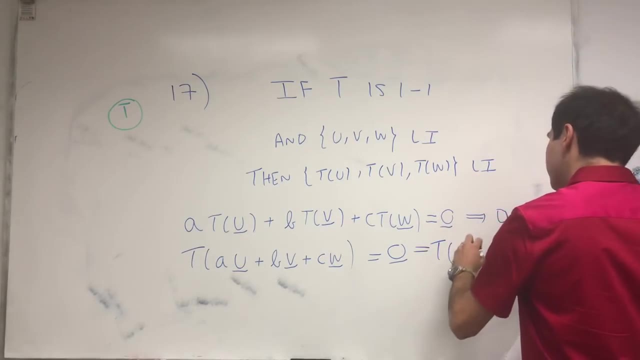 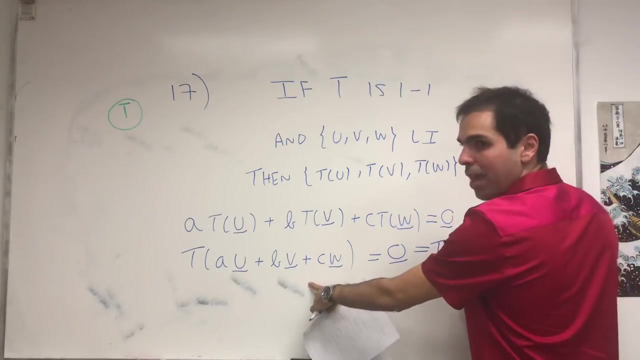 plus c, w equals to zero And in general this doesn't imply that this is zero, But because it's one-to-one it is true, Because, look, zero is t of zero, But one-to-one really means. 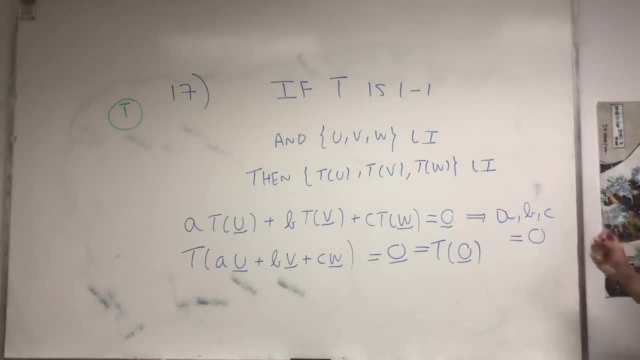 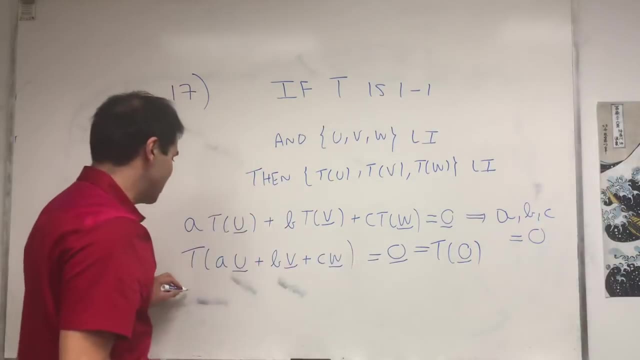 if two things have the same output, they must have the same input. In other words, it's almost like just cancelling out t from this equation. So let me do something a bit illegal. So let's cancel out t And we get. 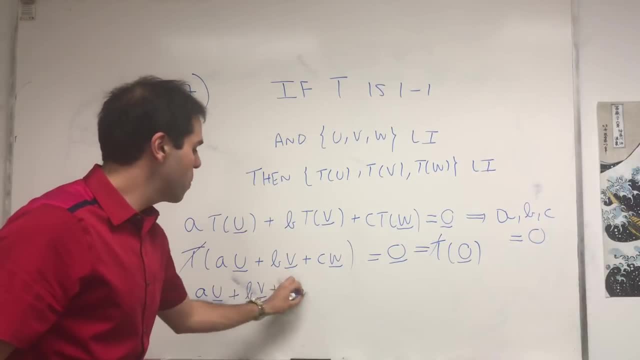 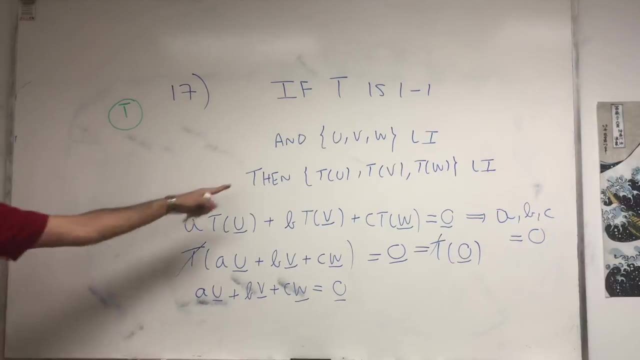 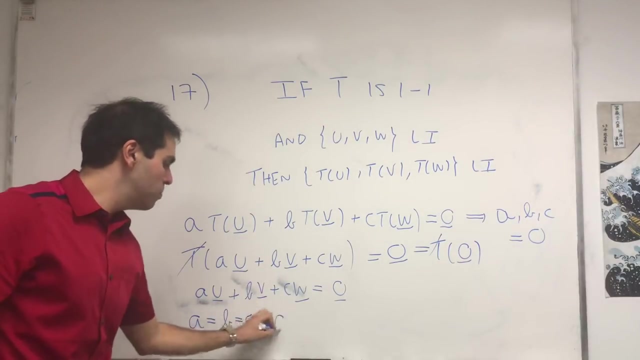 a, u plus b, v plus c, w equals to the zero vector. And again, here we needed the fact that it's one-to-one. Now, because this is linearly independent, we indeed get a and b, and c are zero, which is: 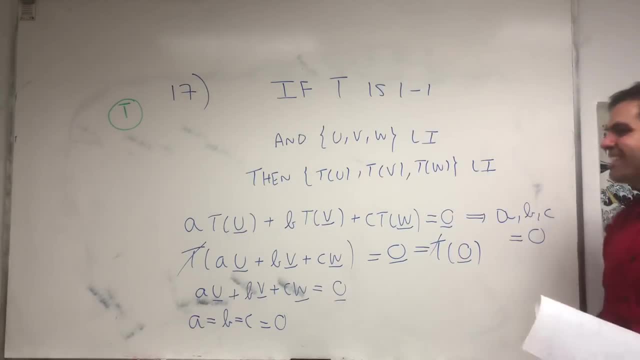 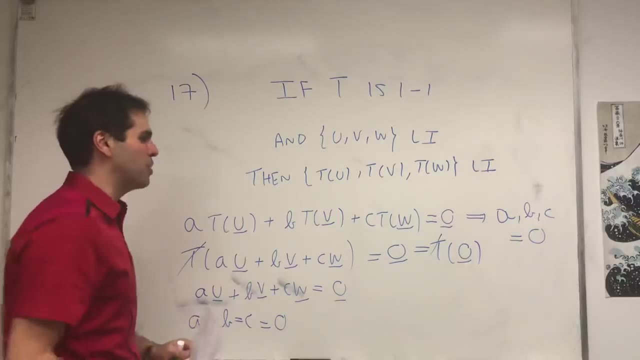 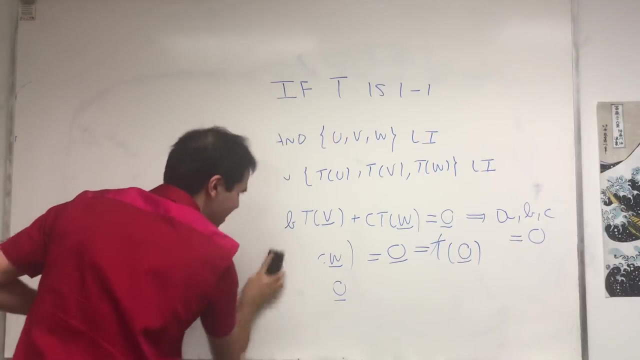 just like we wanted to show. So a very cute linear algebra cookie, if you want, Or maybe I should say a linear algebra Oreo, because of Oreo Great And ta-da. One hour down, almost, and we're done with the first part. 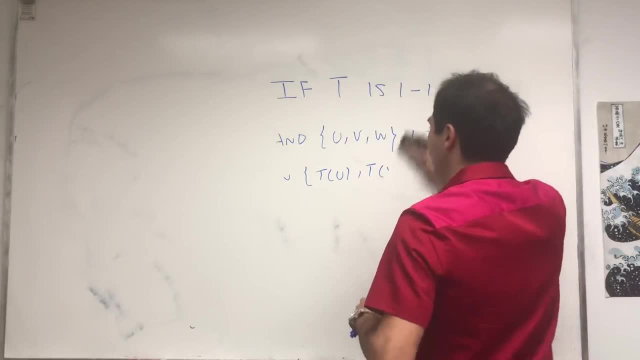 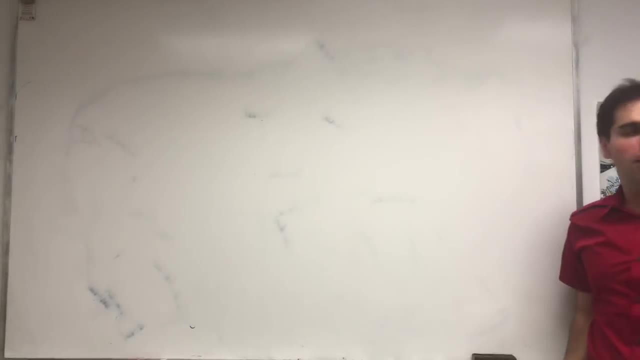 So there are seven parts. So now, hopefully you enjoyed this linear equations part. You know, of course it has to do with what's called pivots and, um, sorry, pivots and one-to-one and linear independence. 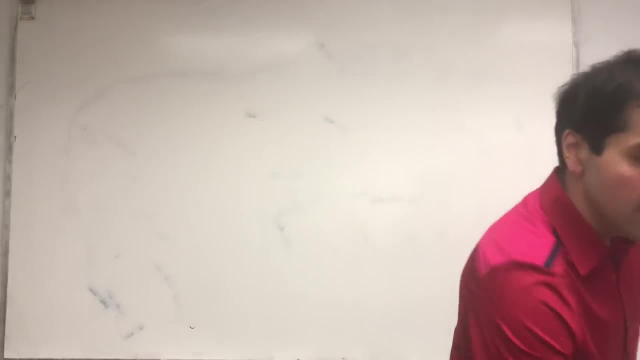 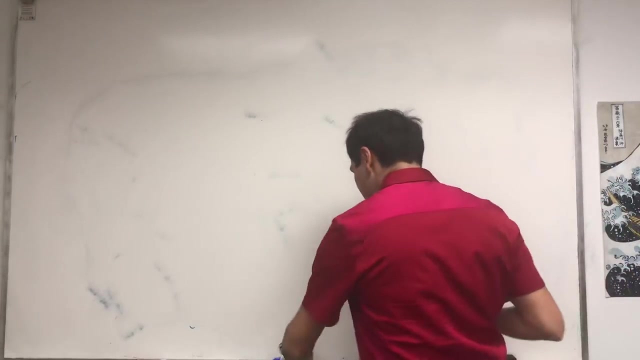 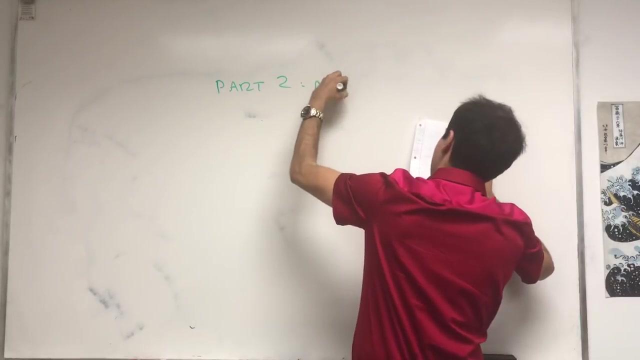 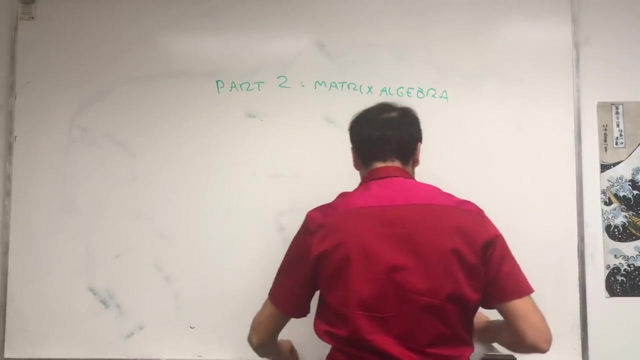 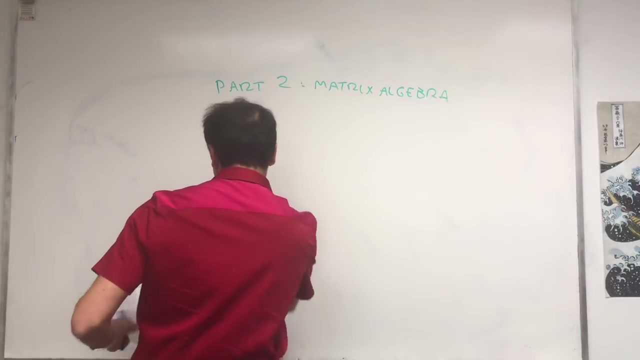 Now let's talk more about matrices. So part two is matrix algebra. So this is the matrix algebra. So this is the matrix algebra. So it's a matrix for a matrix and a matrix is a matrix for a matrix. 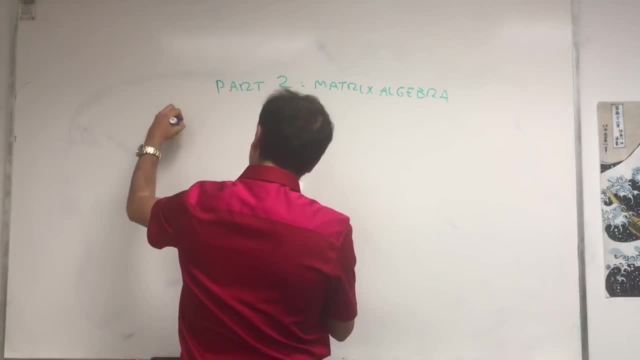 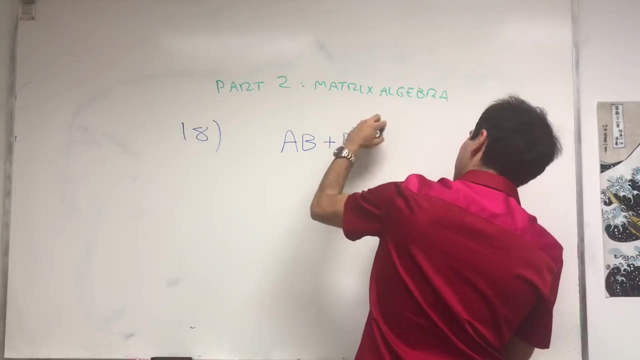 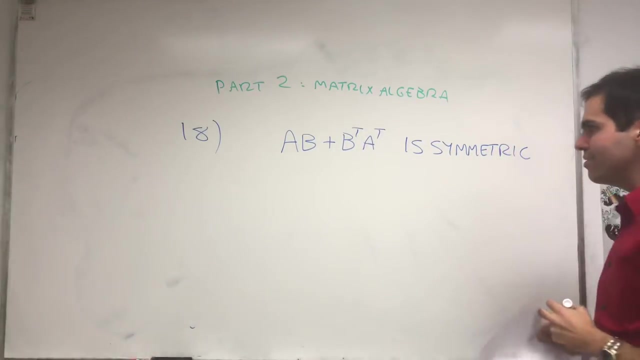 of a, b, b plus b plus 8 plus 8 plus. Is it symmetric? Is it always a symmetric matrix? I had that question actually in my undergrad, so back in 2006,. I had that question on the midterm. Is it true or not? 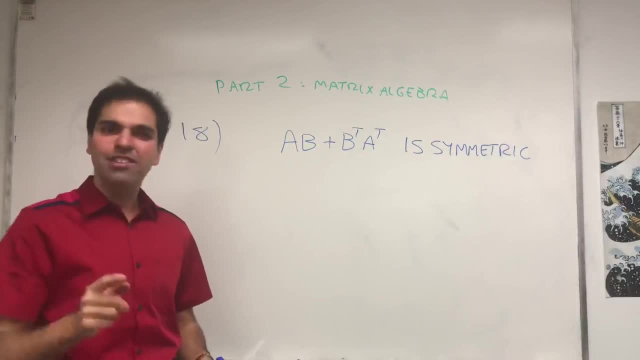 And remember this Padihenu I was talking about. Well, 18 is Tamil and 18 in Tamil is Padinedu. Isn't that awesome? In Telugu it's Padihenu, In Tamil it's Padinedu. 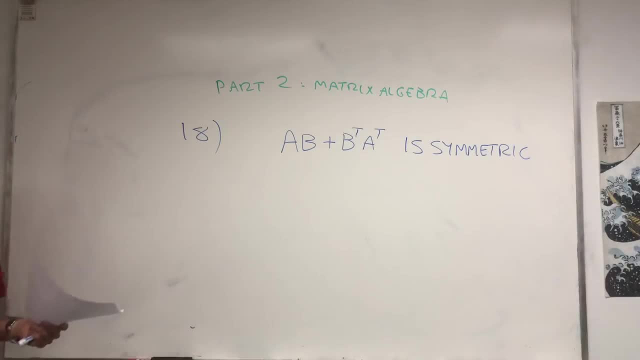 Very similar, But again, unfortunately, I don't really know where those languages come from. So, that said, this weird expression, it turns out it's always symmetric and the best way of checking symmetry is just check if this equals to its transpose. 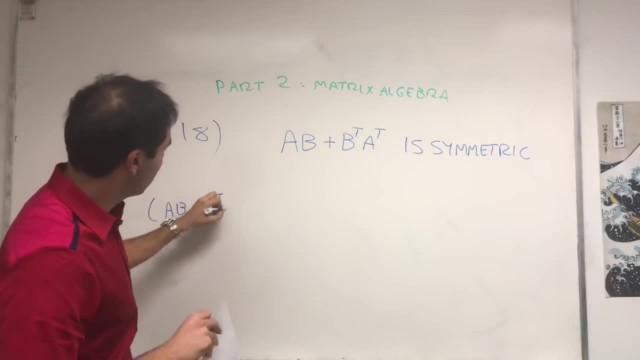 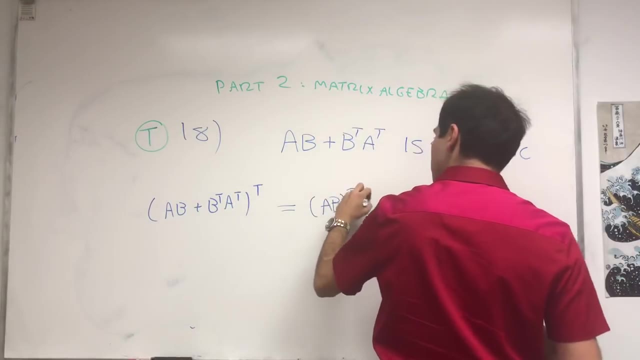 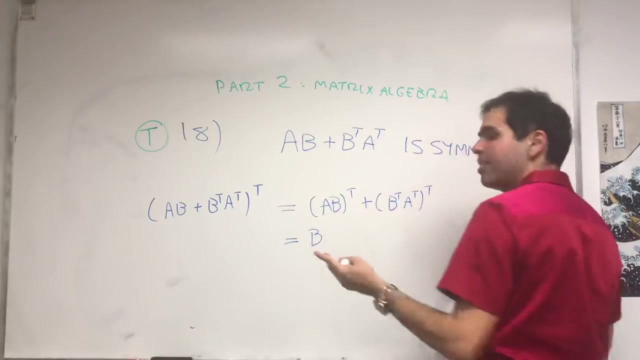 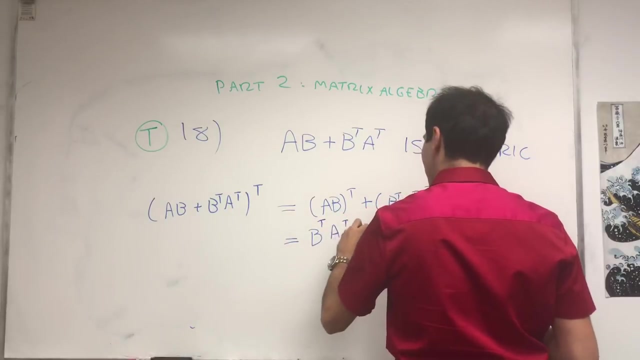 So let's calculate AB plus B transpose, A transpose, transpose. Now the transpose is linear, so it's AB transpose plus B transpose, A transpose, transpose. And here's an important thing For transposes, you flip the tail, So AB transpose is B transpose, A transpose. 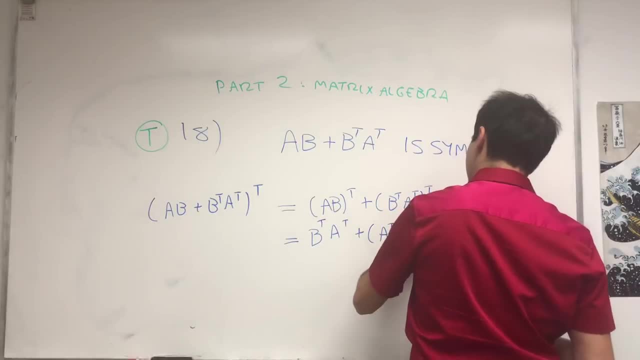 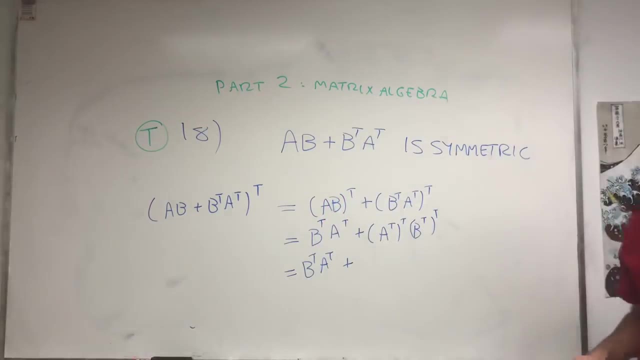 and here: A transpose, transpose, B transpose, transpose, and that's B transpose, A transpose, Now transpose, transpose is like itself. It's almost like inverses, In fact. in terms of dual spaces it is a sort of an inverse. And notice, that's the same thing as 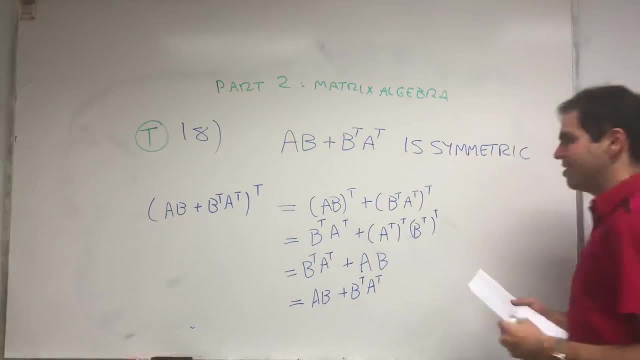 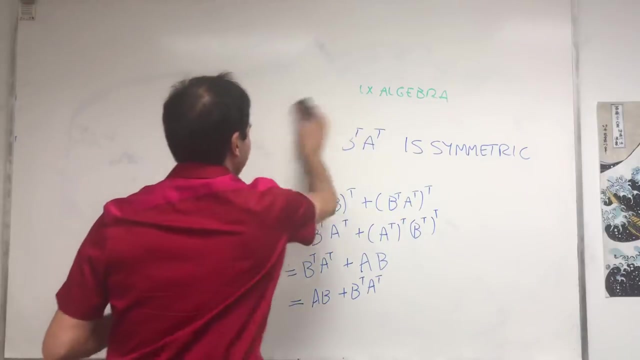 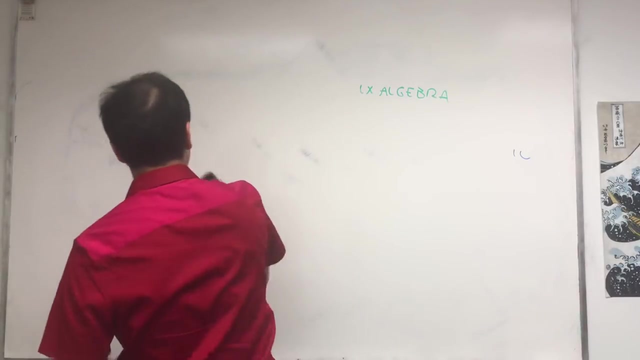 AB plus B. transpose, A transpose. How cool is that? So if you take the transpose of this matrix, you actually get the matrix itself, And therefore it's symmetric. Cool, A very good question, In fact. let's do a little bit more. 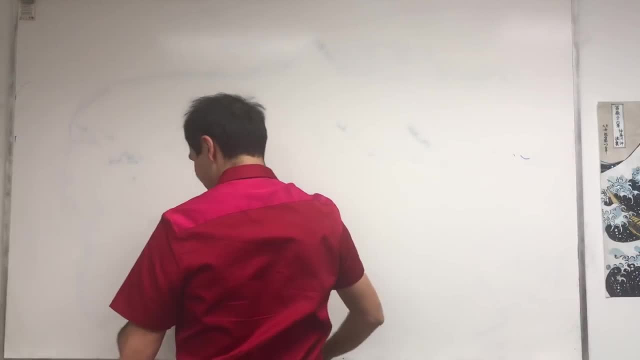 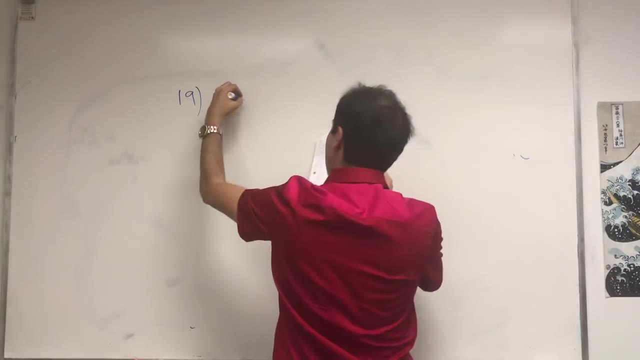 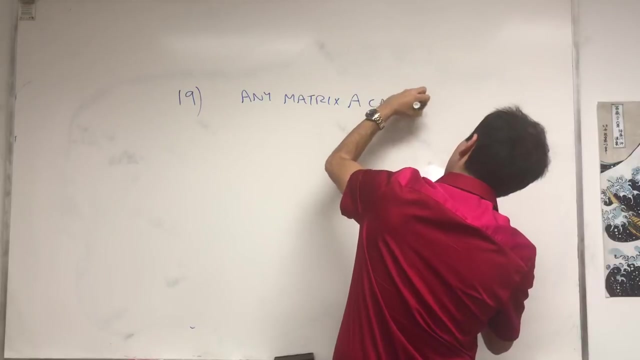 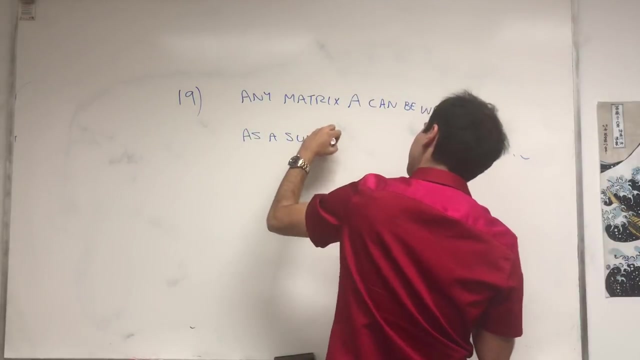 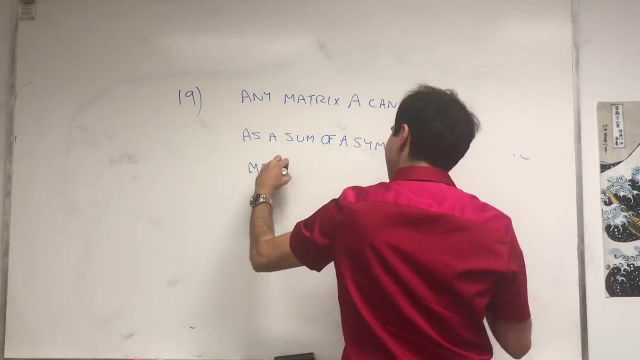 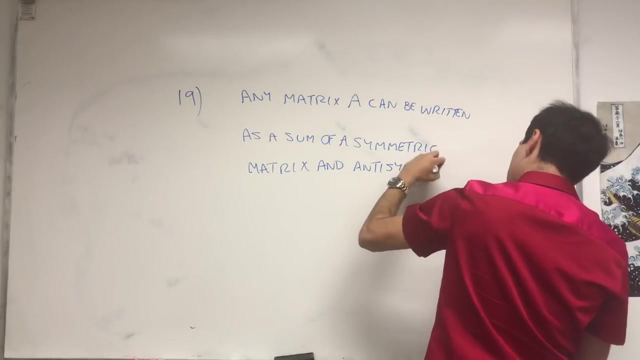 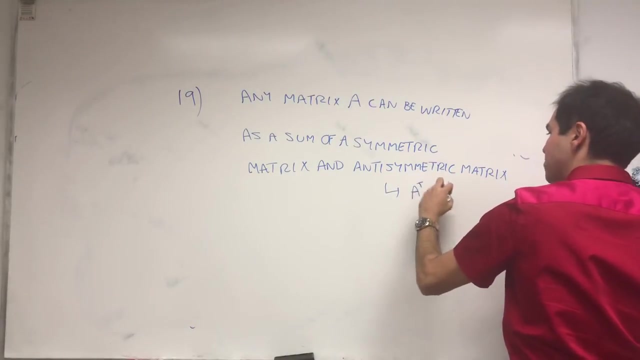 about symmetric matrices. So question 19 is a very surprising fact. if it's true, Any matrix A can be written as a sum of a symmetric matrix matrix and an anti-symmetric matrix. Anti-symmetric just means A transpose is minus A. 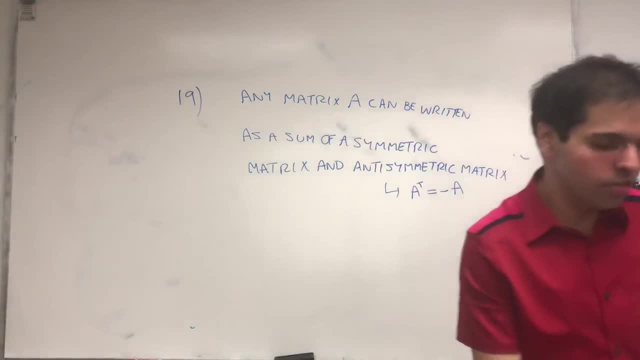 Very surprising fact, and no one talks about this. The question is: is this true or not? Why do people not talk more about this? And it's a problem. I'm already thirsty. It's only question 19, and like I don't know, 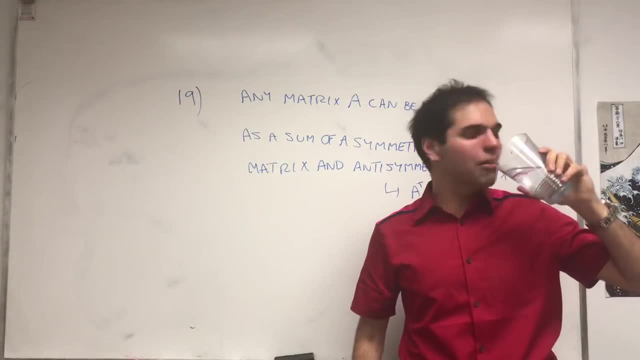 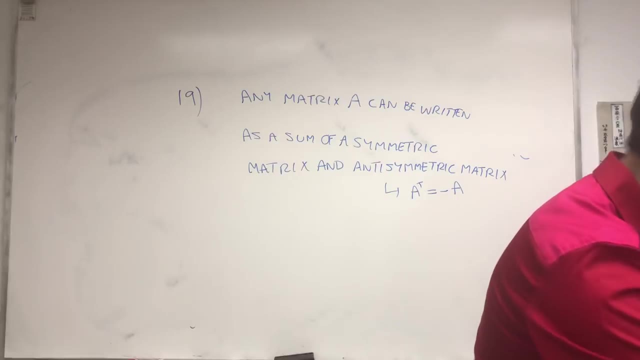 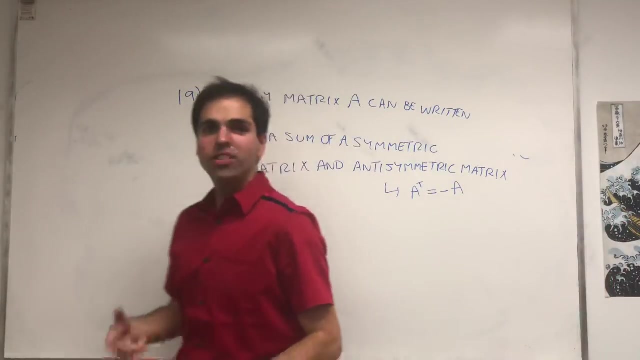 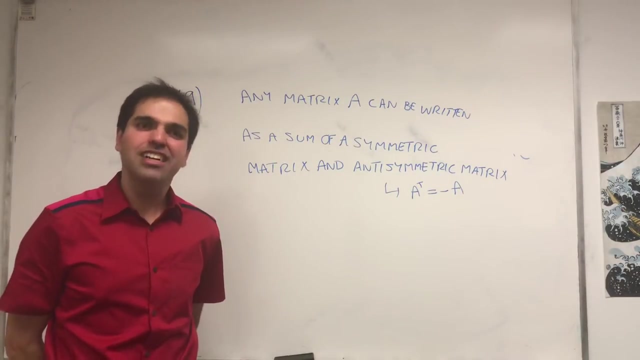 I hope I don't need to go to the bathroom in the next four hours. Okay, And 19,. the most popular language, Turkish, And 19 is, By the way. so my family, so my parents, they always speak Turkish because it's your secret language. 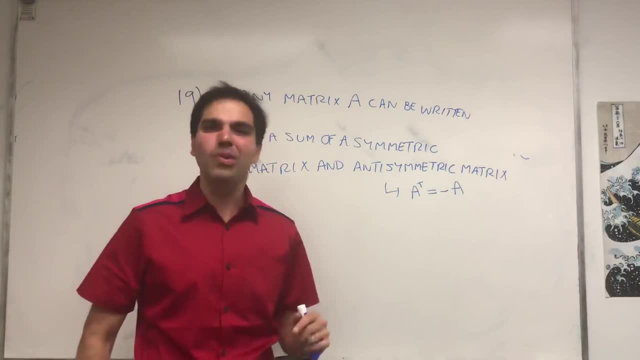 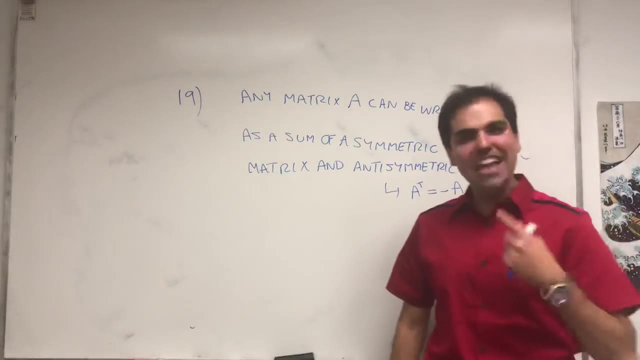 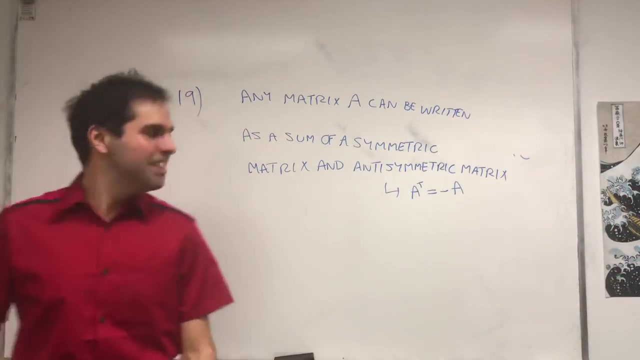 They know I don't speak it, but then I started learning it a bit with Duolingo and now they're like in danger. That's all what I know, Or Ben, I think. So I never get hungry or thirsty in Turkish. 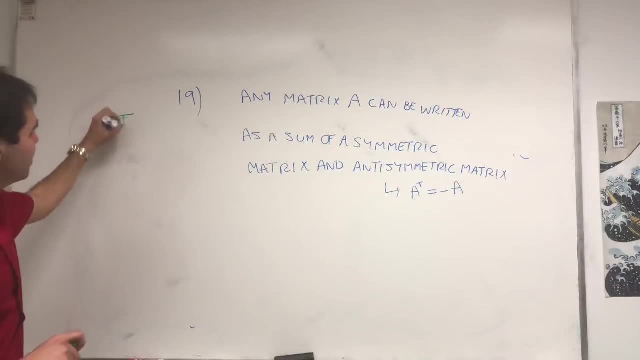 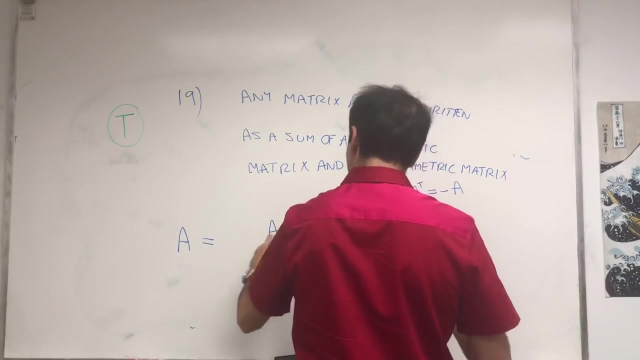 And so this question: surprisingly, it's true, Can you believe it? So it's. I like to call a symmetric matrix decomposition. because here's a decomposition. It turns out A. you can write as A plus A transpose over 2 plus A minus A transpose. 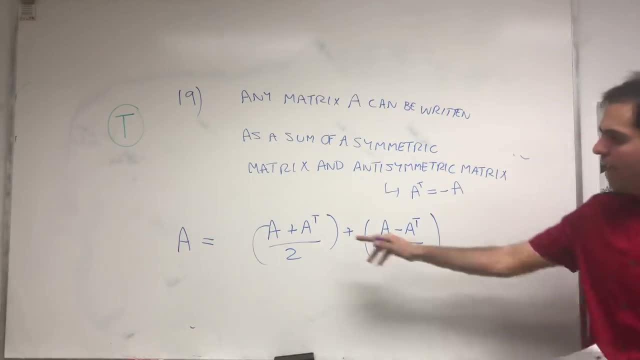 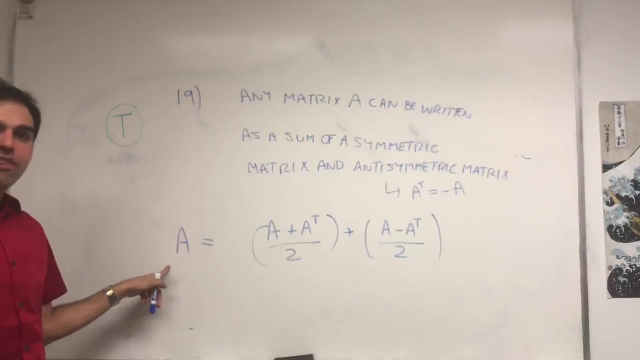 over 2. Because the A transposes cancel out and one half A plus one half A is A, And I don't know if that reminds you of something, but it should. It turns out it's the same decomposition as the fact that any function. 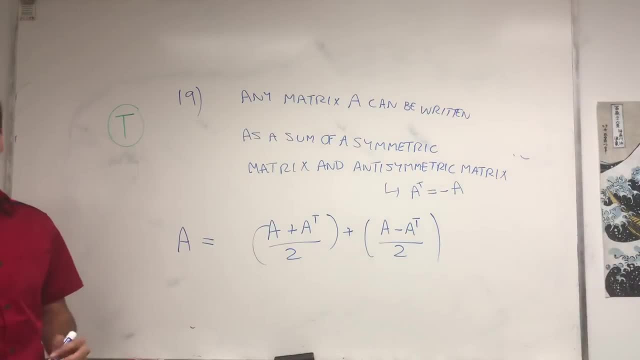 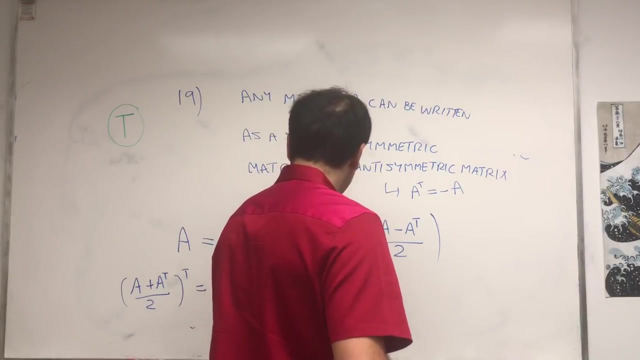 can be written as the sum of an even function and an odd function. And, by the way, why is this symmetric? So A plus A transpose over 2 transpose, that's again one half A transpose plus A transpose transpose, and that's one half A transpose plus A. 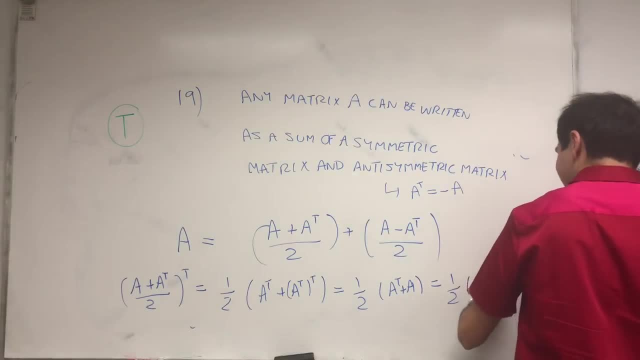 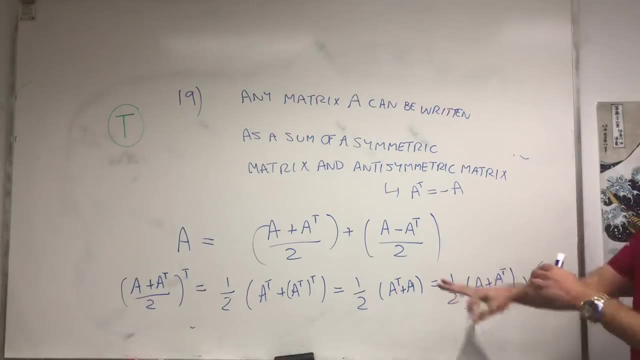 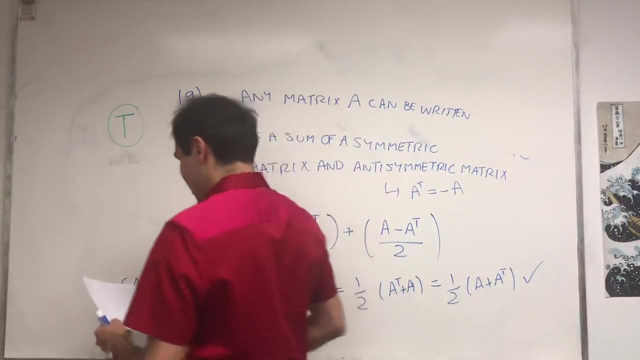 which is the same as one half A plus A transpose. So this is symmetric and similarly you can check, this is anti-symmetric, So any matrix can be written in this form. I have no idea what this would be useful, but this is very cute. 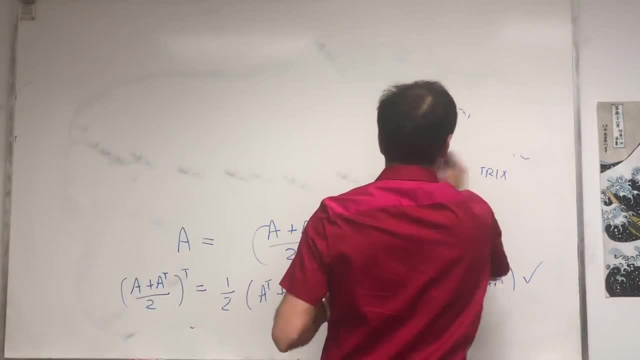 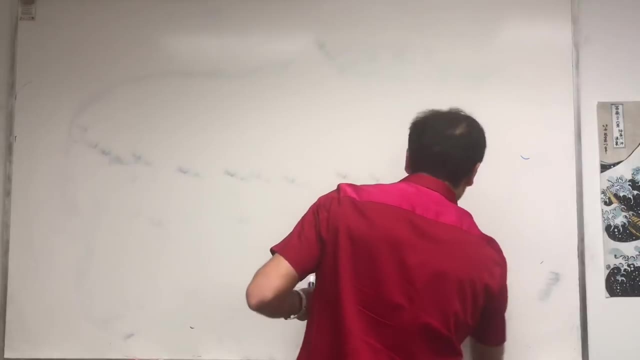 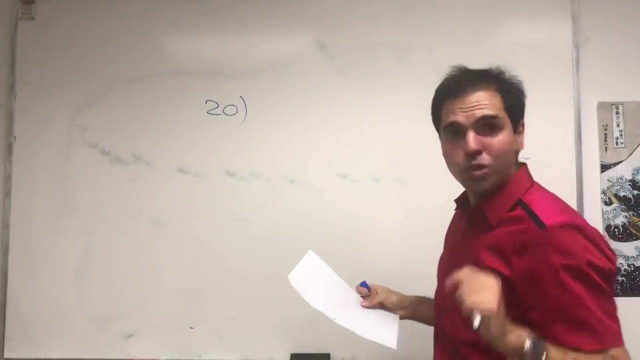 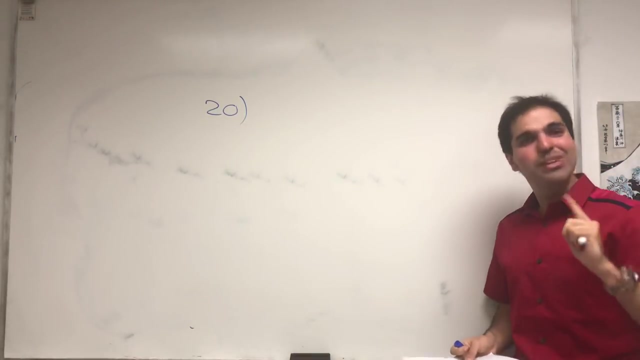 Next one. The next two are very quick actually. This is sort of my sprint part of the marathon. So question 20.. And 20, so Urdu, 20th most popular language and 20 Urdu. is this, which is really cool? 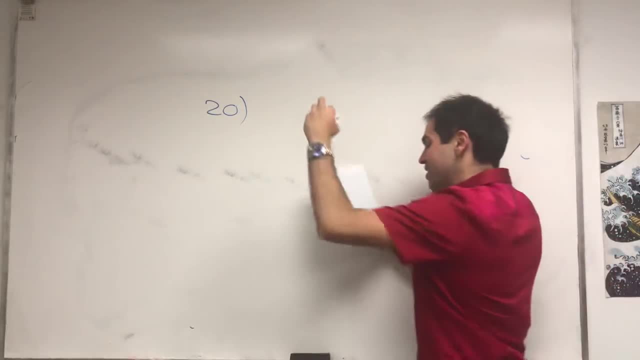 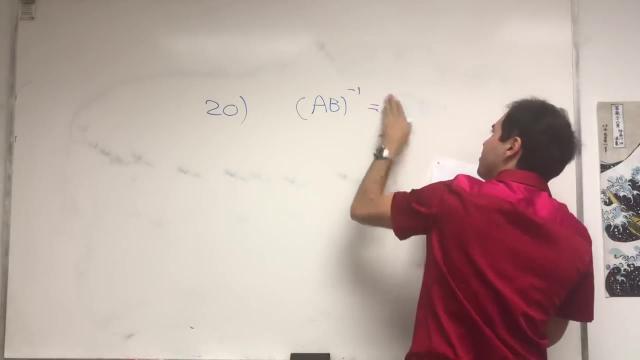 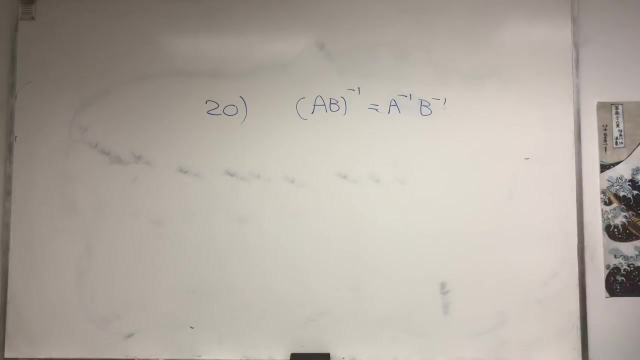 because in Farsi it's beast, So it's very similar. And the question is: is AB inverse equal to B inverse, A inverse, Ah, no, the other one, A inverse, B inverse. So how do I do this? Matrix inverse is like a homomorphism. 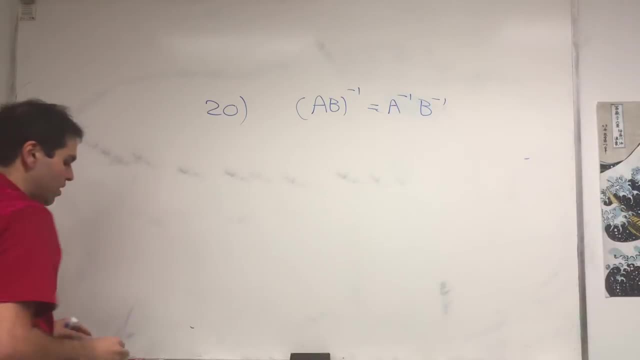 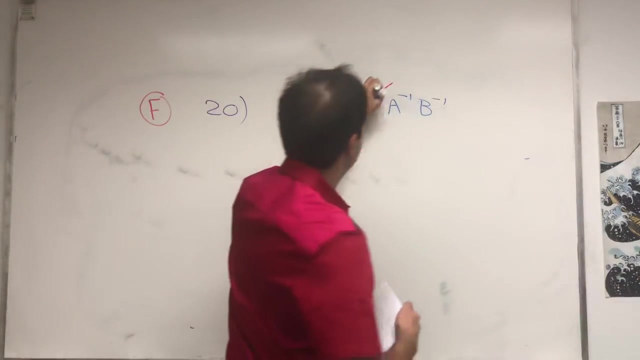 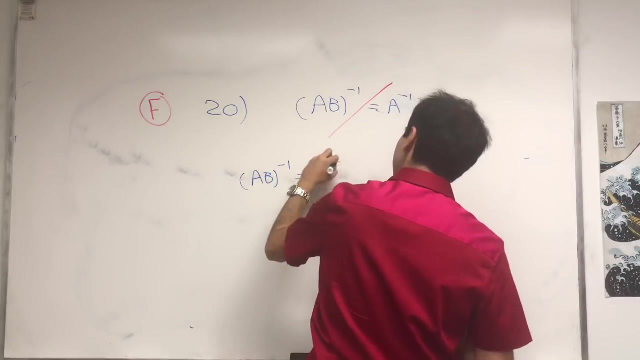 I think that's what they call it, And it turns out. no, because it turns out, you have to do it in the other order And in fact that's how I wrote it at the beginning. AB inverse is actually B inverse, A inverse. 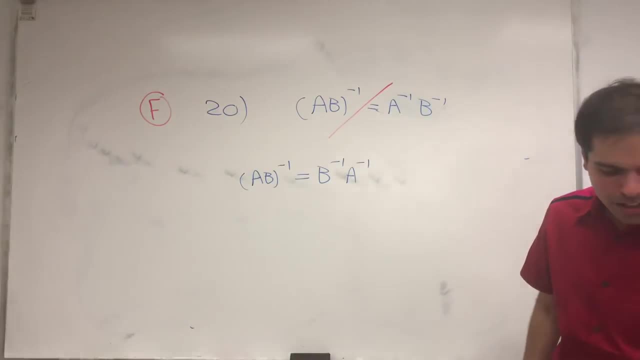 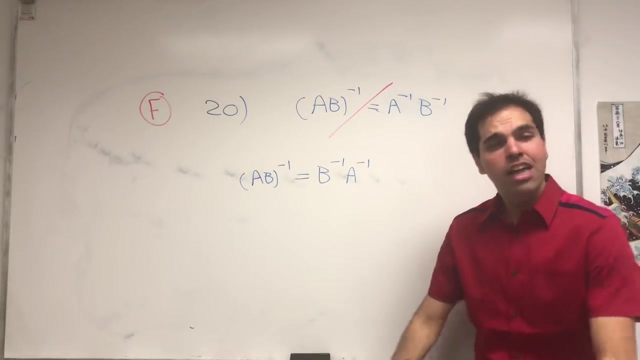 And think about this. I gave this analogy at one point, but in another video. but think of AB as putting your sock on and then putting your shoe on. How do you undo this? Well, first you take your shoe off and then your sock off. 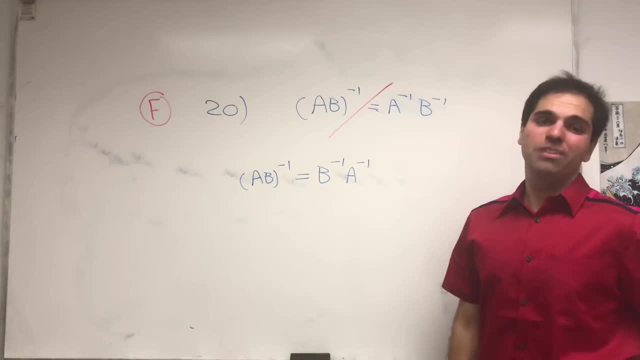 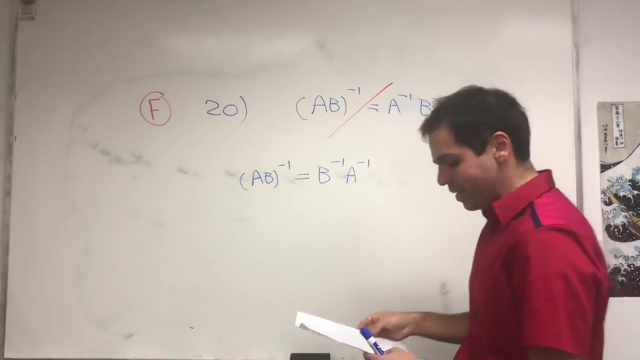 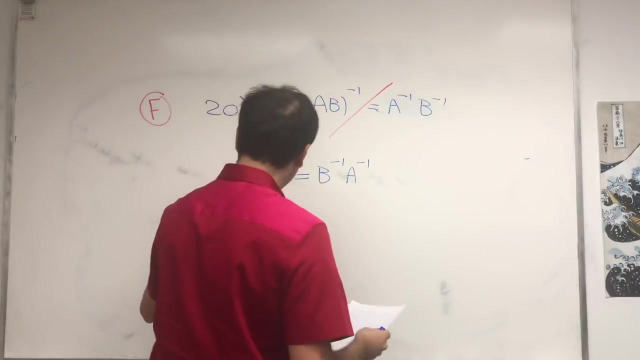 So it's the opposite order really. That's why we have that, And just like transposes AB transpose is B transpose A transpose. Okay, and question 21,, still on the same whiteboard. Is it true if AB equals AC? 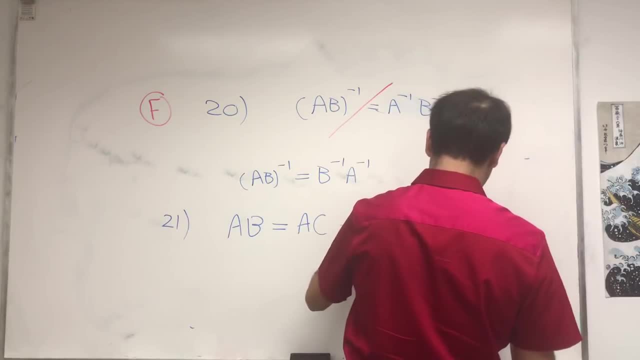 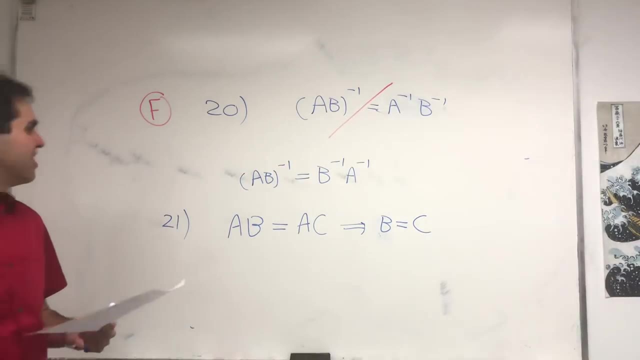 then A, then B equals C And language 21,. a Taiwanese and I love Taiwan. I had such a good time there last year- And Taiwan 21 is li zap it. It's almost like zap it or something. So in other words, 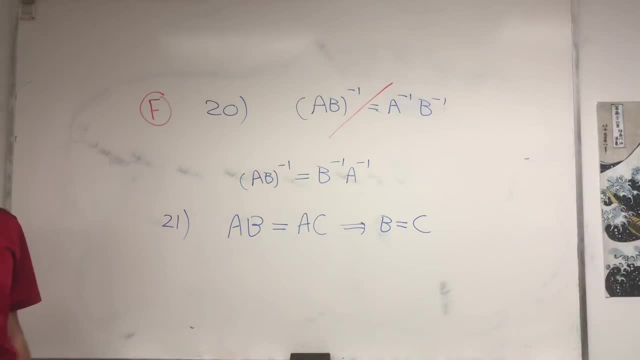 does the cancellation law hold for matrices, even if it's non-zero? Well, it turns out it doesn't hold in general. Let me give you an example. For example, this thing: 1, 0, 0, 0,. 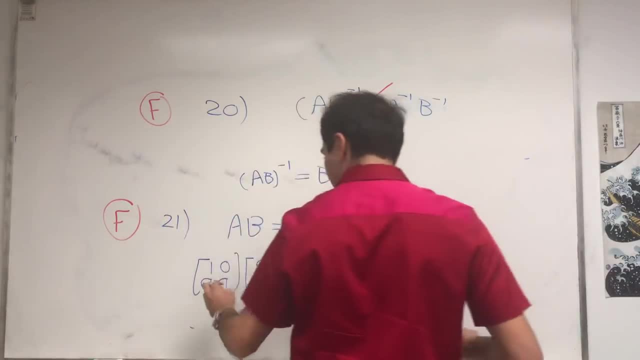 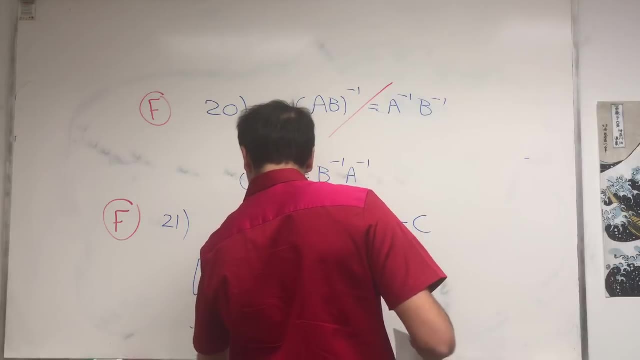 times 0, 0, 0, 1.. You calculate this. I think you get 1, sorry, sorry- 0, 0, 0, 0, and then 0, okay. Why did I do that? 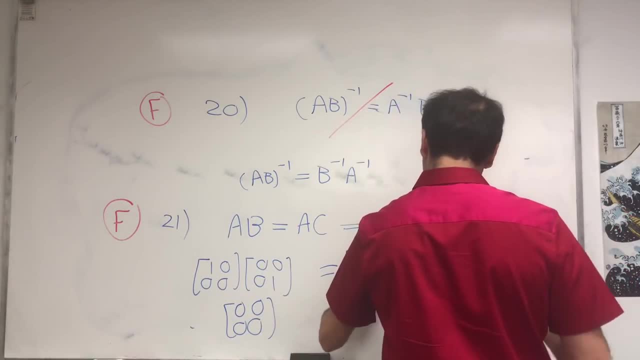 So 1, 0, 0, 0, and then 1, 0, 0, 0, 0, 0, 0, 2.. If you do that, you still get 0, 0, 0, 0.. 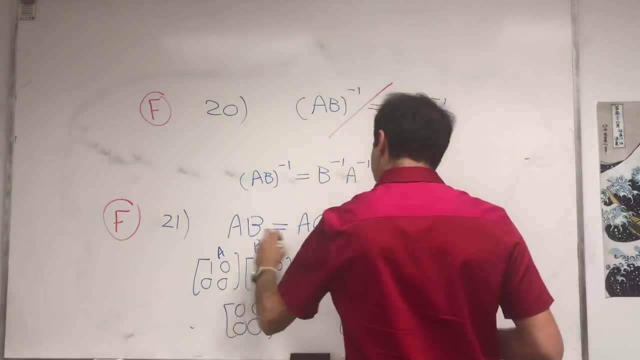 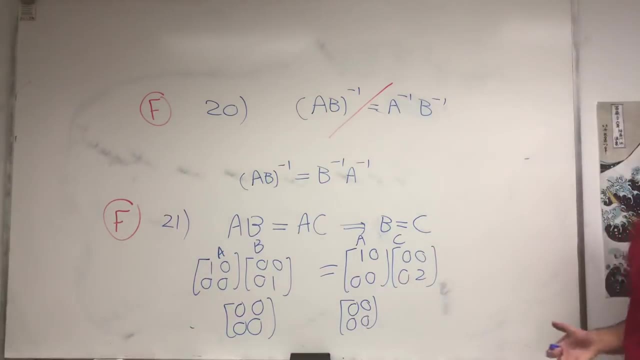 So you see, even though AB equals to AC and A is not 0,, it is not true that this matrix equals to this matrix. You can't just cancel out the two matrices and hope that the result is the same. It only works for what's called invertible matrices. 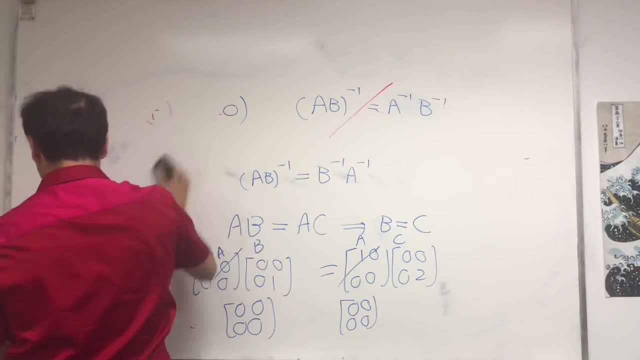 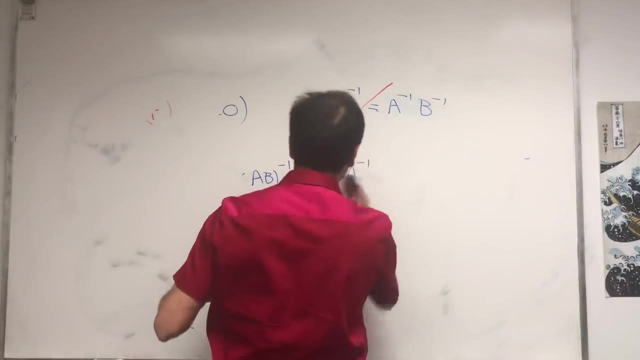 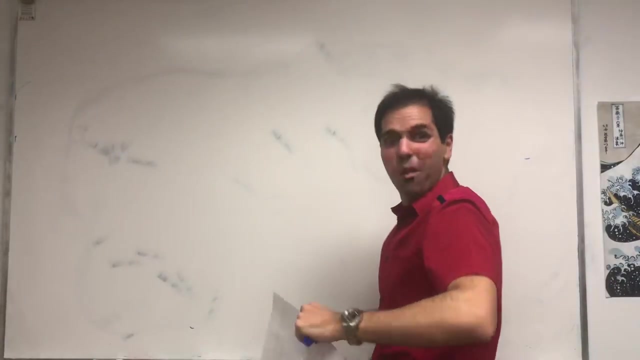 And in fact, let's talk about invertible matrices. So that's one, The point of chapter 2 of this second section, it's simply matrix multiplication. It's very weird, Can't do this. And, yes, we've reached the one-hour mark. 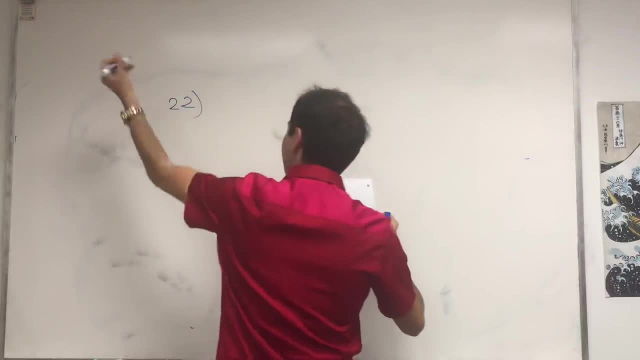 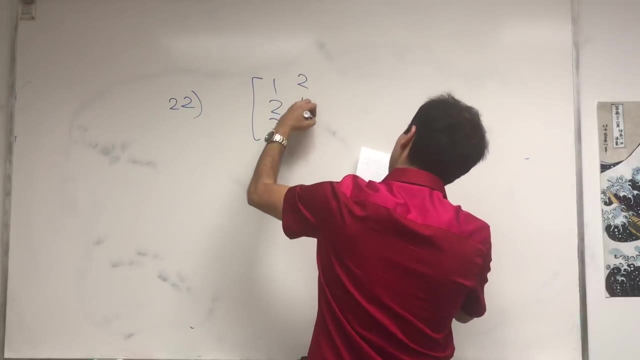 so let's see how it goes. So question 22,. indeed, 20% done almost. Is it true that this matrix 1, 2, 3, 2, 4, 6, 3,, 6, 9,? 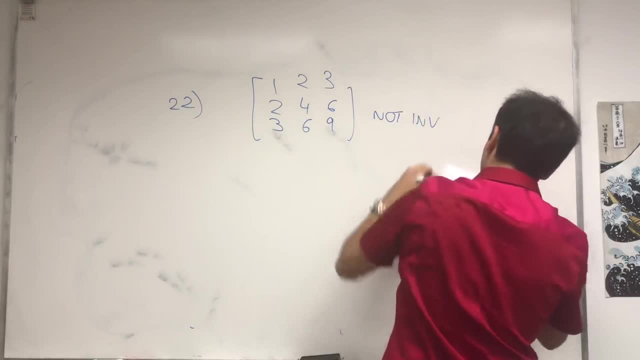 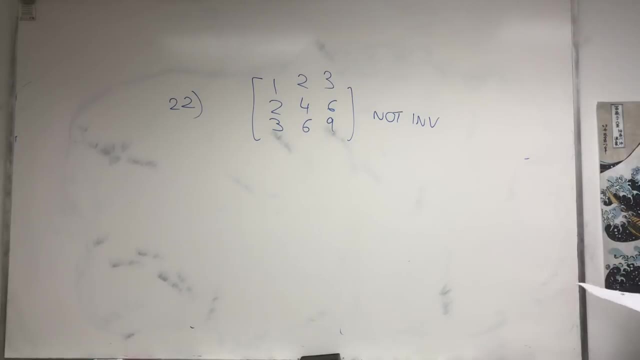 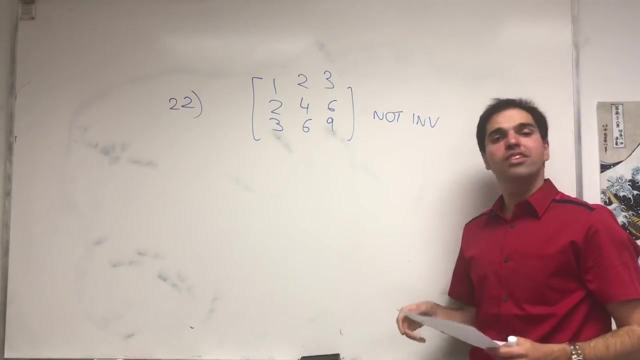 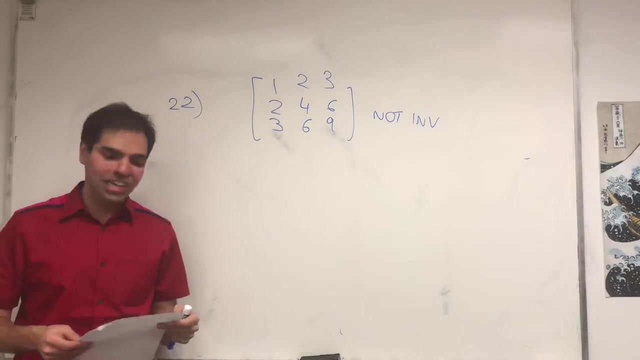 is not invertible And I know people are obsessed with determinants, but don't always use determinants. Sometimes there's an easier way, And so 22th language. 22nd language is another dialect of Chinese, the Jinyu dialect of Chinese. 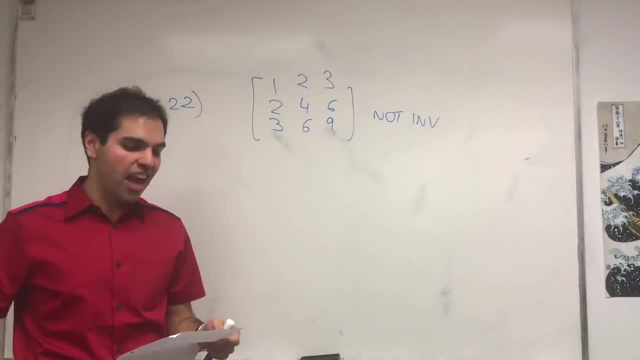 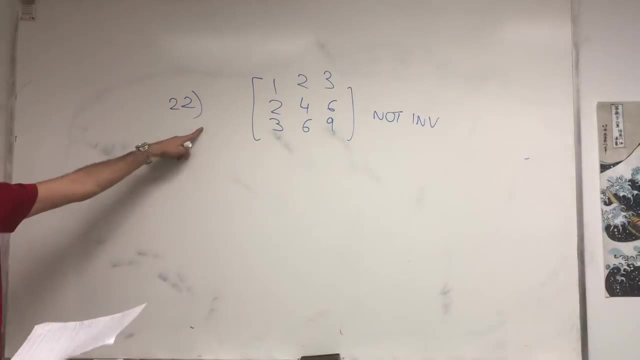 And I like this one too: 22 in that dialect is ar-shi-ar, ar-shi-ar or something. Yeah, Anyway. so indeed, this one, it's true. And again, don't use determinants, Try to use some linear algebra. 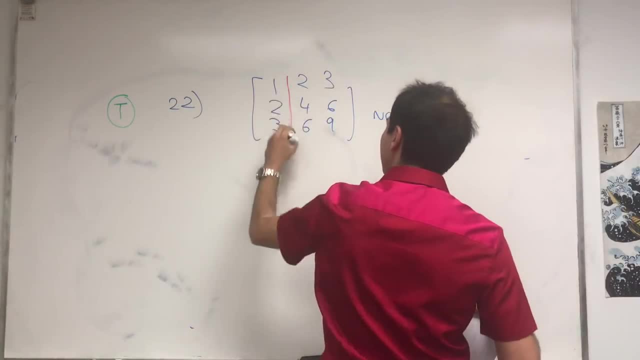 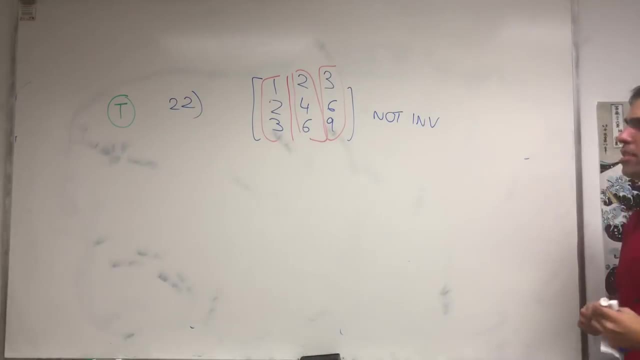 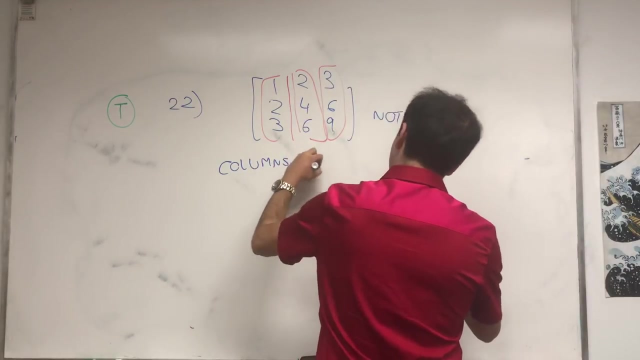 actually I do love determinants, so it's nice. But look at the columns. Well, look, This column is 2 times this column. so the columns, basically, are linearly dependent, Are linearly dependent. And if the columns are linearly dependent, 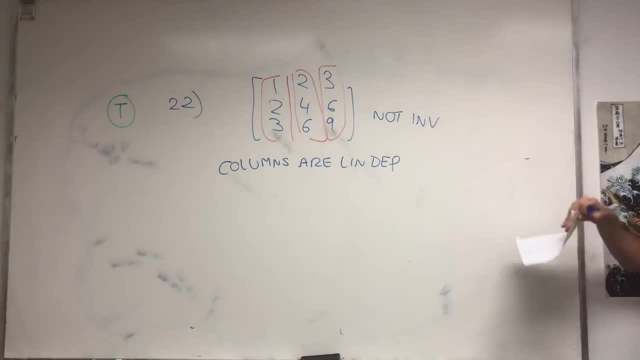 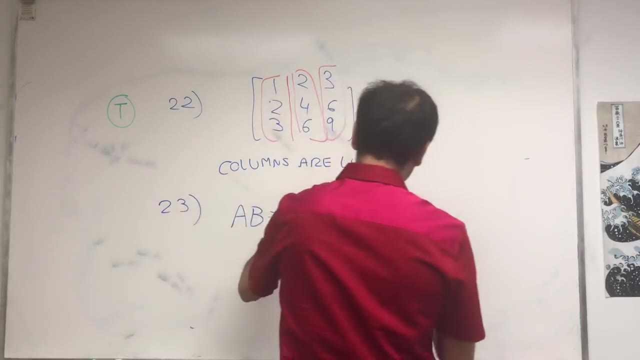 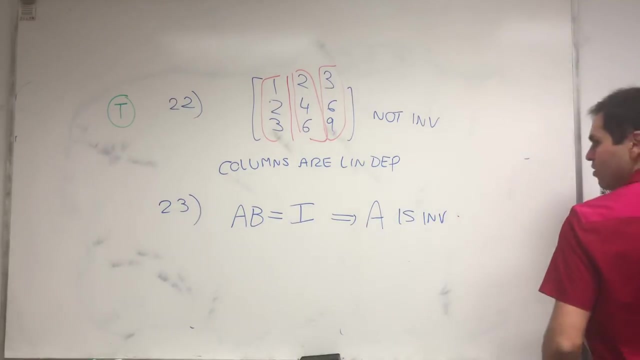 the matrix is not invertible. Or you could also look at the rows, Doesn't matter. Next one: If AB is the identity, then A is invertible. In other words, if you have some matrix B that undoes what A does, 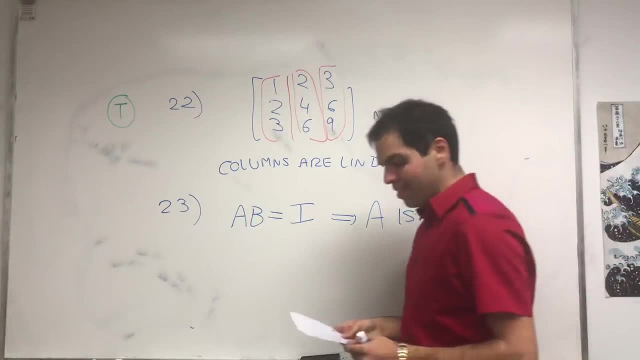 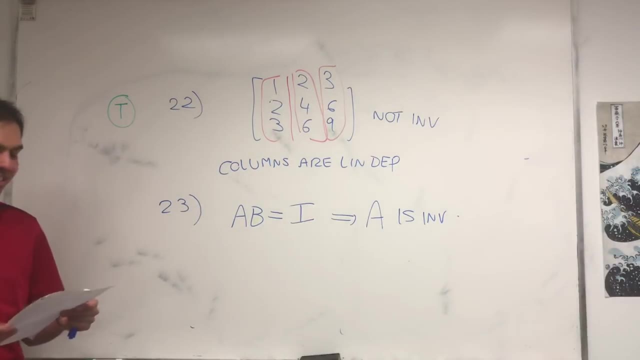 is the matrix invertible. And 23rd language, gujarati. and 23 in that language is trevi-sa. That's really cool, Like there's so many languages. I didn't know that existed, but they do exist. 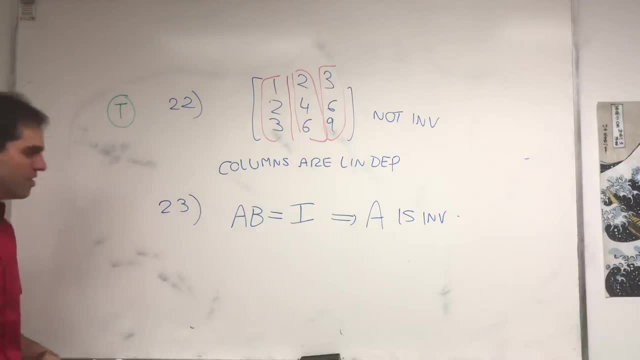 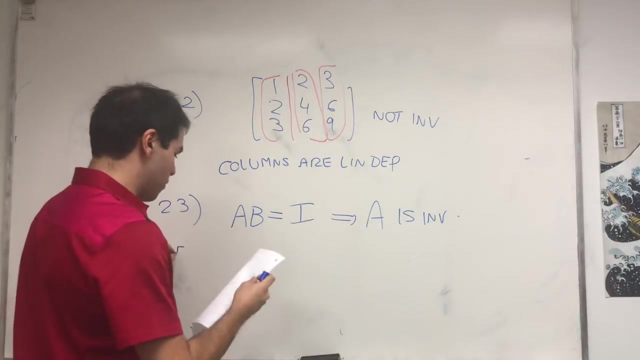 So that's really cool. What is not cool is this one, This question, Because this is actually false And it's very important. If I don't tell you that the matrix is square, do not assume it's square, Because take this example, for example. 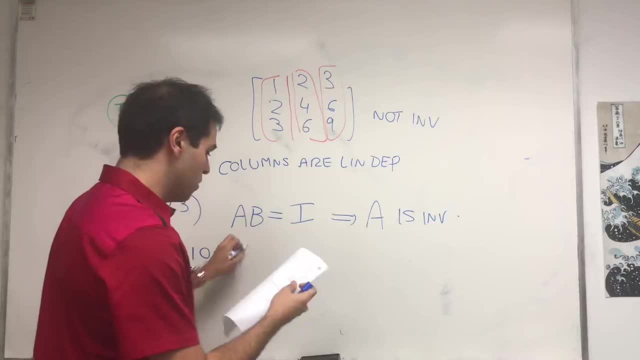 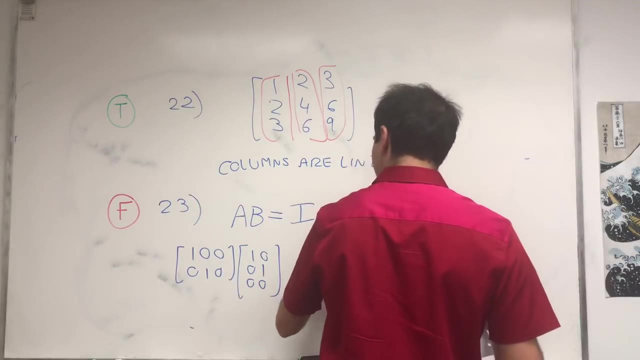 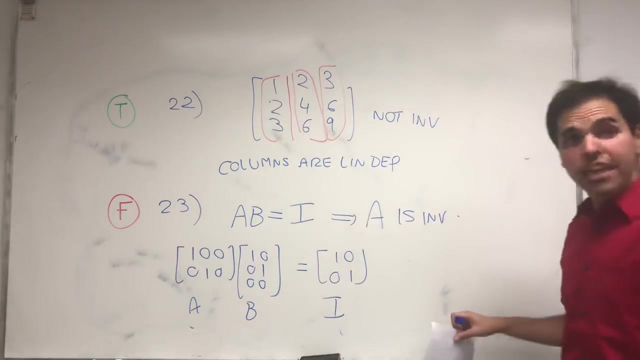 1 0 0 0 0, 1 0, 1 0 0, 1 0 0 And if you calculate that, you get that it's the identity. So AB is the identity, but A is not invertible. 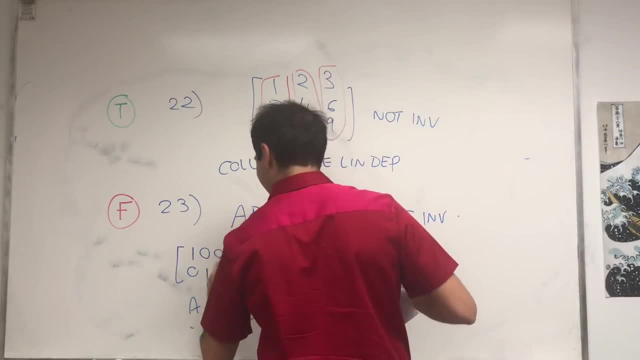 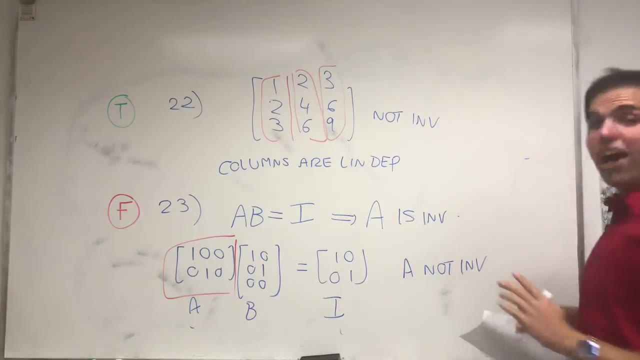 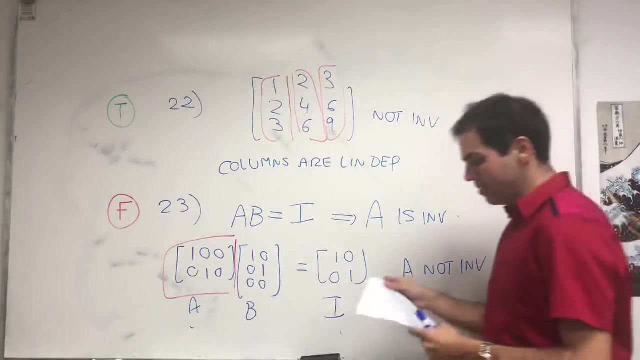 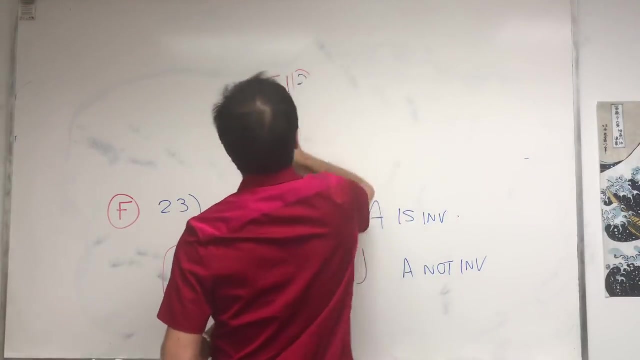 because A is a non-square matrix. And in fact, for the next two questions, let me show you why a non-square matrix cannot be invertible. Kind of stole the surprise, but this is for education, so it's very important, All right. 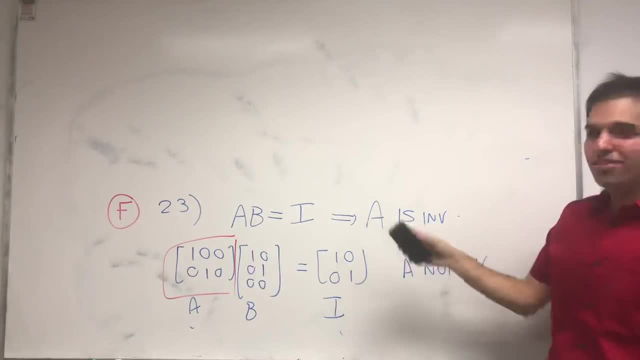 So, again, very important, If it's not square, it's, you know, don't assume it's square. But that said, if A is actually a square matrix- and this is true- then indeed A is invertible, So it has to do with something called. 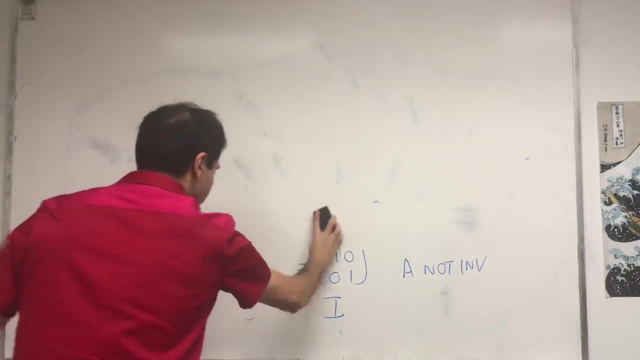 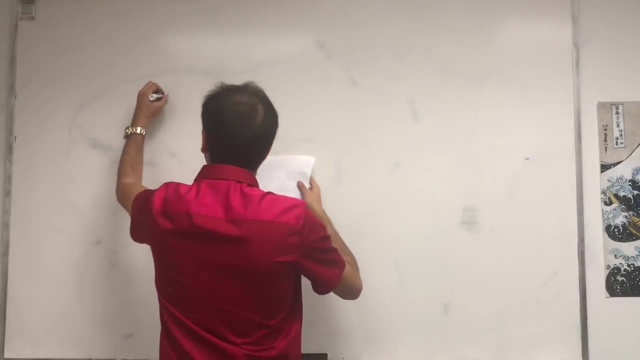 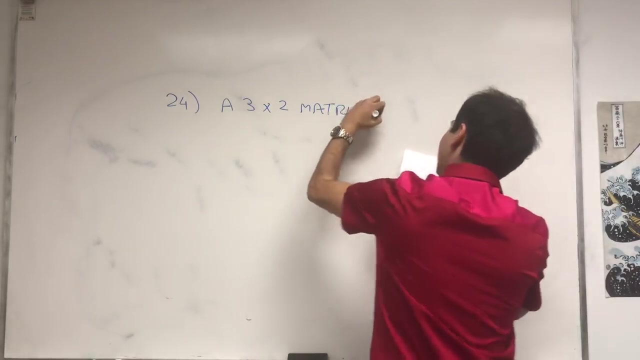 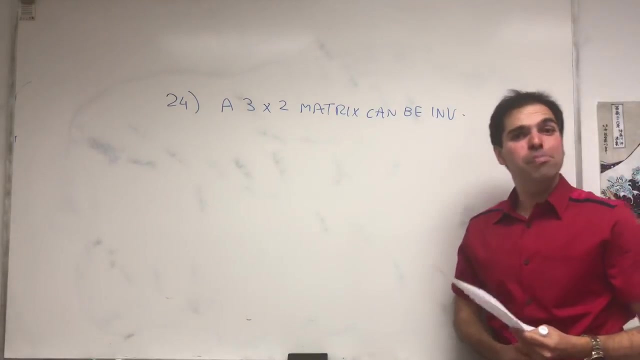 the invertible matrix theorem. So question 24.. A, 3 by 2 matrix can be invertible. 24th language, Polish, And 24 in Polish. is this one's hard? is No, No, No. 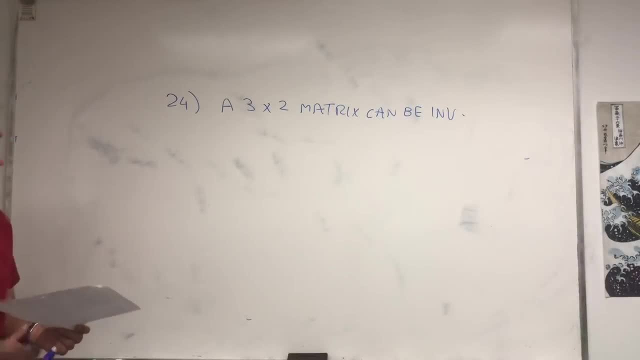 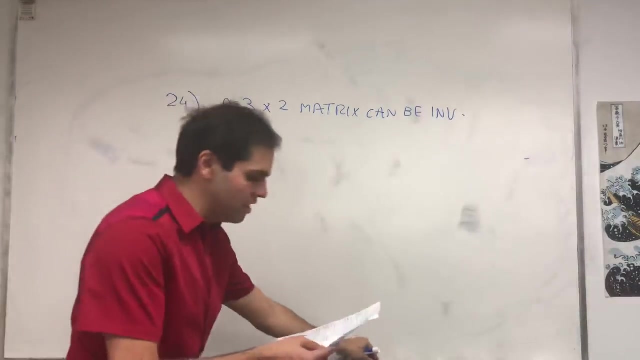 No, Very complicated language, but And so again, sorry for butchering all those languages. I do not know 111 languages, I only know like five-ish. Anyway, can a 3 by 2 matrix be invertible? 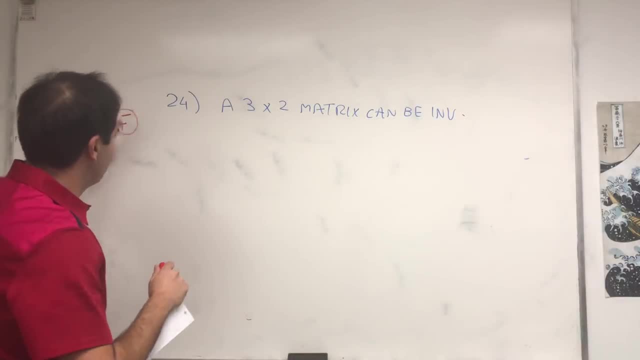 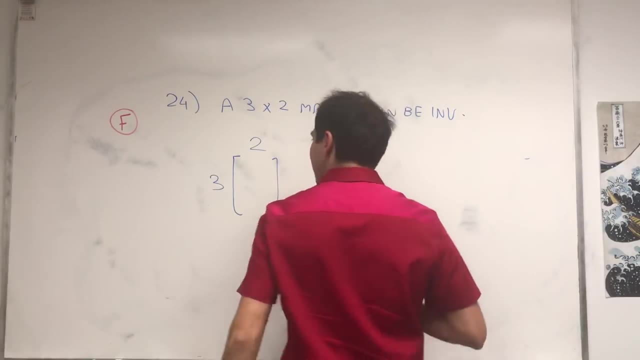 Well, I kind of gave it away before, but the answer is false. And why is it false? Well, let's look at that. Suppose you have a 3 by 2 matrix, how many pivots can it have at most? well, at most it can only have two pivots, it's. 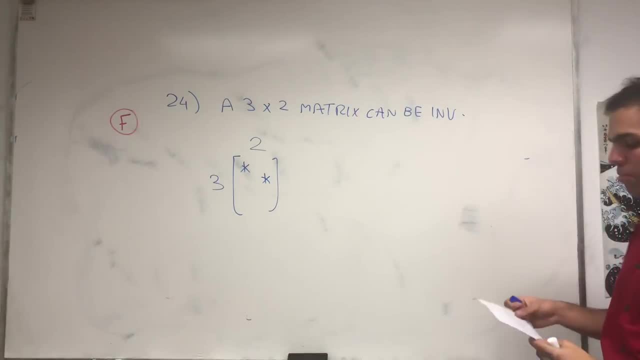 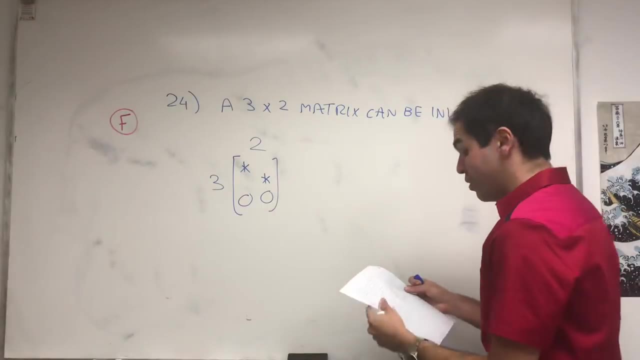 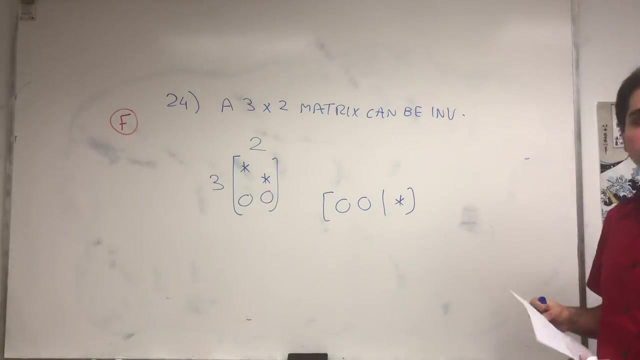 always less than the smaller of the number of rows in the number of columns, which means at least in the row reduced echelon form, the last row has zeros. and what does that mean? it means that for special B we have a row of the form something, something zero, zero, something else, where that something else is not. 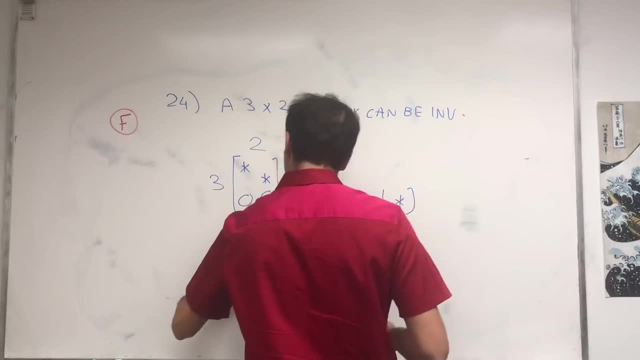 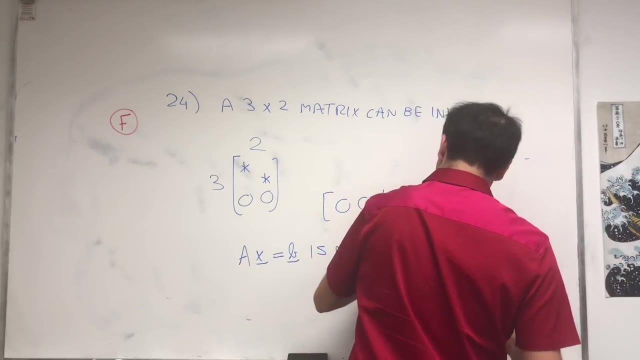 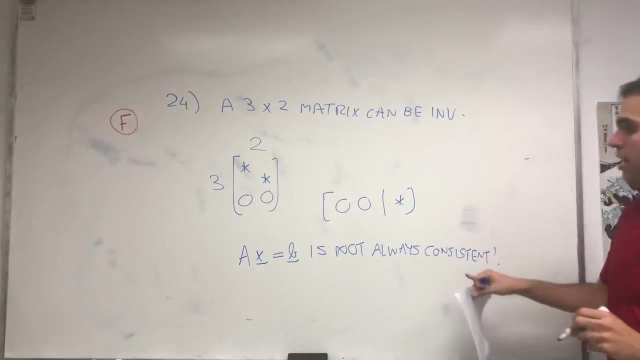 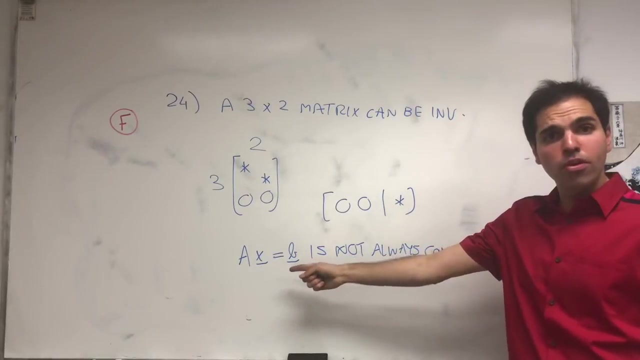 zero, which tells you, remember by the four, ax equals B, is not always consistent. so, interestingly, such a matrix can never be invertible because, look, if a is invertible, then the equation is always consistent. because you can just have X is a inverse B, you can just have X is a inverse B. 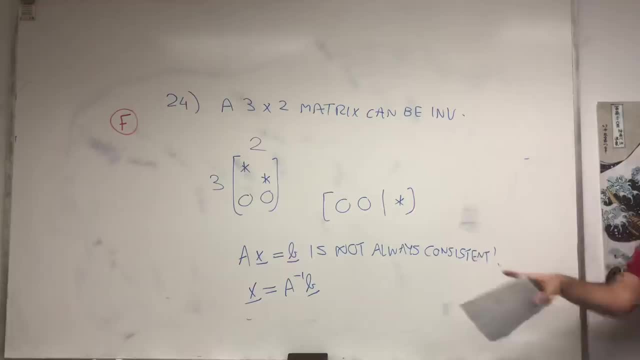 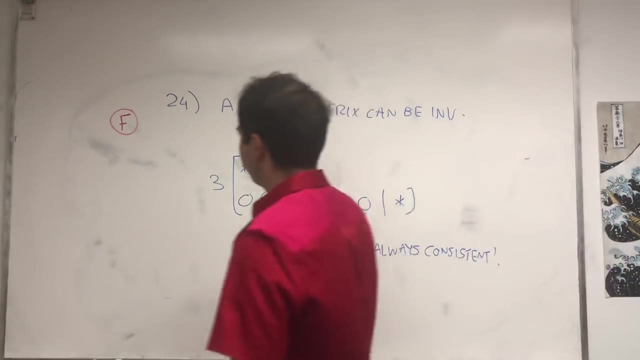 you can just have. X is a inverse B. the point of invertibility is it gives you a unique solution for your equation and therefore for this matrix. it can never be invertible. so it's not that there's some examples that are not invertible, it's that it's never. 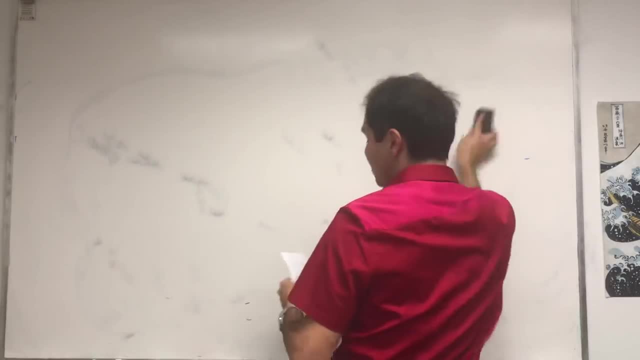 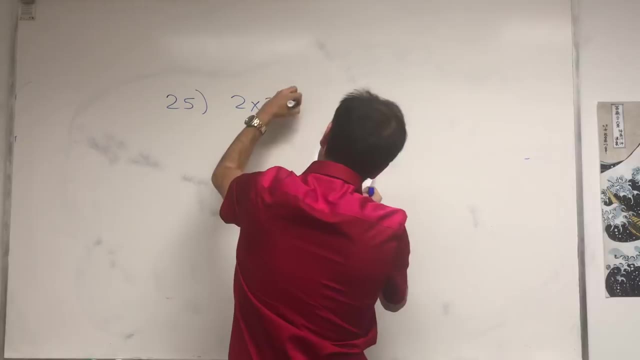 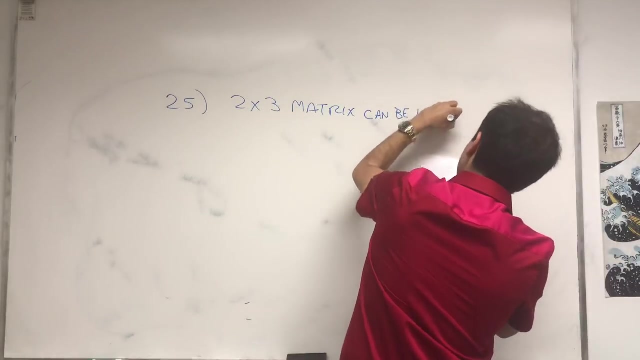 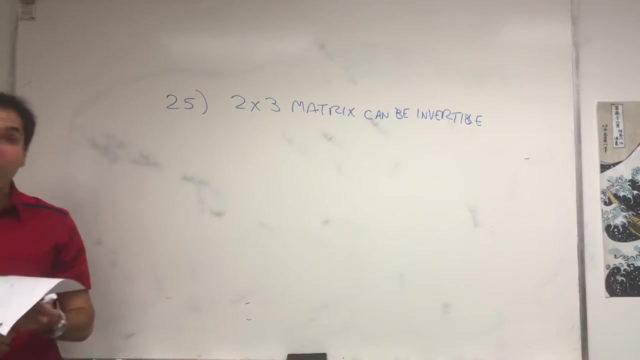 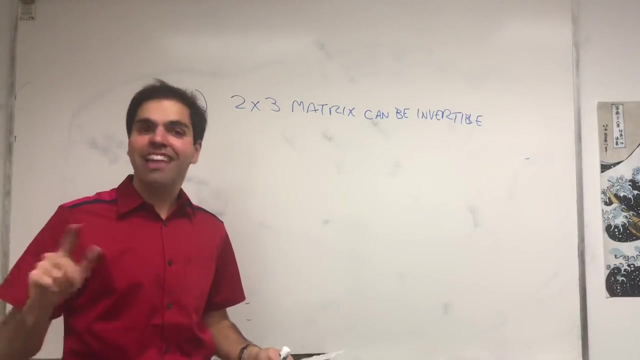 invertible. what about the other scenario? what about a two by three matrix? and so the 25th language. so it's all dialects of Arabic, and this time is the Egyptian dialect of Arabic, and unfortunately I couldn't find info about the different dialects, so I just gonna say all the dialects in Arabic. so just standard Arabic and 25 in. 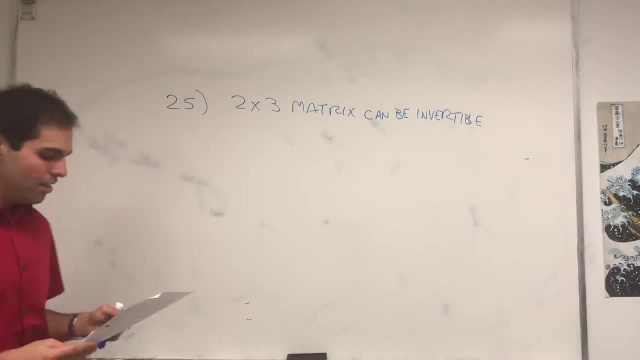 Arabic is Khamsu, Shrina, I think, Khamsa and Ashrina, so 25, and the question is: can such a matrix be invertible? well, similar to the last question, it cannot be, but for different reason. so suppose you have a two by three matrix. 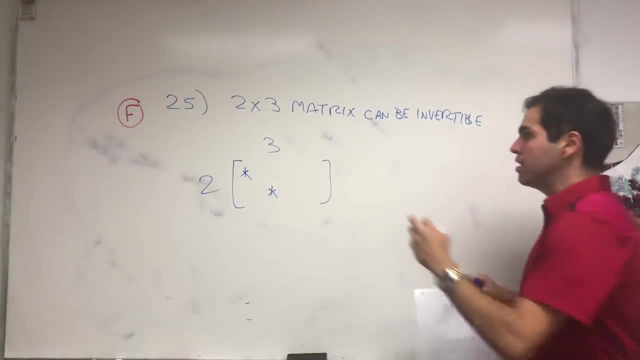 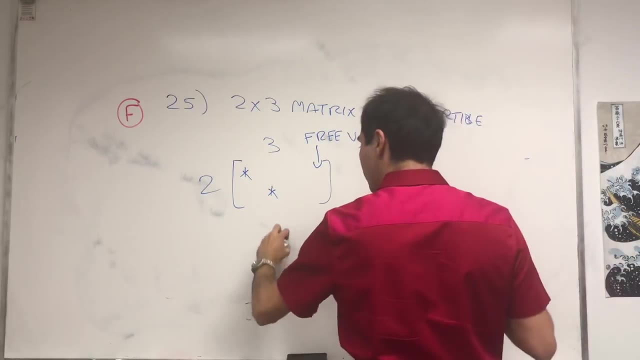 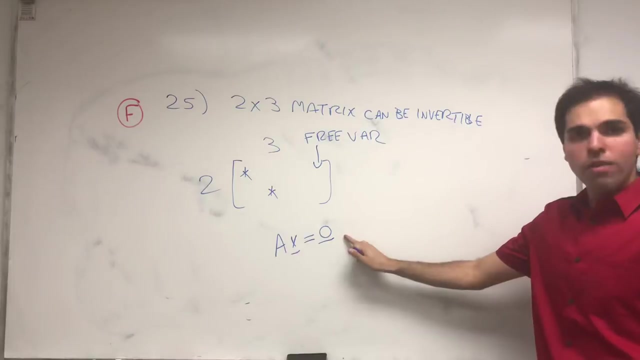 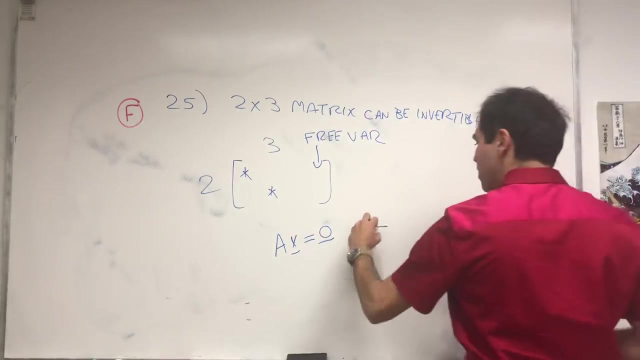 again, it can only have two pivots at most, which means the last column is a free variable. in particular, if you take the equation, ax equals to 0 because it's a free variable and this is always consistent. having the zero solution, this means this has infinitely many solutions. in particular, it does not imply that X. 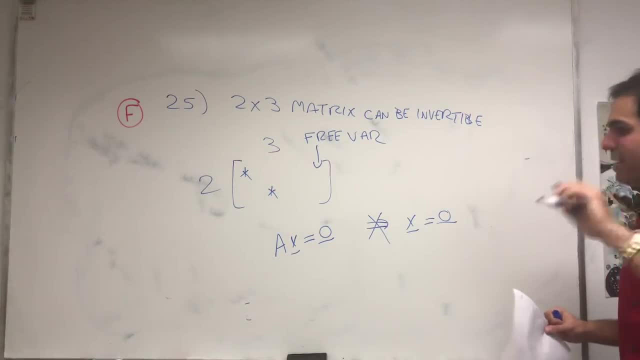 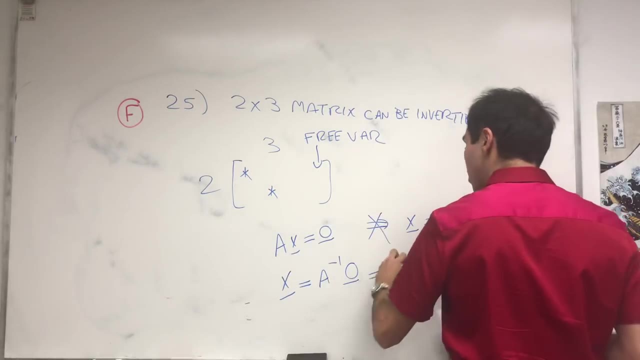 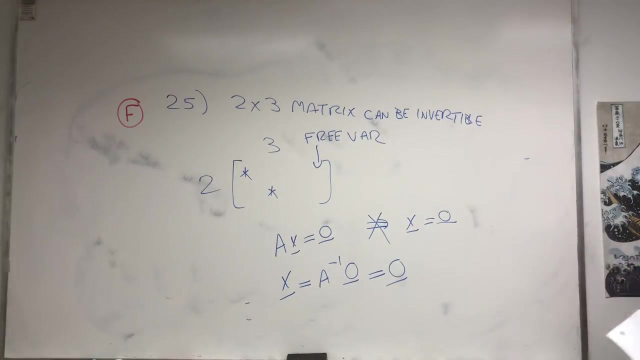 is zero, which is a problem, because if it's invertible, then this means X is a inverse zero, but a inverse zero is always 0. so if a were invertible, then the only solution would be X equals 0, but in this case it's not the case very. 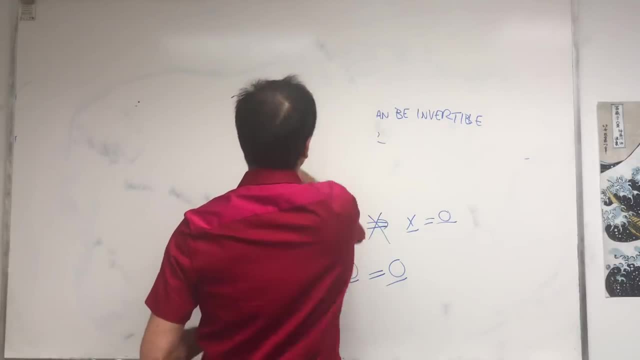 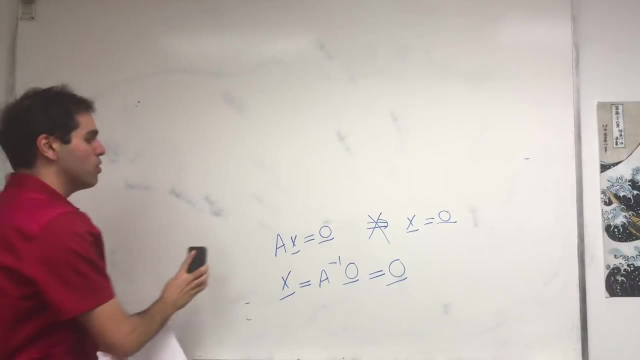 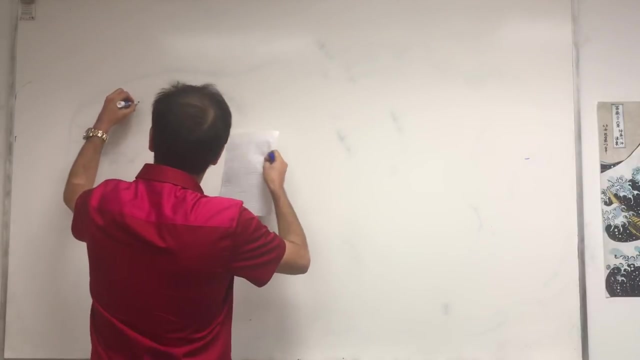 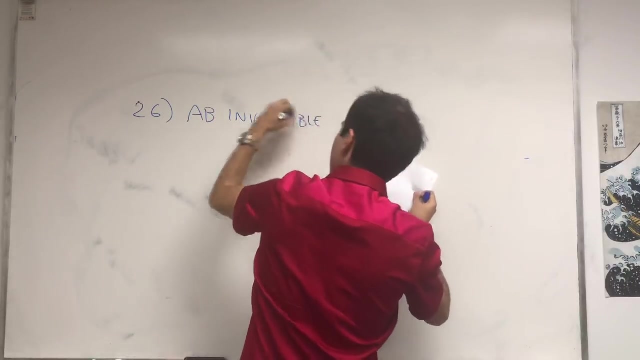 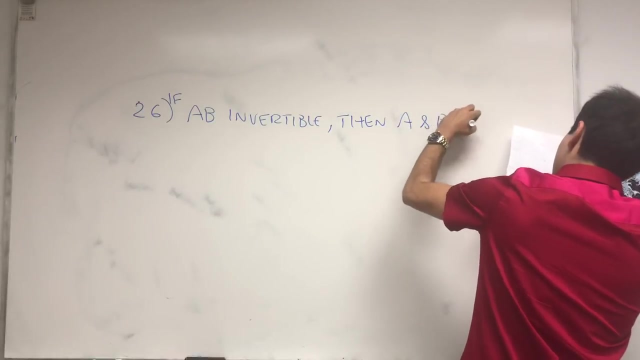 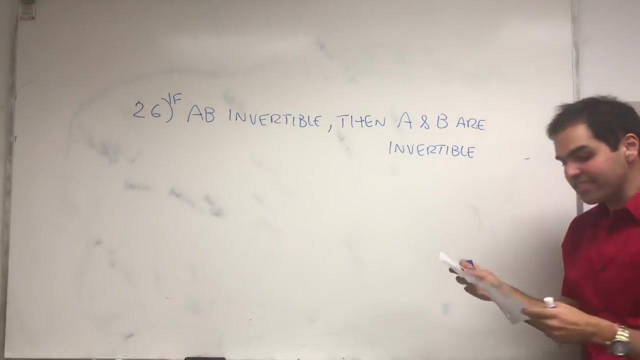 good. so, in other words, what I've shown with the two examples is that a- what's called a nonsquare matrix, can never be invertible. Okay, next question: If AB is invertible, then A and B are invertible. And language 26, Ukrainian And 26 in Ukrainian is again something complicated. 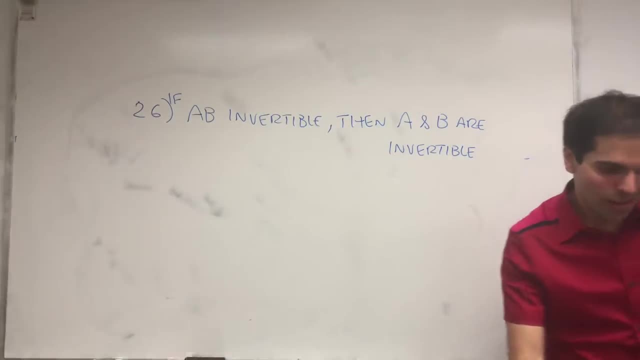 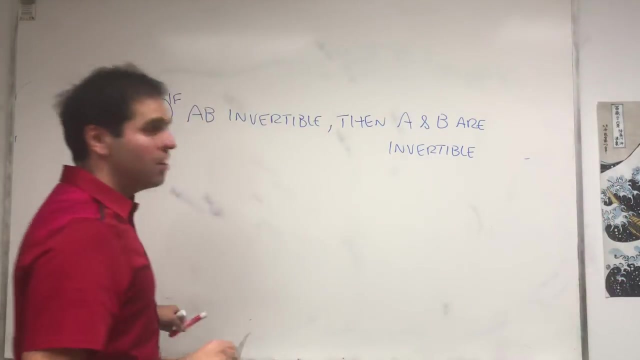 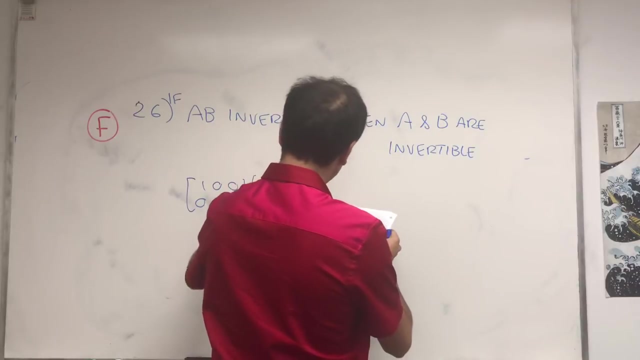 zvadzit shist. And again, unfortunately, this is false Because, remember, unless I tell you a matrix is square, do not assume it's square, Because, indeed, sort of similar example to before, if you take 1, 0, 0, 0, 1, 0, 1, 0, 0, 1, 0, 0,. 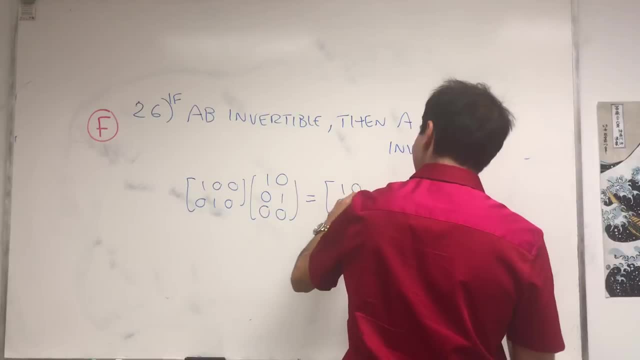 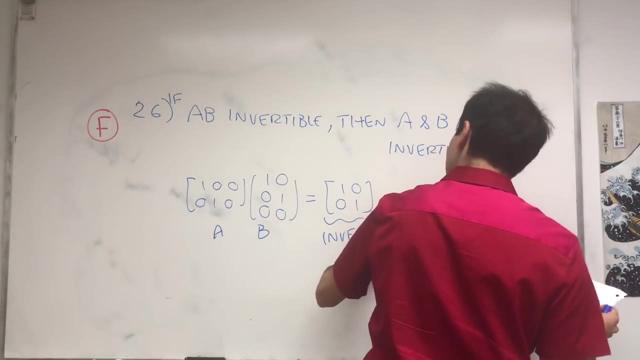 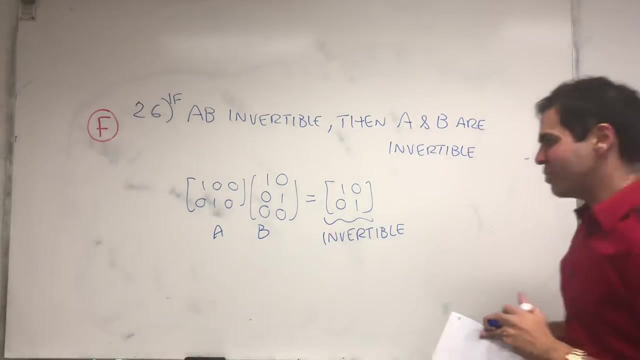 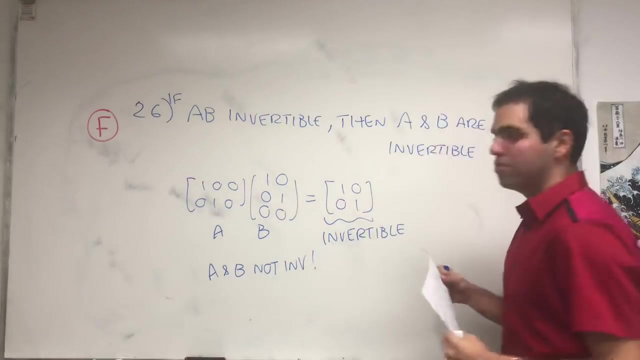 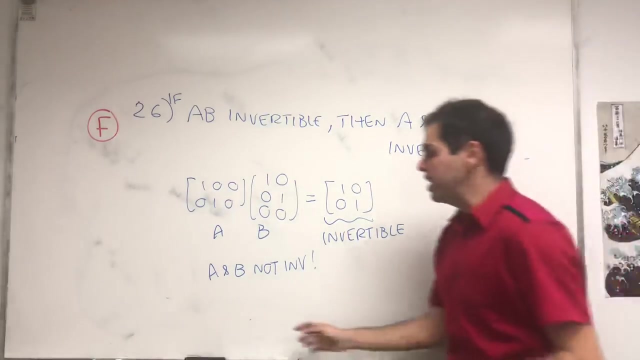 0,. if you calculate this, you get the identity matrix. So AB is the identity matrix which is invertible. So AB is invertible, but A and B, they're not invertible because they're not square. So, and well, you might ask what if they are square? Well, let's see. So let's do the same. 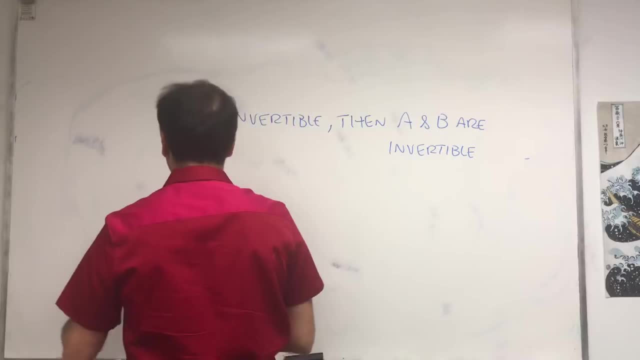 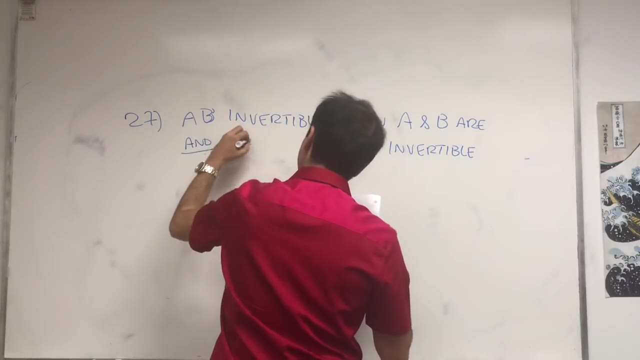 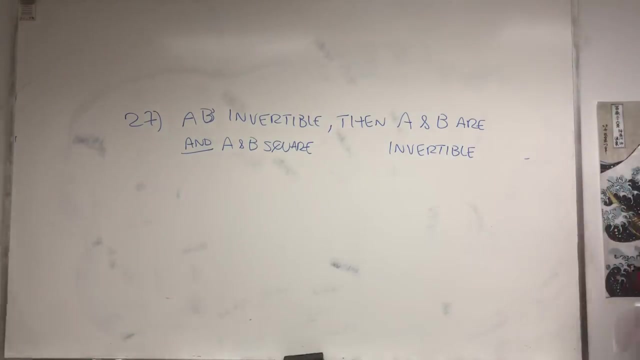 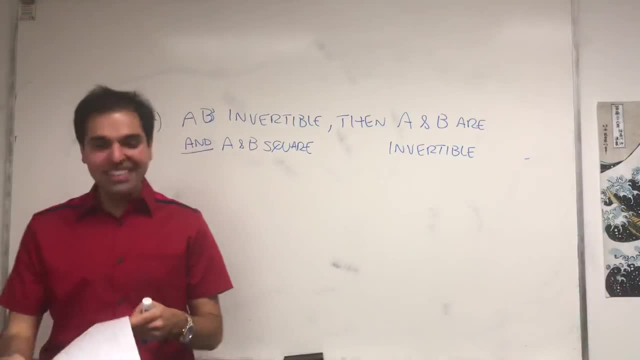 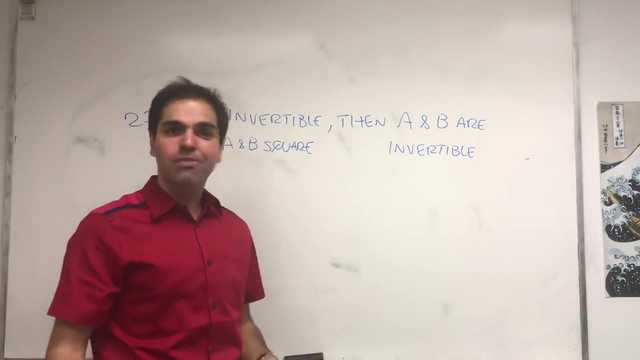 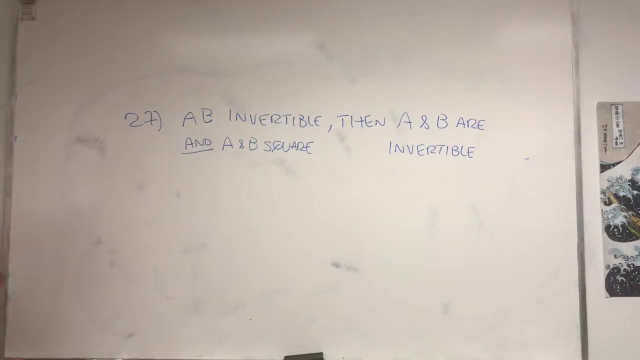 Let's find out. But 27th language is Italian. Ah, fa bene, And 27 in Italian is 27.. Like 27 in French: Ah fa bene. Ah fa bene. Ah molto bene, Ah, poi no, I don't know Italian, unfortunately. 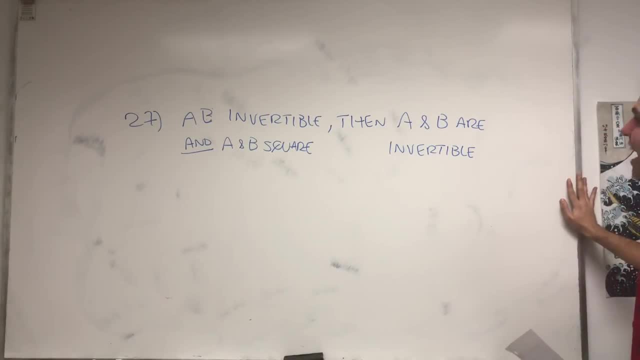 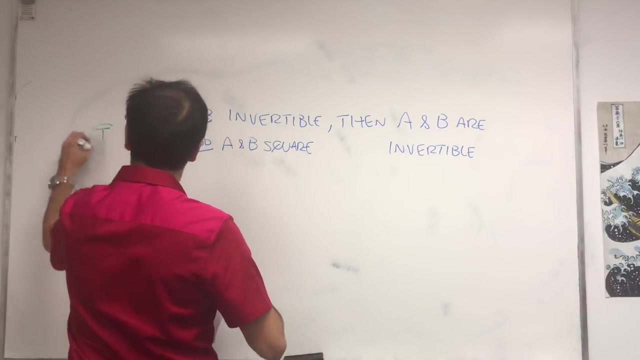 I wish I knew. It's a beautiful language. That's it. Interestingly, if AB is invertible and both matrices are square, then it turns out both components are invertible. So this is really cool. So this is true, And the easiest way I can think of is simply with determinants. 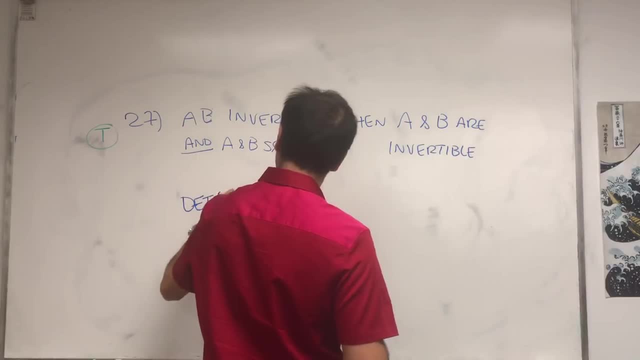 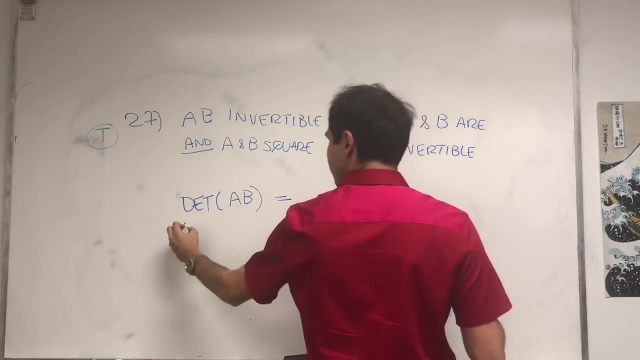 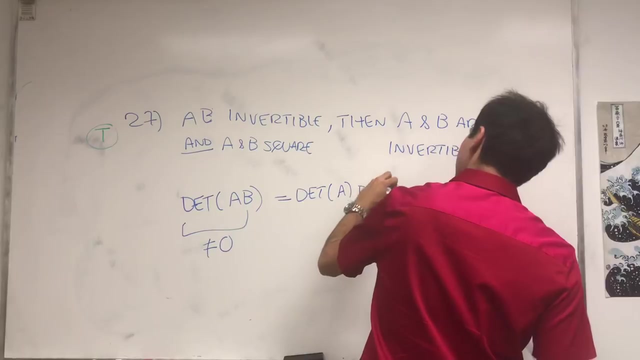 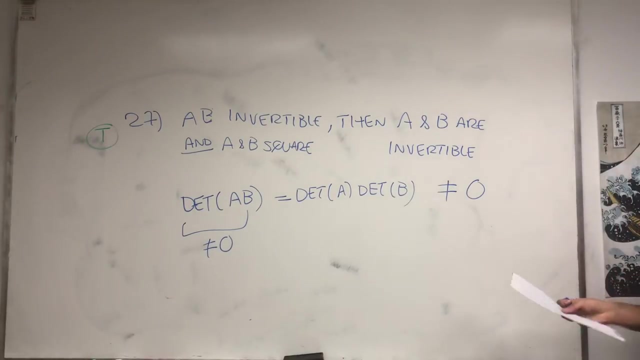 determinants, so determinant of a- b. If determinant of a- b, in that case, because it's invertible, we know it's non-zero, but this is the same as determinant of a times determinant of b. And look if a product of two numbers, it's non-zero. 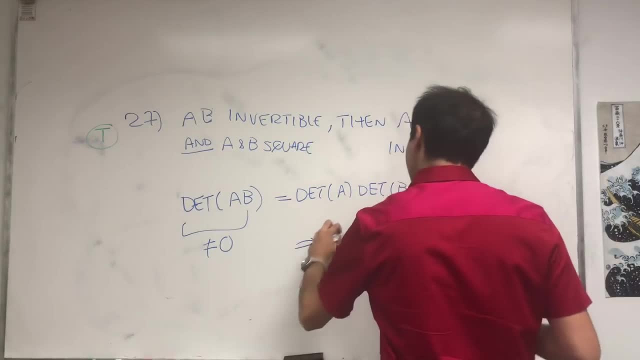 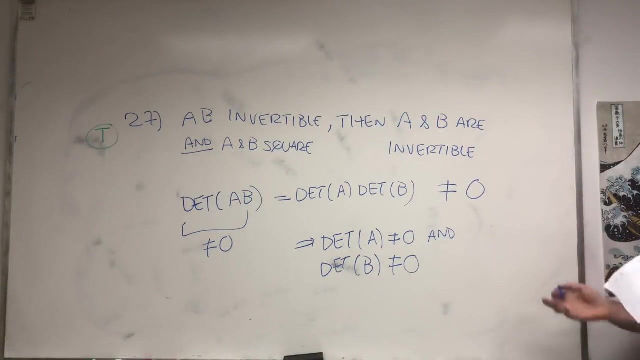 this means both numbers have to be non-zero. So determinant of a is non-zero and determinant of b is non-zero. That is neat. And of course there are other techniques, Because ab is invertible. there's some matrix C. 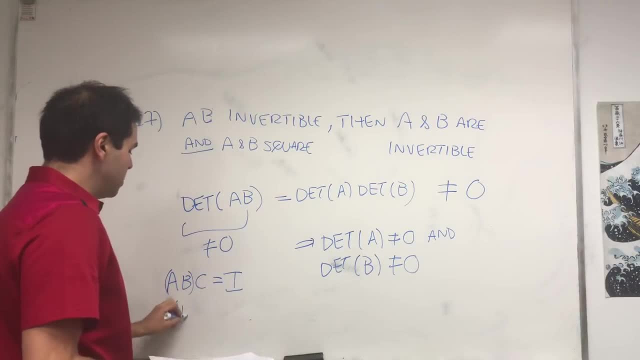 such that abc is the identity. but that means there's some matrix bc such that a times a matrix is the identity And if a is square, that's enough to conclude that a is invertible And same with the other side, with b. 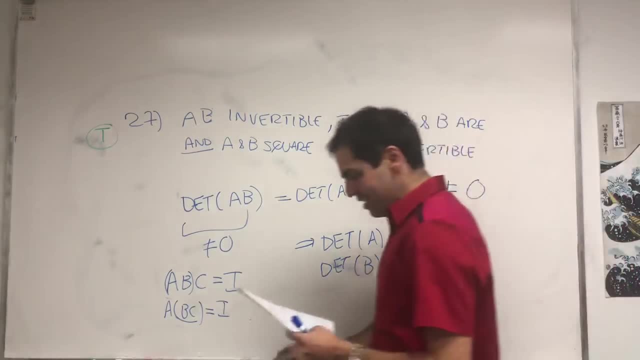 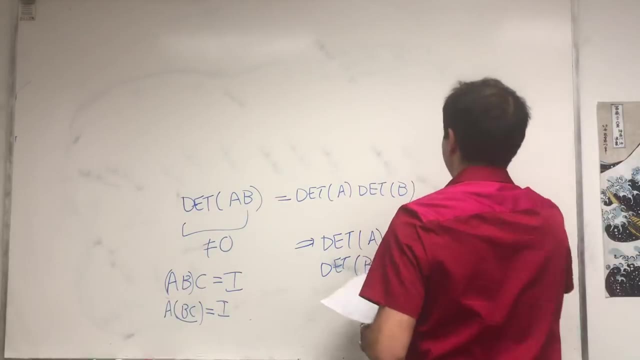 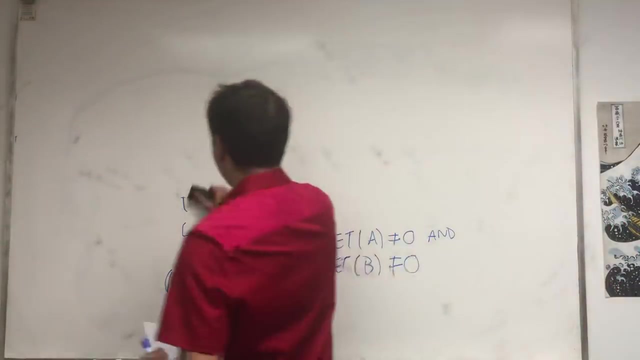 But I like determinants, so I think this is OK. OK, now let's move on a bit to matrix spaces, All space, column space- At least I think that's what we'll do A little bit. OK, we'll talk more in chapter 4 about this. 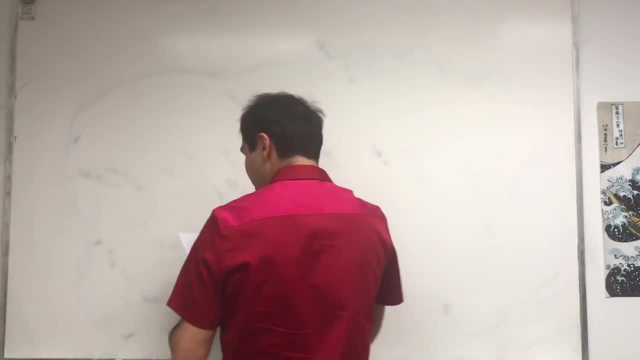 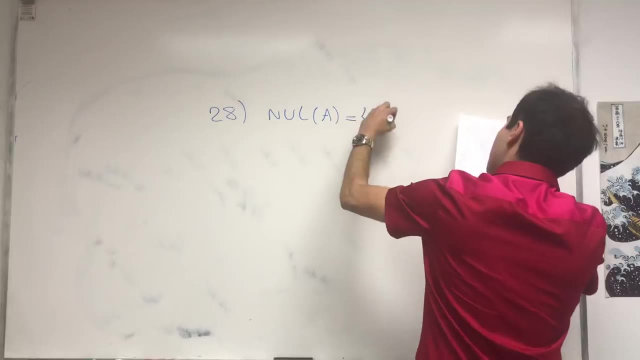 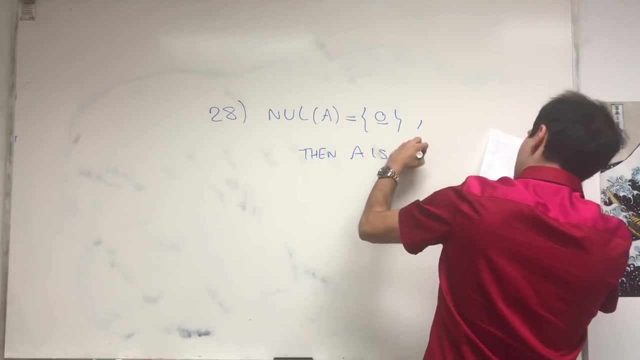 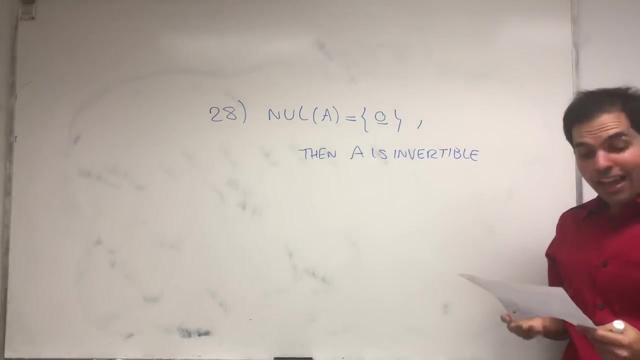 It's a question. If the null space of A is 0,, then A is invertible And language 28 is a dialect of Chinese, the xiang dialect of Chinese, And 28 is a dialect of Chinese And 28 is a dialect of Chinese. 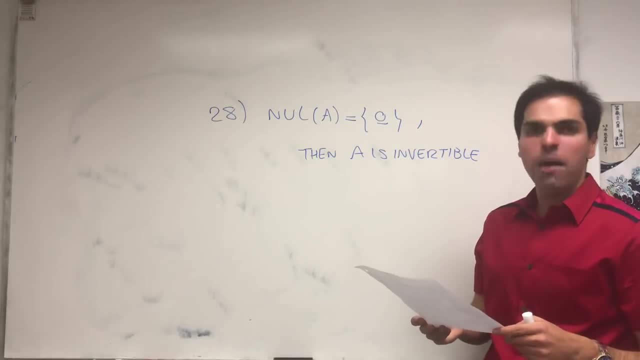 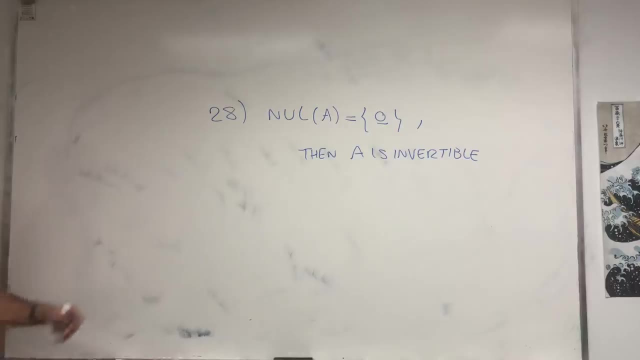 And 28 is a dialect of Chinese And this, at least in that dialect, is like Shabbat. almost OK Again, unless a matrix. I say the matrix is square, do not assume the matrix is square. so indeed, this is false. 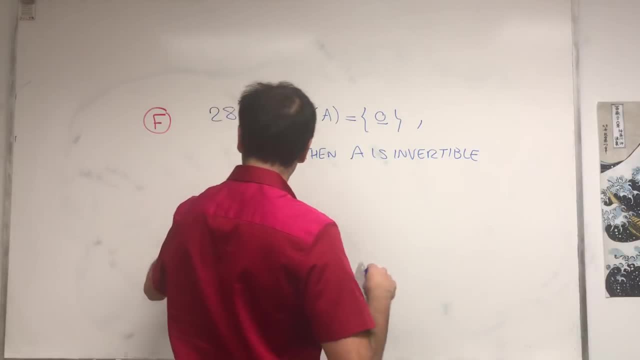 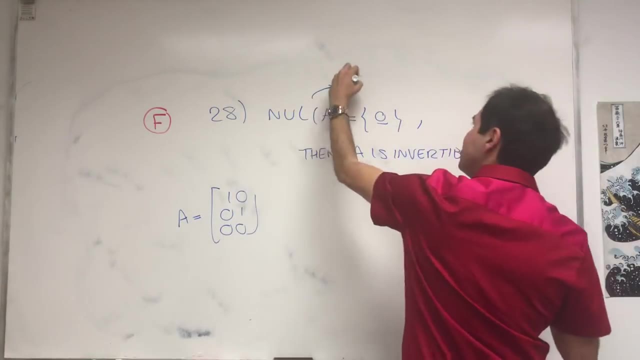 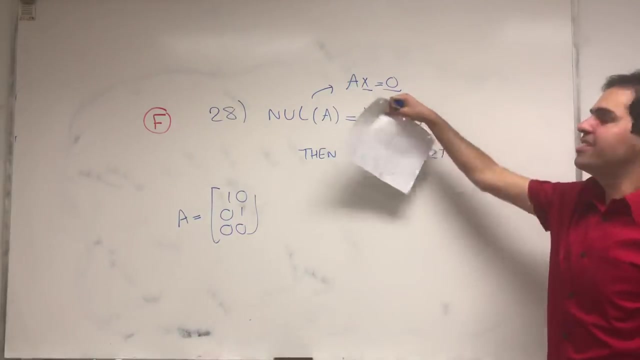 And here is an example. okay, So take this matrix: 1 0, 0, 1. zero. and again the null space has to do with AX equals zero. so the null space- null as in zero- is a set of solutions of AX equals zero. but if you solve AX, 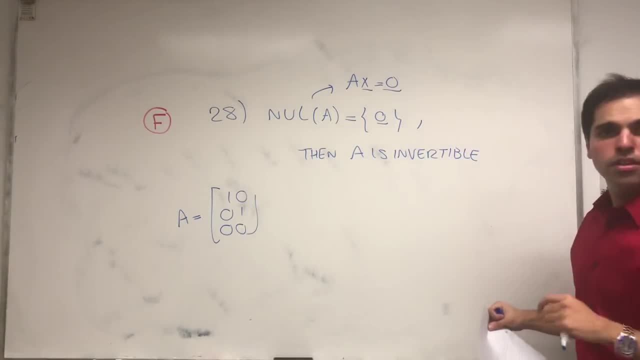 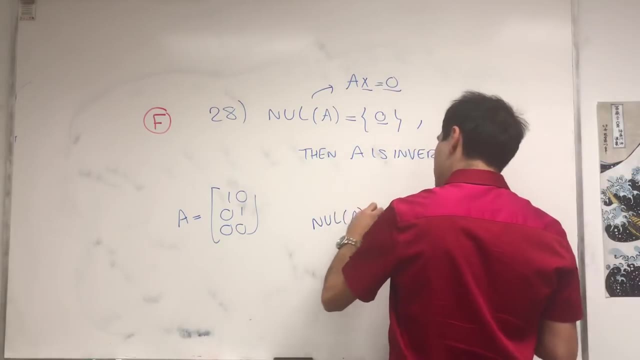 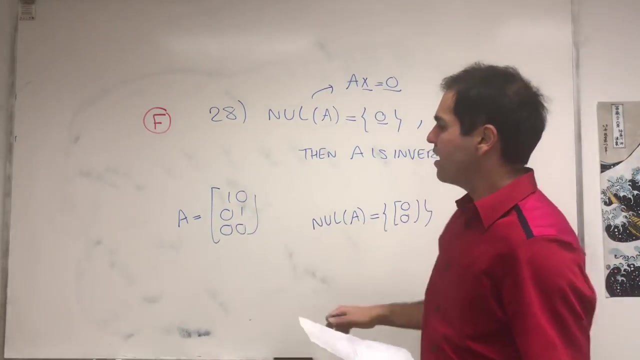 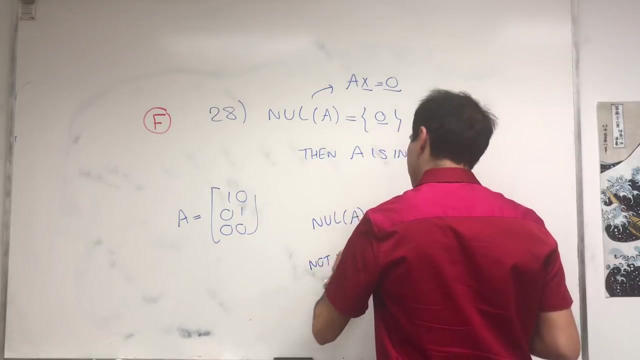 equals zero. notice: there are no free variables, so that's why it only has the trivial solution. so null space of A is indeed just vector zero, zero. if you solve AX equals zero, you get X equals zero and Y equals zero. but A is not invertible because it's not a square matrix. all right, good sheet two done, let 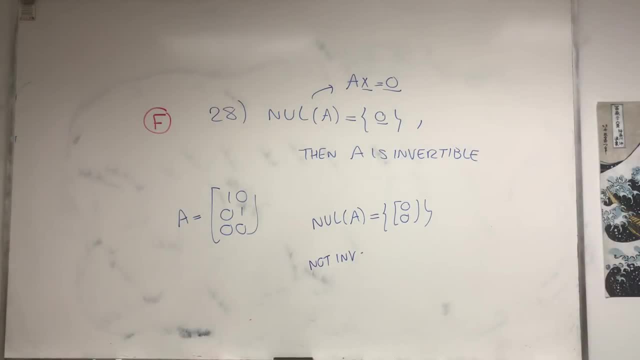 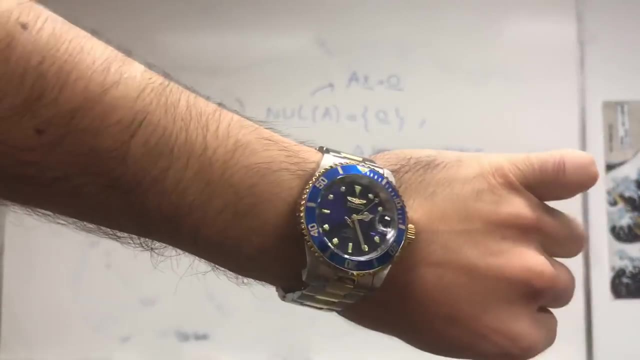 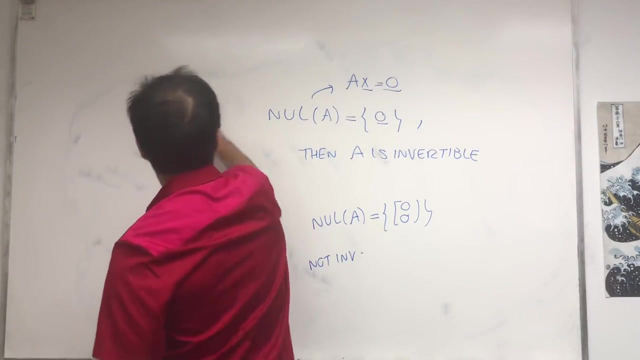 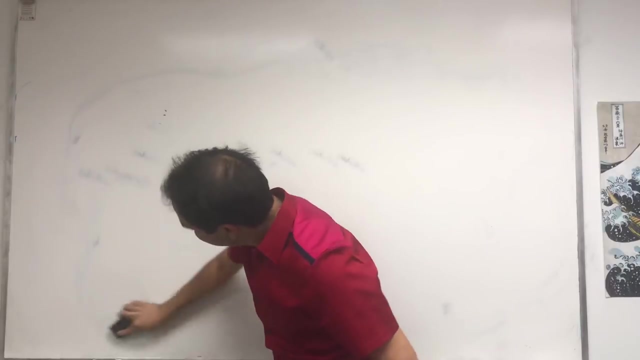 me just check on like the camera, check everything is fine. yes, everything is fine. yeah, look at my thumb and then also just checking the time, right you see? so it's really real time and also the whiteboard got really dirty. well, nothing I can really do. I ran out of this cleaner too, so let's see, okay, question. 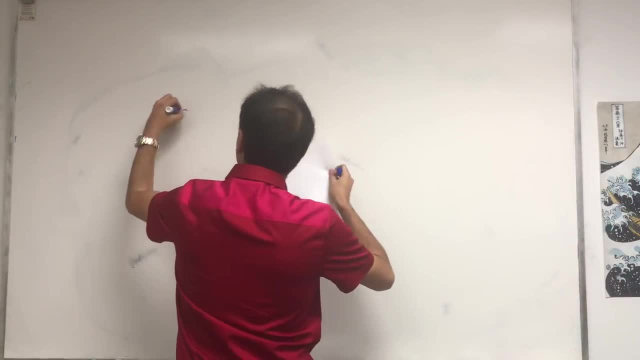 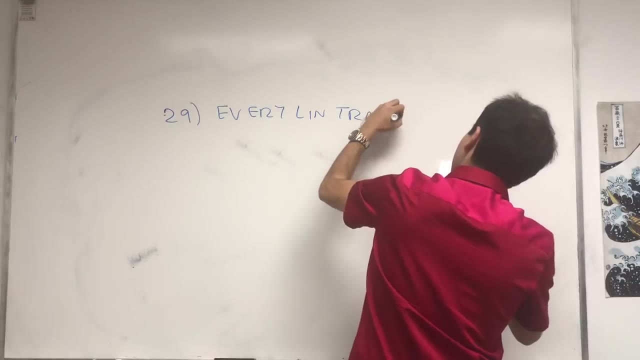 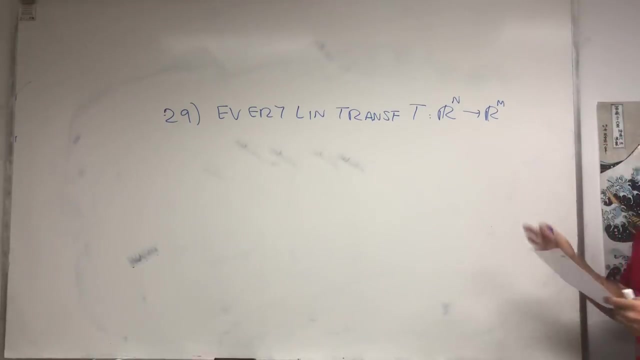 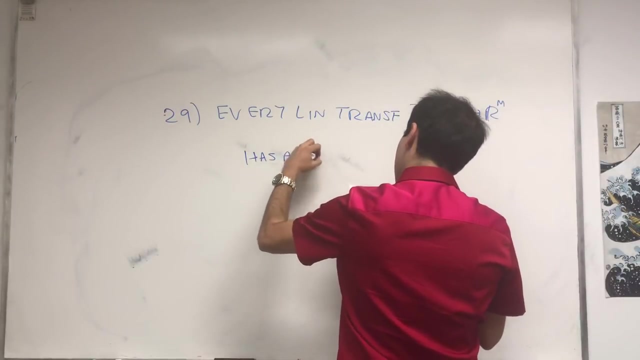 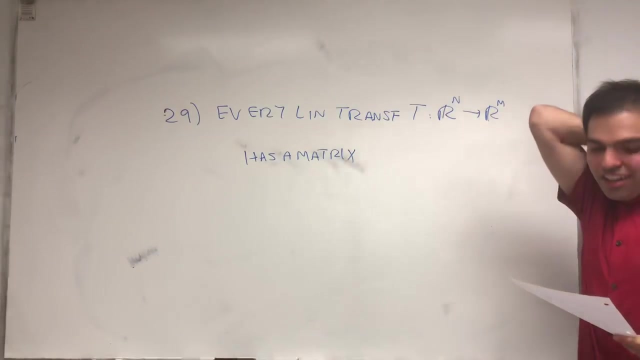 29. every linear transformation per second. the moment f2, it always gets up the word f2. the function f2 is t. sorry, not this way, because I upset the terminal node, but T from t method. while we are talking, are you are nothing but bra. statt er is it crash. is that right? more fail. so if you do the linear transformation from RN to Rf, any one of those has a matrix and language. 29: Ma la la no작. go on, ma lal tom werk wijk vol. haha, oh, this time it does sound correct, Mario le, depending on where a mal là elect is to sayuno cycling boy. ma la, la, la man. okay, Na 71, when the música has been successfully伸伏ado anllamial mobile by choosing the verb for the shape of rapat 생 así como unaPsua" La que te inv para que ven a cambiar a peprusio do follia a ser a pe Energie entre carriera. com editar a buyer? quid pro общímato". 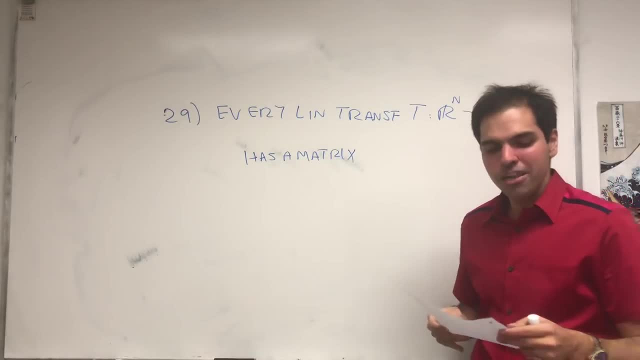 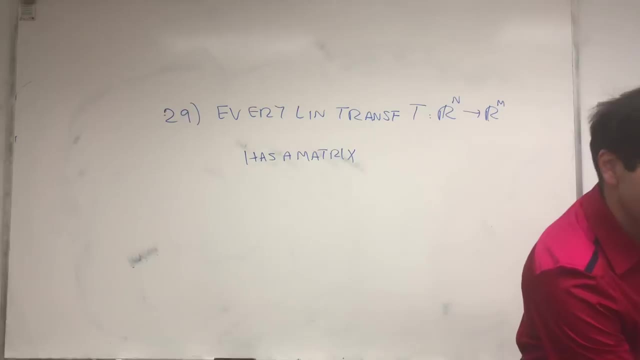 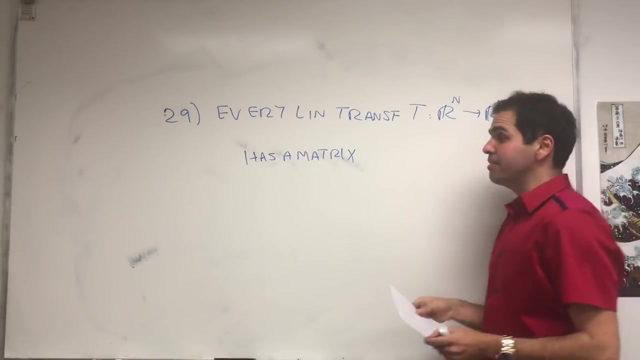 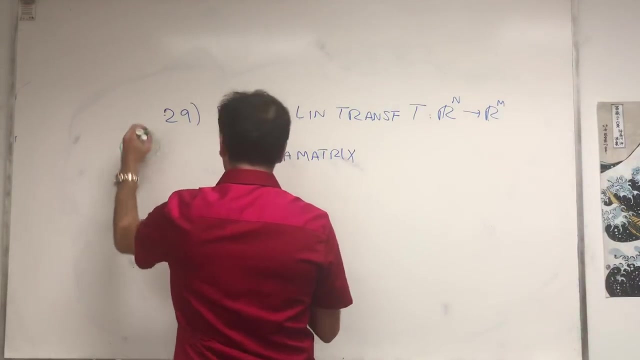 Okay, I think Malaysian. I'm not 100% sure, but the way you say 29 in the language is irupati tontat, So cute. And indeed for linear transformation from Rn to Rn, it is true that it has a matrix. 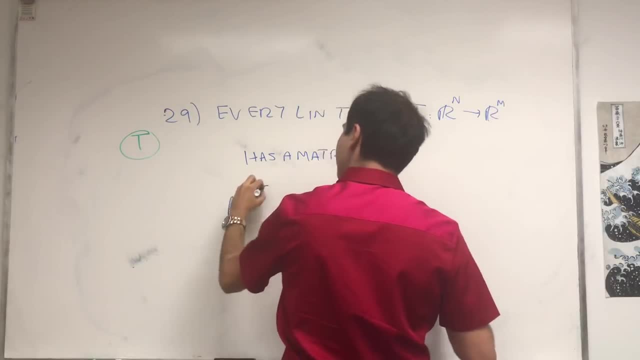 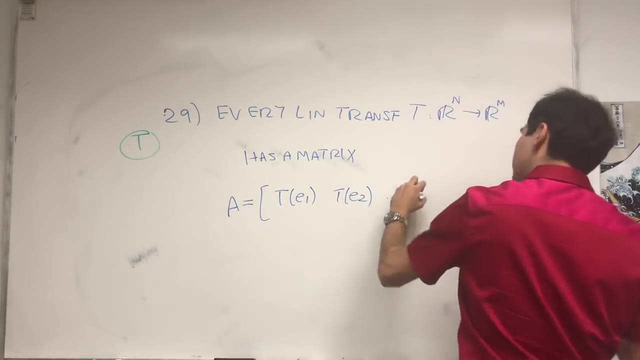 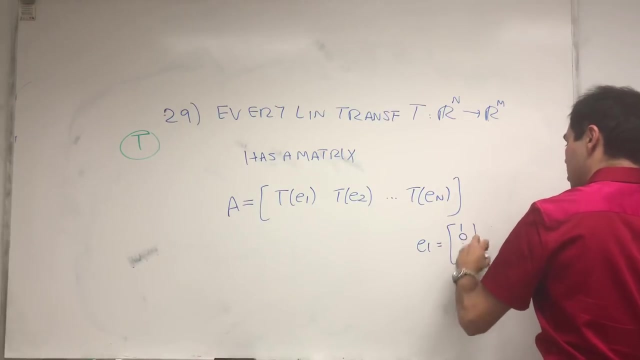 And how do you find that matrix? Simply, you evaluate t at every basis vector. So you do t of E1, t of E2, dot, dot, dot t of En, where again E1 is just, you know, 1,, 0,, 0.. E2 is: 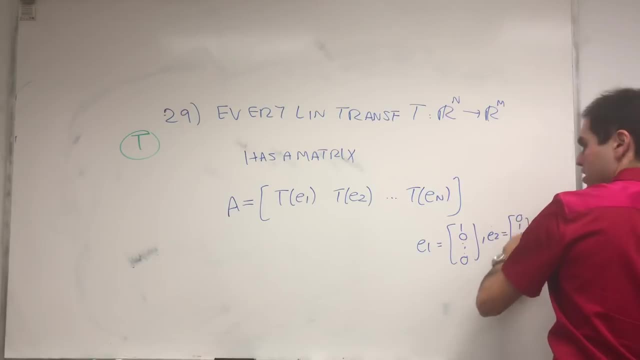 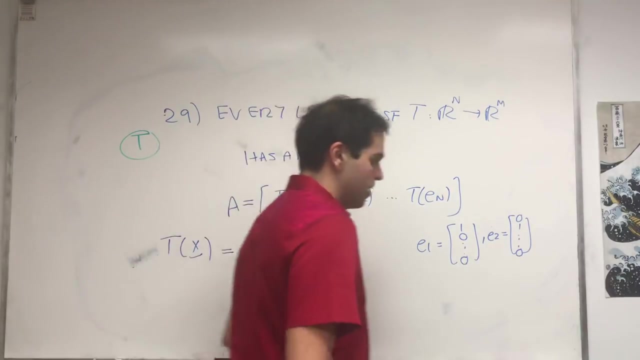 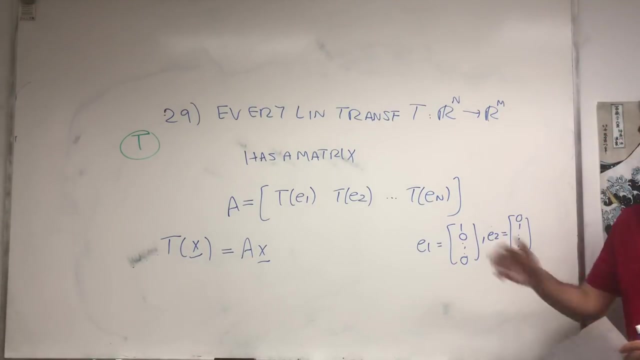 0, 1, 0, 0,, etc. etc. and then you can indeed check that t of X equals Ax, And this is the way, What This is what makes at least elementary linear algebra so useful. For any linear transformation you can extract a matrix. 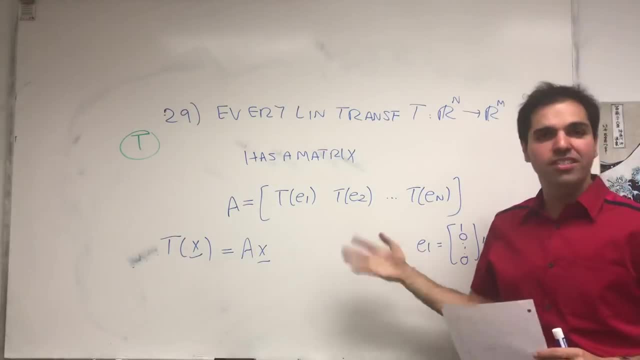 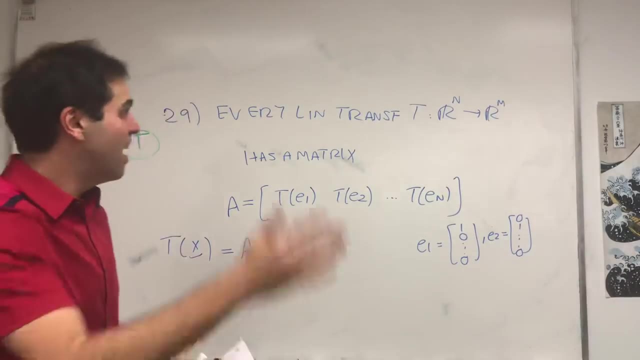 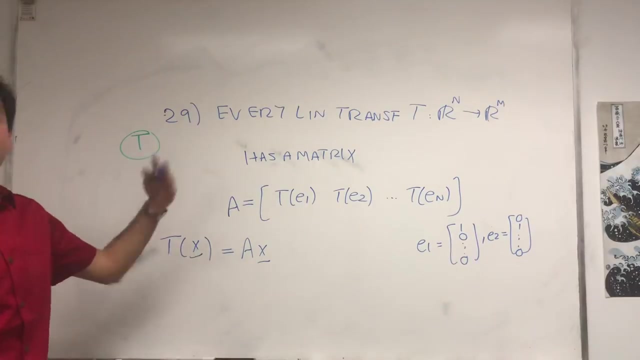 And then just any linear transformation questions just become matrix questions And, very important, this is false in general. It's really, you know, for linear transformations from Rn to Rm, So for infinite dimensional spaces you're kind of in trouble. 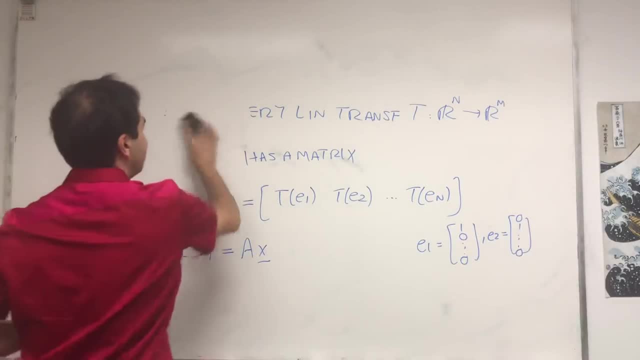 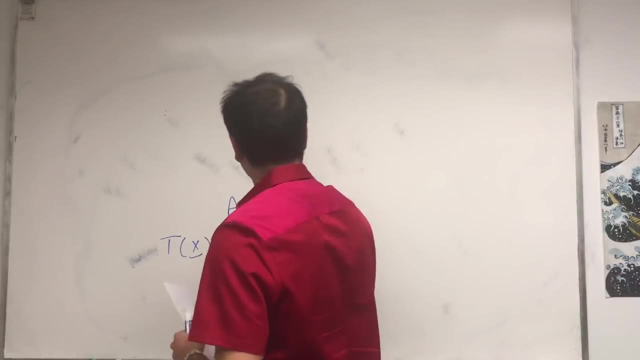 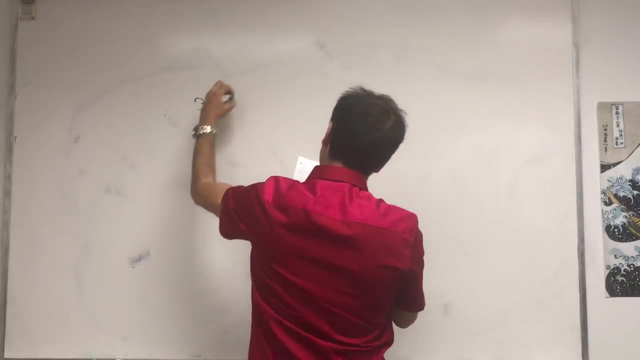 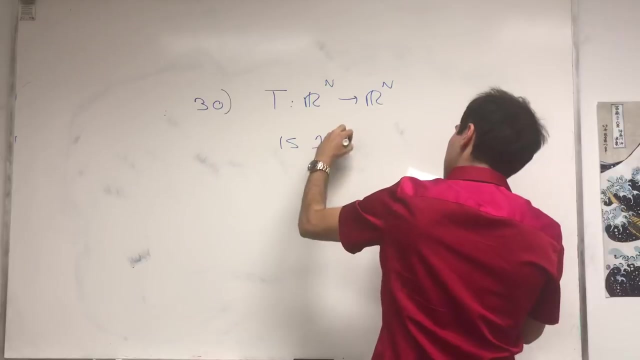 You can't always do that. That's why the calculus and analysis are kind of hard, Because we can't express a function just with a table. We need a lot of info for that. Okay, next question: If a linear transformation from Rn to Rm is 1 to 1, then T is on 2.. 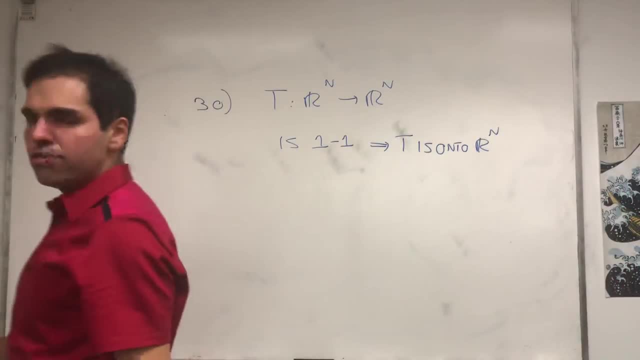 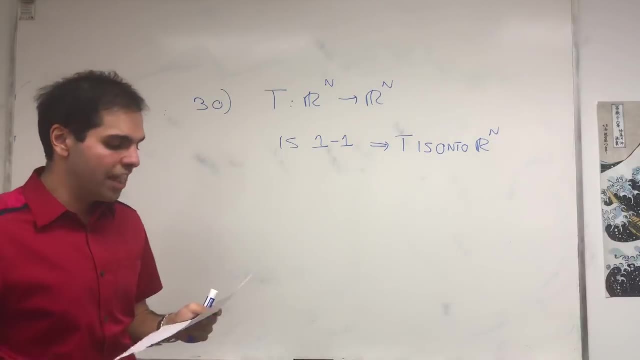 In other words, in this case from Rn to Rm. does 1 to 1 imply on 2?? And 30th language a dialect of Chinese, again the Hakka dialect, And 30 is Sam Su Or Sam Su, something like that. 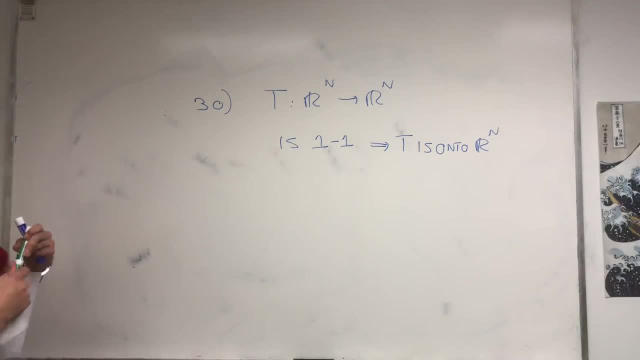 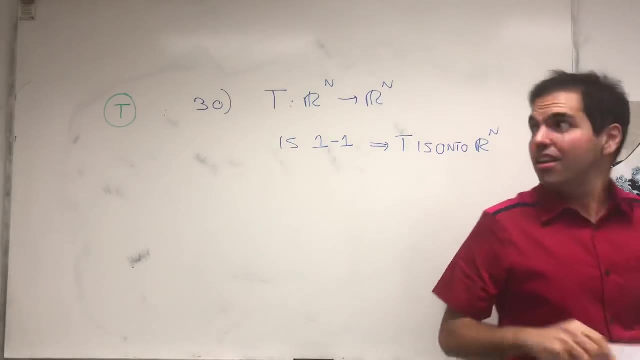 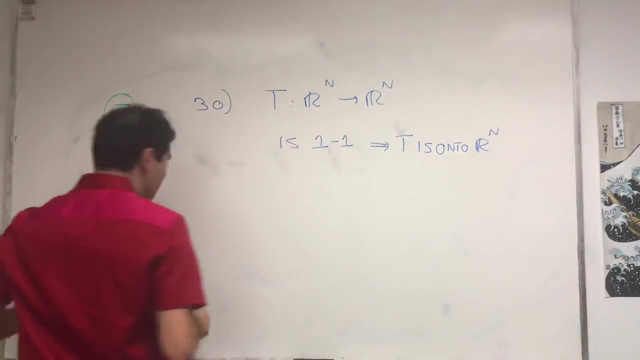 And here's a cool thing- This is actually true. So even though 1 to 1 and on 2 are two different things for Rn to Rn- they're actually the same. And the way to deal with this- again, remember use the fact that T has a matrix. 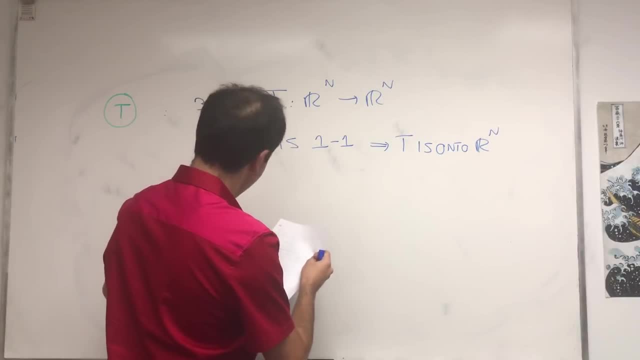 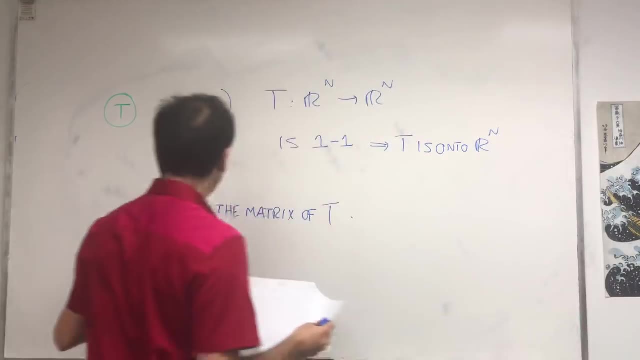 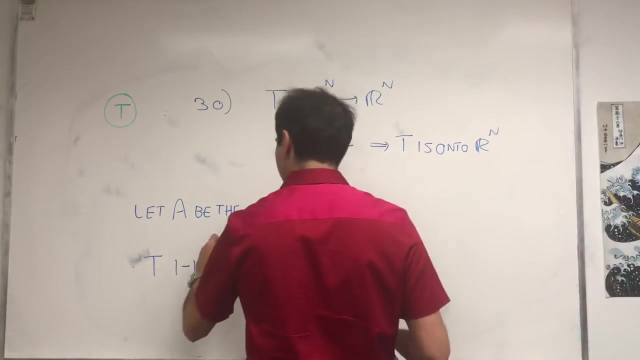 So let A be the matrix of T Of T, Then T 1, 2.. Rn 2, 1.. Well, there's this beautiful theorem called the invertible matrix theorem that gives us like 20 conditions for a square matrix to be invertible. 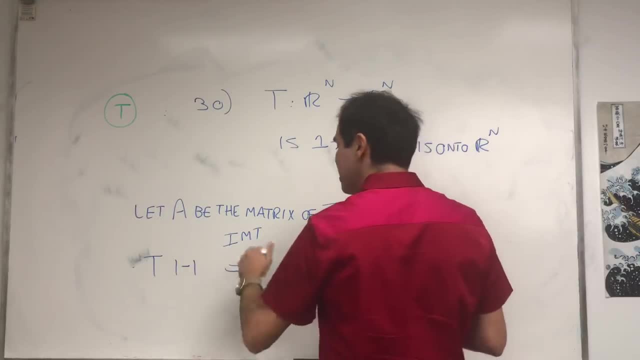 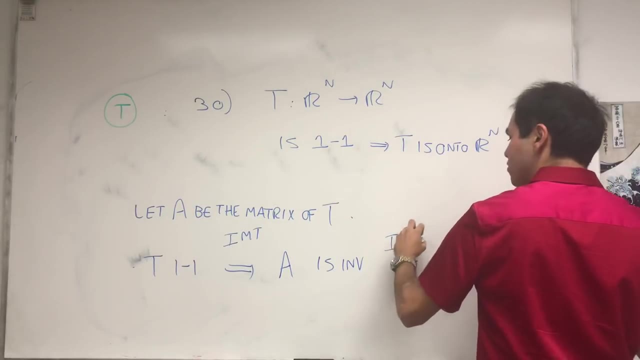 So if the linear transformation associated to A is 1 to 1, this means A is invertible. And another one of those conditions is, just say, that T is on 2 Rn. So important? The important thing is that here the dimensions of Rn and Rn are the same. 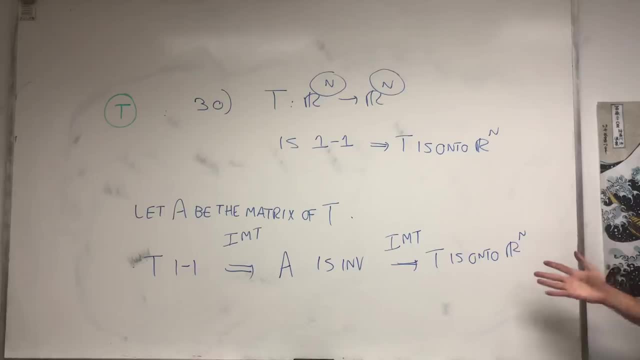 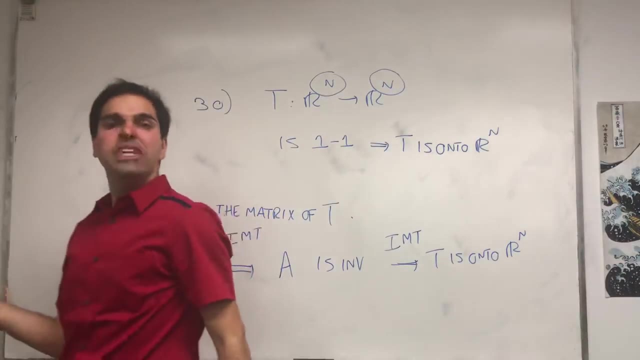 In general this is false. So there are linear transformations which are 1 to 1, but not on 2, and vice versa. So the invertible matrix theorem is kind of nice. It's a buy 1, get 23 kind of deal. 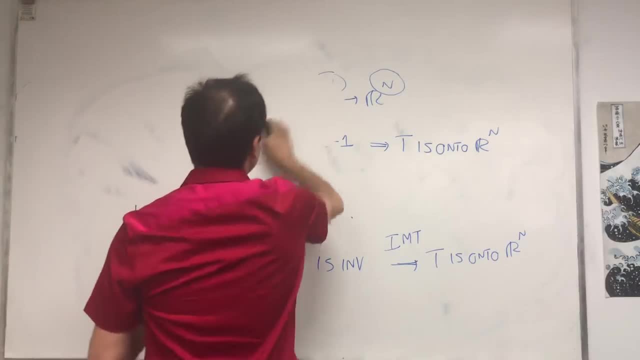 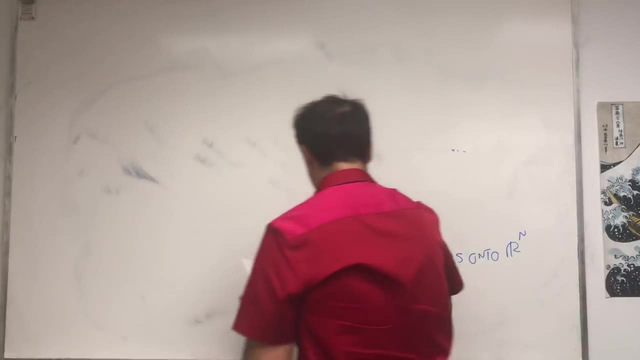 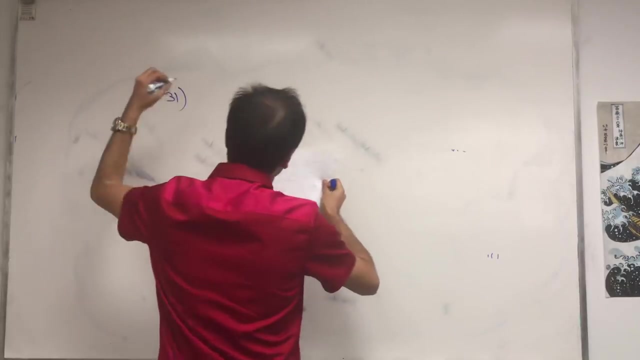 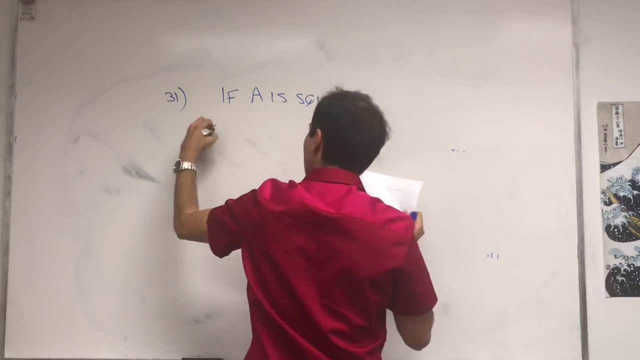 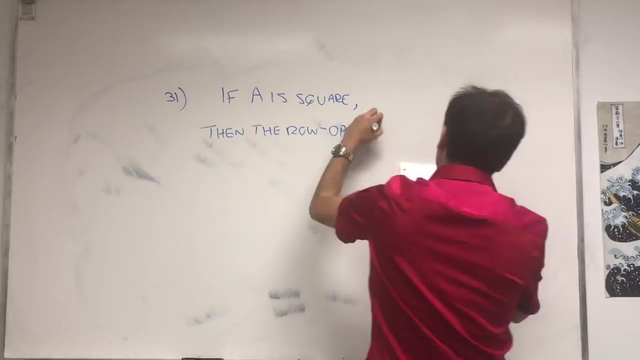 Good, We're almost done with part 2.. So just two more questions. We're going to talk a little bit better about problems with functions. So if A is squared, then the row operations operations that transforms. So no, if you transform. 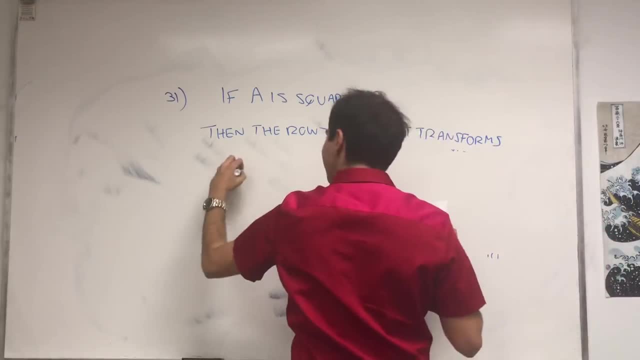 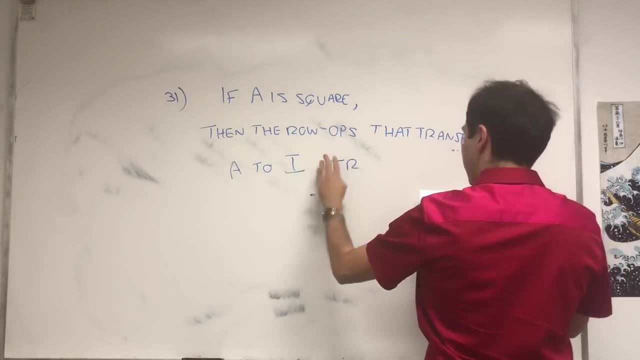 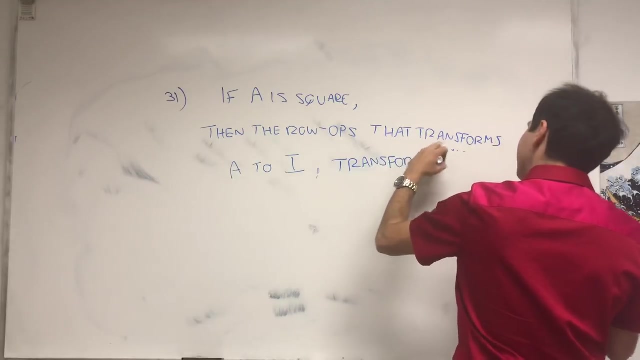 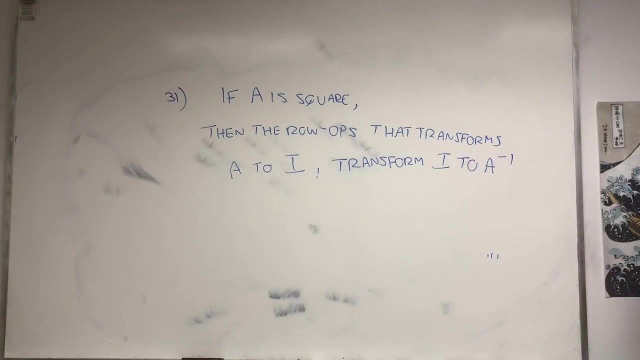 You're awesome. Yes, That's all, Thank you. And if we write it on top value, then what? Now we'll put in a value One, That one to the identity, then the same operation transforms, the same operations transform the identity to a inverse. Long question, but not too bad actually, and I 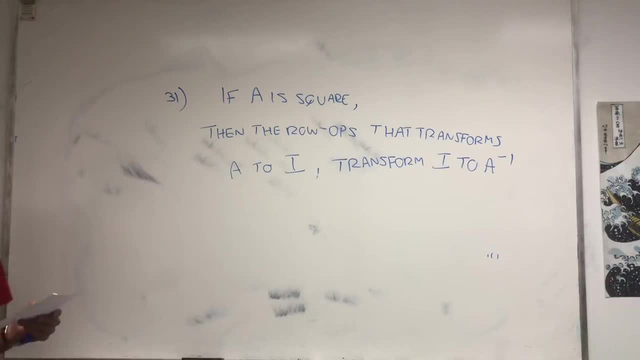 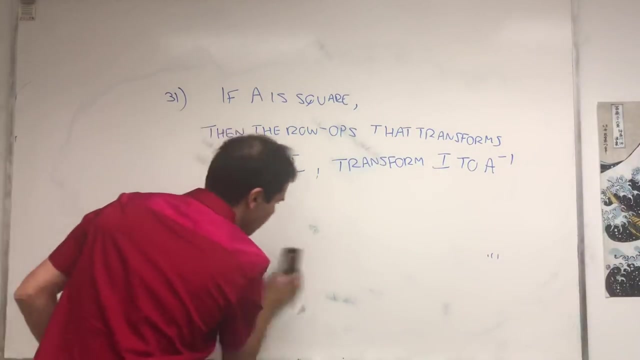 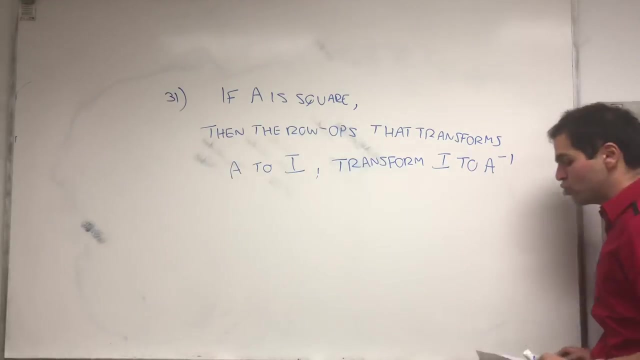 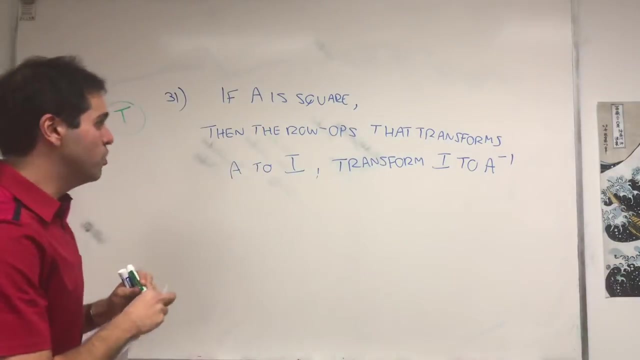 think language 31, so Canada, so not Canada, but Canada or Canada, and 31 in that language is MUATU. okay, and it turns out this is true, and that's what makes the algorithm for invoices, The converting matrices, true, because if you remember the algorithm for finding a, 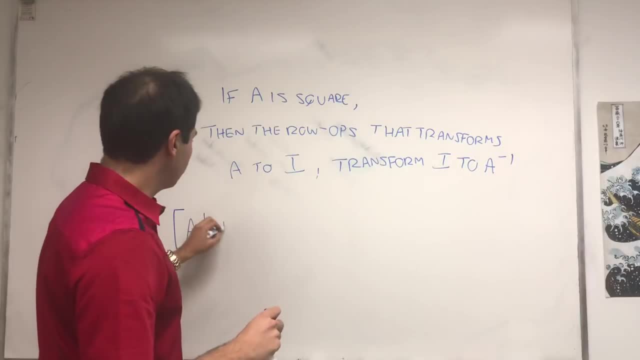 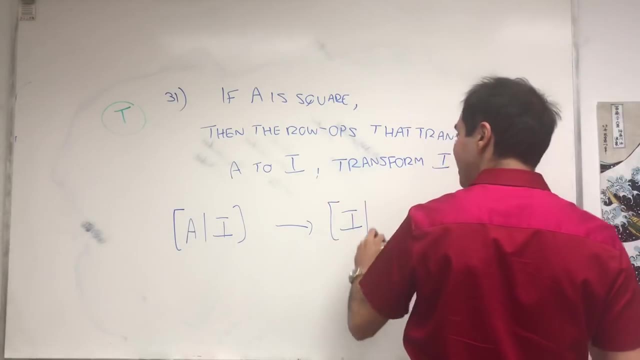 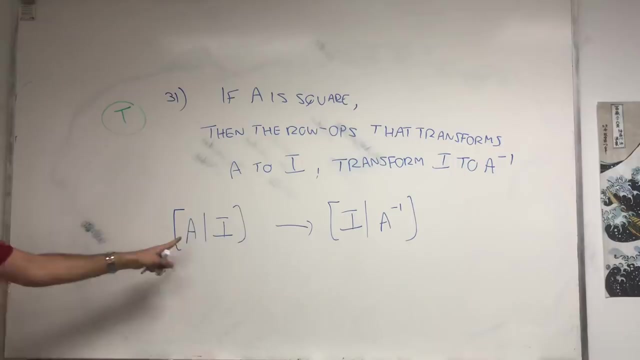 matrix inverse. you do a on the left hand side and I on the right hand side, and with row operations you try to find the identity on the left hand side and a inverse on the right hand side. and this is precisely what this is saying: any row operation that transforms a to the identity transforms the identity to a. 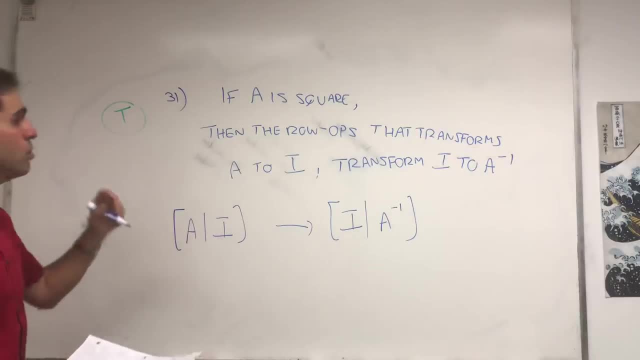 in inverse and if you want to use another proof, so remember, row operations, you can write them in matrices. so, basically, all those row operations, you can write them in terms of a big matrix. and, in particular, what is the same, if you apply the row operations of B to a, you get the identity, but because a is, 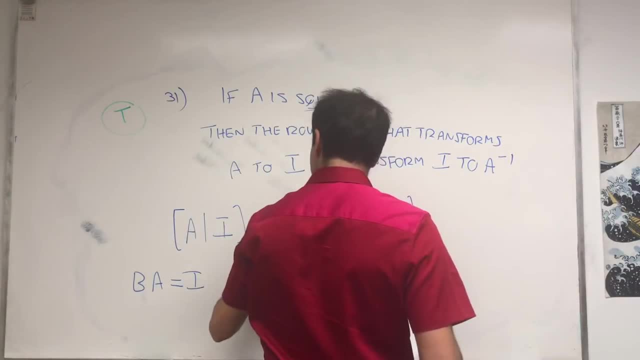 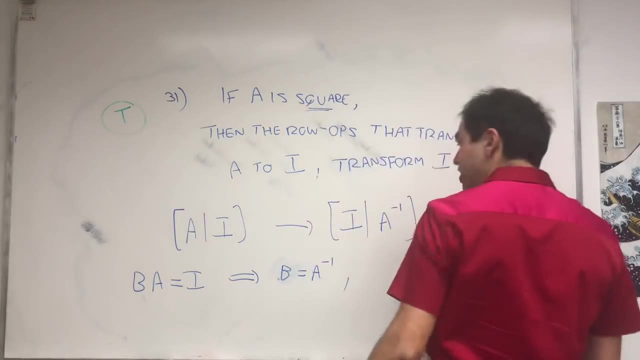 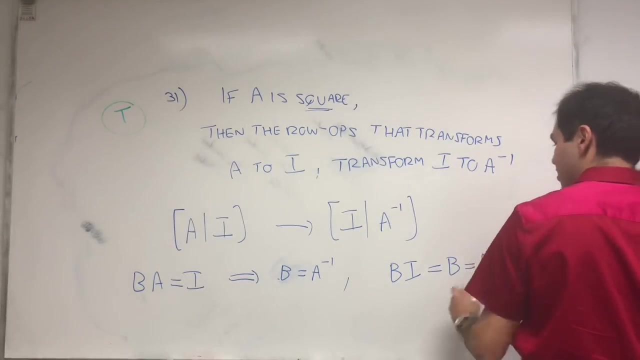 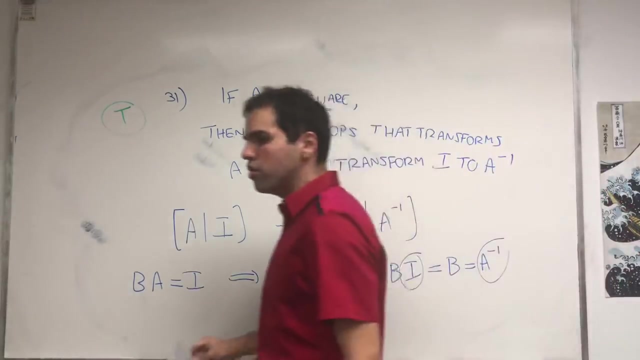 square. this is enough to conclude that a that b is a inverse. and then if you apply B to the identity, you get B, which is a inverse. so B transforms the identity to a inverse. this is useful to think about. you know, matrices, they're not just tables, they're like active things. 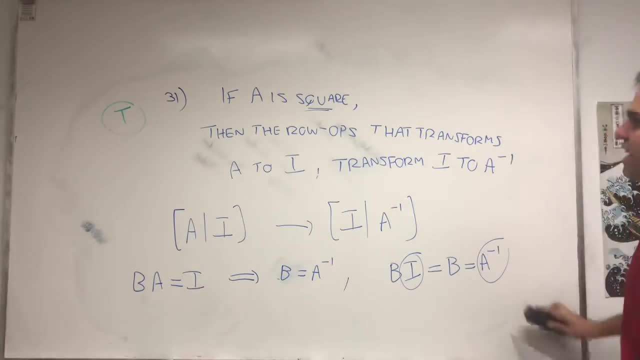 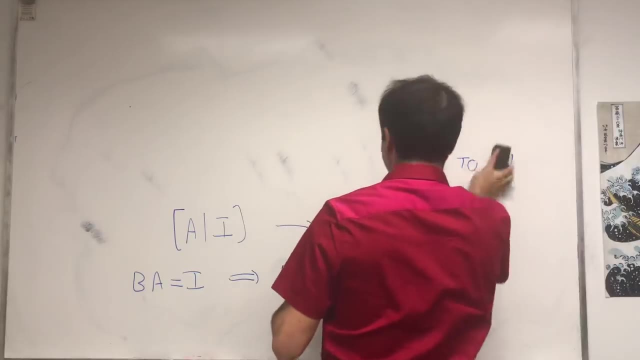 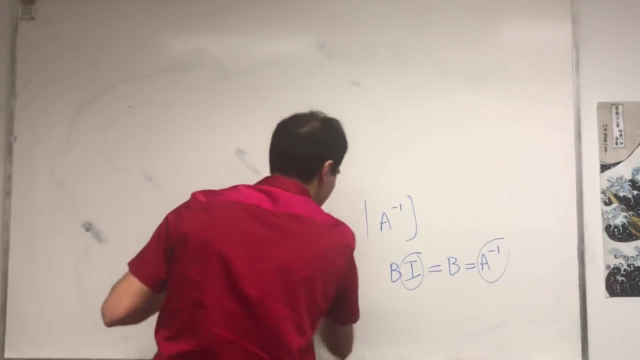 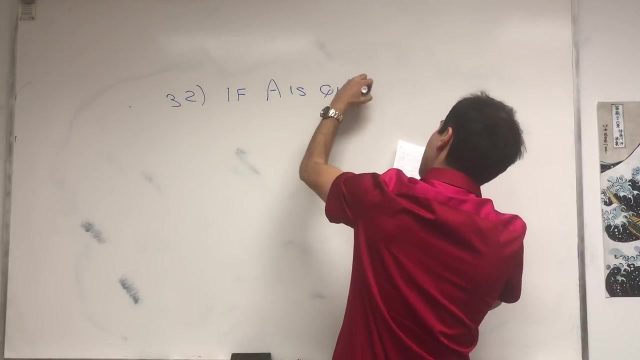 like non-native, things transform things. So here B transforms the identity to A inverse. Okay, last one, question 32, so last one of this section. So if A is square and it has a property that A x equals 0 has only the trivial solution, then A is. 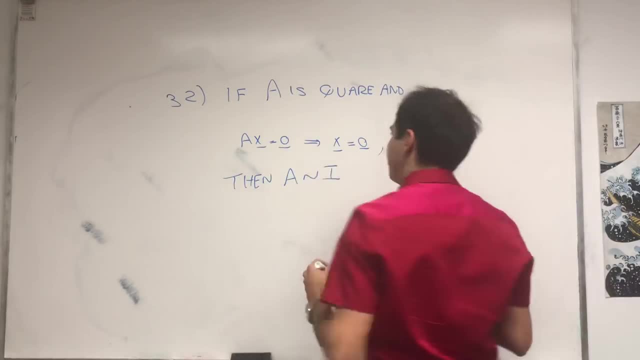 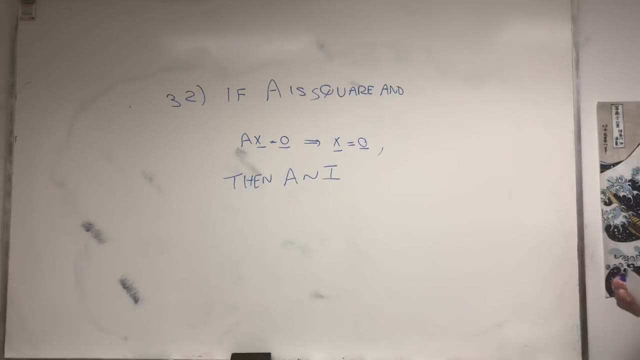 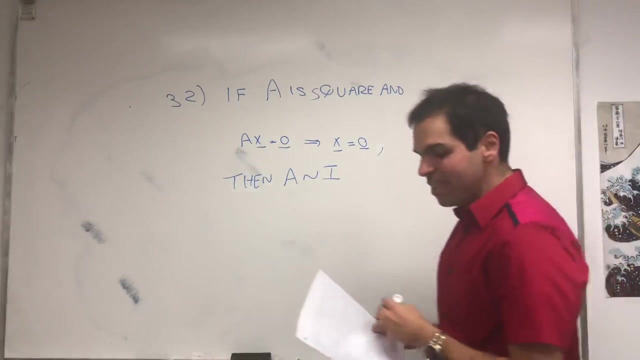 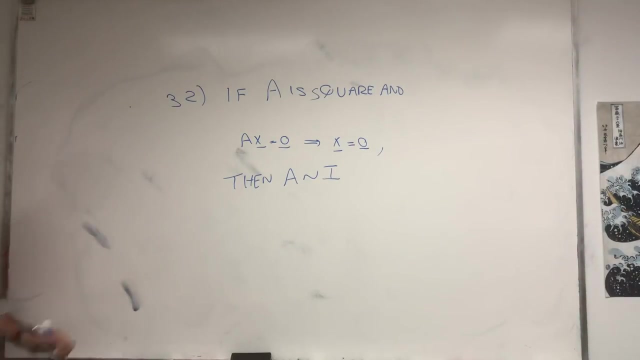 row equivalent to the identity. In other words, for square what is quare? No square. If the null space of A is a trivial space, then A is row equivalent to the identity. language. 32, 32 is aurea. it's interesting, almost like Orion or something, but 32 in aurea is. 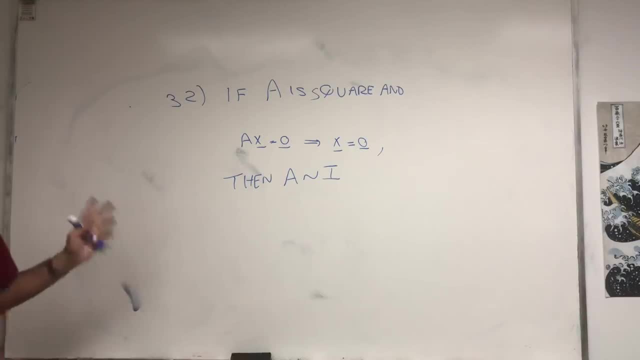 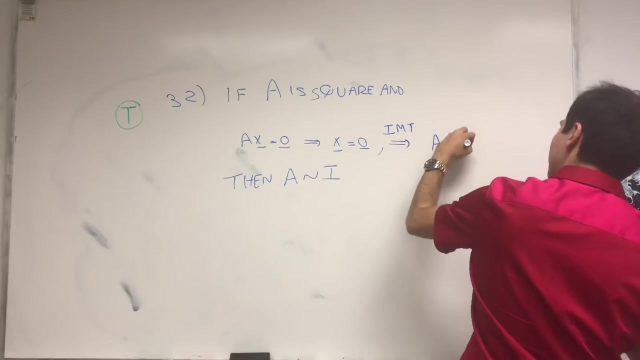 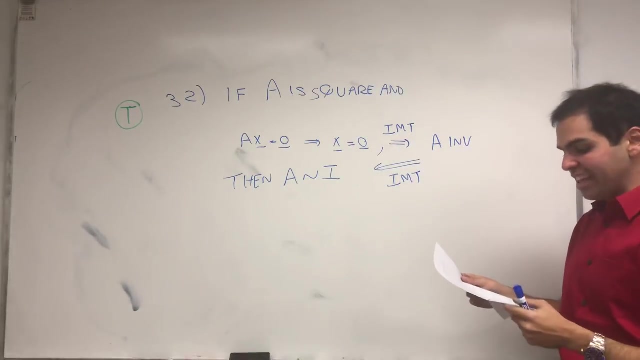 partice And because the matrix is square. this is actually true and basically what happens? this property, by the invertible matrix theorem, implies A is invertible, and again by the invertible matrix theorem we get that A is row equivalent to the identity and we're done. But, very important, this is not true in general. 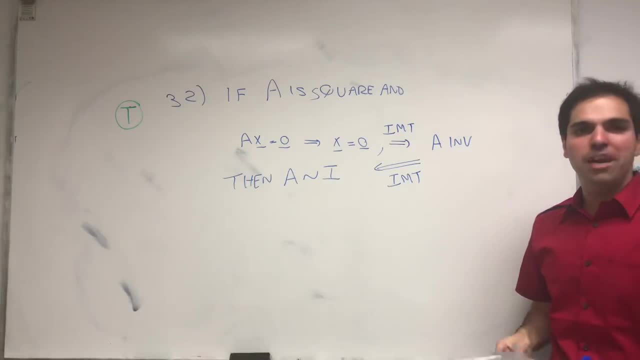 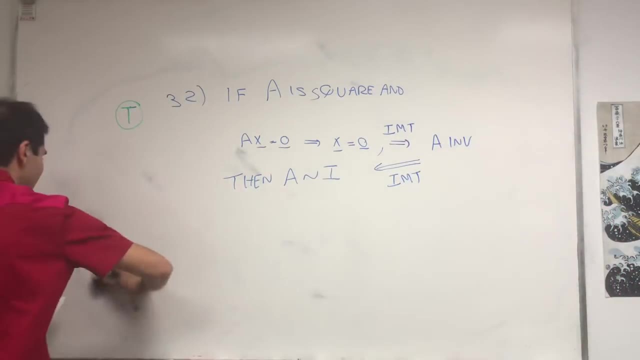 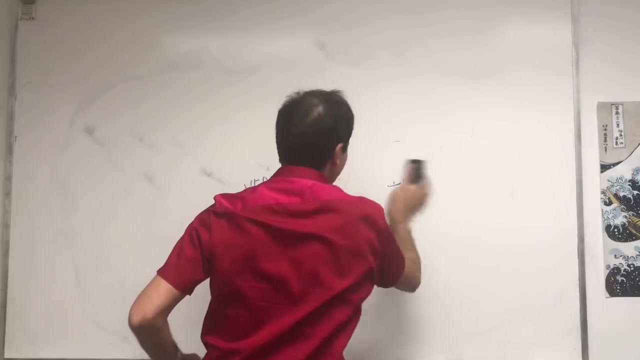 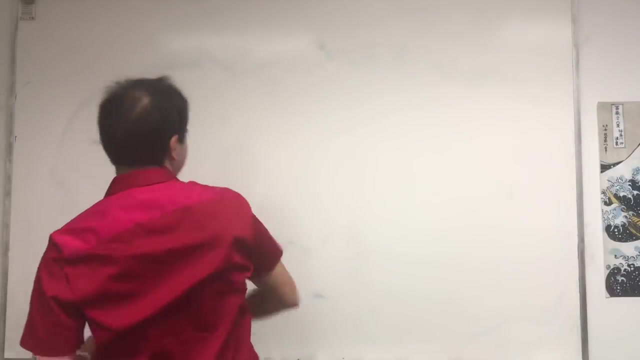 for non-square matrices, like the previous example I've shown with this, no-space of A is zero, but A is not invertible. Great, so that was the second part. let's move on now to determinants. Oh my god, I'm dying. What has Steve done to me? 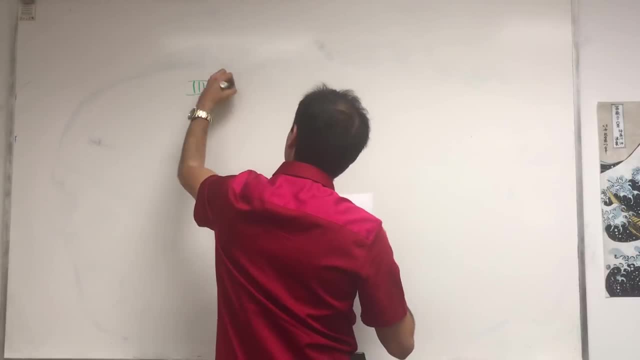 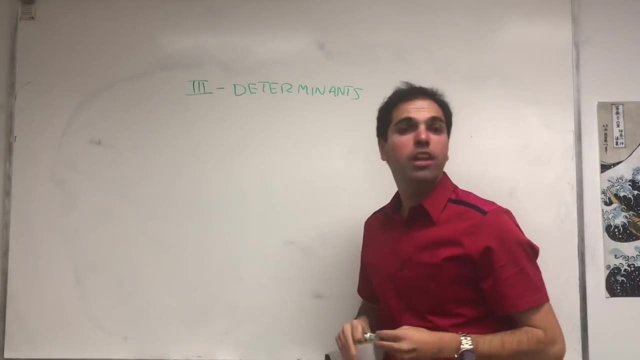 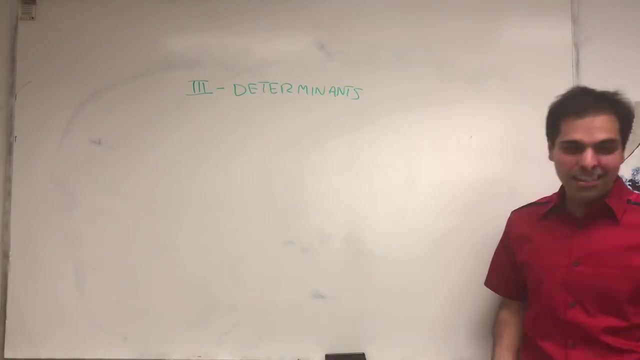 So determinants. By the way you know, I'm supposed to write the final exams now, but look how I'm procrastinating. So even professors they procrastinate. And that said, give me one second, I need to eat something. 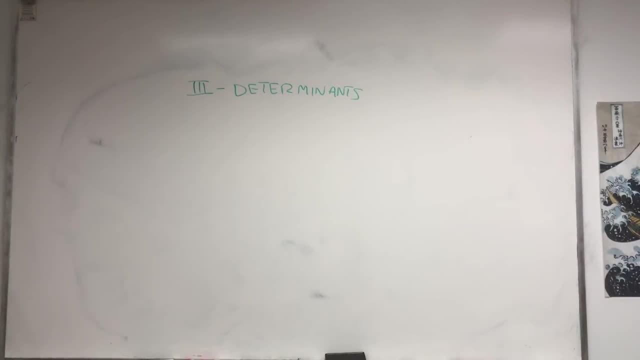 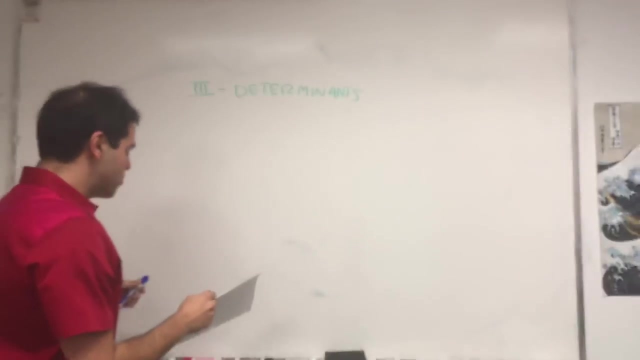 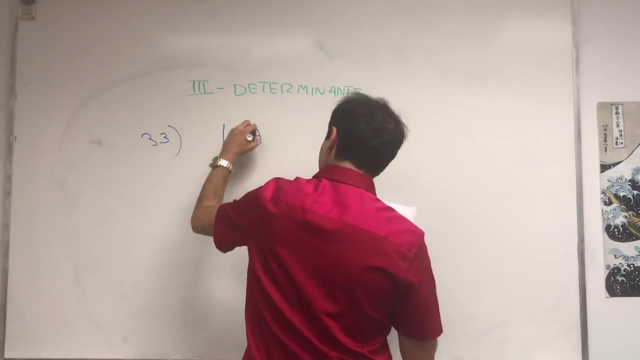 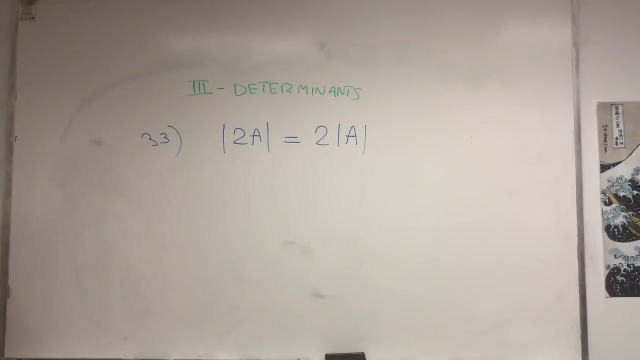 I'm not hungry, I'm not talking for two hours. You're making me crazy. Gotta have my nuts Anyway. so question 33.. The determinant of 2 times A is 2 times the determinant of A. So absolute value here means determinant and assume here it's bigger than a. 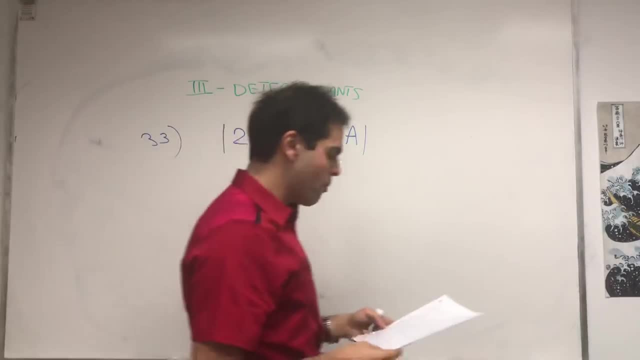 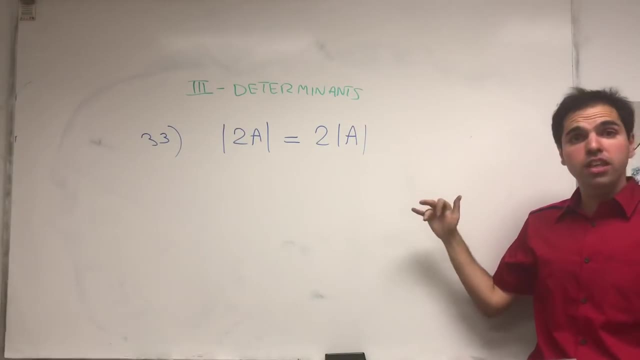 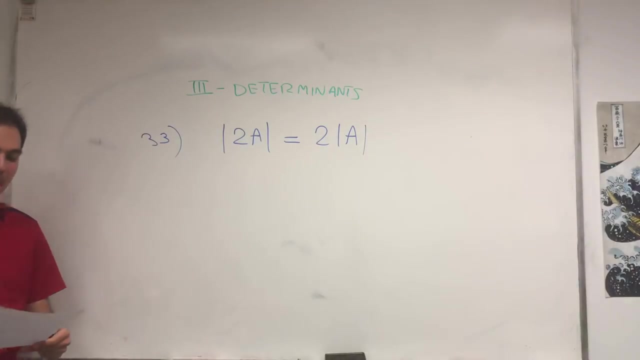 one-by-one matrix. so Language 33 is Punjabi, the western part of Punjabi. There'll be an eastern part very soon, And this is I love this one. 33 in Punjabi is tetti Tetti. How cool is that. 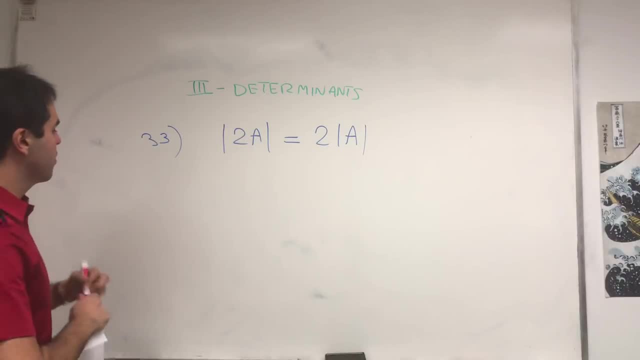 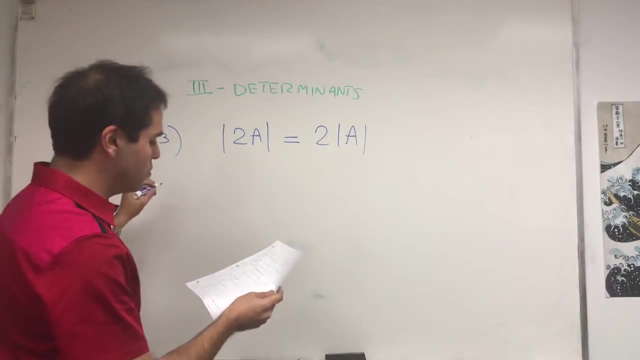 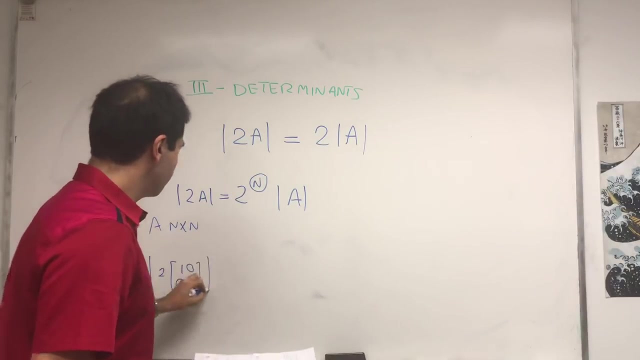 That said, unfortunately this is false. Let me give you an example. So basically it's false because the determinant of 2A is 2 to the N times the determinant of A, where A is N by N. So, for example, determinant of 2 times the identity, it's determinant of 2, 0, 0, 2,. 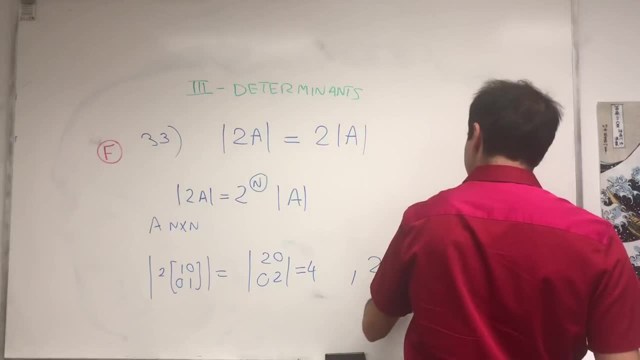 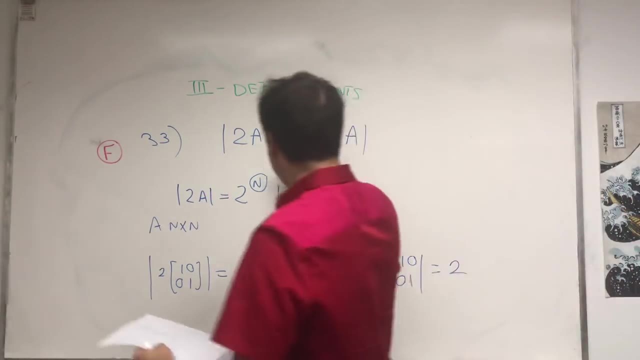 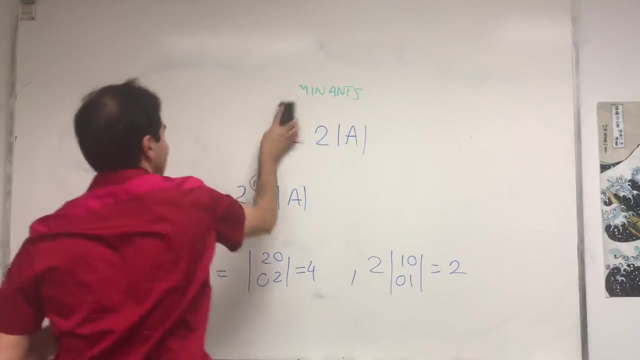 which is 4, but 2 times determinant of the identity is 2.. 4 is not 2,, therefore it's false. So careful, determinants are not linear in that sense. If it's linear, you can just pull out the constants. but that's not true. 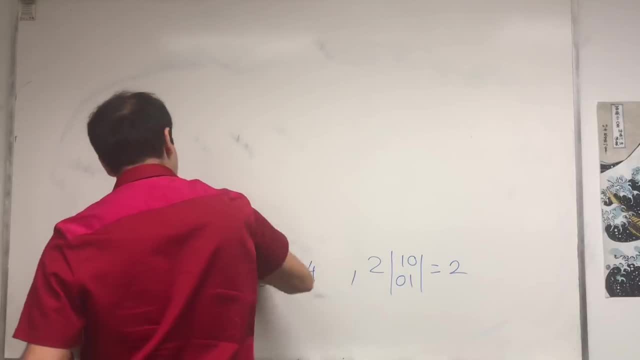 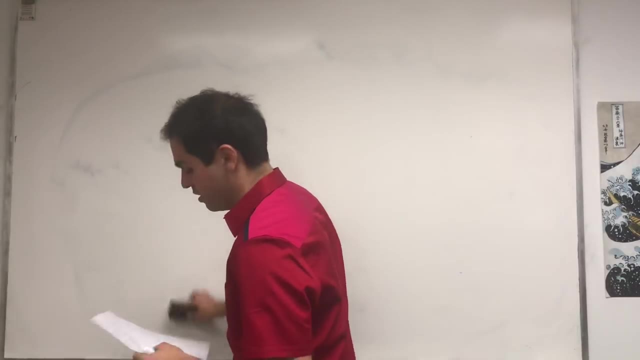 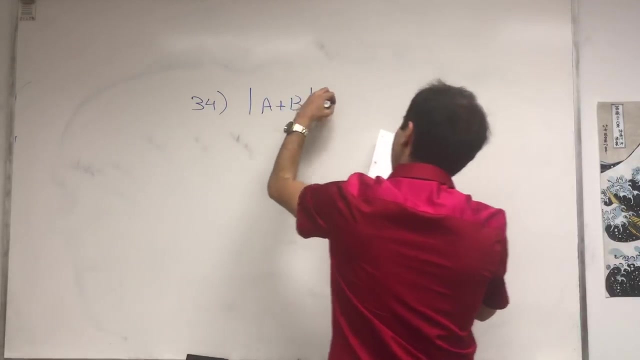 They're what are called? Is that like multilinear or something where for each row you can take out the constant Okay and you're like: well, could it be? additive Is determinant of A plus B. is that determinant of A plus determinant of B? 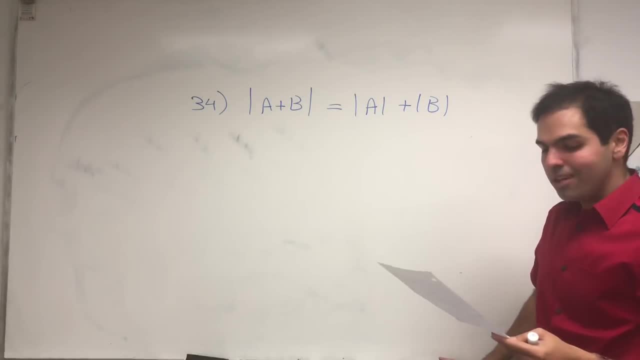 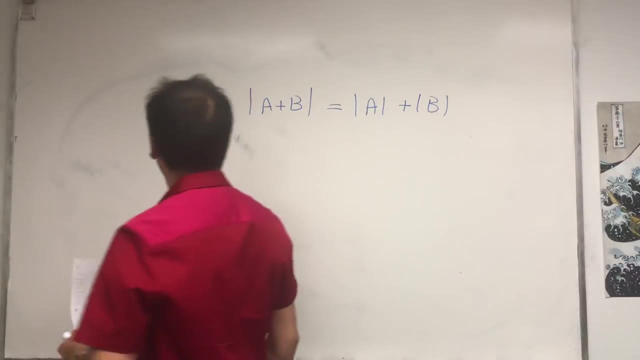 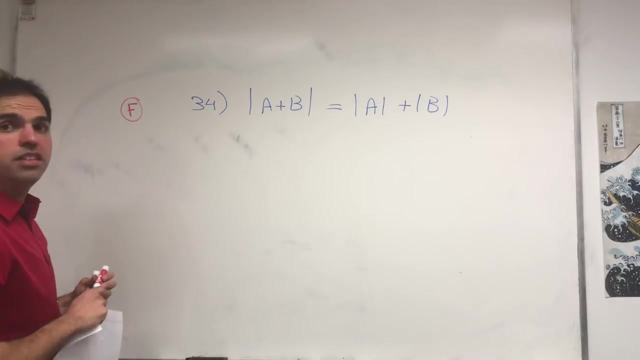 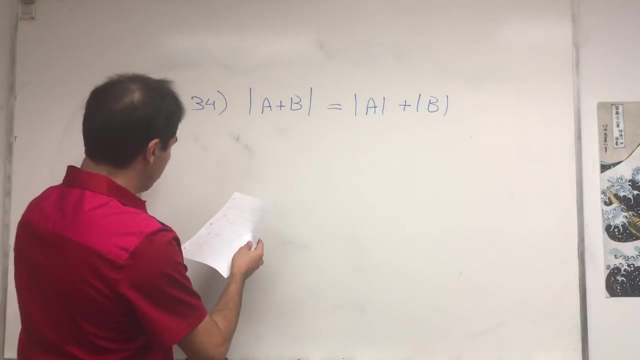 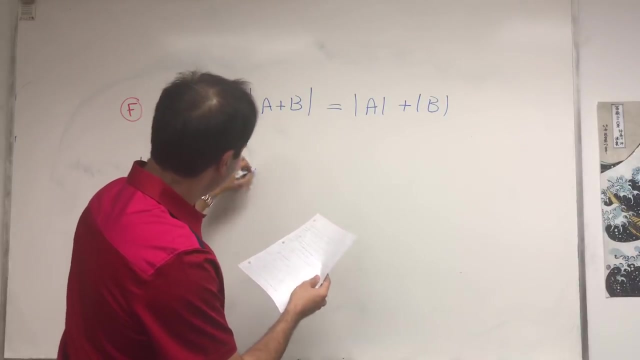 And language 34, sunda, and 34 in that language is tiga pulu mpa So tiga, And this is also false. Determinants are neither multiplicative, well, neither linear, nor additive, because, for example, if you have 1, 0, 0, 0 plus 0, 0, 0, 1,. 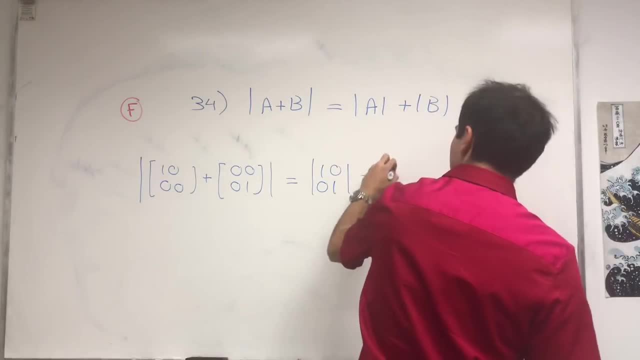 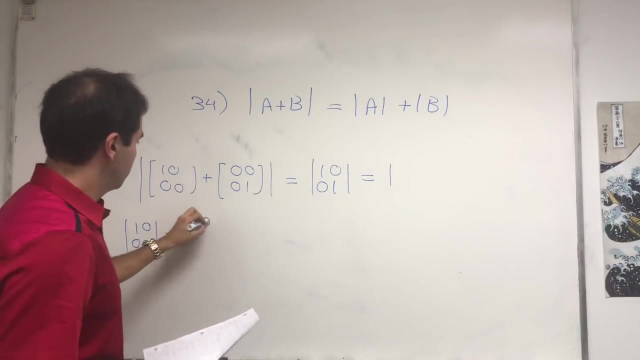 if you add them, you get the identity and the determinant is 1, but the determinant of each of them 0, 0, 0, 1, that's 0 plus 0, which hopefully we agree is 0.. 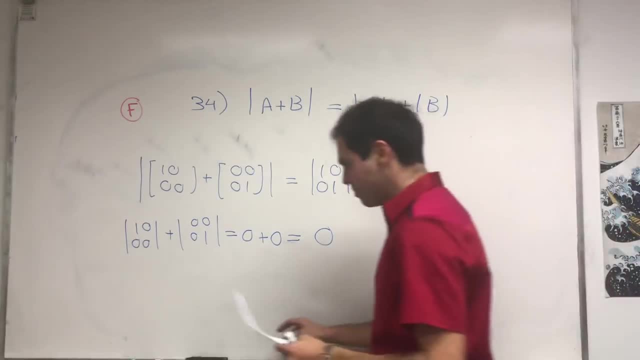 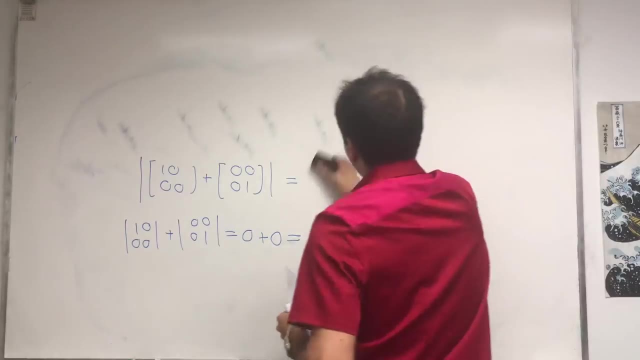 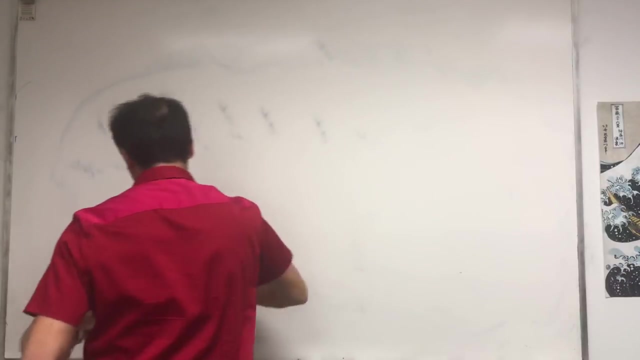 Those are not equal. therefore the claim is false. Ta-da, So determinants are very strange. Oh, we're not even half-third done. oh my god, I might have a chocolate cake shake after that to reward myself. Okay, question 35.. 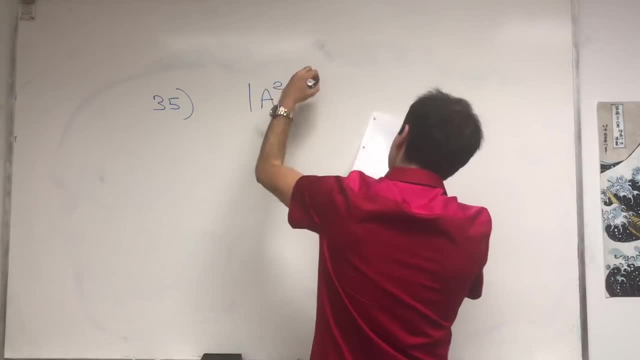 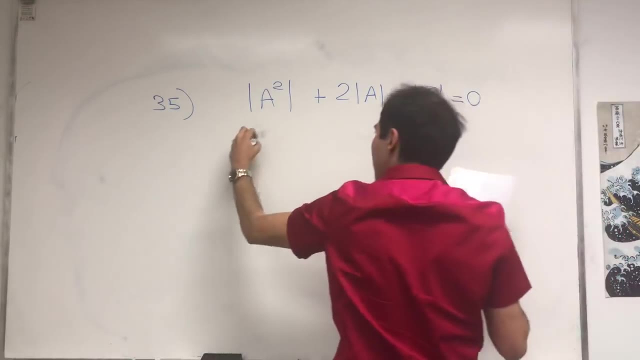 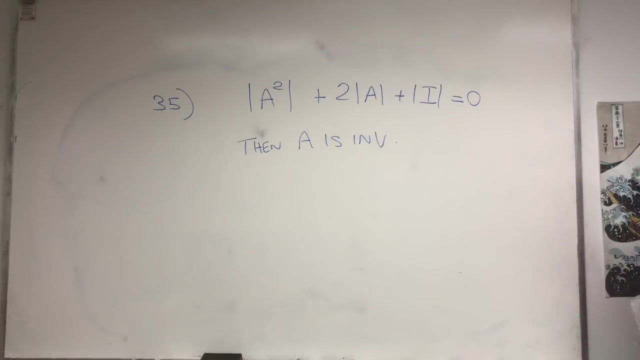 So if that's super interesting, if the determinant of A squared plus 2 times the determinant of A plus the determinant of the identity is 0, then A is invertible. Let's see And remember. I said there was this western part of Punjabi. 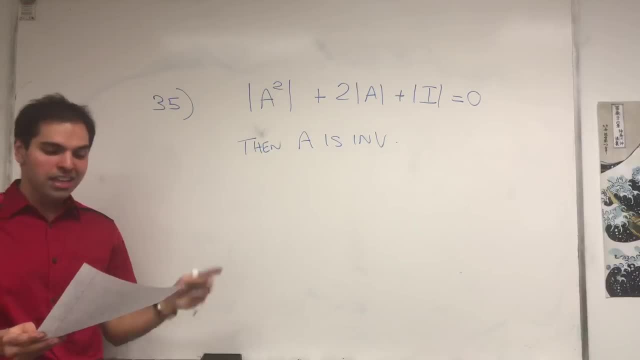 Well, for this question it's the eastern part of Punjabi and so 33 was tetti, 35 is pinti or pinti or something So weird equation we have that. Does that imply A is invertible? 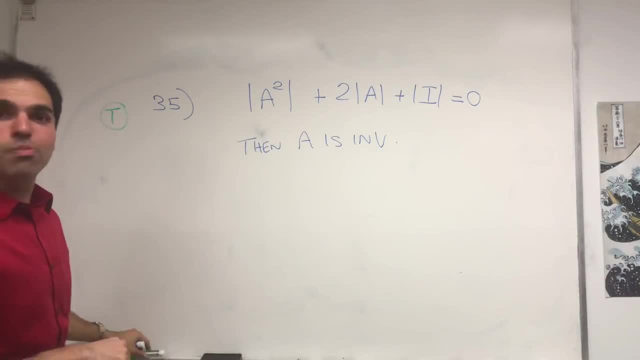 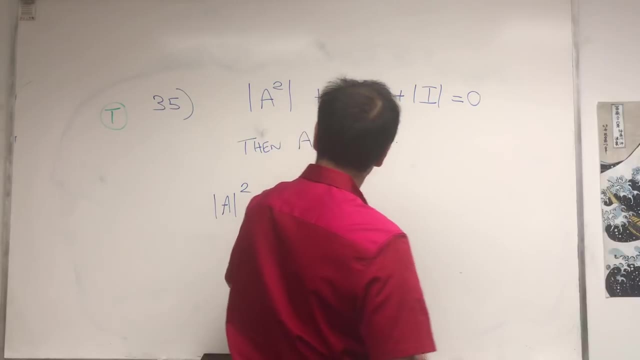 Indeed, this is true because just use the properties of determinants. This is the determinant of A squared plus 2 times the determinant of A plus 1 equals 0, but then let's just x squared plus 2x plus 1,. 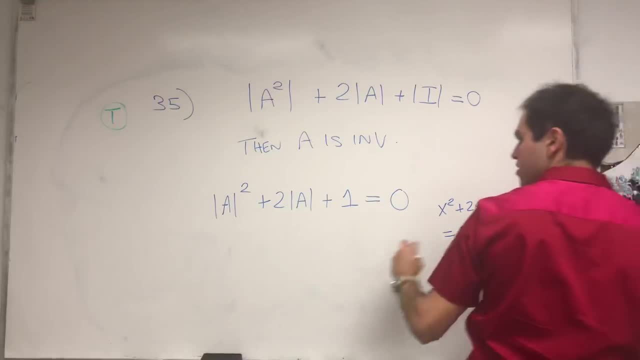 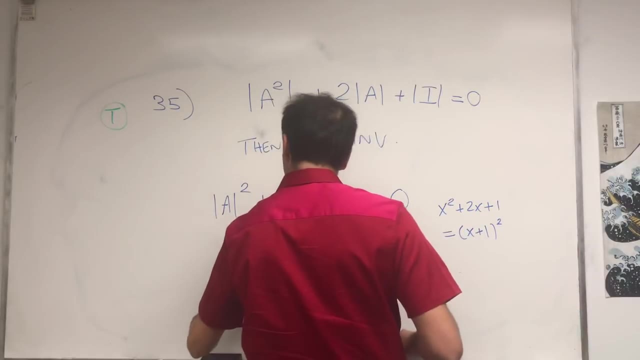 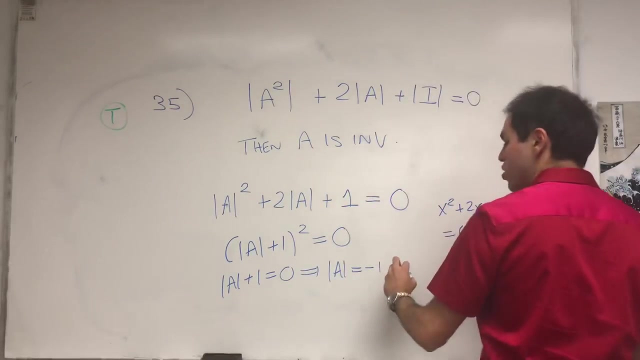 which you can write as x plus 1 squared. So we get: determinant of A plus 1 squared equals 0, so determinant of A plus 1 is 0, so the determinant of A is minus 1, and because the determinant is minus 1,, 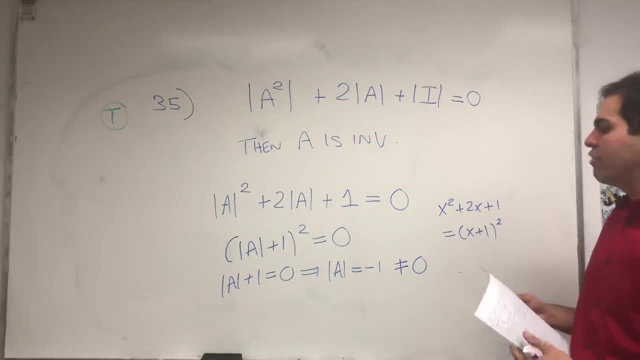 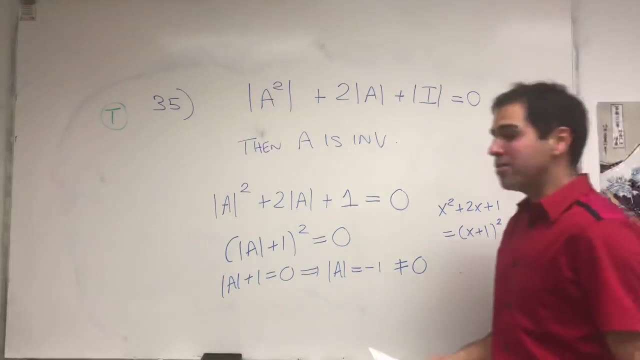 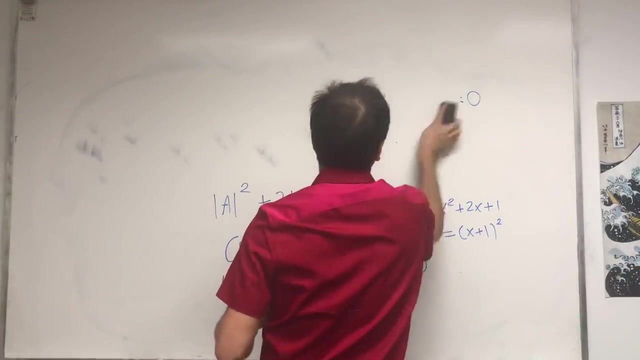 it's not 0, and remember, an easy way to check if a matrix is invertible is: is the determinant non-zero. So because it is non-zero, the matrix is invertible. That's a nice question. My students didn't like that at all. 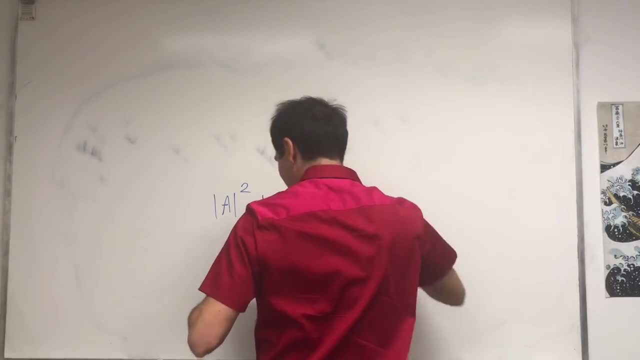 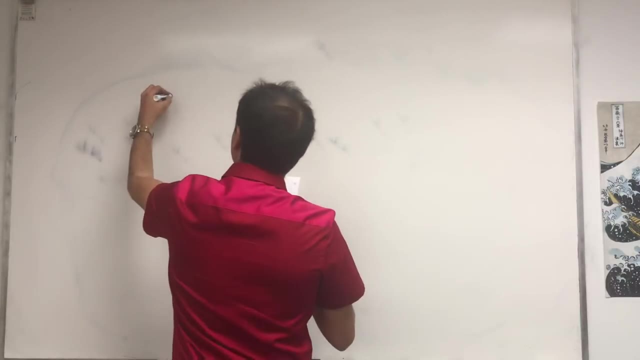 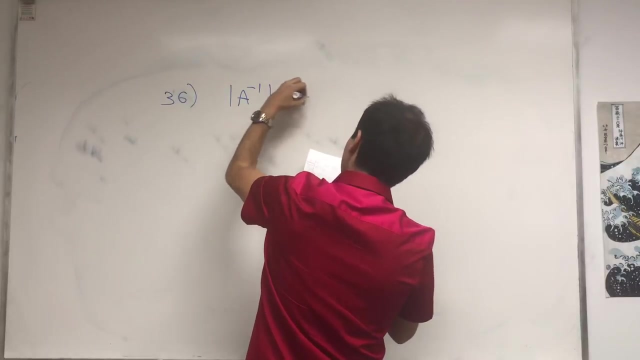 but I think it's cute. Next one, and also pretty quick. So actually, yeah, the next two ones are quick. So I think 36 is the determinant of A inverse equal to minus the determinant of A And 36, Romanian. 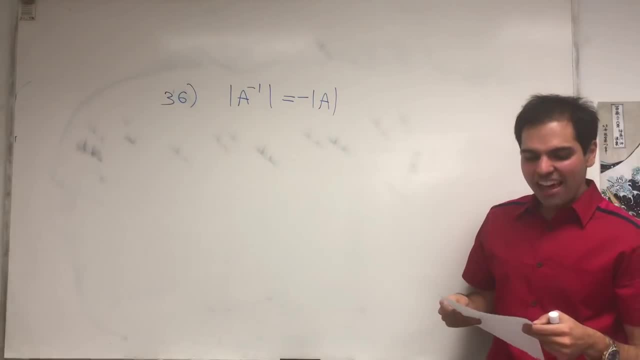 so shout out to Vlad, my Romanian friend, and 36 is sounds almost like French. It's like tres ci ci sa se, Or like tres ci ci sa se, Or almost like a tongue twister, I don't know. 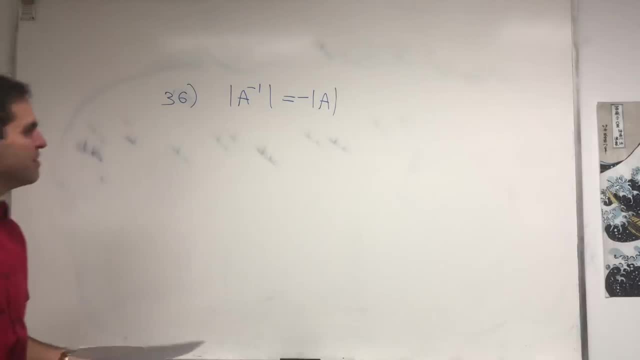 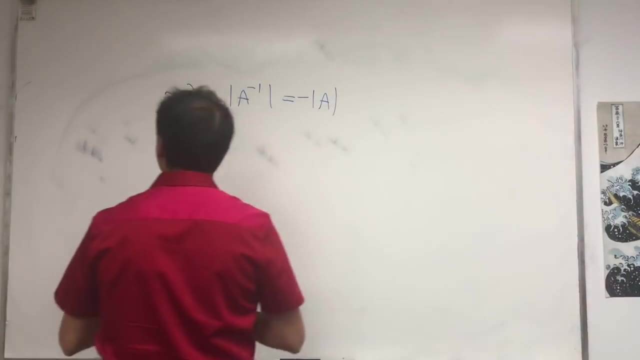 How much wood would a woodchuck chuck? if a woodchuck could chuck wood? I forgot all the German ones, Anyway. in any case, this is false Because the determinant of A inverse is not minus A, it's 1 over the determinant of A. 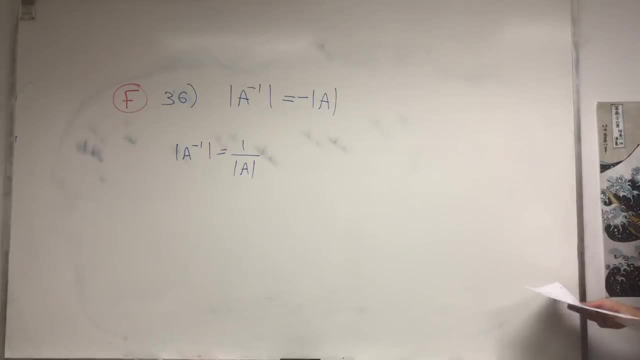 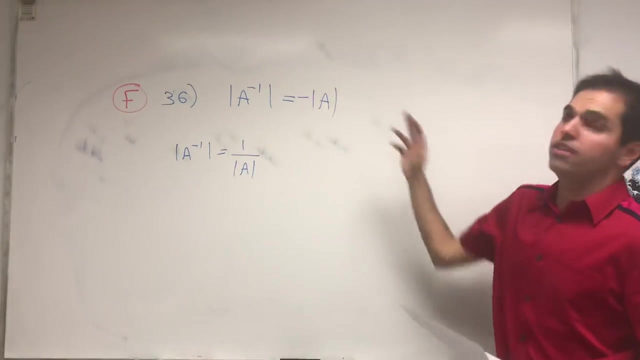 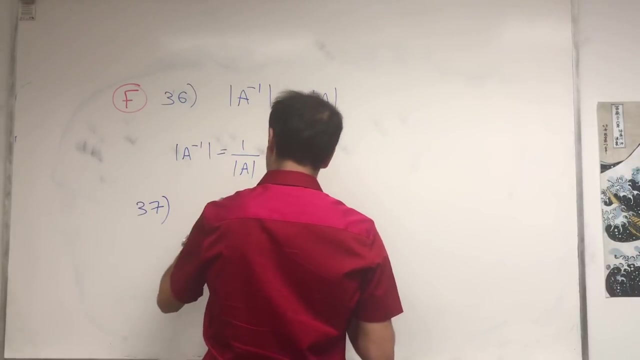 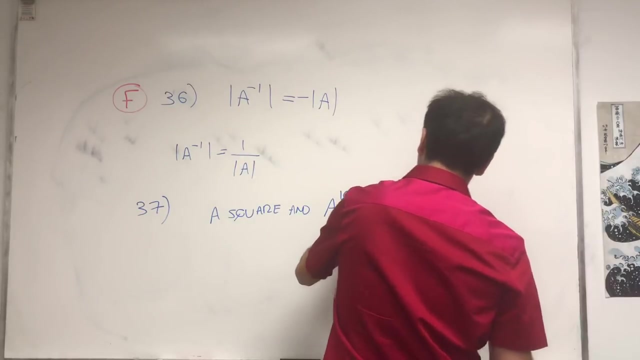 Okay, For example, the determinant of the identity inverse is the determinant of the identity, which is 1, not minus 1.. Next one, Also cool. So if A is square and A to the 100th is invertible. 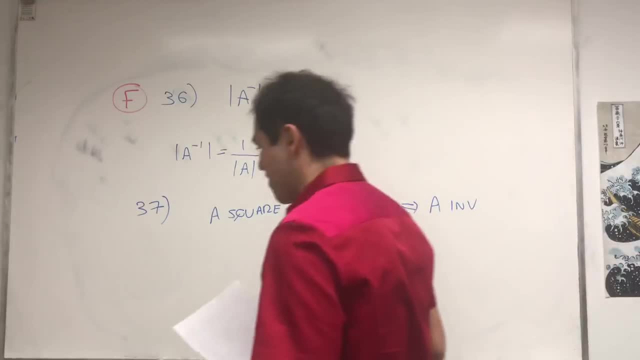 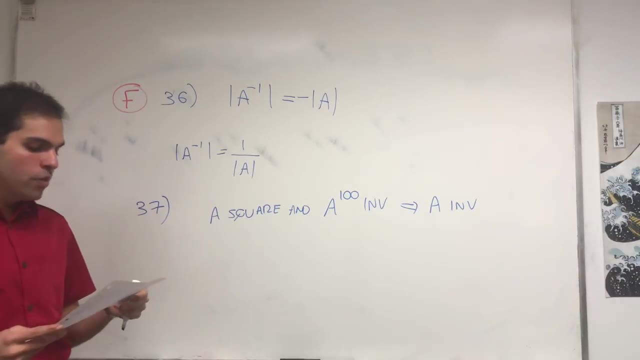 then A is invertible. Anyway, there are many other ways to prove or disprove it. So language 37, butchpuri, like potpourri almost, and 37 is cetis or cetes, 100% sure. 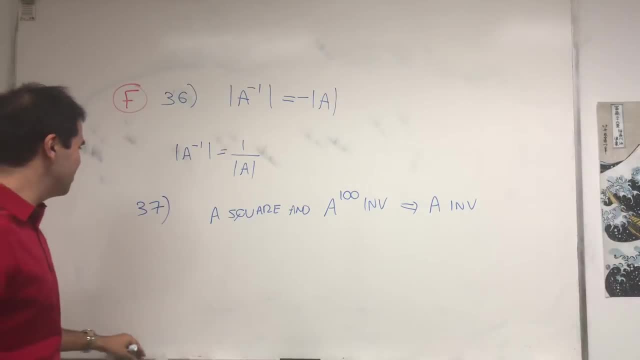 But we are 100% sure that it's invertible. So true Why? Because what do we know? We know that A to the 100th power, because this is invertible, that's non-zero. but this thing is just. 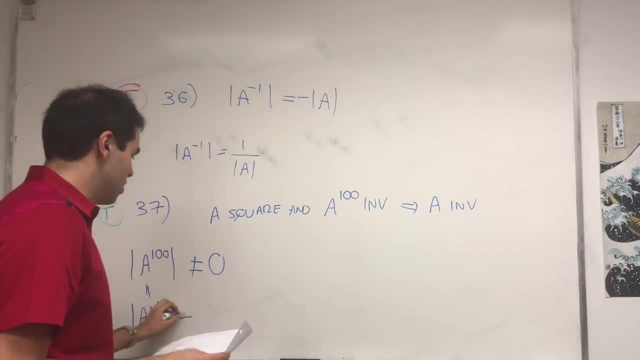 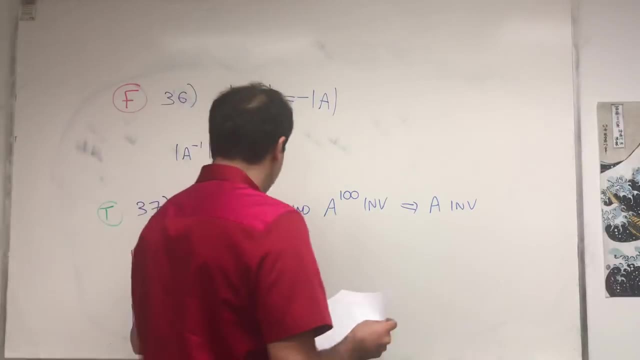 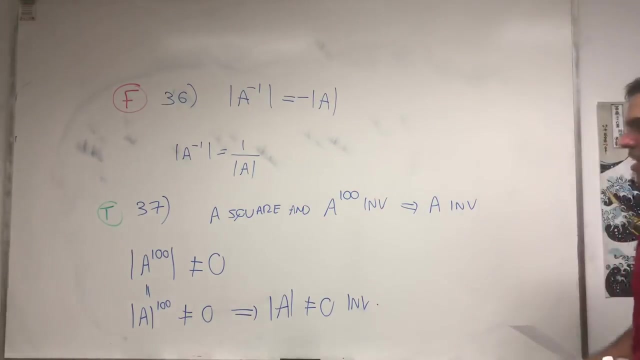 the determinant of A to the 100th power, because it's multiplicative. So basically, X to the 100th is not 0, so in particular, X is non-zero, Invertible, And the next two just have to do with. 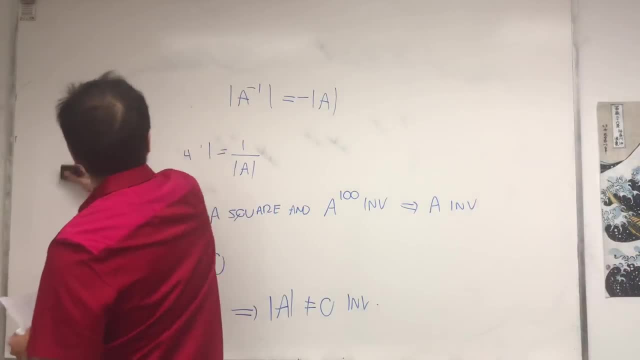 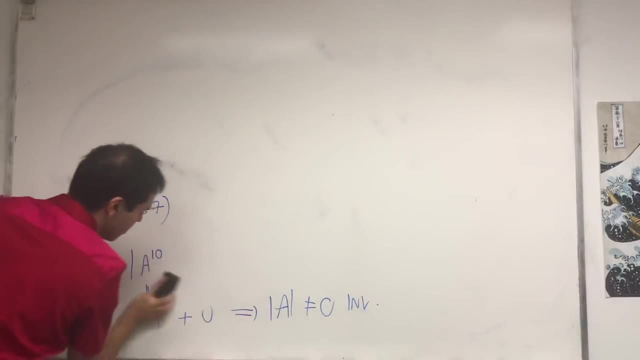 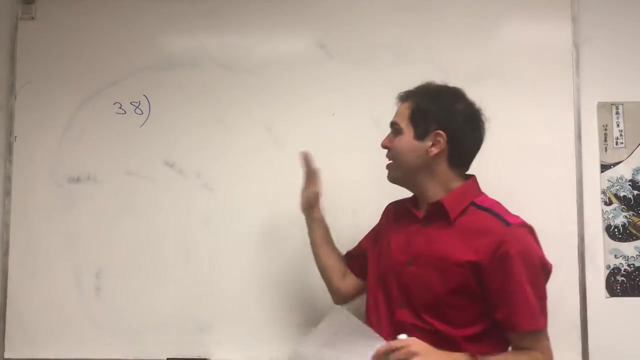 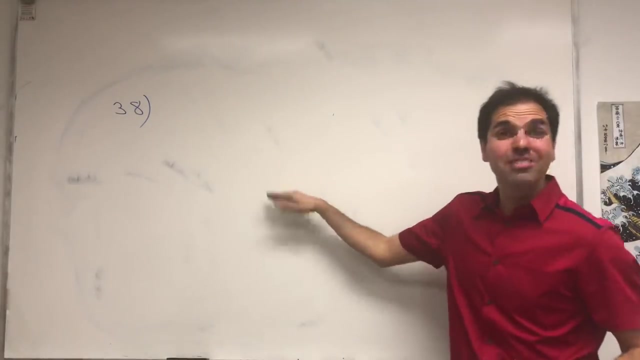 applications of determinants. So Awesome, By the way. it's possible that my phone like runs out of memory. So hopefully not, but it's possible. if it's too long, I may have to do it in two videos, I promise you. 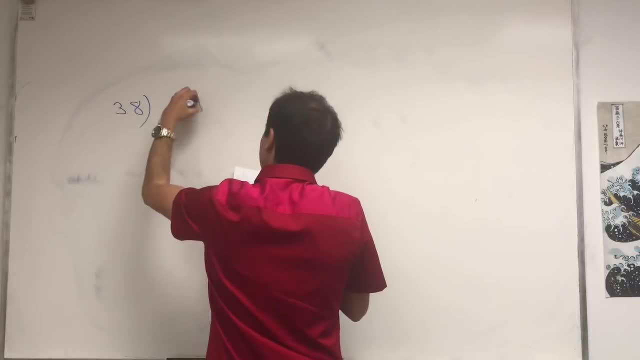 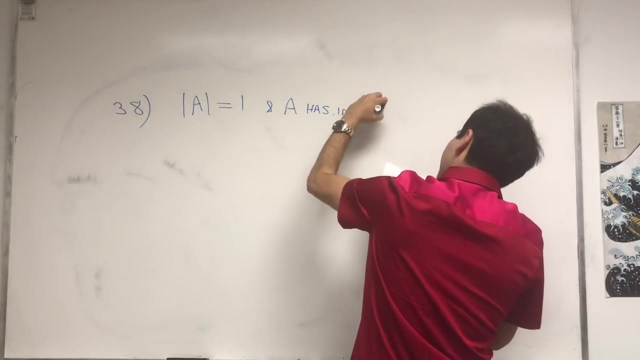 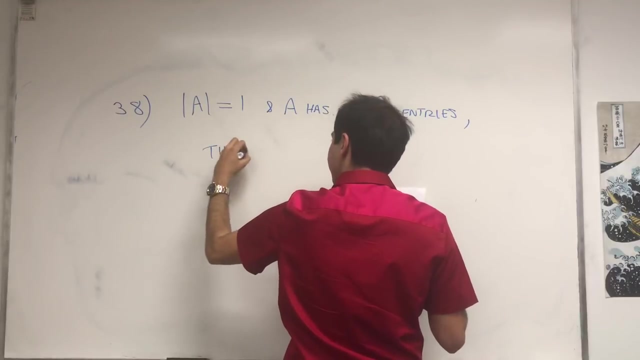 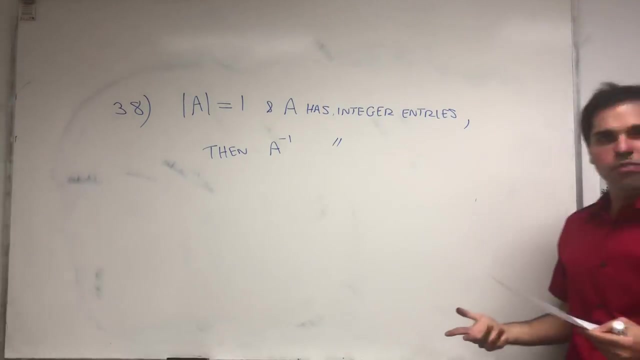 I'm doing it in one setting. So next question: If the determinant of A is 1, and A has integer entries, then A inverse has only integer entries. So, and 38 is the southern version of Azeri, so Azerbaijan. 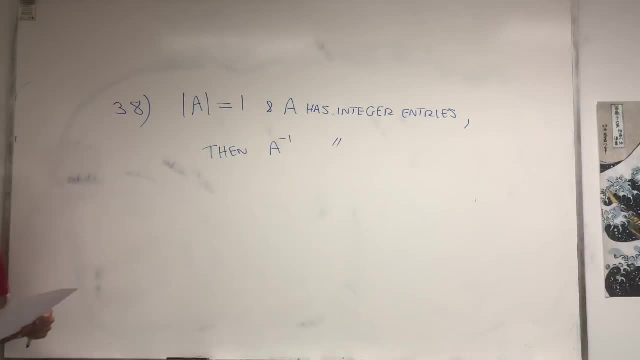 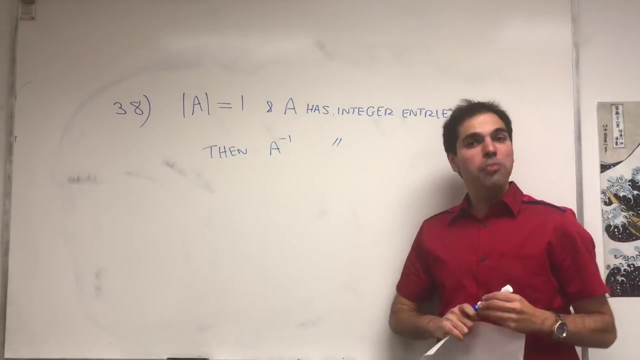 and it's So. it's basically a dialect of Turkish, so that's the language my parents speak. so Actually, there's a cute story. So you know, my last name is Tabrizian, which means who comes from the city of Tabriz. 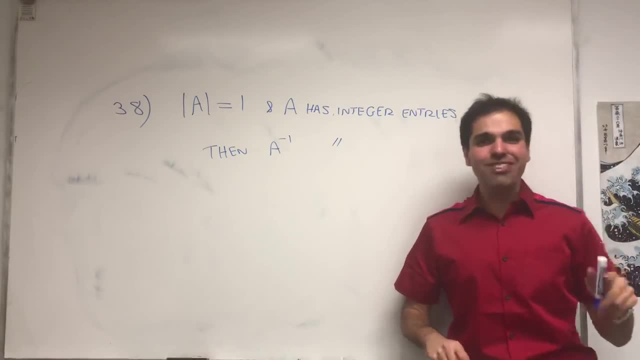 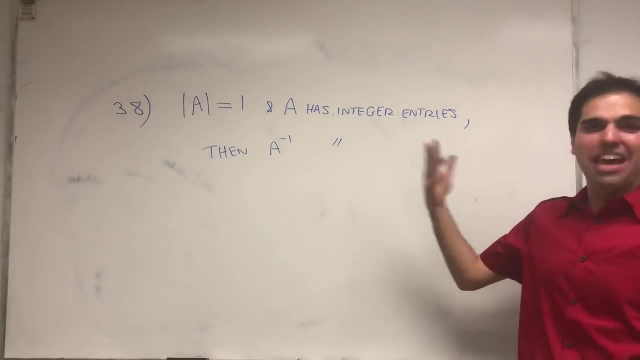 which is in the northern part of Iran, And interestingly it's my dad's last name, but my mom this comes from Tabriz. It's weird. So he's from Tehran, but somehow the language, the name, got transferred. 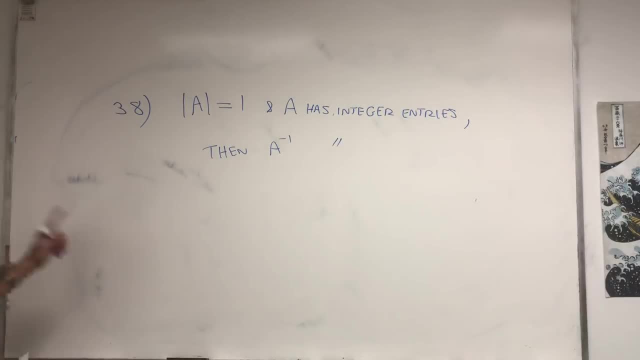 and that's why they can also speak that dialect. Anyway, surprisingly, that's interesting- If usually, if A has integer entries, A inverse does not have integer entries. but if the determinant of A is 1, this is true. 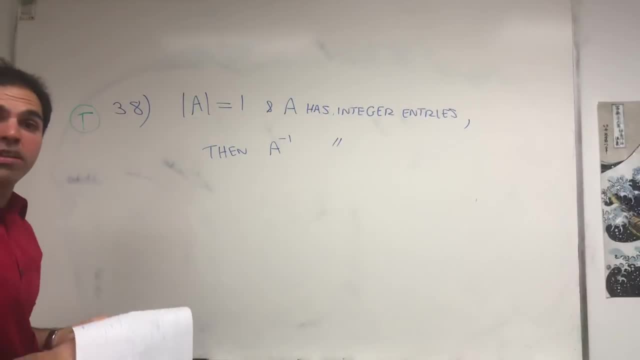 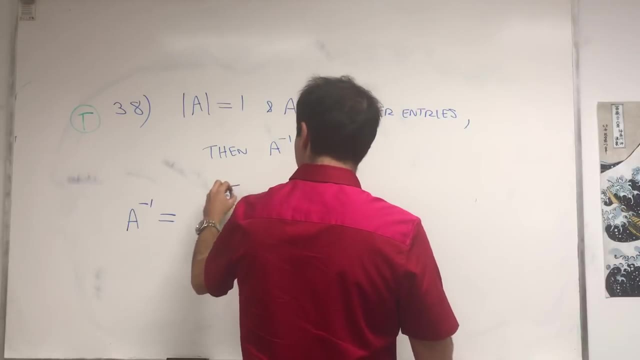 because remember this formula for inverters in terms of determinants: To find A inverse, you just take, uh, a matrix, huge matrix, transpose over the determinant of A and to find that matrix, you just do: cofactor expansion everywhere. 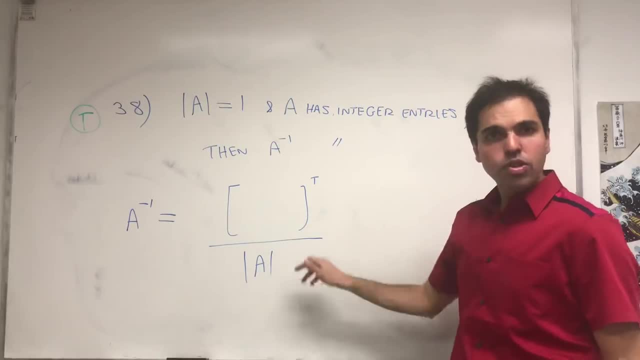 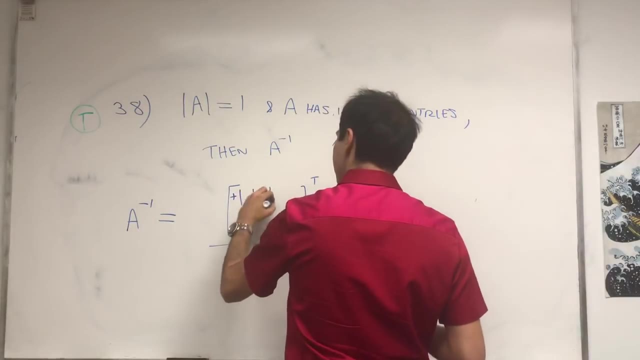 So you use Bomberman, so it becomes plus minus. on determinants: blah, blah, blah. determinants, blah, blah, blah. And look this one by: assumption is 1. And those ones are just bunch of determinants. 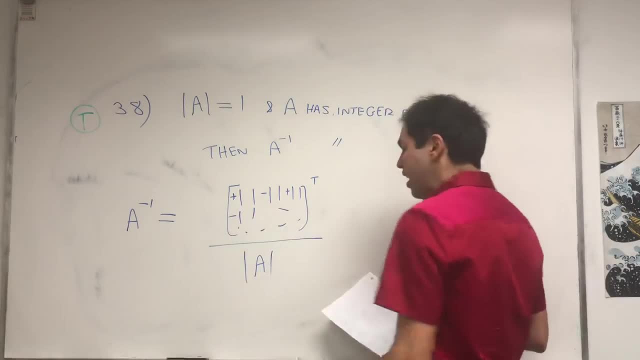 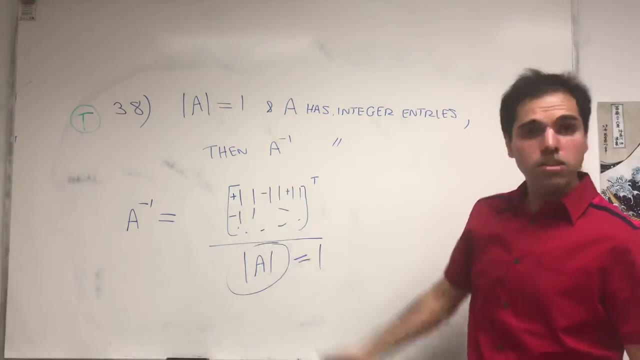 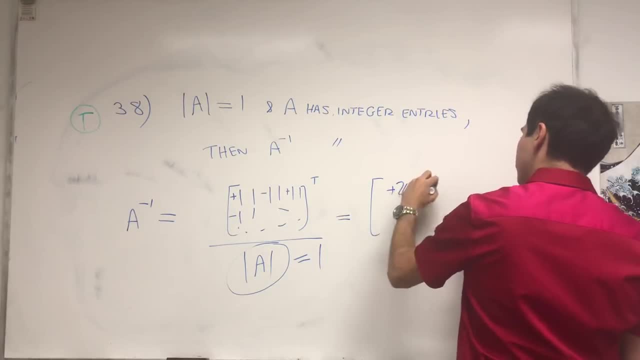 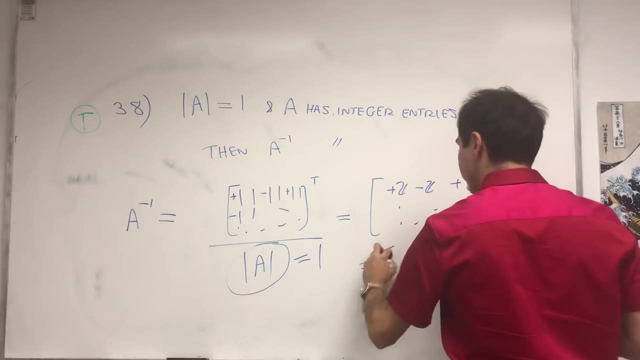 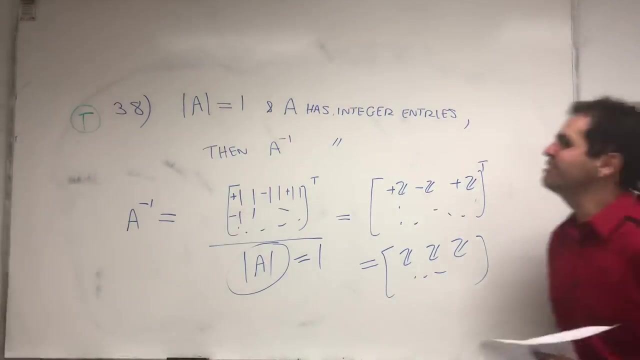 you know plus minus some integer Z Z Z da da da transpose, but that's just bunch of integers as well, because you just flip it. Hopefully not Z Z Z like you're sleeping. 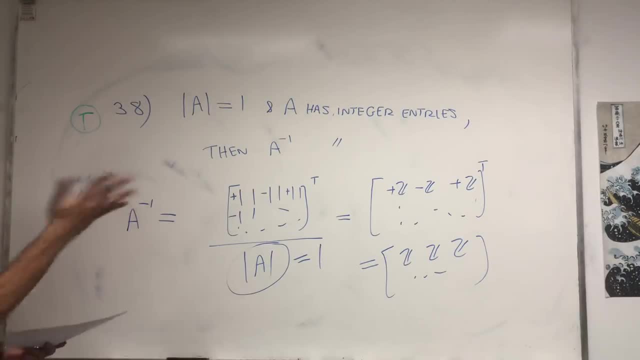 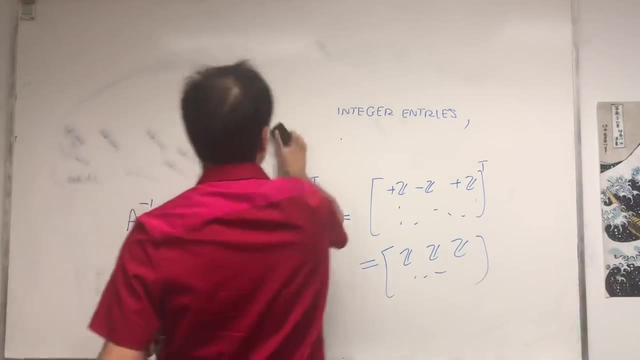 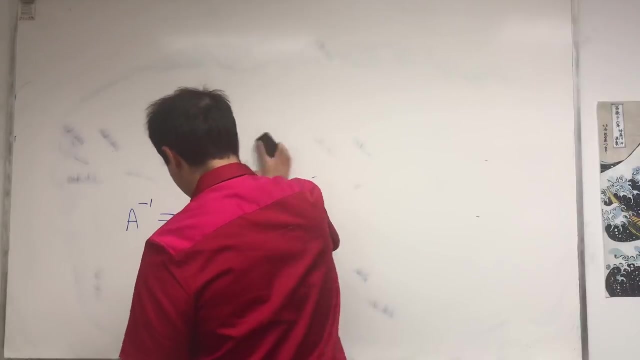 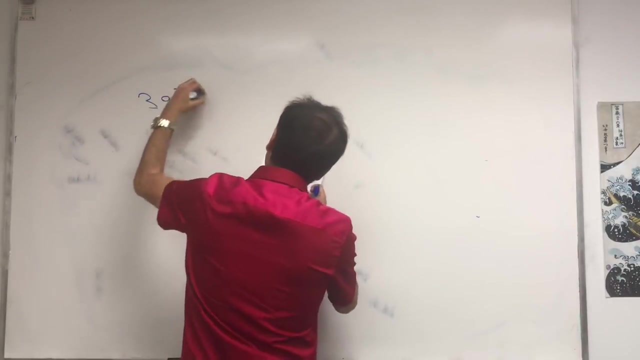 but like determinants. So this is a cute application. I think of this formula because in general it's nice but it's very inefficient. but I think, at least in theory, this is nice okay. so the next one is: I can just realize it's very similar. so if a, if the 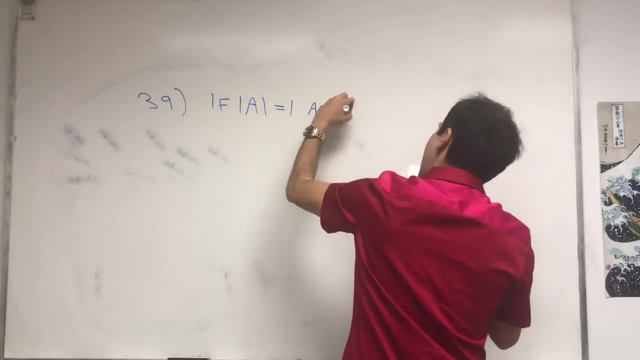 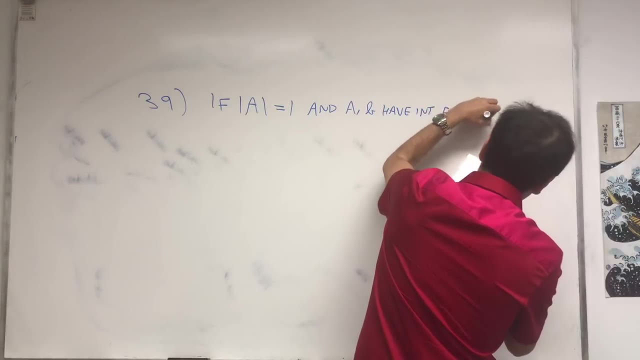 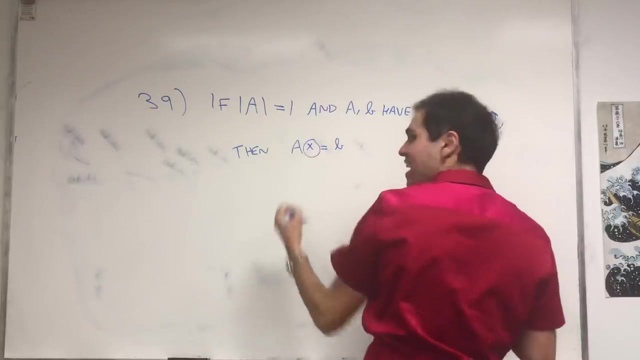 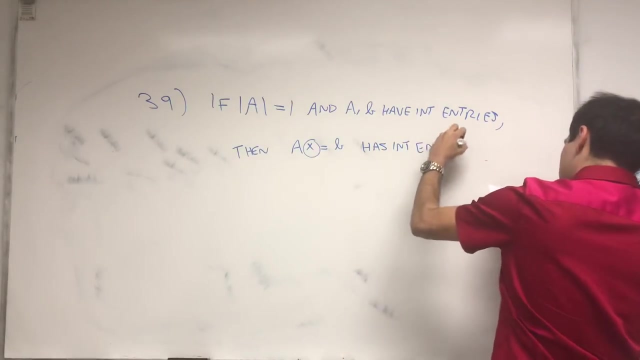 determinant of A is 1 and A and B have integers entries, then the solution of A, X equals to B. so X in A, X equals B has only integer entries. okay, and language 39, finally, for C. so in the western part of Farsi, apparently, and you know, there's a. 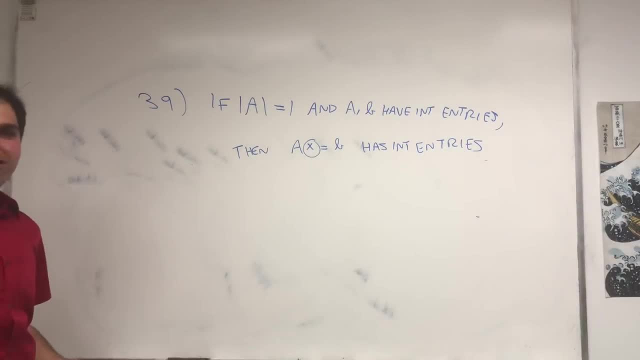 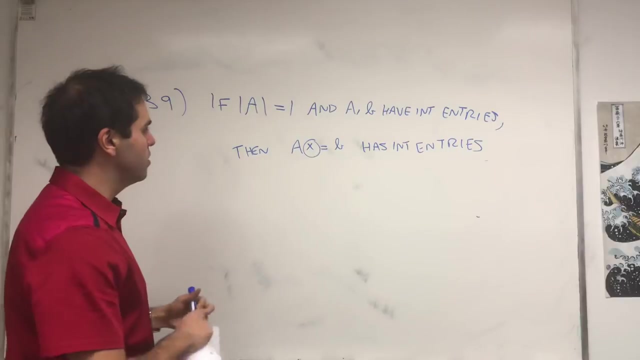 difference and 39 in Farsi is C or no see is 30, norm is 9. so again, in general, the solution to A: X equals B, don't have integer entries. but here it is true, and in fact I just realized, there are two ways of showing this. One is simply: x is a inverse b. 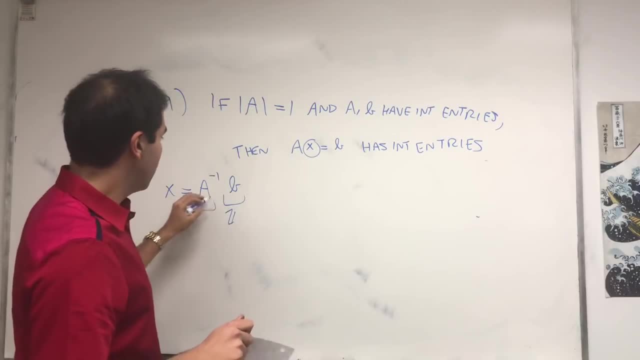 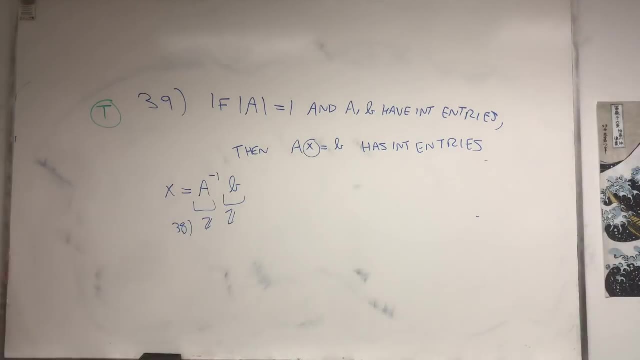 and so b has integer entries. and by 38, we've just shown that a has integer entries. So therefore x has integer entries as well. but I was thinking of something else. I was actually thinking of Kramer's rule, because the ith entry 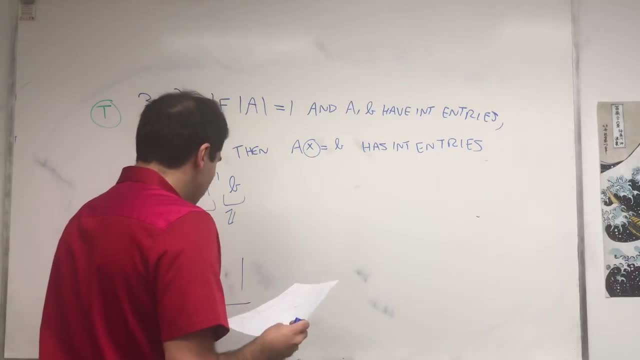 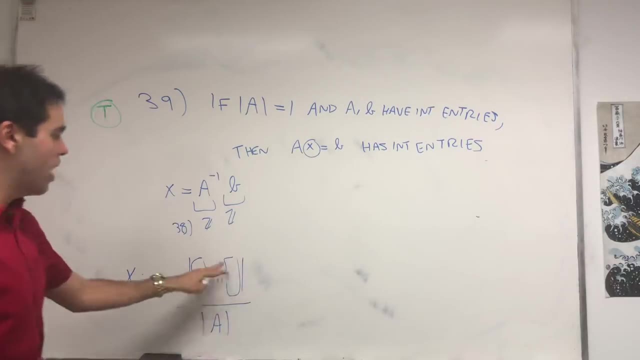 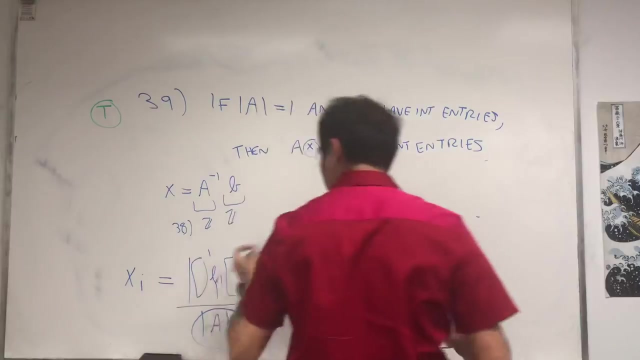 of x. how do you find that? So it's something over the determinant of 1, and the rest is just a. you see, a except the ith column is bi. So because the determinant of a is 1, there is no denominator. so you really have a bunch of. 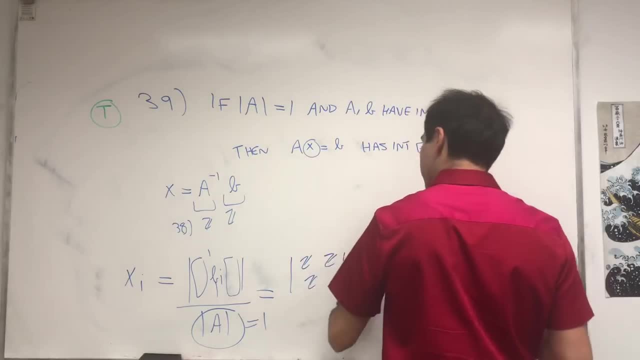 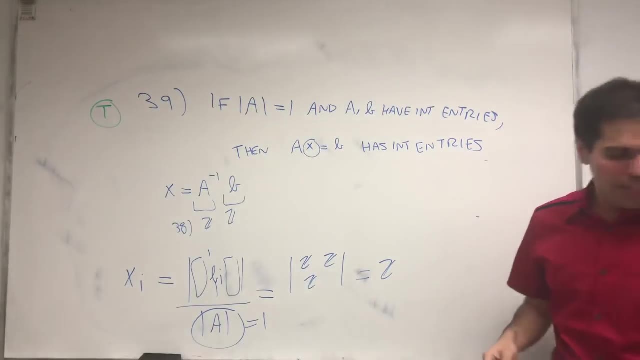 determinant of a bunch of integers, and that's an integer. So two different ways. And with this we're done. With this we're done with determinants. and now let's move on to a huge series of about vector spaces. so part four: 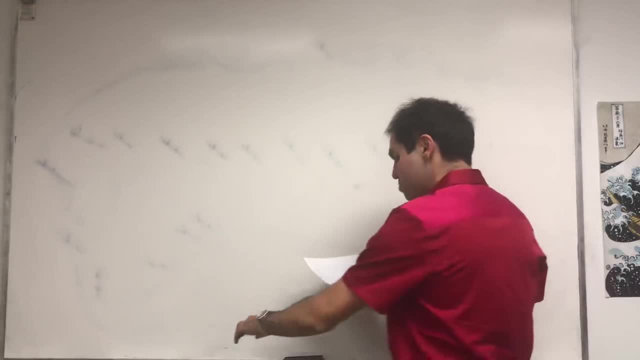 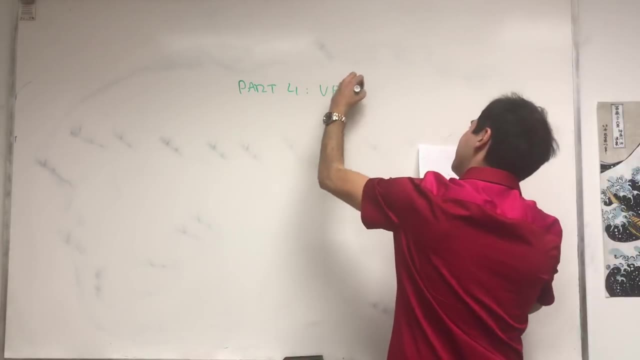 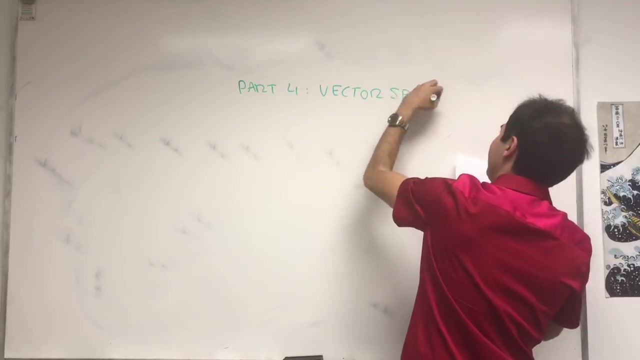 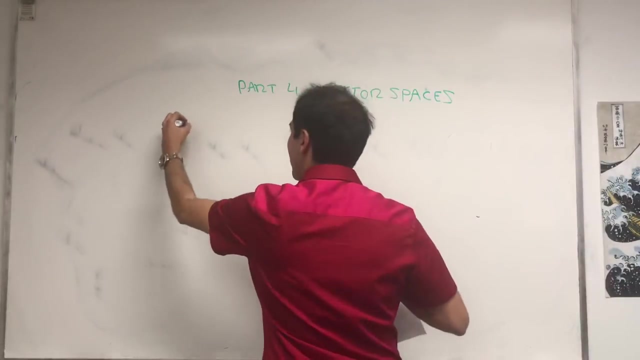 Good, so seven parts in total. Now we're in part four Vector spaces. so, like the heart of linear algebra, Why did I write vector species, No spaces. Question 40. One of my favorite questions. It was on my quiz. 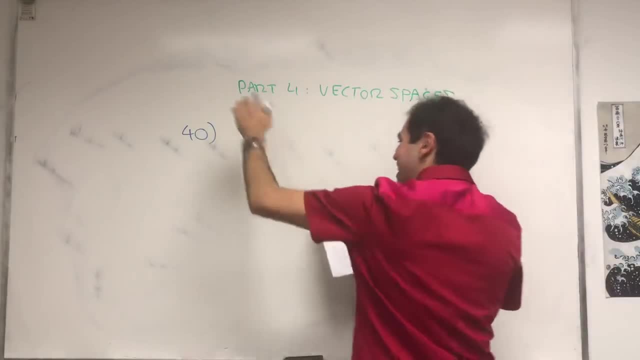 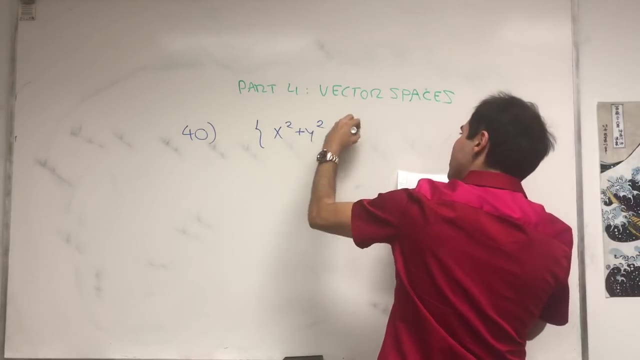 when I took linear algebra, the upper division class, back in 2007.. So the question is: is the set of points x and y such an xy or a y or a z or a z or a y or a z or a y or a z or a z or a z? 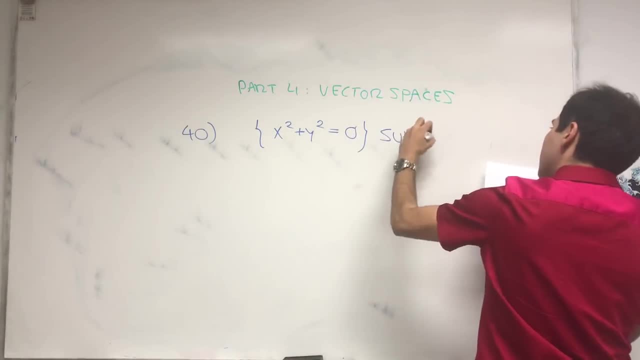 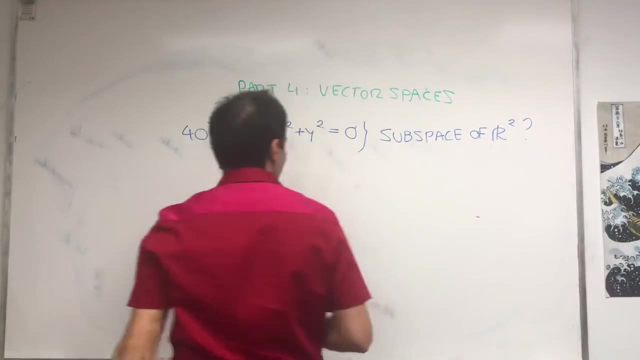 X, Y equals zero. is it a subspace of R2?? Oh, I guess the statement is: it's a subspace of R2, and then you have to say true or false. And language 40 is maithili and unkalis. 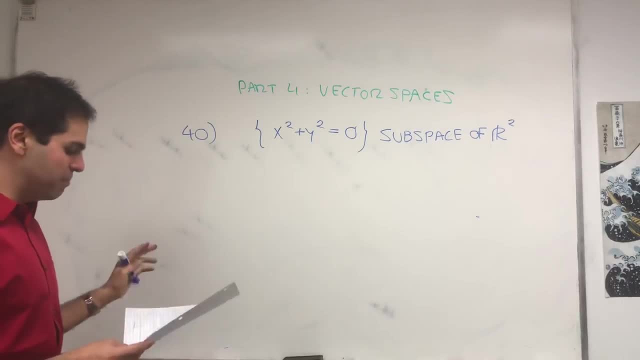 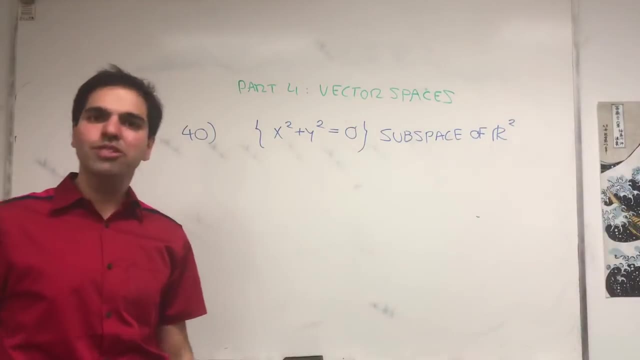 that's how you say it: maithili or maithili. Is it a subspace of R2?? The interesting thing is, if you try to show it's a try to disprove it's a subspace, you might kinda run into trouble. 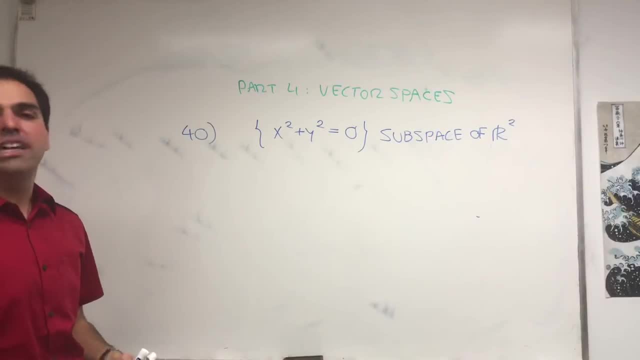 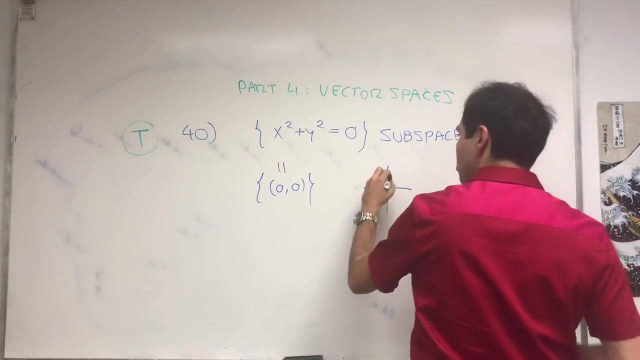 but in general, if you wanna disprove something, find a counterexample, because it turns out there is no counterexample. This is true, because what is this? It's just a circle of radius zero. so it's just this. And the point: zero, zero. 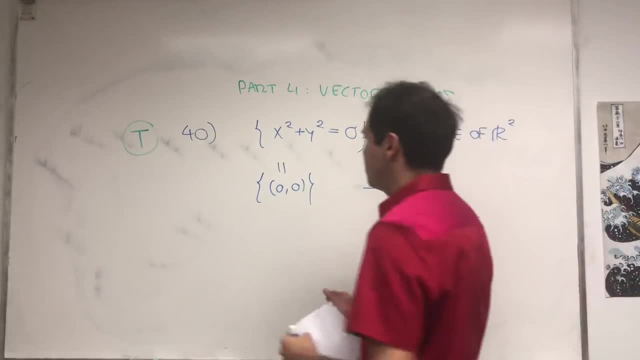 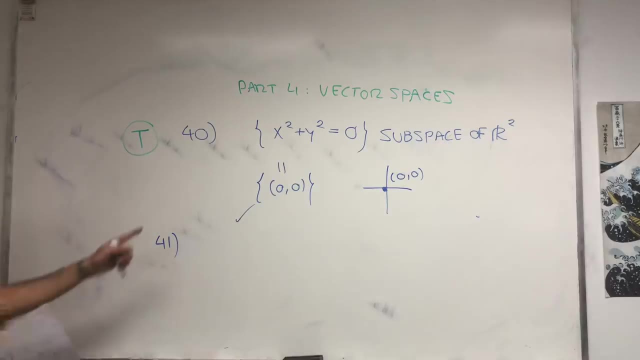 the zero space. it's indeed a subspace, That is true. But again, if you try sort of fake to disprove it, you would say, oh well, the sum of those two things is not necessary in that thing, but indeed it is. 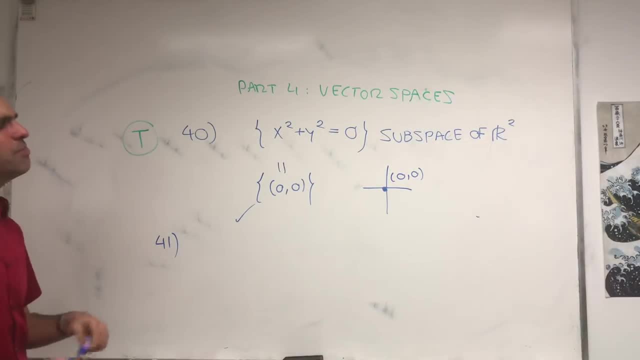 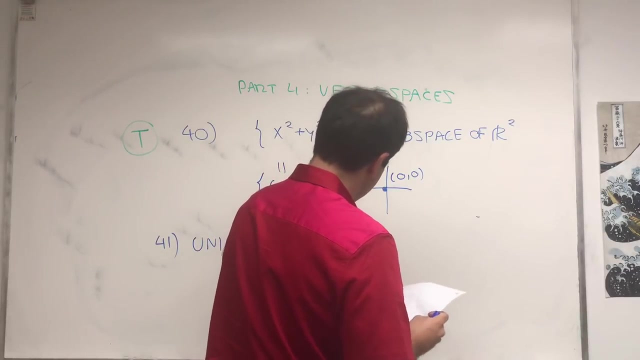 So that's why I think I kinda showed it badly. but if you wanna disprove something, make sure to find a counterexample. Okay, next one: the union of subspaces, let's see, of R2, is a subspace of R2.. 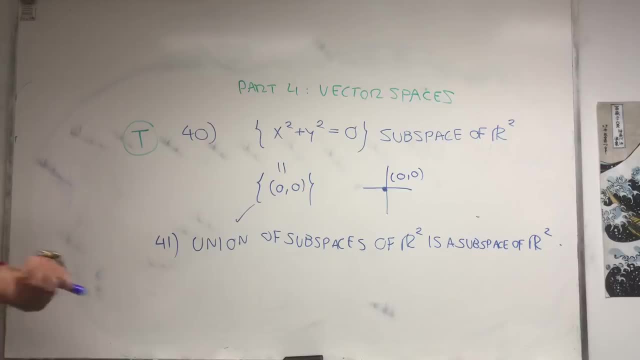 In other words, if you have two sets or two spaces and you sort of put them together, is it still a subspace? Yep subspace And language 41,, Hausa and it's, I think, language in Nigerian. 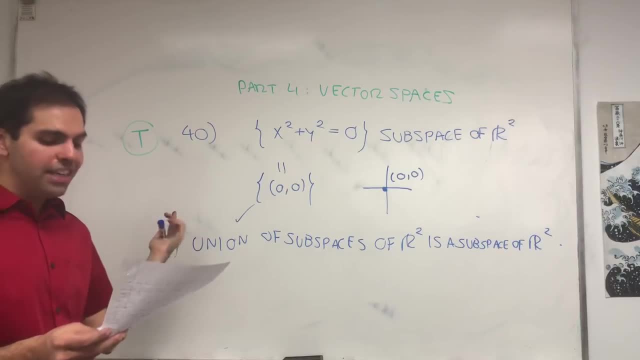 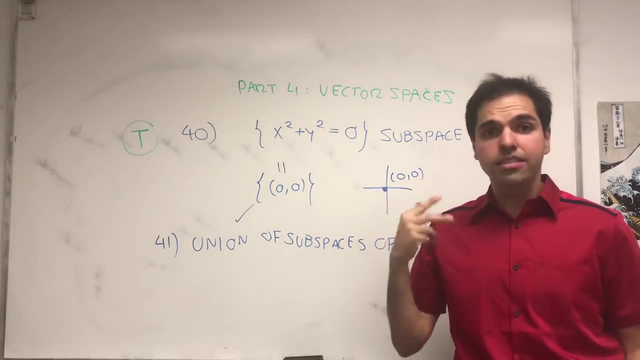 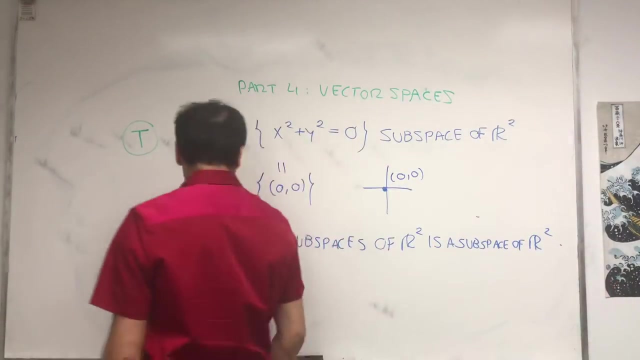 And Bin 41, you say arba in daya, I think like Arabic almost, cause I think is for an Arabic. so maybe a dialect, Not a thing A dialect, And so, interestingly, the union of subspace. 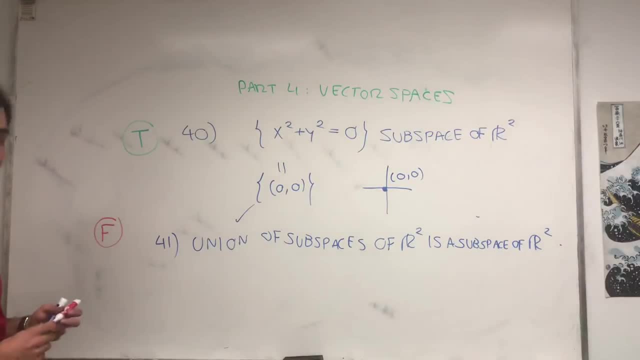 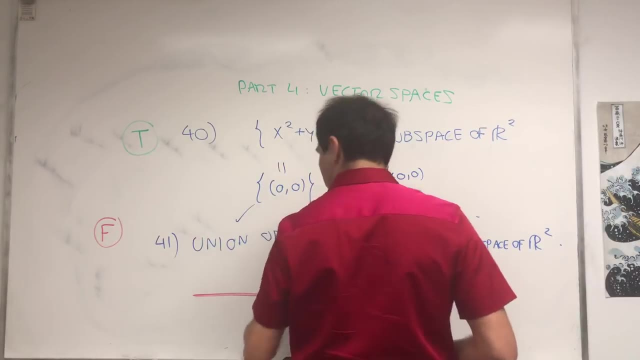 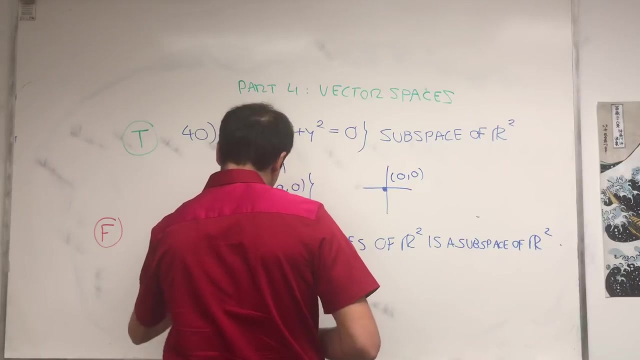 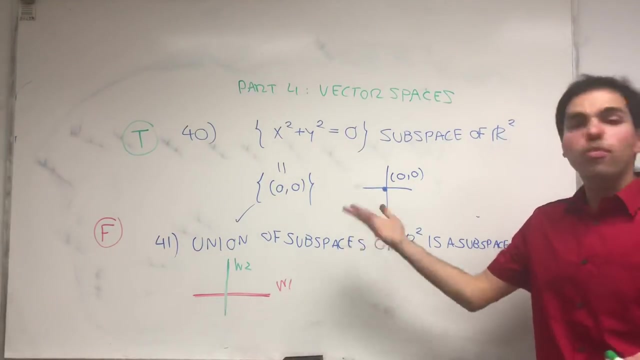 Thisовых of subspaces is not a subspace, because consider the following: in R2, consider, let's say the first one, let's say W1 to be the x-axis and W2 to be the y-axis- you can show separately that the x-axis is a subspace of R2 and the y-axis is a. 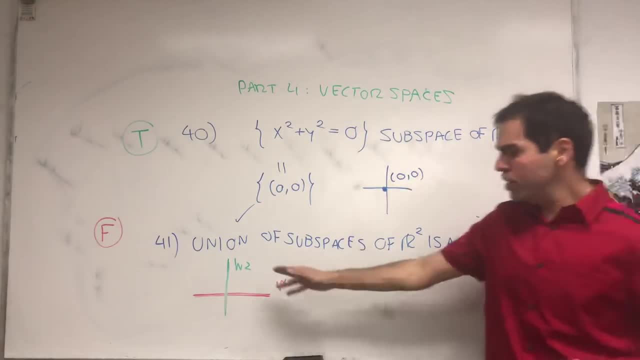 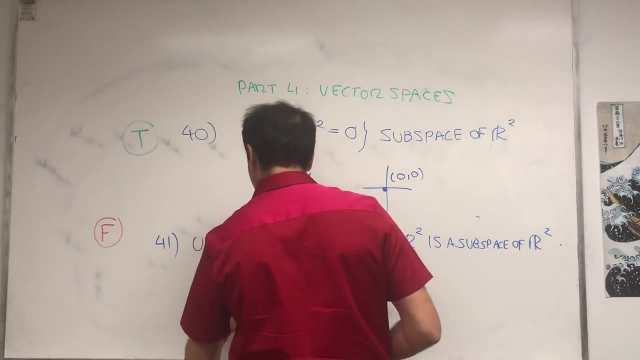 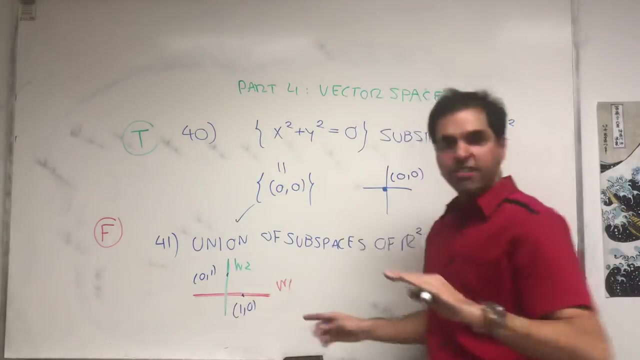 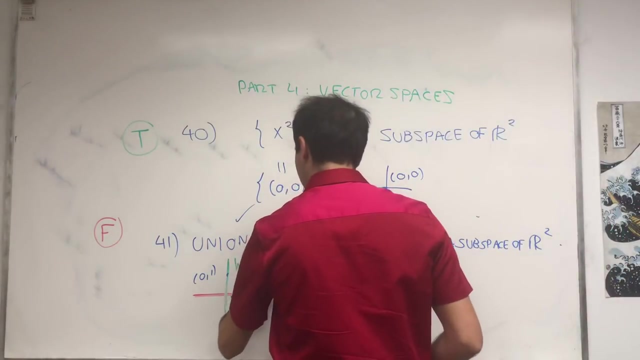 subspace of R2, but the union, which is just the x and the y axis put together. it's not a subspace because, for example, take this point- 1: 0 is on the x axis, 0: 1 is on the y axis. so it's in the either or space, right, but if you add the two, 1- 1, it's not in that. 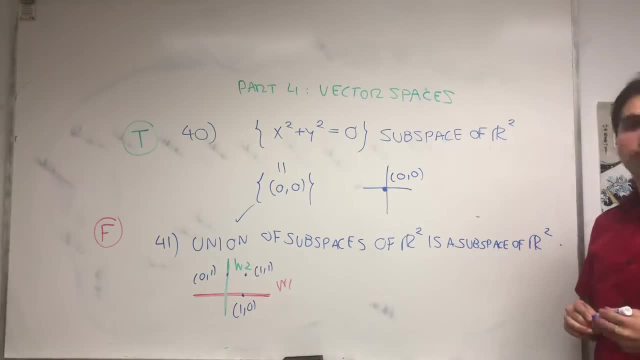 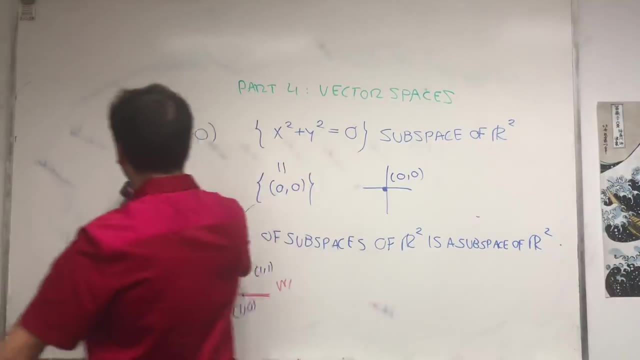 space anymore, so it escapes and therefore it It's not a subspace, And therefore the union of subspaces is not a subspace. OK, good, Oh, my god, we're almost at two hours. Black pen, red pen. I think you won the challenge. 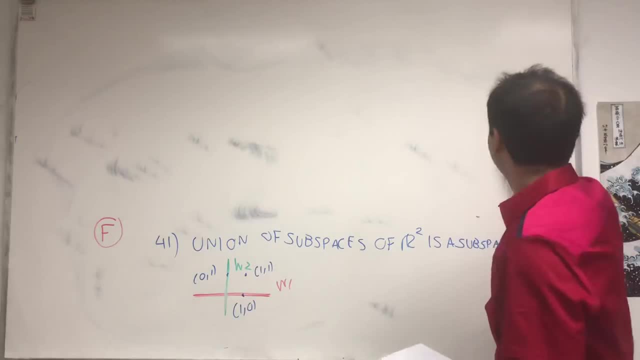 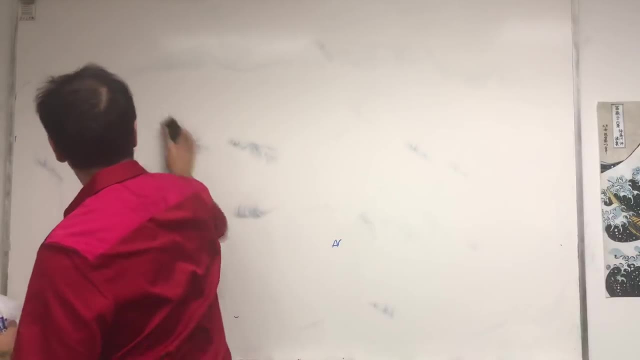 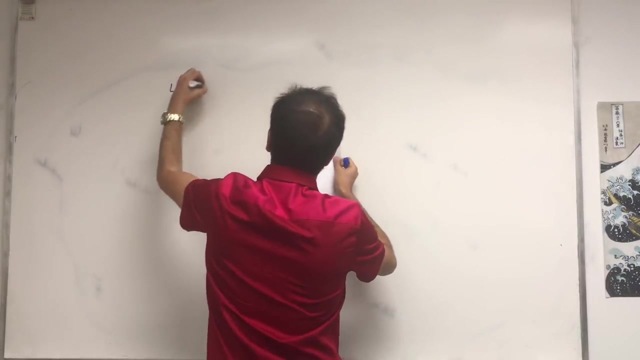 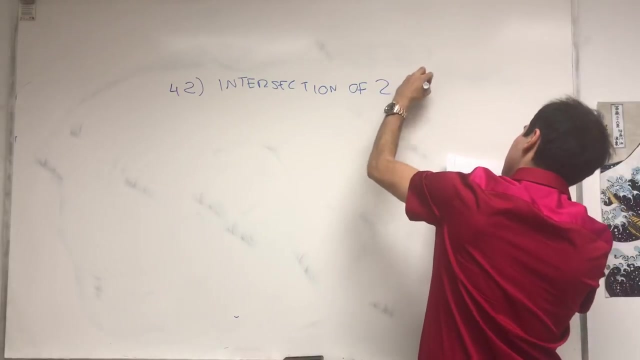 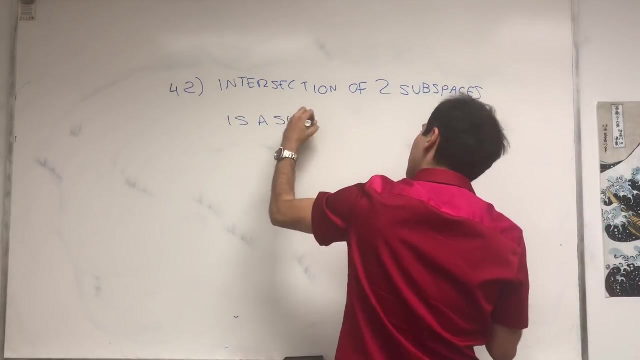 So I think it will take more than two hours to do it. OK, But what about? so we talked about the union. What about the intersection? The intersection of two subspaces is still a subspace. So subspaces, let's say Rn. 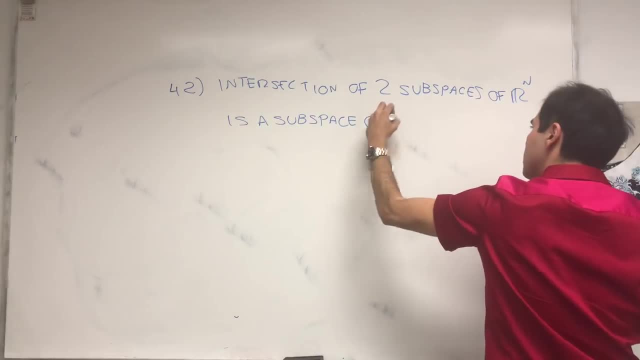 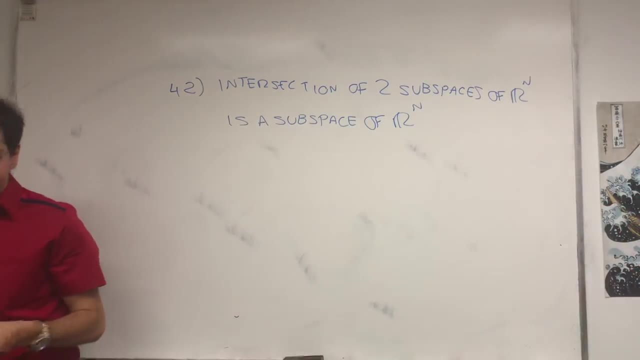 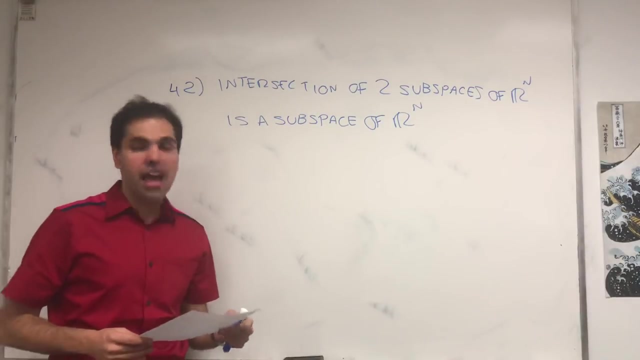 It works for any vector space And 42 is an Algerian dialect of Arabic And again, I'm not sure, I'm not sure the dialect specifically, But in Arabic 42 is, You know, like 42, the coolest number. 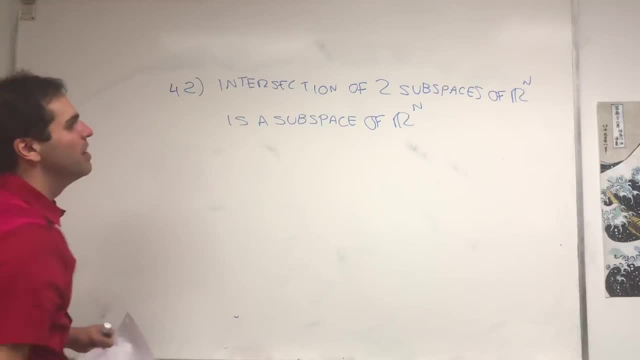 Well, coolest integer number. And, interestingly, even though the union of subspaces is not a subspace, the intersection of subspaces is still a subspace. So This is true And, in fact, the intersection of any number of subspaces. 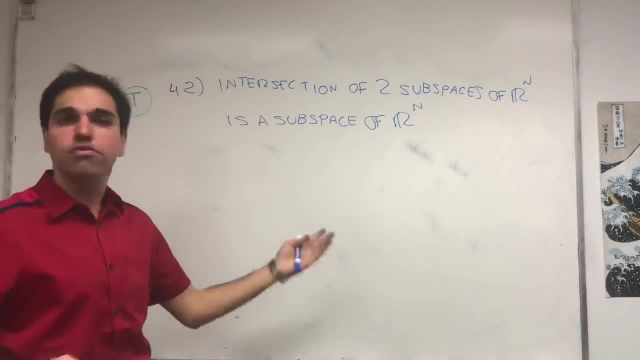 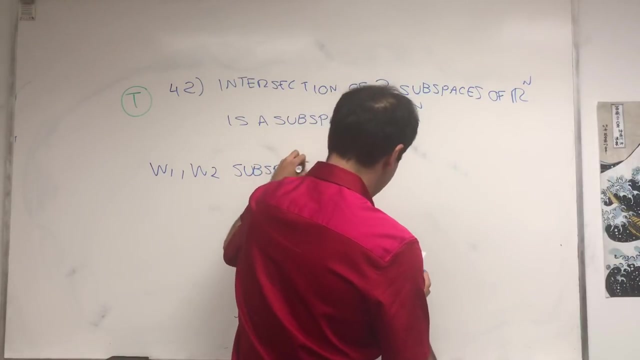 is a subspace, So not just a countable or not just finite, not just infinite, even uncountably infinite, it's still true. But let me do the case for two. So let W1 and W2 be subspaces of Rn. 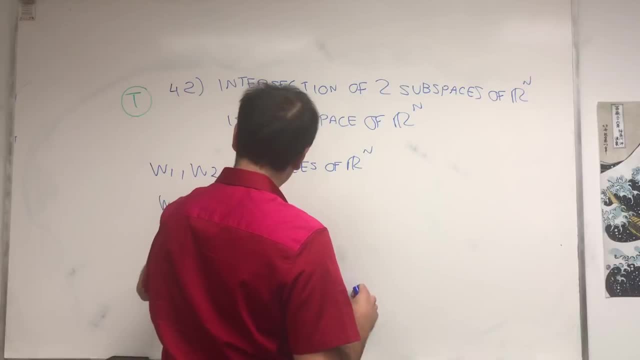 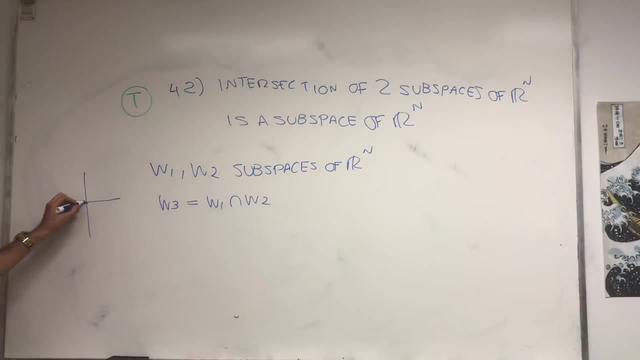 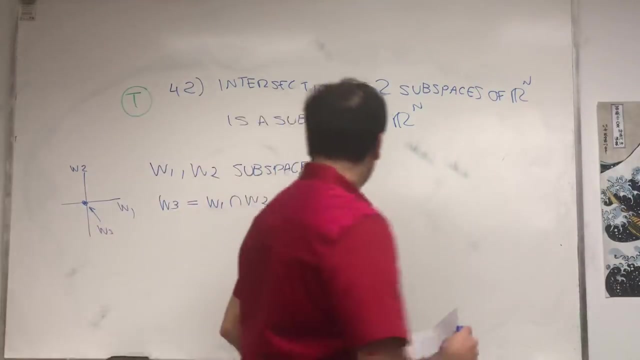 And let W3 be the intersection. OK, So the set of points that is in both of those spaces. So for the x-axis and the y-axis the intersection would be the origin. OK, I'm not going to prove the whole three things properties. 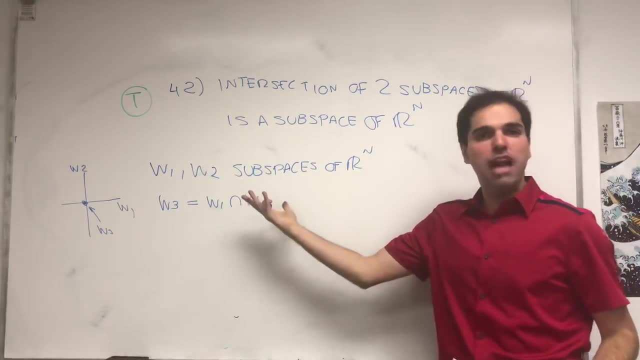 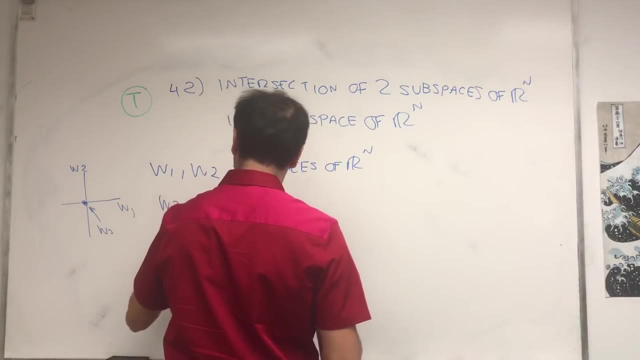 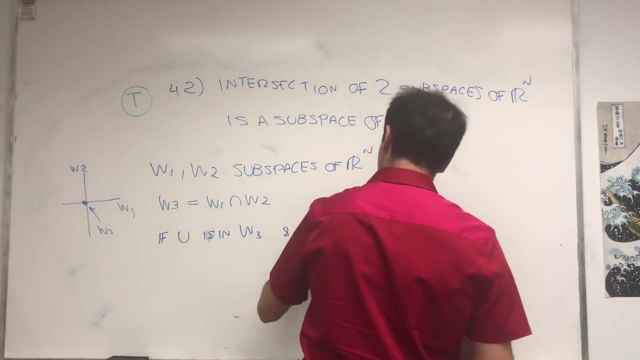 because that would take us in 10 hours. But let me for example show that it's closed under addition. So suppose if u is in, So if u is in, OK, If u is in w3 and v in w3, what does that mean? 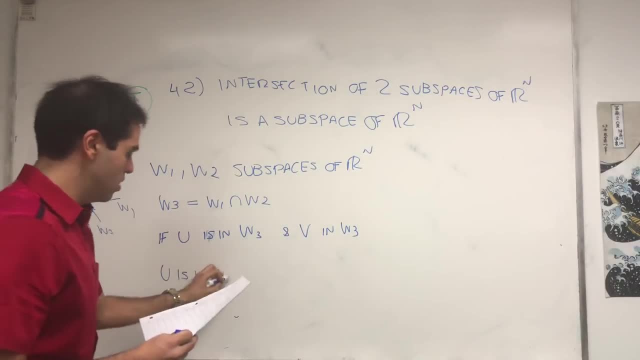 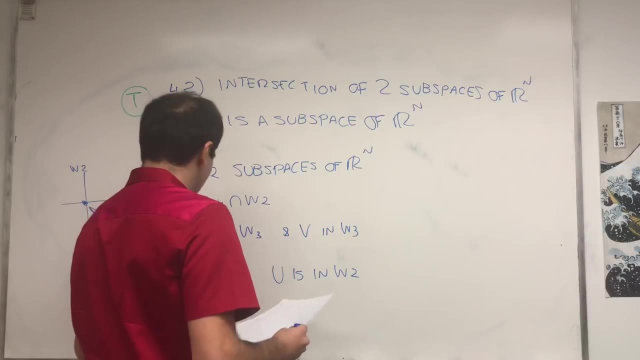 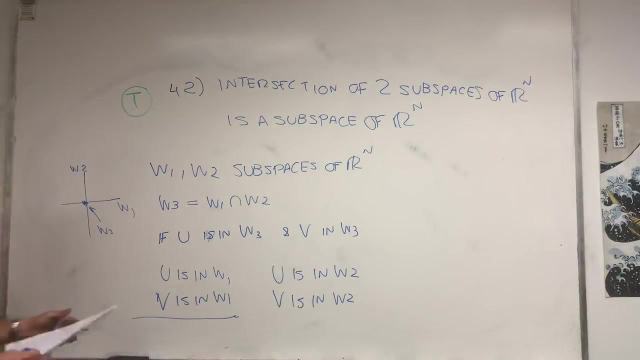 It means that u is in w1 and u is in w2.. And v is in w1, v is in w2.. And so what does that mean? If, Because w1 is a subspace, If w1 is a subspace, the sum of the two is still in w1. 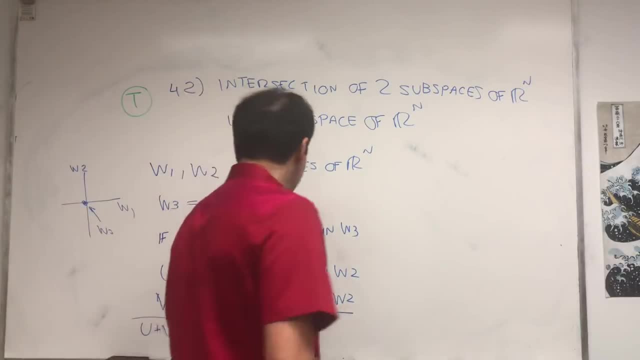 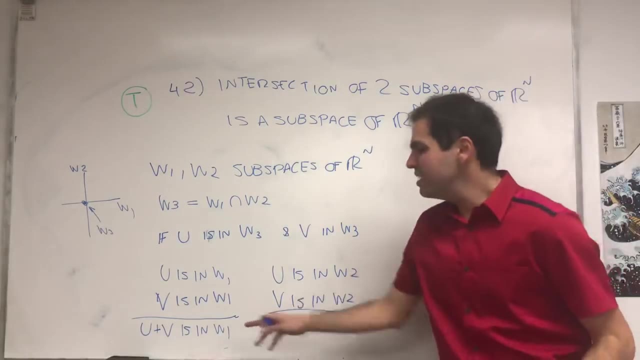 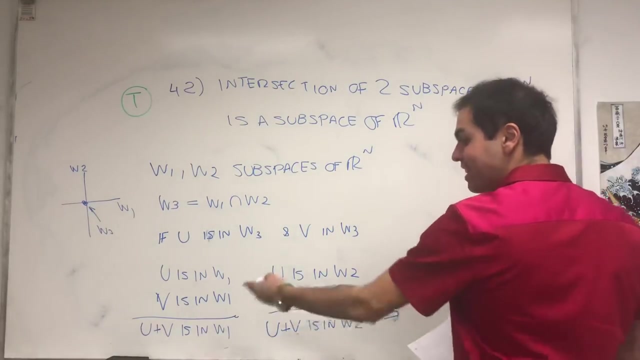 So u plus v is in w1. And similarly u plus v is in w2.. But look, because u plus v is in w1 and u plus v is in w2, because, by definition of the intersection, u plus v is in w1. 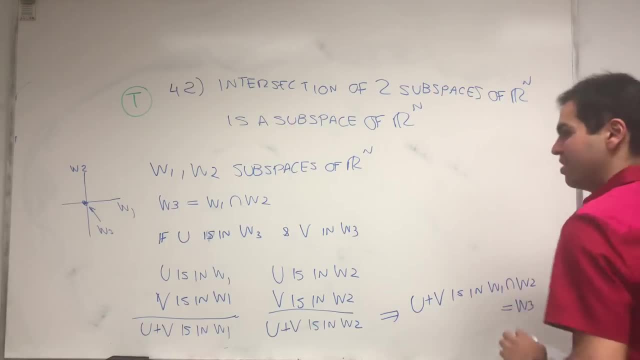 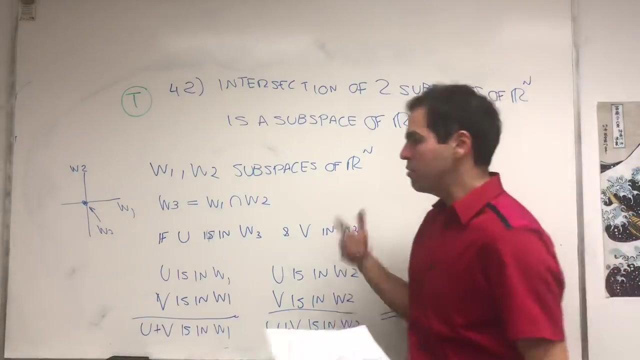 intersect w2.. But that's just w3. So, in other words, we've just shown that the intersection of the two is closed under addition, And that's one of the three properties you have to show. the other two closed under scalar multiplication and the zero vector. 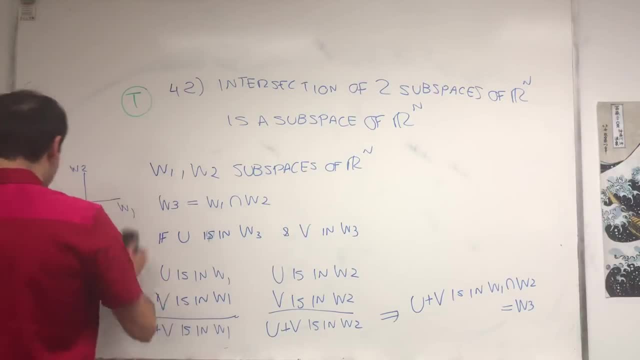 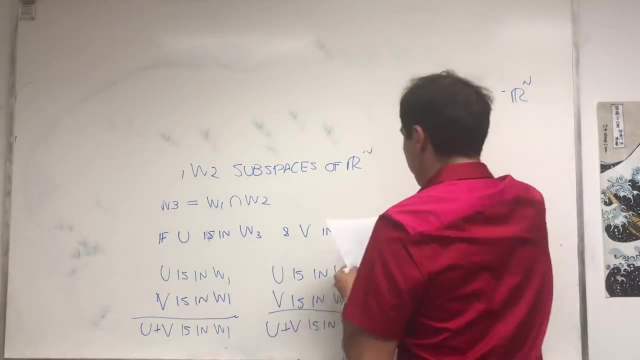 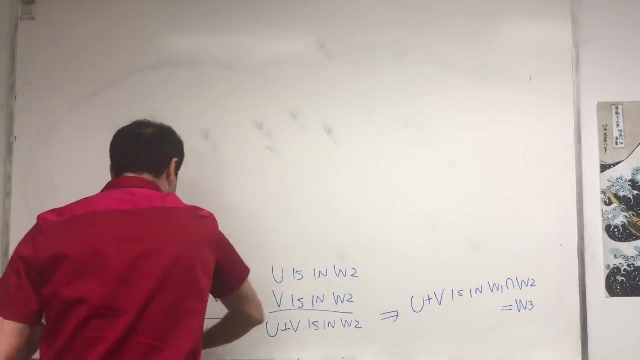 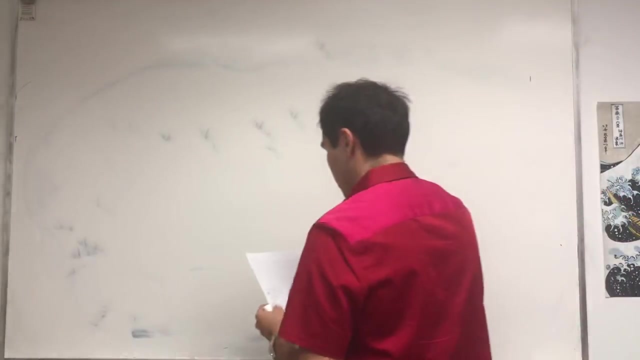 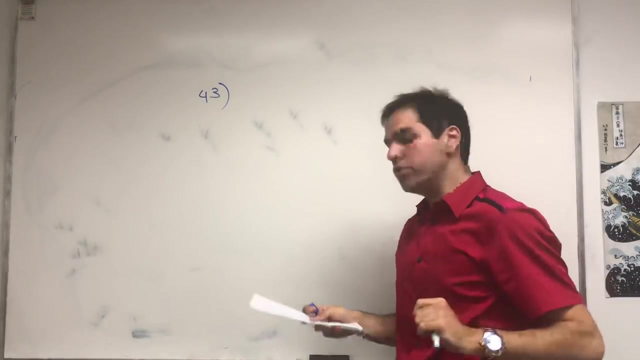 It's very similar to this thing. OK, And now let's talk a bit more about properties of subspace. So we've got a set of subspaces, So here's an interesting question which might or might not be true. So here, v is a vector space w a subspace. 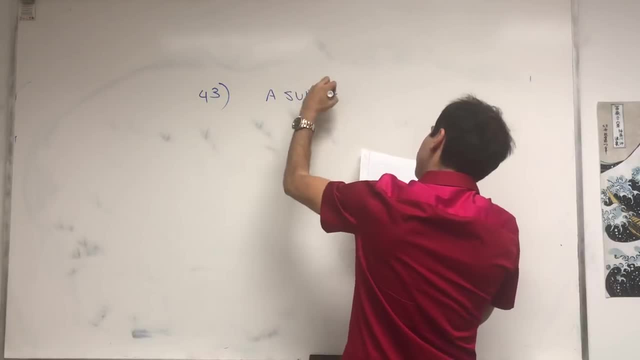 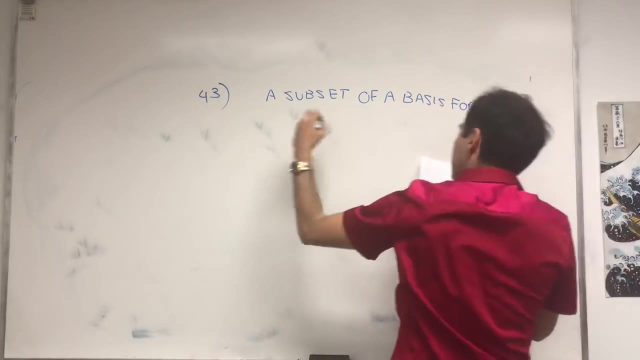 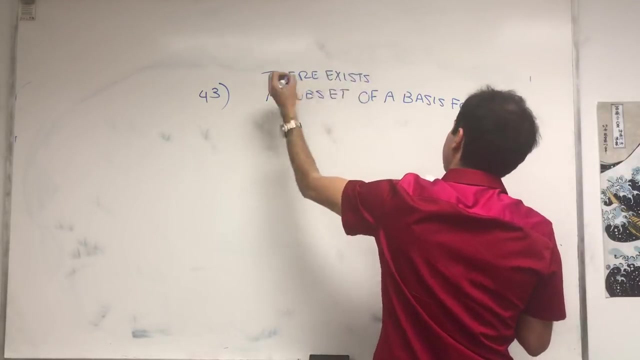 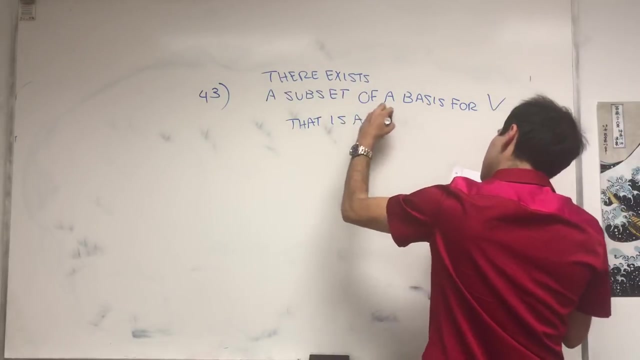 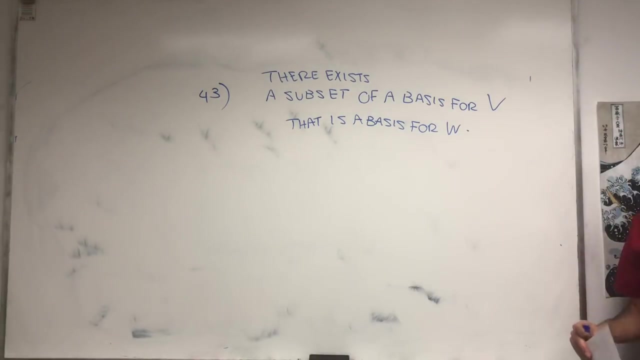 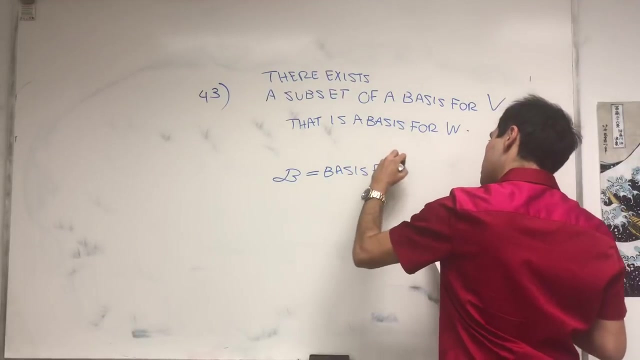 And the question is: a subspace or a subset, or I guess there exists. maybe there exists a subspace of a basis for V that is a basis for W. Let me rephrase it So: given a basis for V, so suppose B is a basis for V, can you find a subset of B that? 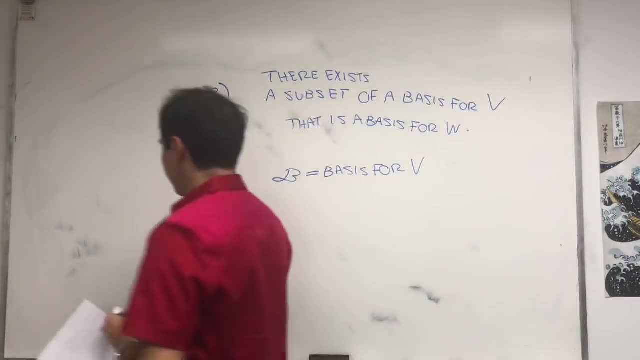 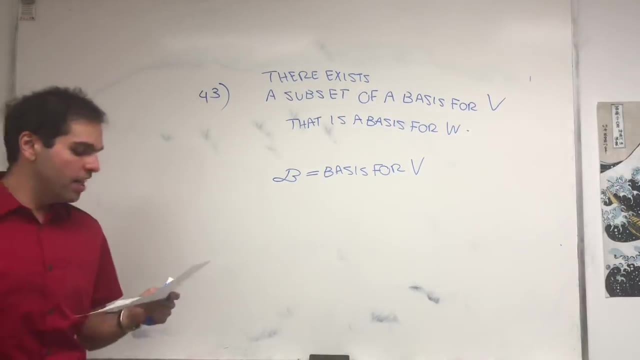 is a basis for your space W, And so 43 is Burmese, so in Burma, and it's Lidzetto, So it's 43.. It sounds like a cool property, It sounds awesome, but it turns out it's false. 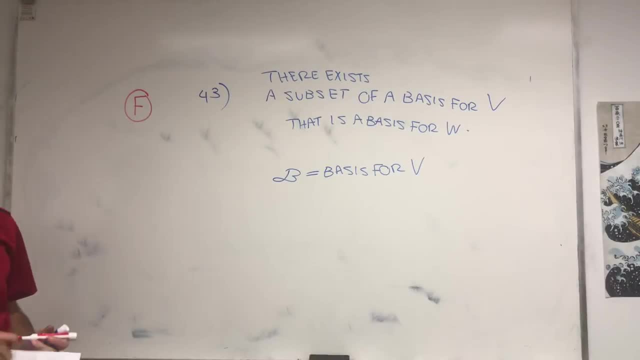 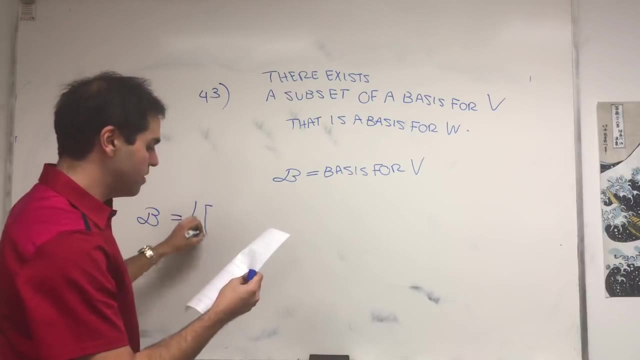 And let me explain to you. I think once you see the counterexample, you'll see what I mean by this question. So consider B, which is the basis: 1, 0, 0, 1, and that's a basis for R2.. 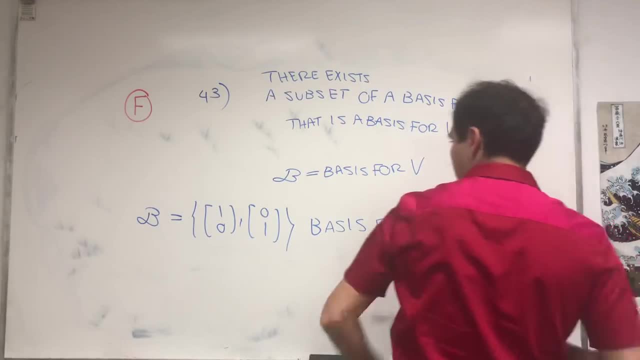 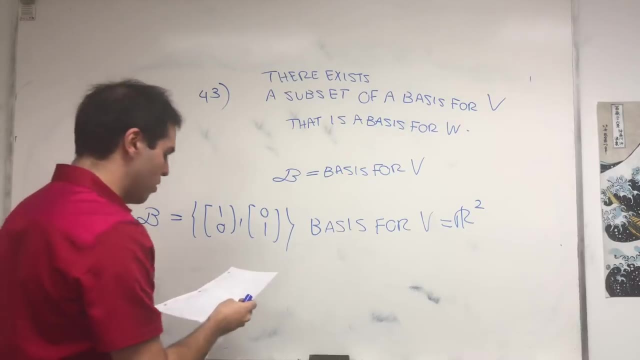 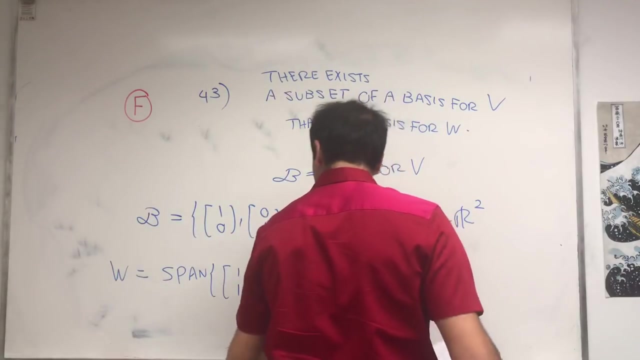 For B, that's R2.. And now consider a subspace, W. so we're fixing B, we're fixing W to be the span of 1, 1.. So in other words, just the line Y equals to X. 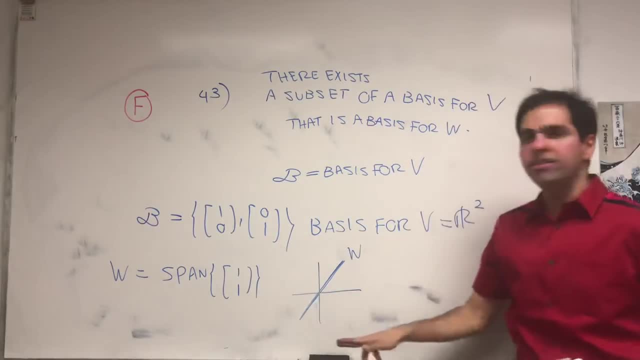 Can you find a subset of 1, 0, and 0, 1 that is a basis for W? Unfortunately not, because you can't find a subset of 1, 0, and 0, 1.. Unfortunately not, because you can't find a subset of 1, 0, and 0, 1.. 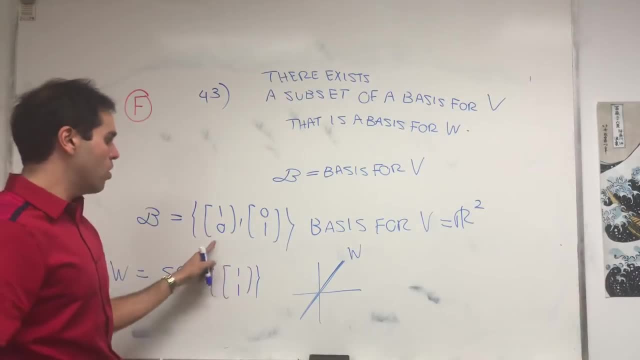 Because the only subsets of this set are 1, 0, and 0, 1,, which is not a basis for W. 1, 0 is also not a basis for W. 0, 1 is not a basis for W. 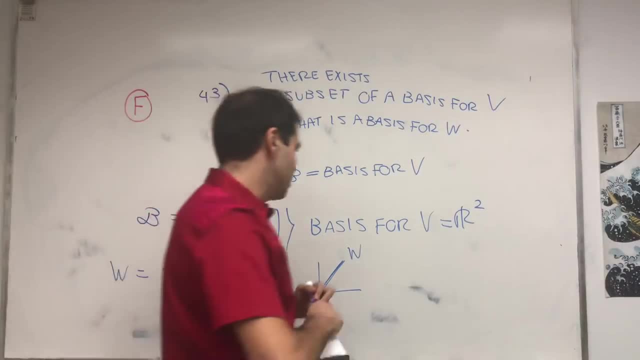 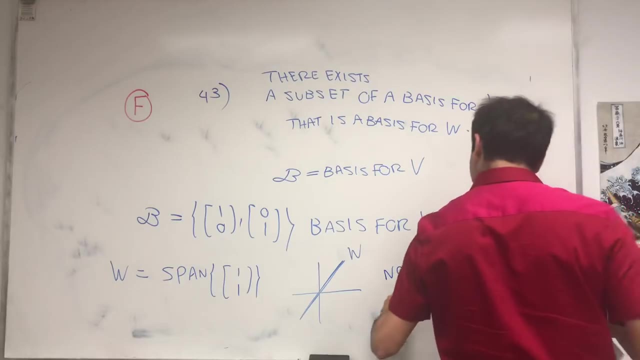 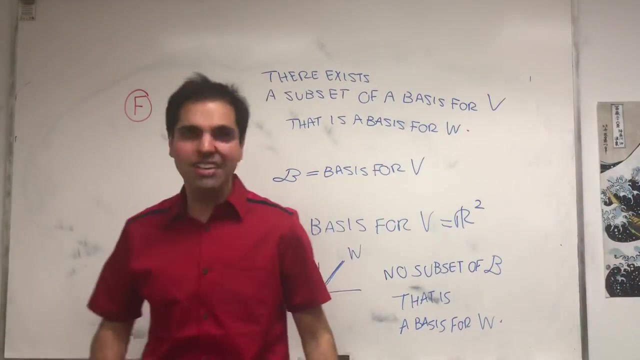 And the empty set is also not a basis for W. So no subset of B that is a basis for W. 0, 0 is a basis for W, And the reason I'm doing this is because there is this opposite statement that says: 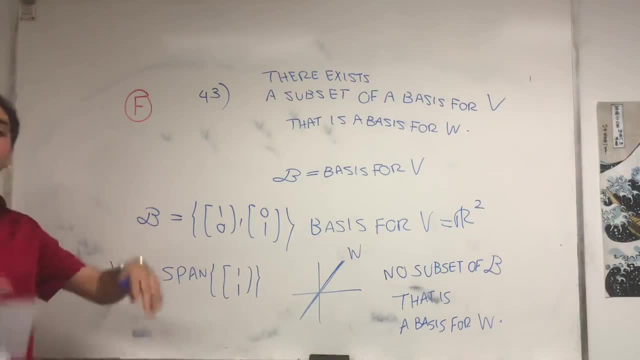 if you have a basis for your subspace, can you find a superset that is a basis for V, And this is indeed true. So if you start with the basis 1, 1 for W, you can actually extend it to get a basis for R. 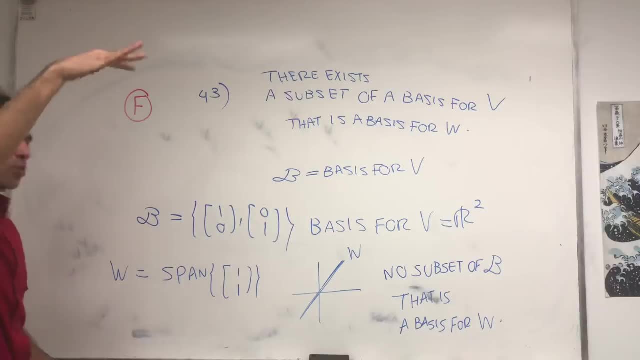 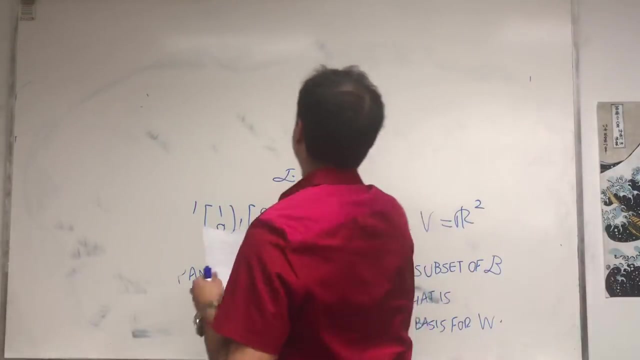 of R2,. but the opposite is not true. You cannot just reduce a basis for V to get a basis for W. Okay, next question, and I'm not going to say anything about this because otherwise I'll- I tend to talk too much and to reveal lots of things, so 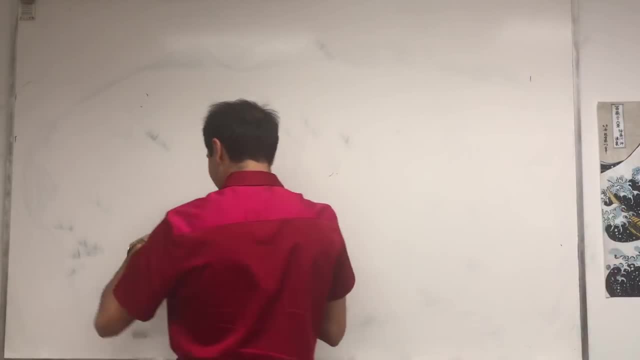 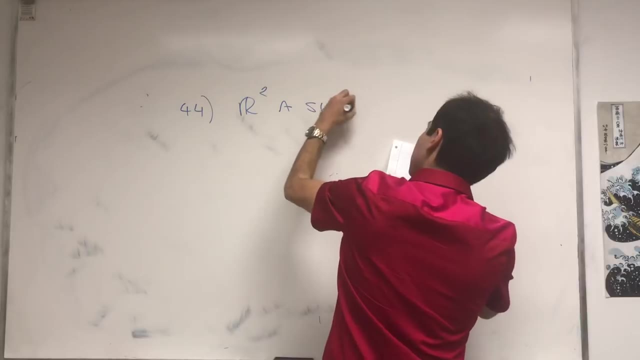 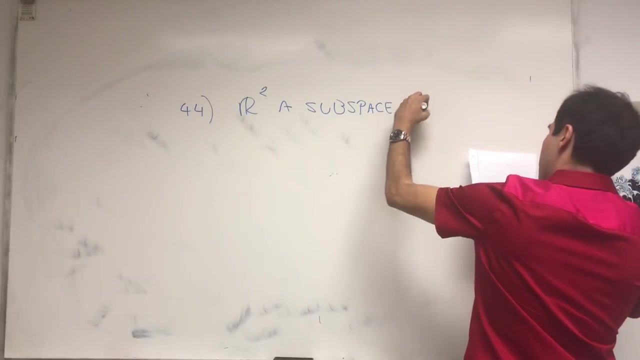 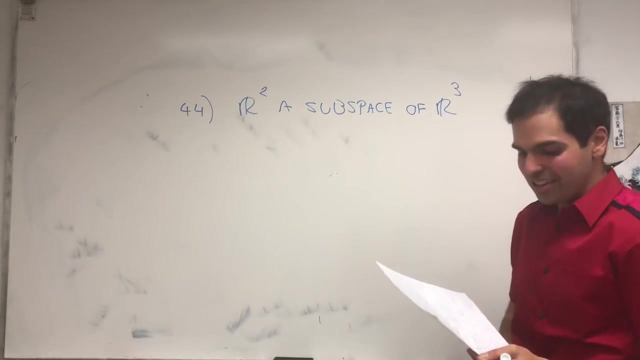 very bad poker face actually. So the next question is: is R2 a subspace? So no, confirm. So R2 is a subspace of R3.. And language 44,: Serbo-Croatian. So Serbia and. 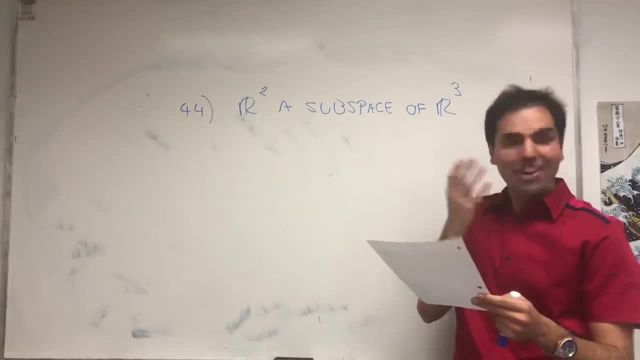 Croatia. and oh my god, okay, I don't know why I'm so confused. Okay, so, language 44, Serbo-Croatian. So Serbia and Croatia. and oh my god, okay, I don't know why I'm so confused. 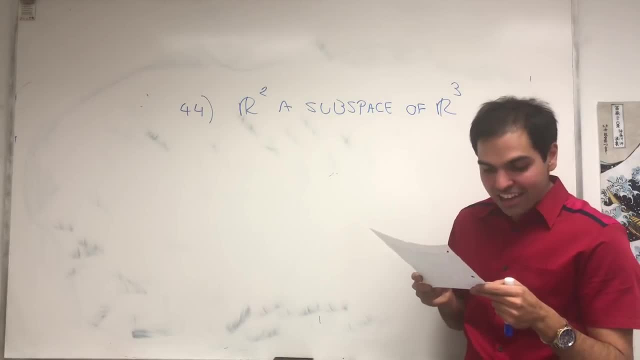 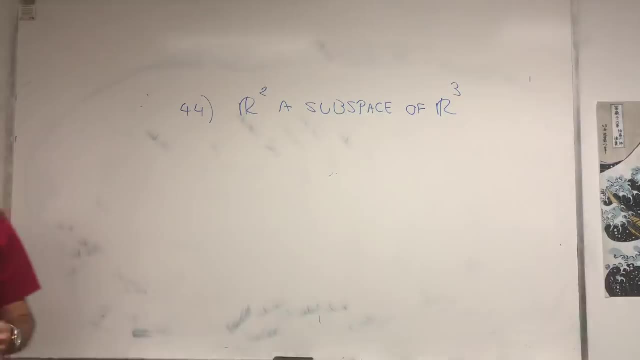 44 in Croatian is: oh Cetur decet cetiri. Okay, That's pretty bad, okay. 44 in Croatian is: oh Cetur decet cetiri. Okay, That's pretty bad, okay. 44 in Croatian is: oh Cetur decet cetiri. Okay, That's pretty bad okay. 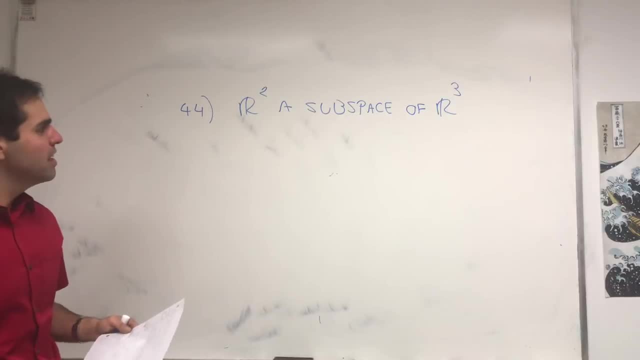 For the easier European languages. I have trouble pronouncing them All right. question: is R2 a subset of R3, a subspace of R3?? Actually false, and that's the question that gets my students every time. So in history we don't have a subspace. 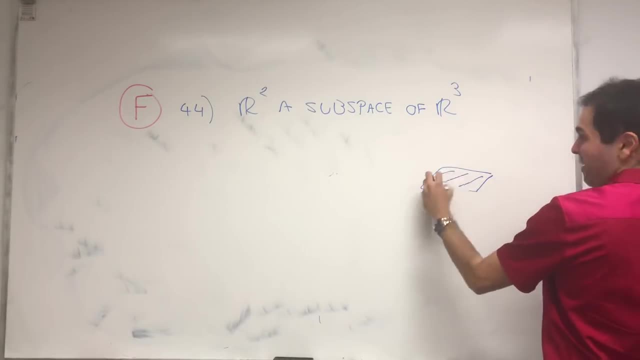 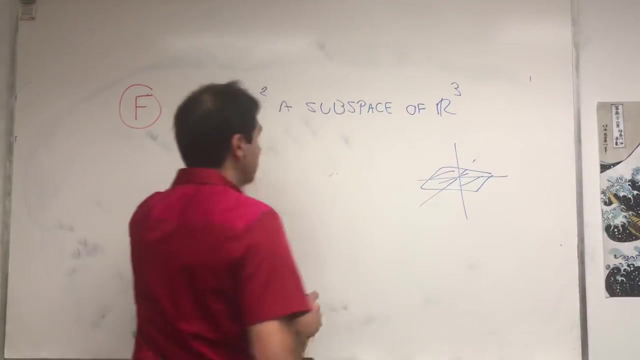 It's true that the xy-plane you see is a subspace of R3,, but the xy-plane that's not R2, it's just R2 with a zero and, in particular, R2 is not a subspace of R3, because it's not a subset. 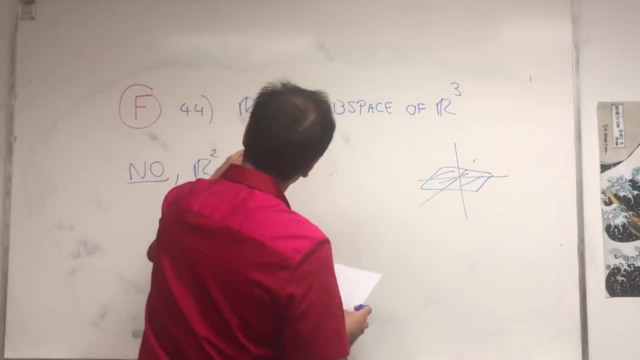 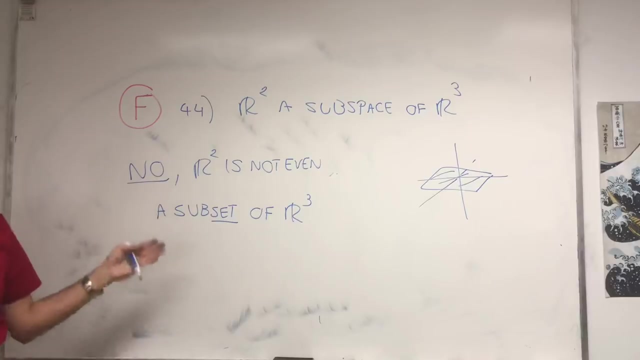 So no, R2 is not even a subset, It's a subset of R3. In other words, if you want to show something is a subspace, you need to make sure that they're both of the same type. It's impossible to compare the vector with the vector. 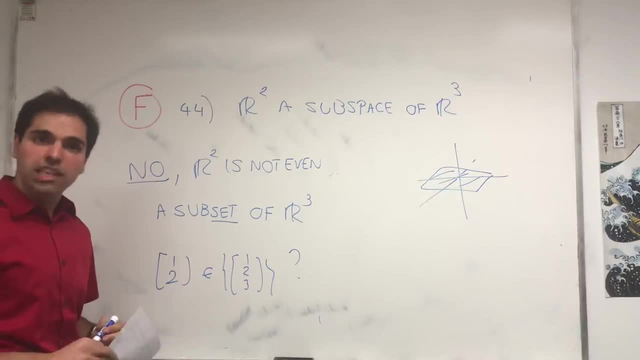 That doesn't really make sense and in fact if you try to input in a computer program that accepts three inputs, The computer program is like I have no idea what you mean and it gives you an error message. So make sure that for subspaces, your two sets are of the same type and, as I said, 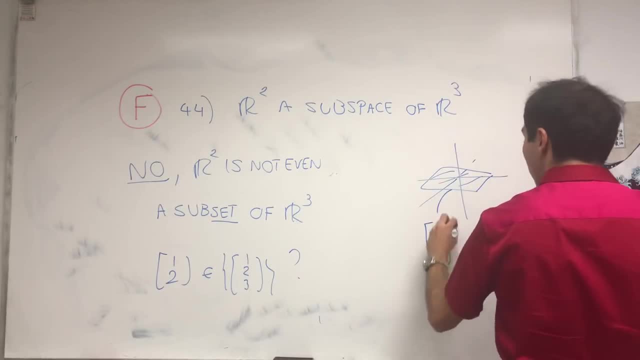 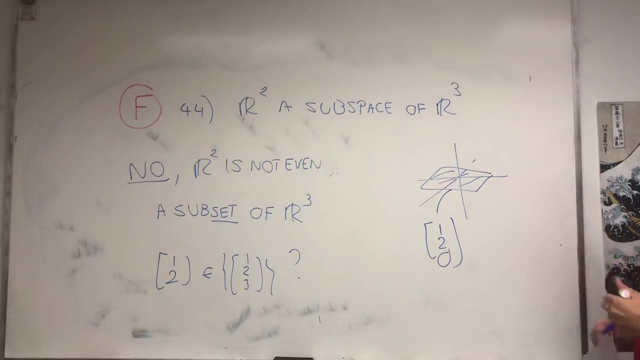 if you think of this as just a .120,, you know like 12 as a vector 120, then yes, then we can start talking about whether it's a subspace or not. So just be very careful. That said, you can actually think of R2 as a subspace of R3, but with the isomorphism. 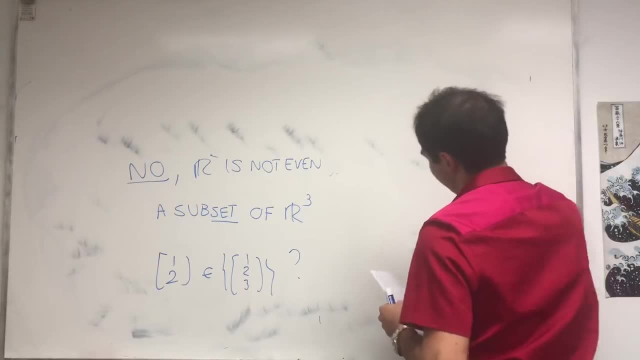 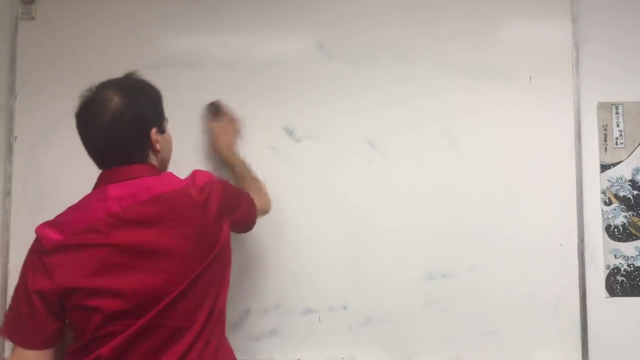 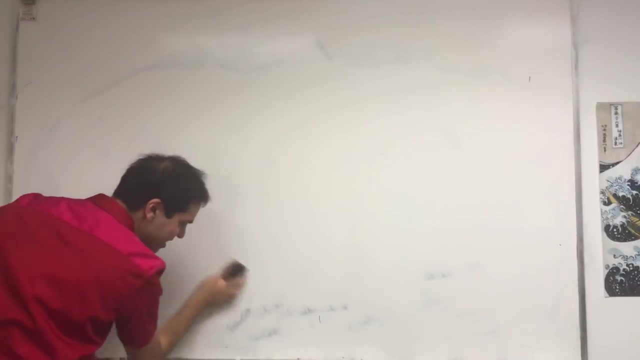 and everything related to that. So your intuition is correct. It's just you need to make sure that rigorously it's correct. Okay, and I'm just spreading this so it looks kind of legible and in fact let me double check something. 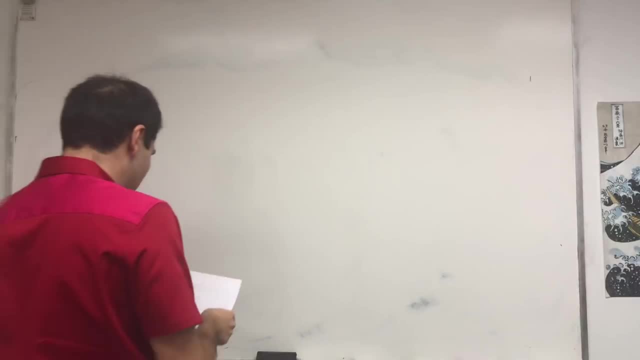 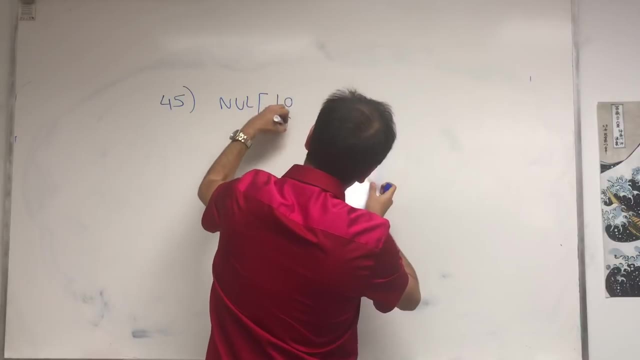 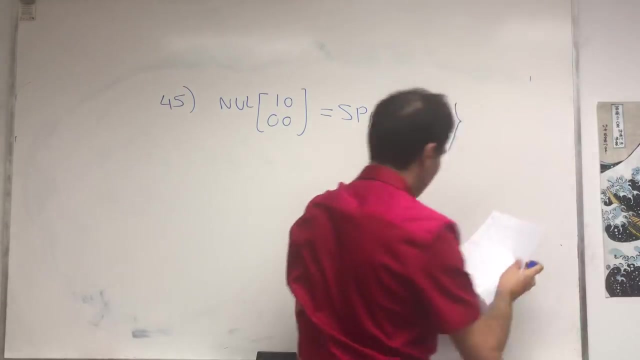 So yeah, almost two hours in counting. So next one. so null space. let's talk null space a bit. null space of 1, 0, 0, 0, is it the span of 1, 0?? 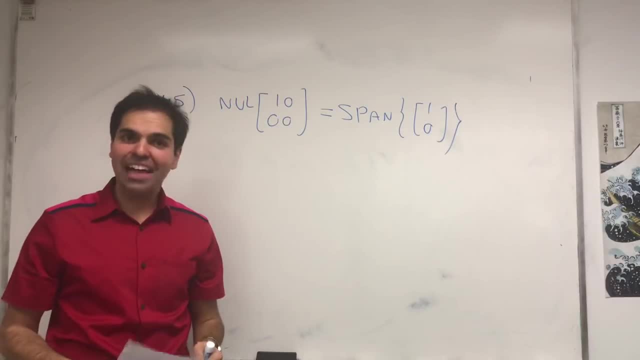 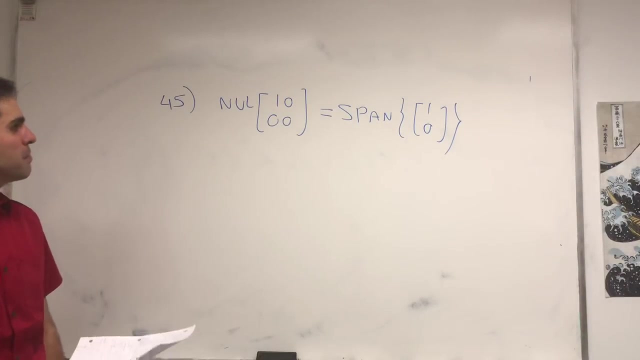 And for the fifth language, another dialect of Chinese, the dialect of Chinese, and it's really cute. It's, It's not, It's. It sounds like sushi. That's why I like it. so So is it true that the null space is the span of this? 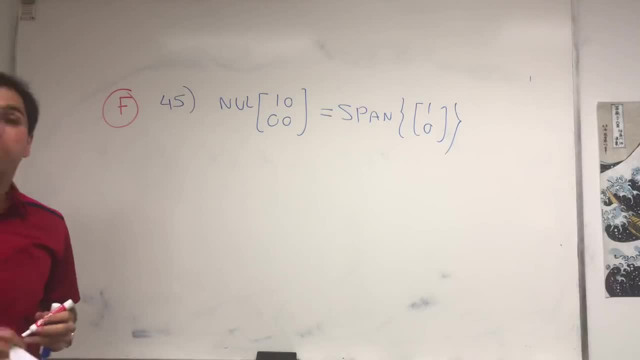 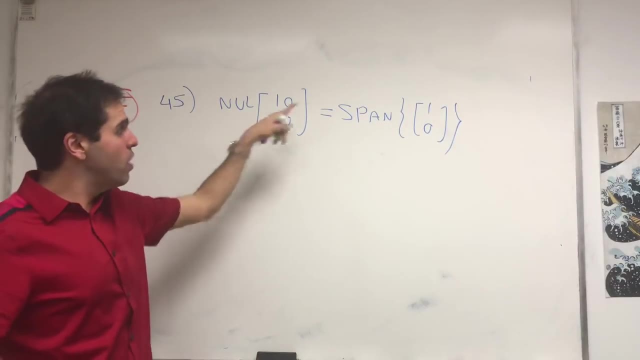 Again, unfortunately false. and this is super important For null space. don't try to find a shortcut. Usually, intuitively, you think: well, it should be 1, 0 because there's a 1, 0 here, but really, as someone who took linear algebra, I think that something really important about this is that there's an increase Or there's a decrease, So what's true is that the Chinese, including that Chinese, have the same sum here and so 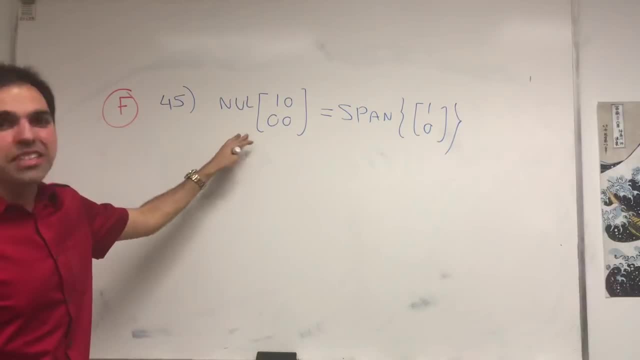 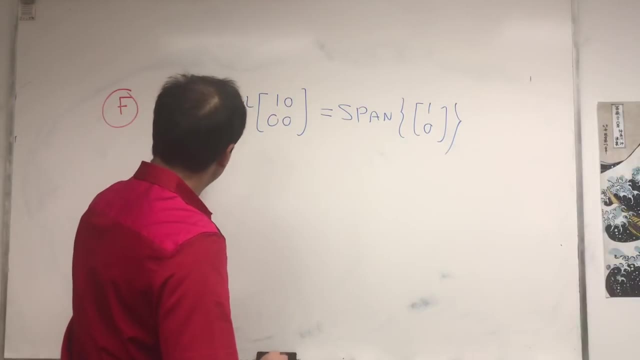 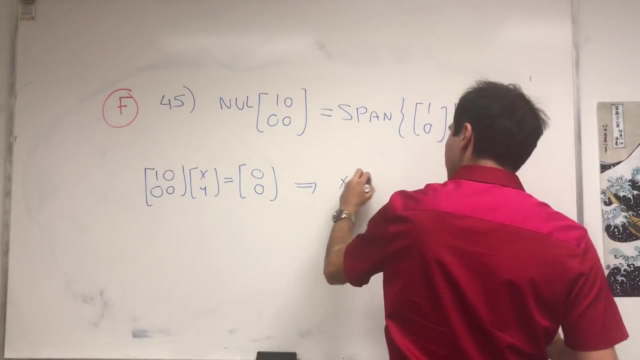 long time ago. I can guarantee you it's much better just to do it slowly. so what is the null space? it's the set of solutions of this equals to 0 and that if you multiply this out, you get x equals 0 and 0 equals 0, and then your. 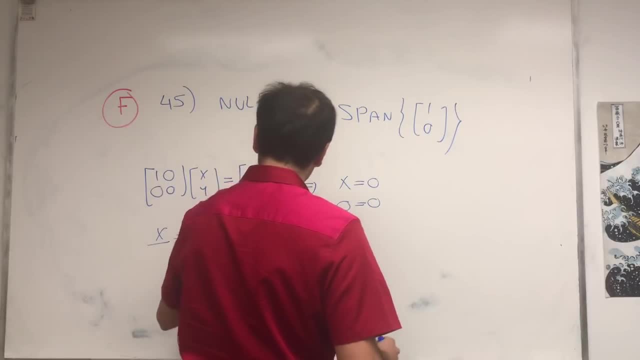 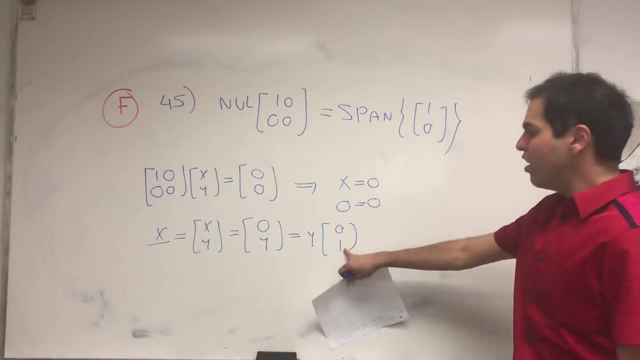 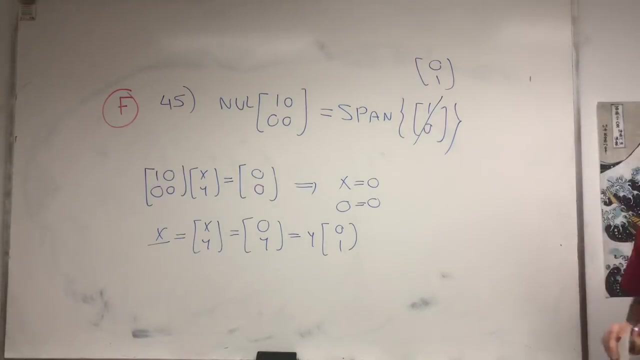 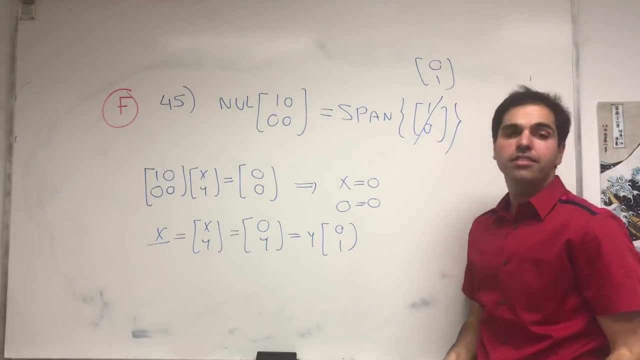 vector in the null space is X, Y, which is 0, Y, which is Y times 0- 1. so you see, your null space is not the span of 1: 0, it's the span of 0: 1 and indeed it cannot be the span of 1: 0, because if you apply that matrix to 1: 0, you don't get. 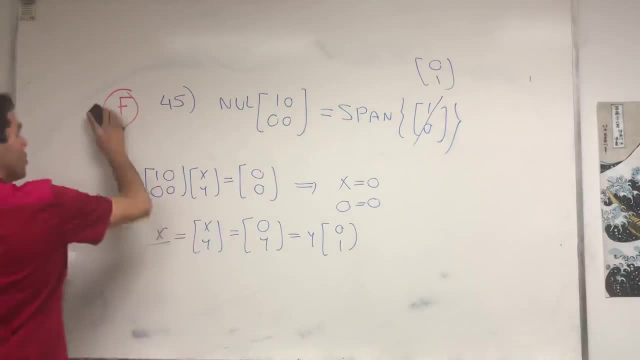 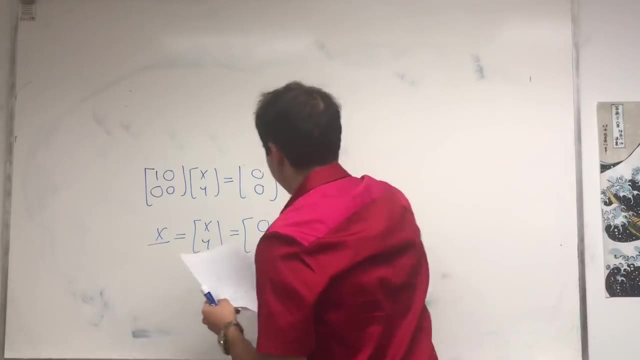 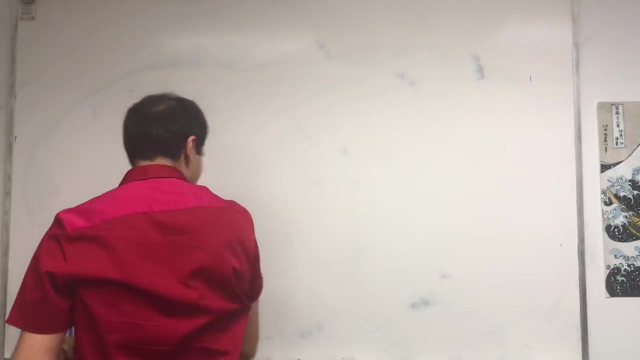 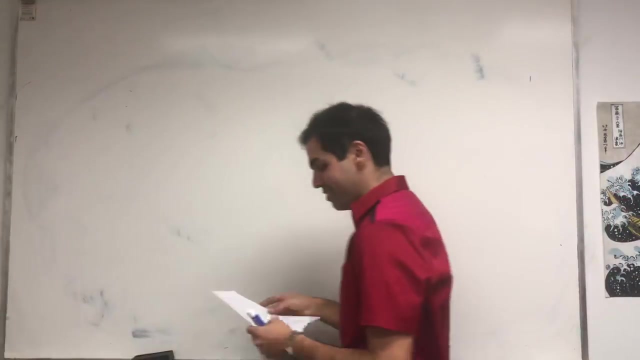 0, so just a cautionary tale. moving on, a little bit more about subspaces. this is a long section, bunch of lots of questions, and you let me see how many questions. so it'll go up to question 70 in that thing. so when we're, we're at 46. 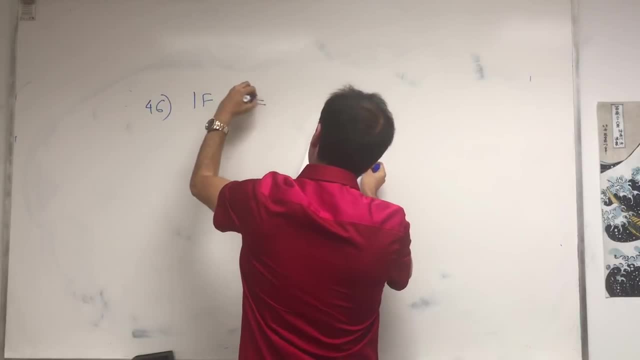 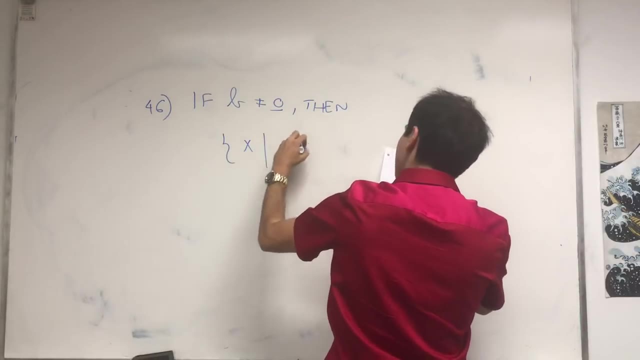 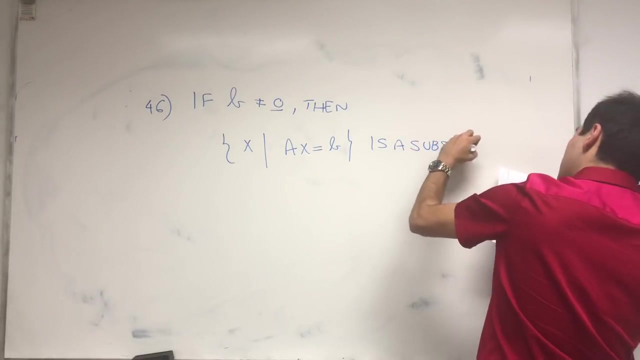 so if P is non-zero, then let's consider something similar to this. so if P is non-zero, then let's consider something similar to this. so if P is non-zero, then let's consider something similar to this: to the null space, the set of X, which AX equals B, is a subspace of RN. so what if? 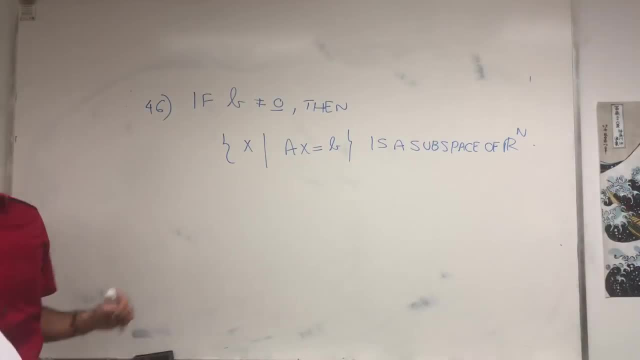 you consider the null space, except, instead of AX equals 0, it's AX equals B. is this or is this not a subspace of RN? and also 46 Awati and 46 is Chialis? this or is this not a subspace of RN, and also 46 Awati and 46 is Chialis? 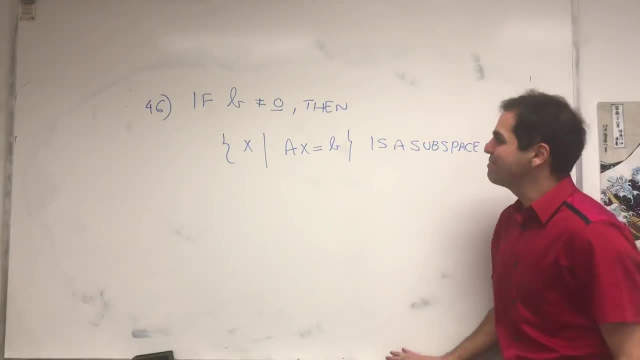 almost like Chialin. if you know who that is almost like Chialin. if you know who that is almost like Chialin. if you know who, that is all right and it is false. so this is kind of all right and it is false. so this is kind of. 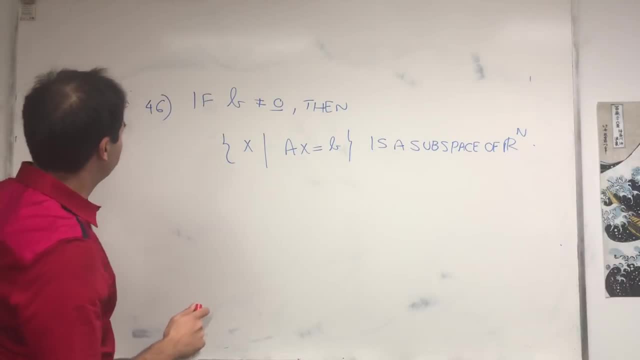 all right and it is false. so this is kind of depressing round lots of false things. depressing round lots of false things, depressing round lots of false things. in fact, this is why we never really talk. in fact, this is why we never really talk. in fact. this is why we never really talk about this. and why is this not a? 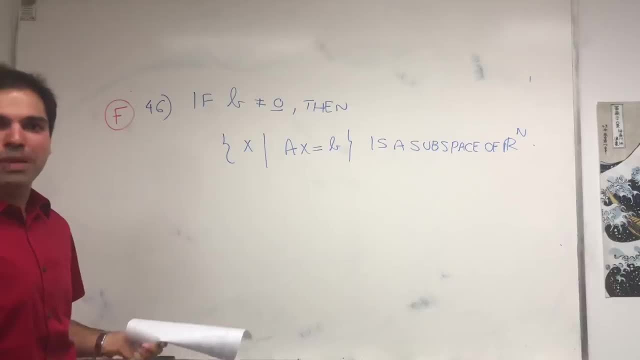 about this and why is this not a about this? and why is this not a subspace? remember to check something is a subspace. remember to check something is a subspace. remember to check something is a subspace. one of the requirements is: is subspace. one of the requirements is is. 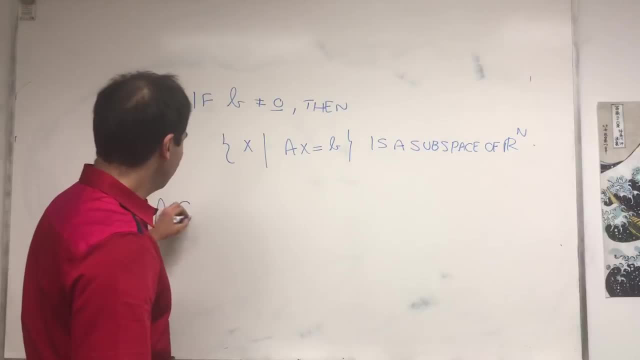 subspace. one of the requirements is: is the zero vector in it? so the question is: the zero vector in it, so the question is the zero vector in it. so the question is: is a times 0 equals B, equal to B, and is a times 0 equals B, equal to B, and. 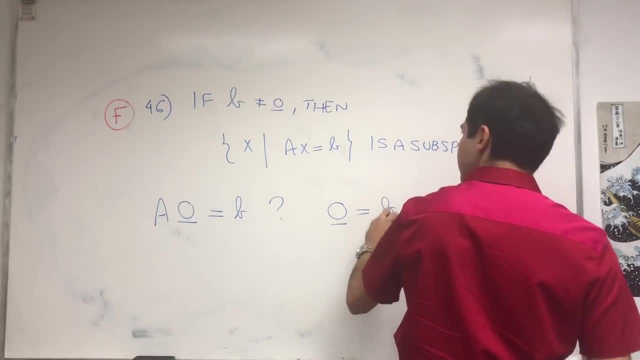 is a times 0, equals B, equal to B, and then, unfortunately it's not because that, then unfortunately it's not because that, then unfortunately it's not because that would imply 0 is B, but we just assume would imply 0 is B, but we just assume. 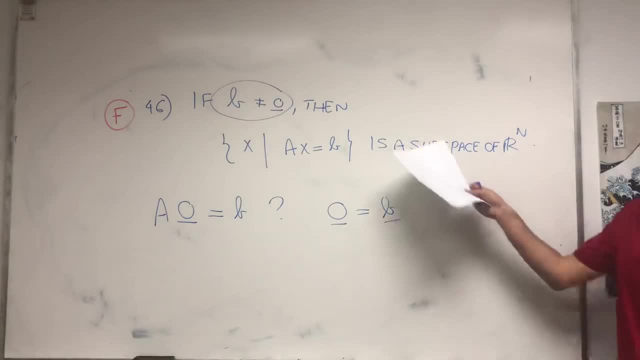 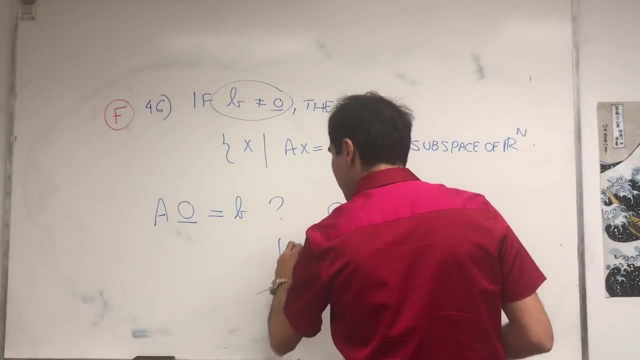 would imply: 0 is B, but we just assume that B is nonzero, so it is not a. that B is nonzero, so it is not a. that B is nonzero, so it is not a subspace. unfortunately it's something subspace. unfortunately it's something subspace. unfortunately it's something called an affine space, because remember, 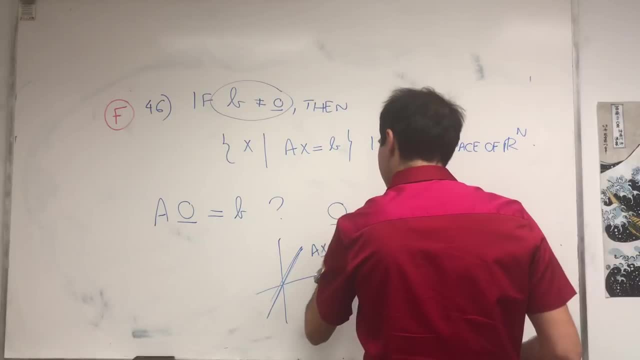 called an affine space because, remember, called an affine space? because, remember, the set of ax equals 0, that's a subspace. the set of ax equals 0, that's a subspace. the set of ax equals 0, that's a subspace, it's the null space. and ax equals B is. 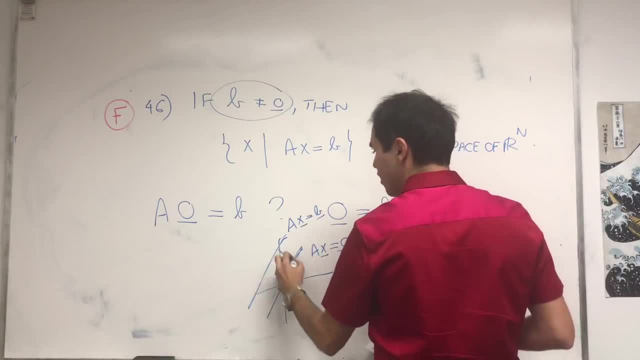 it's the null space and ax equals B is. it's the null space and ax equals B is actually just a translate of this. so if actually just a translate of this, so if actually just a translate of this, so if you translate it by the what's called, 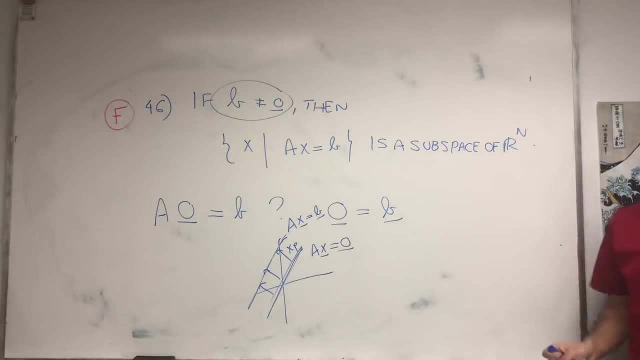 you translate it by the what's called. you translate it by the what's called: remember particular solution? then we remember particular solution, then we remember particular solution. then we actually get ax equals B and that's why actually get ax equals B and that's why actually get ax equals B and that's why not quite a subspace. it's called an. 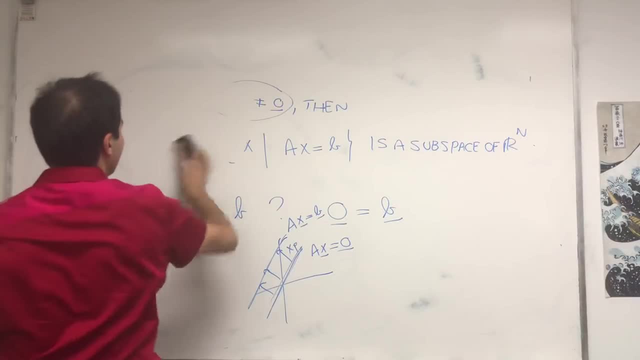 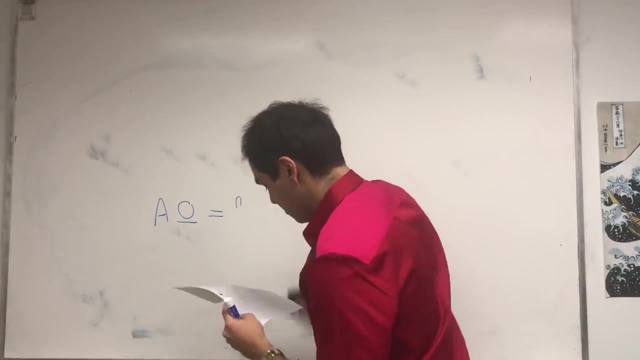 not quite a subspace, it's called an, not quite a subspace, it's called an affine space. okay, another one, let's see affine space. okay, another one, let's see affine space. okay, another one, let's see. can we break this streak of falses? well? 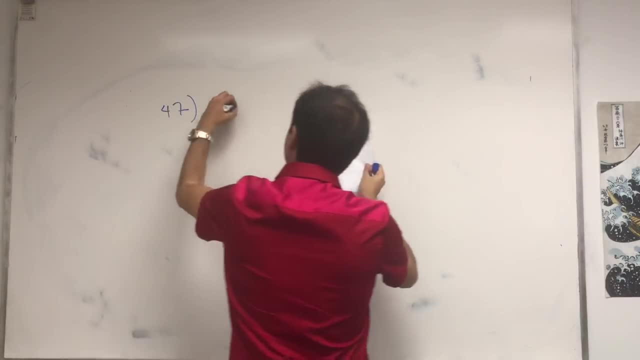 can we break this streak of falses? well, can we break this streak of falses? well, let's see, let's see, let's see. question 47 a, 4 by 6, matrix with two. question 47 a: 4 by 6 matrix with two. 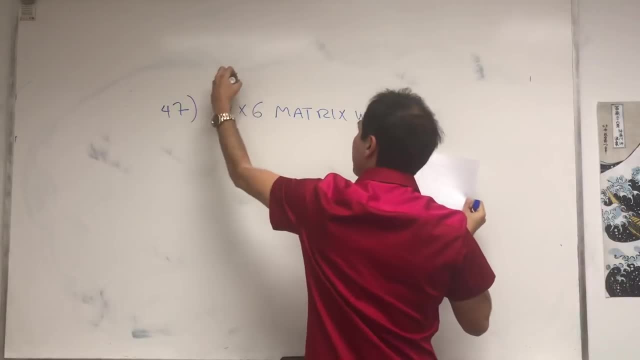 question 47: a 4 by 6 matrix with two pivot columns. so if a sorry if a is a pivot columns. so if a sorry if a is a pivot columns, so if a sorry if a is a 4 by 3, 4 by 3, 6 matrix with two pivot columns. so if a sorry if a is a 4 by 3, 6. 4 by 3, 6 matrix with two pivot columns. so if a- sorry, if a- is a 4 by 3, 6, 4 by 3, 6 matrix with two pivot columns. so if a is a 4 by 3, 6 matrix with two pivot. 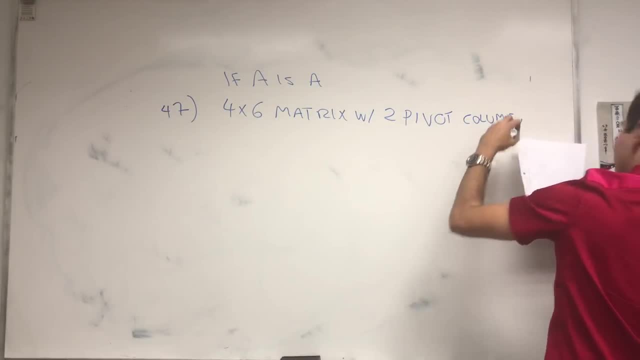 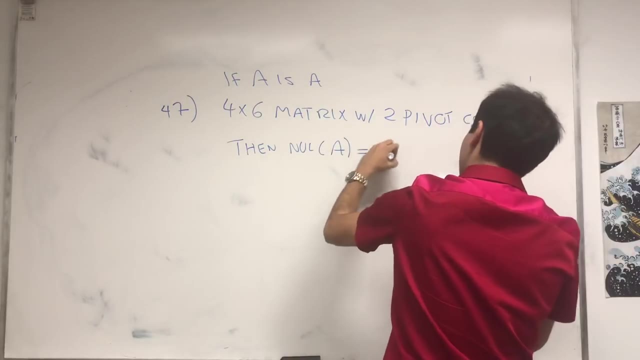 matrix with two pivot columns. so if a is a 4 by 3, 6 matrix with two pivot matrix with two pivot columns, so if a is a 4 by 3, 6 matrix with two pivot columns, then the null space of a equals to our. 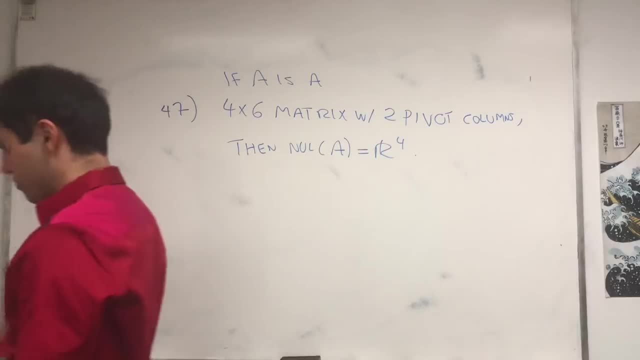 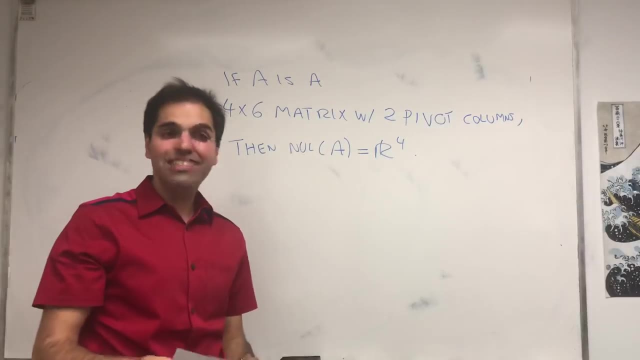 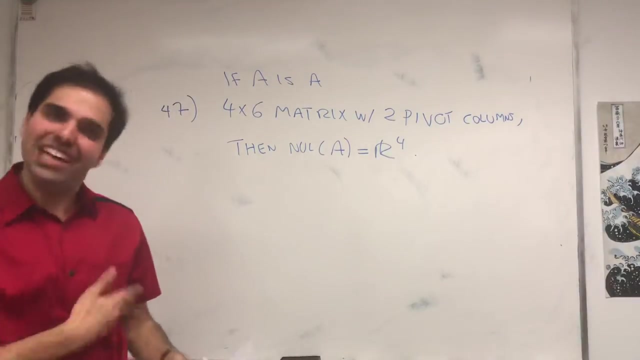 columns, then the null space of a equals to our columns, then the null space of a equals to our form. oh and 47 tie and 47 ties, and see. oh and 47 tie and 47 ties, and see oh and 47 tie and 47 ties, and see. subject: time 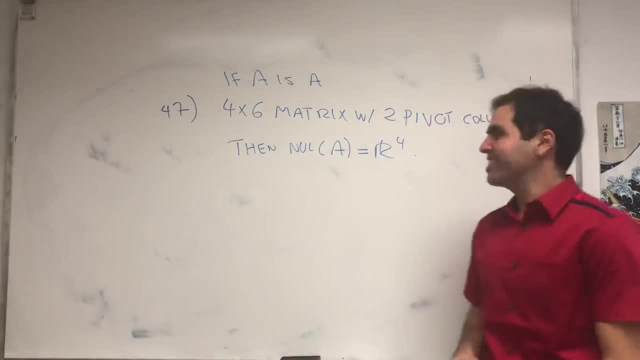 subject time: subject time: i need to learn thai because i'm going to. i need to learn thai because i'm going to. i need to learn thai because i'm going to thailand in like a week actually, oh my. thailand in like a week actually, oh my. 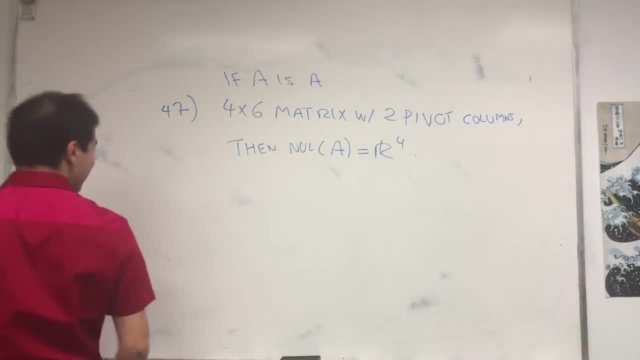 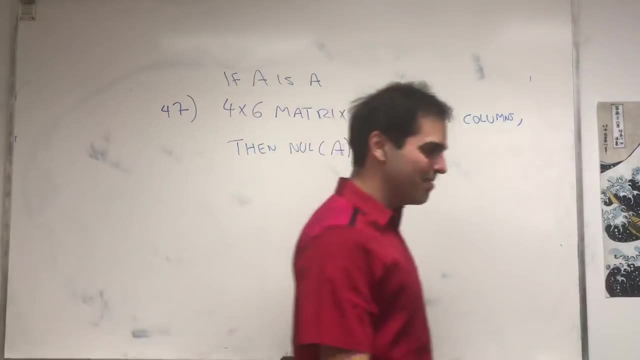 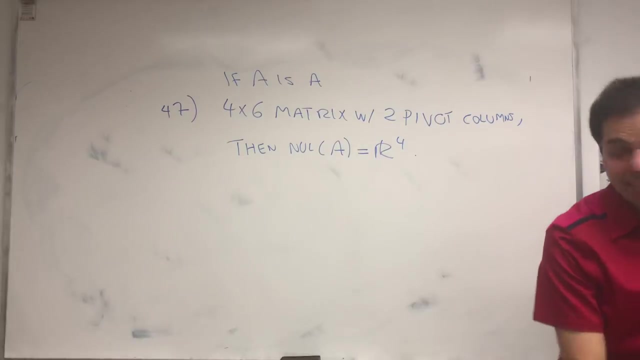 thailand in like a week actually. oh, my god, all the good food. i'm so excited what's called the mango sticky rice, and unfortunately, we did not break the and unfortunately we did not break the and unfortunately we did not break the speak of falses, because this is also 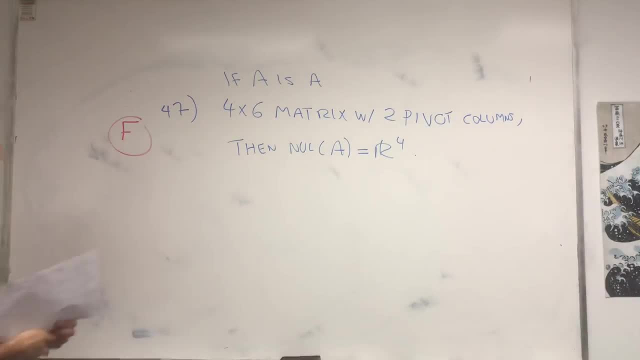 speak of falses, because this is also speak of falses, because this is also false, false, false. in fact, this question doesn't really in fact. this question doesn't really, in fact, this question doesn't really make sense. it's like the same question make sense, it's like the same question. 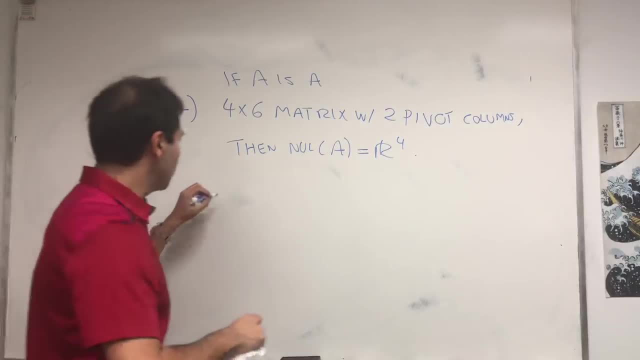 make sense. it's like the same question with r2 is a subspace of r3, because look with r2 is a subspace of r3. because look with r2 is a subspace of r3, because look if a is a four by six matrix. 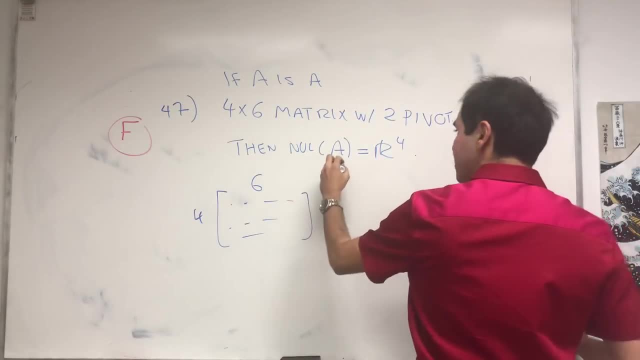 if a is a four by six matrix, if a is a four by six matrix. like that, something like that, right then. like that, something like that, right then. like that, something like that, right then. null space has to do with a x equals. null space has to do with a x equals. 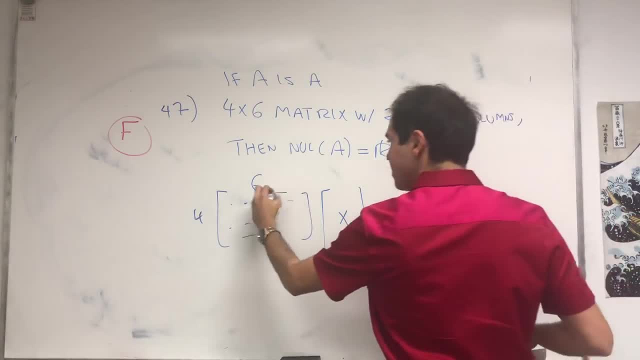 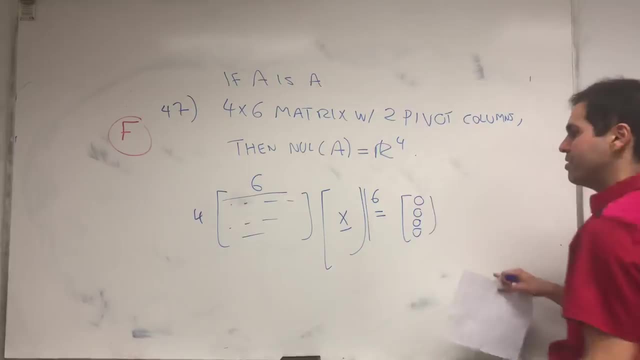 null space has to do with a. x equals zero, zero, zero. and in that case, in order for this to, and in that case, in order for this to, and in that case, in order for this to make sense, x needs to be of size six. so you see, the null space cannot be r4. 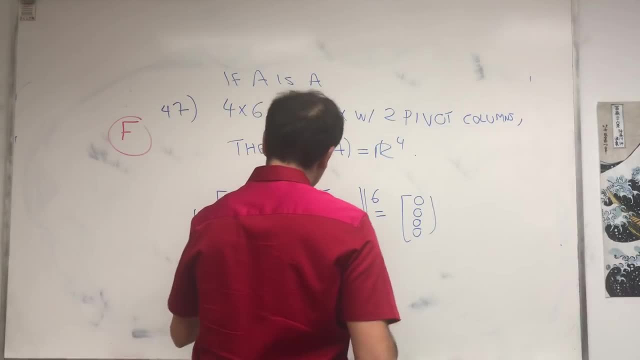 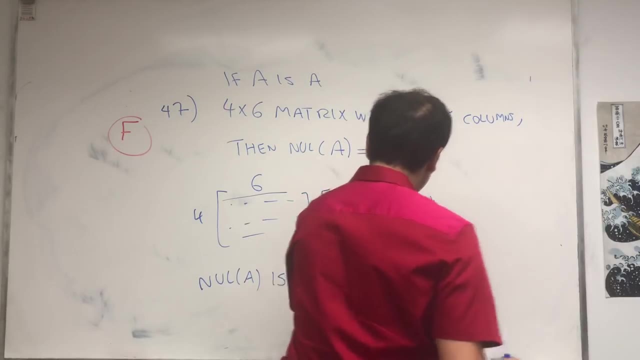 so you see, the null space cannot be r4. so you see the null space cannot be r4 because the null space of a, because the null space of a, because the null space of a is a subset of r6, because if we talk about ax equals zero. 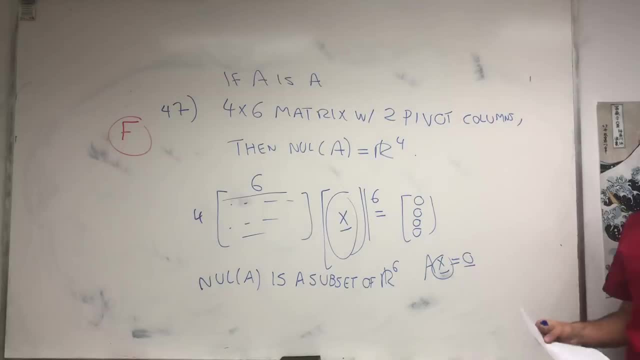 because if we talk about ax equals zero, because if we talk about ax equals zero, in this case, is x needs to be a vector. in this case, is x needs to be a vector. in this case, is x needs to be a vector with six entries, with six entries. 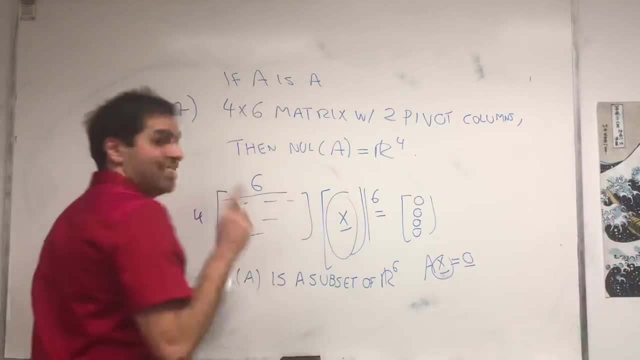 with six entries cannot be a vector with four entries. cannot be a vector with four entries, cannot be a vector with four entries. that said it is true that the null, that said it is true that the null, that said it is true that the null space is a four-dimensional subspace of 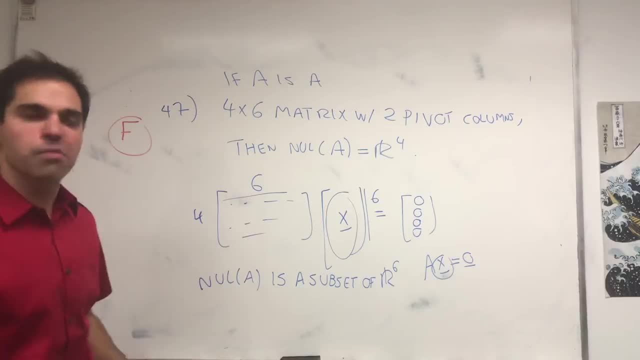 space is a four-dimensional subspace of space is a four-dimensional subspace of r6, and that's from the rank nullity r6, and that's from the rank nullity r6, and that's from the rank nullity theorem, which i'll talk about later. 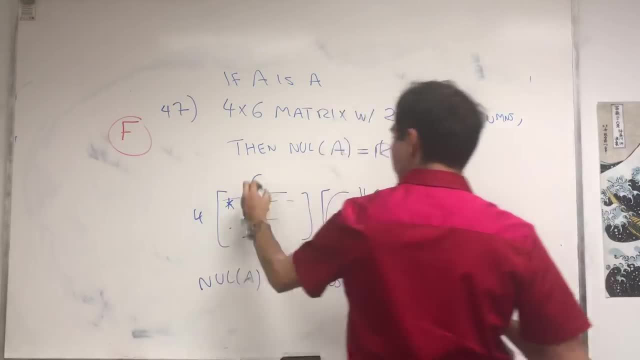 theorem which i'll talk about later, theorem which i'll talk about later, because if you have two pivot columns, because if you have two pivot columns, because if you have two pivot columns, then there's sort of four free variables, then there's sort of four free variables. 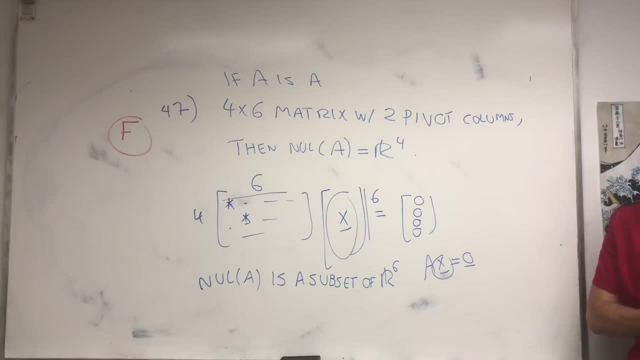 then there's sort of four free variables. so the null space is sort of so. the null space is sort of so. the null space is sort of dimension of the null space is a dimension of the null space is a dimension of the null space is a number of free variables, so it is. 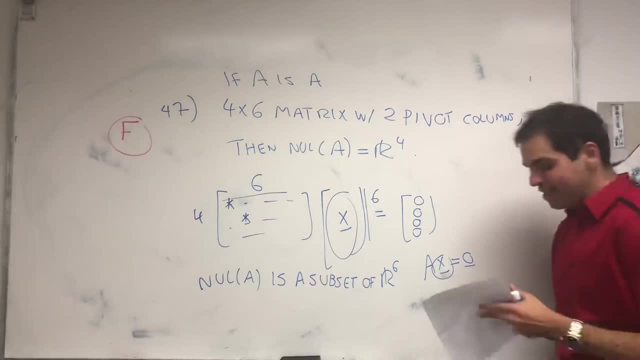 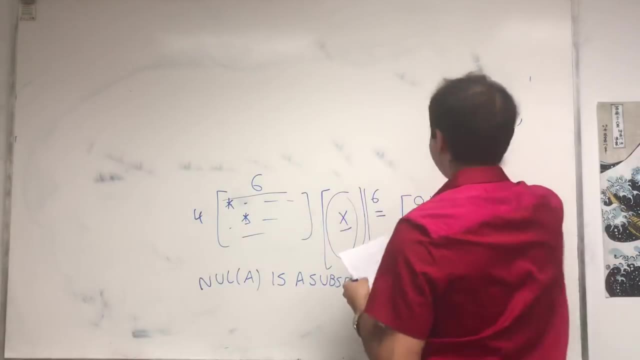 number of free variables. so it is number of free variables. so it is indeed a four-dimensional subspace, but indeed a four-dimensional subspace, but indeed a four-dimensional subspace, but of r6, of r6, of r6. okay, good, maybe now can we break the streak of. 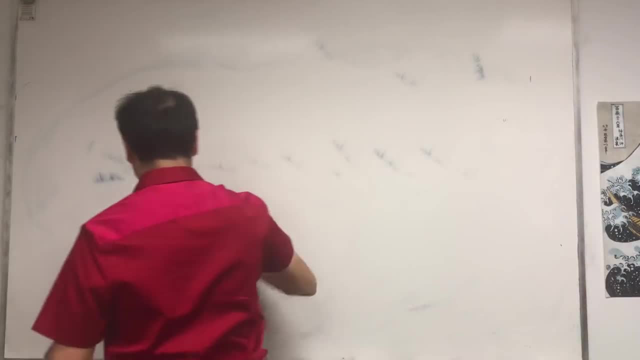 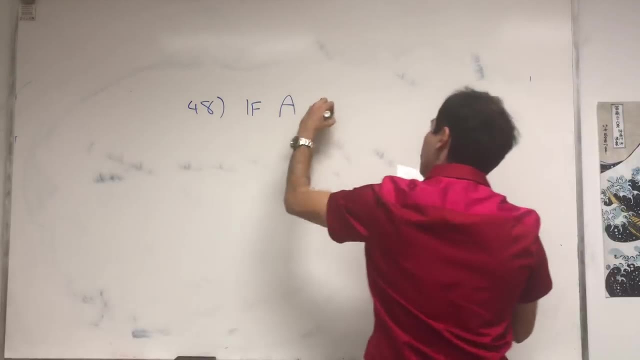 maybe now can we break the streak of. maybe now can we break the streak of: false or true or falses. false or true or falses. false or true or falses. let's see so: 48 if a again a m by n matrix has. if a again a m by n matrix has. 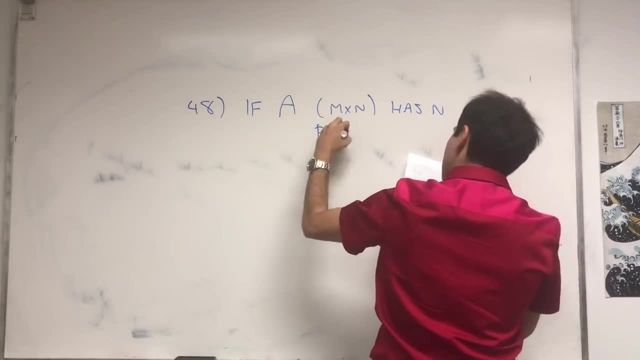 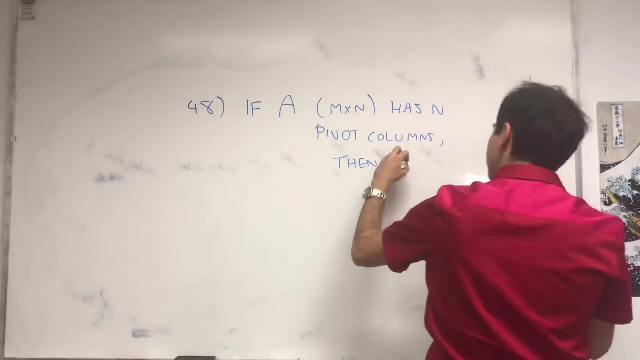 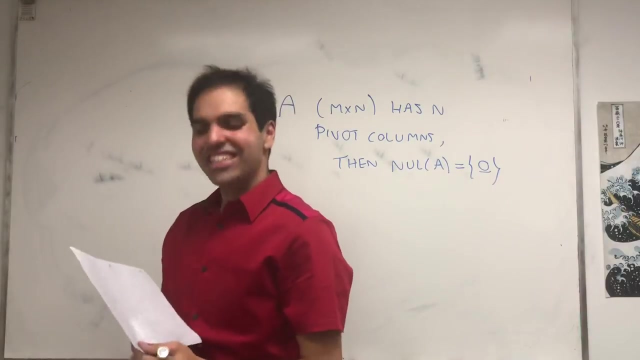 if a, again a m by n matrix, has n pivot columns, n pivot columns, n pivot columns, then the null space of a, then the null space of a, then the null space of a is the trivial space, is the trivial space, is the trivial space and 48 dutch. 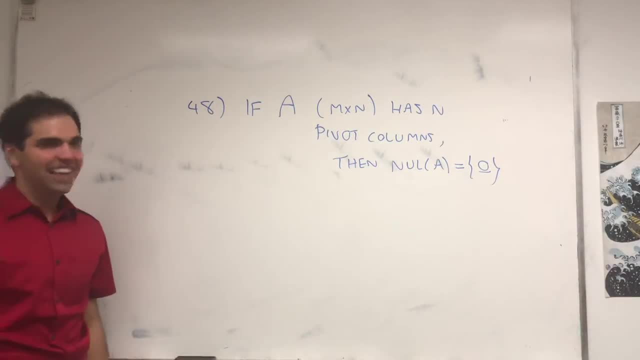 and 48 dutch and 48 dutch and 48 and 48 dutch. i love dutch. it sounds like german. i love dutch. it sounds like german. i love dutch. it sounds like german. but you do a lot of ha ha ha. 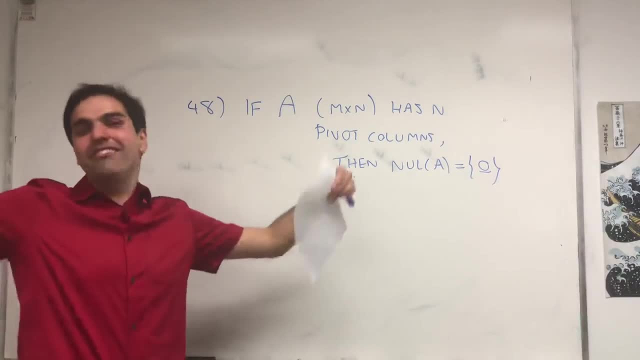 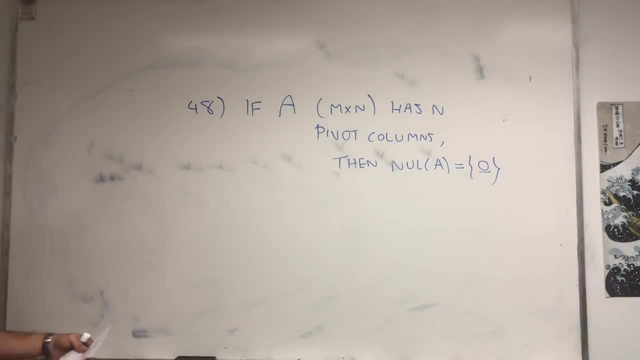 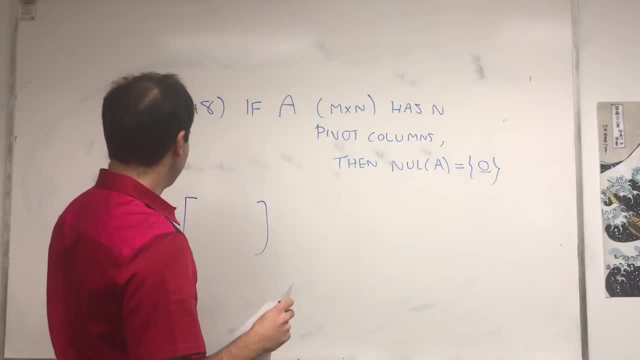 so this is true. and why is that true? because, because, because, well, suppose you have a matrix a m by, well, suppose you have a matrix a m by well, suppose you have a matrix a m by n, and basically what this tells you is n, and basically what this tells you is: 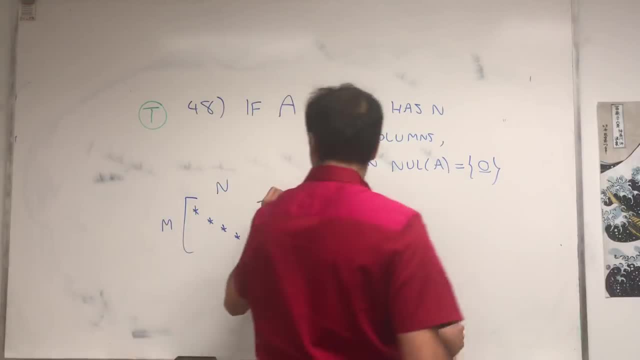 n and basically what this tells you is: there's a pivot in every column, there's a pivot in every column, there's a pivot in every column. okay, okay, okay. and if there's a pivot in every column, and if there's a pivot in every column, and if there's a pivot in every column, there are no free variables. 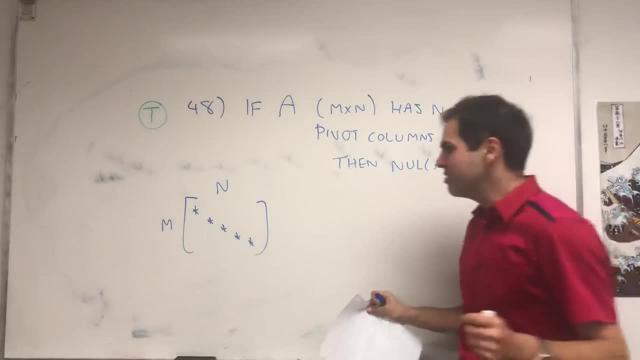 and remember no space sort of measures and remember no space sort of measures and remember no space sort of measures, the free variables, the free variables, the free variables. so in particular, if you have a matrix, so in particular, if you have a matrix, so in particular if you have a matrix like that and you want to solve ax. 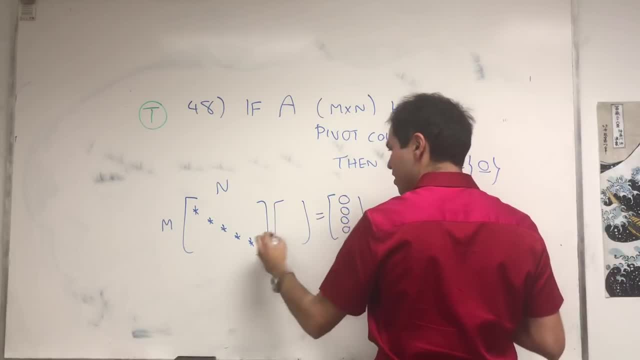 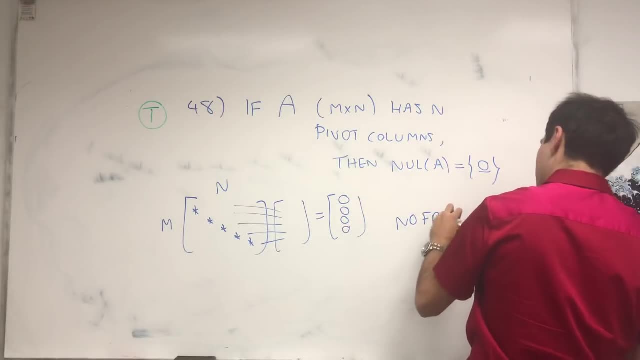 like that. and you want to solve ax like that and you want to solve ax equals to zero, then you know every x is actually zero, then you know every x is actually zero, then you know every x is actually zero. so, so, so, no free variables. so, in fact, ax equals to zero, cannot have. 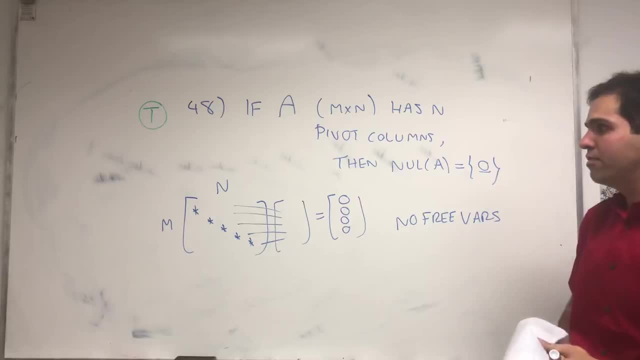 so, in fact, ax equals to zero. cannot have, so, in fact, ax equals to zero. cannot have a non-trivial solution. a non-trivial solution, a non-trivial solution. otherwise you would have had a free, otherwise you would have had a free, otherwise you would have had a free variable. okay, good. 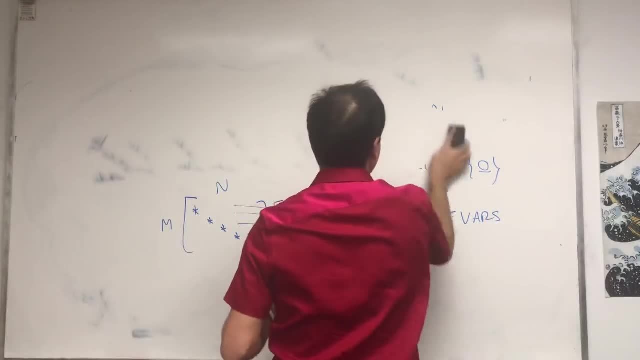 variable: okay, good, variable, okay, good. so we've broken that streak and i so we've broken that streak and i, so we've broken that streak and i taught you about all spaces, taught you about all spaces, taught you about all spaces. but now what about the column space? 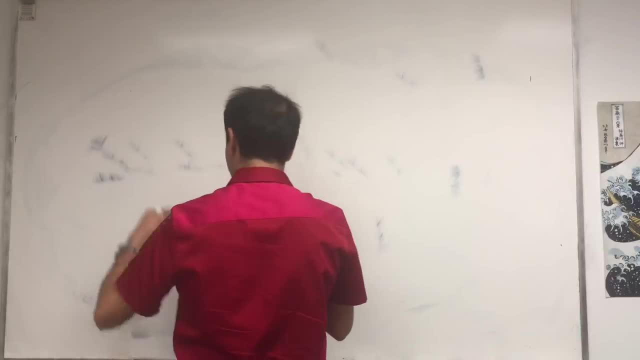 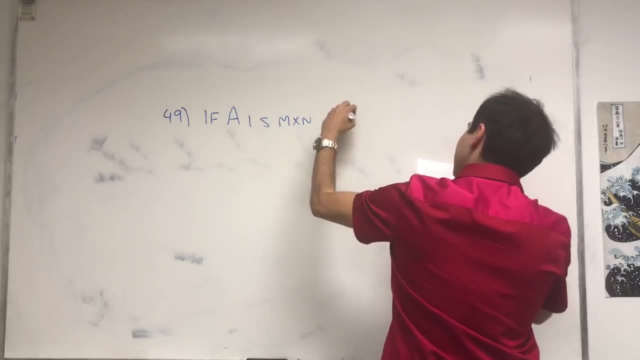 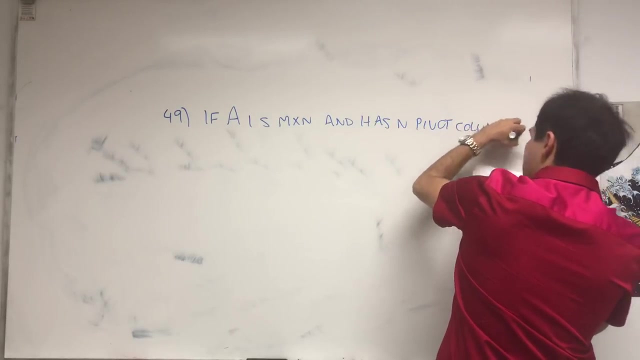 but now what about the column space? but now, what about the column space? so so this time, if a is m by n, so this time, if a is m by n, so this time, if a is m by n and has a pivot in every column, and has a pivot in every column. 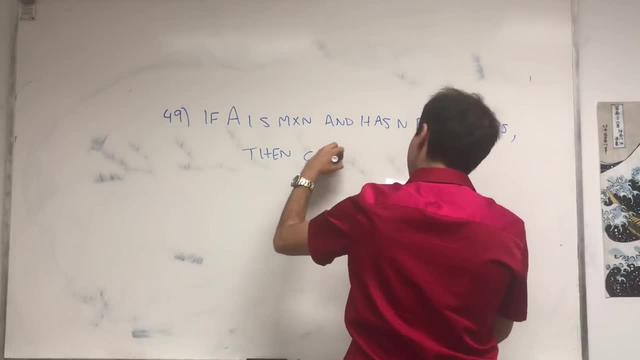 and has a pivot in every column, then the column space, then the column space, then the column space is the whole space. so in this case is the whole space. so in this case is the whole space. so in this case, columns has to with mouth puts, so m 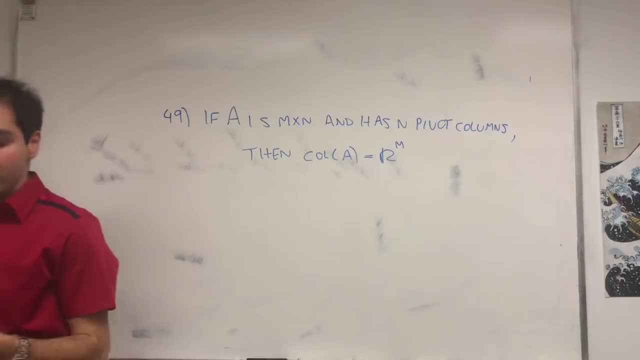 columns has to with mouth puts, so m. columns has to with mouth puts, so m and language 49 again. i've never heard, and language 49 again. i've never heard, and language 49 again. i've never heard. of it, but of it, but of it. but yoruba and. 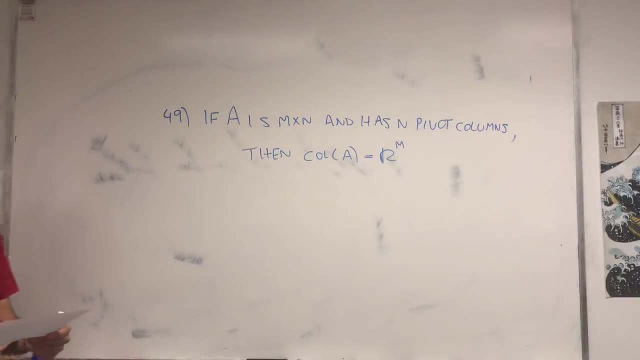 yoruba and yoruba and 49 yoruba is a good g major. let me check, let me check, let me check. good, we're good. oh man, this looks good, we're good. oh man, this looks good, we're good. oh man, this looks really dirty. sorry. 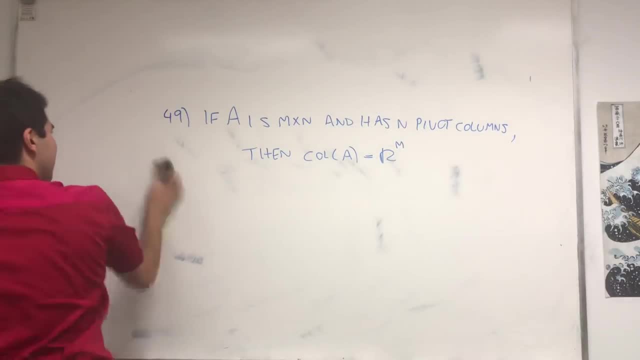 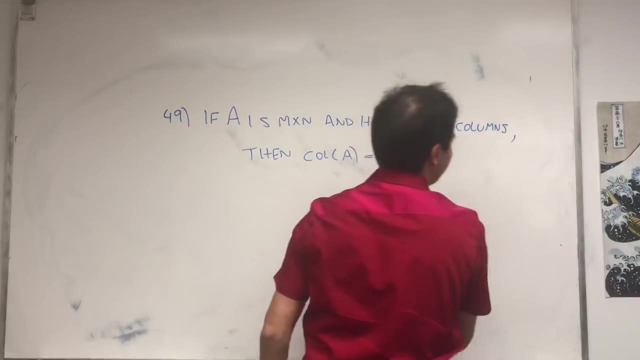 really dirty sorry, really dirty sorry. um, again, i'm trying my best. hey, at least there's a kind of the hey, at least there's a kind of the hey. at least there's a kind of the angle issue. i think is gone. so that's angle issue, i think is gone, so that's. 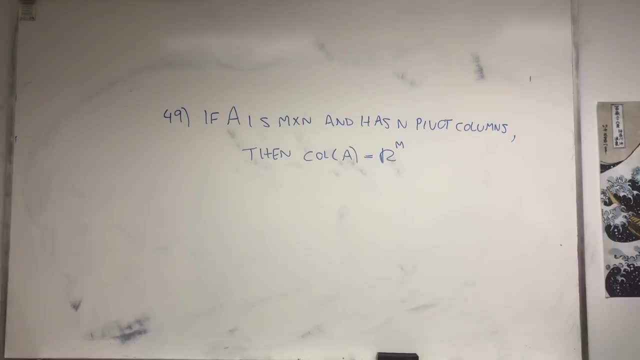 angle issue, i think, is gone, so that's good, i did listen to you guys. good, i did listen to you guys. good, i did listen to you guys. i don't think i didn't listen. let me do something, so i don't know how helpful this will be i. 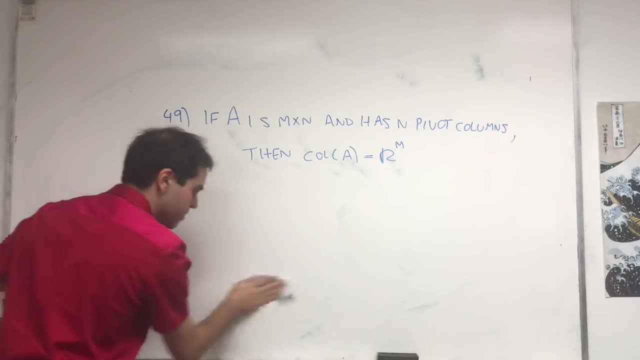 i don't know how helpful this will be. i i don't know how helpful this will be. i do have a do have a do have a spare one here, spare one here, spare one here. okay, okay, okay, i can think about this question long. i can think about this question long. 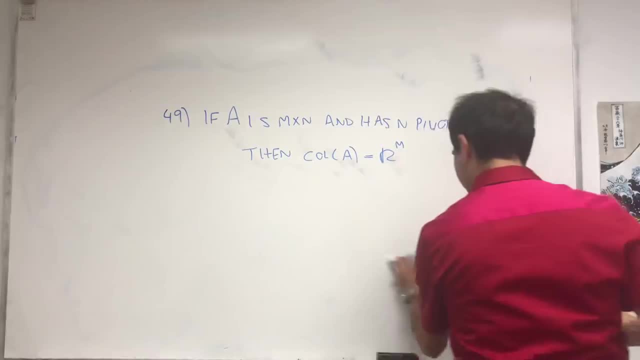 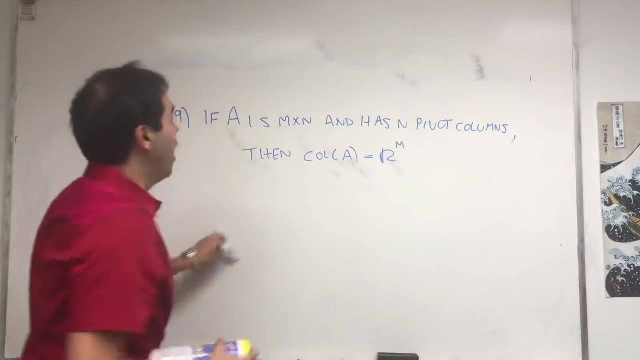 i can think about this question long and hard while and hard while and hard while, trying to fix stuff well, yeah, maybe trying to fix stuff well. yeah, maybe trying to fix stuff well, yeah, maybe, okay, not too bad, yeah, okay. so it turns out if there's a pivot, 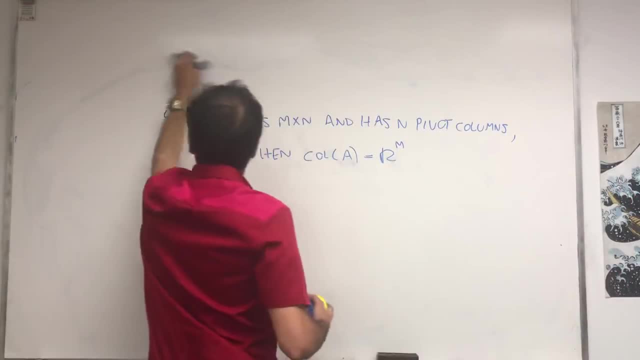 okay, so it turns out. if there's a pivot, okay, so it turns out. if there's a pivot in every column, in every column, in every column, the column space, even in that case, is the column space. even in that case is the column space, even in that case, is not the whole space. so, in fact, the 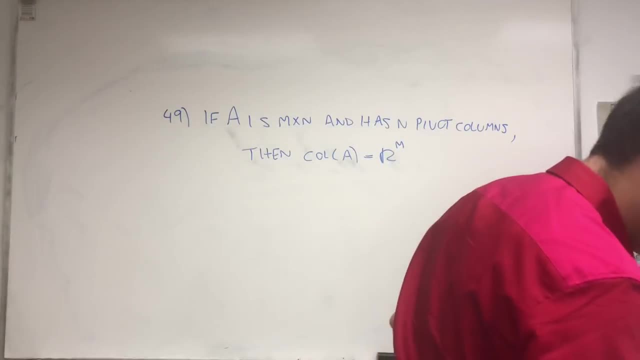 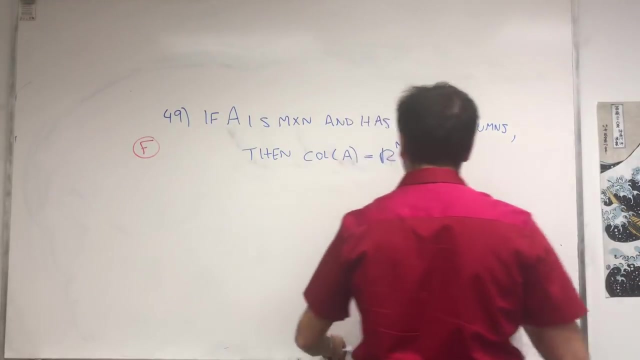 not the whole space. so in fact, the not the whole space. so in fact, the answer is: answer is answer is fun, fun, fun, fun, fun, else else. where did it go? yeah, let me give you an. where did it go? yeah, let me give you an. where did it go? yeah, let me give you an example. 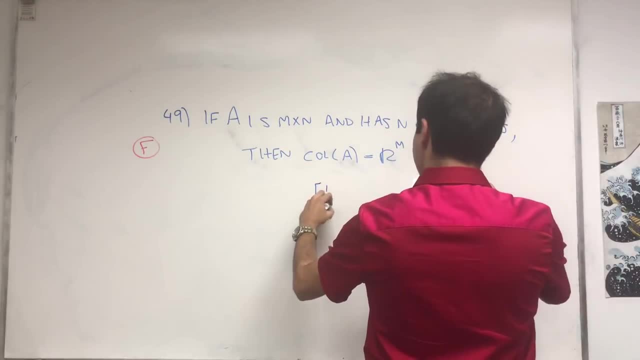 for example, let's say this matrix: so uh. for example, let's say this matrix: so uh. for example, let's say this matrix: so uh, one zero, zero, zero, one, zero, one, zero, zero, one, zero, one, zero, zero, one, zero. yes, it has a pivot in every column. 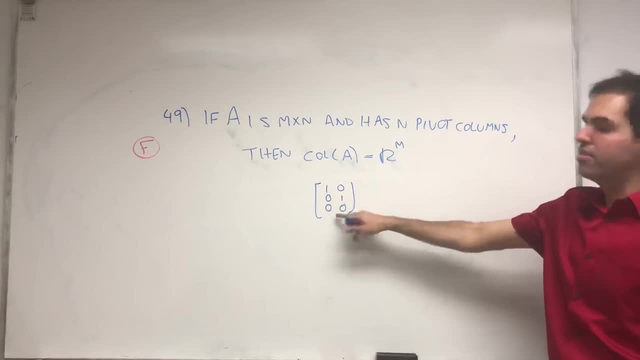 yes, it has a pivot in every column. yes, it has a pivot in every column, but the column space is just something. but the column space is just something. but the column space is just something, something zero, so it's the um. something zero, so it's the um. 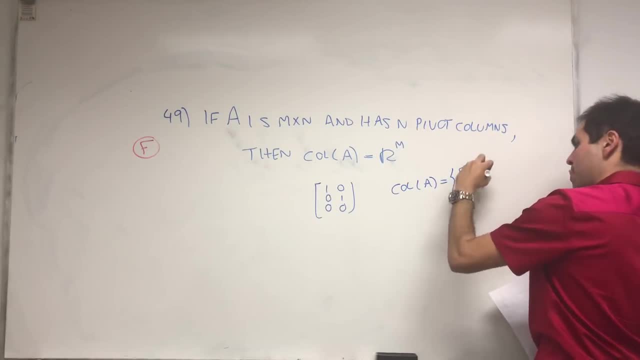 something zero. so it's the um, what's called? what's called? what's called, it's the xy plane. it's the xy plane. it's the xy plane where x, y and r, where x, y and r, where x, y and r. so it's not the same as rth way. 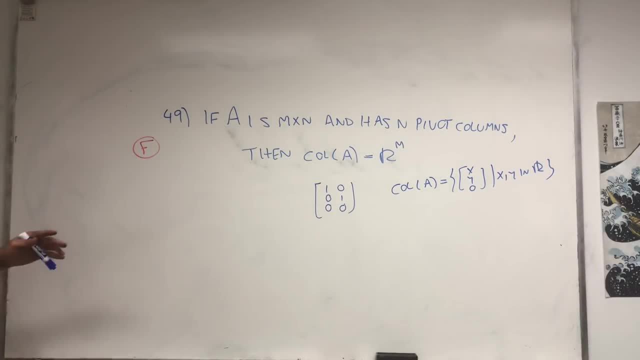 so it's not the same as rth way. so it's not the same as rth way, so be very careful. that said, if it has, so be very careful. that said, if it has, so be very careful. that said, if it has n m pivot rows, then it is true that the 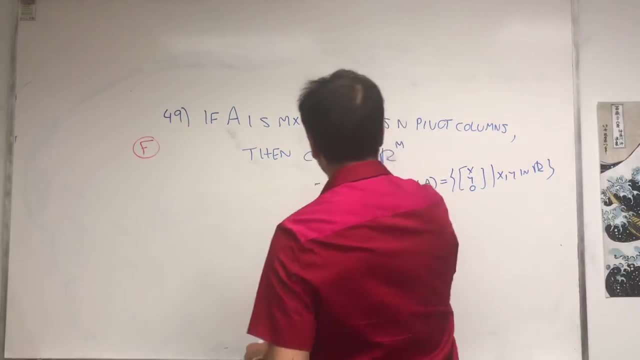 n? m pivot rows. then it is true that the n? m pivot rows. then it is true that the column space is rm. column space is rm. column space is rm. okay, good, that's good. now whoo question 50. so that's good, now whoo question 50. so 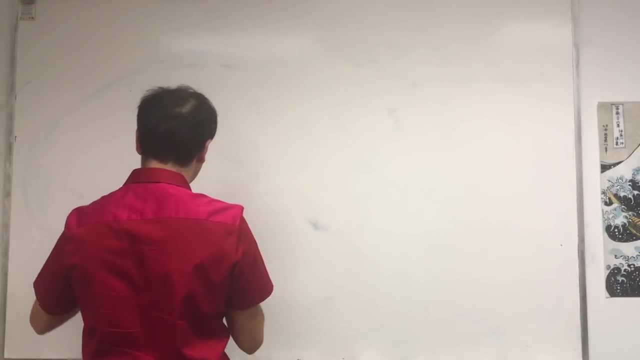 that's good. now, whoo, question 50. so we're almost at the halfway mark. so we're almost at the halfway mark. so we're almost at the halfway mark. so this one, also, this one, also this one also interesting, interesting, interesting. so if a is equivalent to b, then the 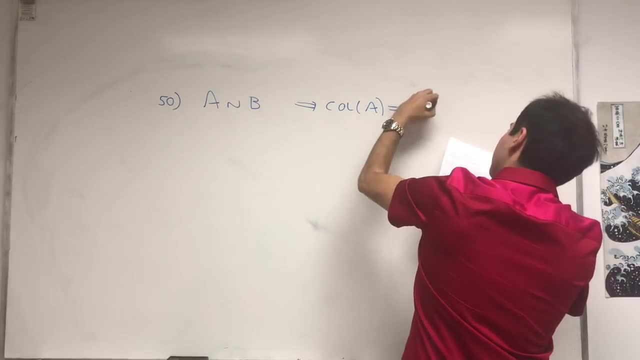 so if a is equivalent to b, then the. so if a is equivalent to b, then the column space of a equals the column column space of a equals the column column space of a equals the column space of b, space of b, space of b. so equivalent means row equivalent. so 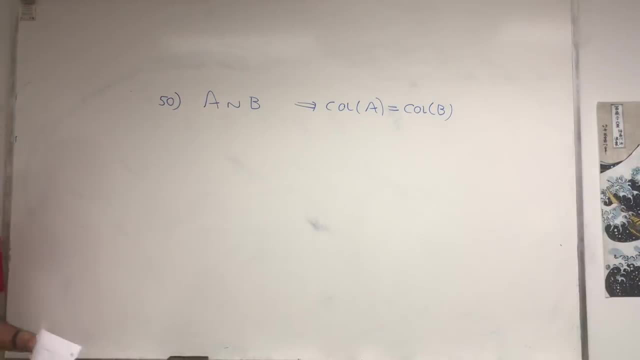 so equivalent means row equivalent. so so equivalent means row equivalent. so, using row operations, if you transform a using row operations, if you transform a using row operations, if you transform a to b, then the column spaces are the same to b, then the column spaces are the same. 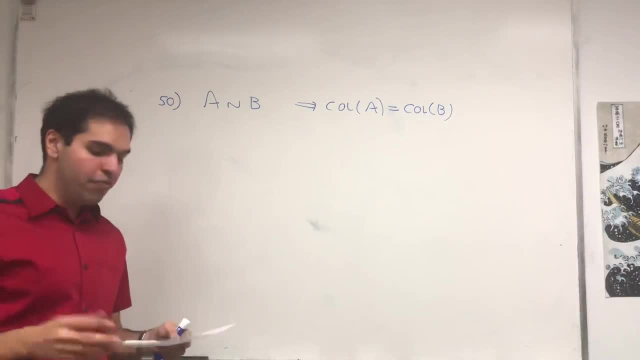 to b, then the column spaces are the same. is that true or not? and is that true or not? and is that true or not? and 50. so language 50 is cindy. 50, so language 50 is cindy. 50, so language 50 is cindy. so almost like hindi, but cindy. and 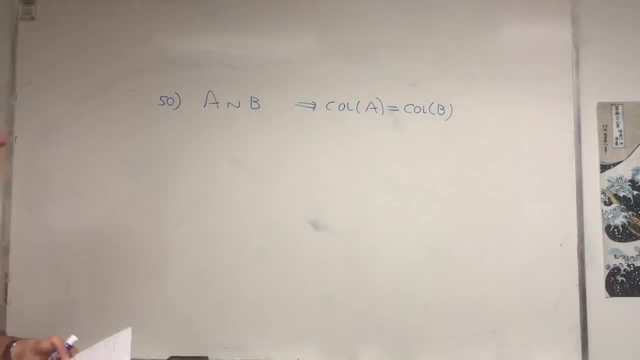 so almost like hindi but cindy. and so almost like hindi but cindy. and 50 is cindy is pajas, 50 is cindy is pajas, 50 is cindy is pajas. i like that it has a nice feel to it. i like that it has a nice feel to it. 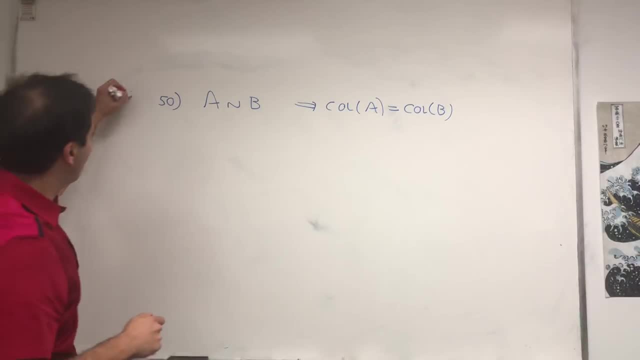 i like that. it has a nice feel to it. okay, and unfortunately, even though row okay, and unfortunately, even though row okay and unfortunately, even though row operations preserve null spaces, operations preserve null spaces. operations preserve null spaces. they do not preserve column spaces for. they do not preserve column spaces for. 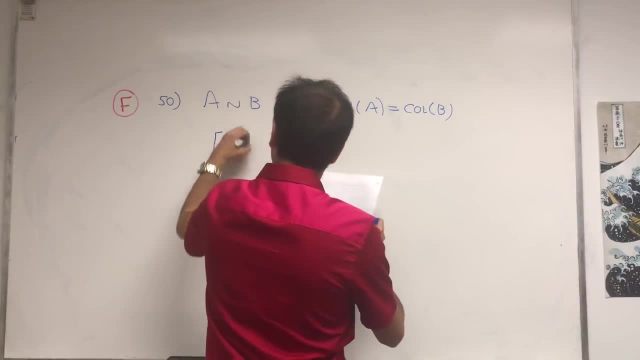 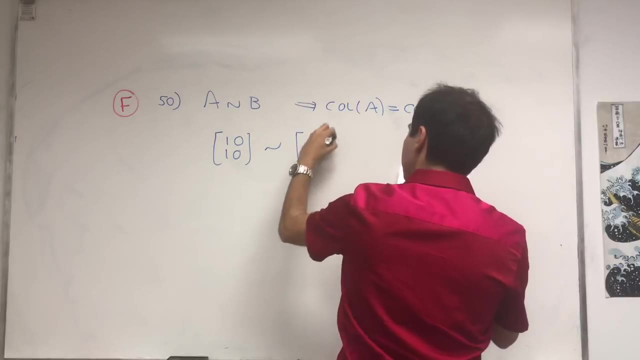 they do not preserve column spaces, for example, example: example: one zero one zero right row. equivalent one zero. one zero right row. equivalent one zero. one zero right row equivalent to to: to so subtract this row from this row, and so subtract this row from this row, and so subtract this row from this row, and we get one zero, zero, zero. 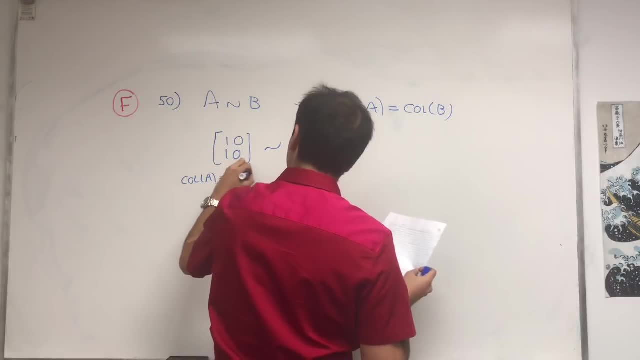 we get one zero, zero, zero. we get one zero, zero, zero. here it's the span of one one. here it's the span of one one. here it's the span of one one: the span of the column. so the span of the span of the column, so the span of. 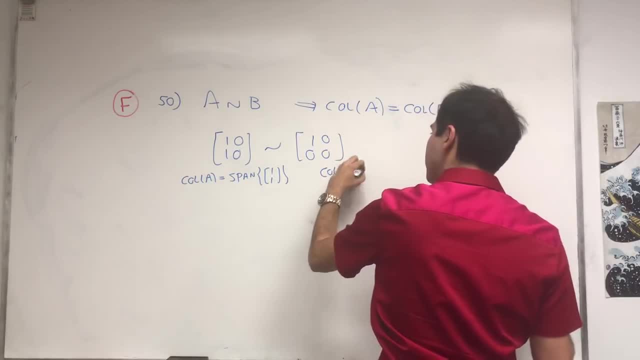 the span of the column, so the span of one one and zero zero. one one and zero zero. one one and zero zero. but here the column space of b it's a, but here the column space of b it's a, but here the column space of b it's a span of. 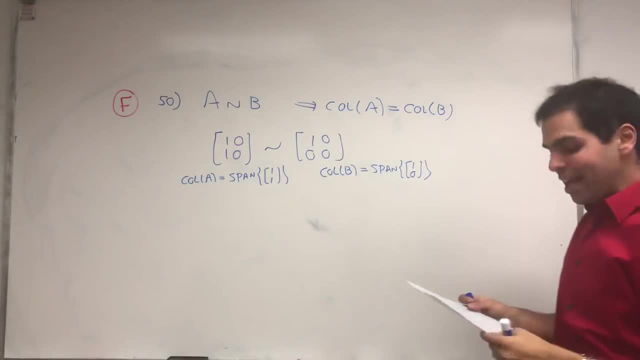 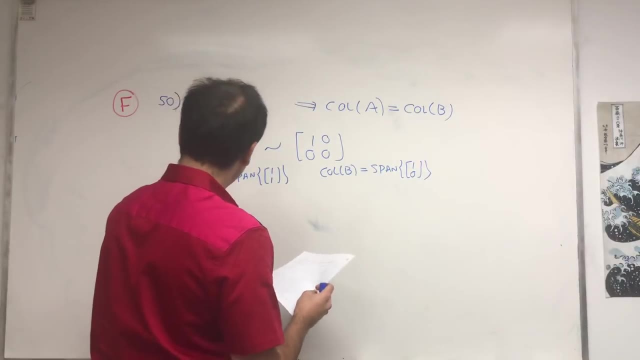 span of span of one zero, one zero, one zero. those two spans are not the same. those two spans are not the same. those two spans are not the same. okay, question 51. okay, question 51. okay, question 51. uh, is the rank of a. uh, is the rank of a. 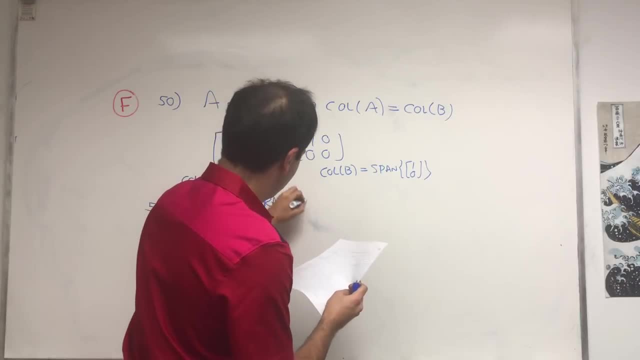 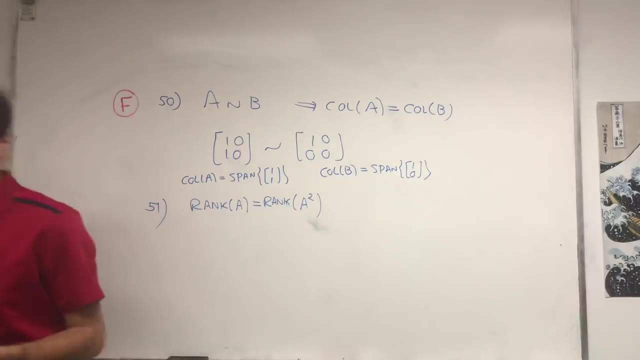 uh is the rank of a the same as the rank of a squared. the rank of a squared. the rank of a squared. and uh 51, so a moroccan dialect. or and uh 51, so a moroccan dialect, or and uh 51, so a moroccan dialect, or arabic. 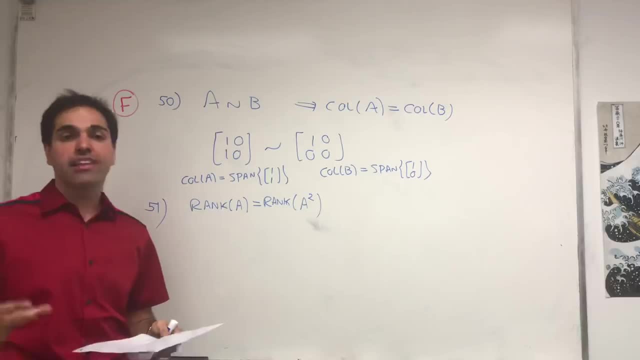 arabic arabic, and at least in arabic 51 is, and at least in arabic 51 is, and at least in arabic 51 is. what so? in other words, if you square a, so in other words, if you square a, so in other words, if you square a matrix. 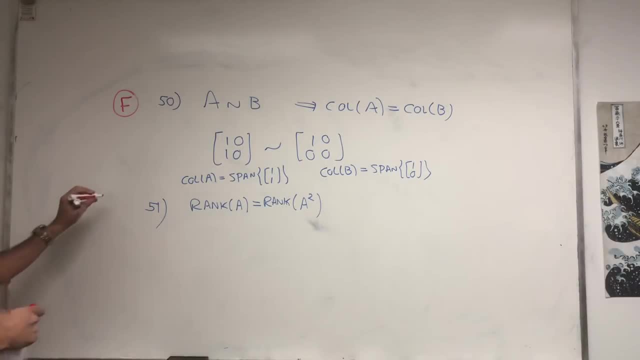 matrix. matrix: is the number of pivots still the same? is the number of pivots still the same? is the number of pivots still the same? and unfortunately, we're back to our and unfortunately, we're back to our and unfortunately, we're back to our false things. 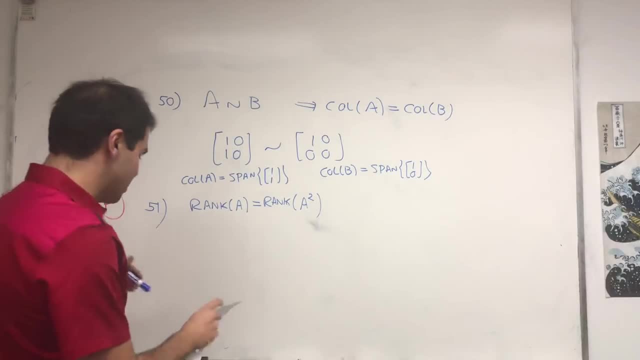 false things, false things. so turns out the rank of a squared. so turns out the rank of a squared. so turns out the rank of a squared is not the rank the same as the rank of a is not the rank the same as the rank of a is not the rank the same as the rank of a, because take a to be the matrix zero. 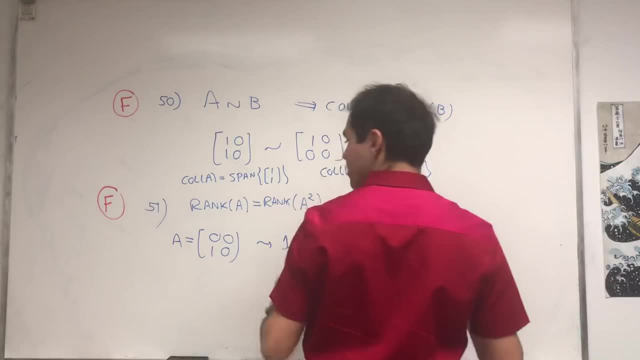 because take a to be the matrix zero. because take a to be the matrix zero, zero, one zero, zero, one zero, zero, one zero. the rank of this is one but a squared. the rank of this is one but a squared. the rank of this is one but a squared. that's zero, zero, one zero. 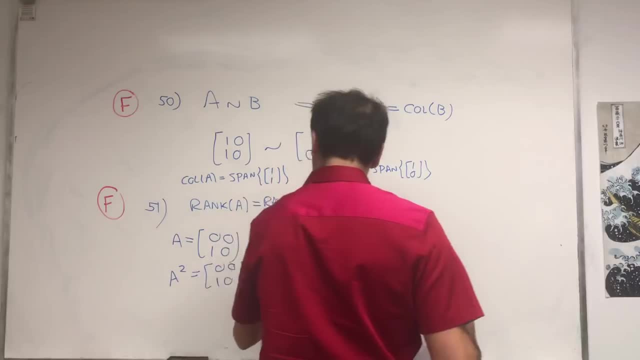 that's zero, zero, one zero. that's zero, zero, one zero, zero, zero, one zero. and if you do that, you zero, zero, one zero, and if you do that you zero, zero, one zero, and if you do that you get zero, get zero, get zero, zero, and then zero, zero, and the rank is: 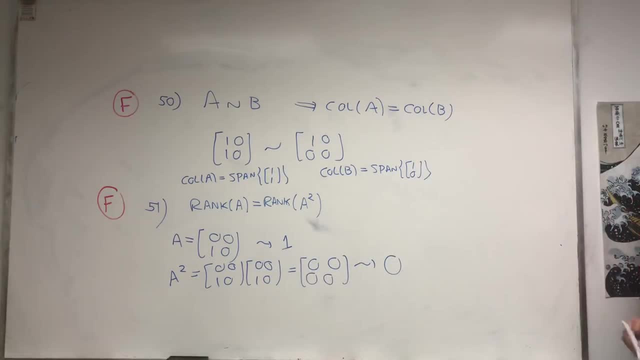 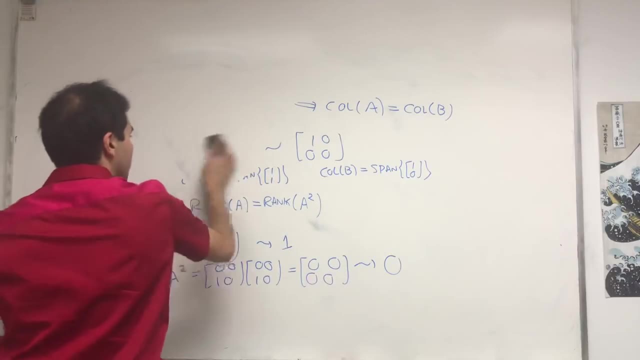 zero, and then zero, zero, and the rank is zero. There are no pivots here, so the rank is not the same. So be careful about this. All right, now let's do some subspaces, some abstract subspaces, So the set of polynomials. 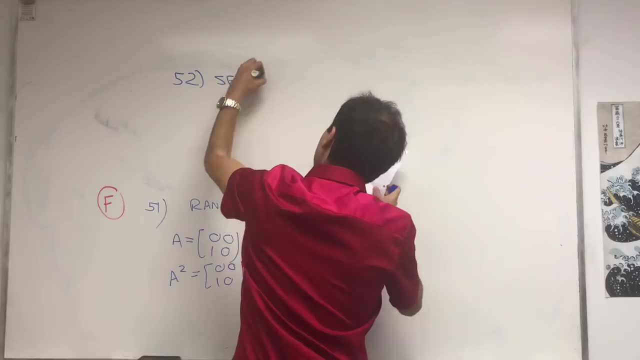 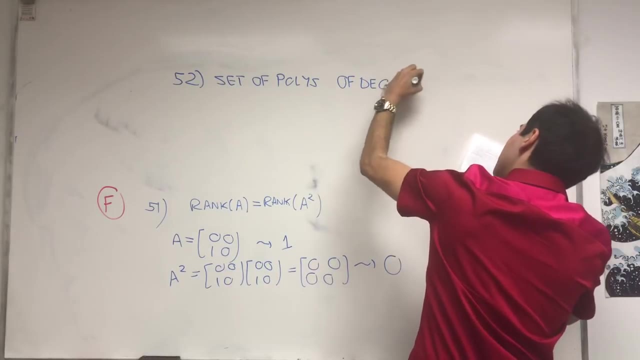 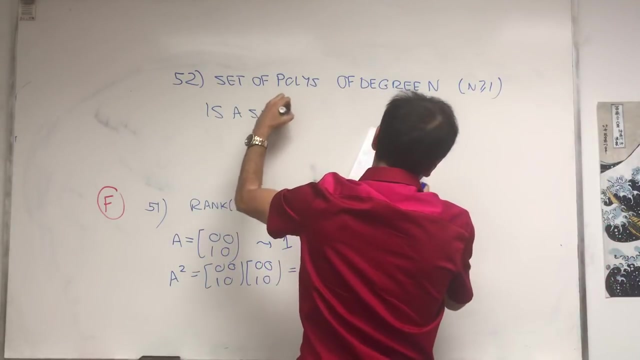 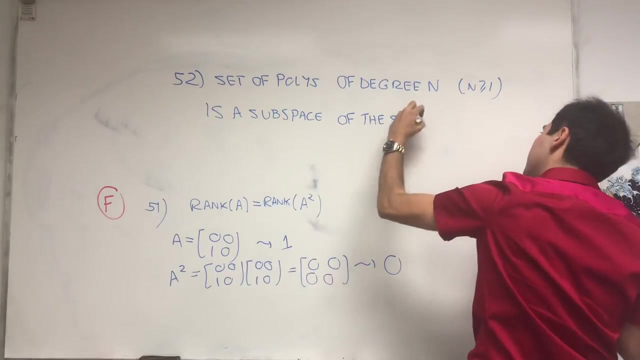 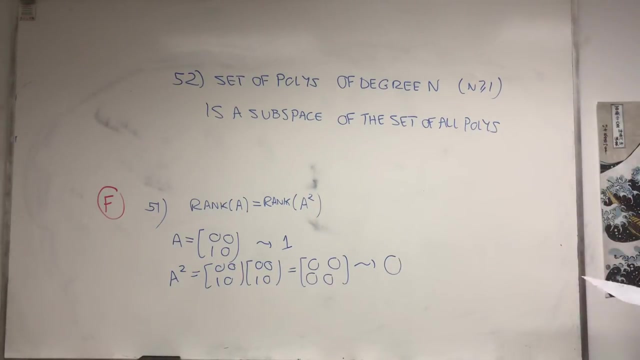 are polynomials of degree. exactly n, And let's say n is greater or equal to 1, is a subspace of the set of polynomials, of all polynomials. Okay and yeah, 52,. another dialect, so the Saudi Arabic dialect of Arabic. 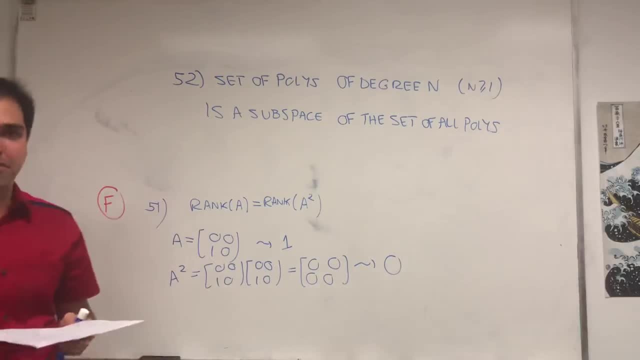 and 52 in Arabic. is I still remember some of that? Okay, the question is again: the set of polynomials of degree exactly n is greater or equal to 1? is a subspace of the set of polynomials of degree exactly n? And let's say n is greater or equal to 1, is a subspace of the set of polynomials of degree- exactly n. And let's say n is greater or equal to 1 is a subspace of the set of polynomials of degree: exactly n. 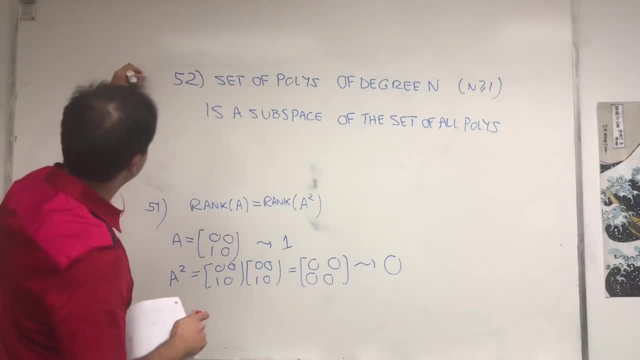 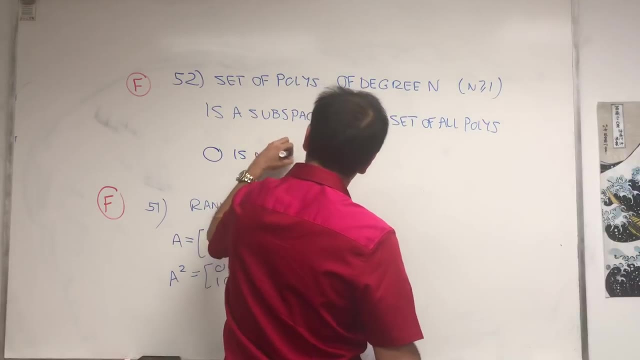 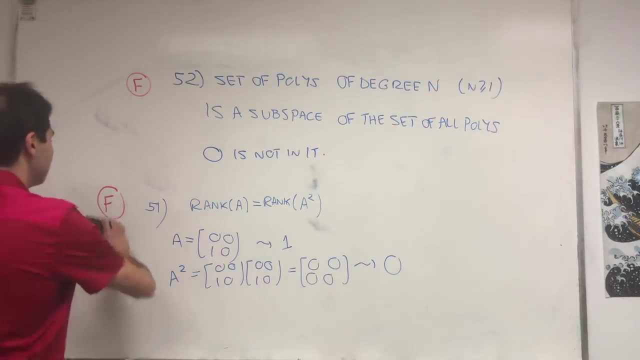 And it turns out it's false, actually for two reasons. First of all, the zero polynomial is not in it. The zero polynomial, I think, has degree minus 1 for some reason, I guess to make some other algebra laws true. 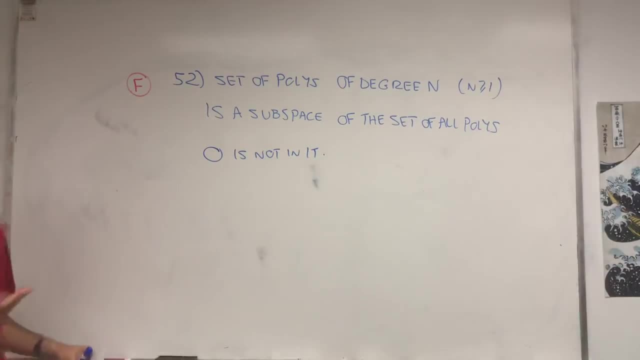 And to make that law, that the degree of f times g is a degree of f plus b, that's the degree of j-th row. So this one does not have degree n for n greater or equal to 1.. And there's another reason. 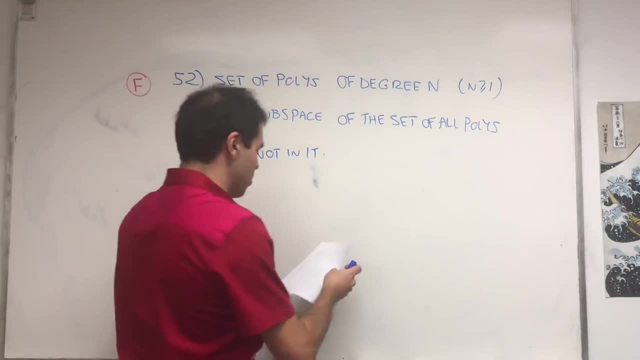 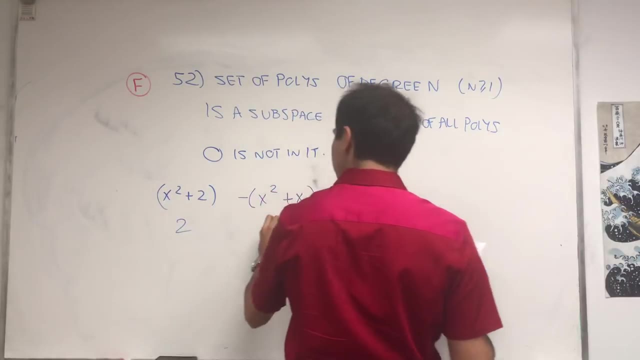 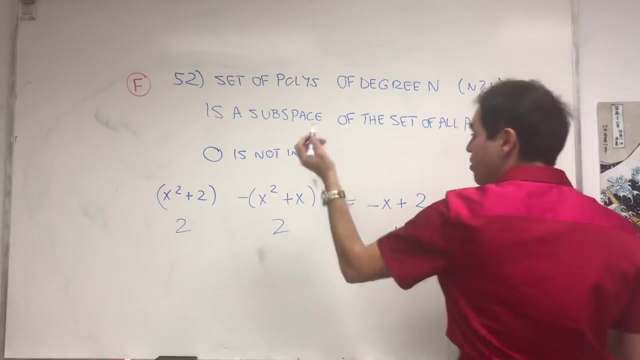 Another reason is it's not closed under addition or scalar multiplication. So if you do x squared plus 2, minus x squared plus x, see this has degree 2, this has degree 2.. But if you subtract it, you get minus x plus 2, and this has degree 1.. 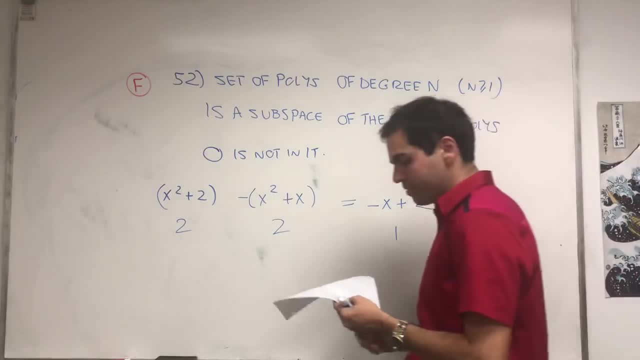 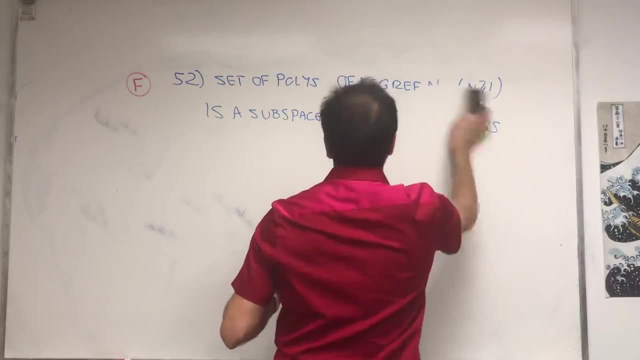 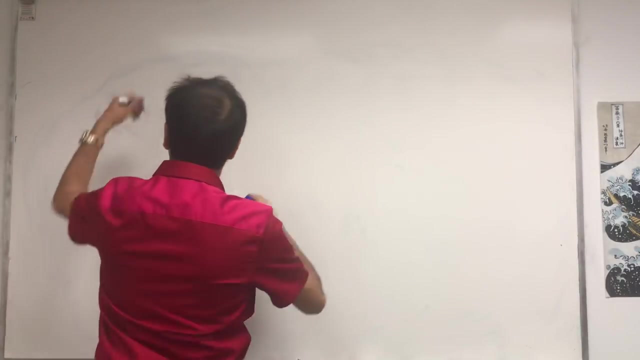 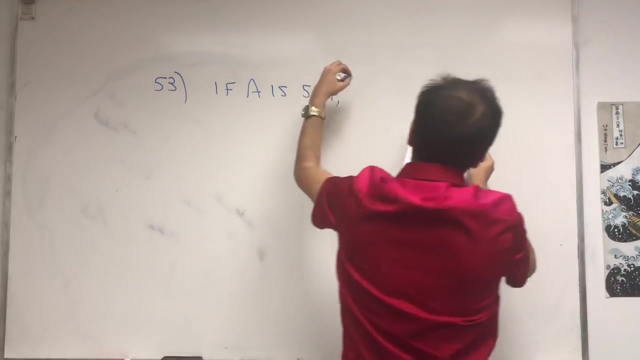 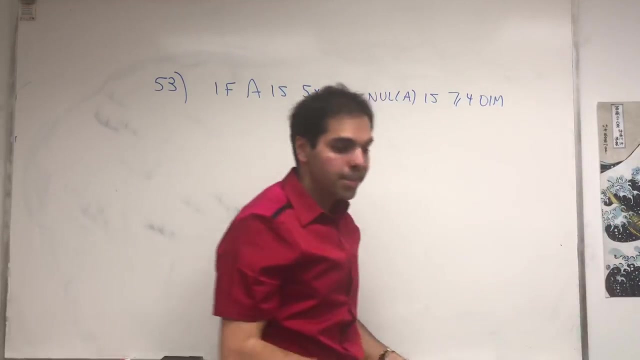 So it's not closed under addition. That's why it doesn't work. OK, good, Question 53.. 53.. So if a is 5 times 9, then the null space of a is at least 4-dimensional. So not saying anything about dimension. 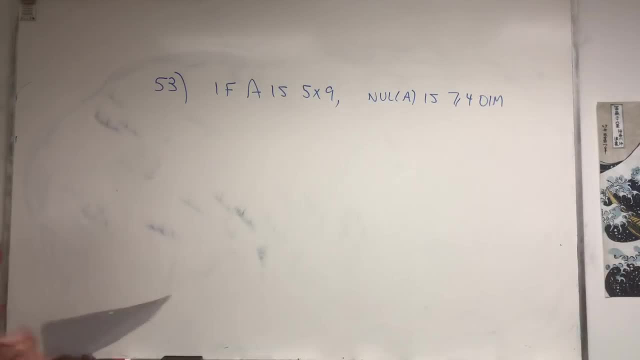 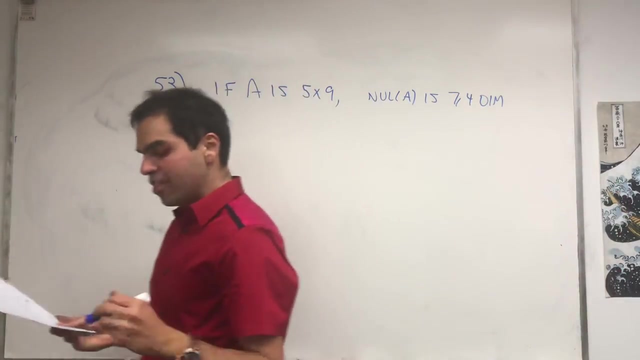 Just that it's 5 by 9.. Just that it's 5 by 9, is it true that basically it has at least 4 free variables And 53rd language is the northern dialect of Uzbekistan And 53 is? 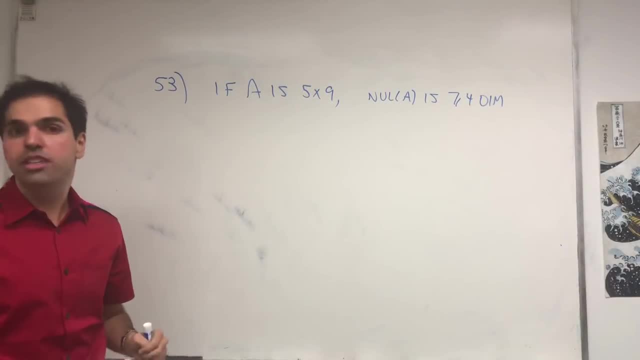 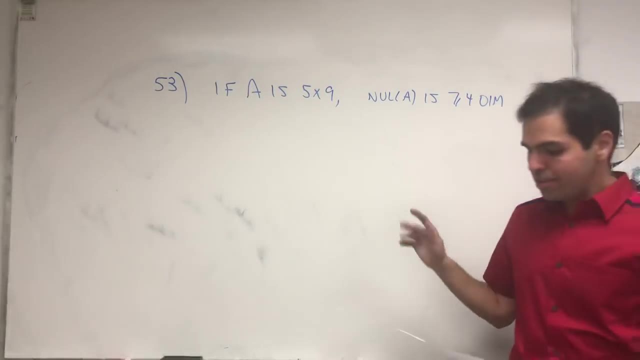 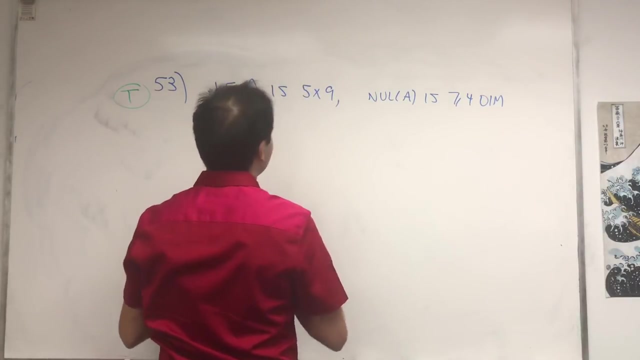 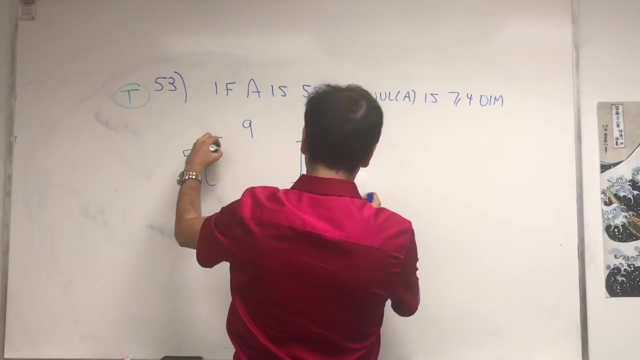 And I think it's similar to Turkish. I know is 3 in Turkish, So is 53. And let's see Turns out this is true. So we've broken our false script again, Because if you have a 5 by 9 matrix, so 5 and 9, well, it has at most 5 pivots. 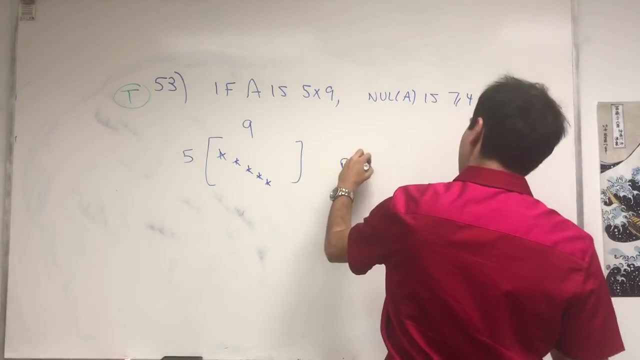 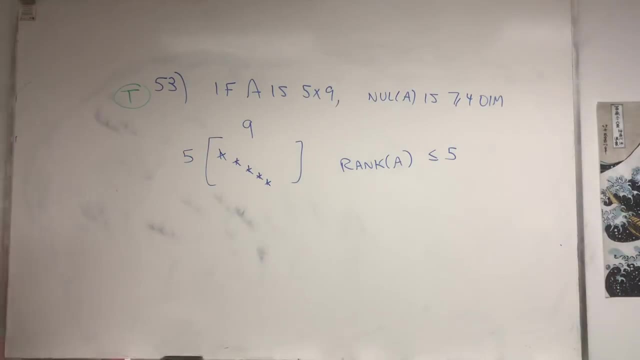 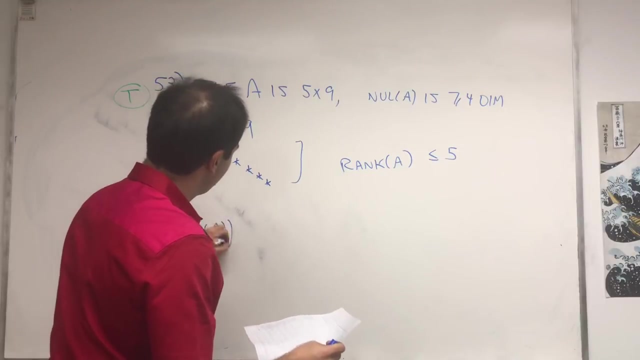 So, best case scenario, it has 5 pivots, So the rank is at most 5. And we want to relate the rank with the null space, So let's use it Rank nullity theorem. So the dimension of the null space of a is the number of columns. 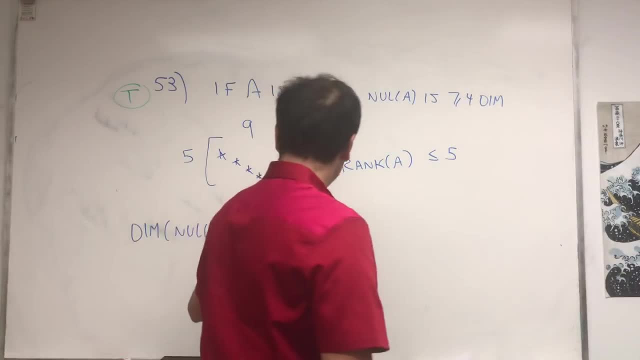 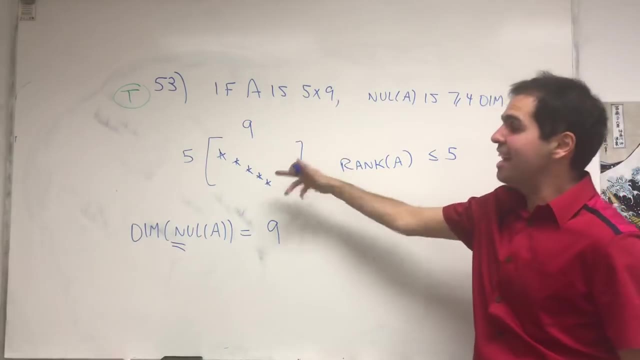 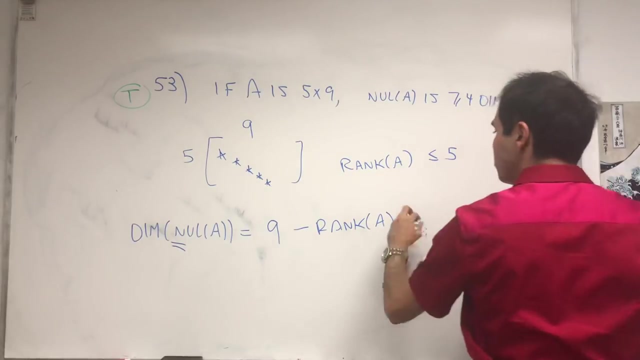 So careful. not the number of rows, So 9.. And again, rank nullity. just remember n as null space. So it's n minus whatever, So 9 minus rank of a. And because we're doing minus, we're flipping this. 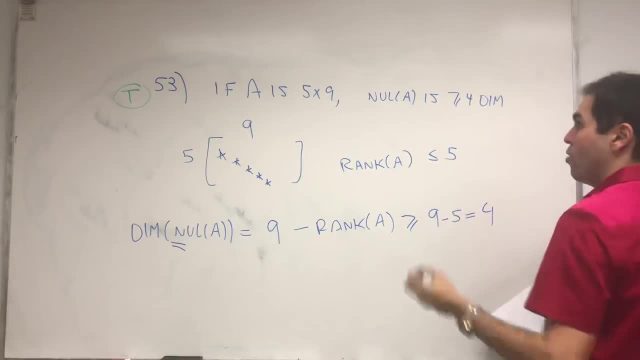 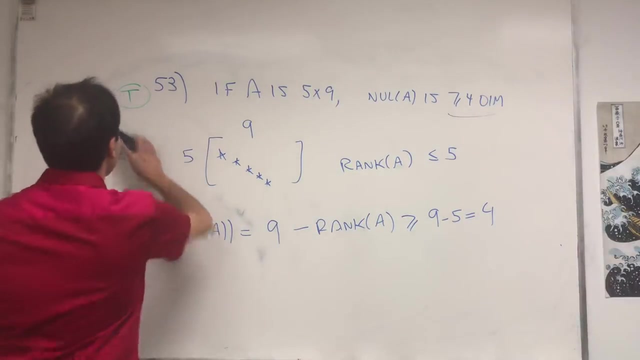 So greater or equal to 9 minus 5,, which is 4.. That's exactly what we wanted. We wanted that it's at least four dimensional. All right, good, And now some more abstract things. So question 54.. 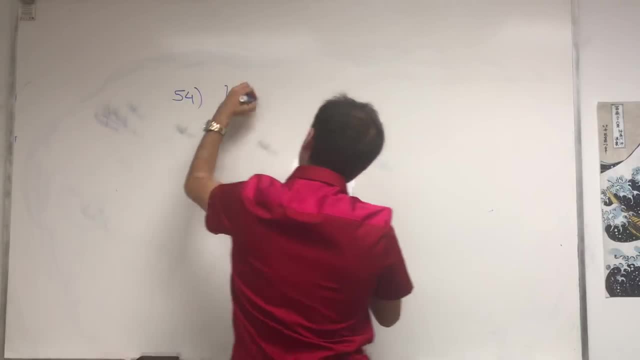 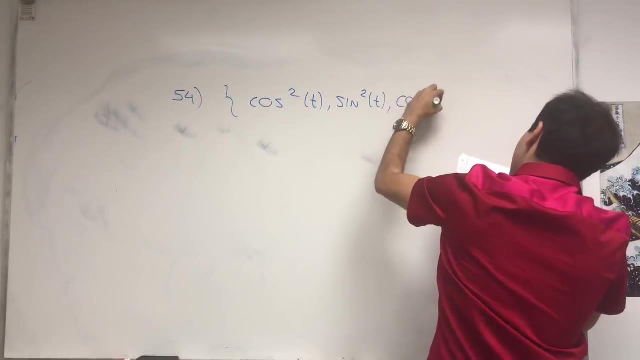 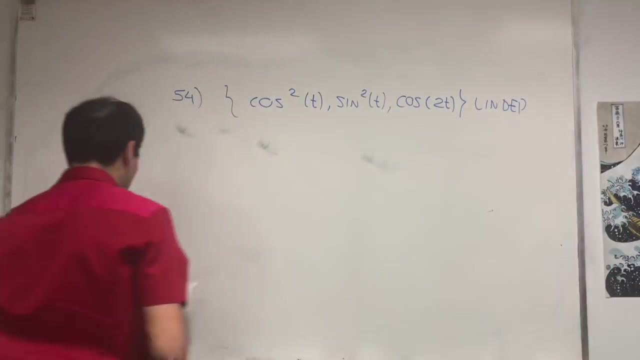 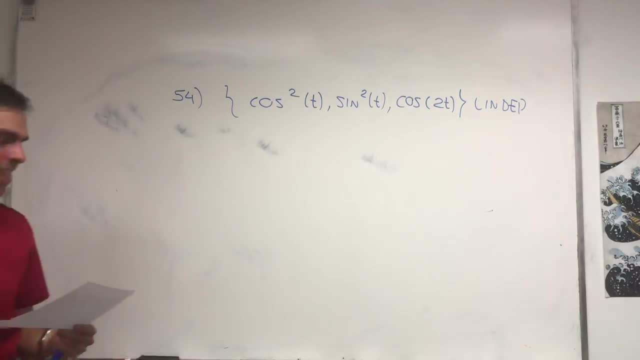 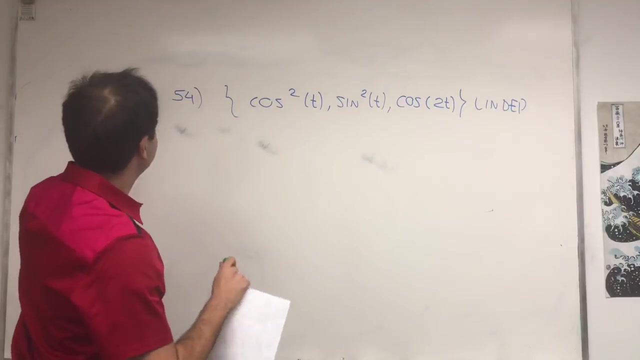 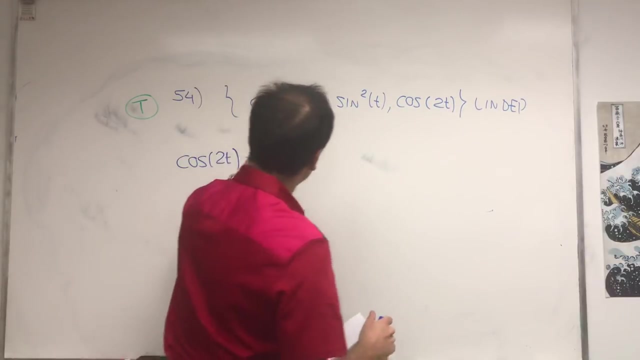 True or false? And 54 is Malay, So 54 Malay is lima pulu enam. In other words, is there a relationship between those three abstract vectors? And you bet there is, because, remember, cosine of 2t is just cosine squared of t minus sine. 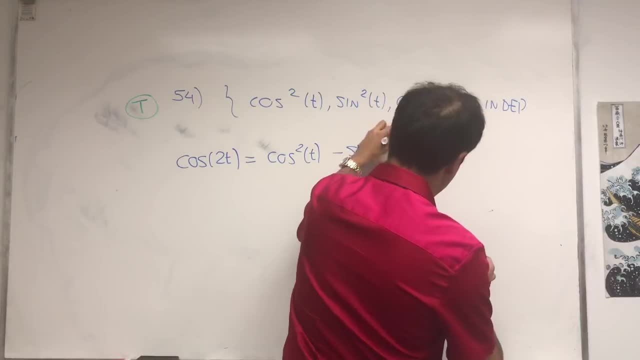 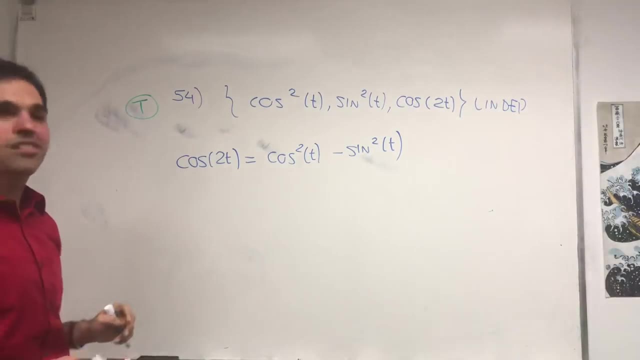 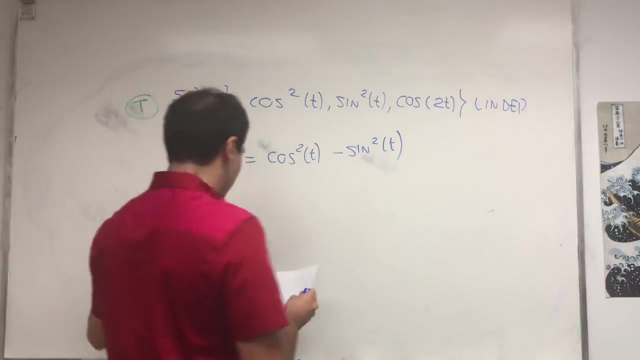 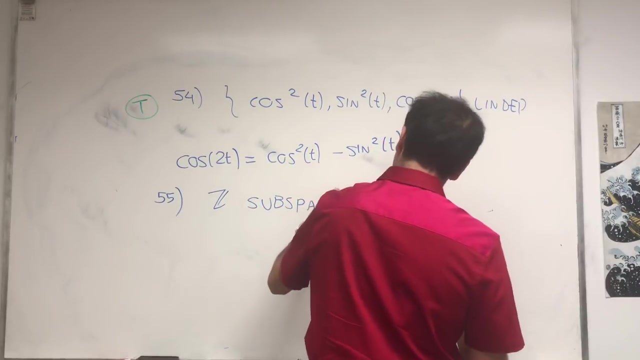 squared of t. So it is true that there's a relation between those three vectors and therefore it's linearly dependent. So linear independent means there's no relationship between the two. OK, Next question: Is the set of integers a subspace of the real numbers? 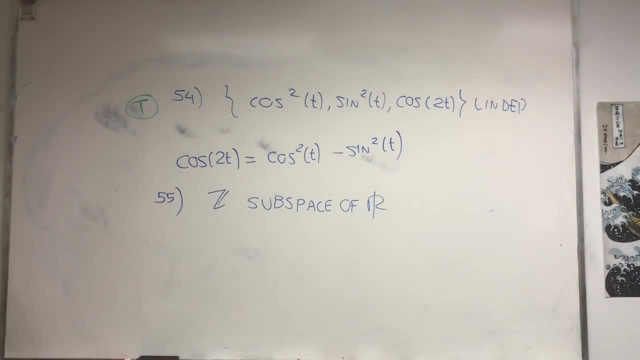 So interestingly it is closed under addition and the zero vector is in it. But the question is: is it a subspace? And language? 55 is Amharic and 55 in that language is Hamisa Amisiti. 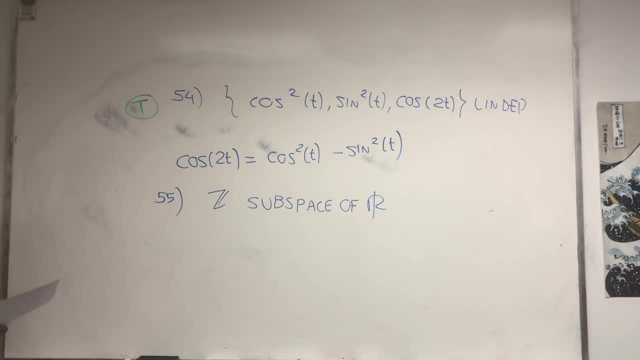 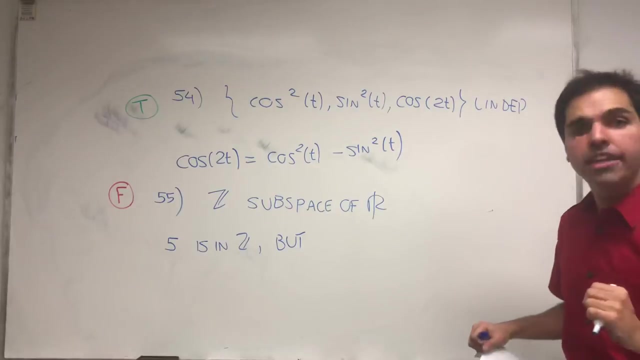 And how it turns out. it's false because even though the zero vector is in it and it's closed under addition, it's not closed under scalar multiplication because, for example, 5 is in z, it's an integer. but remember multiplying. you can multiply by any number. 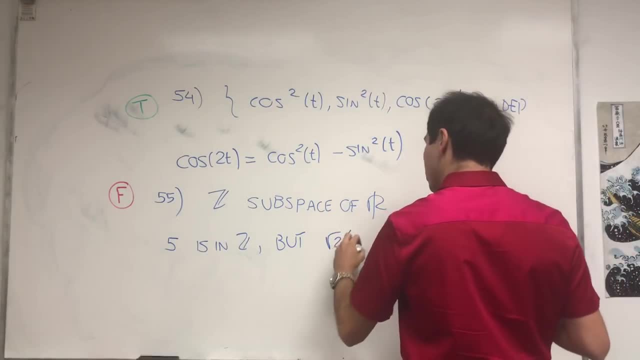 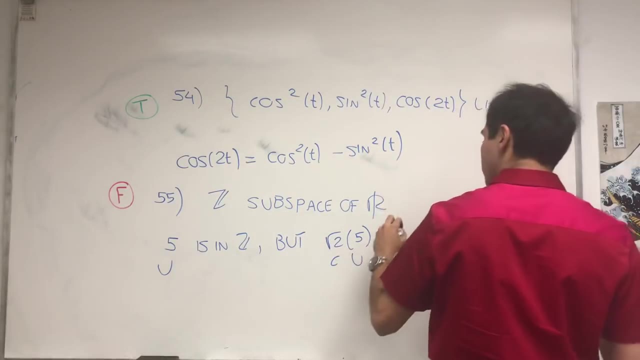 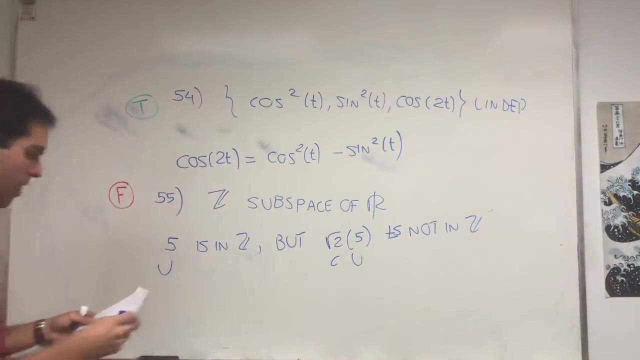 you want, at least in this case, real numbers. So square root of 2 times 5,. so if this is u, this is cu. that's not in r, it's not in z, So it's not a subspace. 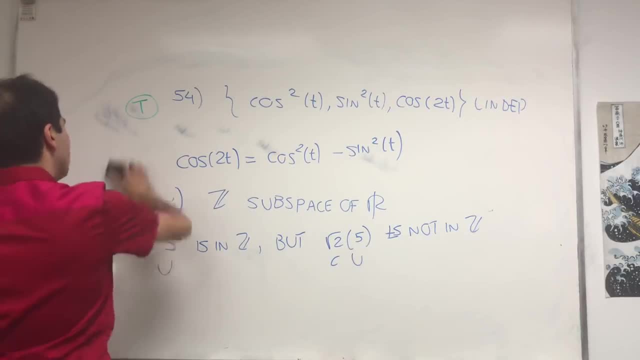 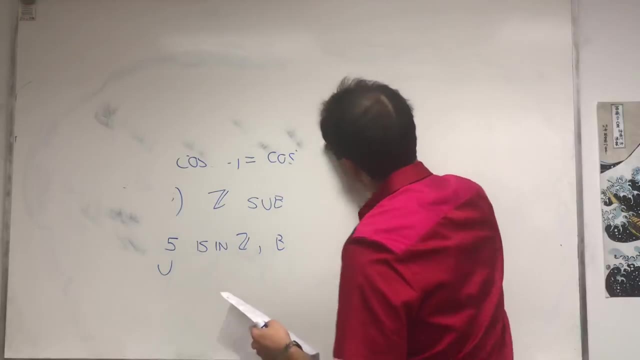 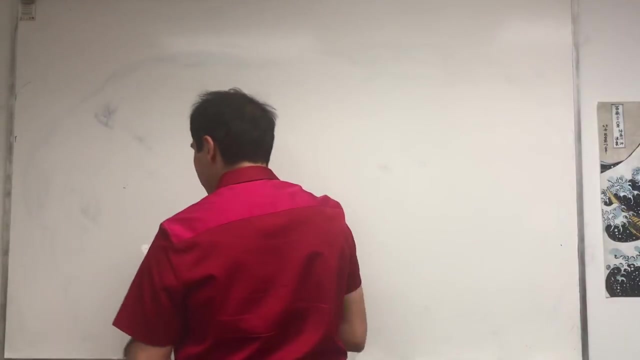 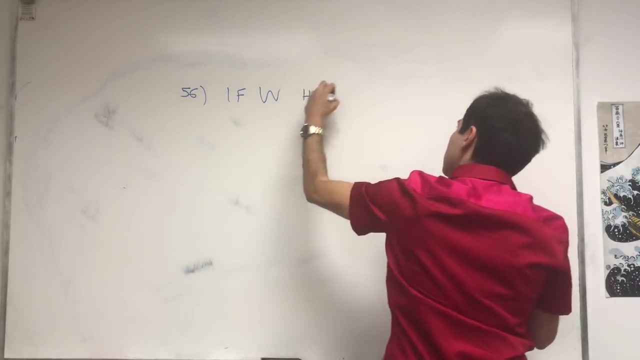 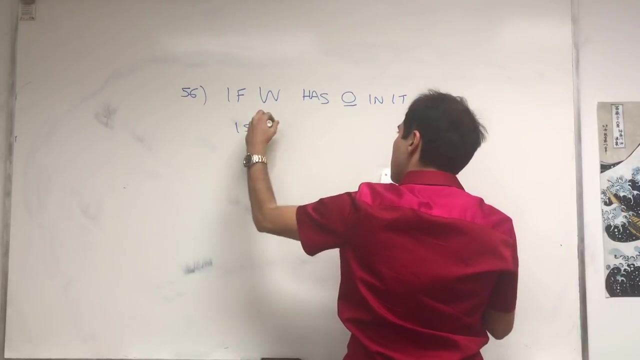 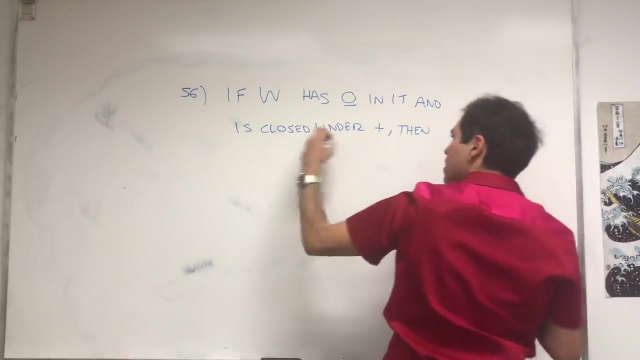 OK, So let's deal more with subspaces. So I want to show you the next three examples that the three properties of subspaces are absolutely essential. So question 56. If w has zero in it and is closed under addition, then w is a subspace. 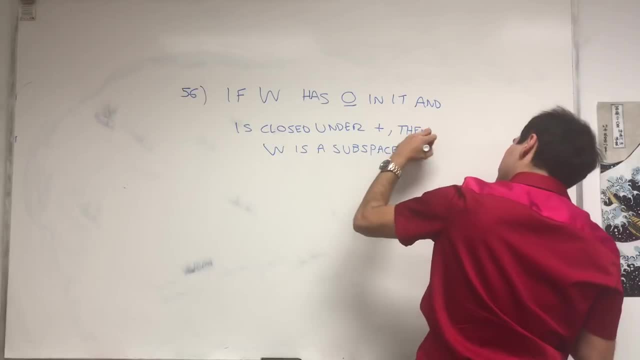 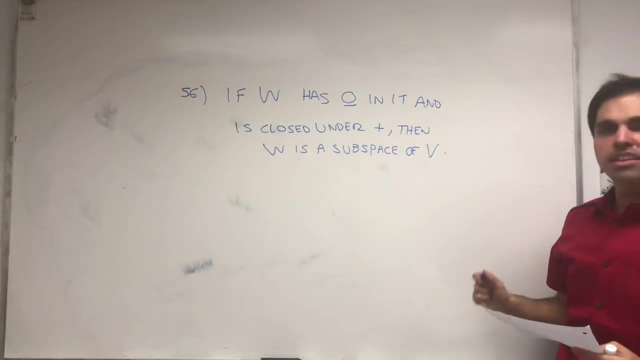 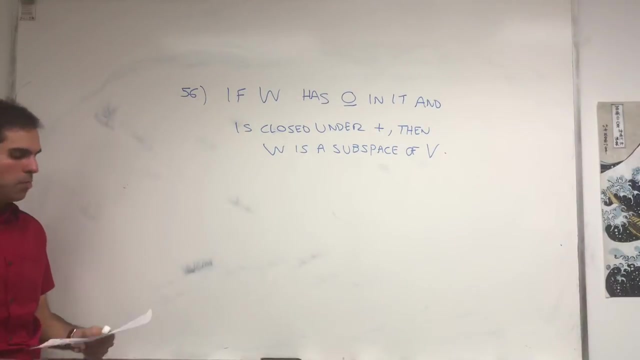 Let's say of b. So suppose w is a subset of v that has the zero vector of v in it and is closed under addition. Is it a subspace? In other words, do we need the third property that is closed under scalar multiplication? 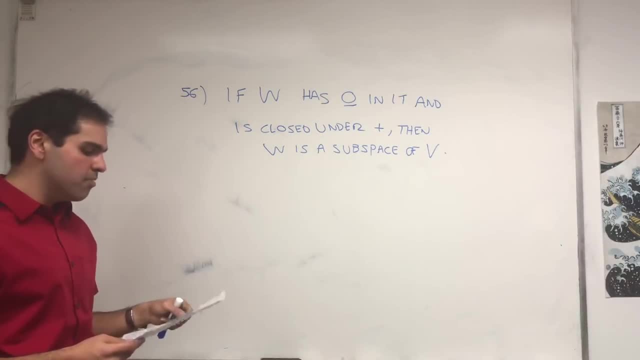 And 56, so Indonesian, and apparently I may have made a mistake, but I found 56 is lima pulu enam, which is surprising Too similar to 54. So I may have written it in a wrong way. 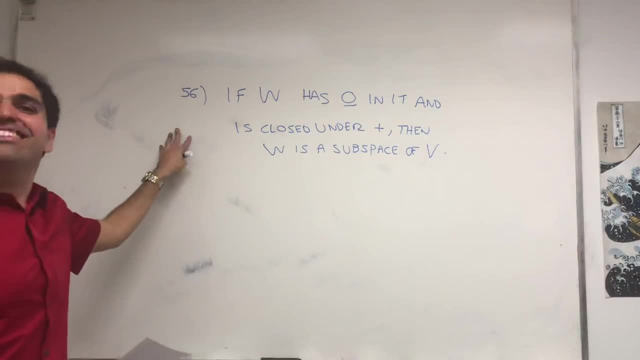 All right, So is that true? And, by the way, this is the halfway mark, So after that let's see. So far we did two hours and 20 minutes. Can I finish it under five hours? We'll see. 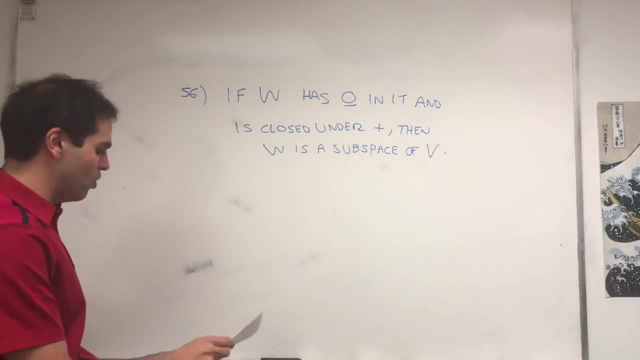 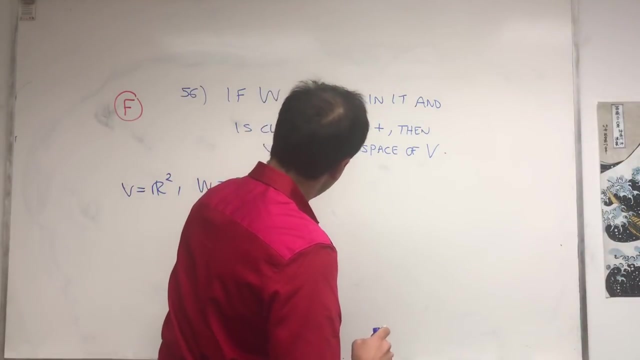 I'm dying already, And it turns out this is false, And let me give an example. So let v be r2, and w be the first quadrant. By the way, there's a video expanding on that. So this is this. 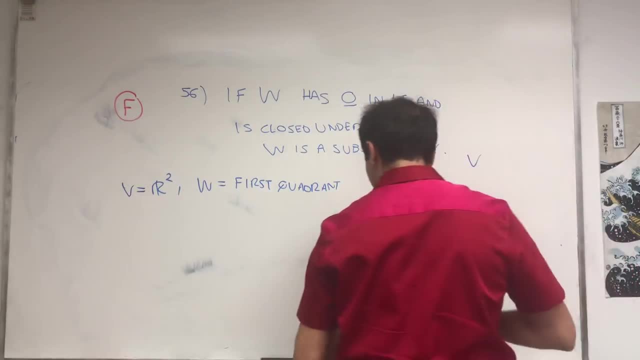 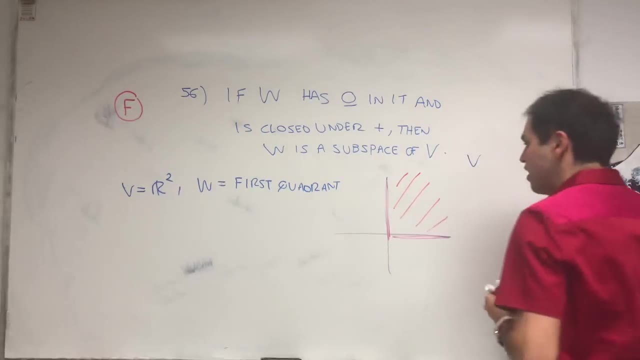 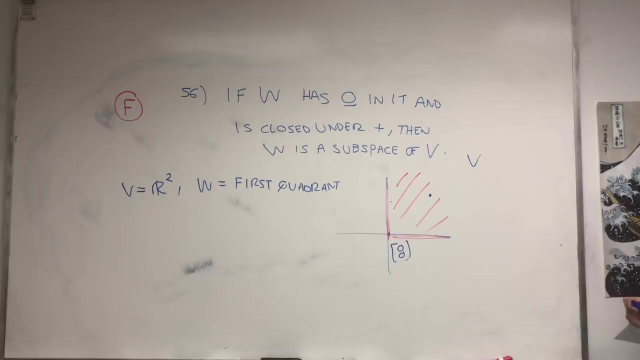 So v is r2, and w is just the first quadrant here over here, including the axes. Then indeed, you see, the zero vector of v is in w, And if you take two vectors here and you add them, you still get a vector in w. 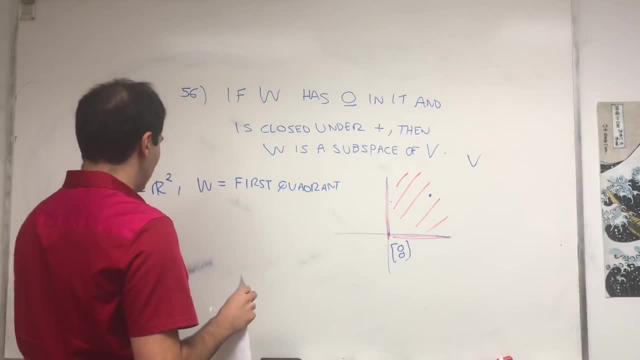 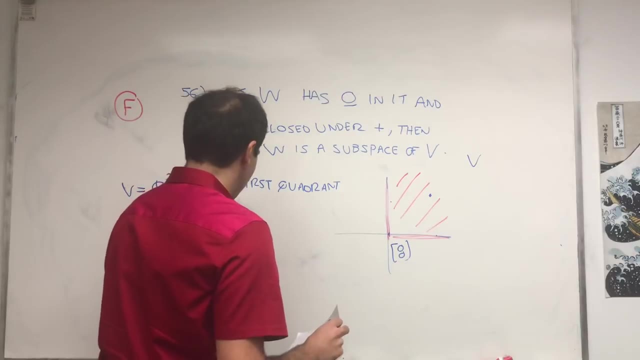 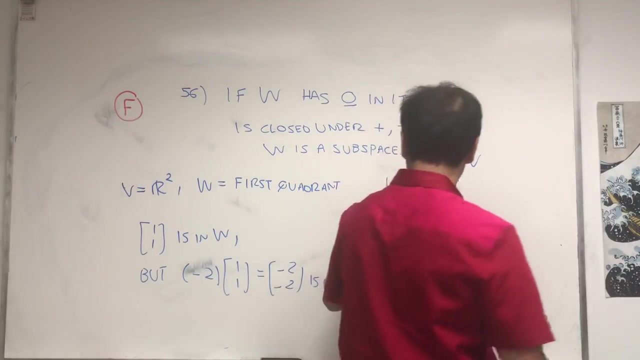 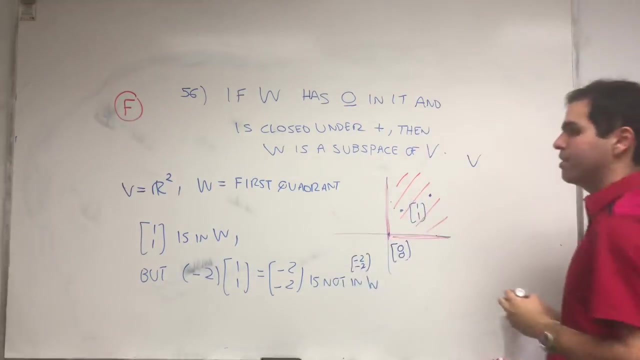 But it's not close under addition Because, for example, one one is in w but let's say minus two times one one, which is minus two, minus two is not in w. Otherwise, if you take this vector here and you scale it in the opposite direction to get minus 2, minus 2, it. 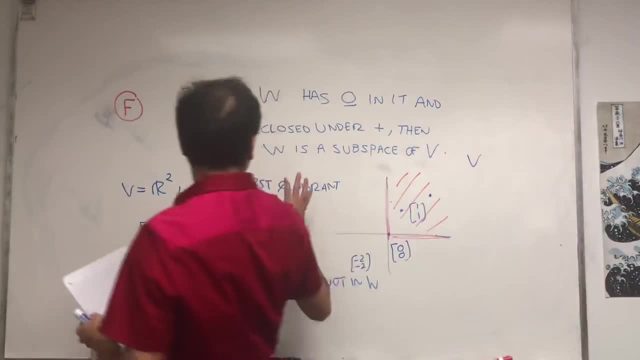 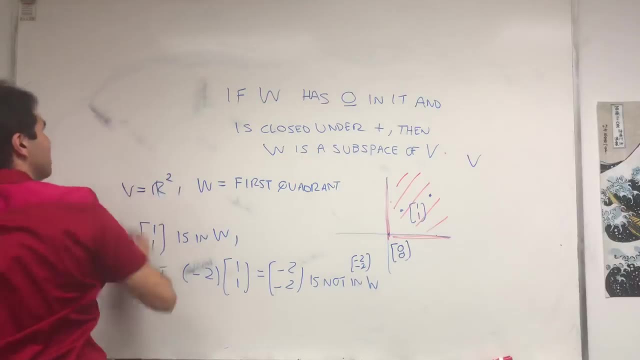 escapes from the subspace. so in other words, the scalar multiplication part is essential to this problem. okay, and of course you may have guessed what about the other ones? so this time let's do the same thing, but instead of plus. the only thing I'm changing is scalar multiplication. 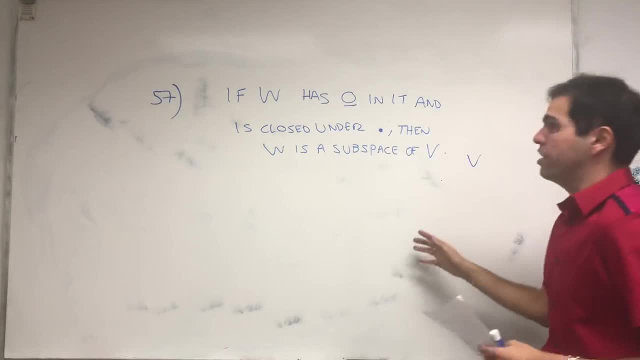 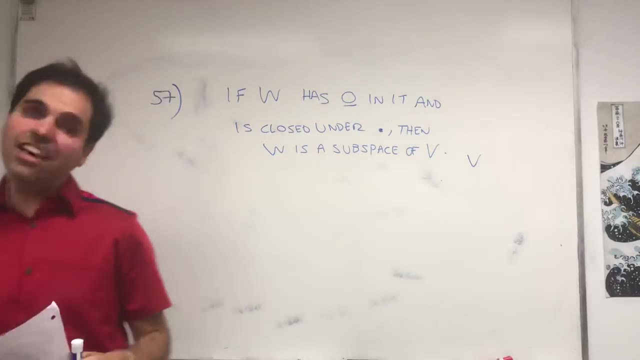 in other words, if you have a subset that has a zero vector and it's closed under scalar multiplication, is it a subspace? in other words, is the closed under addition essential or not? and 57th language, ikbo. and 57 ikbo is iri ise asa. 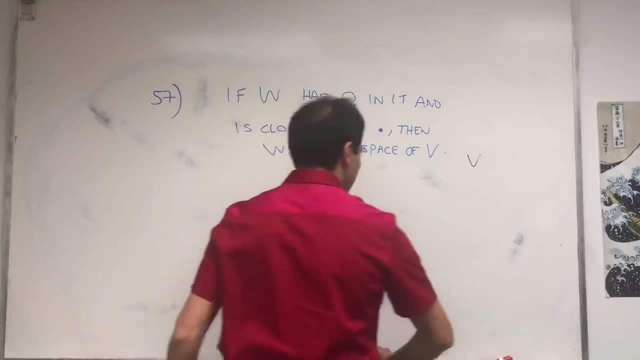 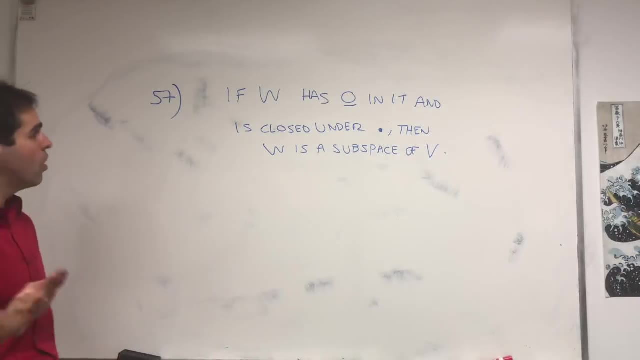 I'm not making those up. I know you're like maybe he just says gibberish, but no, no, I looked that up and it actually took me- like I'm not kidding, it took me two hours to figure out all those languages. so that's good anyway. so of course you may have guessed, the three properties are essential. so 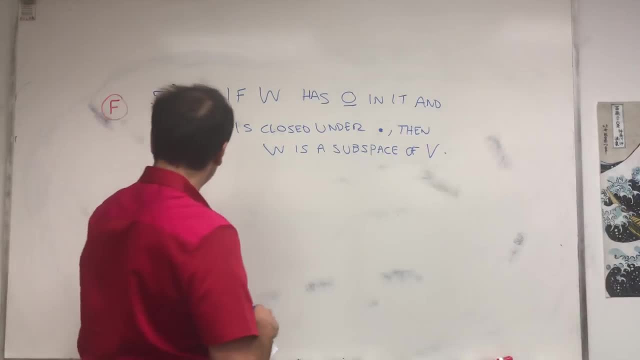 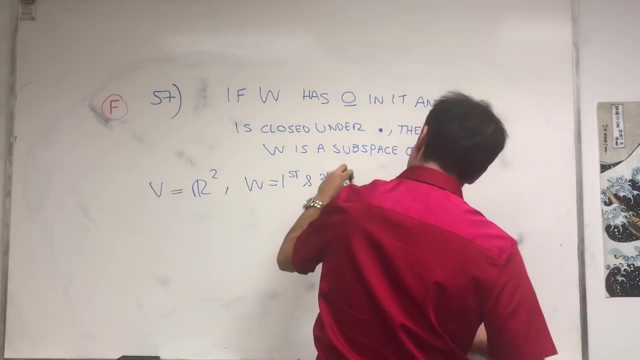 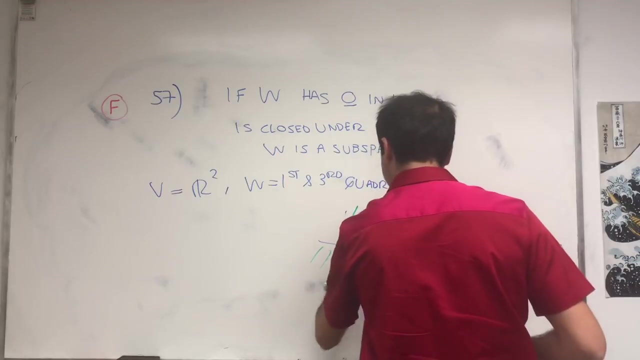 this is still false and very similar counter example: V is R2 and W is the first and third quadrant, and then W is just this one, and this one together with the axis. of course you can check that the zero vector is in it, that's not a problem. 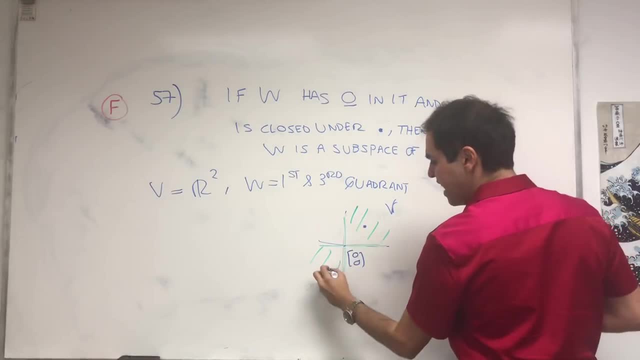 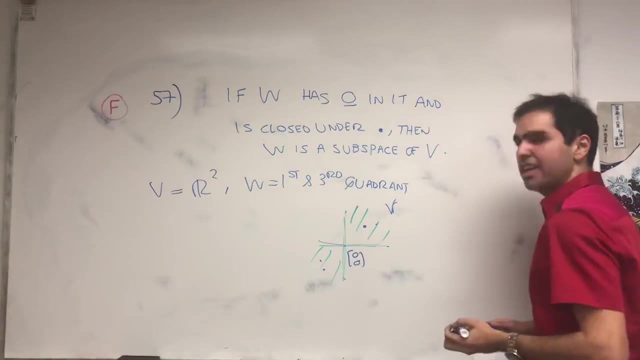 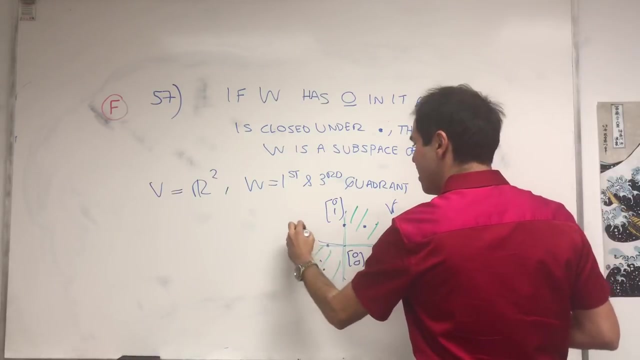 and also, if you have a vector here, you scale it, you still get a vector in W. and similarly, if you have a vector here and you scale it, you still get a vector in W. that said, it's not closer, in addition, because 0, 1 is in it and a minus 1, 0 is in it, but if you add them, 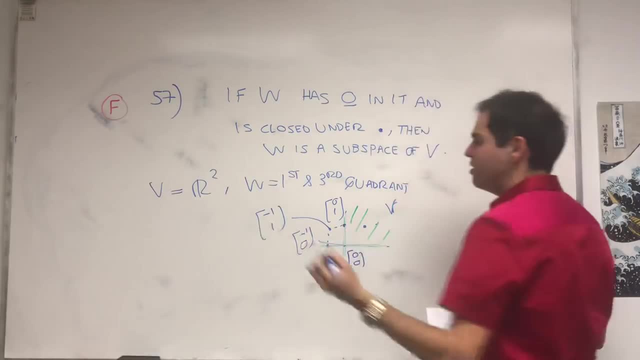 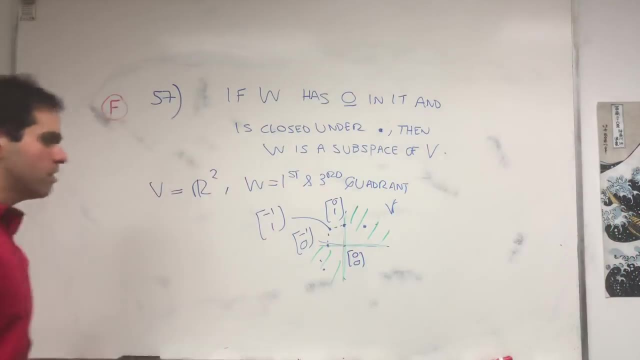 you get the vector minus 1, 1, which is not in that space anymore, so it escapes, and that's what we needed. that you know. let's call that having the axes- I'm not doing this for some reason, but it's for the axes. and yeah, in fact you could have. 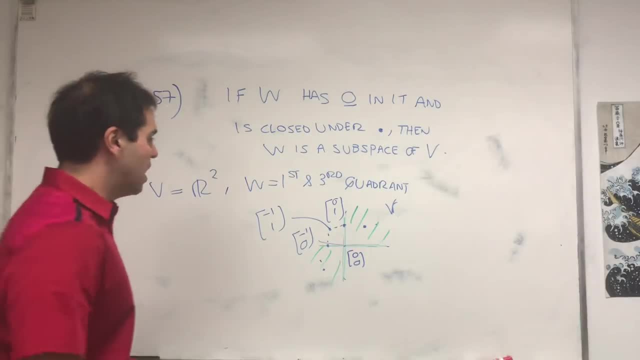 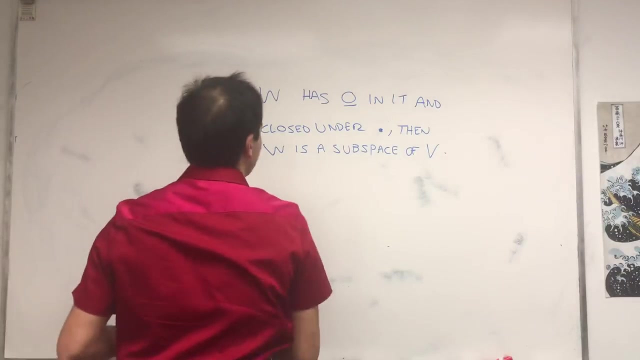 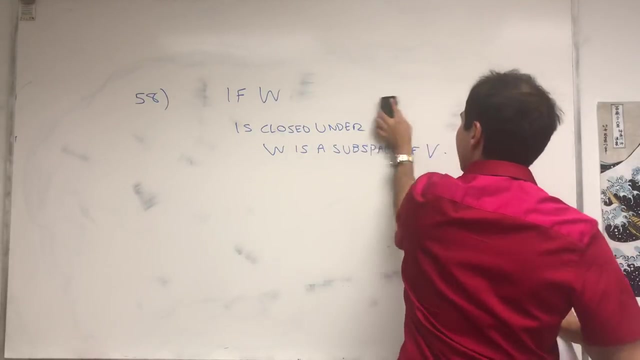 just chosen the X and Y axis. that would also have worked, so so that's good. in other words, those close under a scalar. it's a close under addition is essential, and you may have guessed the next question. you may have guessed the next question is if W is closed under addition and 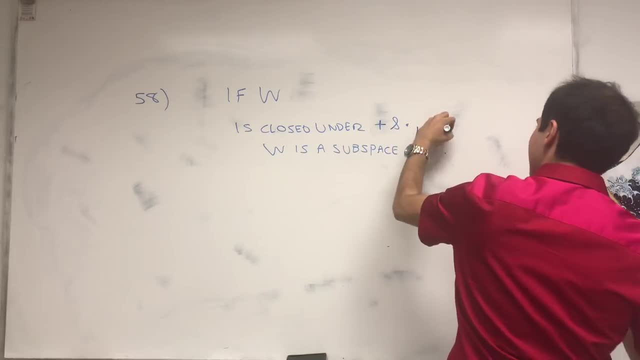 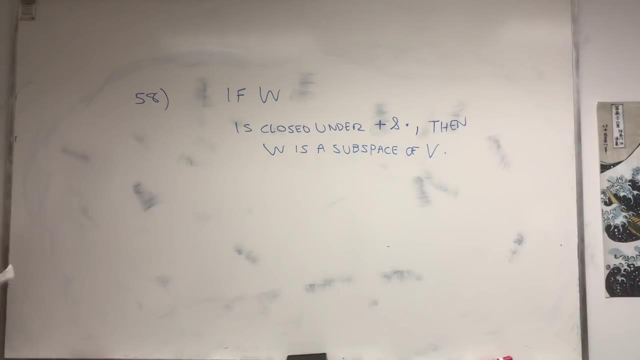 scalar multiplication, then W is a subspace of B. this one's kind of interesting. so 58 tagalog, so tagalong, I guess almost, and it's limanpun, limanpun valon, I think it's Filipino right, something like that. so this one is interesting. so it is false, and because 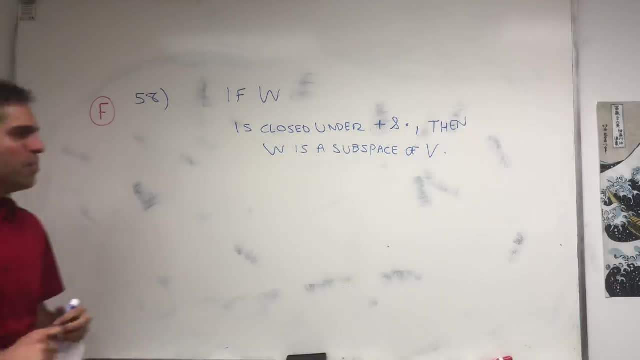 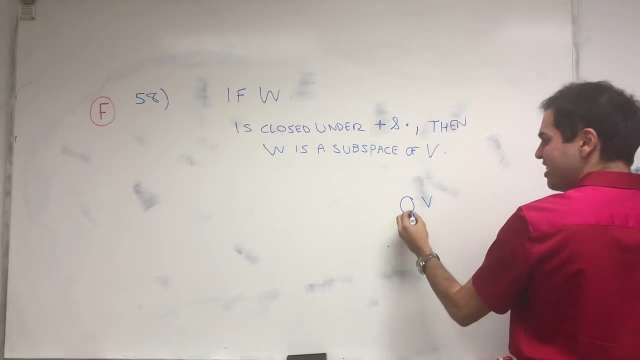 all we need to show is that the zero vector is not in it. but here's the thing: if there's an element in w, let's say an element V, if it's closed under addition, that was going to multiplication- it means zero v is in it and therefore the 0 vector is in it. So really the only obstruction to 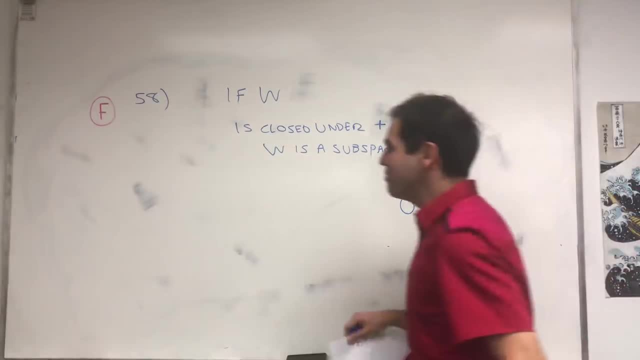 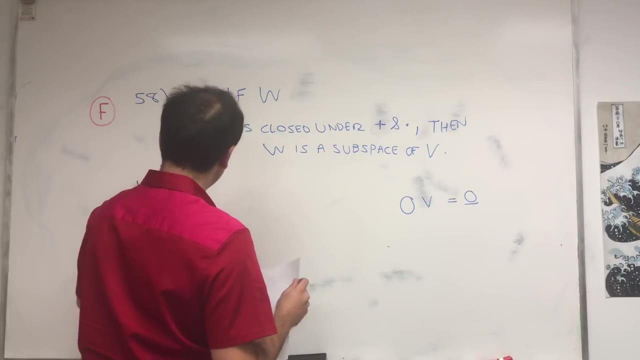 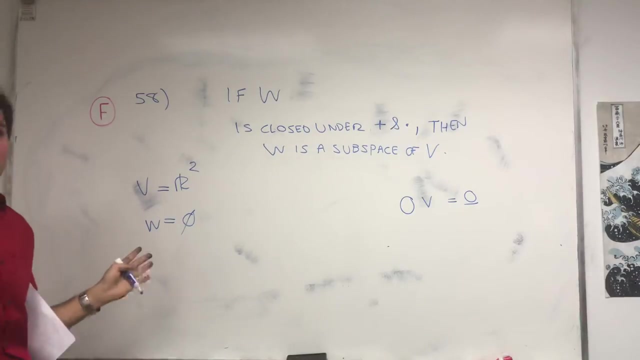 this is if w has no elements. So basically, let v really be anything, but let's say r too and w be the empty set. You see, this is what's called vacuously true. So it is true that if you had elements u and v, then u plus v. 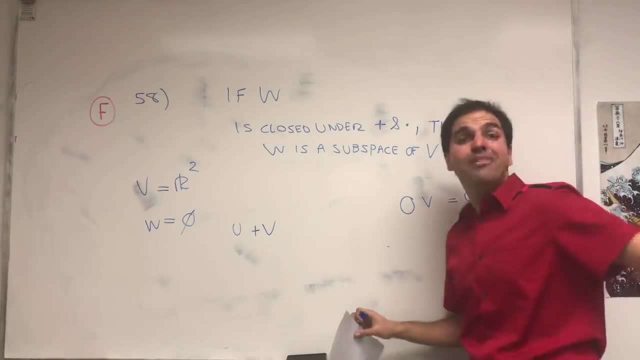 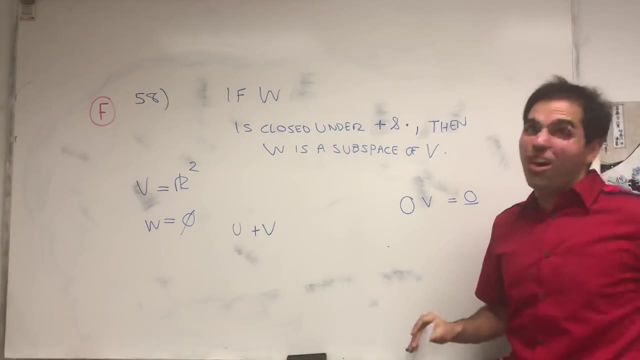 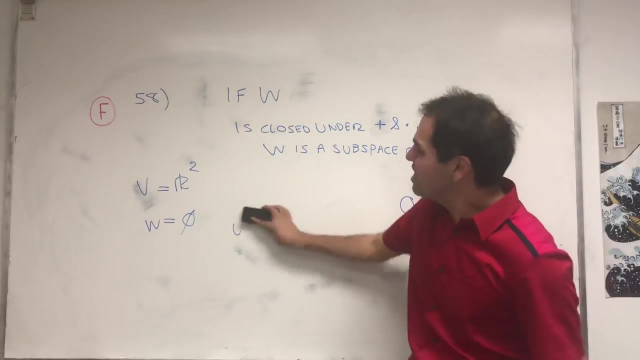 would be in it because there are no elements. In other words, it's not false that if u and v are in it, then u plus v is in it. And also it's not false that if c is a number and u is a vector, then c- u is in it. So trivially it's closed under. 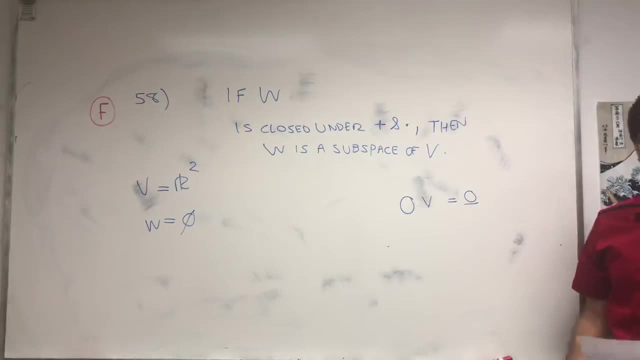 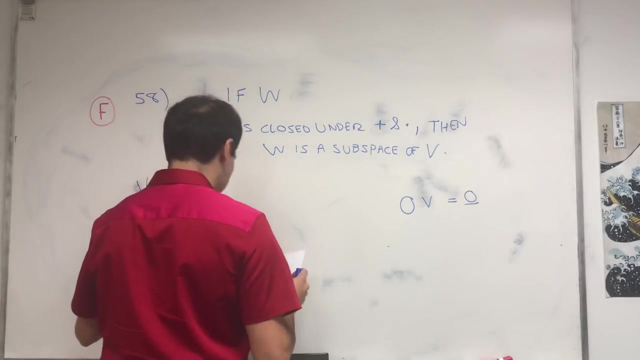 scalar multiplication. Subtitles by the Amaraorg community addition. But the 0 vector is not in it because nothing is in it. That's kind of a brain teaser. So 0 is not in w. So in math we really take the approach of if. 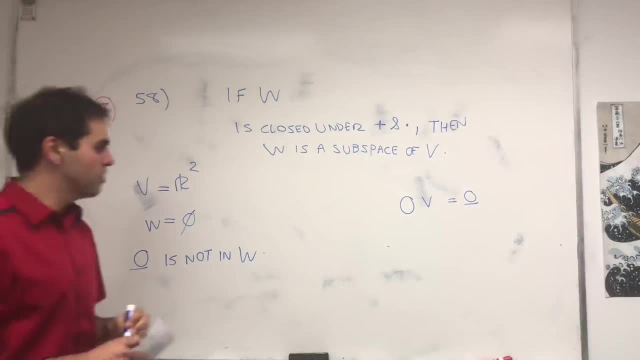 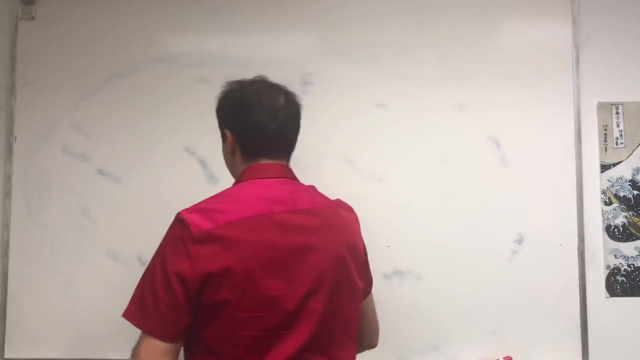 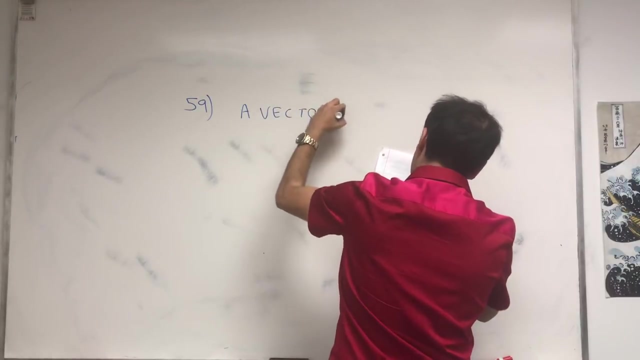 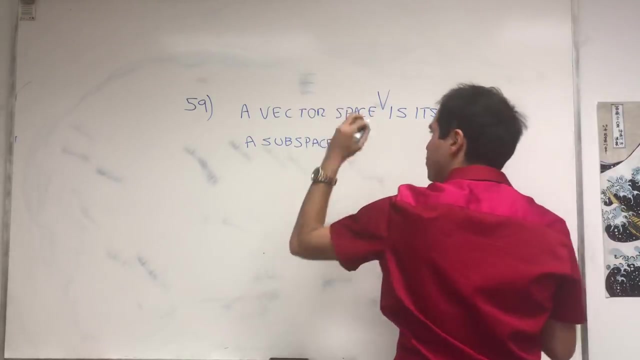 it's not false. it must be true More like a promise, not something that actually happens. Okay, question 59.. A vector space is itself a subspace, So a vector space v is itself a subspace of something else, of another space, of a vector space. 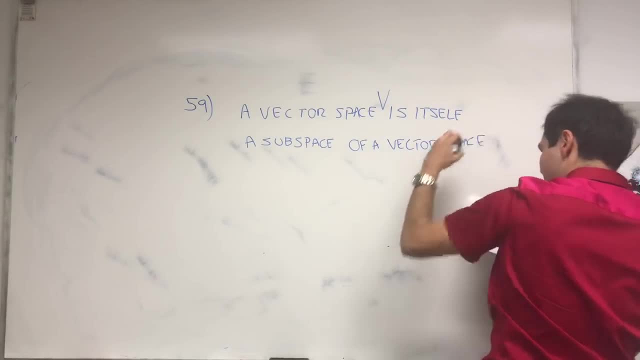 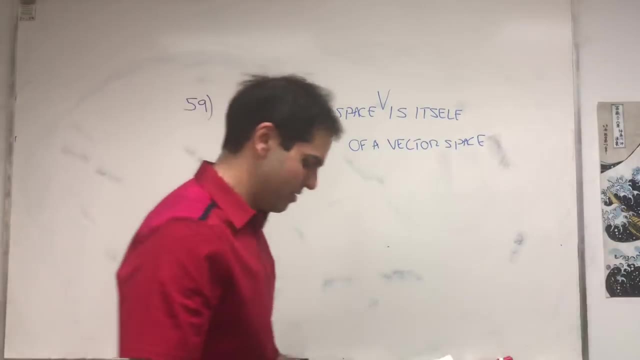 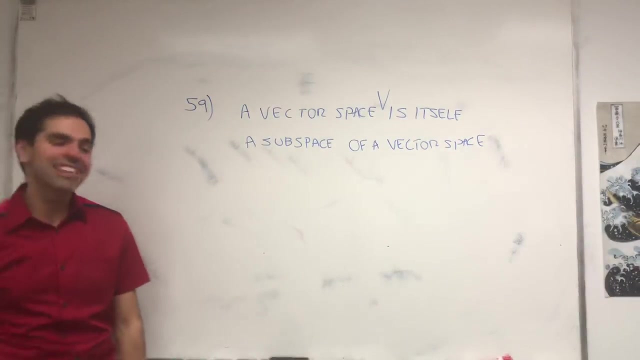 Next question 59 is really obvious because they outline thought-t出овал thoughts, And 59, nepali and onsati And very sat and very onsatisfied, or ways of saying satisfied, say, not satisfied, hot morales, ass or cocoa. And the answer is true, and actually the interesting thing is now, of course, the 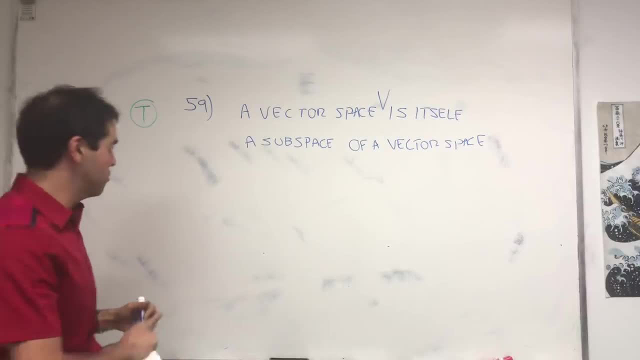 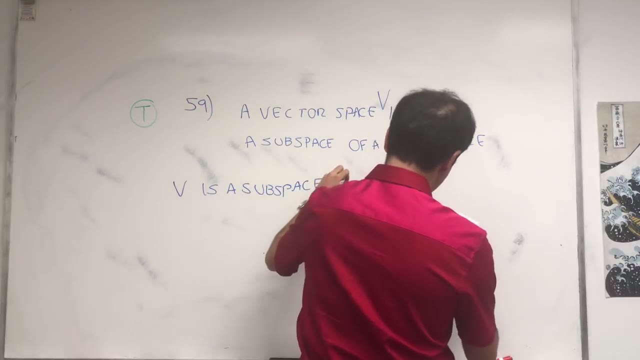 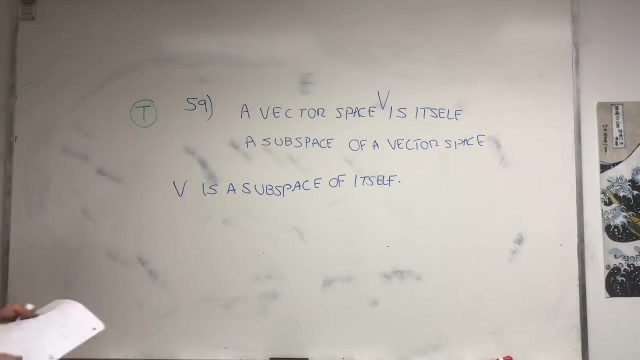 vector. space is a subspace. It's a subspace of itself. So v is itself an morgen, so v is itself a subspace, is a subspace all of itself. All right. and the next ones? they deal a bit with column spaces. 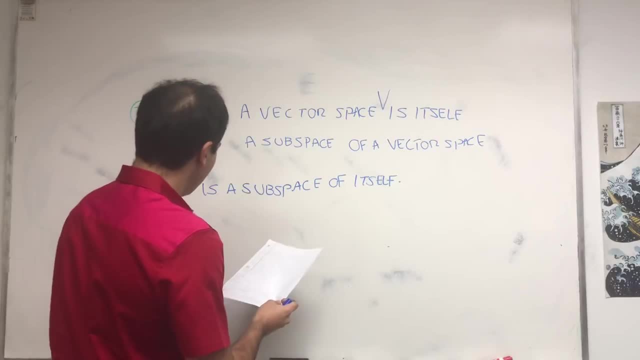 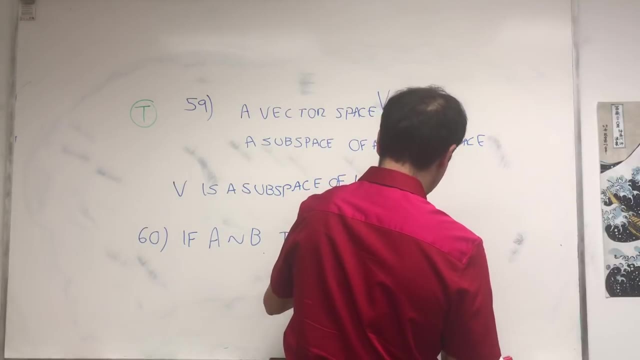 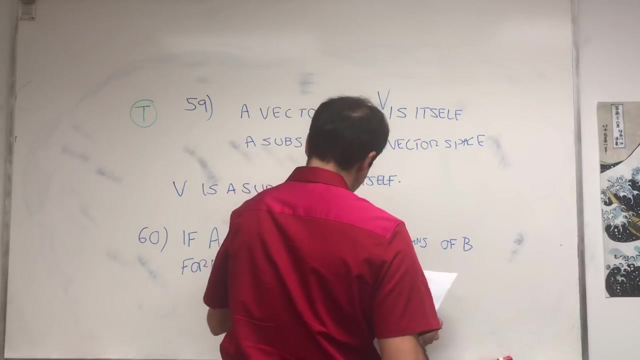 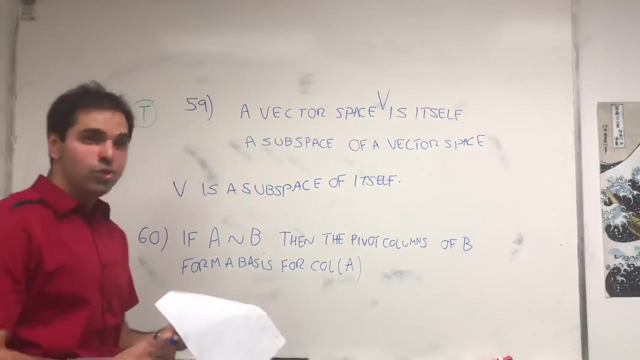 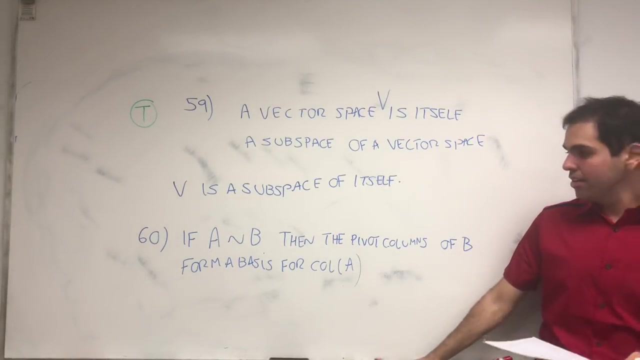 So if A is row equivalent to B, then the pivoting columns of B form a basis for the column space for column A And this language. Sixty is the Sudanese dialect of Arabic And Sixty is setun. What does this say? 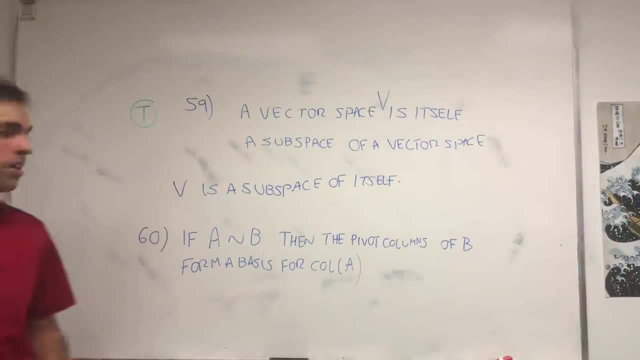 Is it true that if you row, If you row reduce the matrix A to get a matrix B, then you can just pick the pivot columns of the new matrix as your basis for the column space of A? Fortunately, this is false. Let me give you an example and explain then what happens. 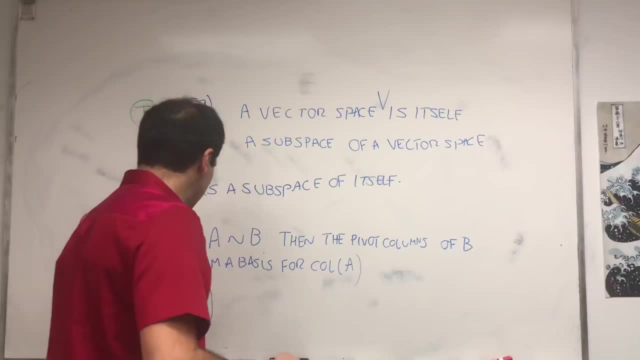 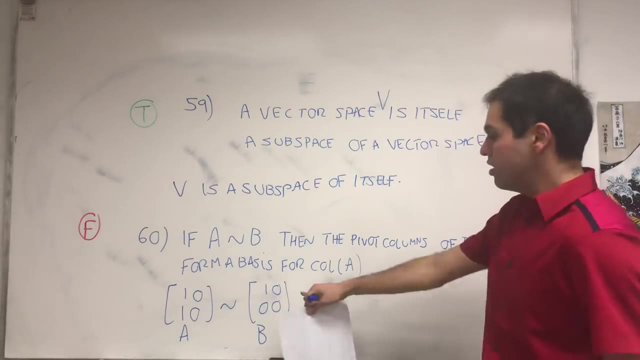 Again, consider the matrix 1, 0, 1, 0.. So this is A You row. reduce it to 0, 1, 0, 0, 0 to get a matrix B. The only column with a pivot is the first column. 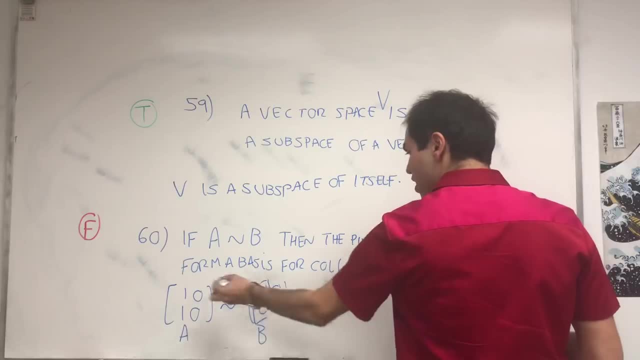 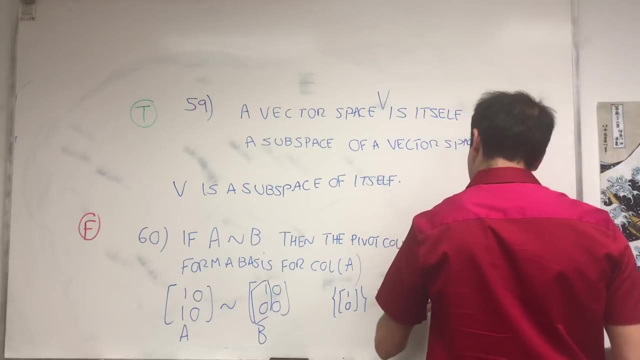 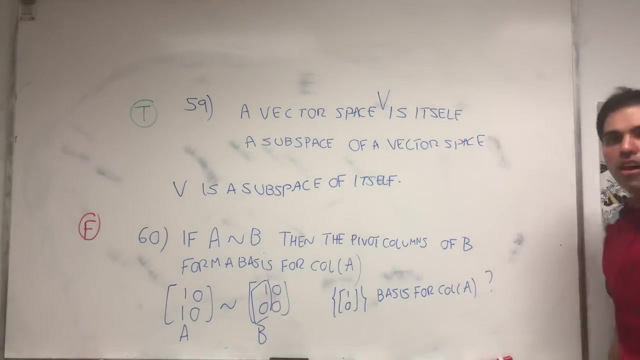 And the question is: well, is 1, 0 a basis, a basis for column space of A? It cannot be, because 1, 0 isn't even in the column space of A. The column space here is the span of 1, 1.. 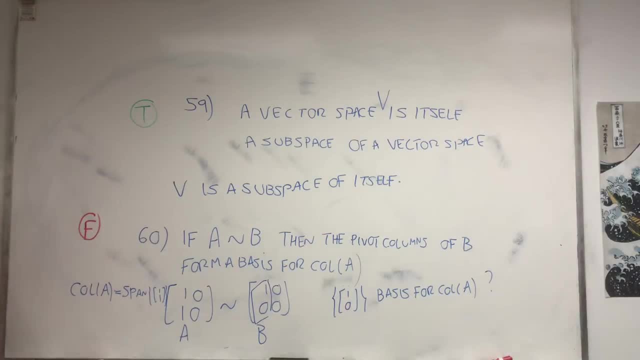 And this is why, If you want to find a basis for the column space, you row reduce and then you go back to the original matrix. So you row reduce A to get the row echelon form. You're like, oh, there's a pivot in the first column. 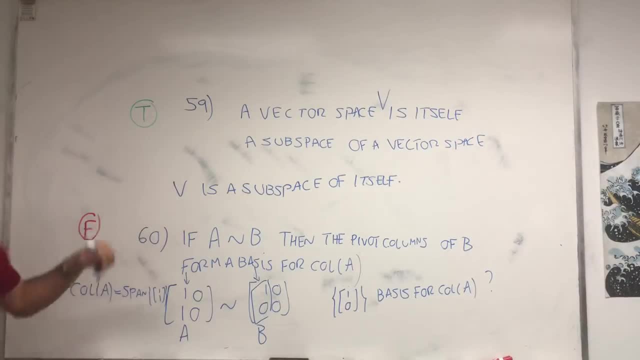 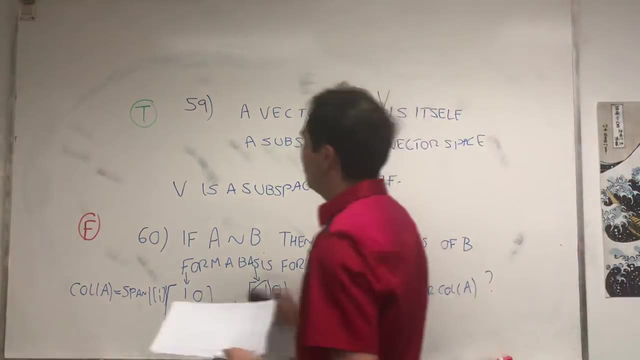 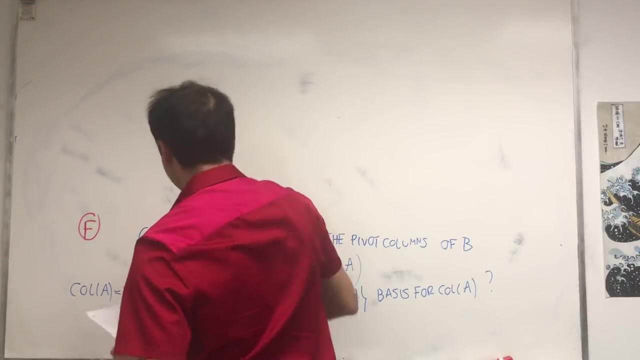 That's why you have to go back to the first column of A to find a basis for the column space. So Let me go back. Be very careful, All right, next question: I'm kind of related to this, So question 61.. 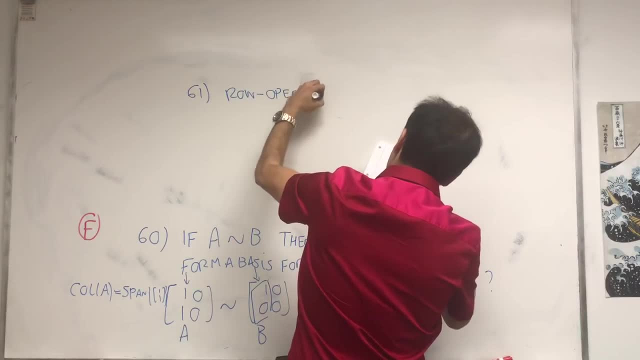 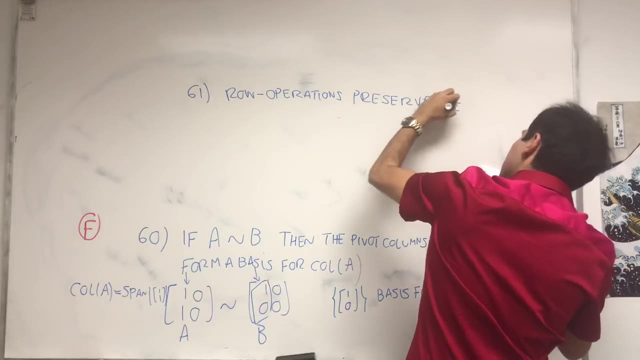 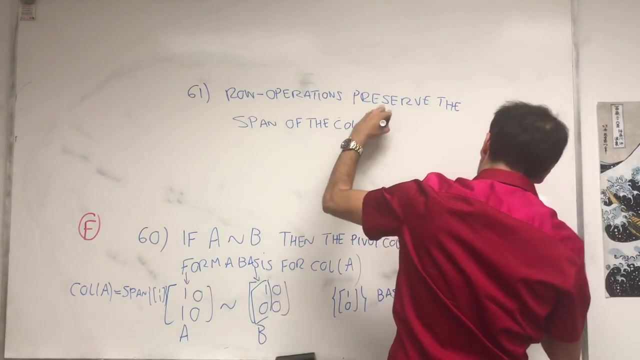 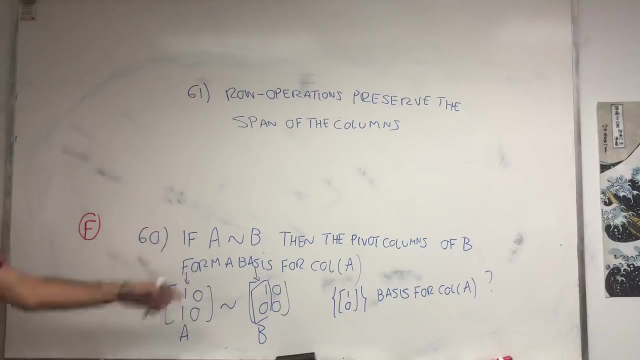 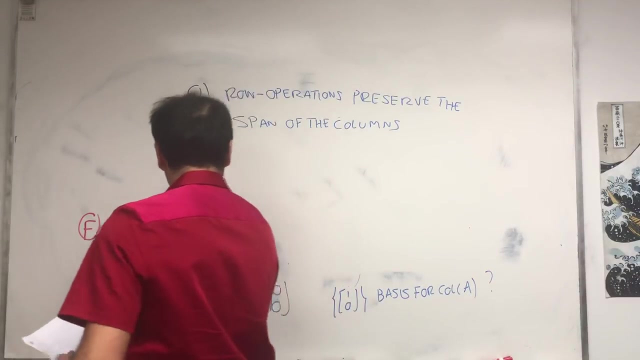 Row operations preserve the span of the column of the column. In other words, if you row, reduce a matrix A to get a matrix B, is the span of the columns the same thing. Let me keep that for me. Well, at least I'll write it again, maybe if it's false. 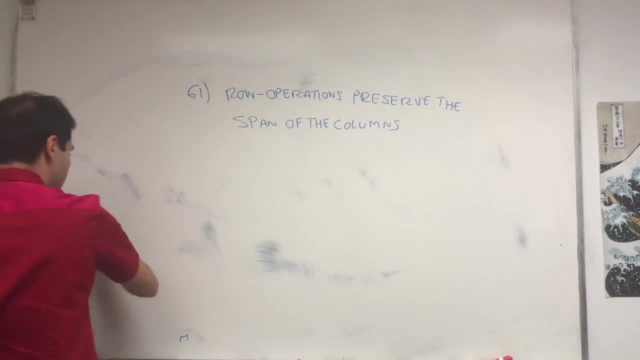 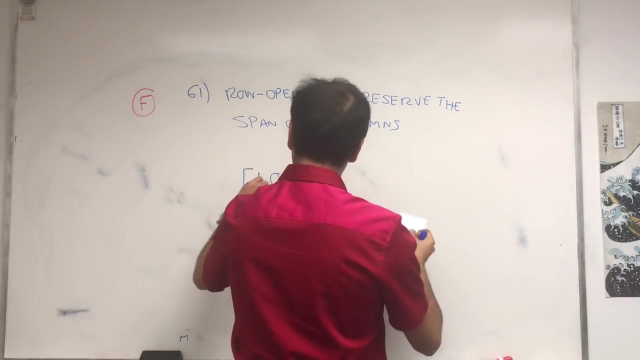 And 61, so a version of Punjabi, so Saraiki and 61 is Saatik, And unfortunately this is false And in fact the same example I erased is a good counterexample, because again, consider 1, 0, 1, 0, and 1, 0, 0, 0. 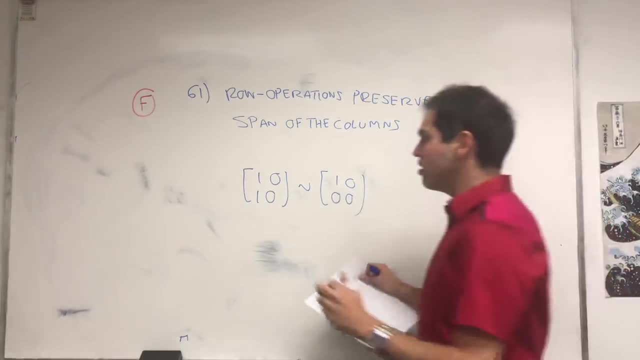 So you use row operations to do that. But look now the span of 1, 1, and 0, 0,, which is the span of 1, 0, 0, and 1, 0, 0, 0.. So you use row operations to do that. But look now the span of 1, 1, and 0, 0,, which is the span of 1, 1, 0, 0, and 1, 0, 0, 0.. 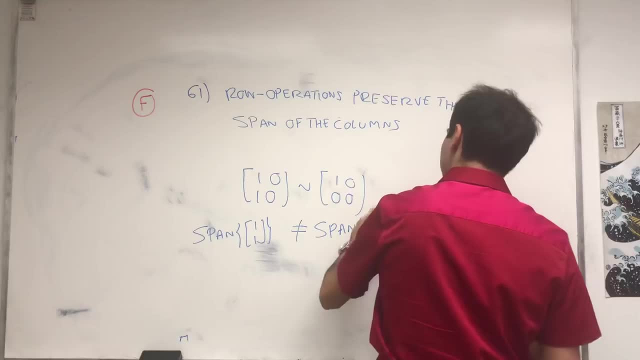 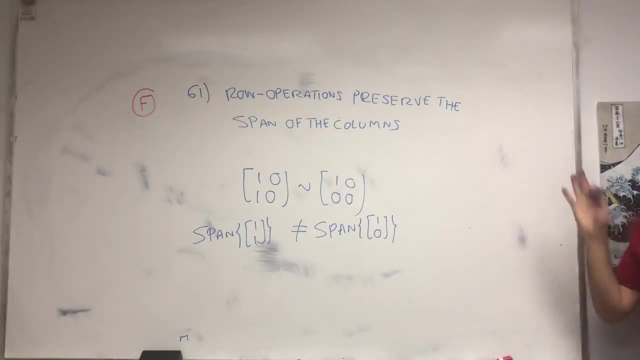 is not the same thing as the span of 1, 0.. So the span of those two columns and the span of those two columns are not the same thing. So row operations do not preserve the span, And that's why to find a basis for the column space, 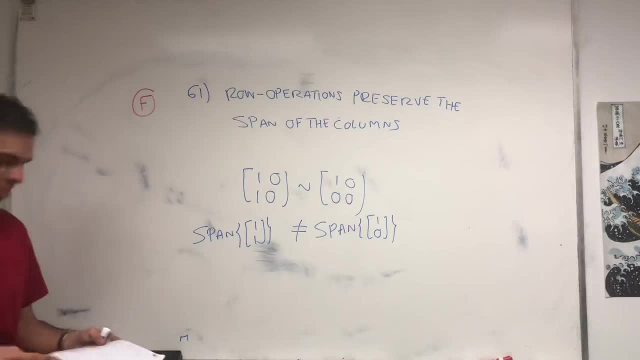 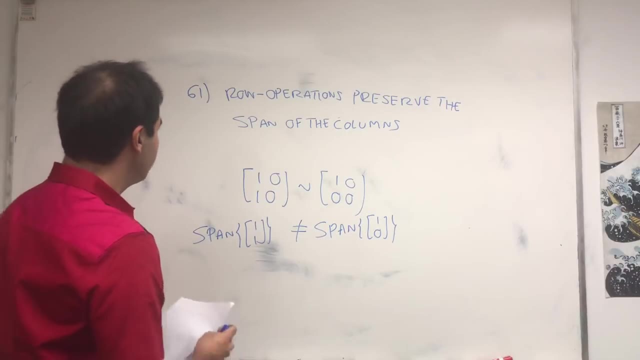 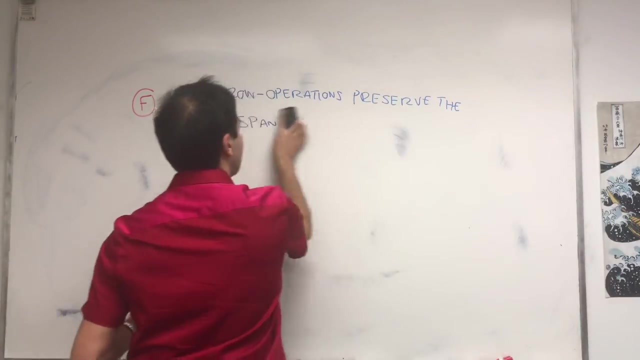 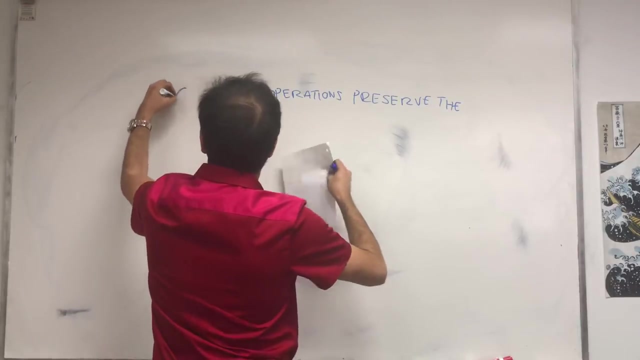 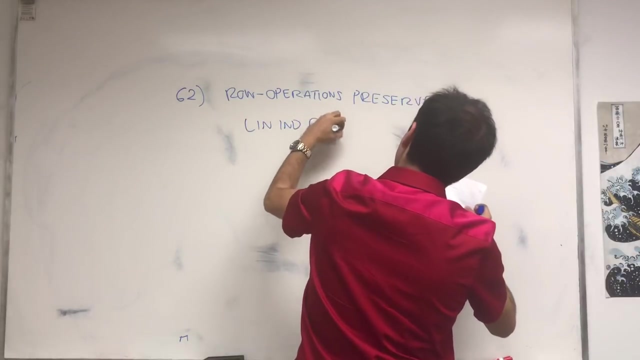 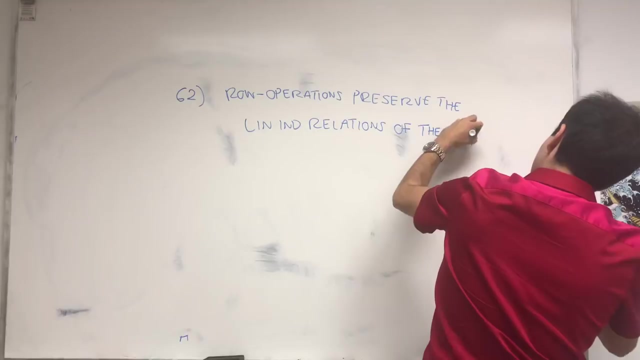 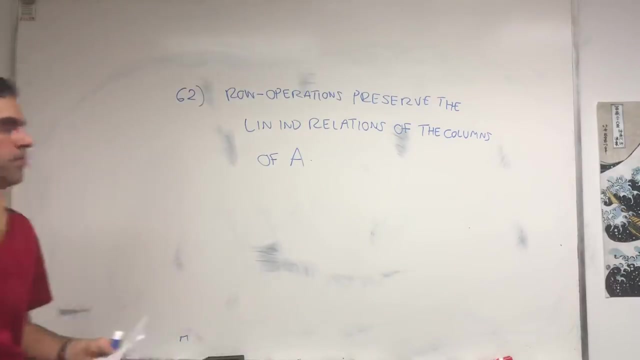 you have to go back to your original matrix, Otherwise this doesn't work. Okay, that said, maybe, or maybe not. what about linear independence? So do row operations preserve the linear independence relations of the columns? Okay, So we know that row operations destroy the span. 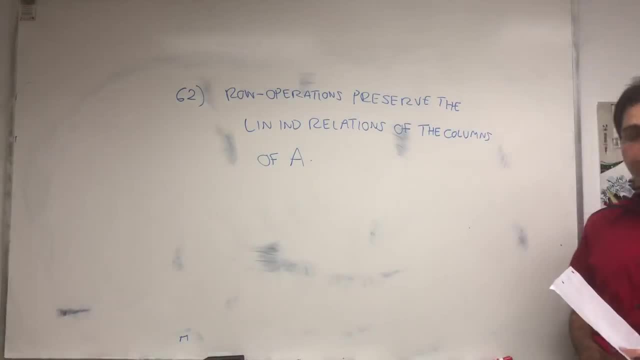 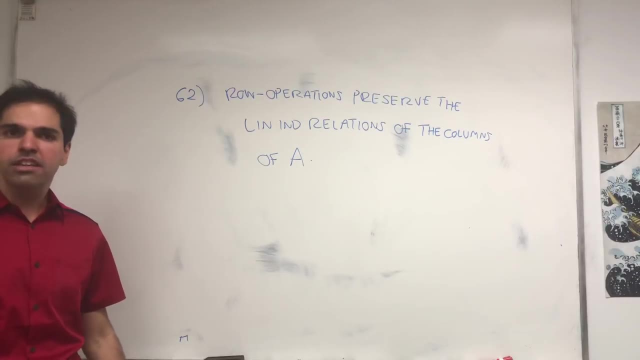 The question is: do row operations destroy the linear independence relations or not? So if, for example, the columns 1,, 2, and 4 are linearly independent, will the columns of the new matrix 1,, 2, and 4 still be linearly independent? 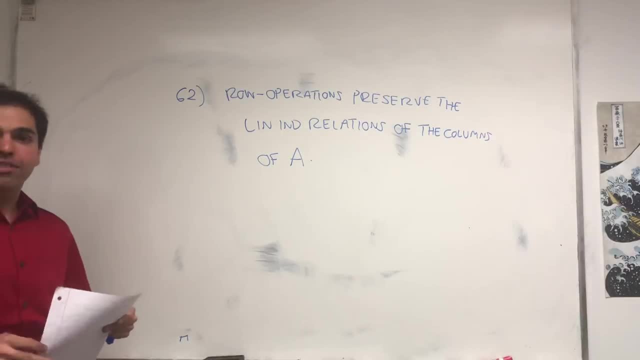 62,, so Cebuano, so a version of Filipino, and it's, oh my god, Canumanukduhaka. Crazy, wasn't it? And even though row operations destroy spans, row operations preserve linear independence. And let me explain to you why. 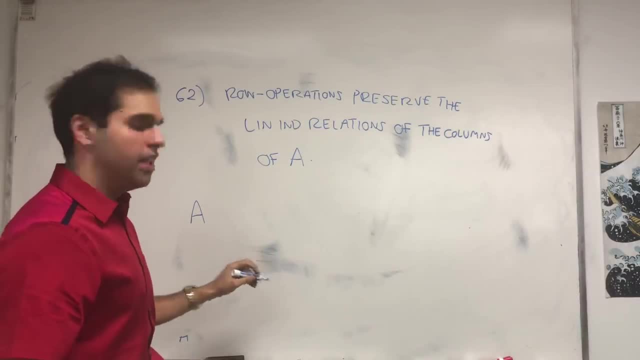 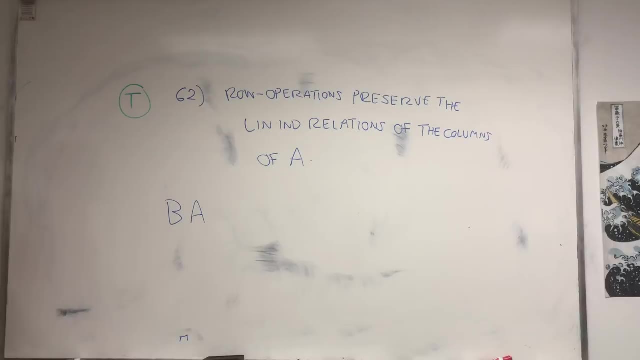 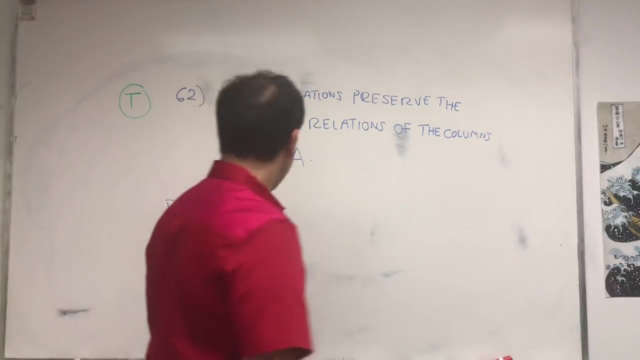 So if you row reduce a matrix A, it's really applying another matrix B to it. where B is the what's called is the product of elementary matrices. Okay, And look, suppose A, let's call it, let's say a matrix with three columns. 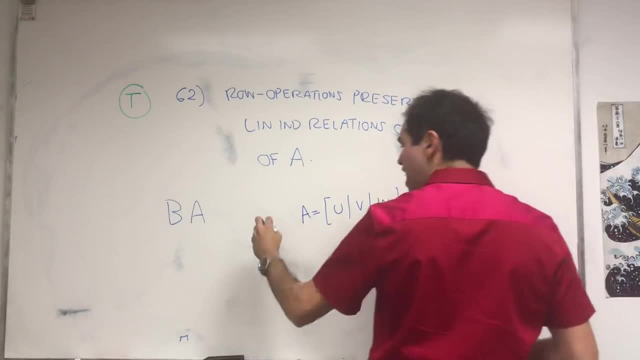 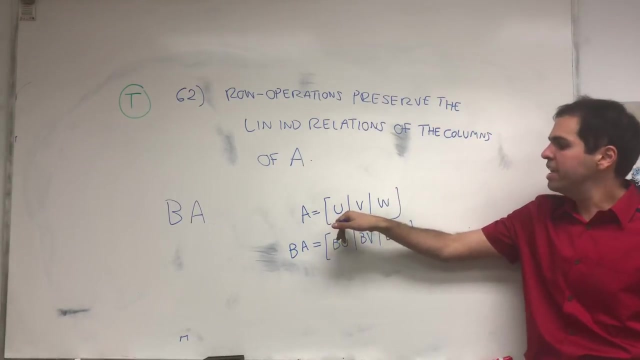 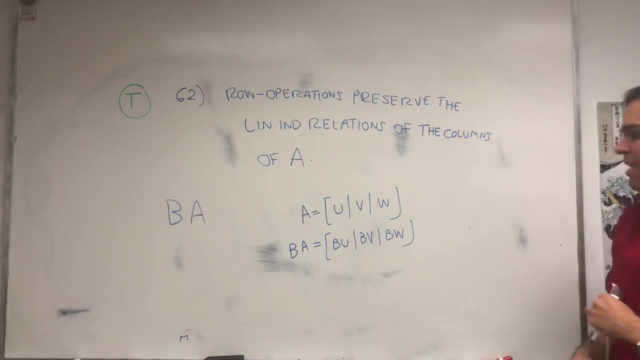 U, V, W. Then let's call it then: Ba is Bu, VV and VW. And just for sake of simplicity for the explanation, let's assume that all three columns are linearly independent. If not, you just throw away the linear independent ones. 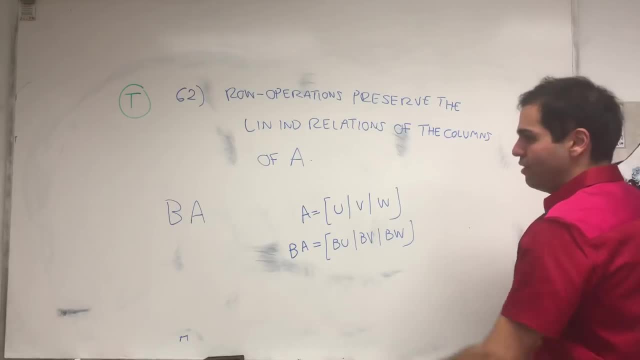 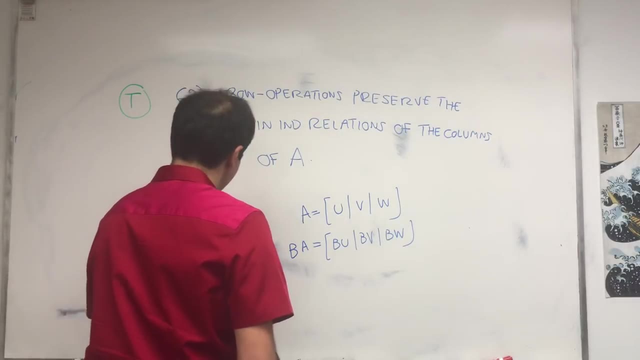 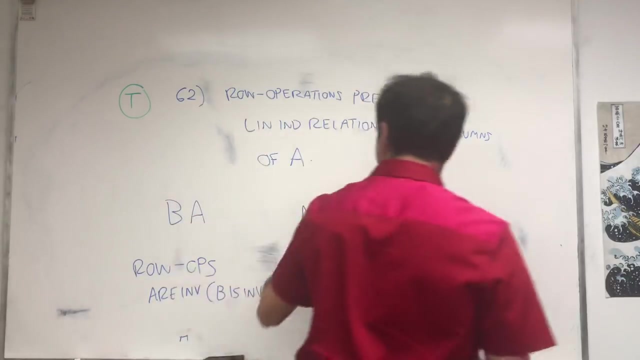 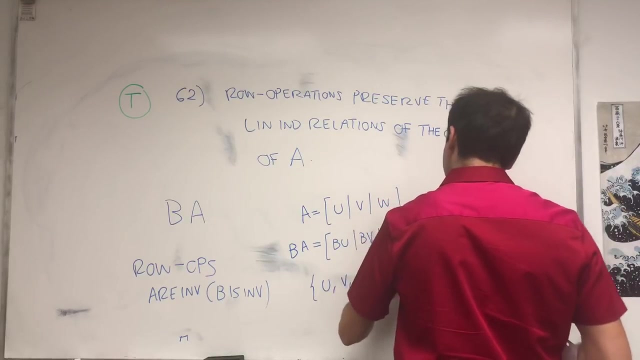 and basically remember row operations. they are invertible. So this is the main thing. So row operations are invertible. So in other words, B is invertible, And this is very similar to a question I did before- If U, V, W is linearly independent, 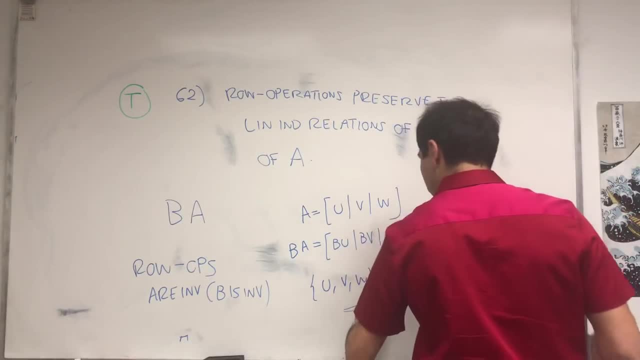 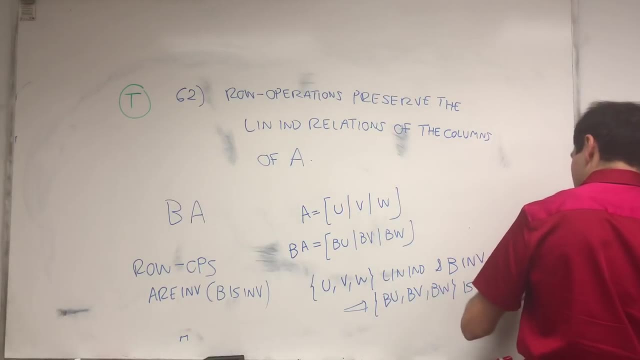 and B is invertible, then it turns out it's still true that Bu VV VW is linearly independent. I phrased this with one-to-one and onto. I said, if you have a linearly independent set and a one-to-one linear transformation. 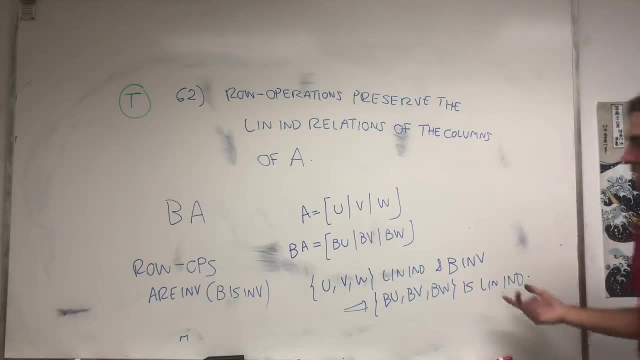 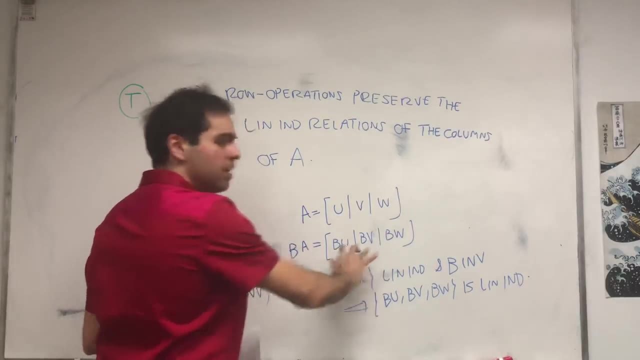 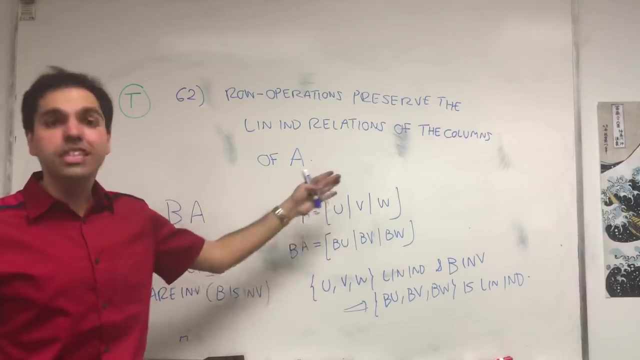 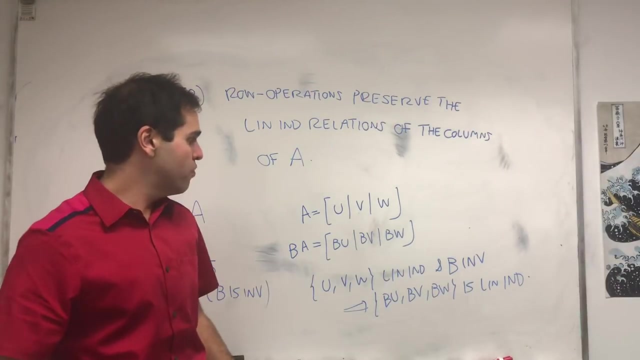 then the new set is still linearly independent, And in fact this is why if the starting columns are linearly independent, then the end columns are also linearly independent, And vice versa, and same for linear dependence. So really, if let's say, just the third one was superfluous, 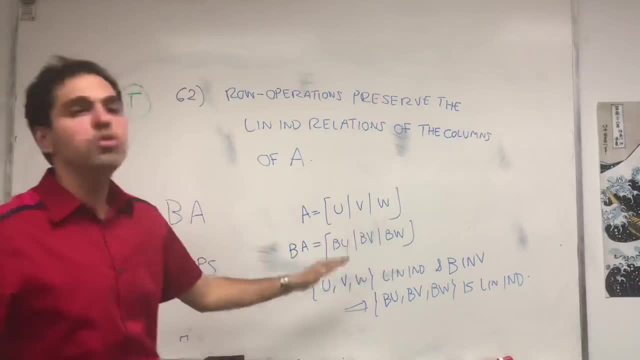 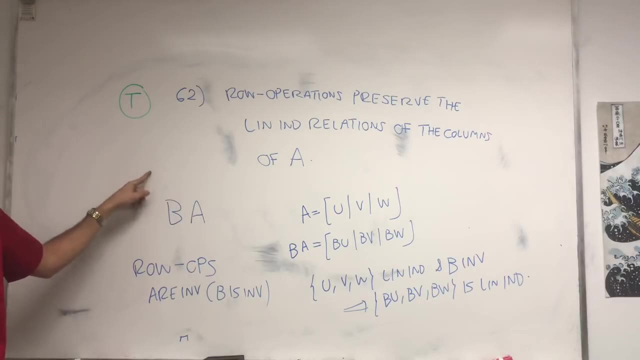 then you would just throw that away And you would still get Bu and BV is linearly independent, and vice versa. So this is why with row operations, you can go from one matrix to the other one without worrying about linear independence or not. 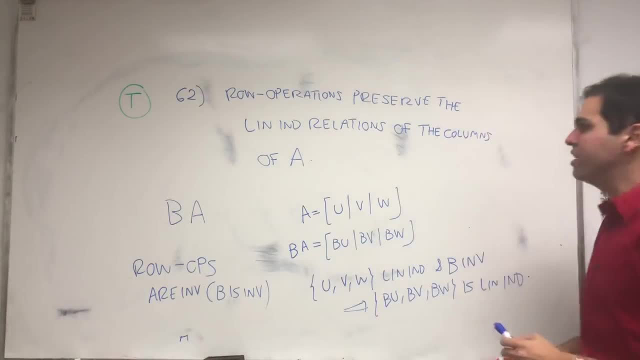 So row operations are very nice with linear independence relations And this is why this algorithm for finding column spaces it's very useful. So if you do one zero, one zero, and then one zero, zero, zero, even though this destroys the span. 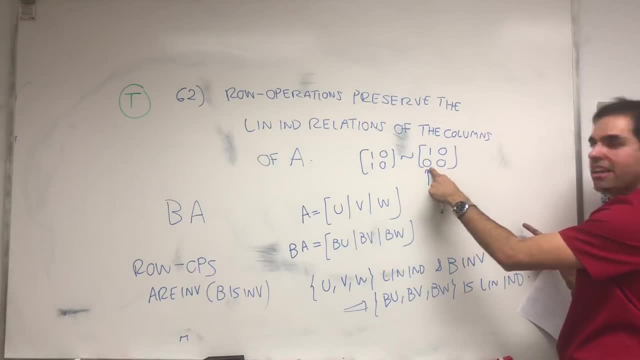 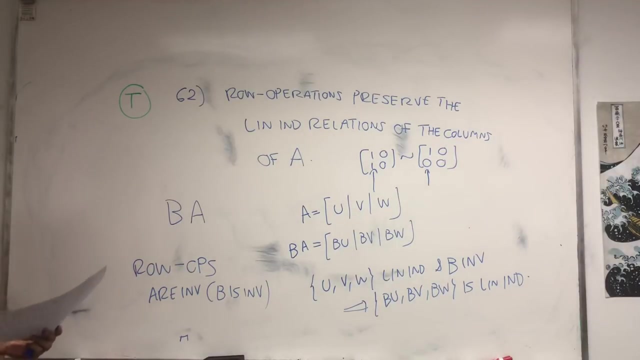 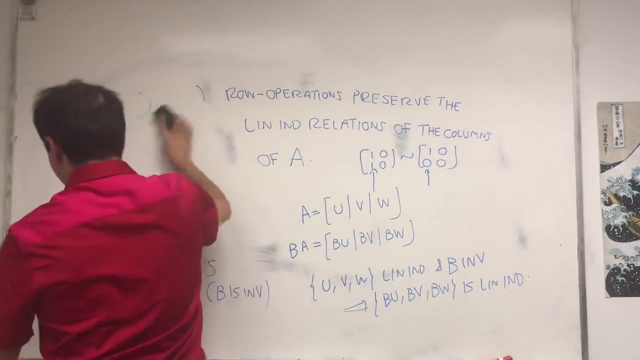 because this column is linearly independent. we know that this one is linearly independent And therefore a basis for the column space, Because a linearly independent set that spans it's a basis. Okay, good, And let's see. 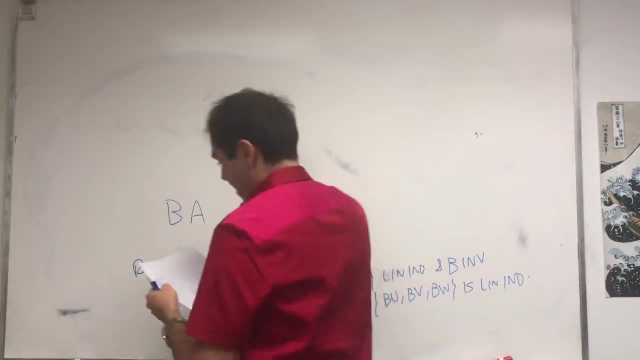 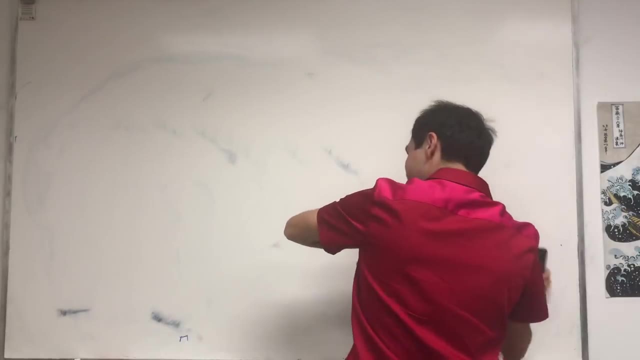 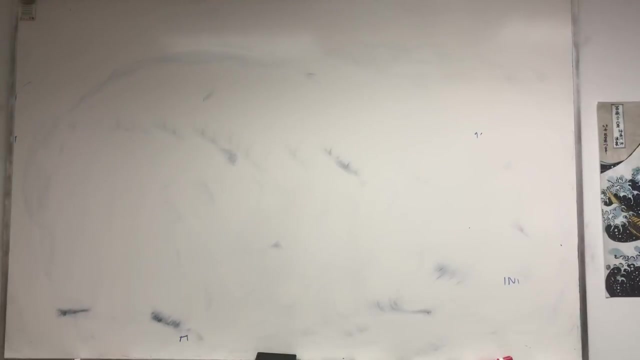 In fact, I may have given away the next question, So question 63.. Let's see, Holy crap, We're almost, are we like? yeah, we're almost at the two hour, maybe three hour mark. Oh my God. 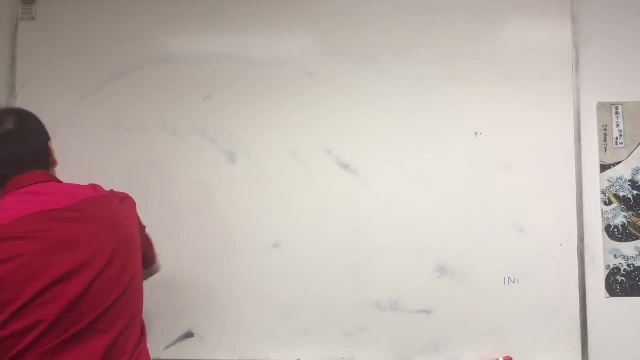 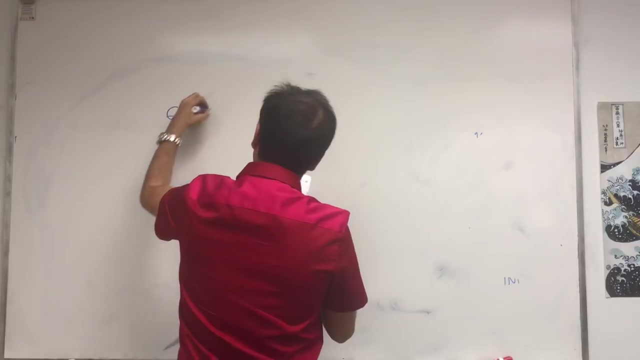 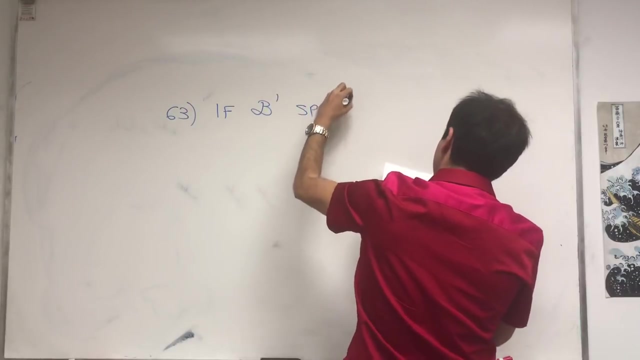 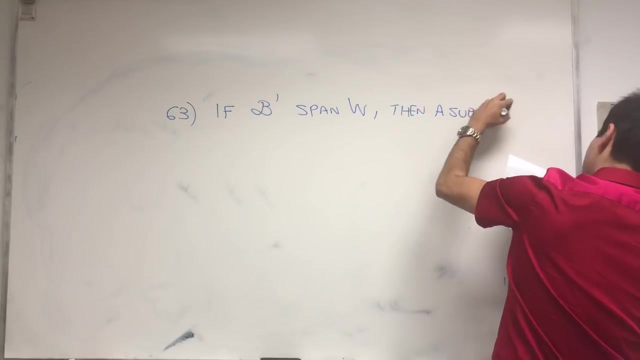 we're almost at the three hour mark. Man, it's a nice run today, So Next one, So 63.. If a basis, or sorry, a set, spans a subspace, then a subset B of B prime. 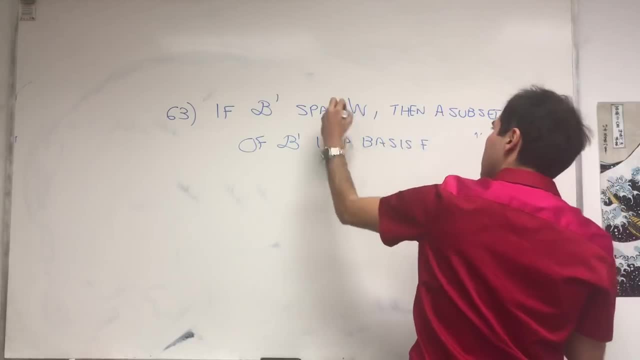 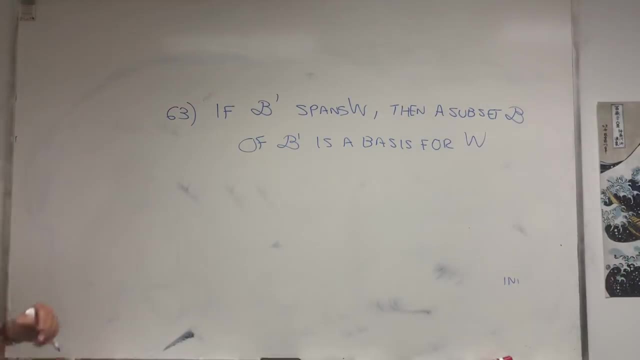 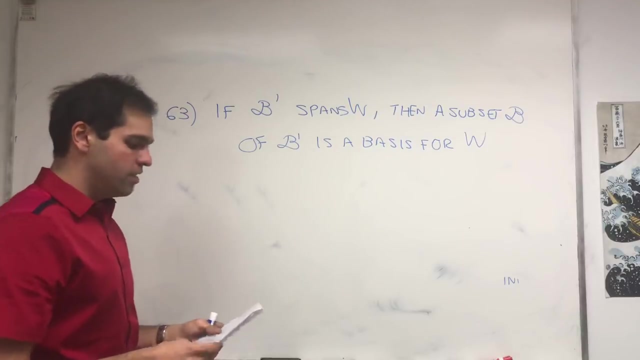 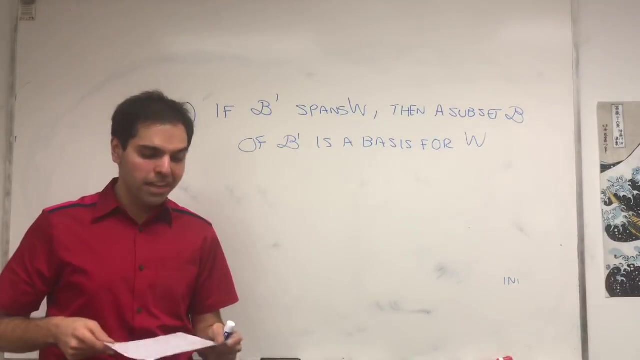 is a basis for W Because you have a subset, a subspace and a spanning set. can you extract a basis from this? And 63 is the Lebanese version, the dialect, so Northern Lebanese version of Arabic. And 63 is: 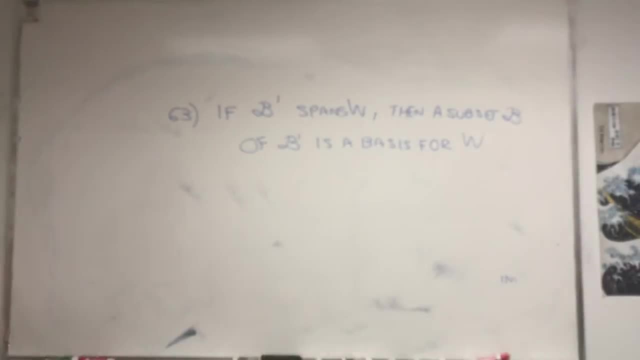 thaler wa sutun. And indeed this is true. This is one of the fundamental facts of linear algebra. So if you have a spanning set, then you can extract a basis, For example- let me tell you so- in R2,. 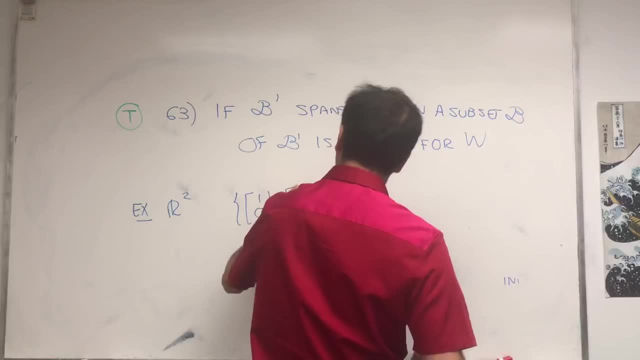 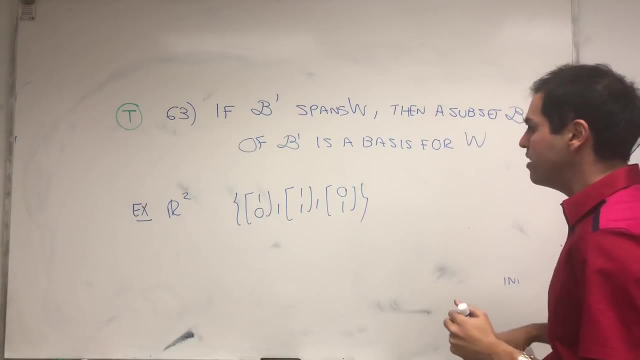 the following set: you can check that it spans one, zero one, one and zero one. So you can check that it spans R2.. It spans the whole space And what it says is: you can sort of extract a basis from this. 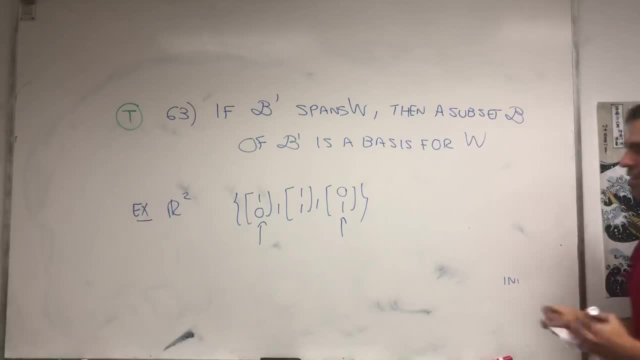 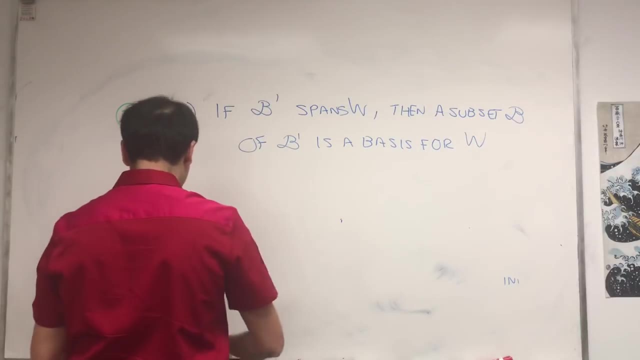 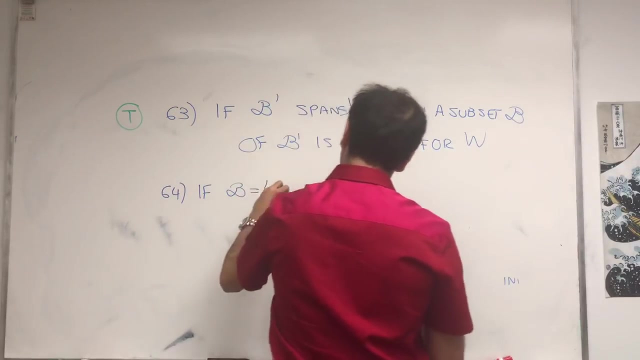 And in fact one zero and zero one is a basis. So this is true. What about the next? the next ones are kind of related, So 64, if a set, let's say V1 up to Vn, is linearly independent. 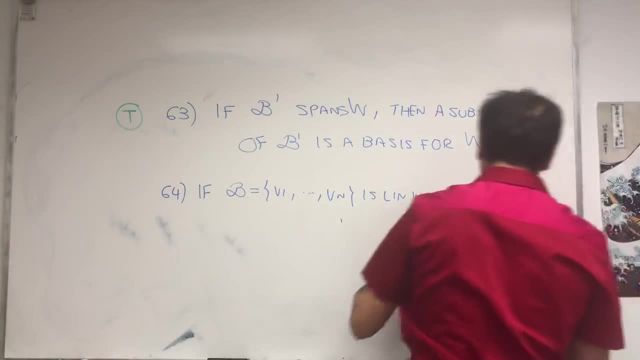 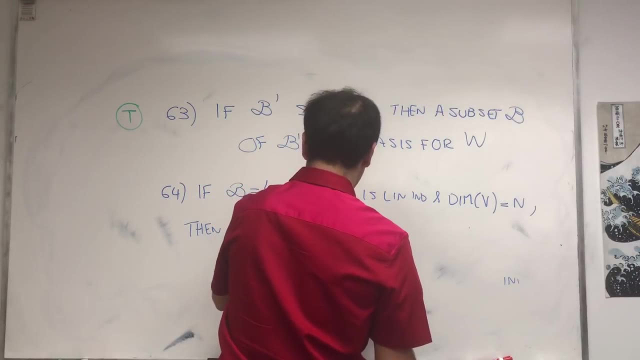 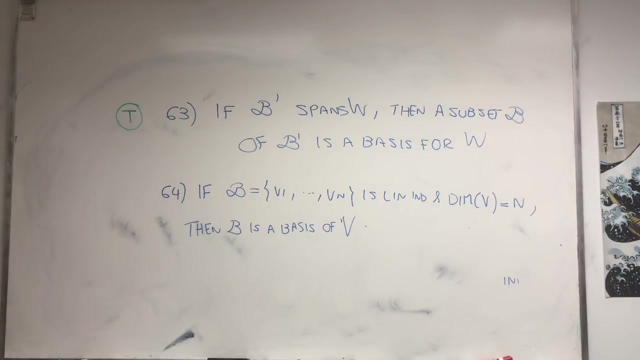 and the dimension is n, is it true that V is a basis Of V? In other words, if you have a linearly independent set with enough vectors, is it a basis. And before I say that, so 64th language. 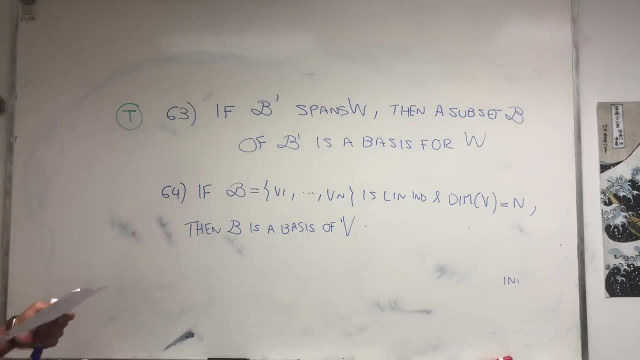 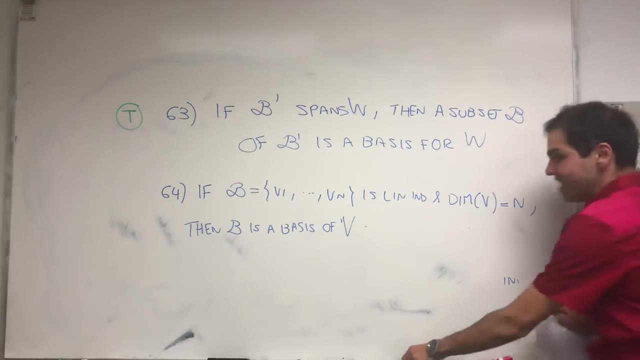 northeastern, eastern version of Thai, then it's huksepsi, Almost like Pepsi Huksepsi, And indeed this is true. So the nice thing is, if you know the dimension, then you don't have to show that it spans. 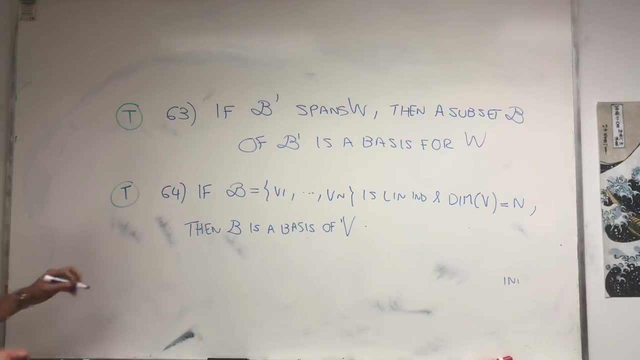 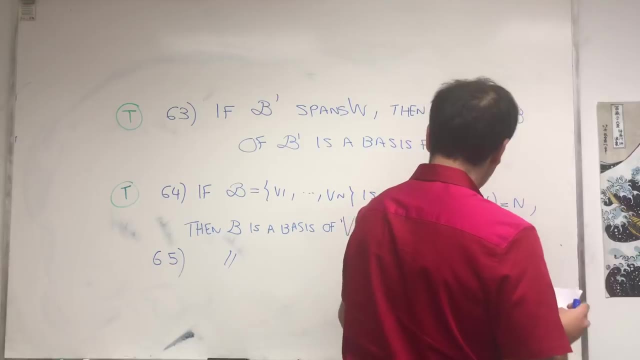 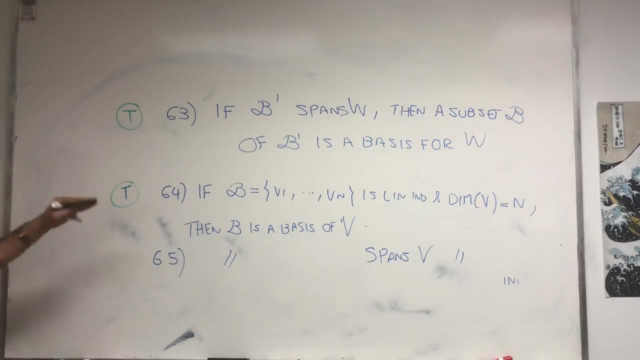 All you need to figure out is if it's linearly independent. So that works. Next question: Same thing, but it spans V. So if you have a spanning set for V, that's sort of small enough. so it has just n vectors. 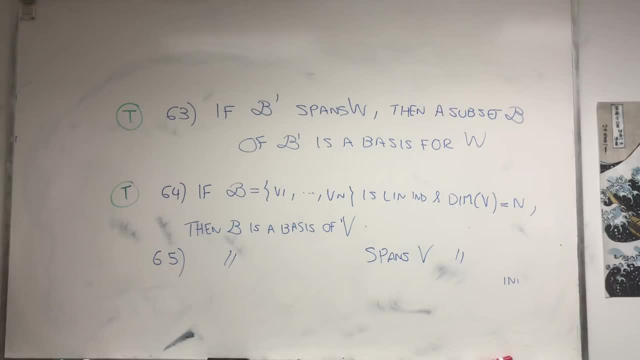 with the dimension. is it a basis? And 65 is asamis, pokok, poksosti, poksosti, I don't know, or pokoksti or something, And this is also true. So a set that spans. 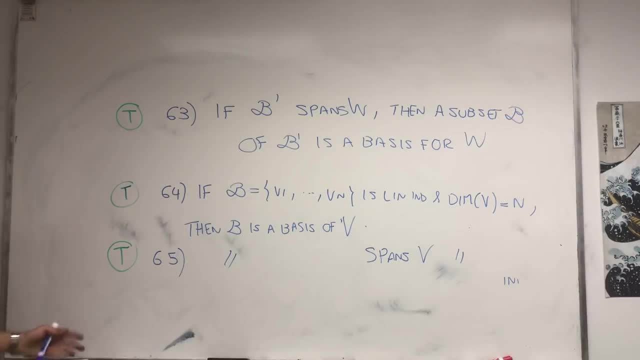 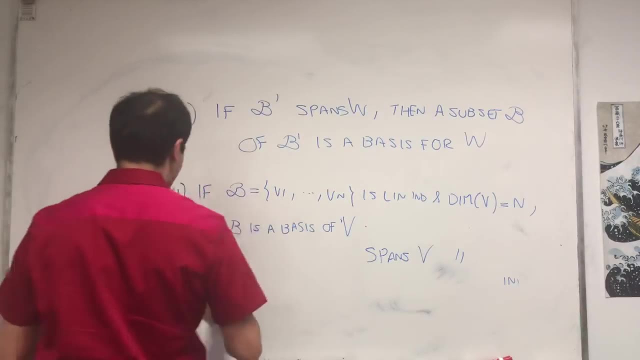 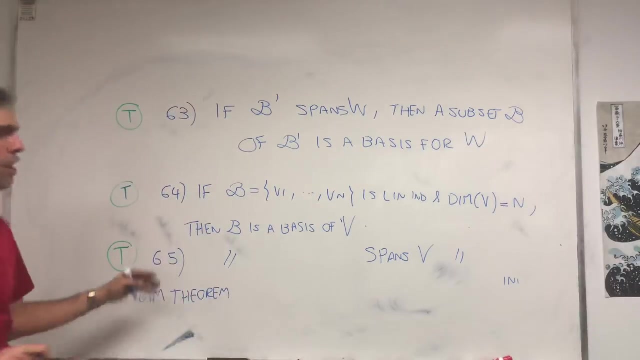 and that has not too many vectors. it's also a basis, OK, And all those two things are called the dimension theorem, If you want to look them up. This is what makes dimensions so nice If you have a set, a big set that's linearly independent. 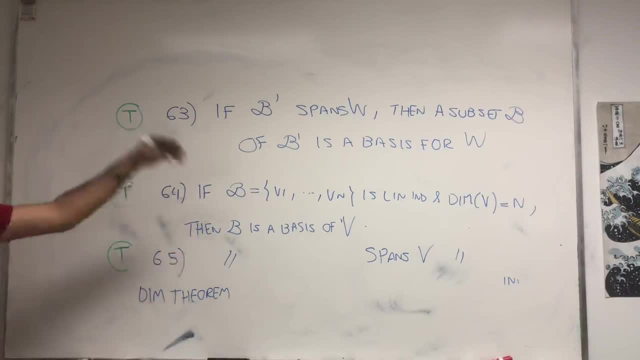 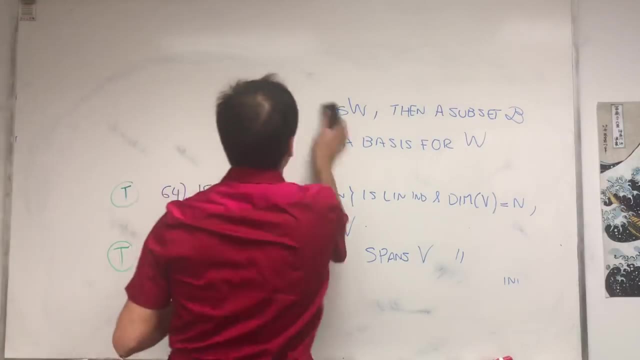 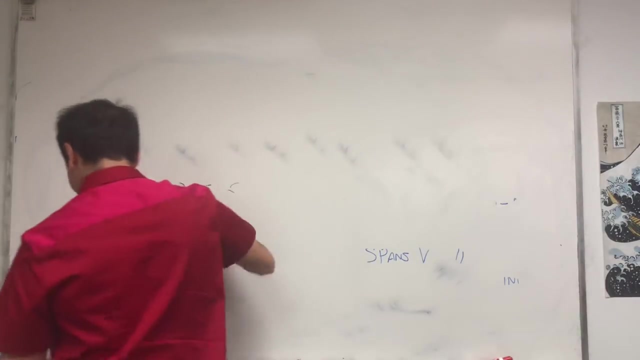 it's probably a basis. If you have a small set that spans a vector space, it's probably a basis, Because it's all about the base. About the base, No problem, OK, Next question. That was again a sprint, like we're caught up with questions. 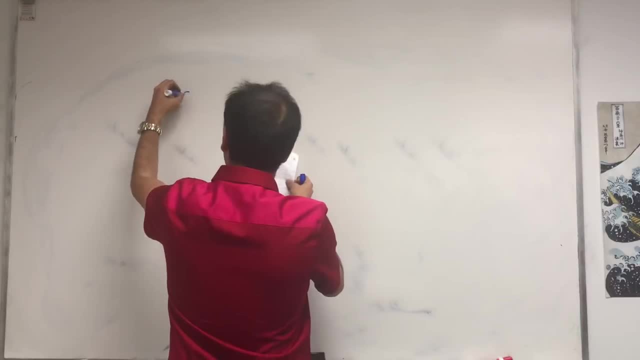 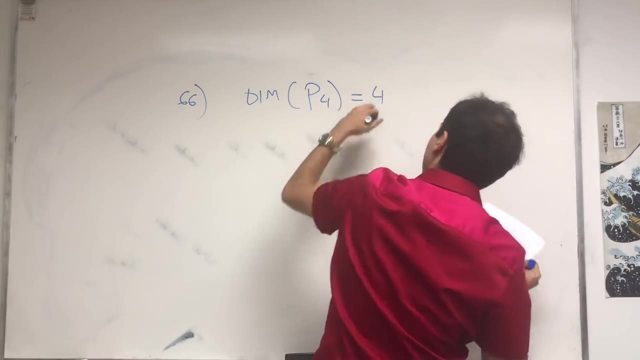 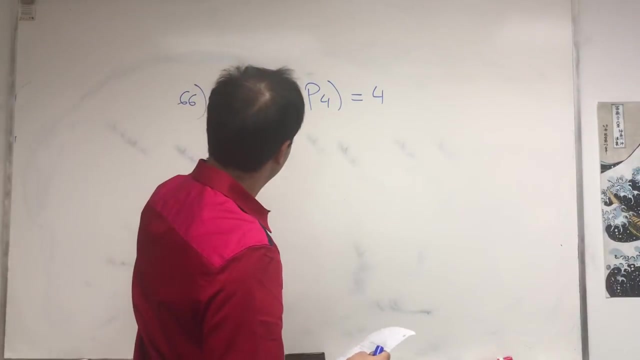 So question 66.. That picks on root 66.. So is the dimension of the set of polynomials of degree less than or equal to 4, you know like, for example, x to the 4th minus 3x squared plus 2.. 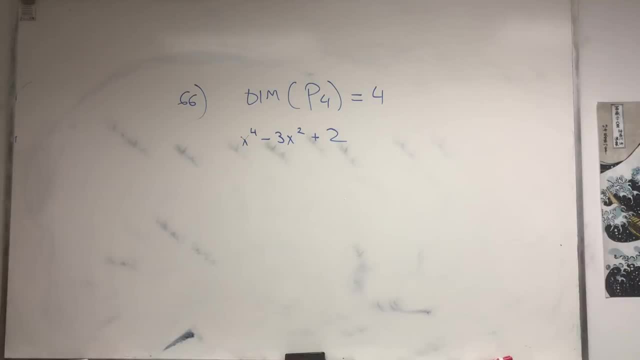 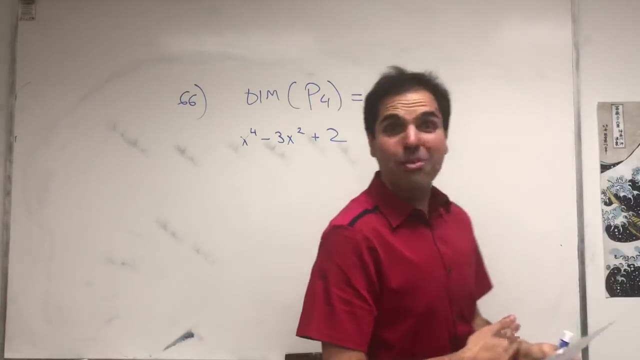 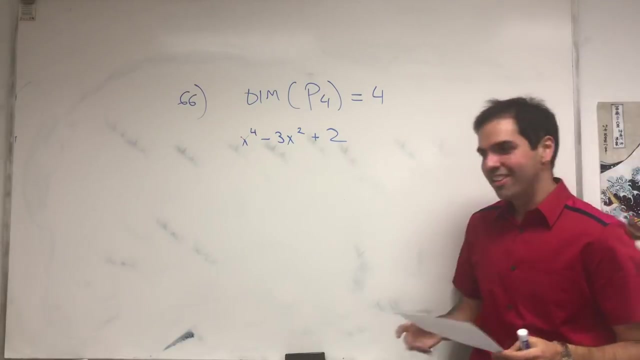 That's in P4, because it has degree less than or equal to 4.. Is the dimension equal 4?? I think the language has become harder than the math. So 66 is Hungarian and it's almost sounds like Dutch, but it's Hungarian. 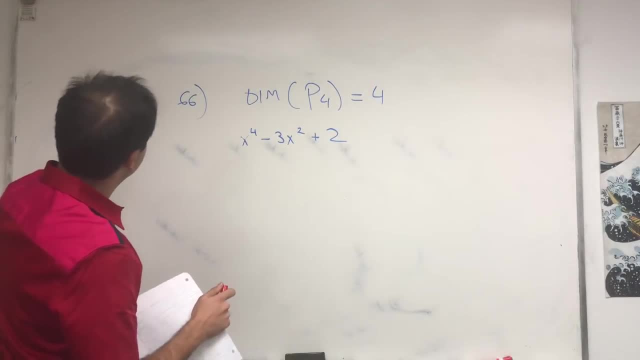 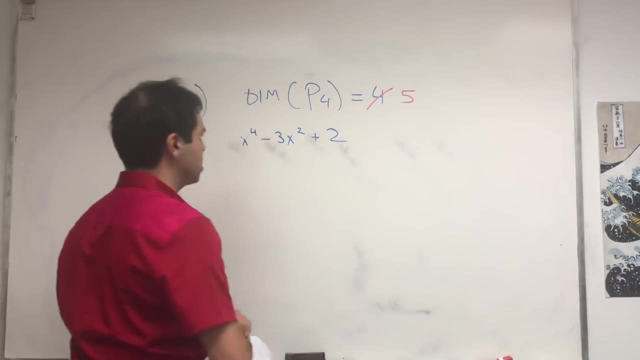 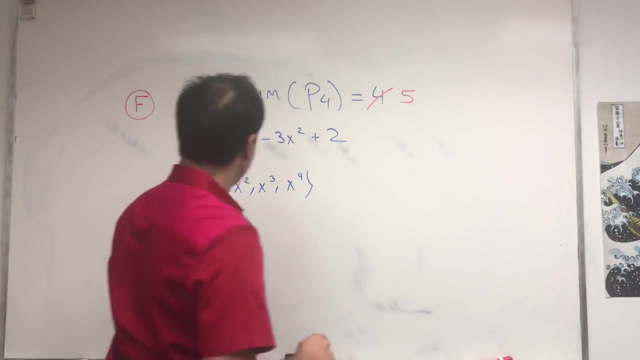 And unfortunately this is false. It turns out the dimension of P4 is actually 5. And that's because let's find a basis. A basis is 1x x, squared x, cubed, x to the 4th, which has 5 elements. 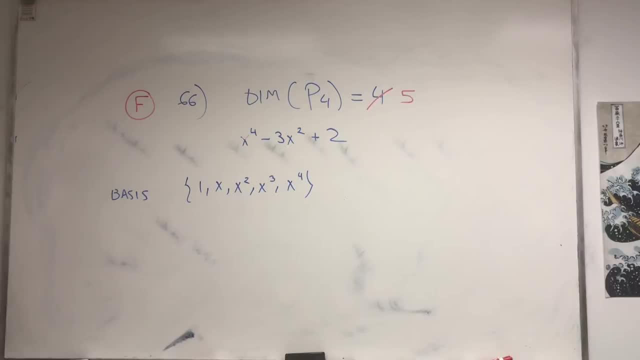 Again, to find a dimension, just find a basis and count how many elements there are. And here we have 1,, 2,, 3,, 4, 5.. So dimension of P4 is 5.. And now let's move on a bit to coordinates. 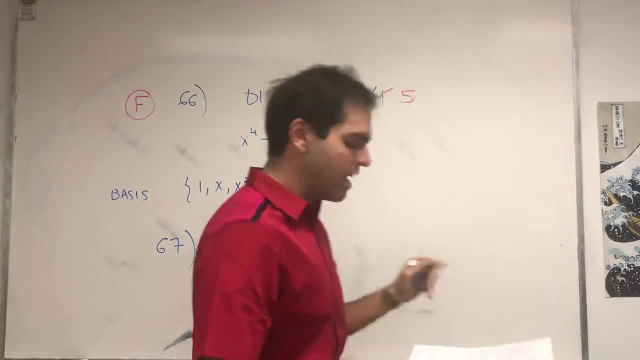 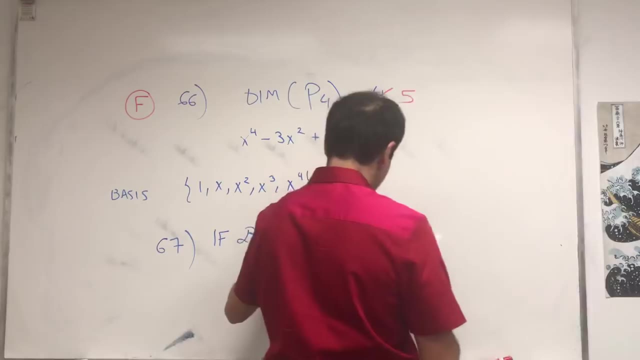 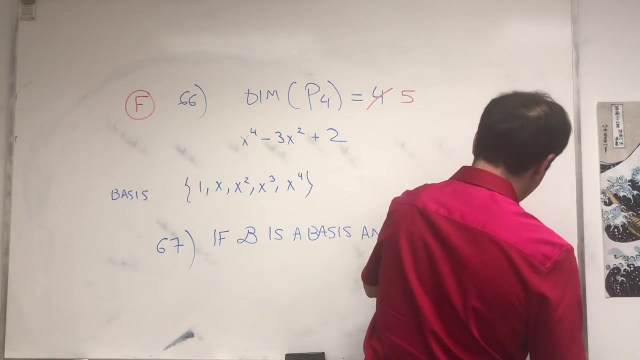 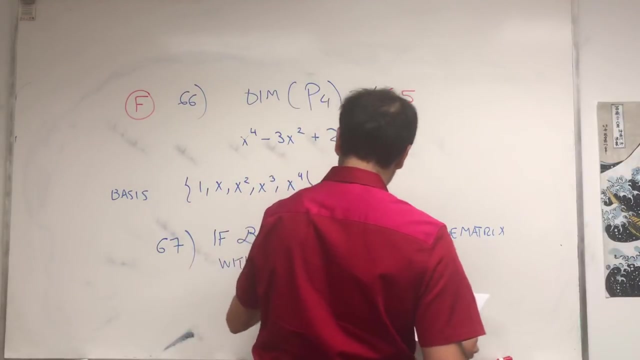 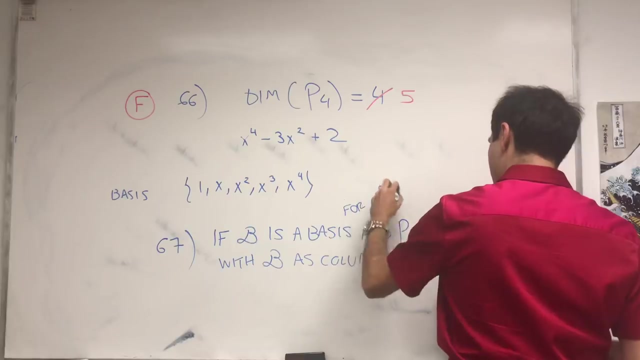 So I think the last four questions, or the next three questions, and then one more has to do with coordinates. So if P is a basis and P is the matrix, with B as columns- and I think here is a basis for Rn or something- Then we have that P. 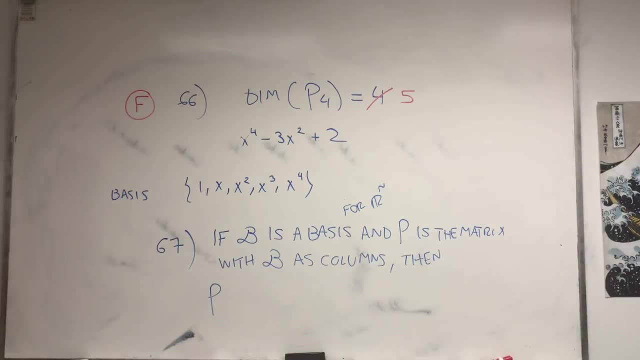 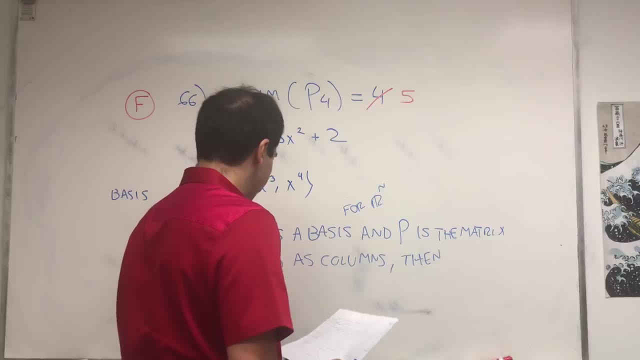 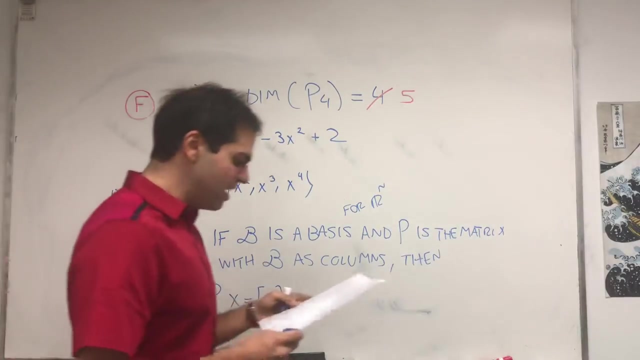 so it's what's called a change of coordinates matrix, I think, from B to the standard basis. Then we have P of x equals to xB. That was like xD And 67,. oh, so it's in Bangladesh, so Chitagonian. 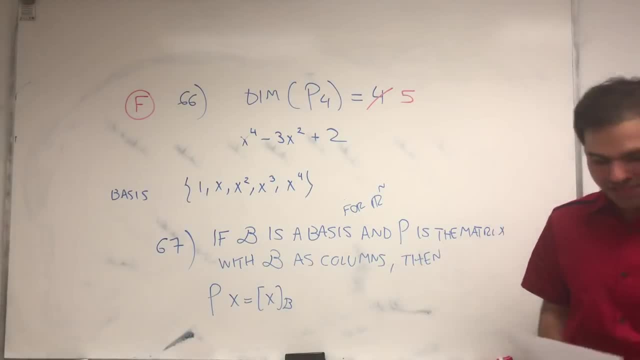 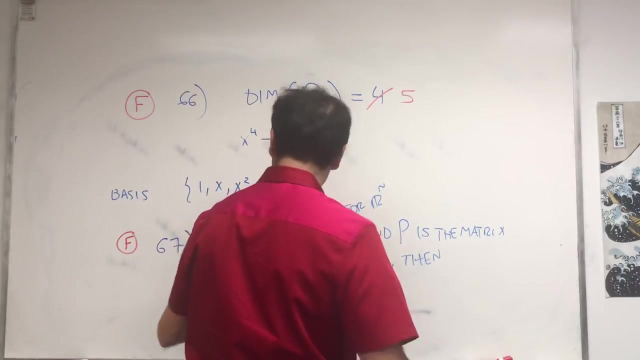 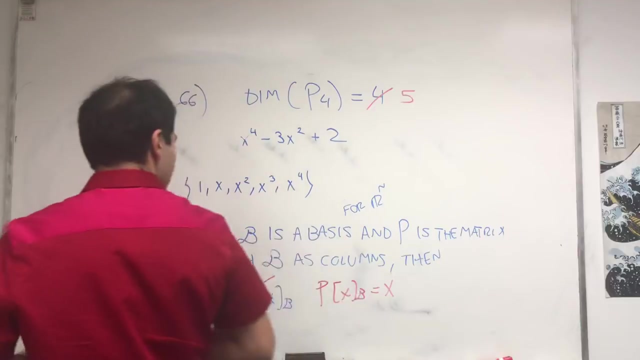 and it's oh, very cute: Satasati, Satasati, Okay, And unfortunately it's the other way around. So what is true? So it's false. What is true is that it's false And it's really. P of xB equals to x. 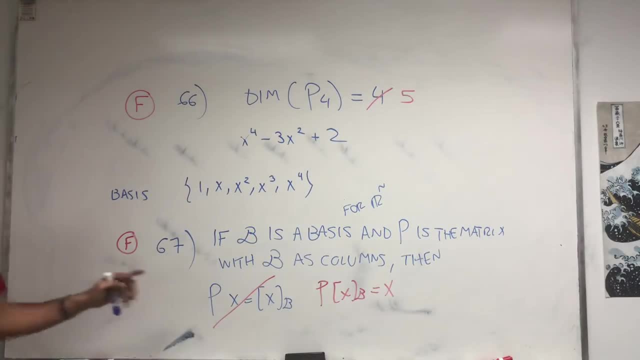 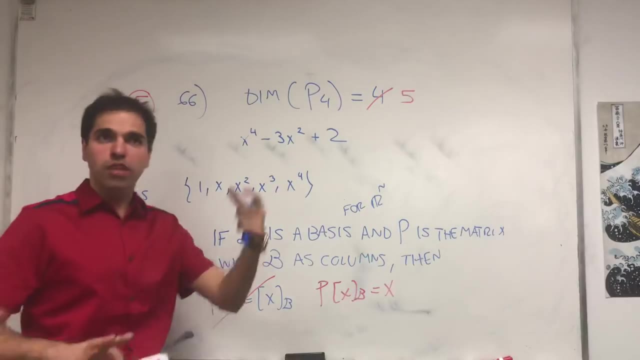 And the way to think about this. I always like to think of xB, so the coordinates of x with respect to B. I like to think of them as a barcode. So if you have an apple, the barcode will be like 124 or something. 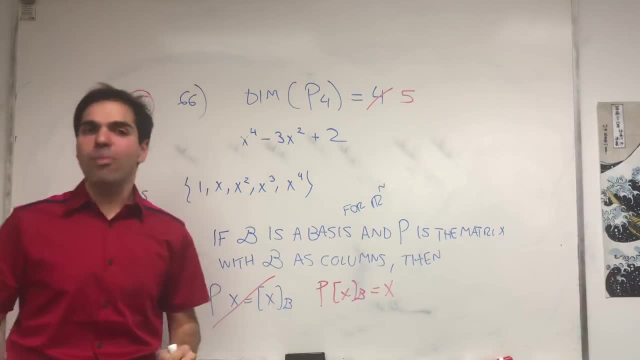 And P what it does. it reads the barcode. It's like a barcode scanner, So it takes a code as its input and it spits out what it is Like. it says, oh, the barcode is 124,. and then bam. 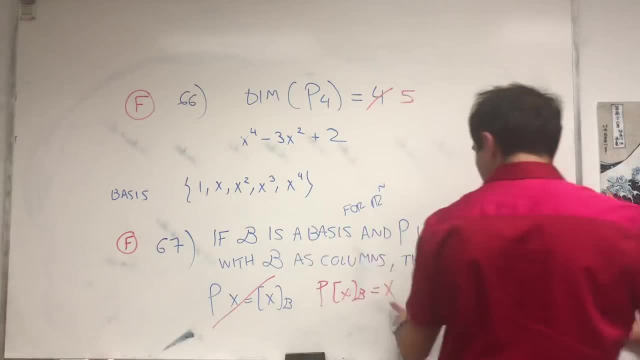 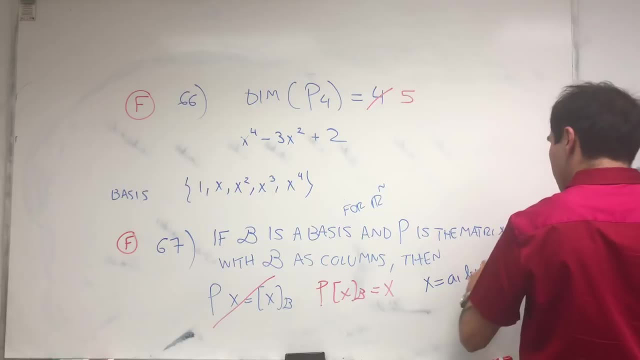 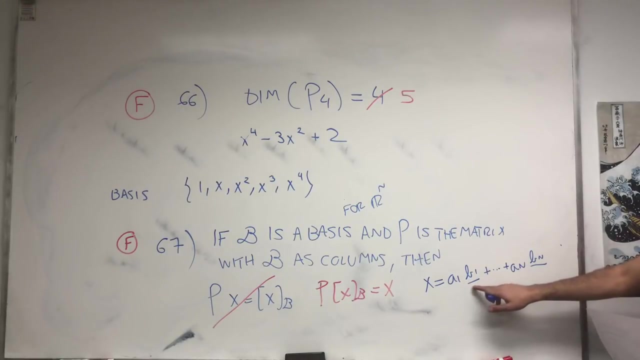 it tells you it's an apple. And why is that true? Because what are coordinates? Suppose x is, let's say, a1, b1, plus dot, dot, dot plus an bn. Okay, so where bi are the basis vectors? 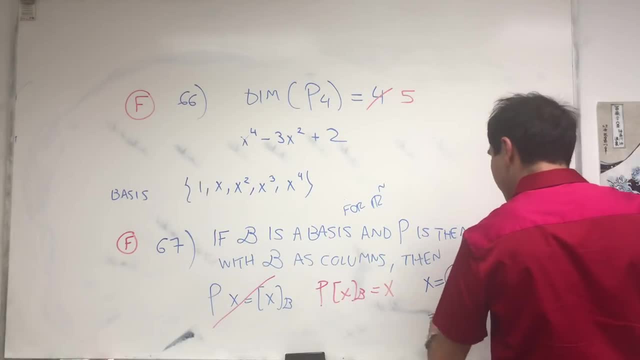 and then ai, they're the coordinates. Well, that's the same thing as saying b1, dot dot dot bn of a1, dot dot dot an, And this, by definition, is P. It's the matrix. 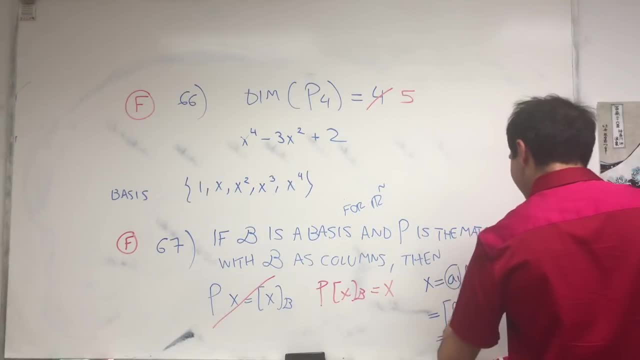 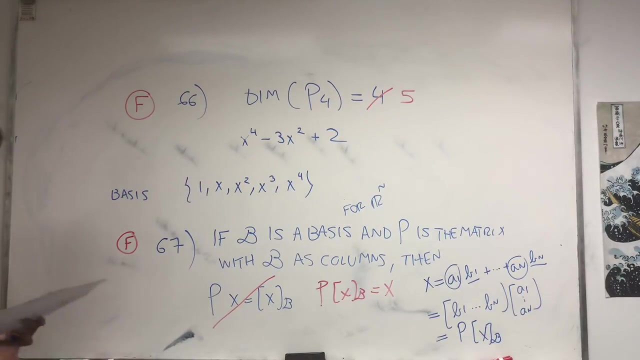 whose basis vectors are the b's. So no, not the b's, And ai, those are the coordinates. So x is P of xB. So you see, that's why this is true and it's not the other way around. 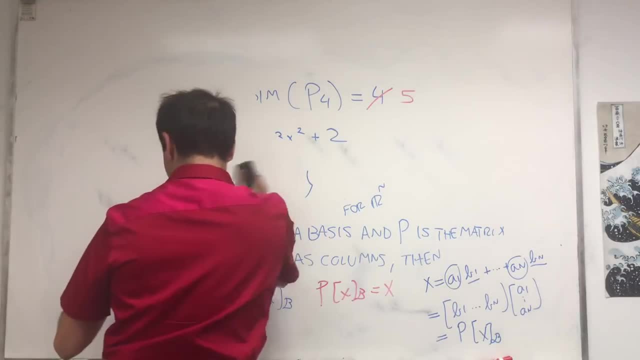 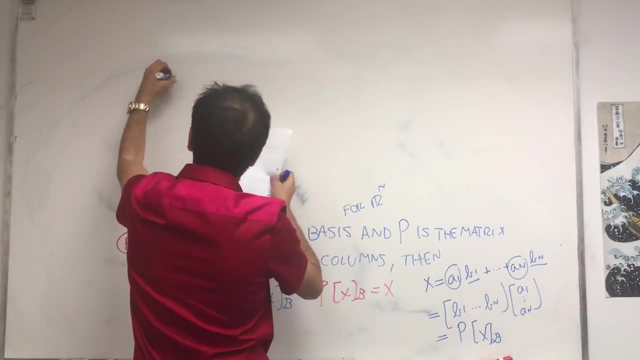 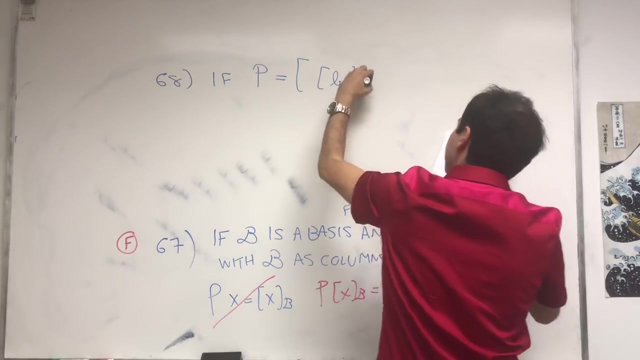 Okay now, similar to this: more change of coordinates. So we have a matrix of b1,, b2,, b3,, b4,, b5,, b6,, b7,, b8,, b9,, b10,, b11,. b12,, b13,, b14,, b15,, b16,, b17,, b18,, b19,, b20,, b21,, b22,, b23,, b24,, b25,, b27,, b28,, b30,. b31,, b32,, b33,, b34,, b35,, b36,, b37,, b38,, b39,, b40,, b41,, b42,, b43,, b44,, b45,, b46,, b47,. b48,, b49,, b50,, b51,, b52,, b52,, b53,, b54,, b55,, b56,, b57,, b58,, b59,, b60,, b61,, b62,, b63,. b64,, b57,, b58,, b59,, b60,, b61,, b62,, b62,, b63,, b64,, b65,, b67,, b68,, b69,, b70,, b71,, b72,. b72,, b73,, b74,, b75,, b76,, b78,, b79,, b80,, b81,, b82,, b82,, b83,, b84,, b95,, b95,, b96,, b97,. 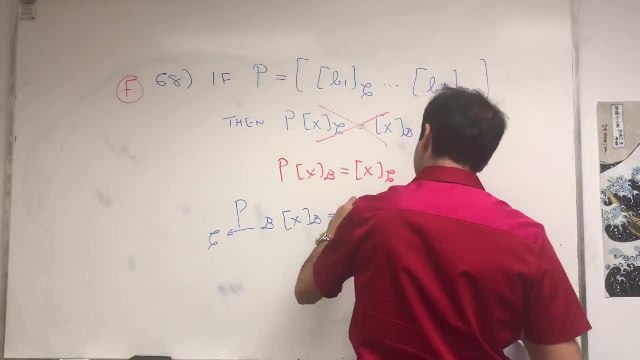 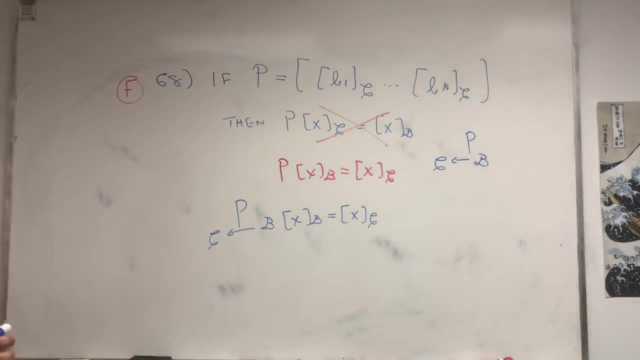 b98,, b99,, b10,, b11,, b12,, b13,, b14,, b15,, b16,, b17,, b18,, b19,, b20,, b21,, b22,, b23,, b24,. b25,, b26,, b27,, b28,, b29,, b30,, b31,, b32,, b33,, b34,, b35,, b36,, b37,, b38,, b39,, b40,, b41,. b42,, b43,, b44,, b45,, b46,, b47,, b48,, b49,, b50,, b51,, b52,, b53,, b54,, b56,, b57,, b58,, b59,. b60,, b61,, b62,, b63,, b64,, b57,, b58,, b59,, b60,, b61,, b62,, b62,, b63,, b64,, b65,, b67,, b68,. b69,, b70,, b71,, b72,, b72,, b73,, b74,, b75,, b76,, b78,, b79,, b80,, b81,, b82,, b92,, b93,, b94,. b95,, b96,, b97,, b98,, b99,, b10,, b11,, b12,, b13,, b14,, b15,, b16,, b17,, b18,, b19,, b20,, b22,. b23,, b24,, b25,, b26,, b27,, b28,, b29,, b30,, b32,, b33,, b34,, b35,, b36,, b37,, b38,, b39,, b40,. b41,, b42,, b43,, b44,, b45,, b46,, b47,, b48,, b49,, b50,, b51,, b52,, b53,, b54,, b55,, b56,, b57,. b58,, b59,, b60,, b61,, b62,, b62,, b63,, b64,, b65,, b67,, b68,, b69,, b70,, b61,, b62,, b61,, b62,. b63,, b64,, b65,, b65,, b67,, b68,, b69,, b68,, b69,, b69,, b70,, b71,, b72,, b72,, b73,, b74,, b74,. b75,, b76,, b78,, b79,, b80,, b81,, b82,, b82,, b83,, b84,, b95,, b96,, b97,, b98,, b99,, b10,, b11,. b12,, b13,, b14,, b15,, b16,, b17,, b18,, b19,, b20,, b21,, b22,, b23,, b24,, b25,, b26,, b27,, b28,. b29,, b30,, b31,, b32,, b33,, b34,, b35,, b36,, b37,, b38,, b39,, b40,, b41,, b42,, b43,, b44,, b45,. b46,, b47,, b49,, b50,, b51,, b52,, b53,, b54,, b56,, b57,, b58,, b59,, b59,, b60,, b61,, b62,, b62,. b63,, b64,, b65,, b67,, b68,, b69,, b70,, b71,, b72,, b72,, b73,, b74,, b75,, b76,, b78,, b79,, b80,. b81,, b82,, b82,, b93,, b84,, b95,, b96,, b97,, b98,, b99,, b10,, b11,, b12,, b13,, b14,, b15,, b16,. b17,, b18,, b19,, b20,, b21,, b22,, b23,, b24,, b25,, b26,, b27,, b28,, b29,, b30,, b32,, b33,, b34,. b35,, b36,, b37,, b38,, b39,, b40,, b41,, b42,, b43,, b44,, b45,, b46,, b47,, b48,, b49,, b50,, b51,. b52,, b53,, b54,, b55,, b56,, b57,, b58,, b59,, b60,, b61,, b62,, b62,, b63,, b64,, b65,, b67,, b68,. b69,, b70,, b71,, b62,, b62,, b33,, b34,, b45,, b46,, b47,, b48,, b49,, b50,, b51,, b52,, b53,, b54,. b55,, b56,, b56,, b57,, b58,, b59,, b59,, b60,, b61,, b62,, b63,, b54,, b56,, b57,, b58,, b59,, b60,. b61,, b62,, b62,, b63,, b64,, b65,, b67,, b68,, b69,, b70,, b71,, b72,, b72,, b72,, b73,, b74,, b74,. b75,, b68,, b78,, b79,, b80,, b80,, b81,, b82,, b83,, b84,, b95,, b96,, b97,, b98,, b90,, b91,, b92,. 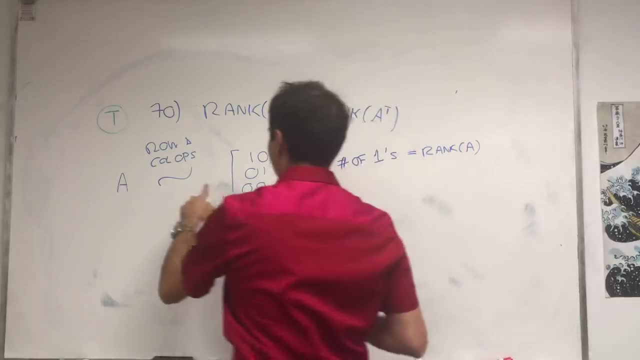 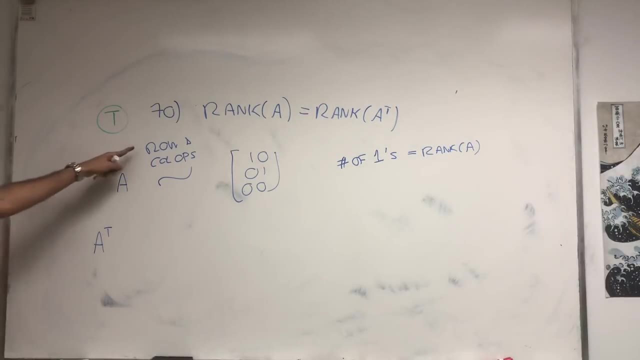 b93,, b94,, b95,, b95,, b96,, b97,, b97,, b00,, b00,, b00,, b10,, b10,, b11,, b12,, b13,, b14,, b15,. 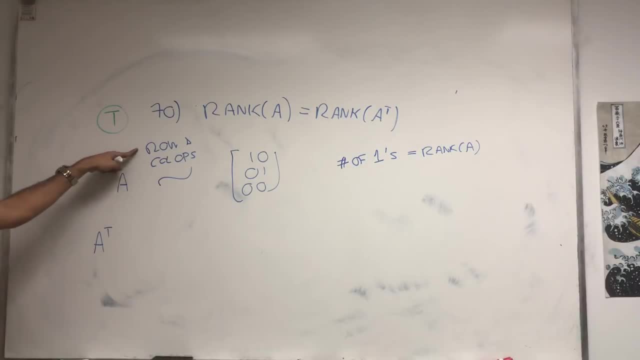 b16, b17,, b17,, b18,, b20,, b21,, b22,, b24,, b25,, b25,, b26,, b27,, b27,, b28, b29,. means that, using column operations and row operations, we can transform it into: 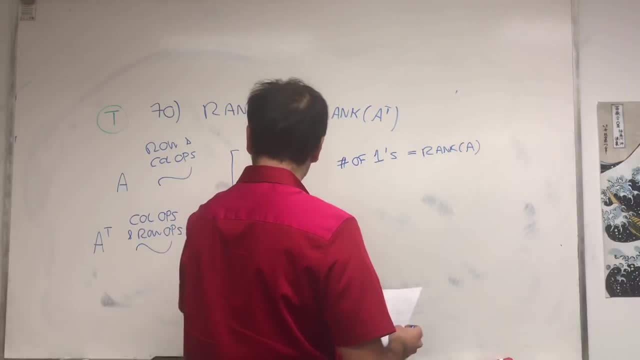 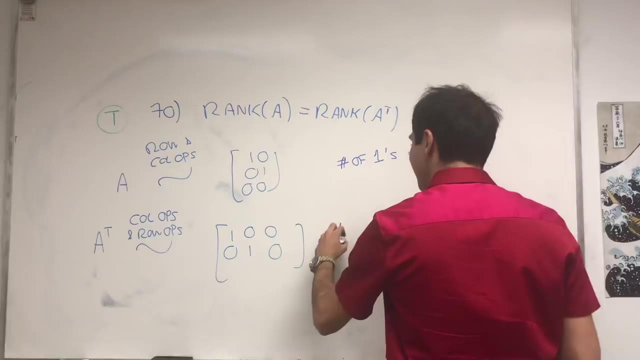 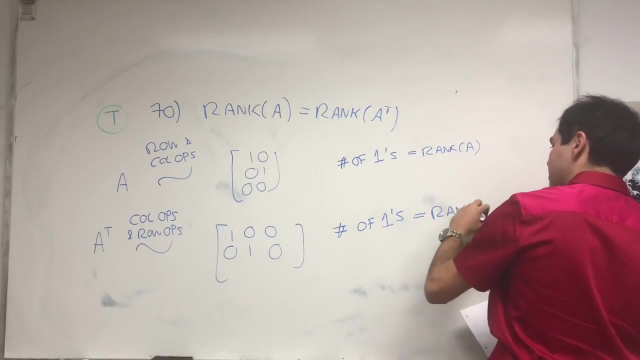 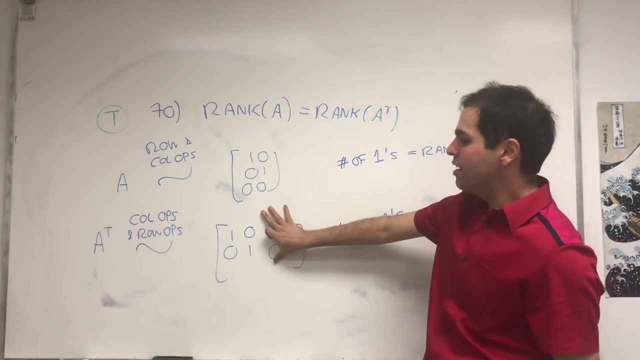 something similar: one zero zero, one zero zero. basically the same matrix, but transpose. so really, by definition of this theorem, so the number of ones, well, that's by definition the rank of a transpose. but because those matrices are exactly the same thing but flipped, the number of ones, well, it's also equal to. 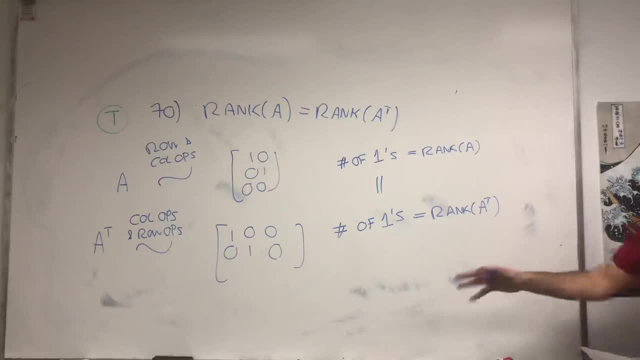 the number ones of a. you see, the number of ones don't really change because we applying the exact same transformations, you see, and that's why the rank of a is equal to the rank of a transpose. so this is true. how cool is that? and again, that's by using column operations as well. so be careful. 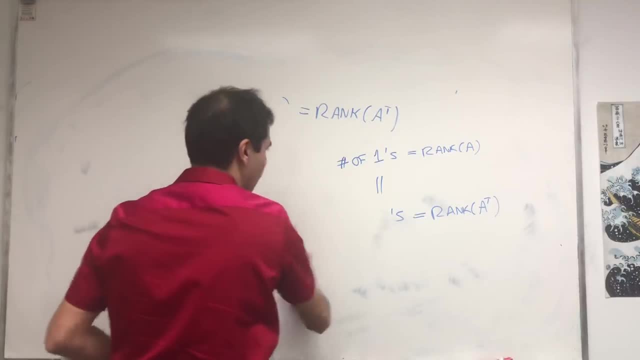 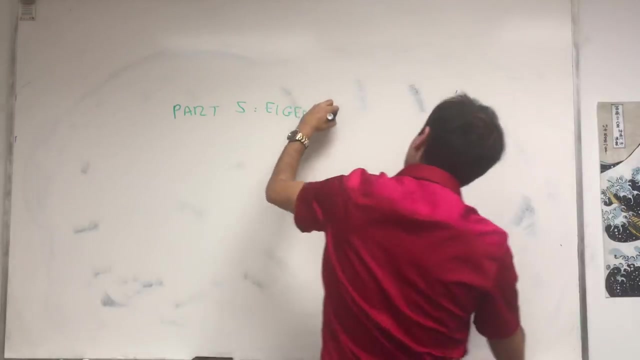 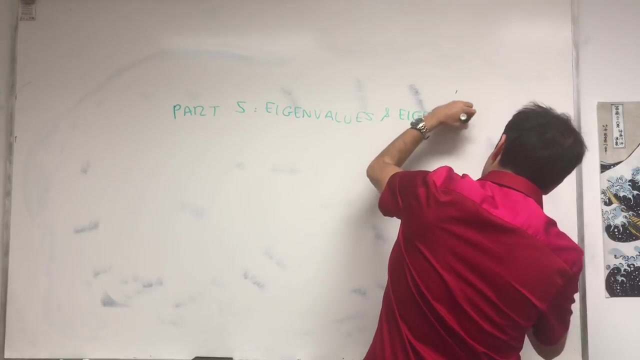 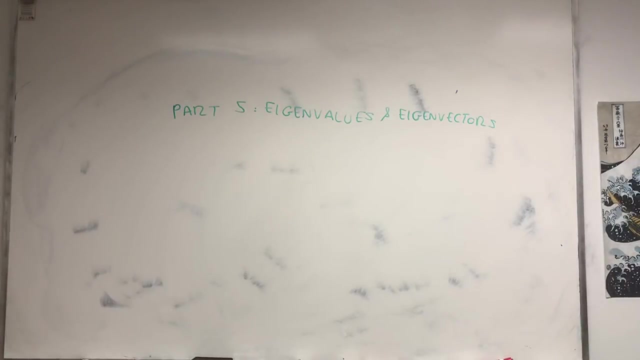 okay, And with this we are done with the fourth part, and now let's move on to eigenvalues and eigenvectors. woo, So part five, eigenvalues and eigenvectors. Let me check again if everything is okay. Yup, life is still good. so we still have, I think, memory. 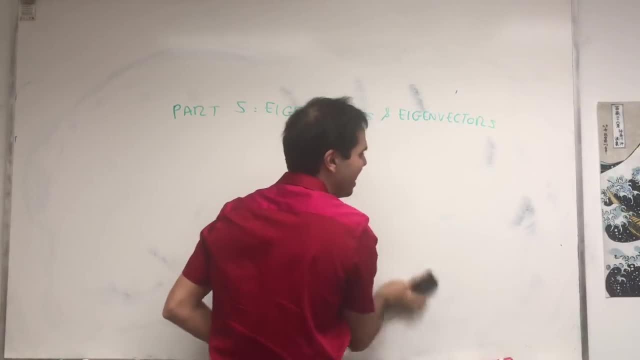 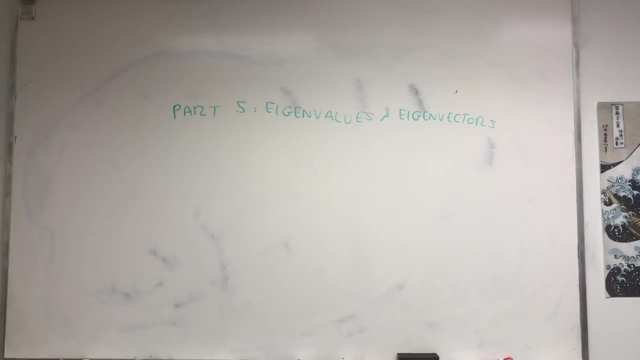 Eigenvalues and eigenvectors, because if I can do it, so can you. Let me eat some nuts more sorry, I feel. Okay. so next question: Okay, we're almost at the three hour mark, so let's see. 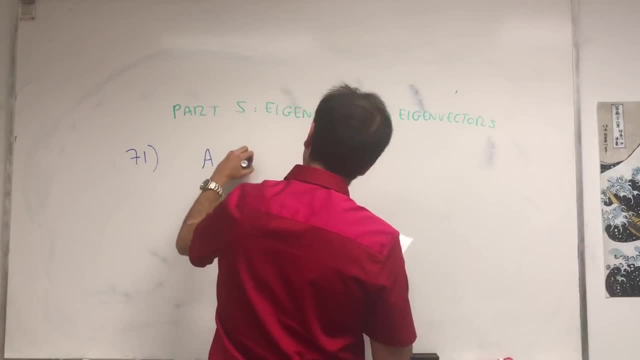 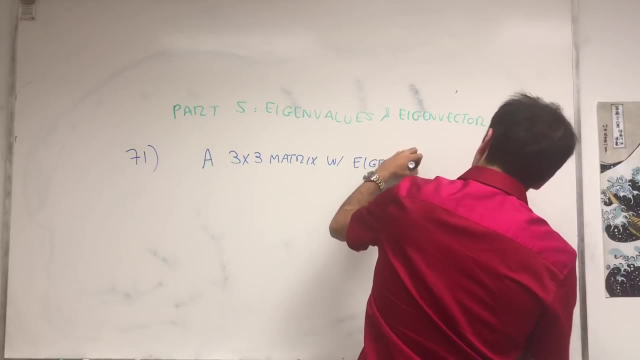 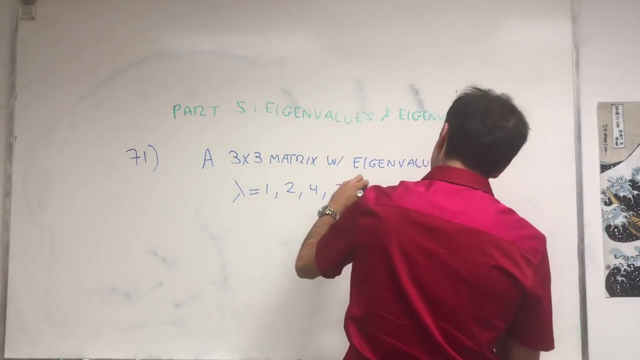 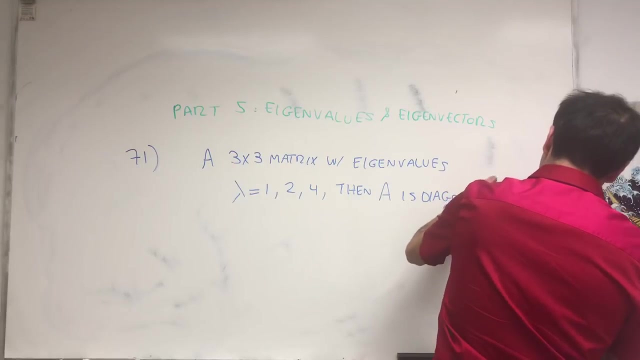 So I'm gonna do one. If A is a three by three matrix with eigenvalues one, two and four, then A is diagonalizable, Diagonalizable, And A is the diagonal And language. 71, Haryanvi. 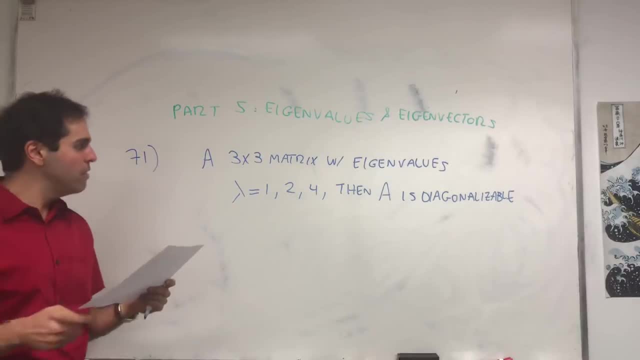 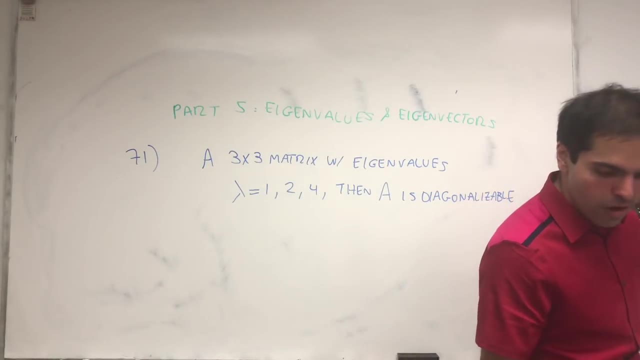 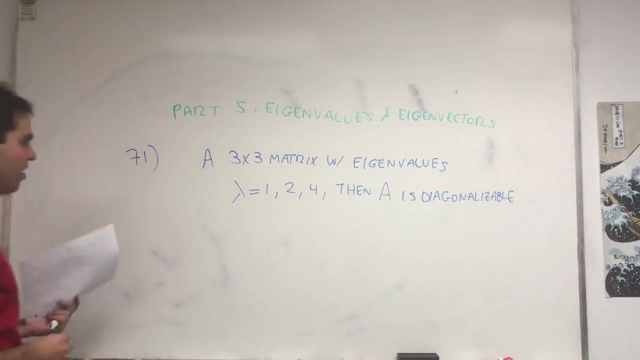 So I think a dialect of Hindi maybe. and 71 is Ikadav. Okay, That's the all. Not long, No, not too bad. Okay, So if you have three eigenvalues, different eigenvalues, and you have a three by three matrix, 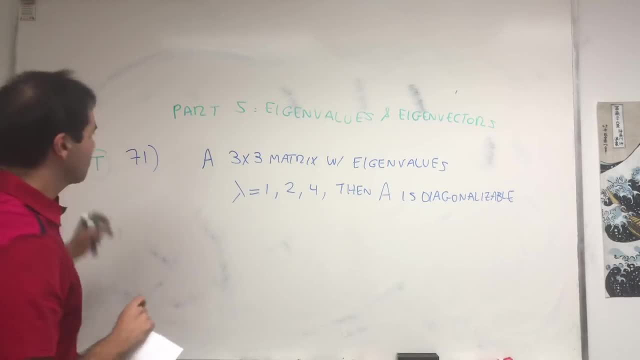 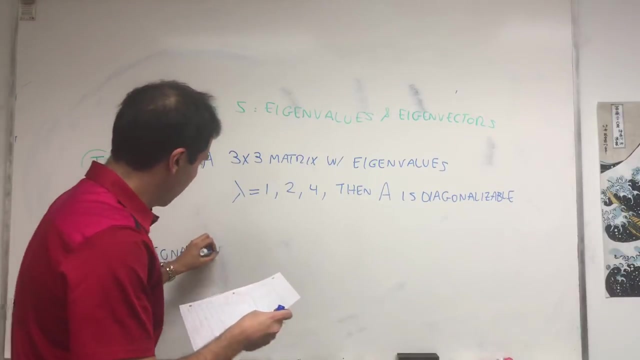 is it diagonalizable? Well, you bet it is. But remember very important to check: if a matrix is diagonalizable, you really have to look at the eigenvectors. So diagonalizable if, and only if, you have three linearly independent. 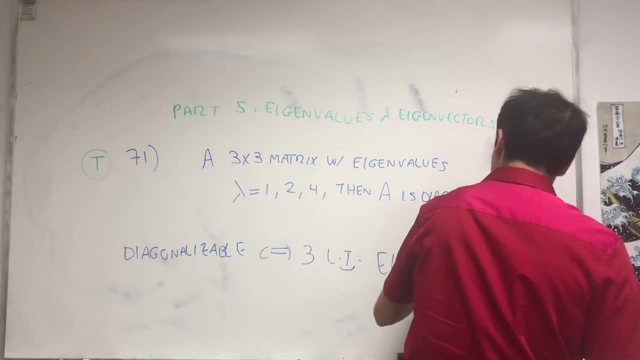 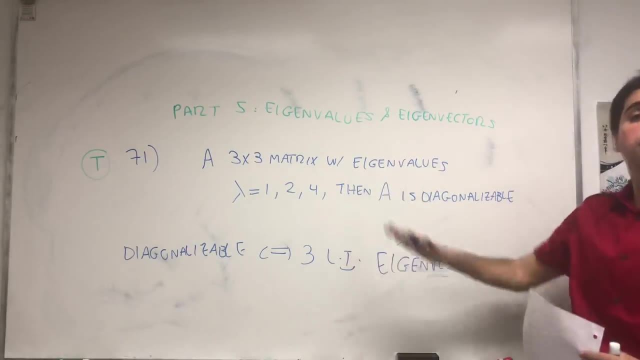 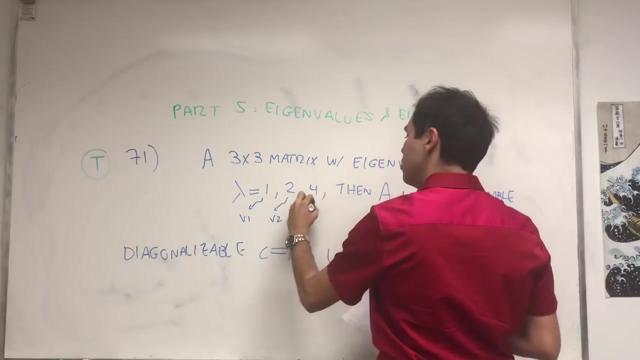 eigenvectors. so that is like the ultimate test of diagonalizability. If you have three different eigenvalues, then look, you get an eigenvector with one, an eigenvector with two and an eigenvector with four. 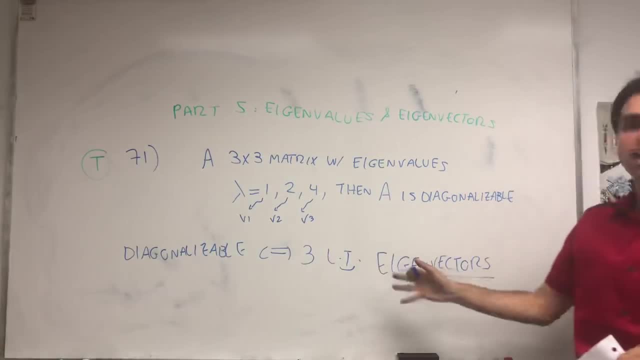 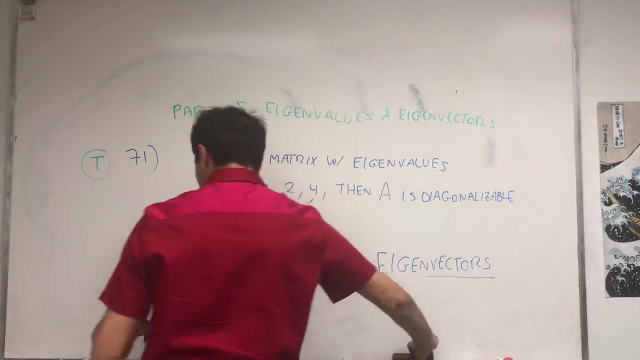 And there's this beautiful theorem that says those will be automatically linearly independent. So because you have an eigenvector for each eigenvalue, you do have three linearly independent eigenvalues, And therefore you're good. Okay, but now 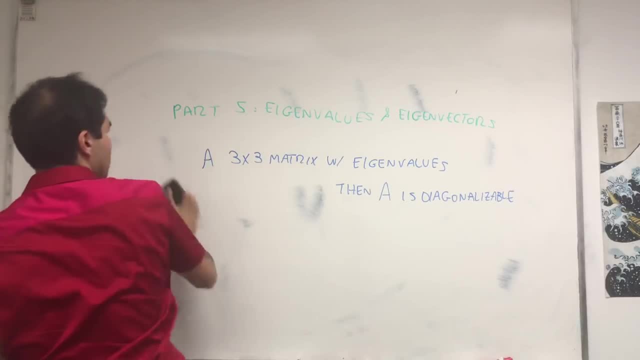 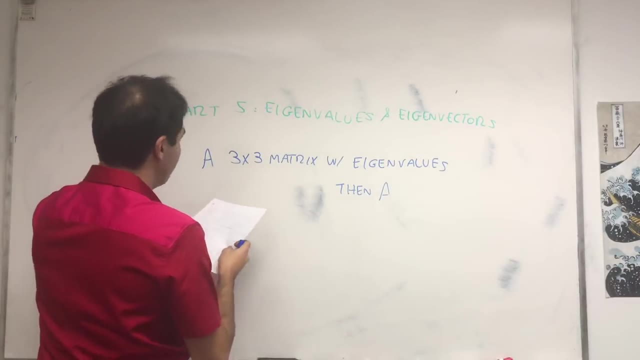 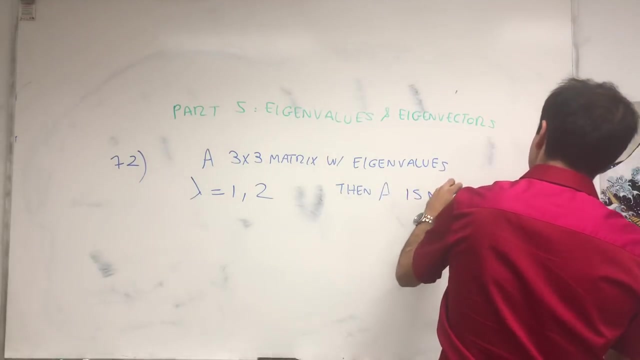 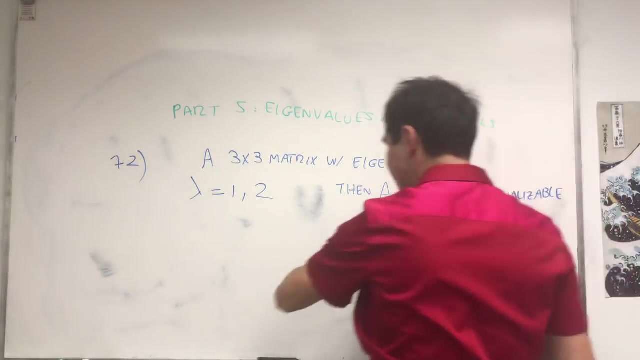 let's do the same thing. But what if some eigenvalues are repeated, So 72,. if A is a three by three matrix with eigenvalues one and two, then A is not diagonalizable And 72 is a more body. so maybe Hindi, a dialect of Hindi? not sure. 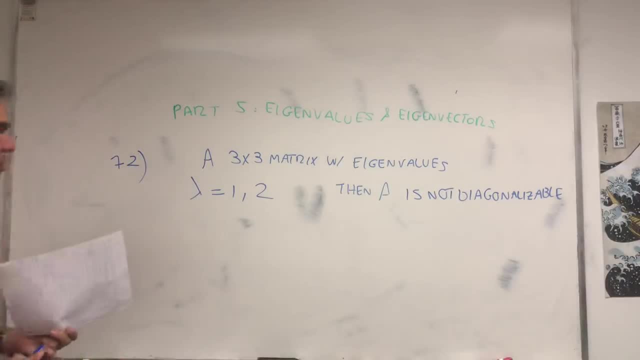 and 72 is Bahadur, So almost like it's better but it's Bahadur. And again, very important to check if a matrix is diagonalizable or not, you have to look at the eigenvectors, just because it has. 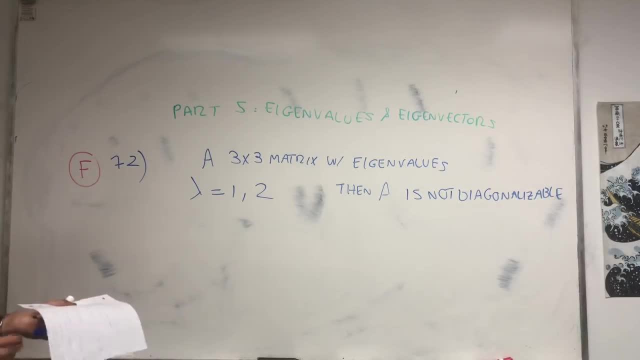 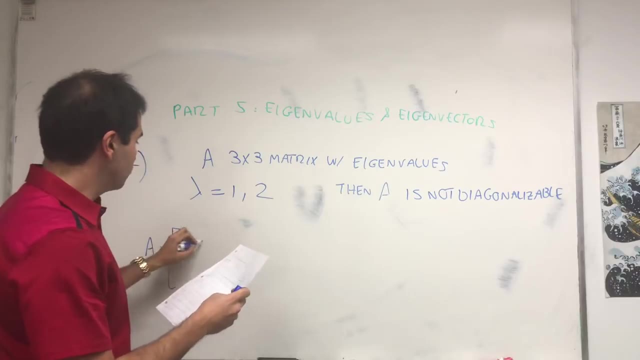 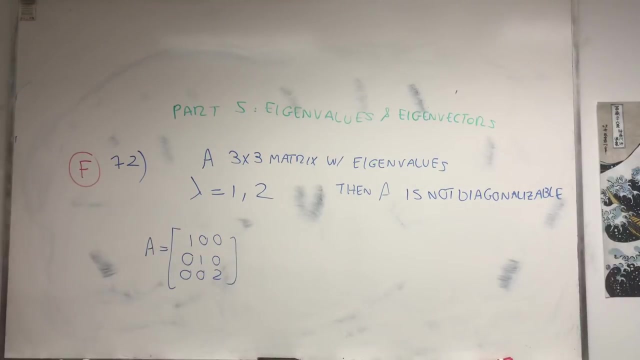 two eigenvalues doesn't mean it's not diagonalizable And, in fact, out of a defaulting matrix A which is one zero zero zero one, zero zero zero two. Well, you can check that the eigenvalues are one and two. 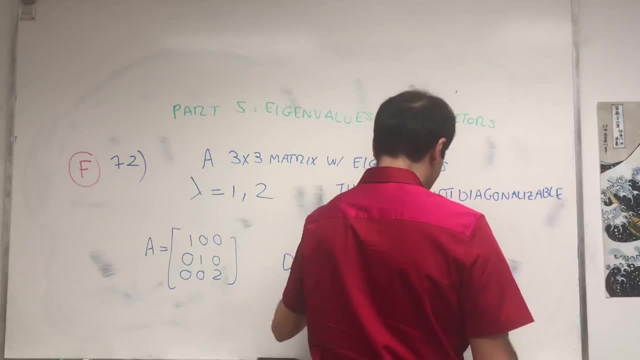 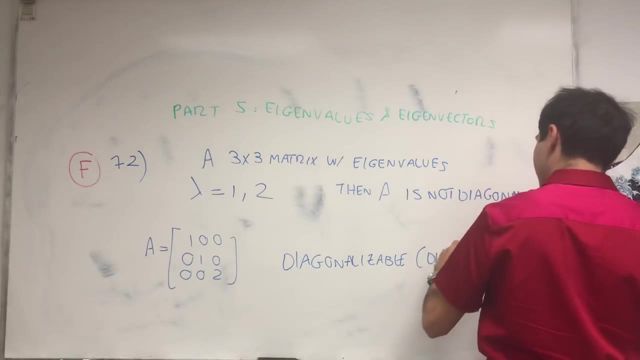 but it is diagonalizable because it's diagonal. I know it confuses a lot of students because they just use that definition, but remember, diagonalizable means it can be turned into a diagonal matrix. Well, if it's already diagonal, then surely it can be turned into a diagonal matrix. 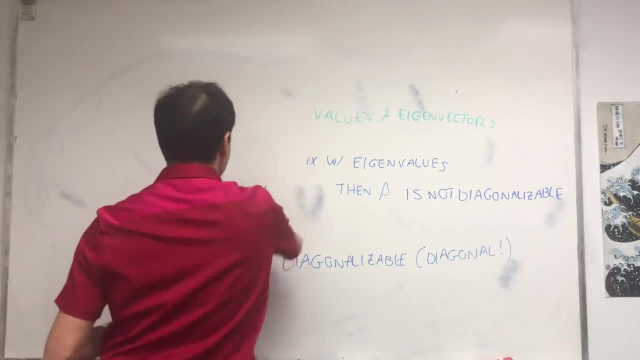 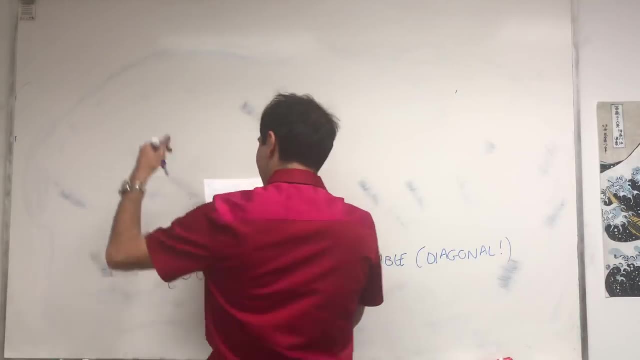 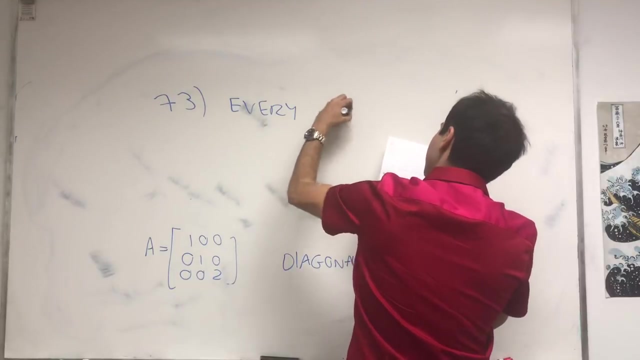 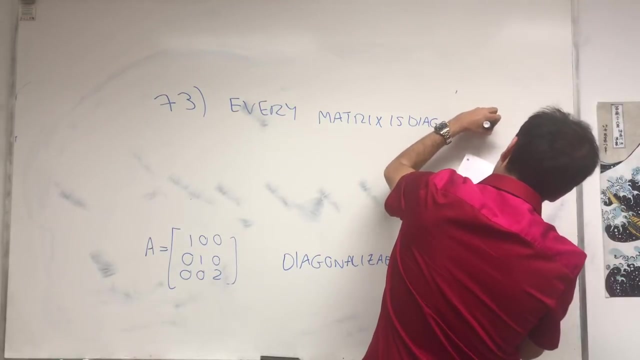 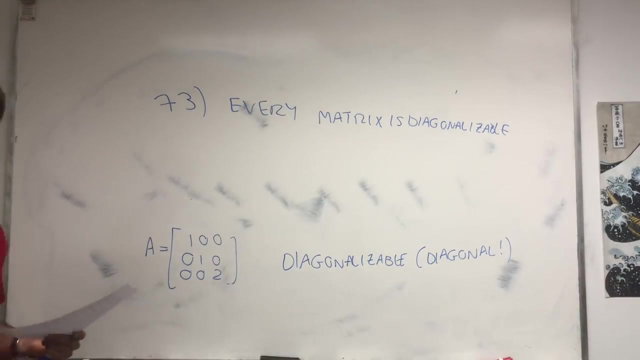 So that is okay. Well, now, of course you may wonder: is every matrix diagonalizable? Because surely not every matrix is diagonal. but let's see, Every matrix is diagonalizable. And the 73rd most popular language- I think one of the hardest languages- is Czech. 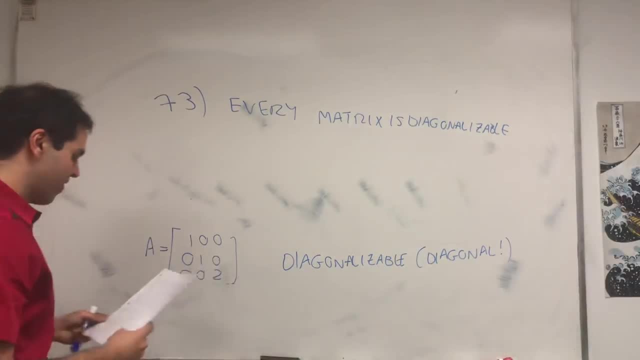 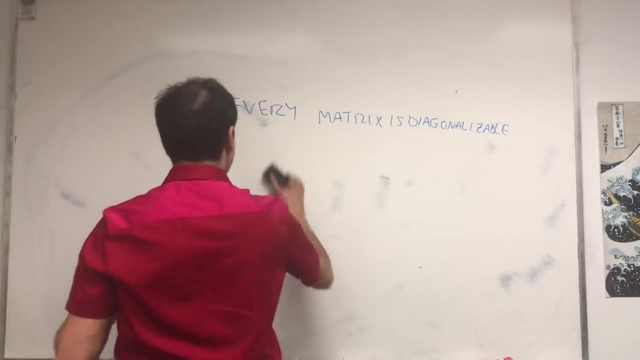 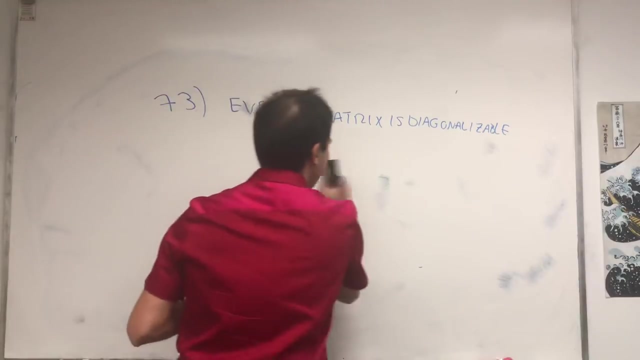 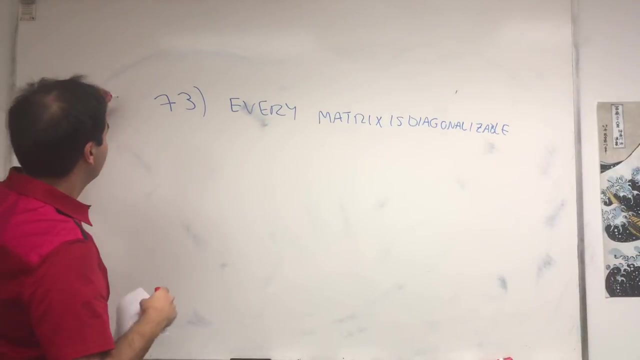 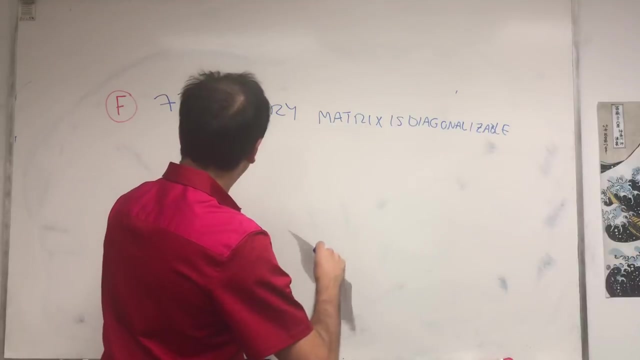 and it's, or Our friends, you know, from our neighbors, from Austria. Sadly, every matrix is not diagonalized. So not every matrix is diagonalizable. And let me give you the most important example, which is one one, zero one. 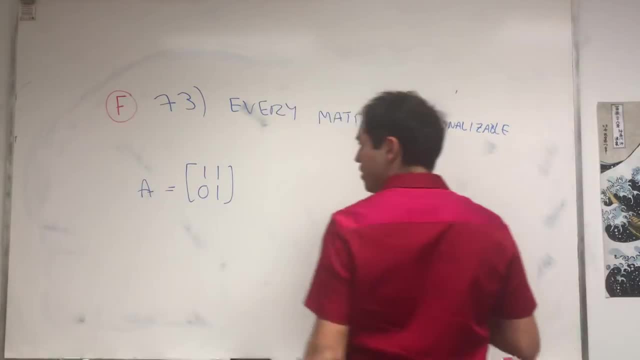 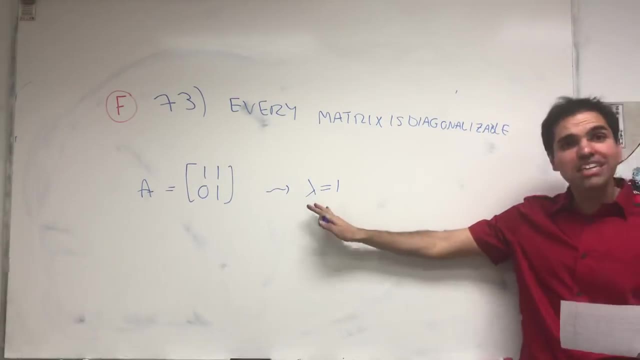 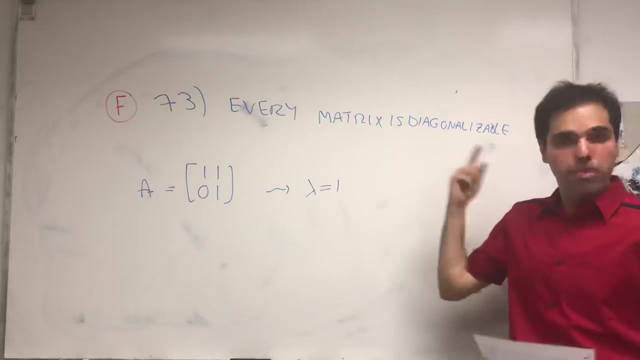 And if you find the eigenvalues we get lambda equals one, But careful, this does not mean it's not diagonalizable. It's possible that you have one eigenvalue and it's still diagonalizable. Think like the identity matrix. You really have to look at the eigenvectors. 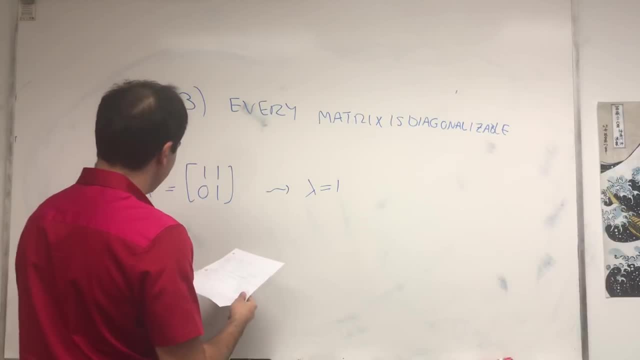 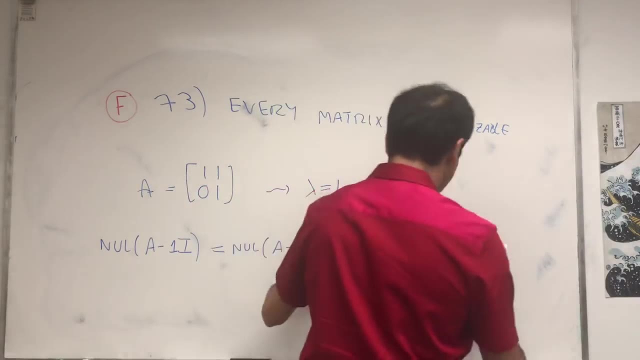 to check if it's not. And now so, null space of A minus one I. well, that's null space of A minus I, And that's a null space of, in this case, zero one, zero, zero. 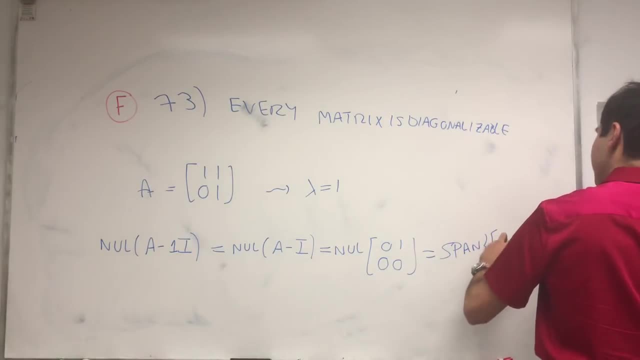 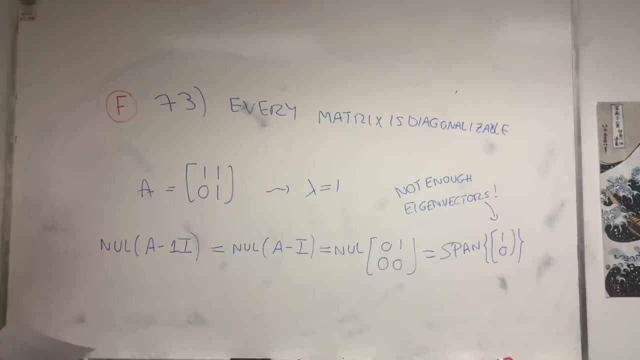 And if you find the null space, you get that it's a span of one zero. So you see, for this matrix there are not enough eigenvectors. So there are basically not enough eigenvectors to construct this matrix. matrix P with A equals PDP inverse. 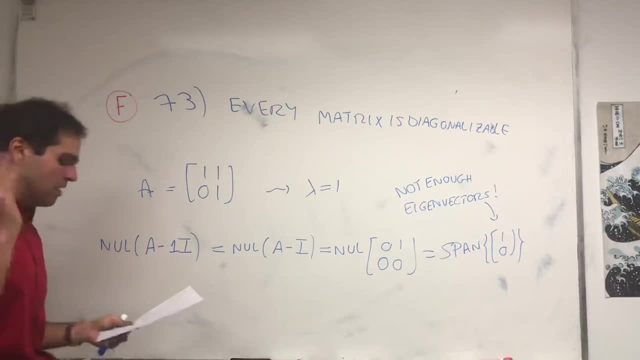 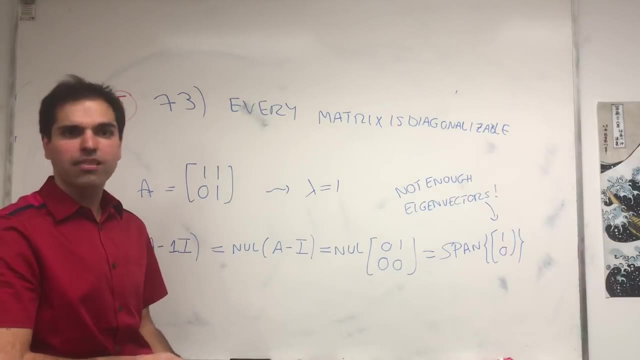 And that's why this matrix is not diagonalizable. So again, just to show that the matrix is not diagonalizable, you really have to look at the eigenvectors. If there's not enough, then it's not diagonalizable. If there are enough eigenvectors, then you're good. 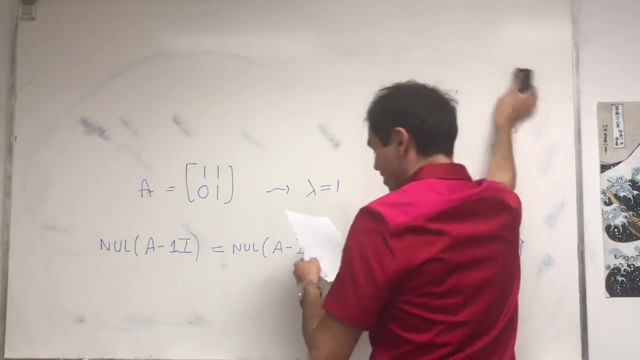 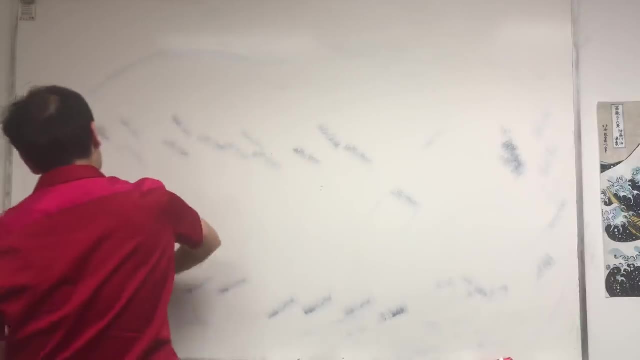 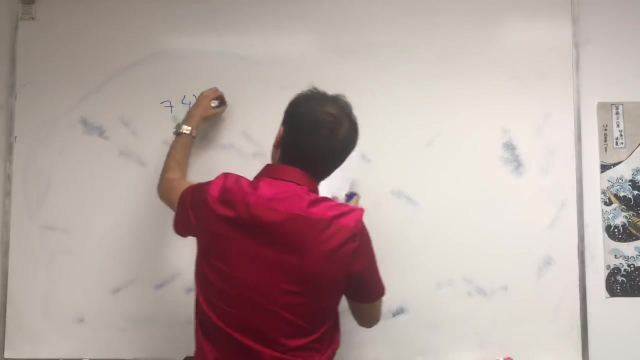 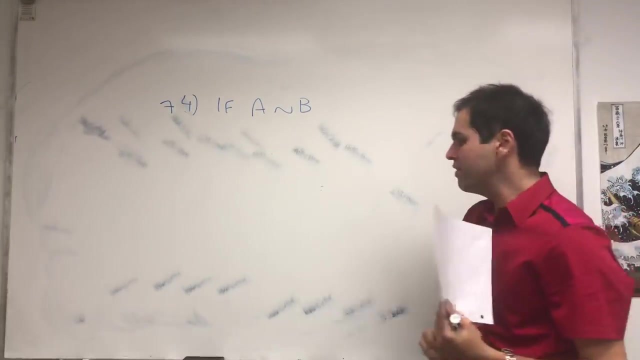 OK, Now let's do a couple of questions with similarity. So this one is cute. So if A is similar to B, so very important, before I use squiggle to say rho equivalent, this time I mean I use squiggle for similar. 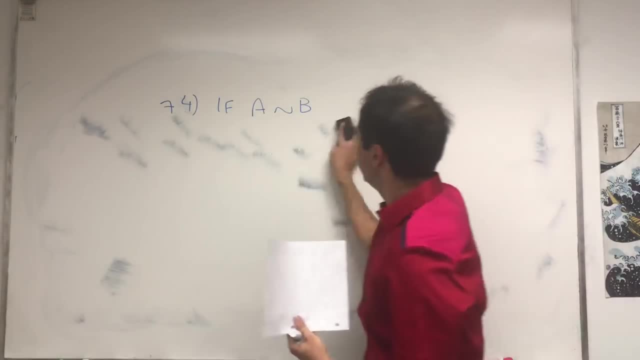 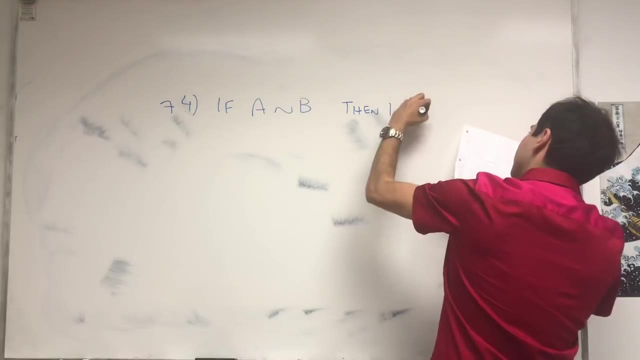 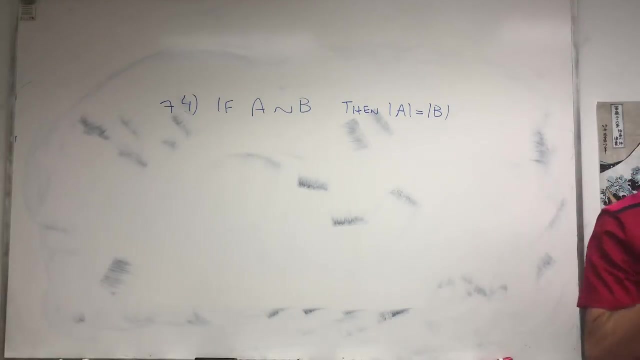 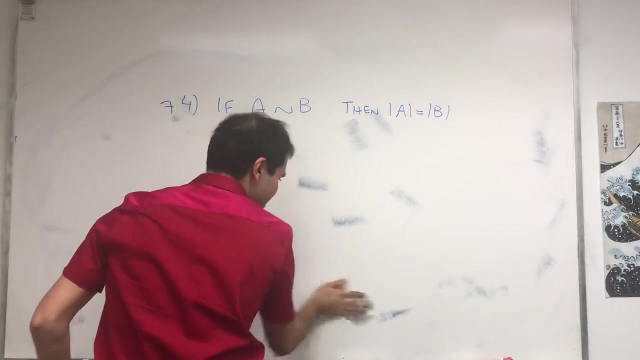 So if A is similar to B, then they have the same determinant. the determinant of A- squiggle happy, OK, That's quick- equals the terminate of b and dying. by the way, everything hurts again. gotta do it. I think it's one of the things you gotta do once in your life. oh, maybe. 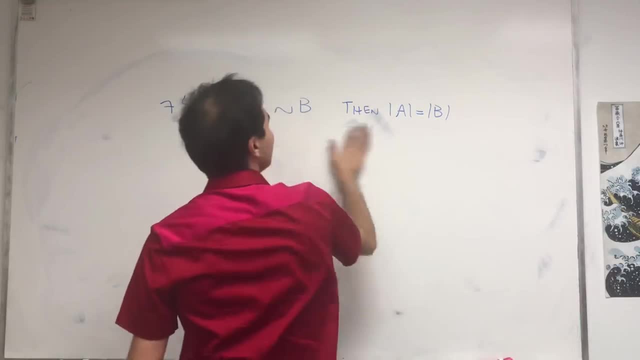 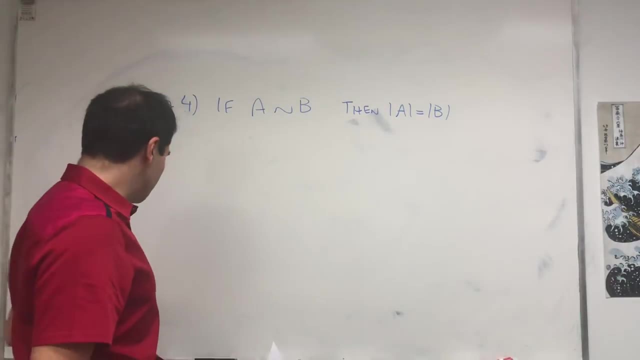 again. let's see. I'm sure tomorrow I'll wake up. I'm like, ah, this was fun, let's do another one. so if a is similar to b, then the determinant of a is equal to the determinant of b. indeed, this is true. and 74th language, ah. 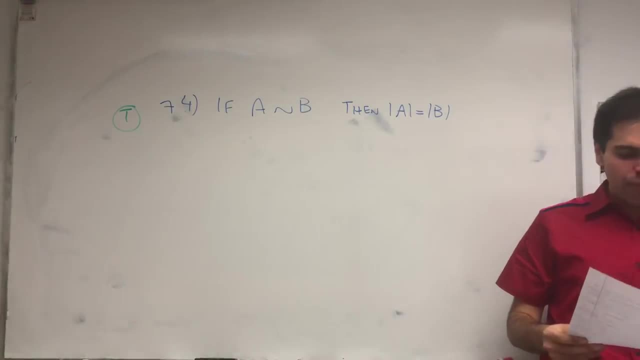 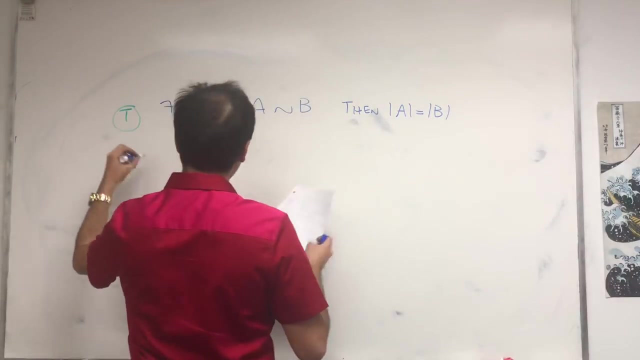 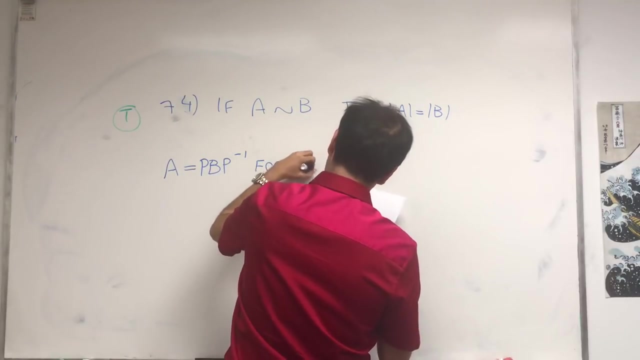 Calimero, it's Greek and it's evdomita tessera. as I said, it's true, because a similar to b means a equals to pb, p-inverse, and for some p, and then that just means the terminal a is the determinant of p, b, p. 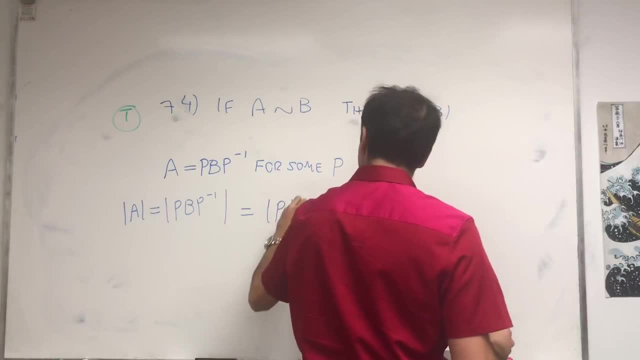 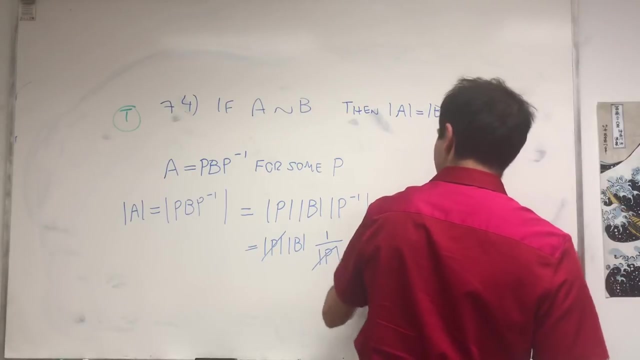 inverse determinant is multiplicative. so the terminal of p, the terminal of b, determinant of p inverse, and that's the terminal of p, the terminal of b, the terminal of p inverse is 1 over the terminal of p. boom, boom. this cancels out and you get the determinant of b. 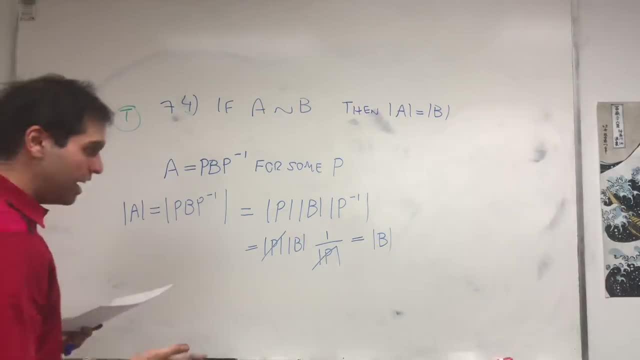 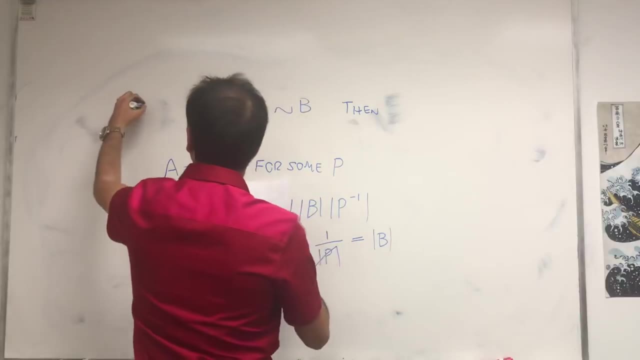 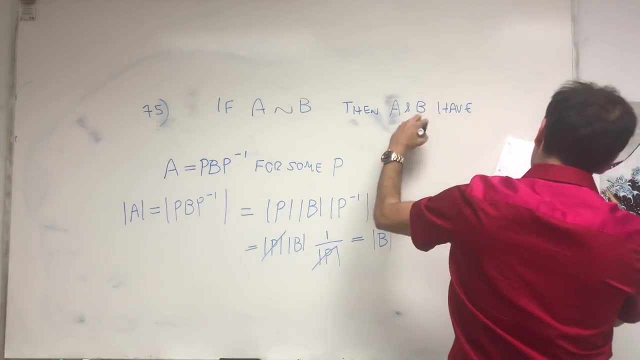 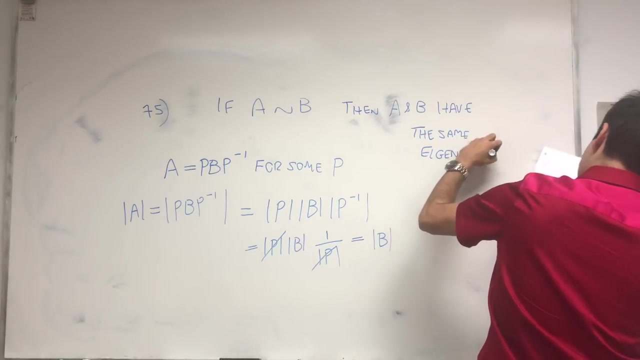 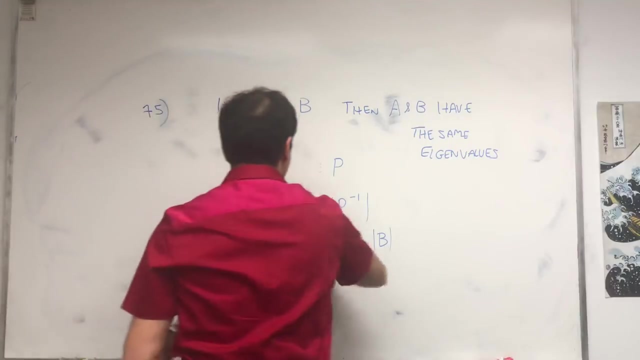 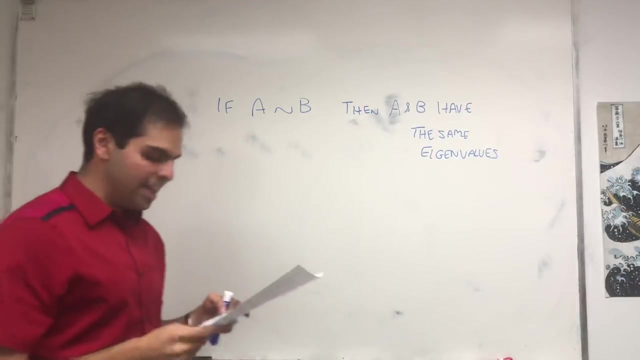 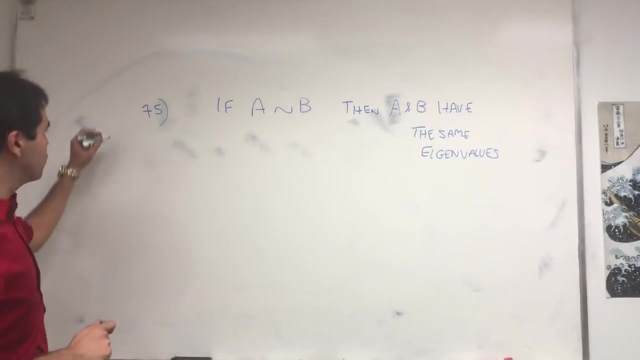 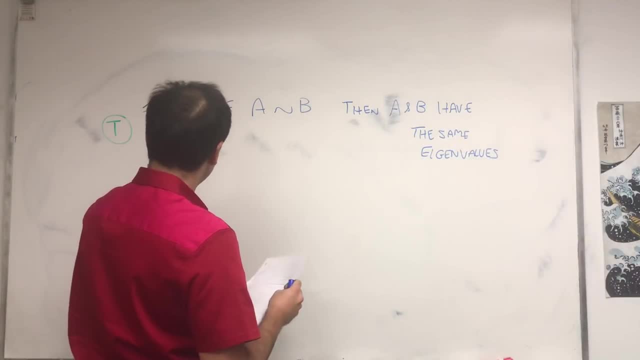 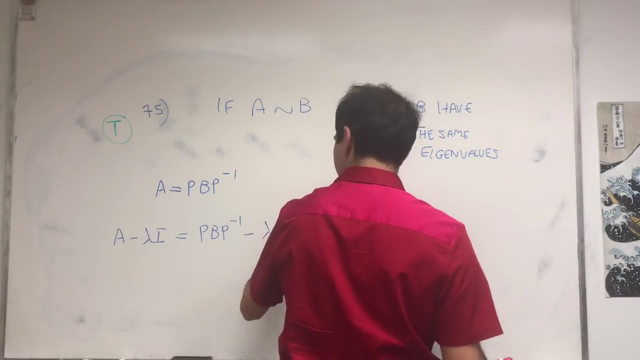 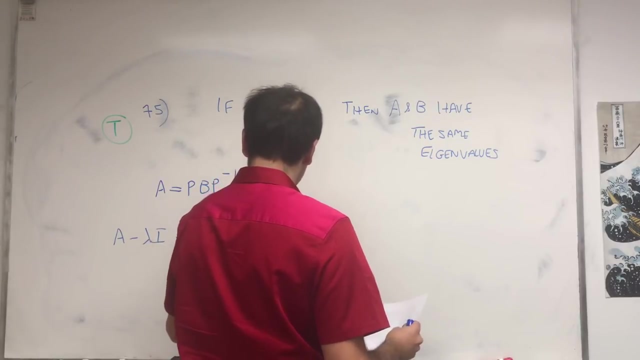 magic spell or something, and a is pbp inverse. and then let's look at a minus lambda i, that's pbp inverse minus lambda. and then let's write this as pp inverse, because then we can just factor out p, pb, p inverse minus lambda p inverse, but that's just p, and now we can factor out p inverse. 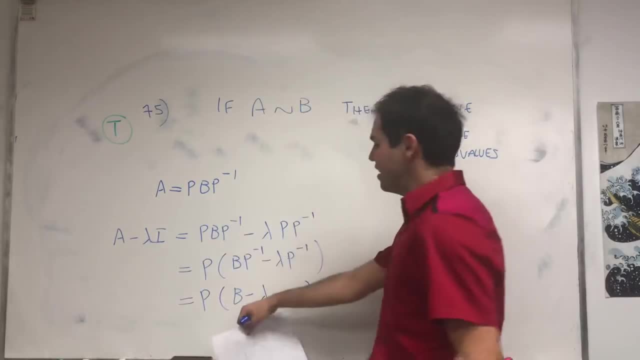 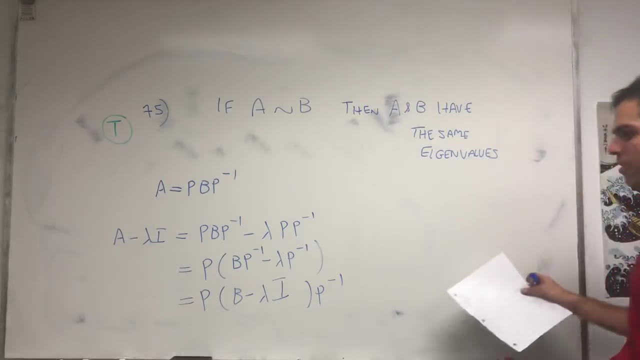 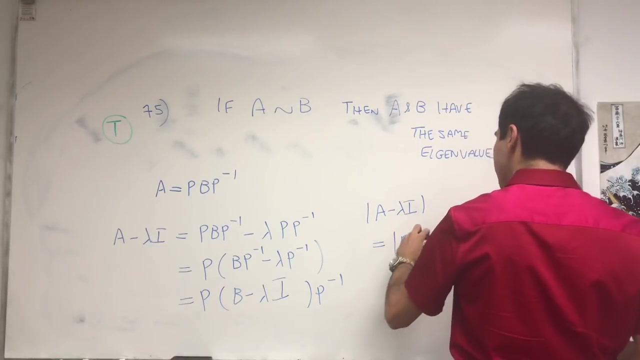 and b minus lambda. but it doesn't make sense to subtract a constant from b. what they really mean is lambda i and, in particular, if you take the determinant of a minus lambda i, that's the determinant of p, b minus lambda i, p inverse, and that's really- uh again, determinant of p. 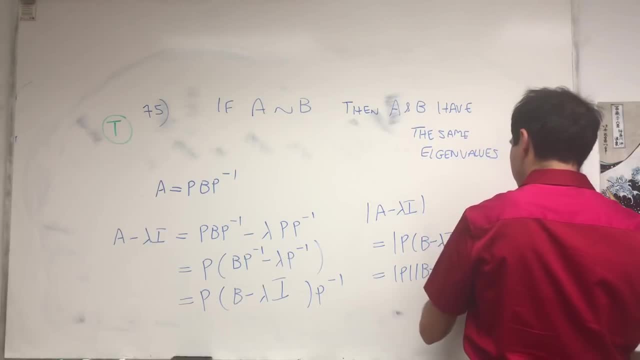 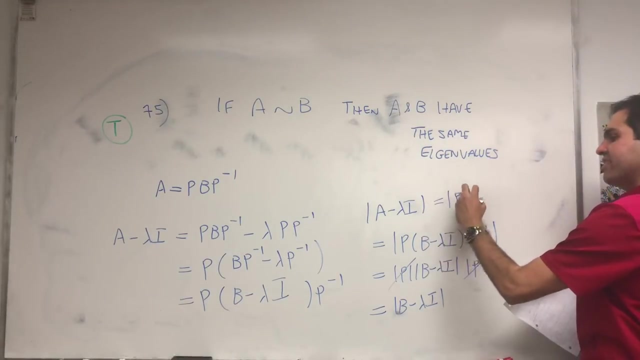 determinant of b minus lambda i. determinant of p- inverse pbp- but similar to before. ah, similar, we can cancel it out. so this is the determinant of b minus lambda i. in particular, the characteristic equations of a and b are the same, so if one of them is zero, then the other one is zero, and the one one, this one- is zero, then the other one. 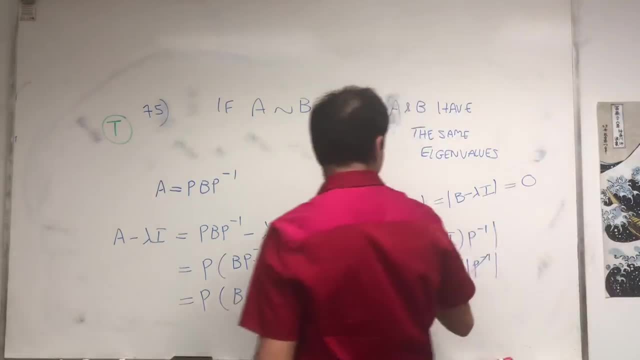 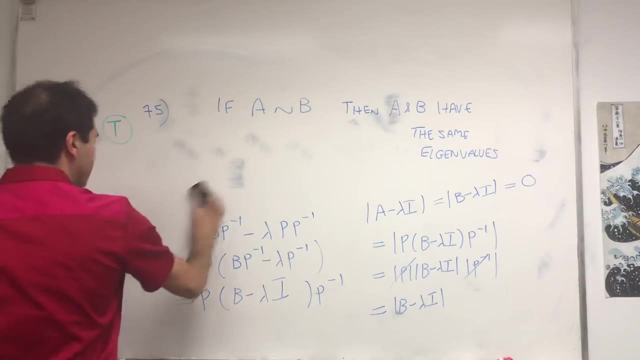 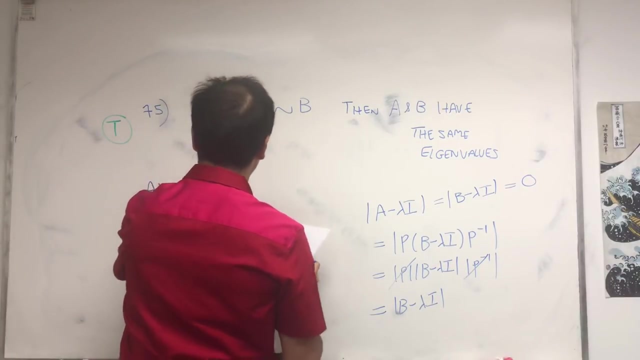 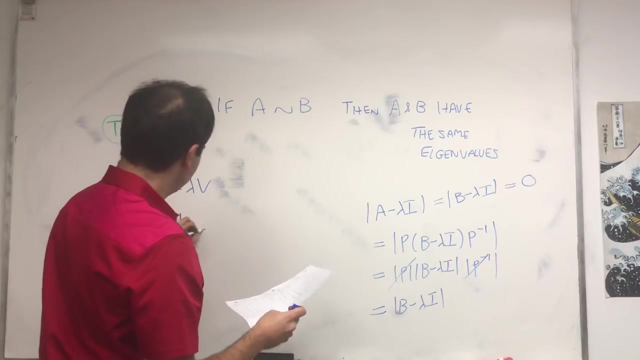 is zero. so if lambda is an eigenvalue of a, then lambda is an eigenvalue of b, and vice versa. okay, if you didn't like this, there's another way. so if a suppose lambda is an eigenvalue of a, so av equals to lambda v. that just means pbp inverse. v is lambda v. so multiplying by p inverse we get bp. 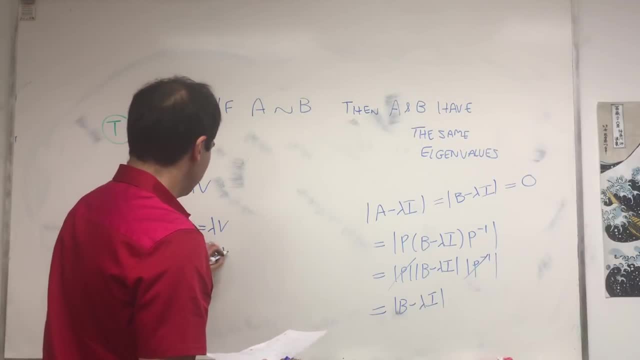 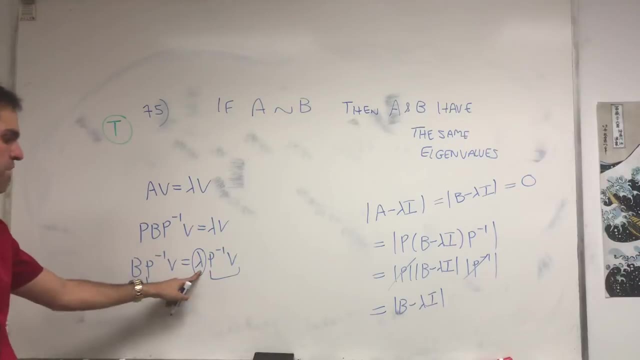 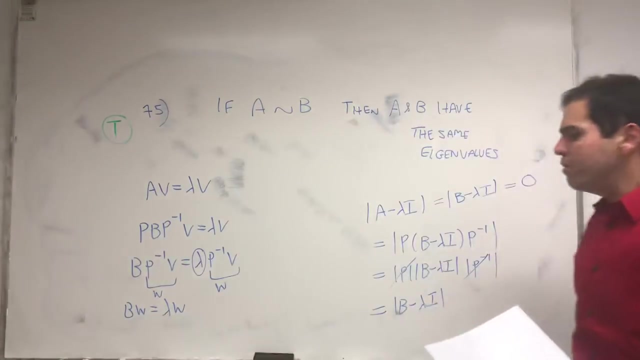 inverse v is lambda at p inverse v. but that just means that lambda is an eigenvalue of b, because you know, if you let this to be w, you get bw equals to lambda w, and if v is non-zero and p is invertible, then p inverse v is also non-zero. so we do get that. 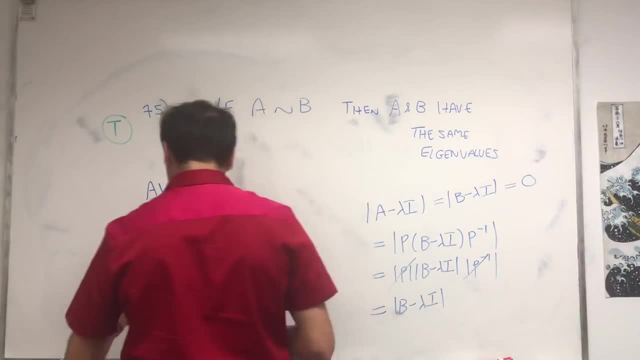 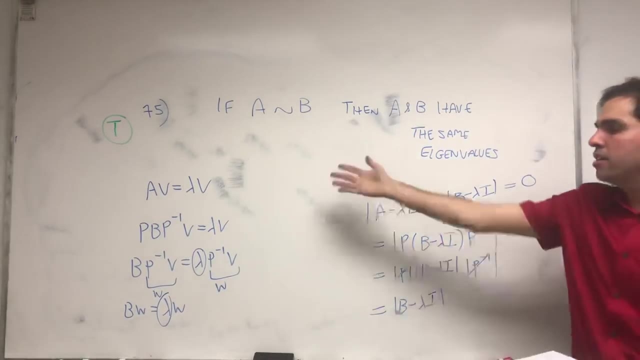 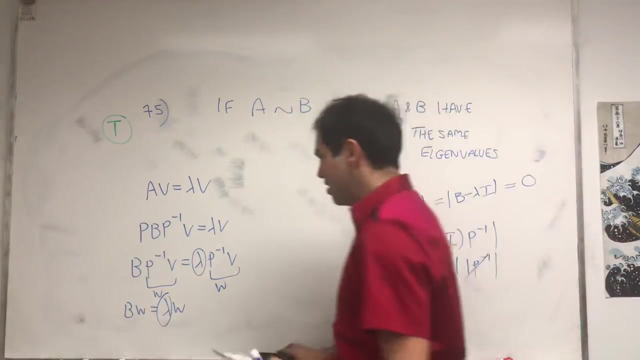 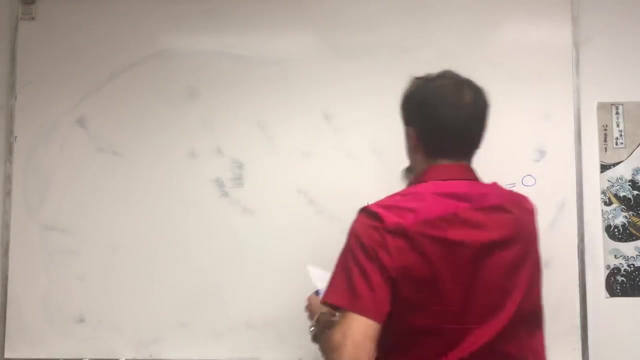 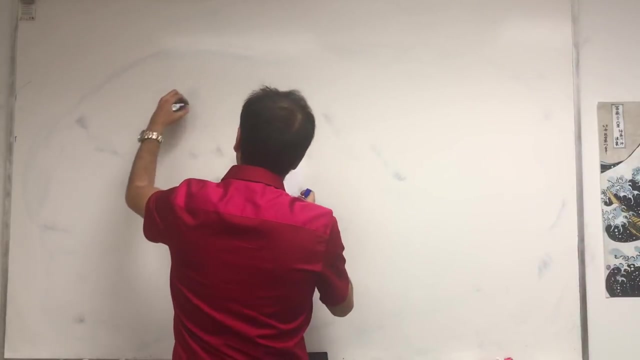 lambda is an eigenvalue of b and and similarly we can also assume lambda is an eigenvalue of b. in the same way, we can show that lambda is also an eigenvalue of a, so this is true in particular. i can keep that in mind. is it true or not that the determinant of a is the product of the eigenvalues of a? 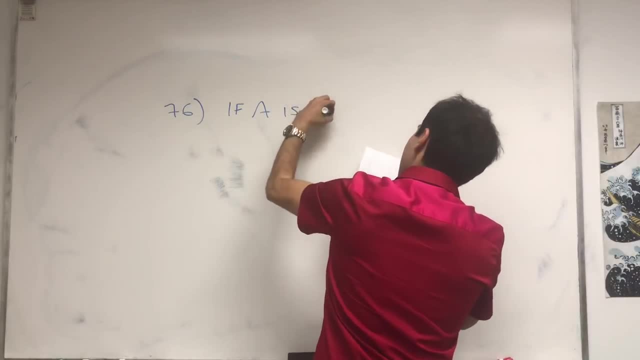 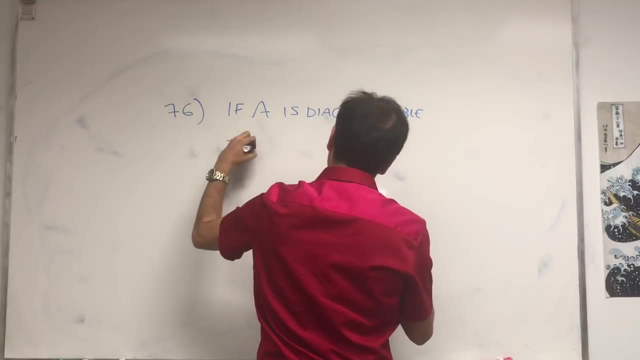 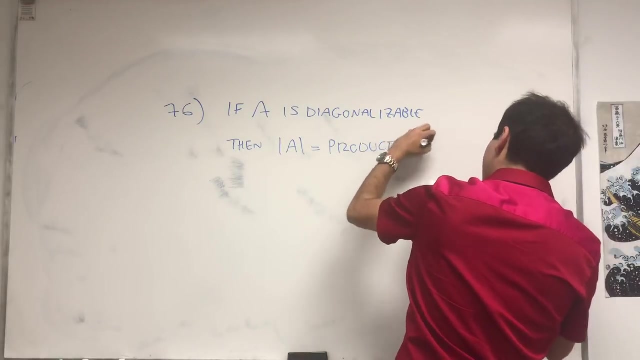 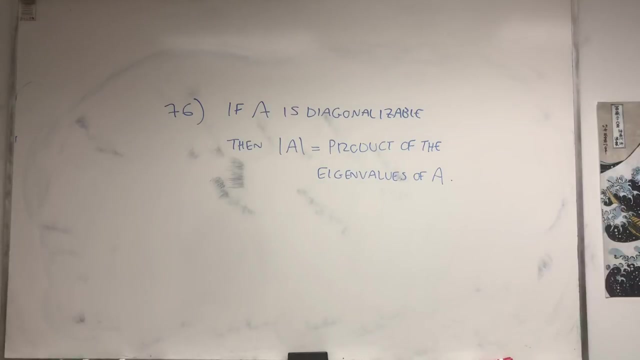 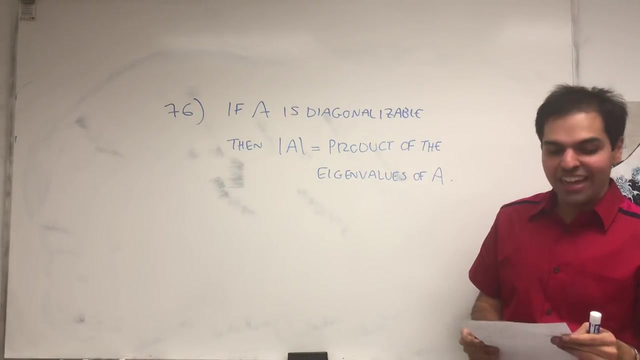 and let's say, if a is diagonalizable, then a determinant of a is the prada, so the product of the eigenvalues. okay, so, and good language. 76. oh, my god, i think the language is harder to pronounce in the number. chatis, carhi, chatis. 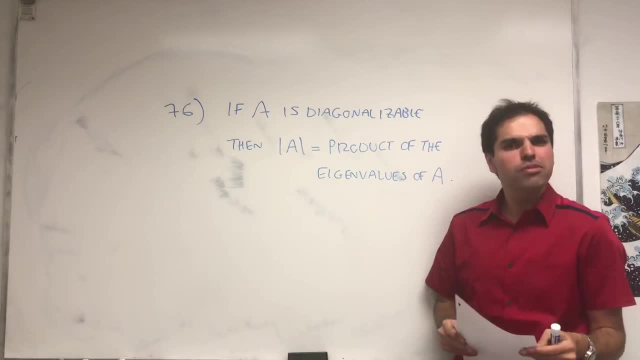 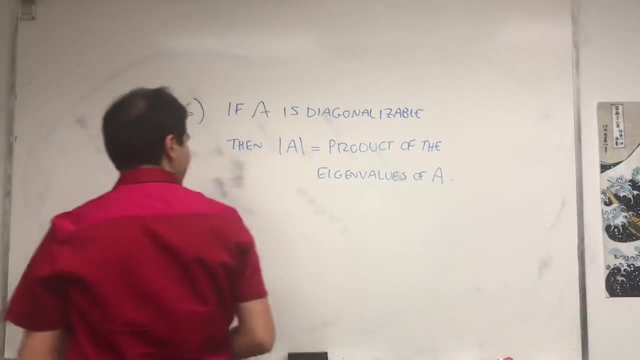 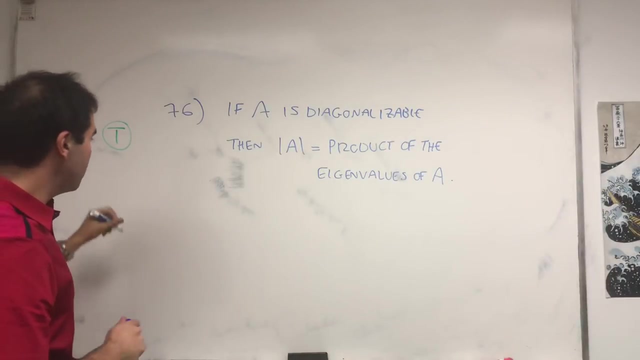 carhi, carhi, and it's, i think, a version of hindi, not sure, and 76 is all right, and indeed this is true. it follows from the previous thing because, look, if a is diagonalizable, a is pdp inverse, and we've just shown before that the determinant of a 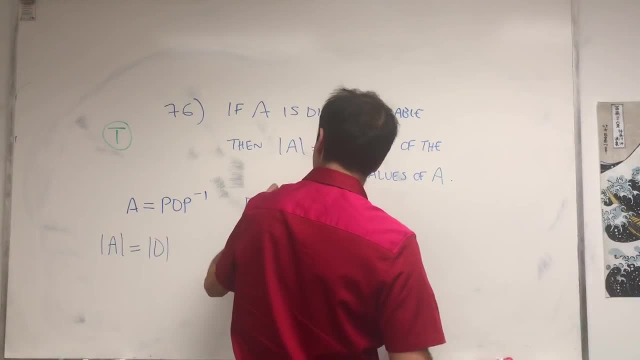 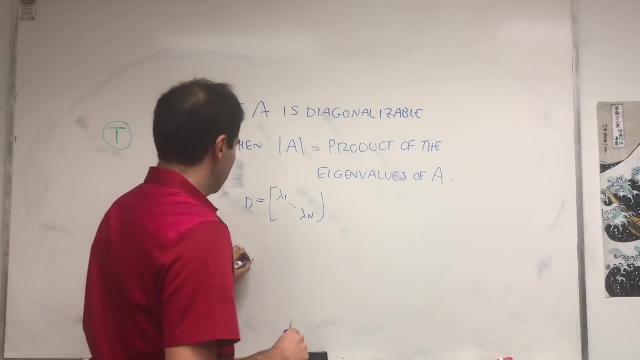 is the determinant of d? but look, d is the matrix of eigenvalues: lambda 1, lambda 2, lambda n, lambda 3, lambda 1- and the determinant is just a product. this Antwort butา protein. so the determinant is the product of the eigenvalues of a. 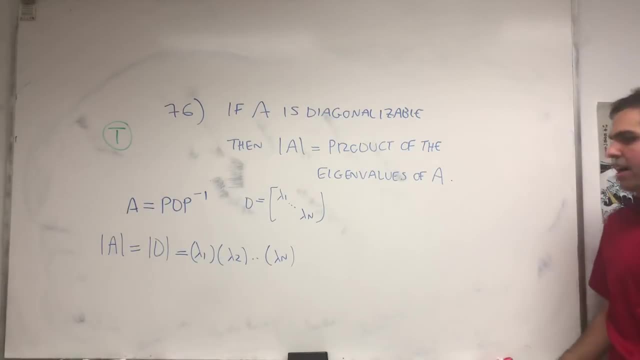 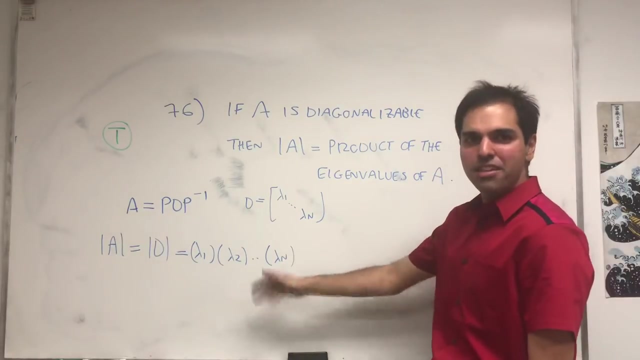 and similarly, the trace of a is the sum of the eigenvalues of a and in fact, or other authors like axler, they define the determinant to be the product of the eigenvalues and they prove all the properties of determinants using that way. but really no comment on these occurrences. 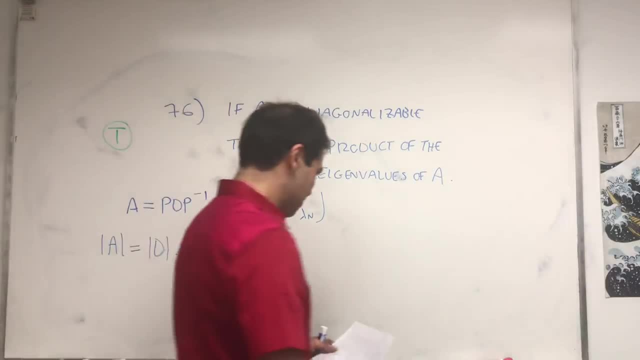 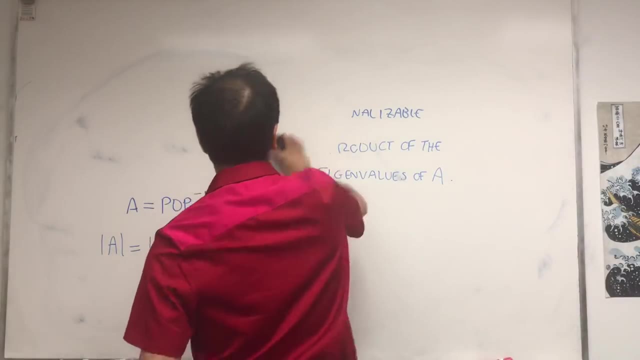 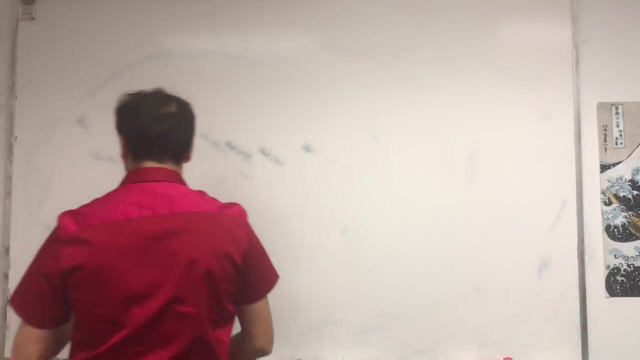 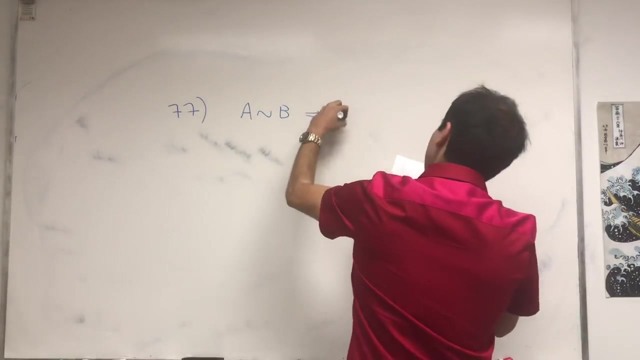 but know common that's not agree, right, really no comment about this. not my favorite approach. okay, so now we've shown that if a is similar to B, then a and B have the same eigenvalues. well, what about the eigenvectors? so if a is similar to B, do a and B have the same. 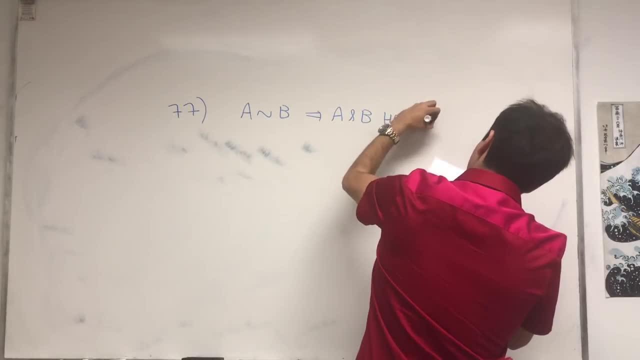 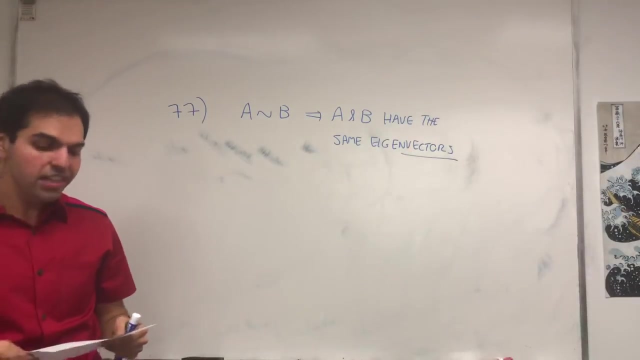 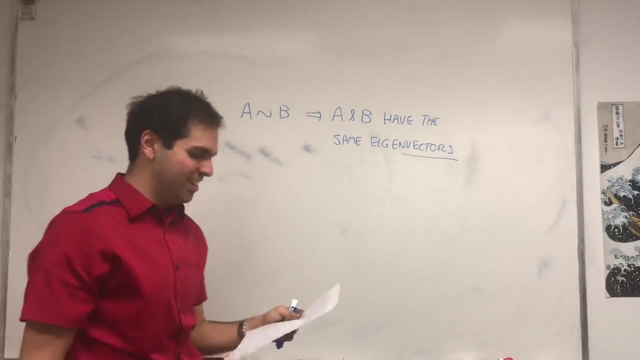 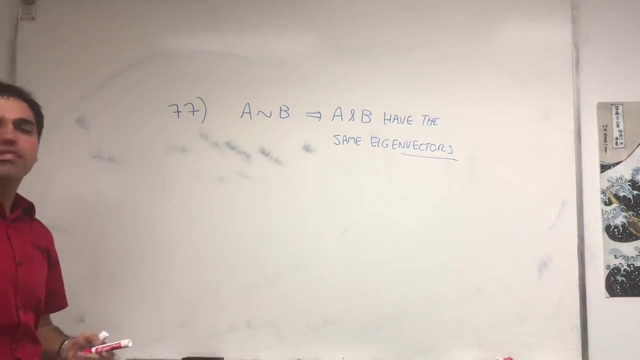 eigenvectors and 77 so they come. so Hindi, I think, and it's satatar. so before was chihatar, now it's satatar. and interesting, Lee, even if similarity preserve the eigenvalues, similarity does not preserve the eigenvectors, and here is why let's do a little proof by contradiction. 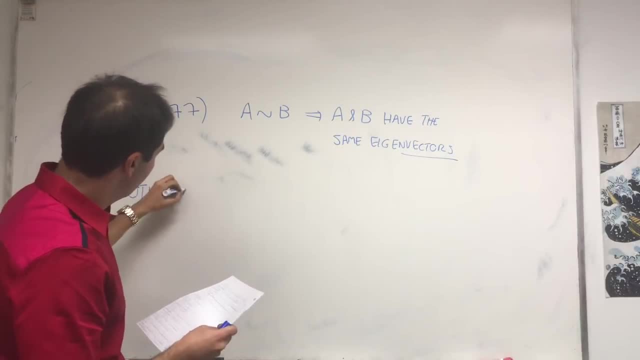 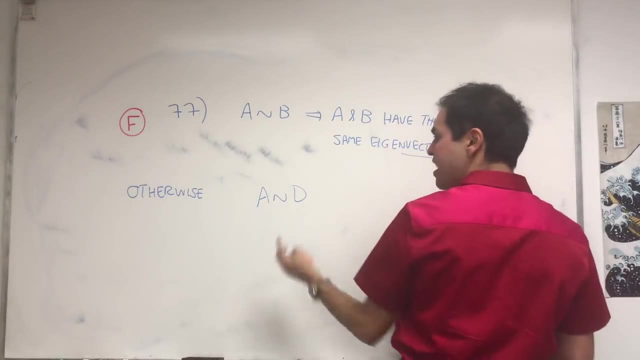 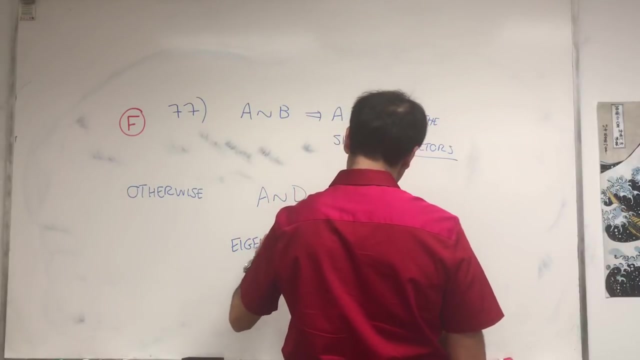 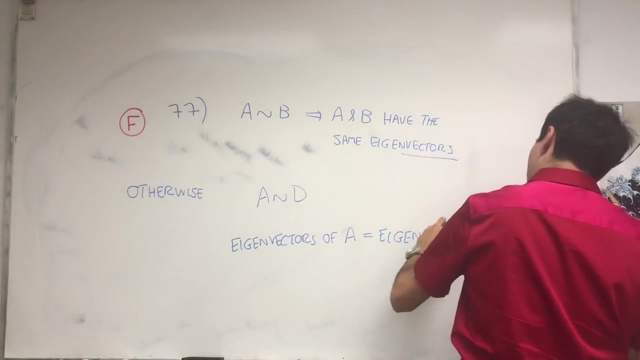 otherwise, what would that mean, suppose, if it is diagonalizable? if a is diagonalizable, then is a similar to a diagonal matrix, so the eigenvectors of a equal to the eigenvectors of D of D. but look, these are diagonal matrix and the eigenvectors of a diagonal matrix is just 1, 0, 0, 0, etc. etc. 0 0, 0, 1. so what? 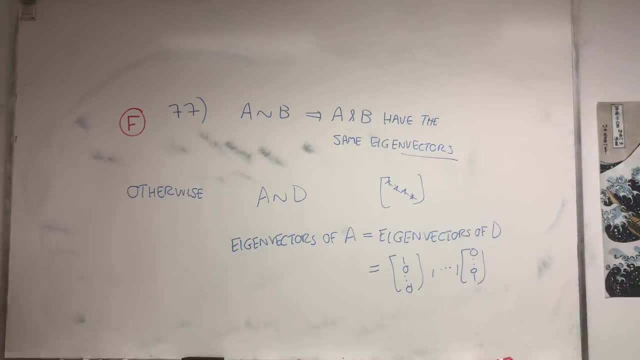 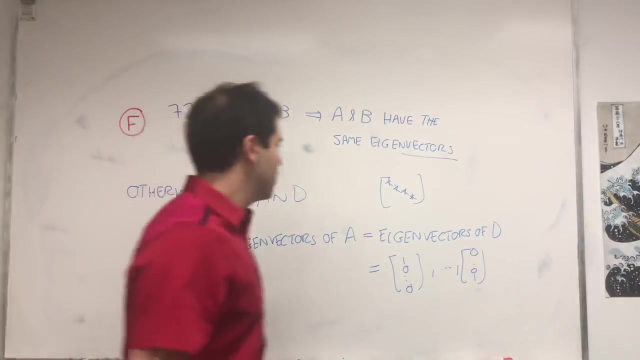 that would mean is that the only eigenvectors of any diagonalizable matrix is just the standard basis vectors and maybe a multiple of those, which is gibberish. so in other words, if this were true, any diagonalizable matrix would just have the e1 up to en as eigenvectors. and that's not true, or come up with any. 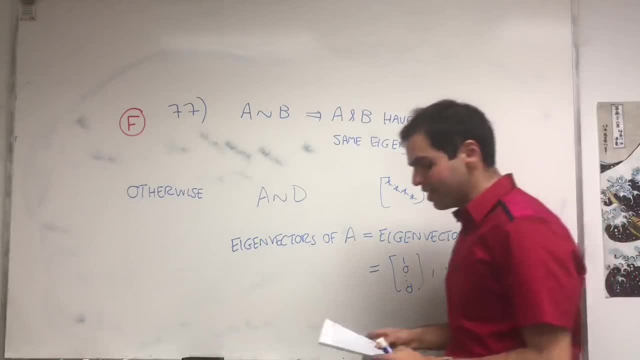 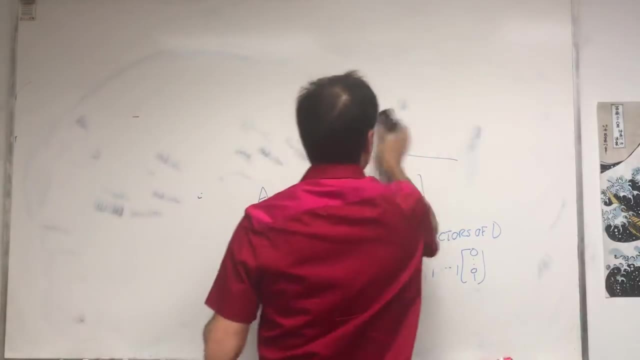 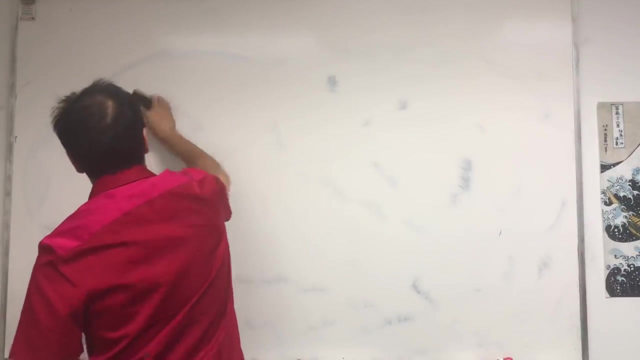 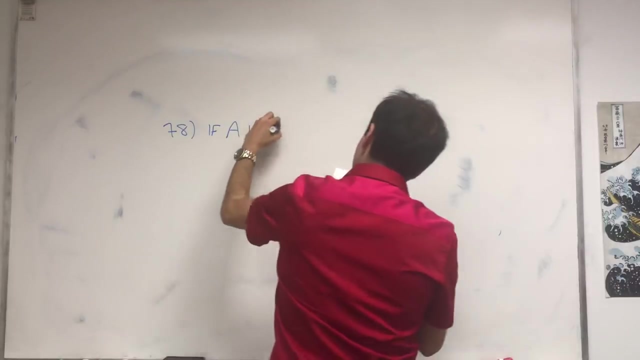 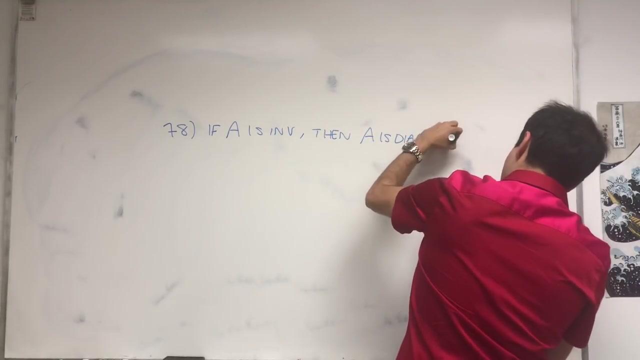 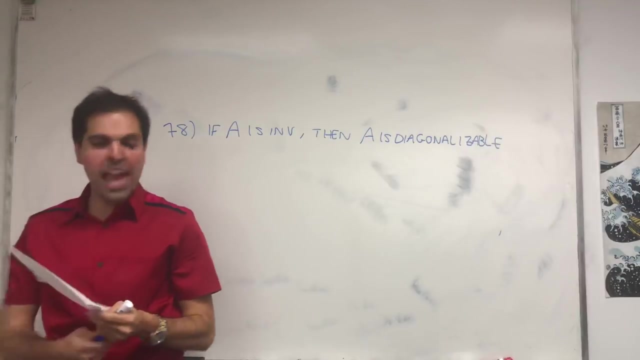 other example of similarity and then show that the eigenvectors are not the same. okay, next question: let's see if diagonalize ability has to do anything with invertibility. so 78: if a is invertible, then a is diagonalizable. 78 language, so the minbei dialect of Chinese and it's all are really cute. 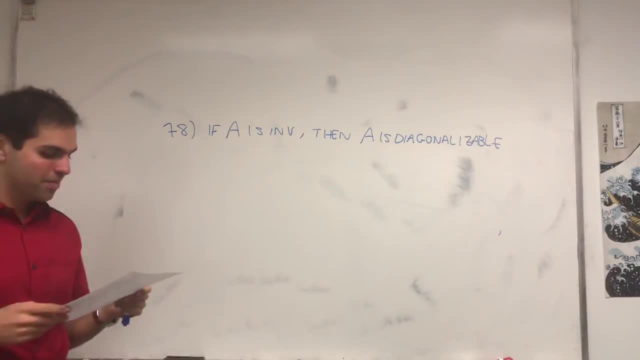 though chichi bop or chichi bop sounds almost like bimbi bop, very cute. so, and it turns out it's false. so invertibility has nothing to do with diagonalize ability. for example, take a. Invertibility has nothing to do with diagonalizability. for example, take a. 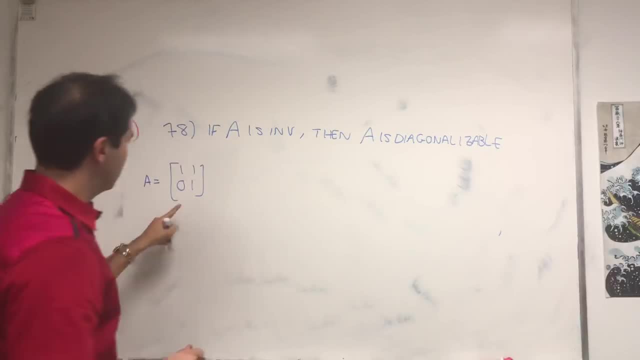 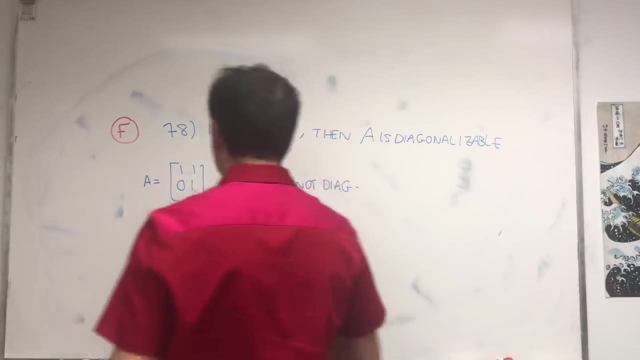 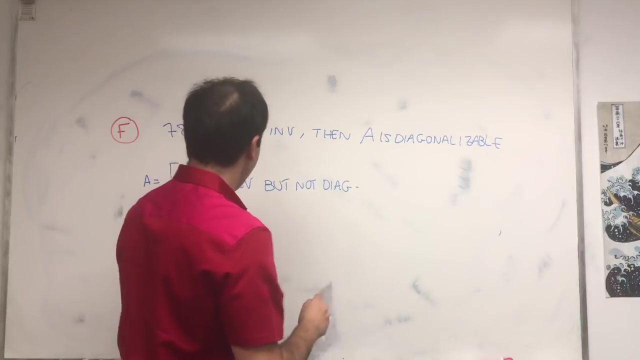 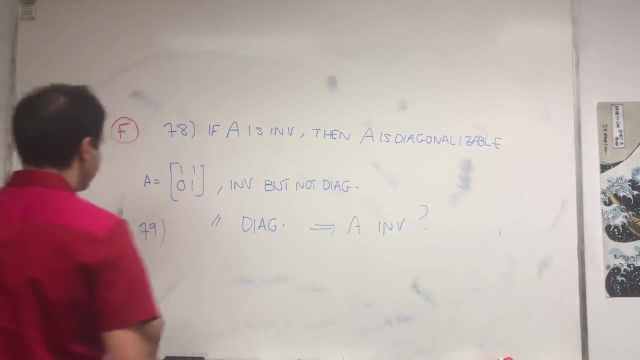 to be one, one, zero one. well, it's it, invertible, but not diagonalizable. we've shown in a previous example that this is not diagonalizable. well, what about the converse? so if a is diagonalizable, is a invertible. and Oh, Belarusian. so hey, Mac. 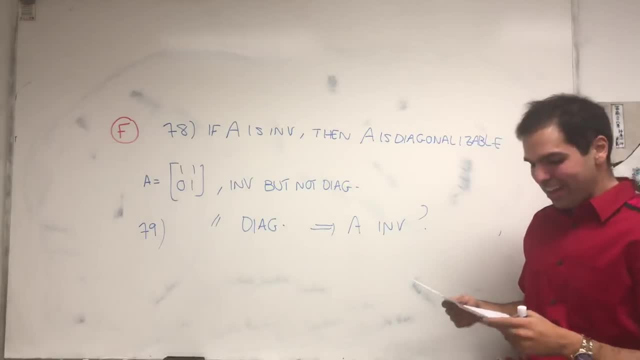 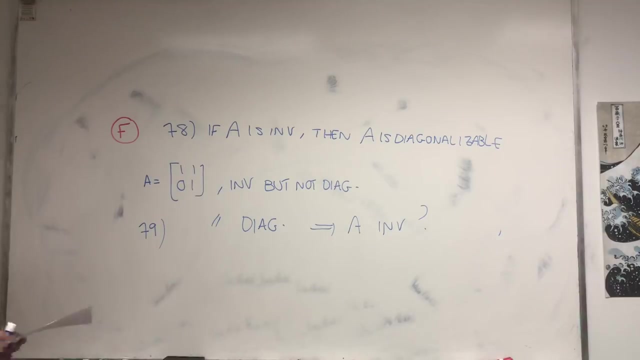 and my friend Max and it's all gone. CM Z: Alright, yes, vlog. sorry for butchering it. what something? Russian cuz. I wasn't CM, was that seven or something? so see em z. yeah, sigui tj's. anyway, it's false, so sorry. the statement was this, okay, sorry. talk to you in a little while. 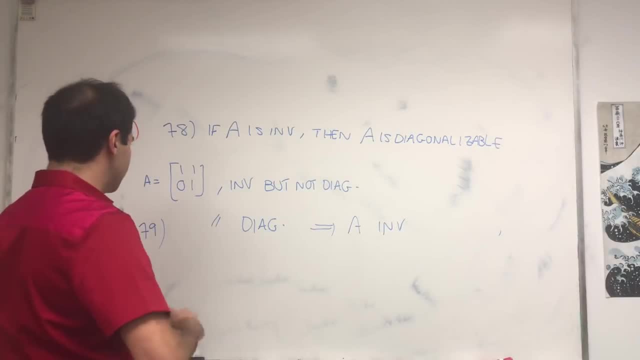 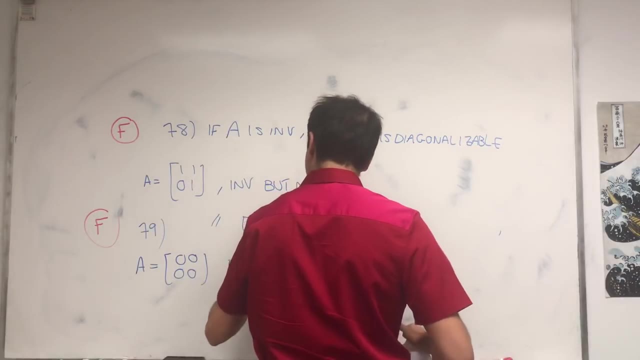 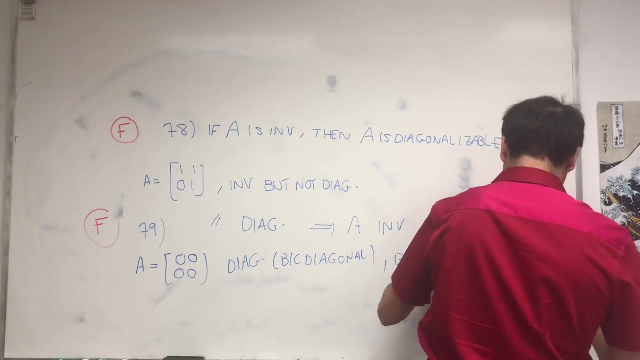 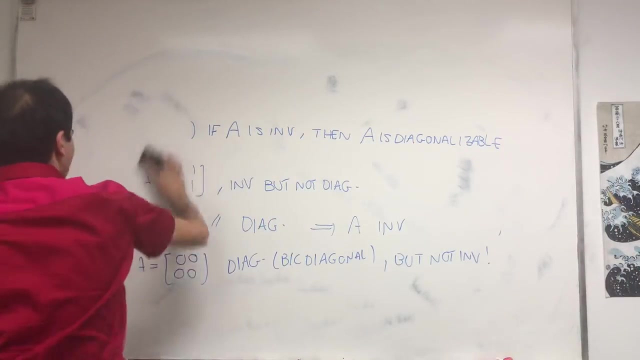 and it's false. For example, think of the easiest diagonal matrix, think the zero matrix. Well, look, it's diagonalizable because it's diagonal but not invertible. So in other words, diagonalizability and invertibility have nothing to do with the switch a to the b. 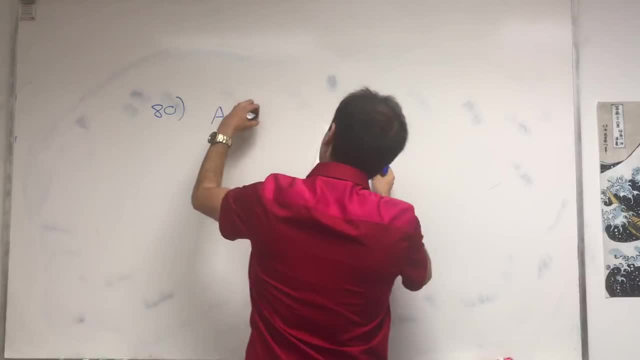 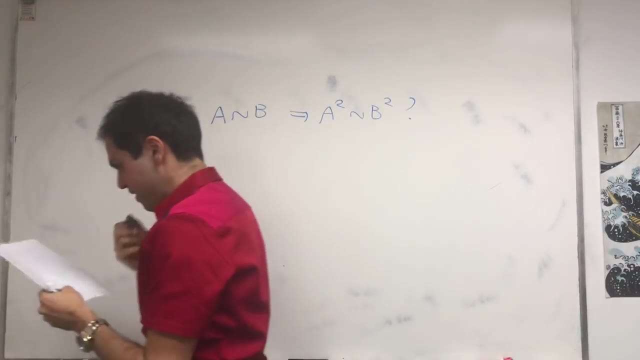 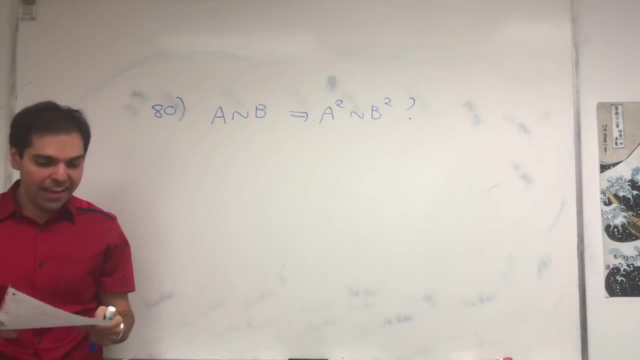 Okay, another one, so that's also cute. If a is similar to b, does that mean a squared is similar to b squared And a needs language. so I think a dialect of Thai, or like Zhuang and a d, is Pai-et-sib. 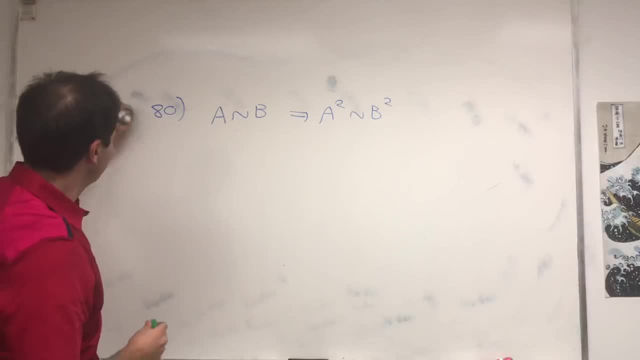 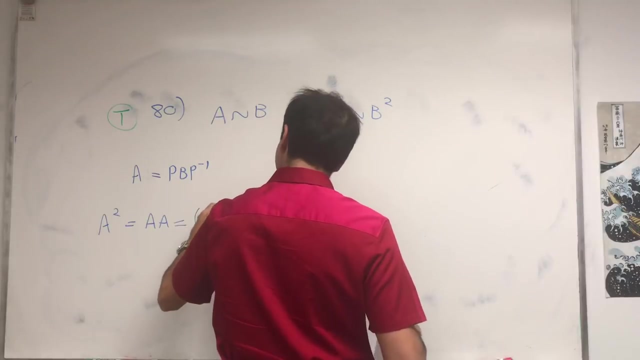 Let's figure out if it's true, but let me also already say it is true, because what does similarity mean? It just means that a is p, v p inverse for some matrix P, and that a squared is just a. a Eigenvalues are anonymous or something. so p b p inverse, p b p inverse. 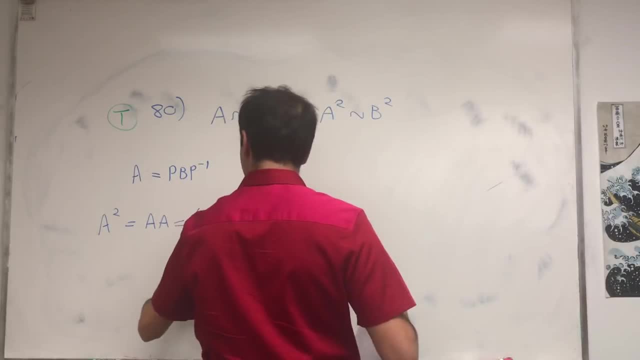 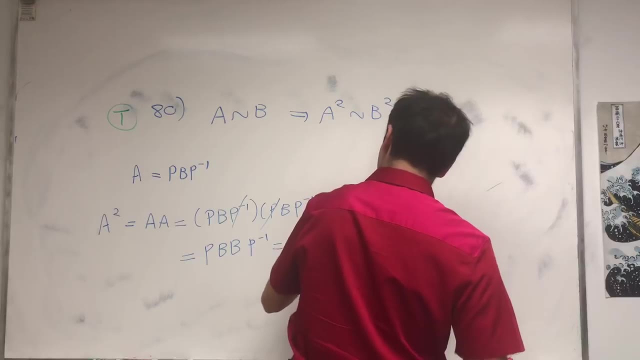 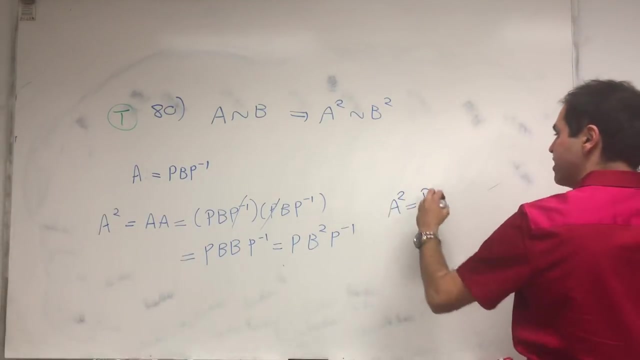 But look p inverse and p, they cancel out and you just have p, b and j. No, p, b, b, p inverse, and that's p, b squared p inverse, In other words, a squared equals to some matrix turns out the same matrix: P times b squared p. 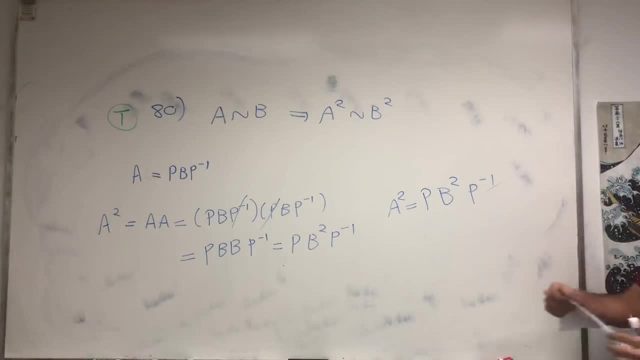 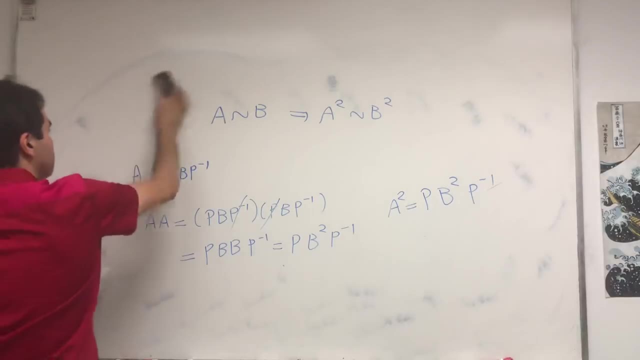 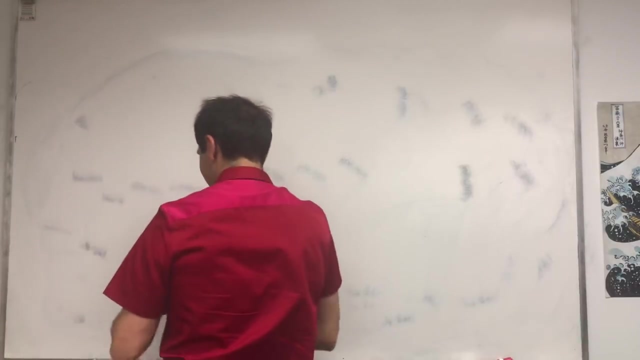 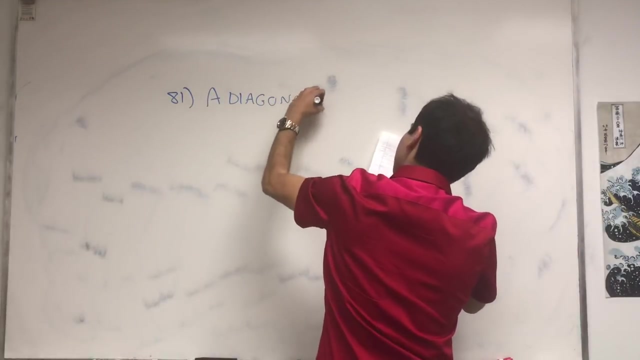 P squared times, p inverse, and that's just the definition of similar. So that's good, All right, and talking about this a bit more, question 81.. So a diagonalizable. So if a is diagonalizable and invertible, then so is a inverse. 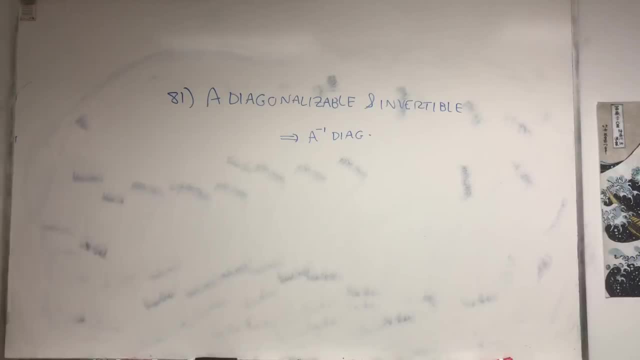 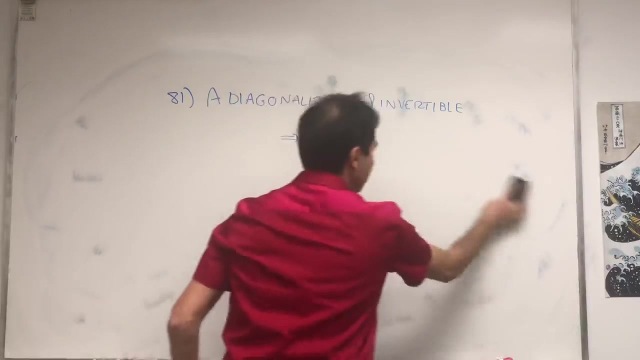 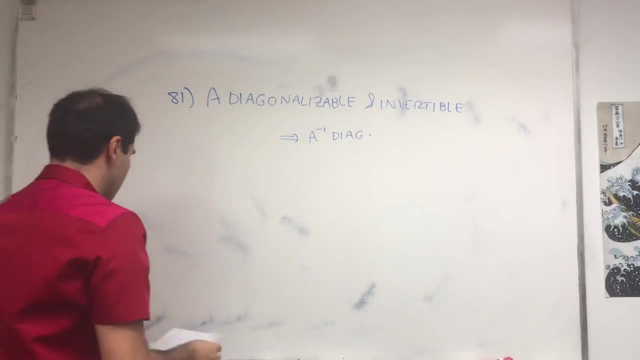 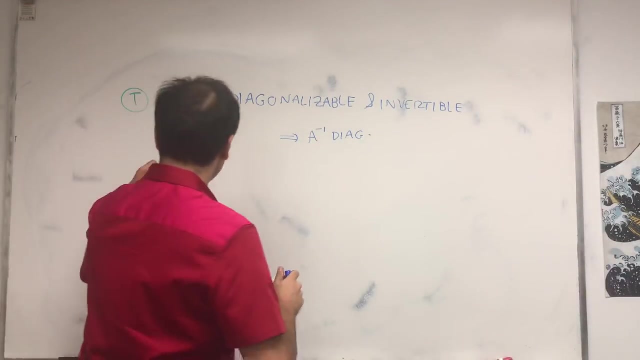 Diagonals, And 81, another dialect of Arabic, so the not g dialect of Arabic, and it's waheed wah thamanoon And my whiteboard is just completely blue now. But indeed this is true and I think the best way to deal with diagonalizability is simply p, b, p inverse. 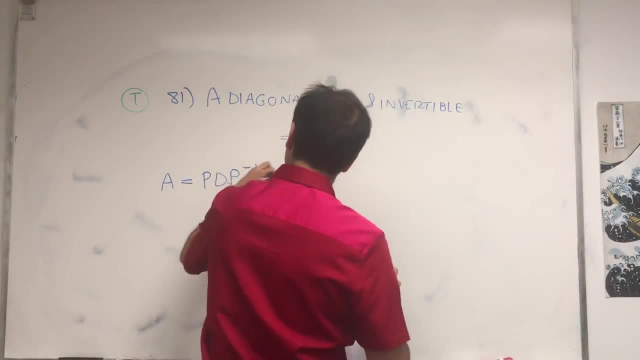 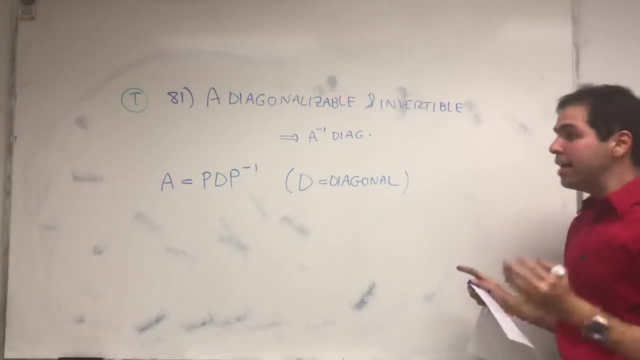 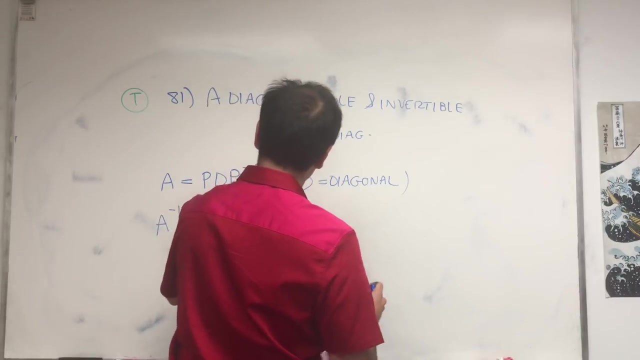 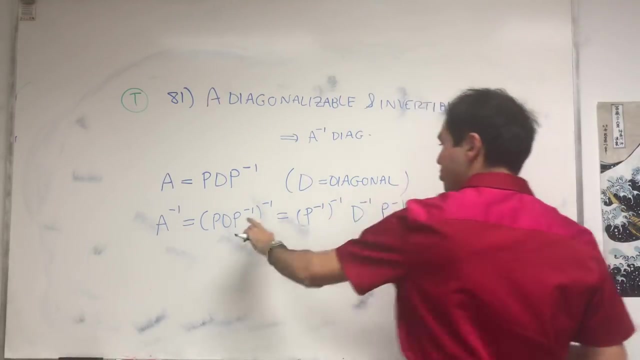 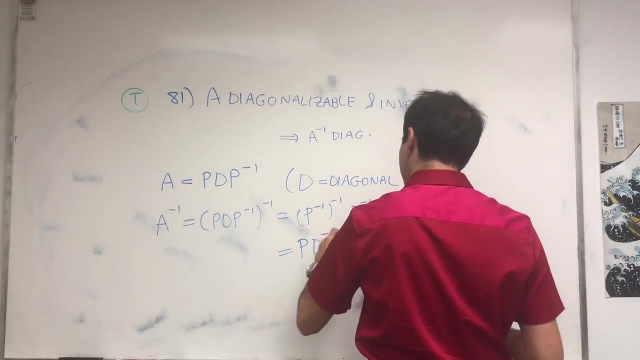 So if a is p, d, p inverse, where d is diagonal- that's a definition of diagonalizable, it's similar to a diagonal matrix- then a inverse is p d, p inverse inverse and a diagonalizable, And that's p inverse inverse, d inverse, p inverse. so you just flip all the three things and you get p, d inverse, p inverse. 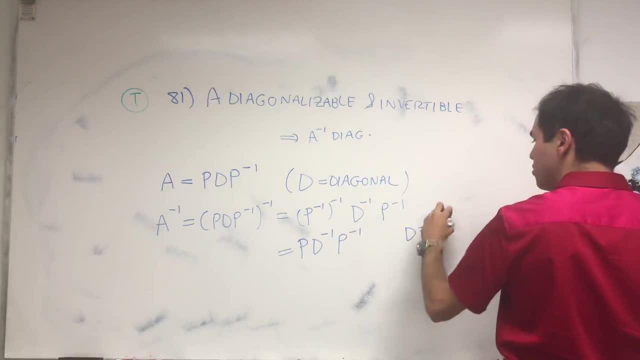 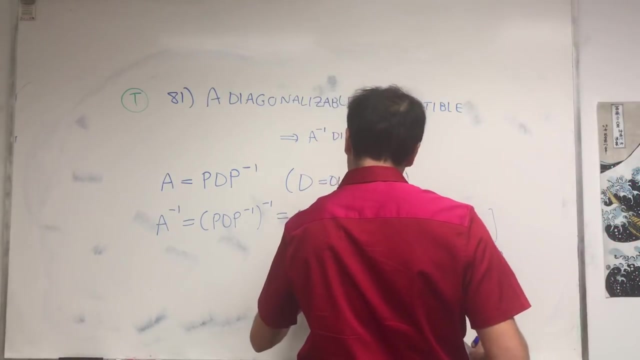 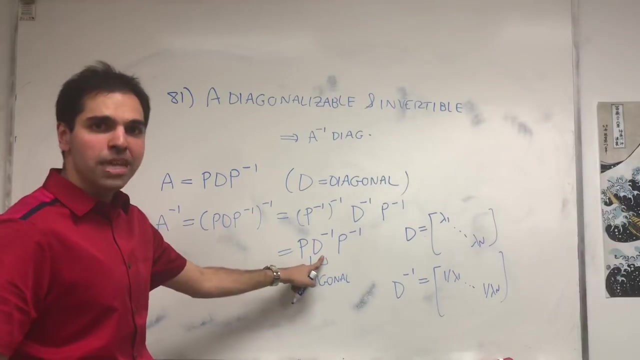 But look what is d inverse? So d is just a matrix with eigenvalues and d inverse- it's still diagonal. It's just a matrix with eigenvalues 1 over lambda. The point is, this is still diagonal And therefore a inverse is p times a diagonal matrix times p inverse, and that's just a definition of diagonalizable. 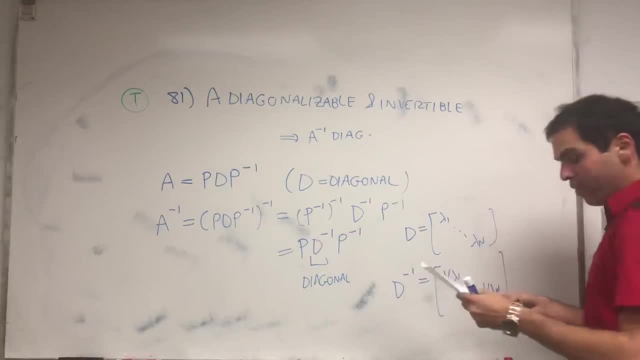 And one little thing. so remember, if a is invertible, then the eigenvalues are non-zero, so indeed, we can take reciprocals of every eigenvalue. So this is really legit. So remember, if a is invertible, then the eigenvalues are non-zero, so indeed, we can take reciprocals of every eigenvalue. 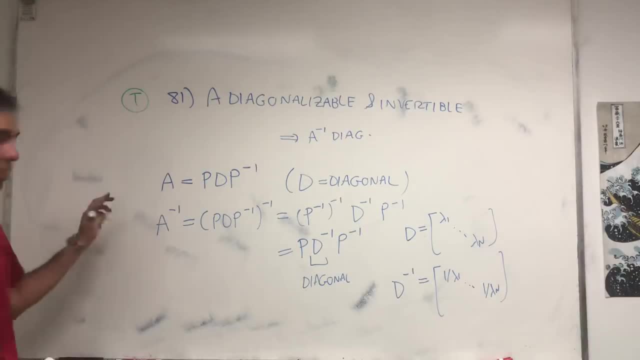 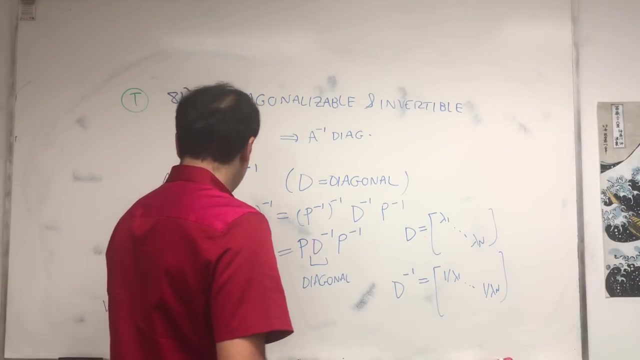 So this is really legit. There's another way of doing this. So if a v equals lambda v, then multiply by inverse, So v is a inverse lambda v, so that's lambda a inverse v, and we know that it's v, so a inverse v equals 1 over lambda v. 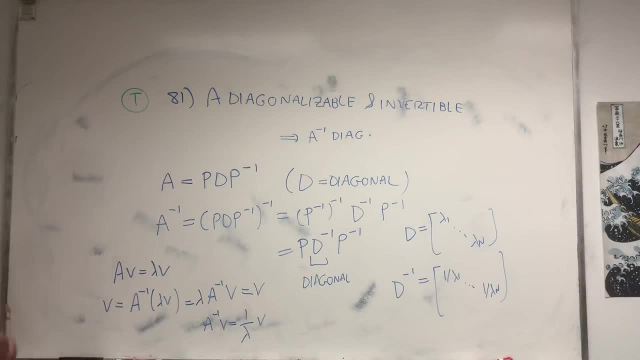 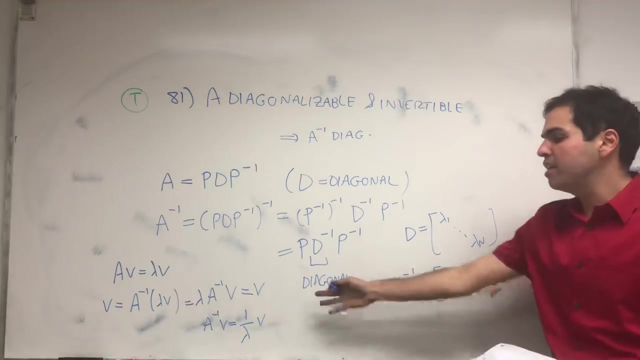 In other words, for every eigenvalue of a, for every eigenvector of a, it's the same eigenvector for A inverse. In particular, A and A inverse have the same eigenvectors. So if A has enough eigenvectors, A inverse also has enough. 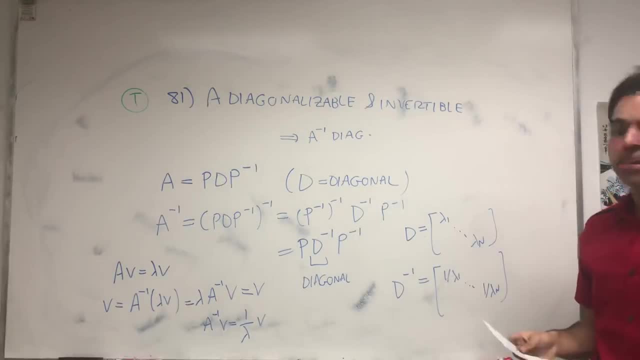 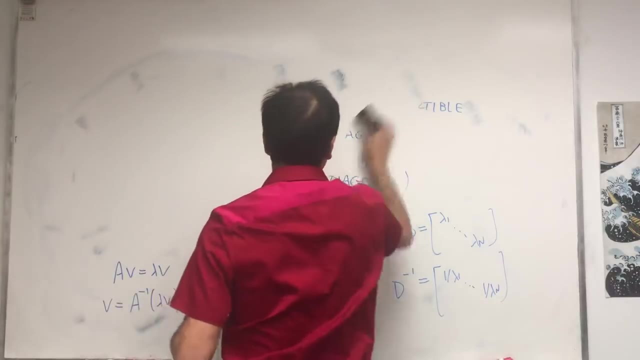 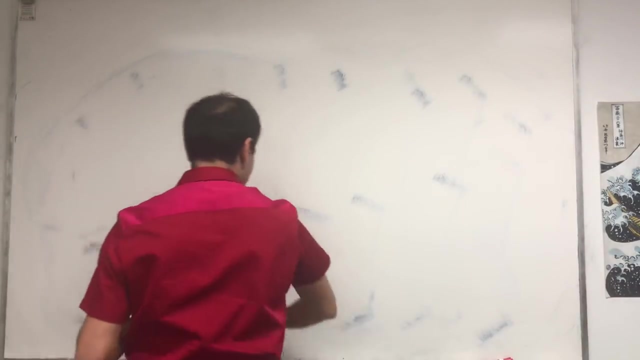 eigenvectors. So A diagonalizable implies A inverse diagonalizable. Okay, good, But that was just an exercise for showing diagonalizability And then just a couple of more properties. Let's see how many questions does this have? Okay, 86,, not too. 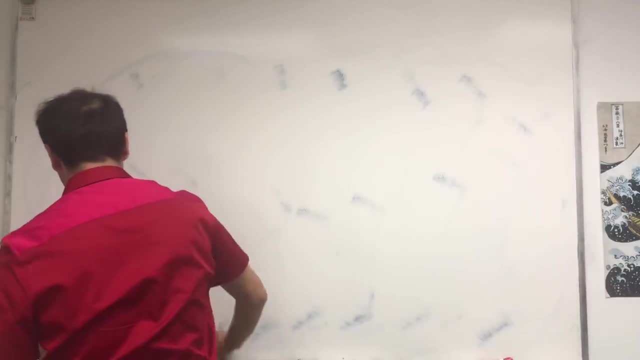 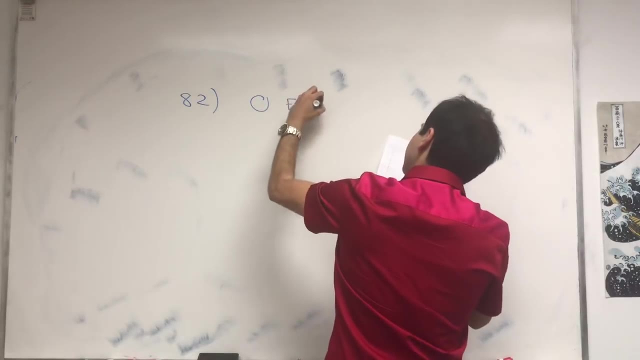 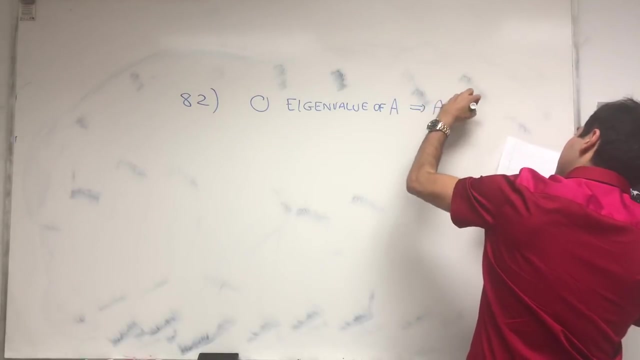 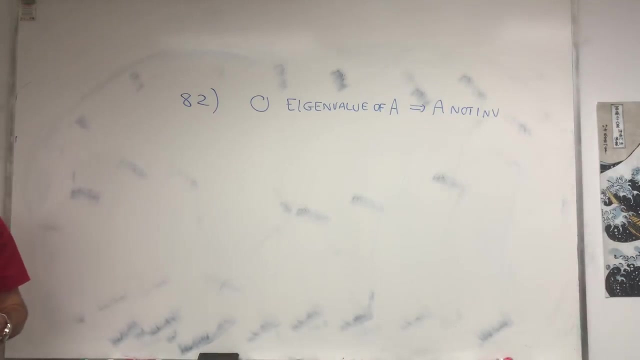 bad. So we're already at 82.. So 82.. So 0, an eigenvalue. if 0 is an eigenvalue of A, then A is not invertible And number 82 is well northern part of Pashto and 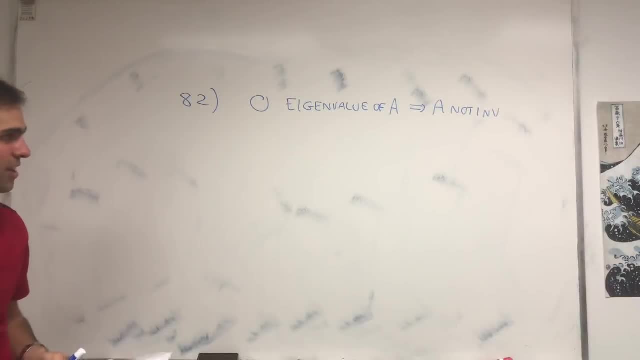 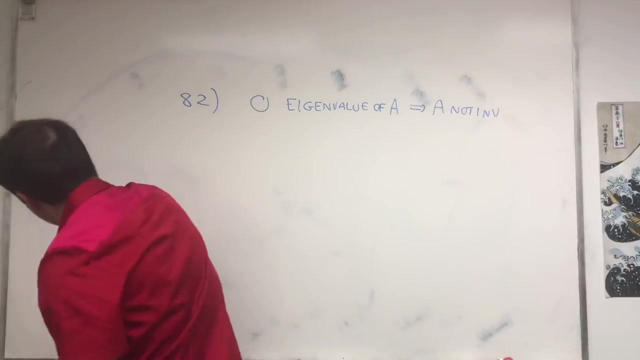 it's Af-Tee-ah, Isn't it? It's Mikael Atier, the famous z ağ. Oh, this is dough Asfio. and this is true, Be true to your heart, just like this question: What does it mean by definition? 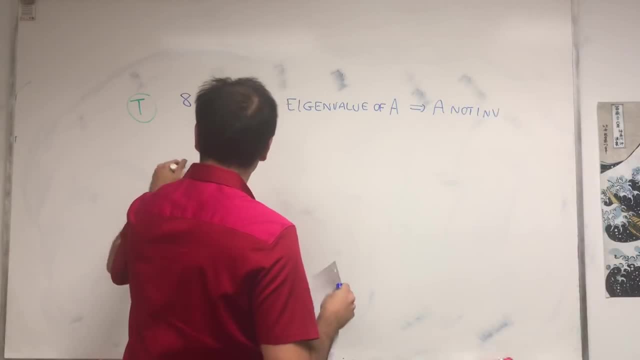 for 0 to G. What does it mean, by definition, for 0 to G be an eigenvalue? it really means determinant of a minus 0, i it's 0.. Because eigenvalues are numbers which make the determinant of a minus lambda i: 0.. 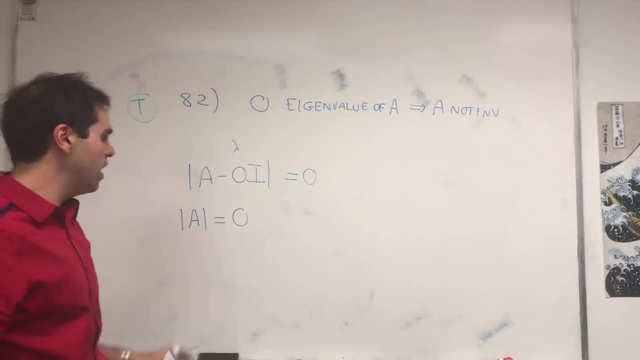 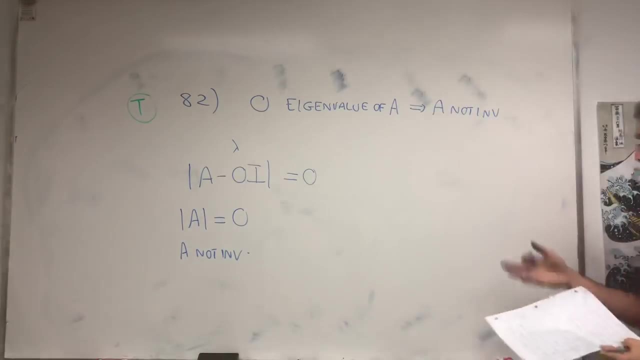 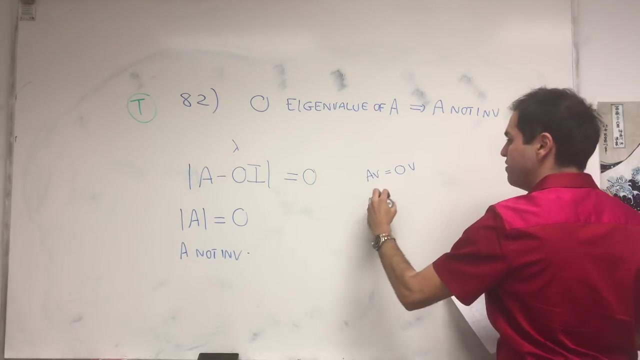 And in particular, this just becomes a determinant of a, which is 0. So a is not invertible. Or another way is right. if 0 is an eigenvalue, then there's a non-zero vector that makes av equals to 0v. 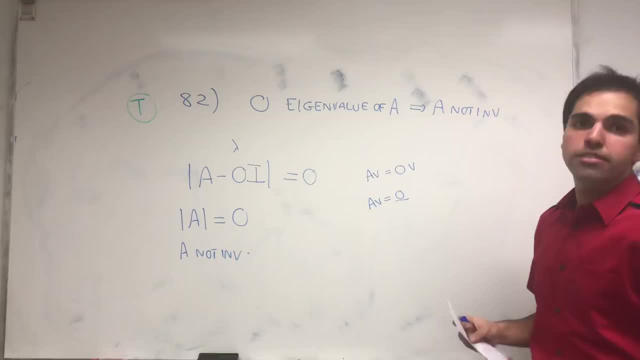 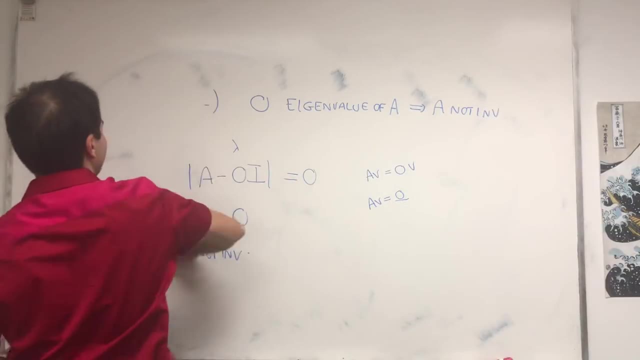 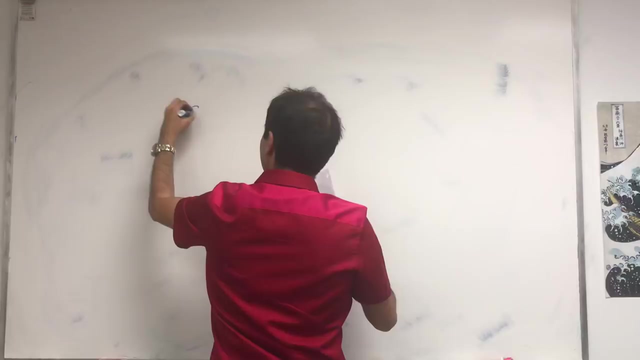 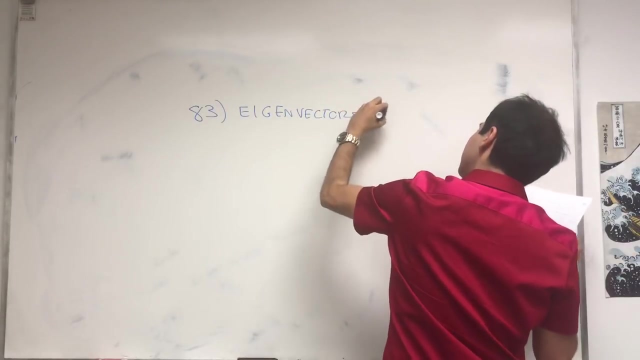 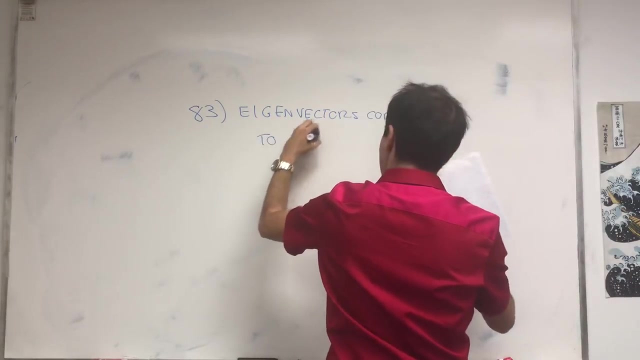 So av is 0. So the null space of a is non-zero, And this also guarantees that it's not invertible. Next question, one of my favorite questions: So eigenvectors, So eigenvectors corresponding to different eigenvalues. 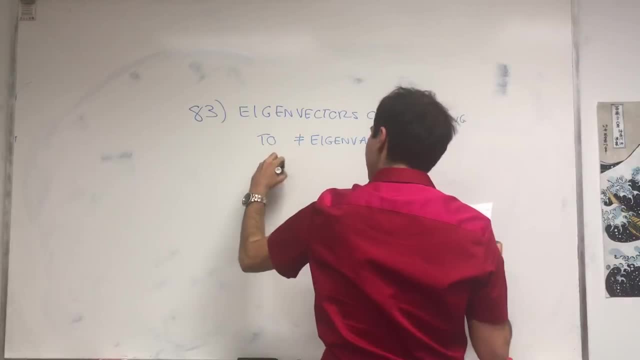 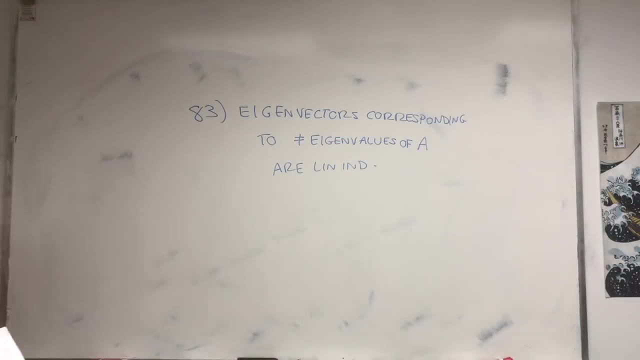 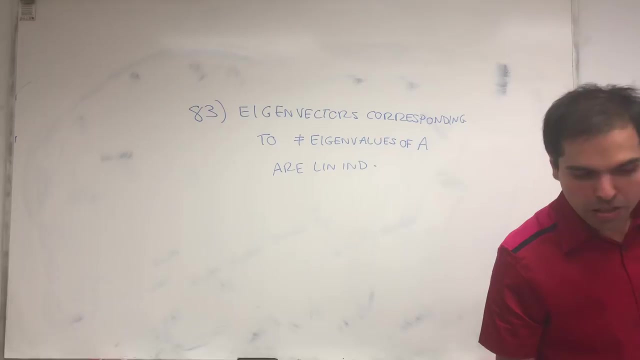 eigenvalues of a are linearly independent, And that's what made the first question work. if it's true, Because we had different eigenvalues and already said, well, all the eigenvectors must be different as well, And let's see if it's true or not. 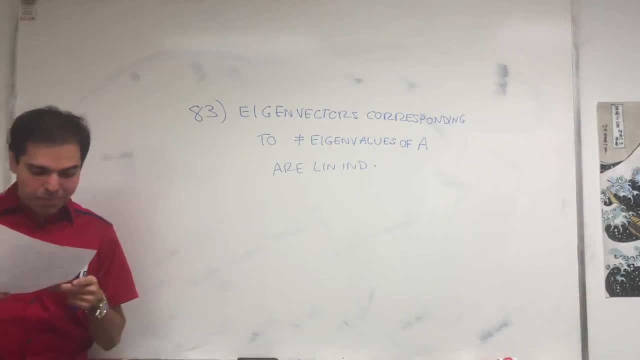 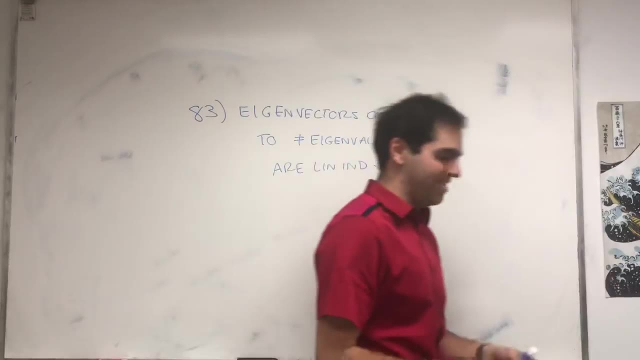 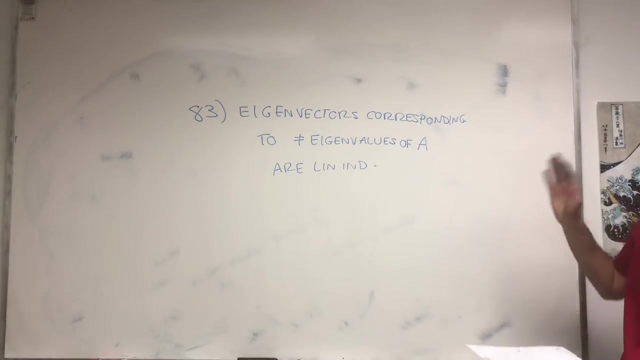 So ad3, it's Somali, And then- oh, it's interesting- Sadex, e, o, c, etan. It's very sad, but it's Sadex, A sad version of FedEx maybe, And of course, this is so awesome. 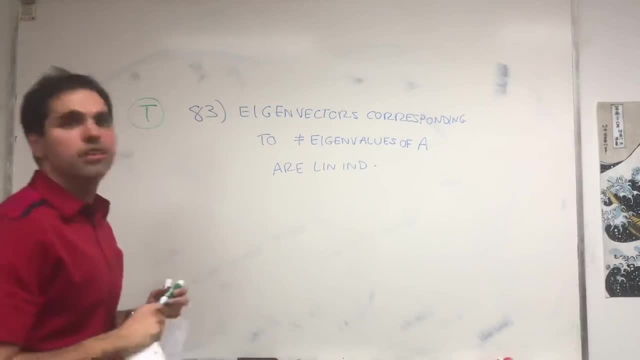 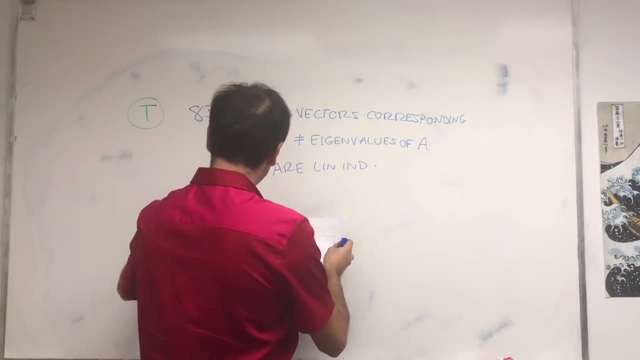 It's got to be true And let me show it to you. In the case of two eigenvectors, in general you would have to use induction. But suppose av plus bv, au plus bv equals to the 0 vector. We have to show that a and b are 0.. 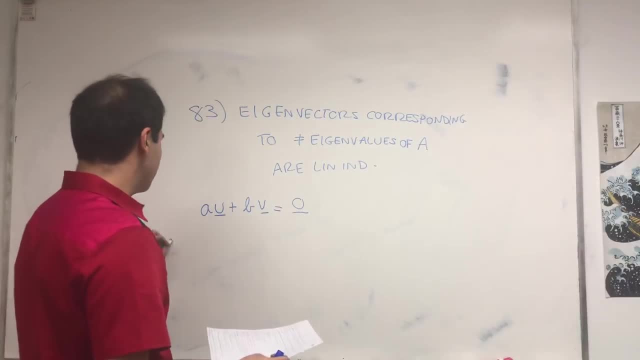 Look, on the one hand we can apply the matrix A to it, So A of au plus bv, that's A times 0.. A times 0 is the 0. This one you can fall out. So aau plus bav. 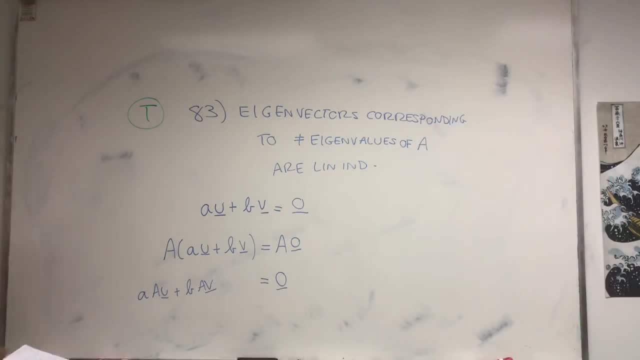 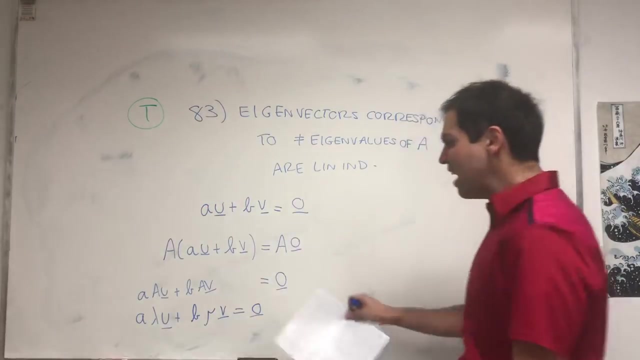 This is true Now. u and v are eigenvectors, So au is lambda u And bv, so av is another eigenvector. Let's call it mu, because we like cats and bunnies. So we get a lambda u plus b, mu, v equals 0., 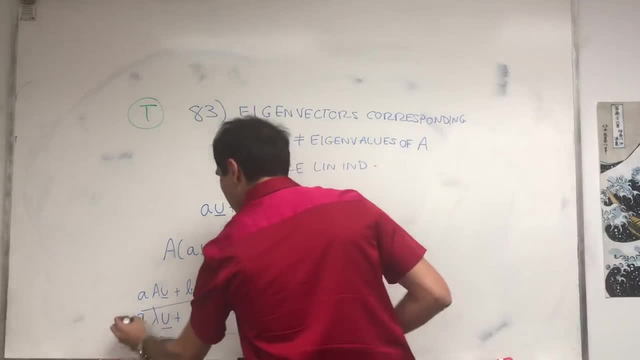 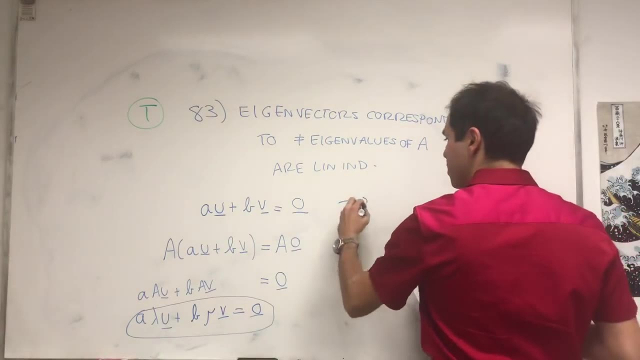 That's on the one hand, That's one equation that we have. On the other hand, this thing: we want a lambda to appear. So let's just multiply this by lambda. If you multiply this lambda, you get a lambda u plus b lambda v. 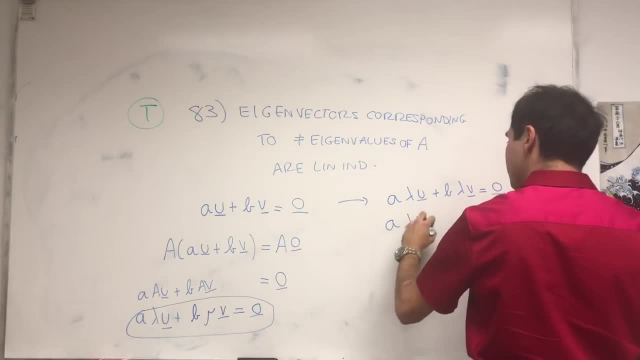 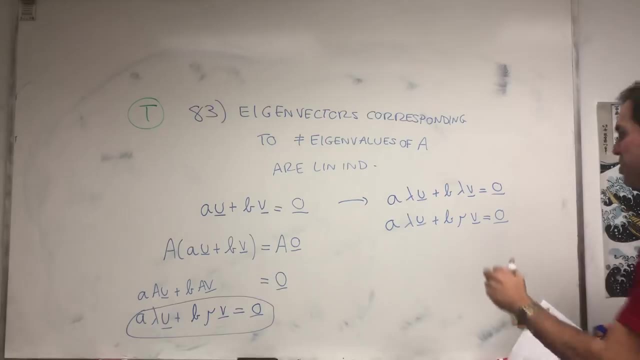 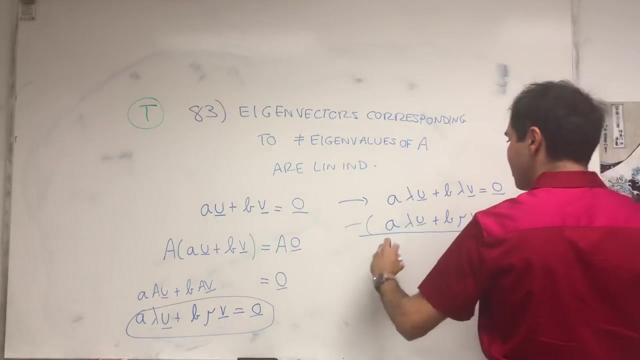 equals 0. And we also have the other equation, a lambda u plus b mu v equals to 0. So it's a nice movie, except it's a mu v. And then you have those two equations, Just subtract them. So this and this cancel out. 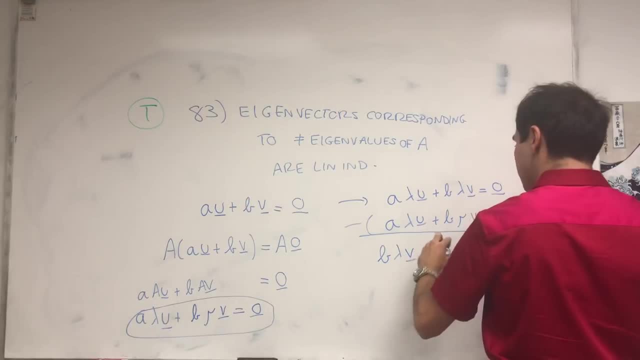 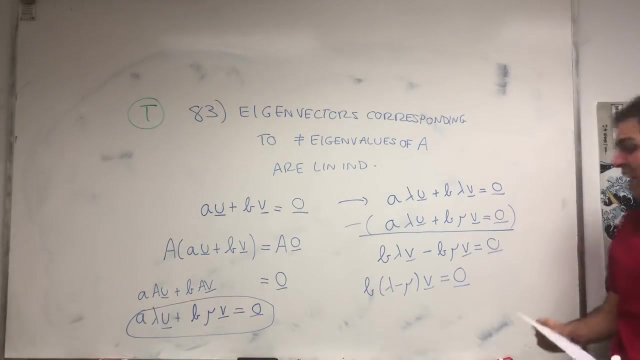 And this you just get: b lambda v minus b mu v equals 0. And you can factor this out. So b lambda minus mu v equals 0. And remember our eigenvalues were different. So in general this doesn't tell us much. 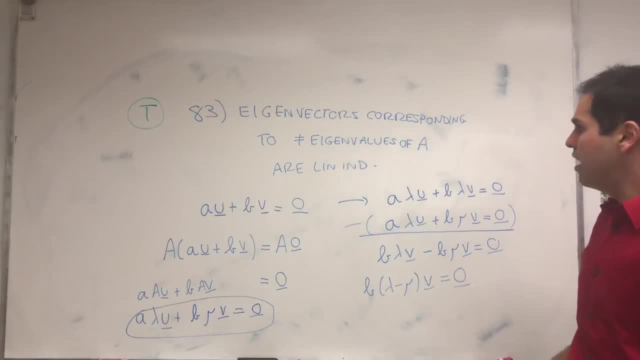 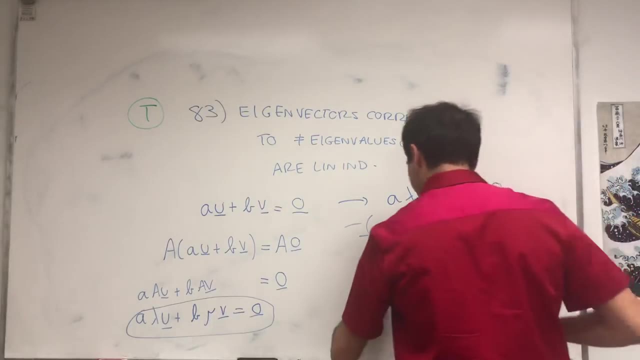 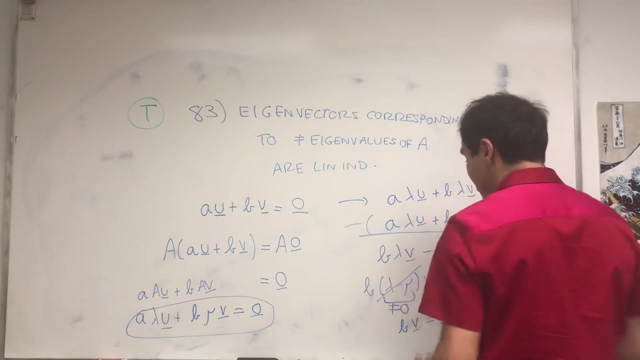 And in general, eigenvectors are not always linearly independent. But because this is a mu, this is a lambda, And mu and lambda are different, This is non-zero, So you can actually cancel this out. So you get bv equals 0.. 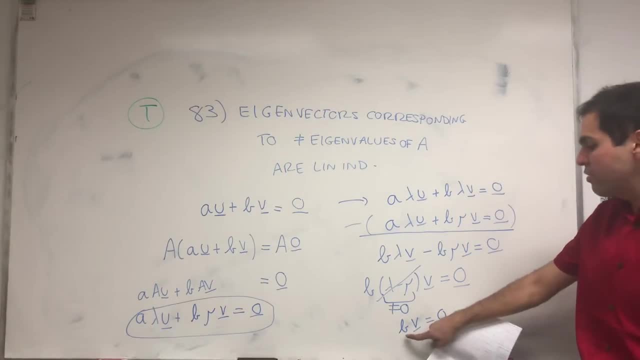 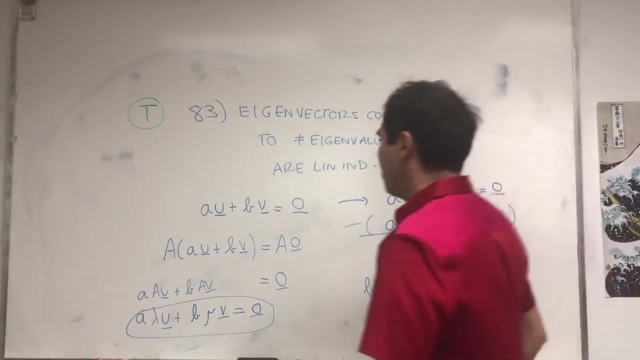 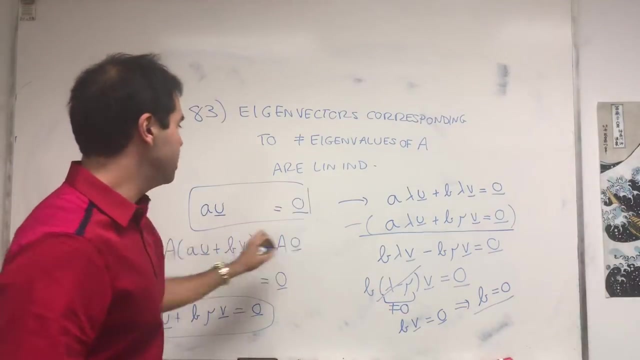 And remember: eigenvectors, at least in this case, are non-zero. So the only way that bv is 0 is if b equals 0.. So b equals 0.. So we can just cancel out, Subtract this And we get au equals 0. 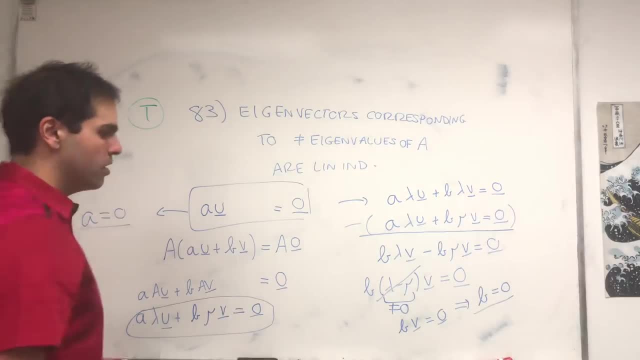 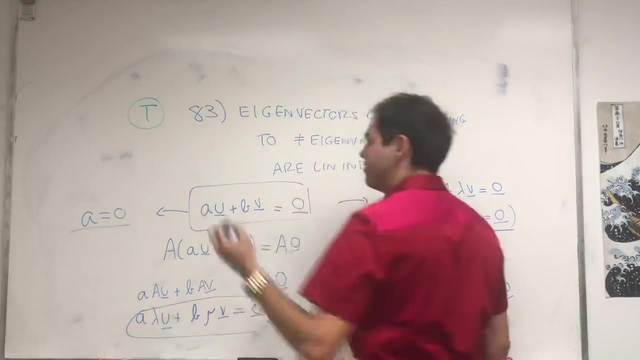 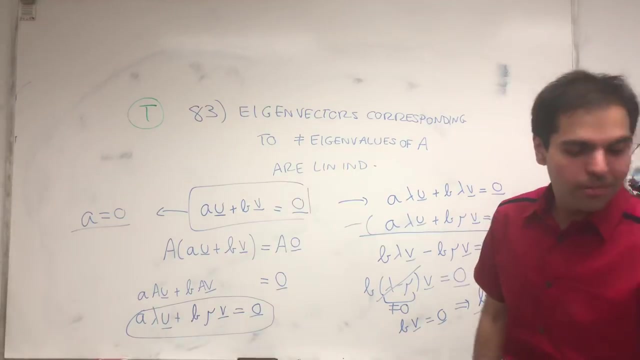 And then, by the same spiel, we get a equals 0.. So the only linear combination of a and b, u and b that gives us 0 is the trivial linear combination. So they are linearly independent And in general, as I said, you have. 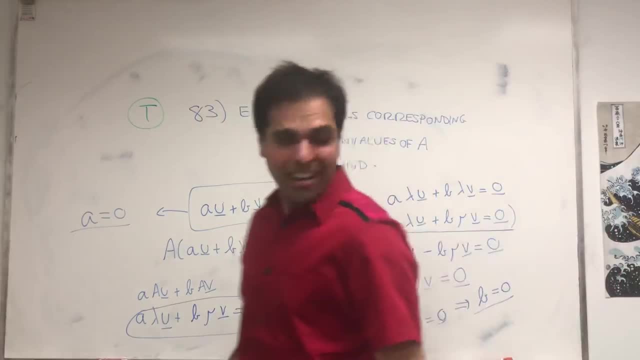 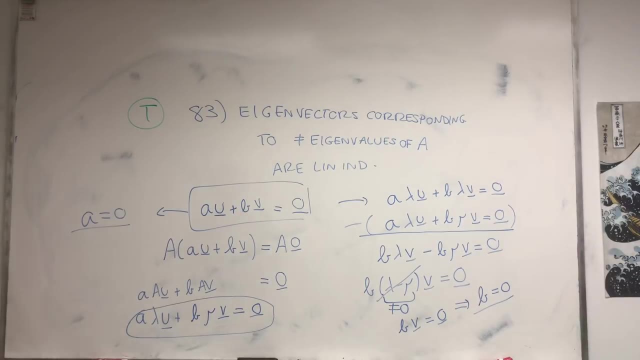 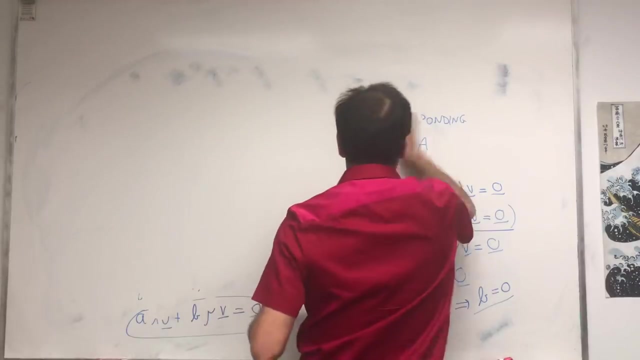 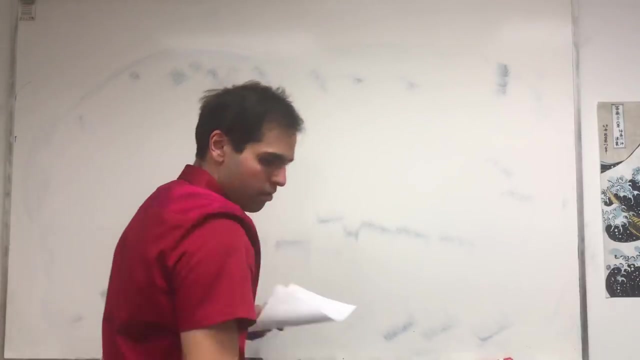 to use induction to prove that. OK, Almost done. So, more or less, I guess. Hello, Beautiful, OK. So three more questions on this section And then we'll move on to orthogonality. Let's see, Did I get it? 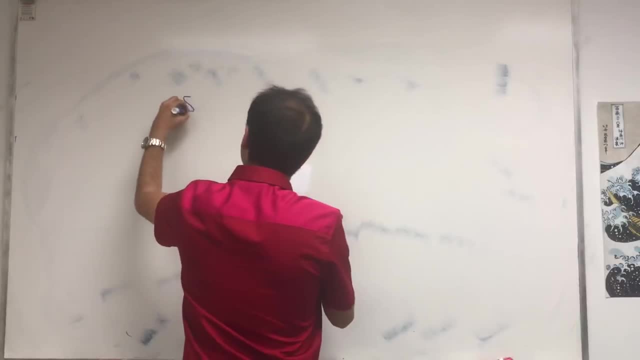 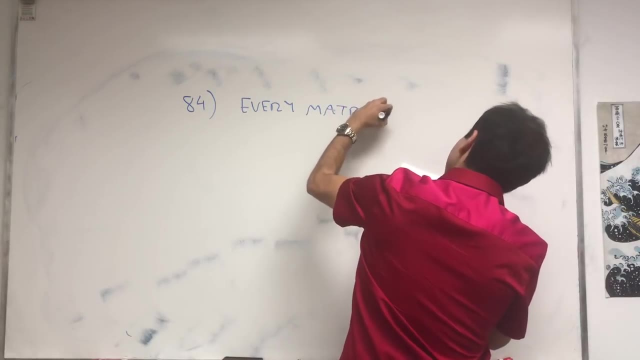 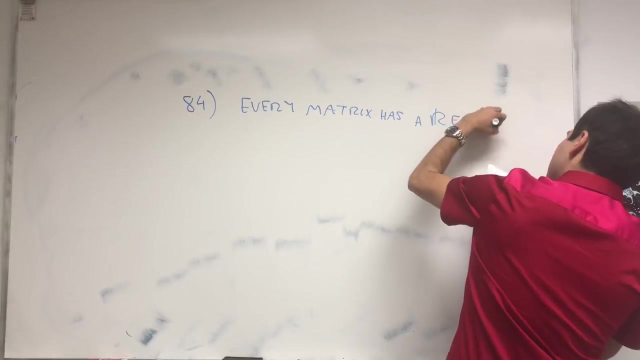 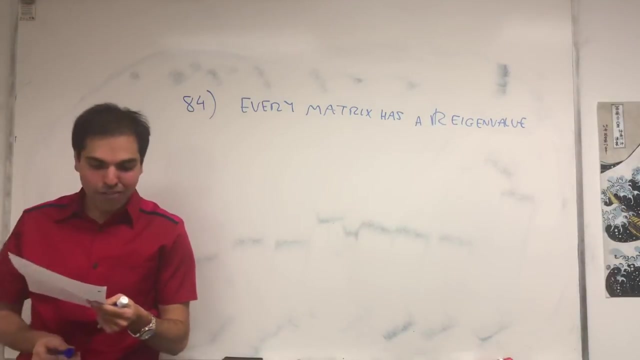 Yeah, I did Somali, I already said. So next question 84. Every matrix has a real eigenvalue. It has a real eigenvalue, All right, OK. So 84th language, Malagasy, And it's kind of cute. 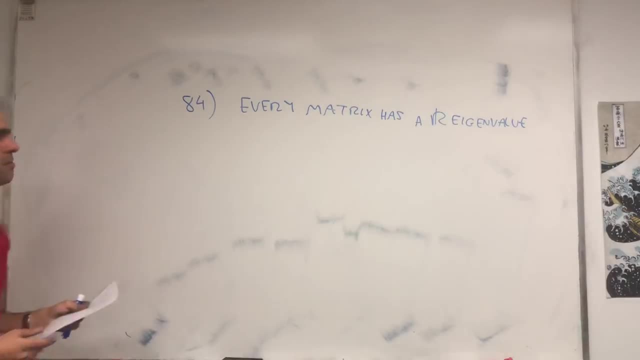 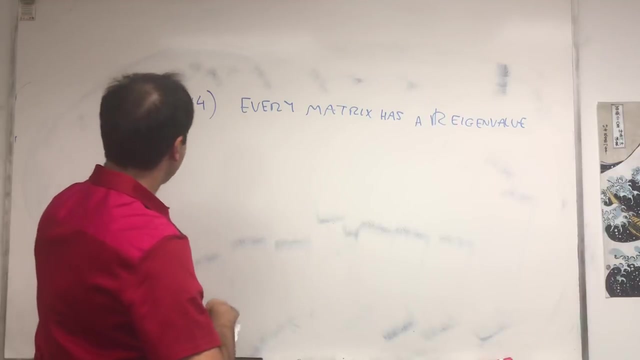 Valo polo e fatra, And I'm hungry. Polo in Farsi means rice. So now I'm on rice. Let's see. And unfortunately not every matrix has a real eigenvalue. Consider the following matrix, I think: rotation maybe. 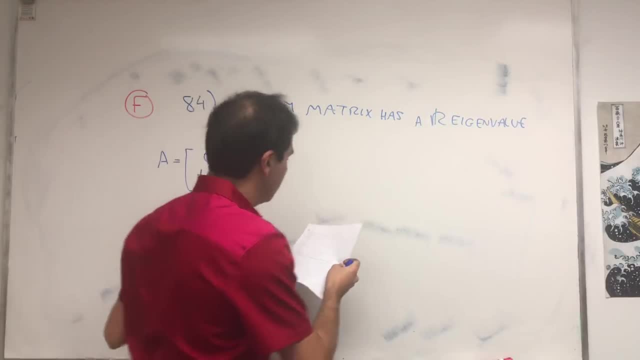 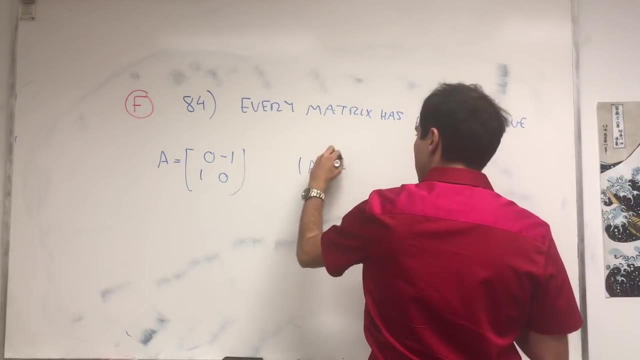 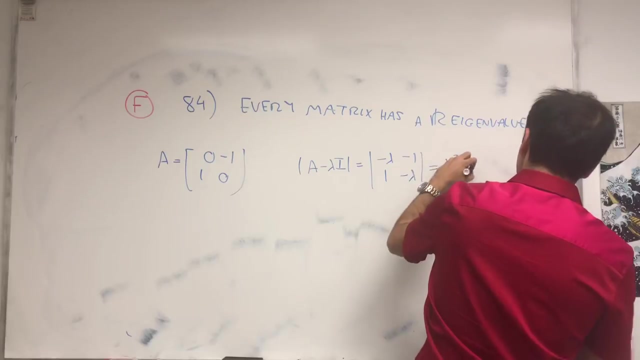 A is 0, minus 1, 1, 0.. And well, in this case, determinant of A minus lambda i, it's determinant of minus lambda minus 1, 1, minus lambda, That's lambda squared plus 1.. 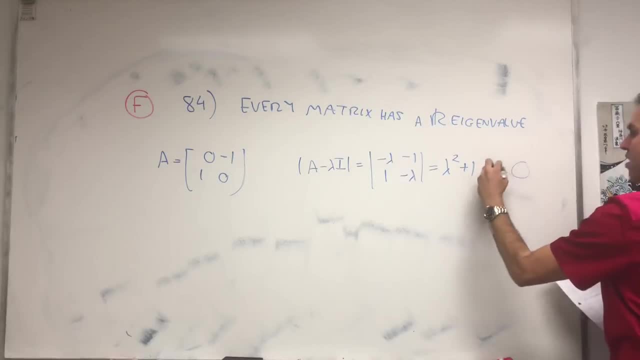 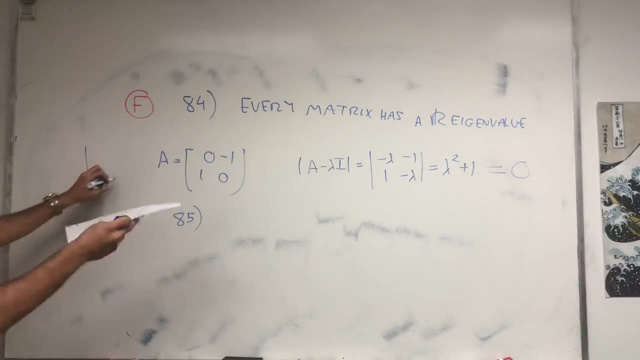 And unfortunately this never has a real root. So not true that every matrix has a real eigenvalue And in fact it makes sense. I don't know, I don't know exactly which stretching this is, But rotations in general don't have real eigenvalues. 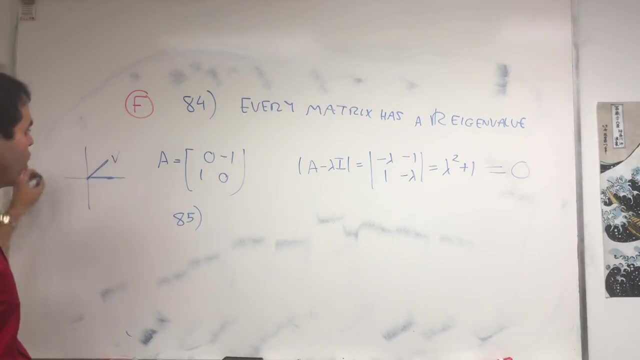 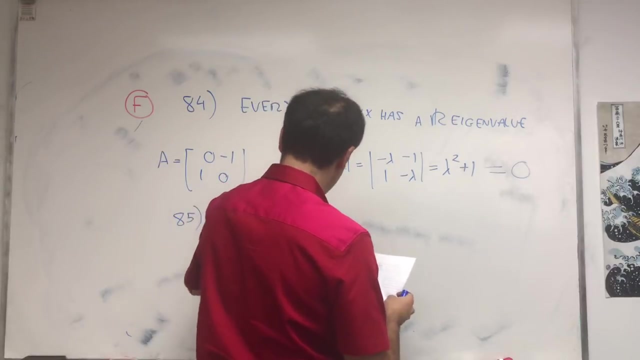 Because if you start with a vector v, there's no way to rotate it to get a scalar multiple of this v. So also intuitively, it makes sense. But now what about the other question? What about complex eigenvalues? Has at least a complex 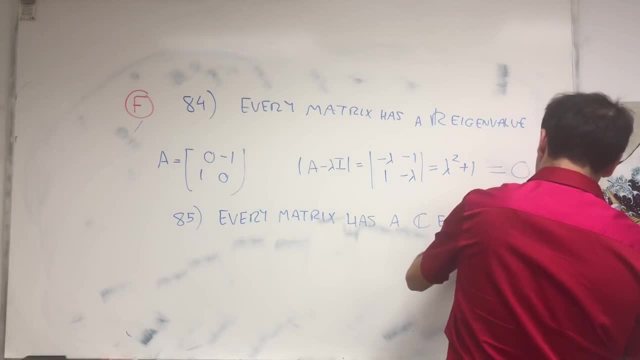 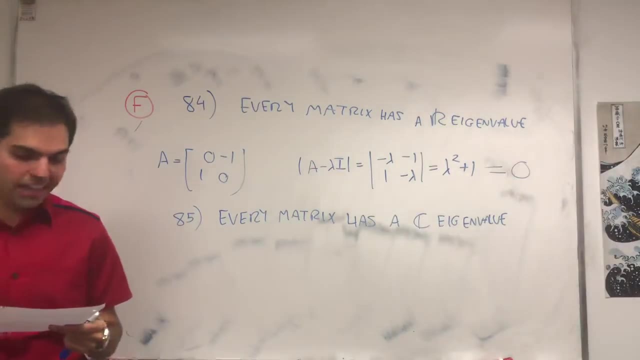 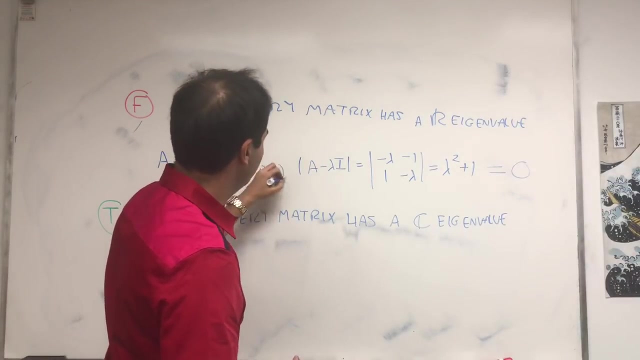 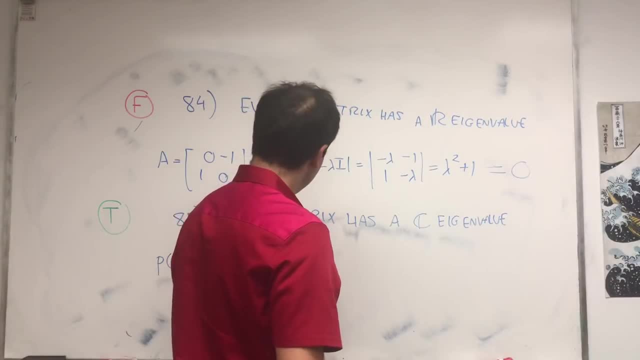 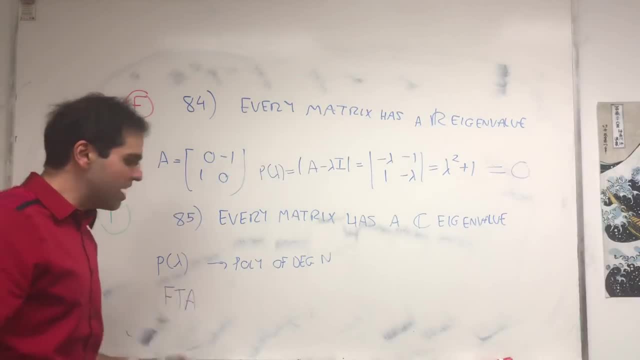 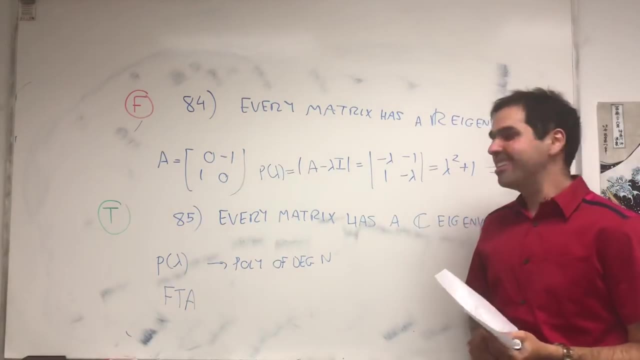 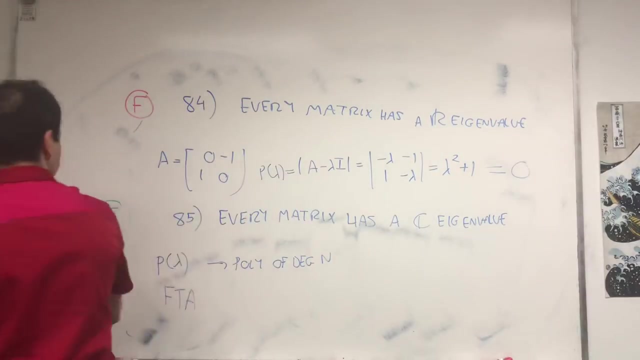 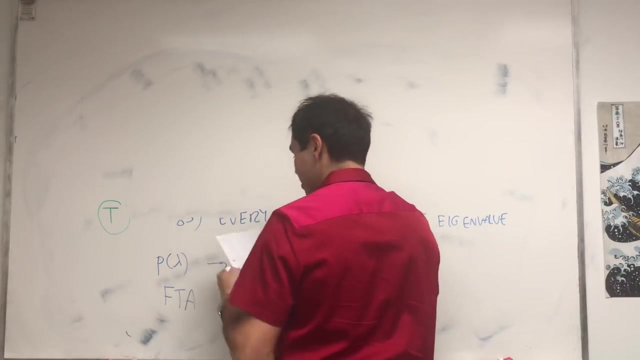 So there's full known industrial non-PCM and Patricia Bell with the mystic polynomial. It is a polynomial every Wyoming, only It is a polynomial of the degree of m, some degree. And there is this beautiful thing question on eigenvalues and eigenvectors. Sounds too good to be true. Let's see if it's. 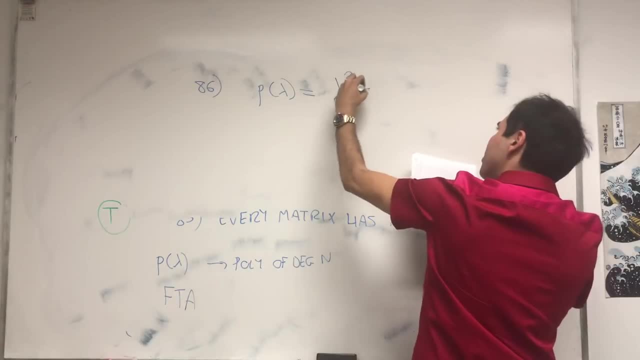 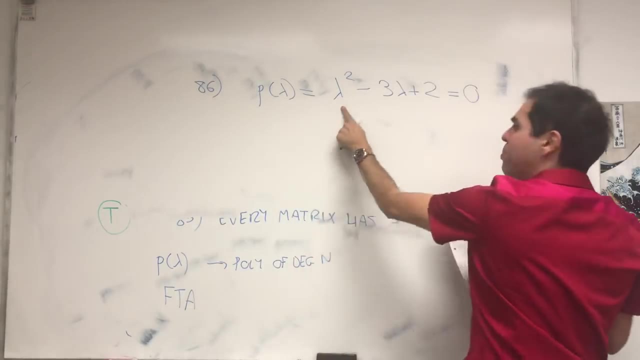 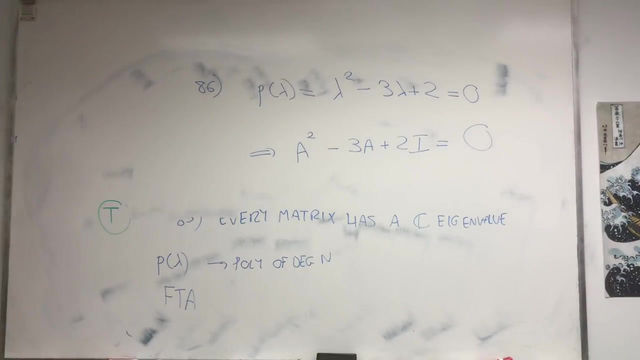 true. Suppose a matrix has characteristic polynomial lambda. squared minus 3. lambda plus 2 equals 0.. Is it true that you can plug in a for lambda? So is it true that a squared minus 3a plus 2i equals to the zero matrix. So can you just naively plug in a matrix for. 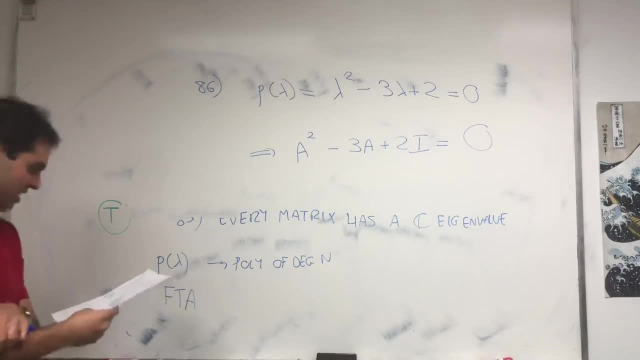 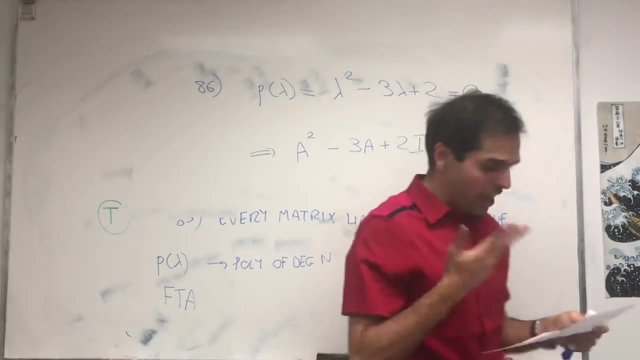 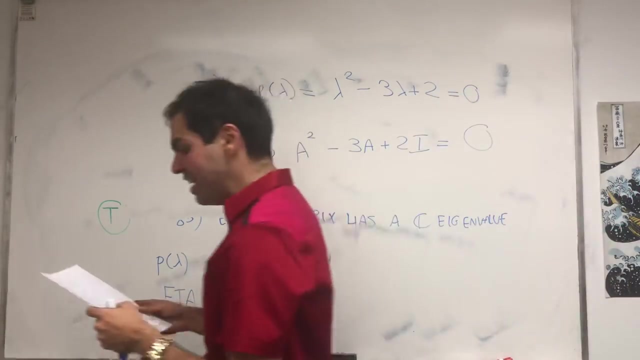 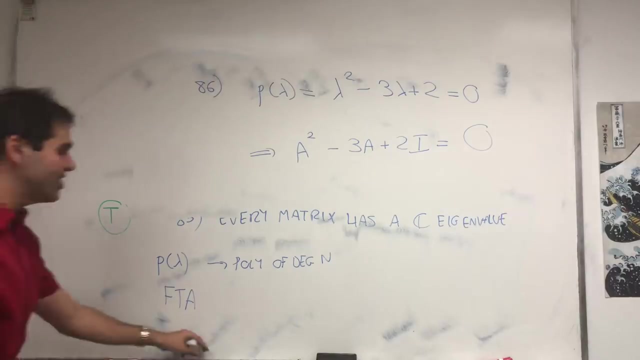 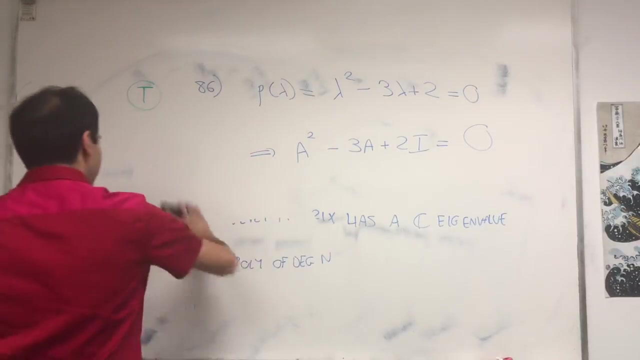 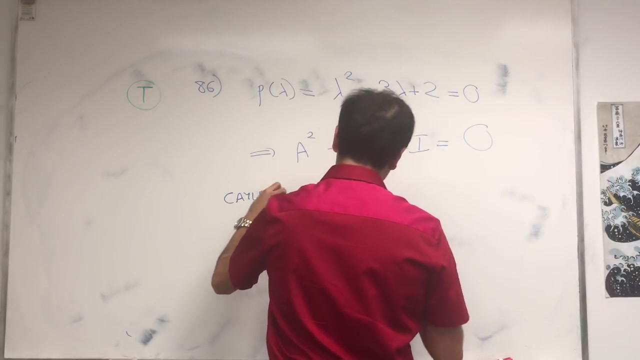 its characteristic polynomial And 86 languages. I can't even read it And the language is sorry. the number is So Um and as beautiful as it sounds, it's actually true, And this result is one of the deep results in linear algebra. It's called the Cayley Hamilton theorem. Cayley Hamilton theorem. 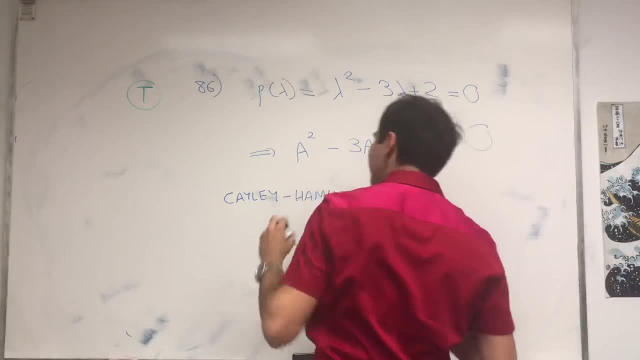 And I have this friend. I still have him. he still exists. I have this Cayley Hamilton dance Where, whenever we saw each other when we talked, Dr O'Keeley Hamilton would like dance in circles. So that was fun. but just to remind you. 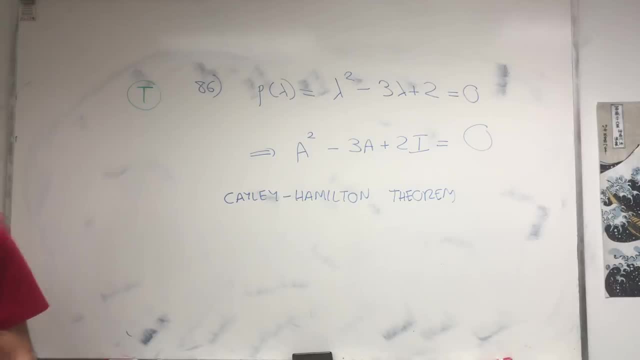 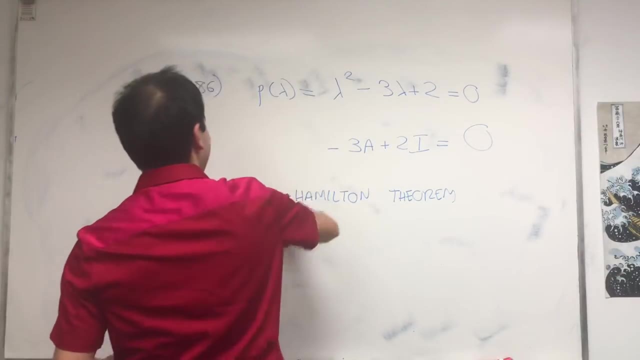 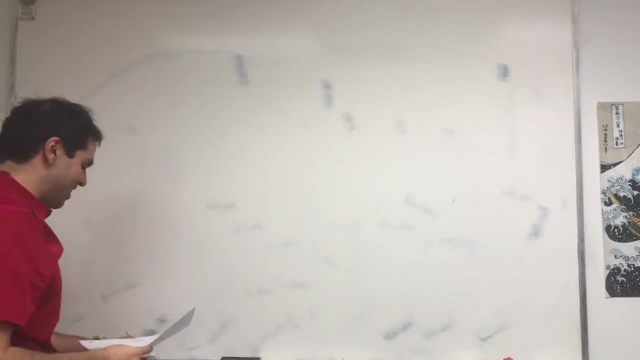 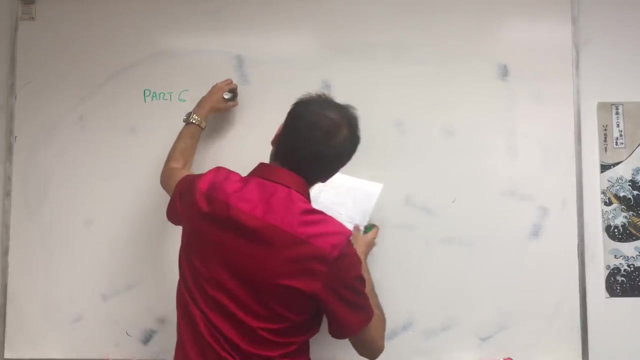 how important this theorem is. All right, congrats. we are done with the fifth part, and it's three, like three hours and 30 already elapsed. And now let's do well, orthogonality. so part six, Orthogonality and least squares. 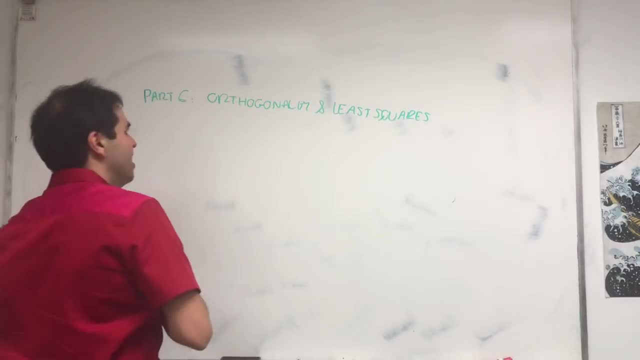 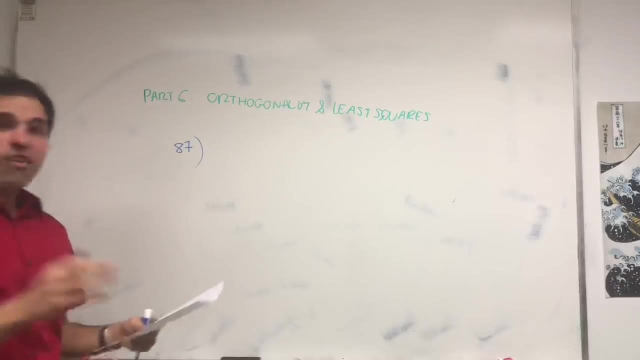 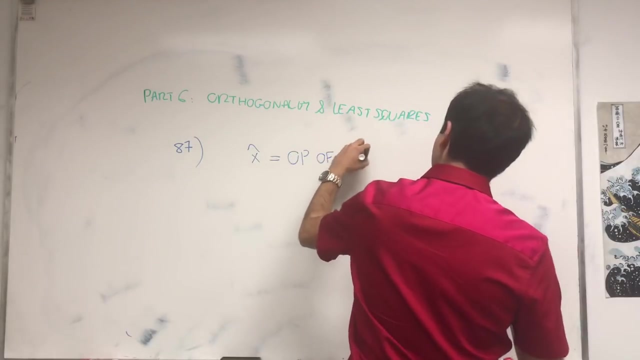 Oh my God, there's more than 20% left. oh, okay, All right. so first question, And whenever I write X hat- very important- it's an orthogonal projection of X on a subspace. Okay, so again, X hat will always be. 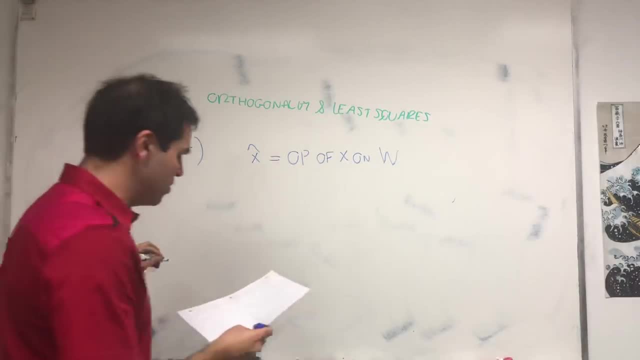 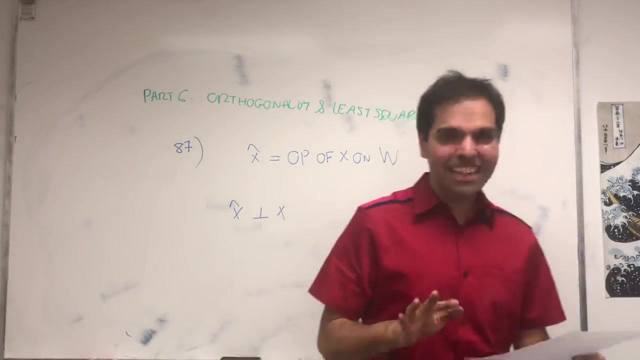 the orthogonal projection of X on a subspace W, And the question is: is X hat, is it perpendicular to X? Okay, 87th language: it's called Zulu And I think it's one of the craziest ones. 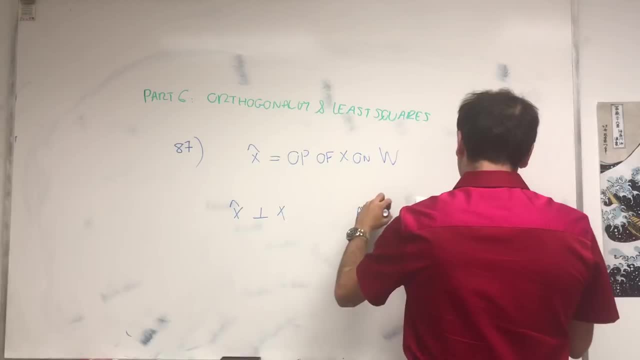 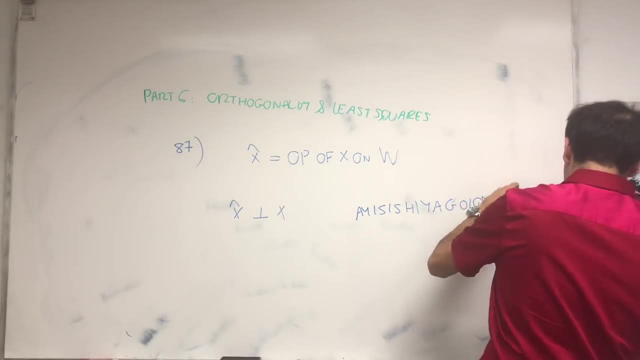 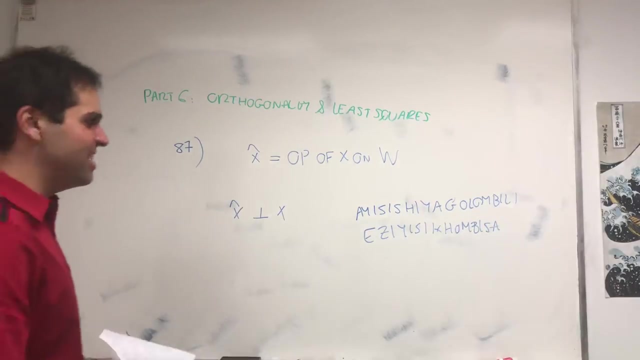 It's: let me, let me write that. So That's how you say 87 in Zulu. so Crazy, oh my God. It's weird because the language itself is short, It's Zulu, but you get stuff like this: 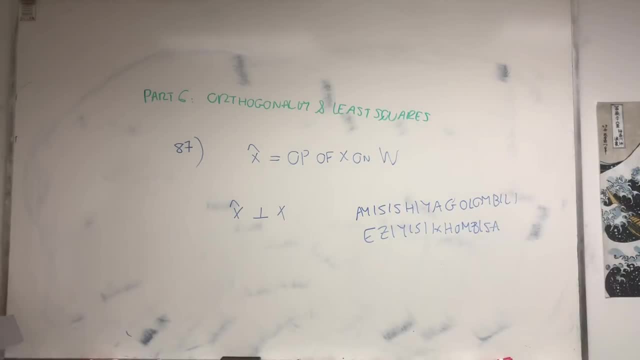 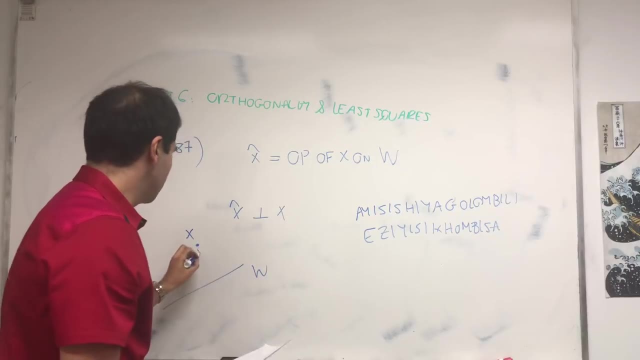 All right, and usually for those things it's good to just draw a picture. So suppose you have X and a subspace W and you project it to get X hat. Then let's see, are the vectors X and X hat perpendicular? 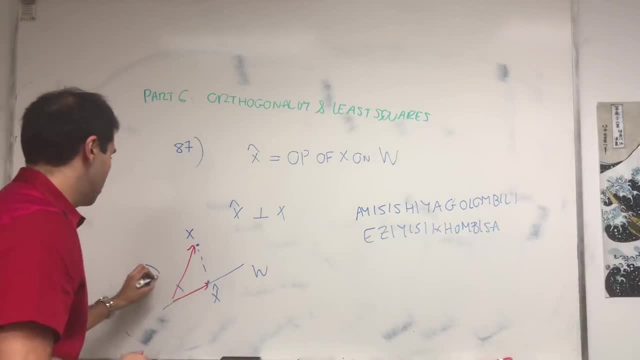 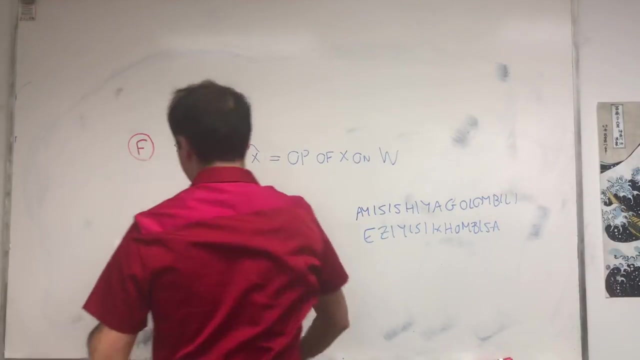 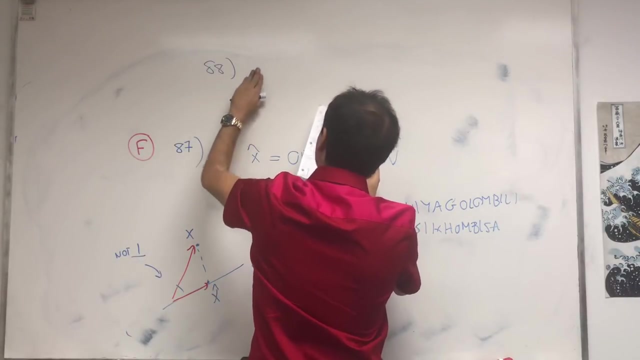 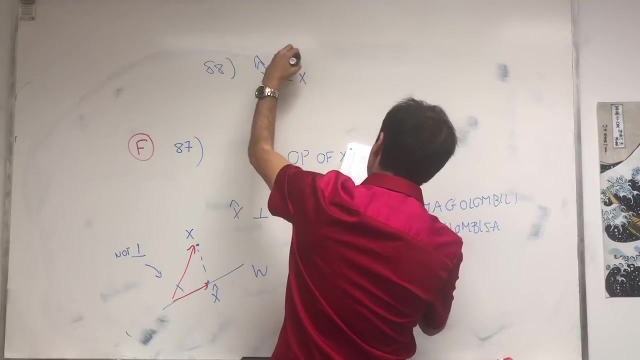 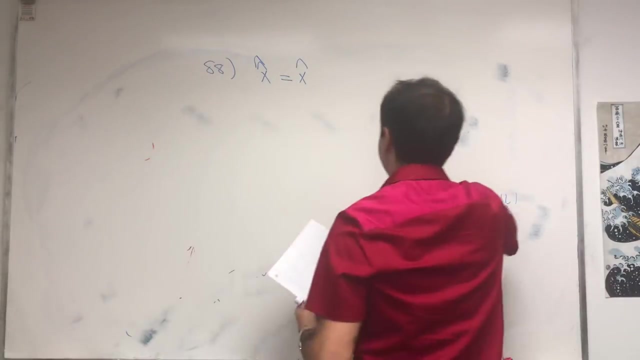 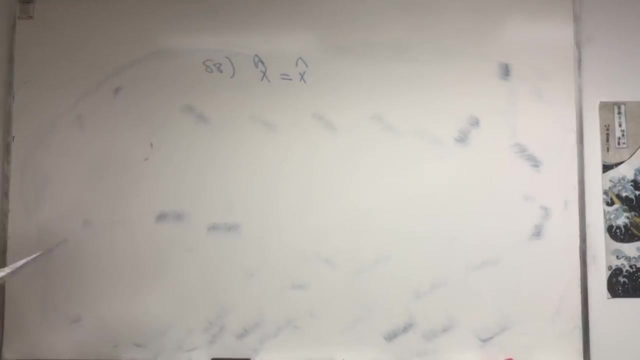 Well, not really. so they're not orthogonal, It is false. All right, talk more about this. so 88, I'm sorry 88- if you have project X on W and you project this again, do you just get X hat. well, let's see, so is true that X, hot hat is Xo checked and 88. so I think 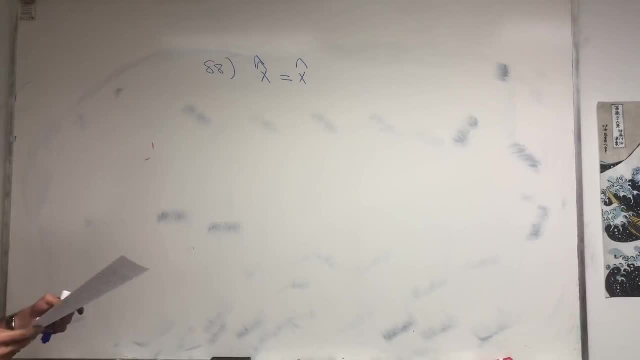 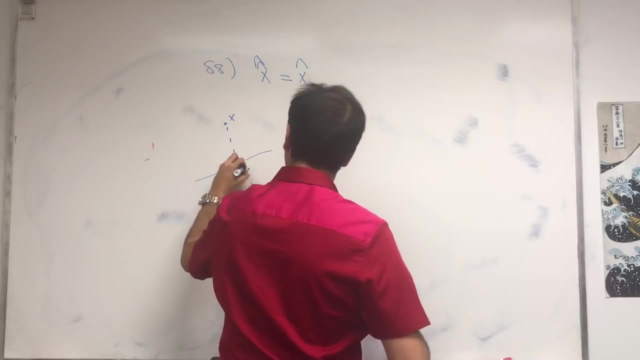 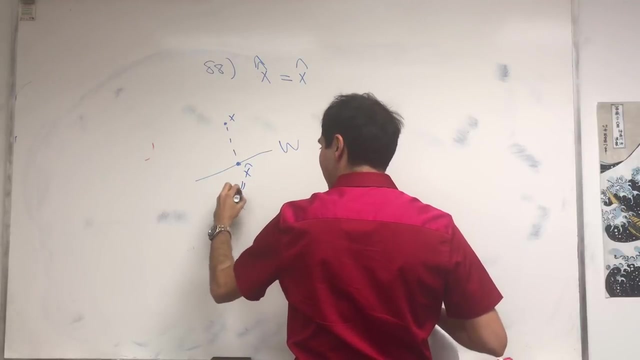 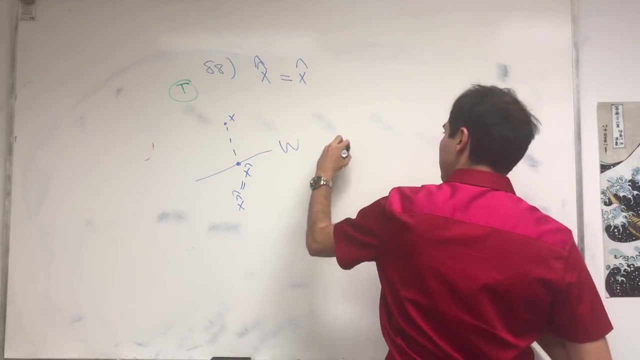 Bulgarian or Zendes said eOS, em. again, let's draw the picture. so this is x, this is x hat. well, if you take this and you projected again, then it's the same thing as xaf. it is true, and really the reason is that X hat is in W, so if you project, 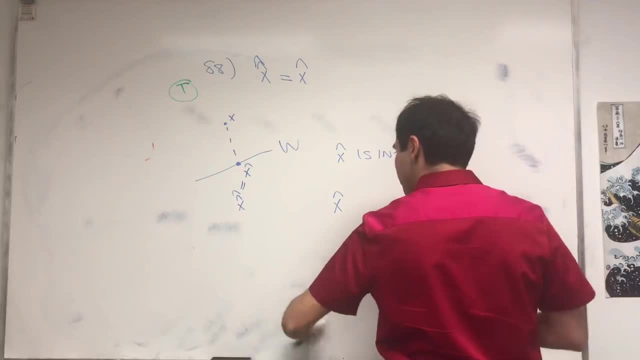 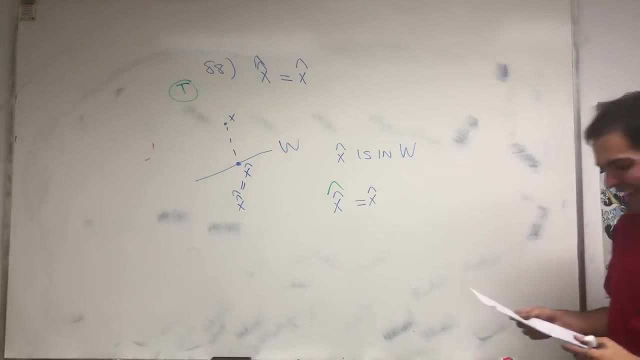 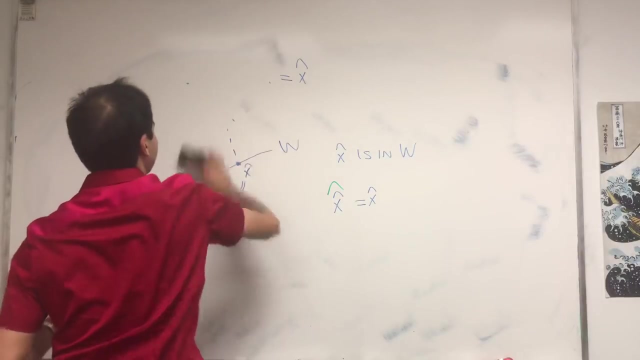 something in W, again in W, then you just get the same thing. so X hat hat equals to X hat lots of hats. but that's fine and okay. the next one is really cool. so I remember when I T8 for linear algebra we had this question and that's what. 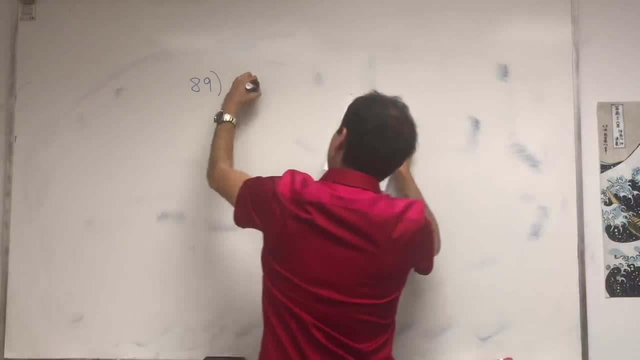 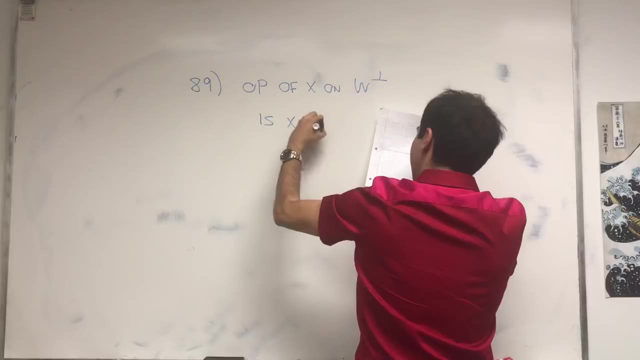 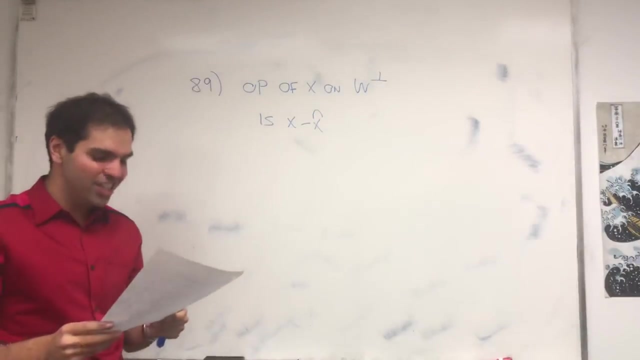 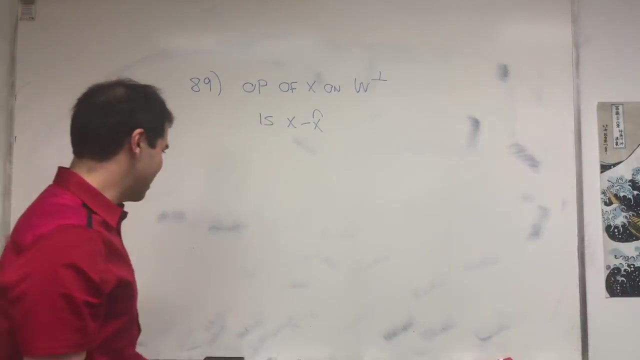 did. the picture is very important, so the orthogonal projection of X on the perpendicular space is just X minus X hat, so 89 Swedish, yeah, and then 89 in Swedish is at you know, you know, very cute, I should talk to you about that. I could talk to you Oreo, like that. 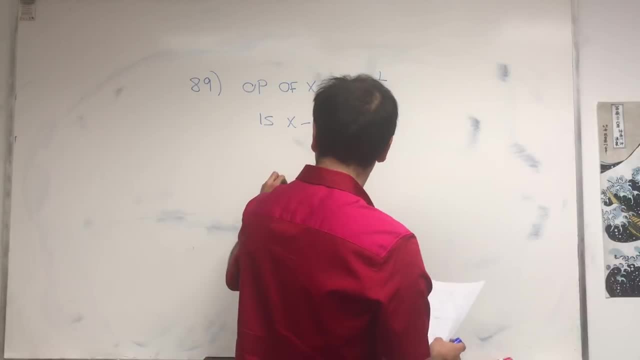 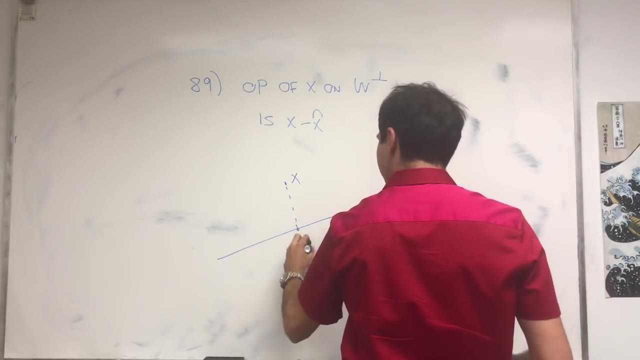 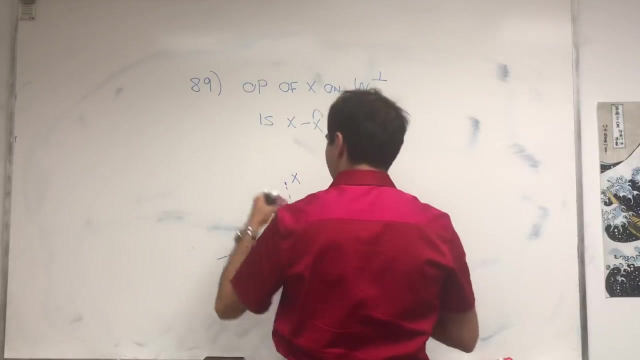 Oreo at your new, okay. so anyway, let's see, suppose you project X on W, then you get X hat. what is W perp? so W with this hat it's the space that's perpendicular to W, so that's W perp, anything that's perpendicular to any vector in W, if you. 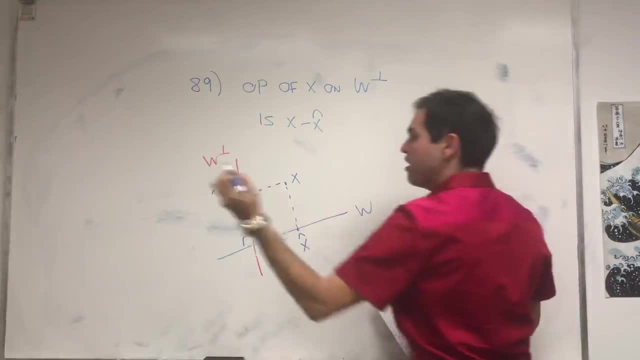 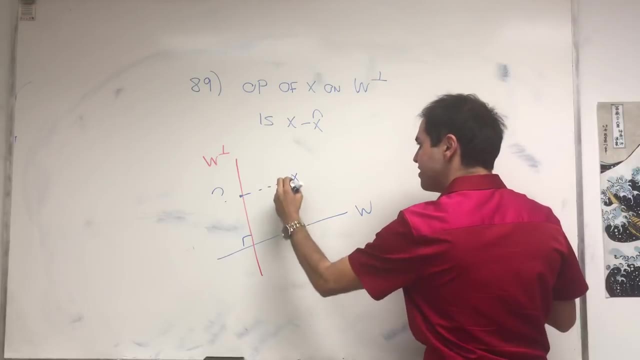 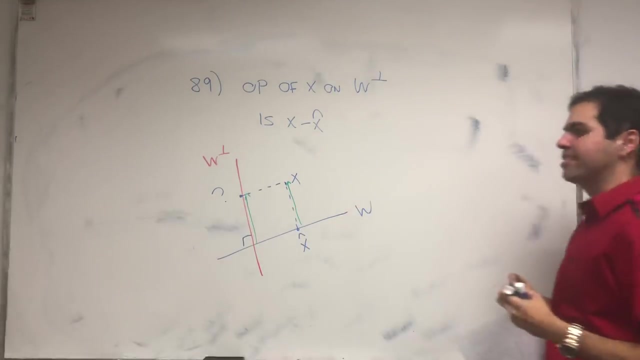 squish X on this w perp, you get whatever our answer is. And the question is: is our answer x minus x hat? Well, look, x minus x hat is this vector. but because parallel vectors are equal, it's actually the same thing as this vector, so it is the same. So x minus x hat and x minus x hat. 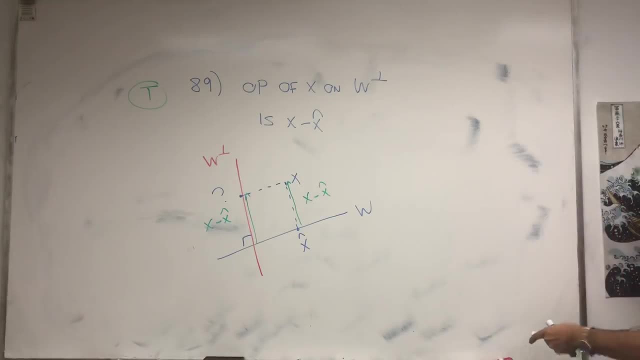 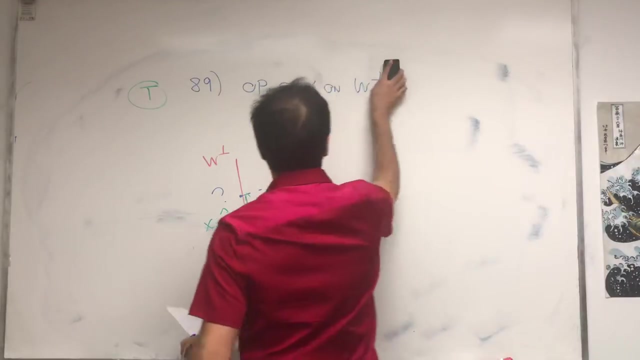 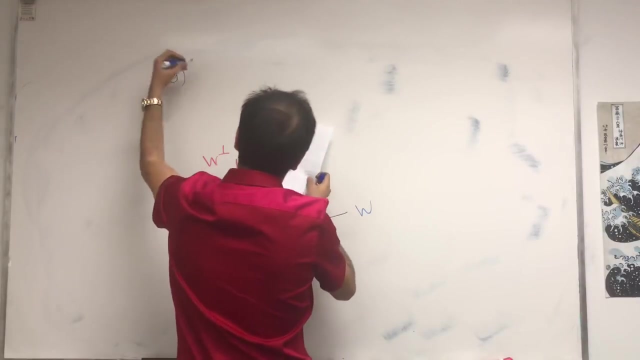 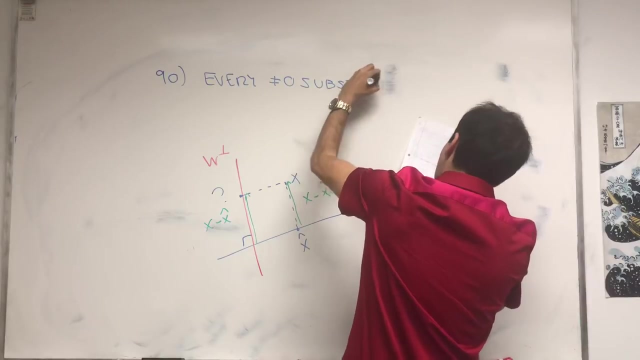 So, indeed, this is true. Cool huh, I like this question. Now next question. Well, orthonormal basis is nice, but is it true that every non-zero subspace has an orthonormal basis? Yes, Since—. 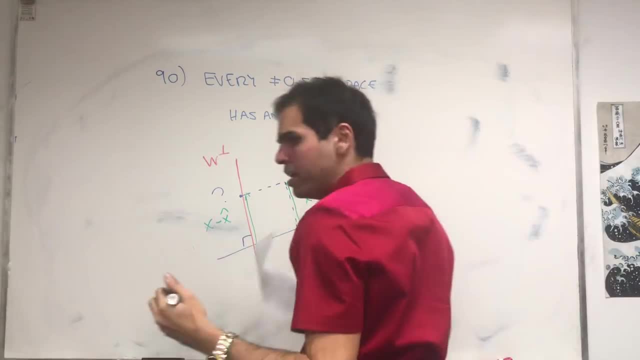 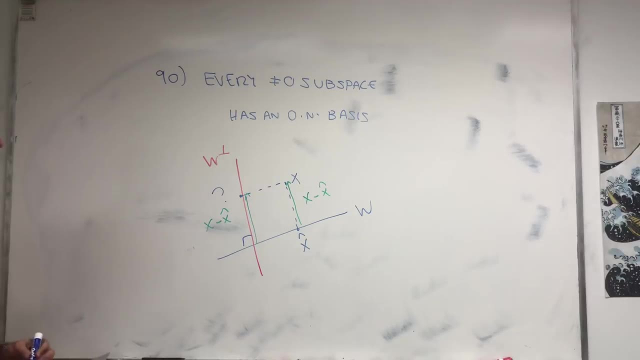 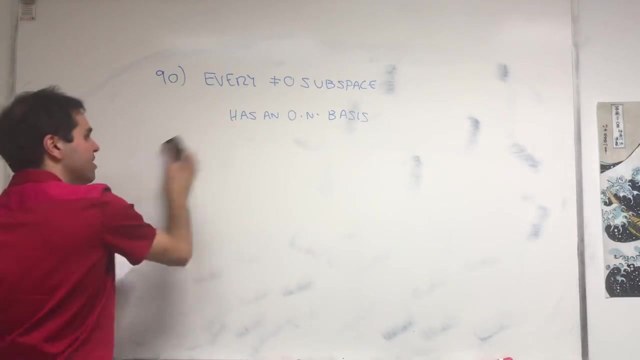 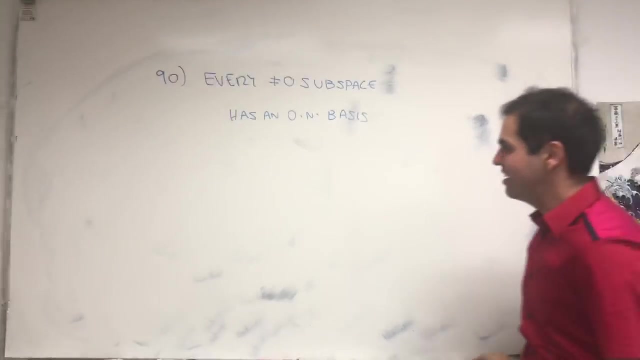 Yes, So orthonormal means the length of each vector is one and the different vectors in that set are perpendicular. Ninetieth language: oh, Lombardi. right, So the Lombard version of Italian, and it was, it's in Italian- 90 is novanta. 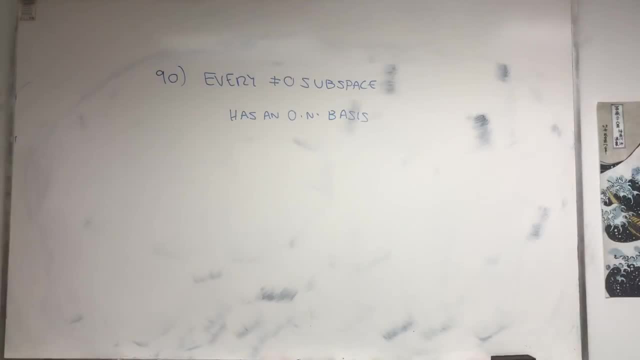 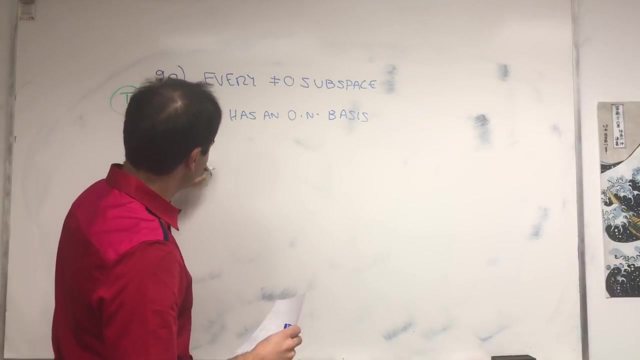 Andiamo. Okay, and indeed this is true. and how do you find this? Well, first of all, every non-zero subspace, or in fact any subspace, has a basis. So find a basis and the process to make this orthonormal, that's called the Gram-Schmidt. 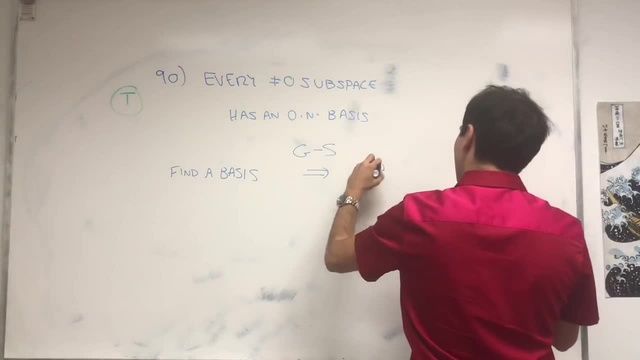 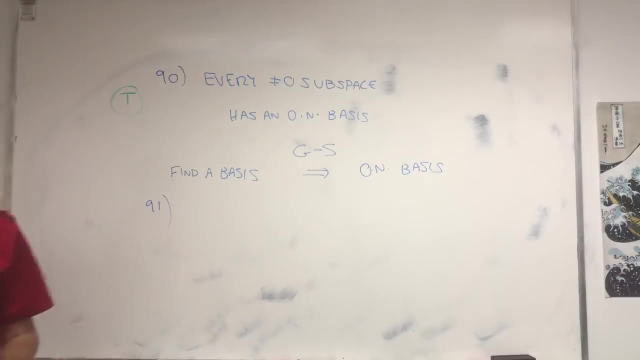 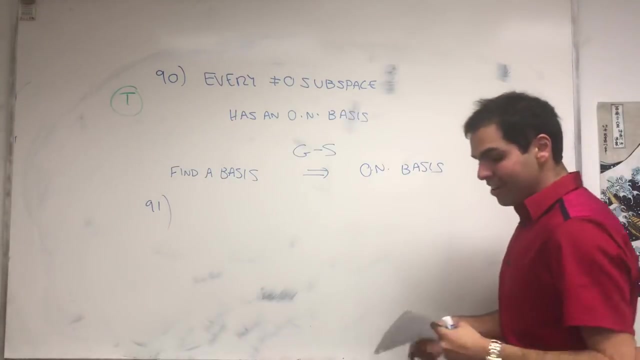 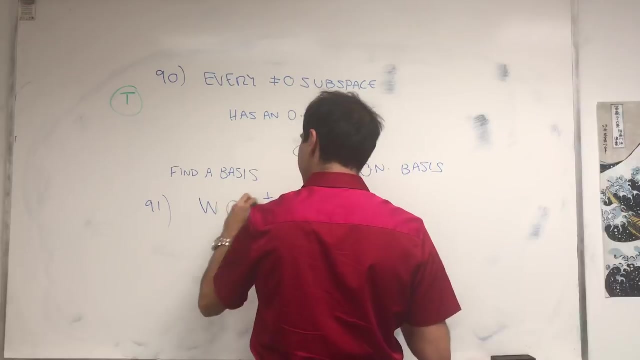 process. So apply the Gram-Schmidt process to get an orthonormal basis. That's why Gram-Schmidt is so useful For any basis. you get an orthonormal basis and we're still alive, very good. Next question: so consider W and its perpendicular space. do they just have a zero intersection? 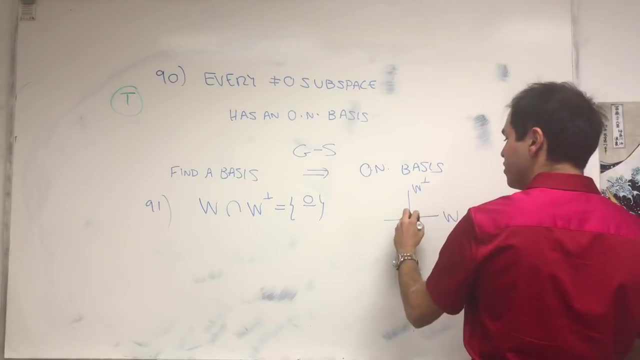 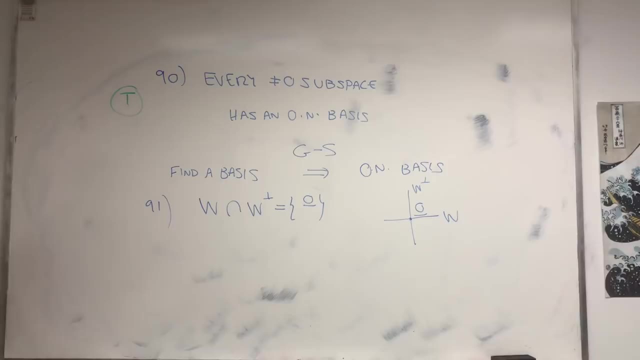 So, in other words, if you have a subspace and you have a perpendicular space, do they just intersect in the zero vector? Okay, And 91st language is the western part of Oromo and it's Toko-Sagartama, Toko-Sagartama. 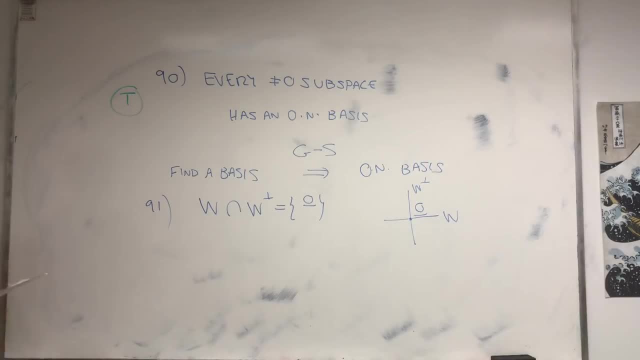 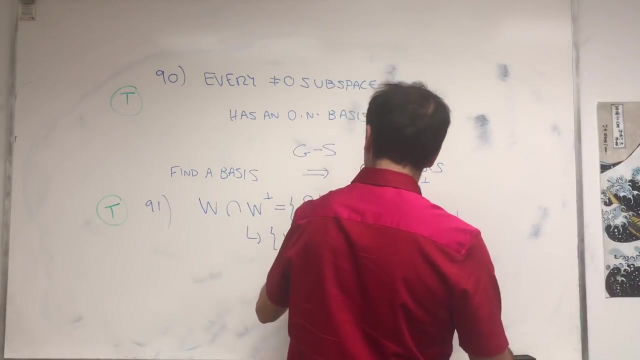 And at least in the picture, that is true. so it turns out, it is true. and what is W perp? Again, it's the set of vectors that are perpendicular to every vector in W. So yx, yx and yx. 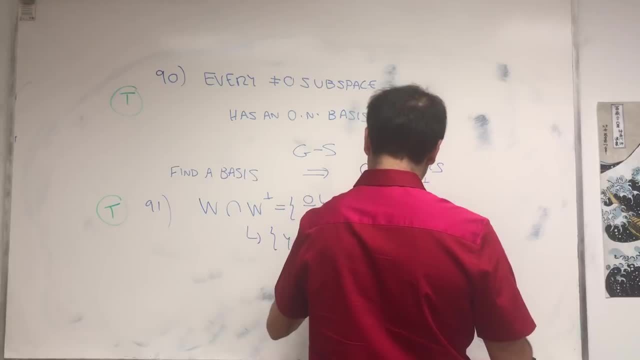 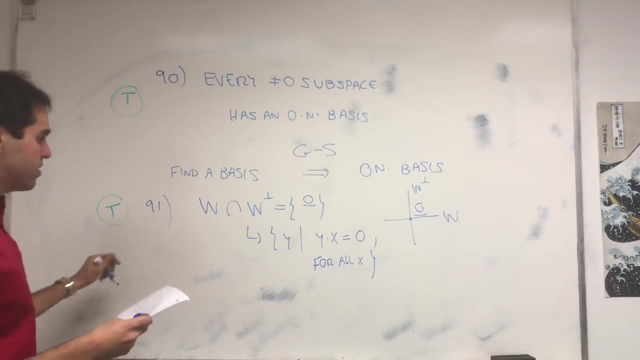 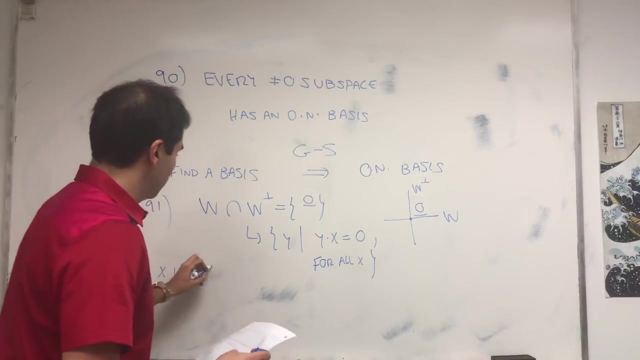 So yx is zero for all x. Okay, now suppose x is in W, in W. So suppose, I guess. suppose x is in W, intersect W perp, then x is in W and x is in W perp. 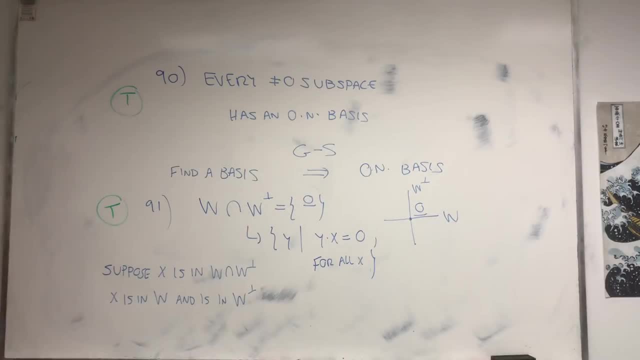 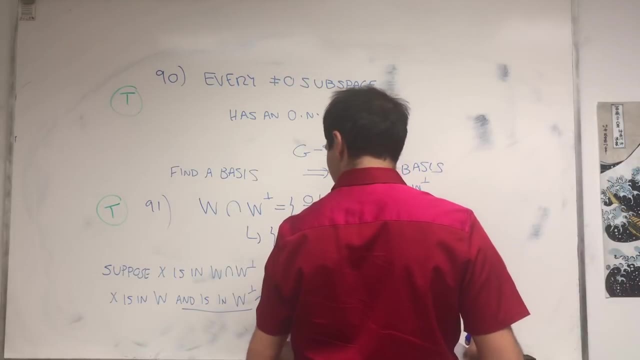 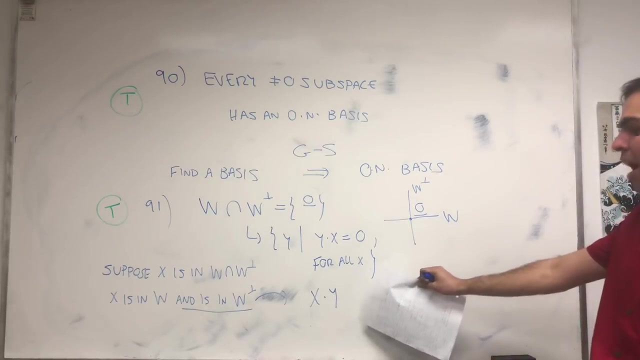 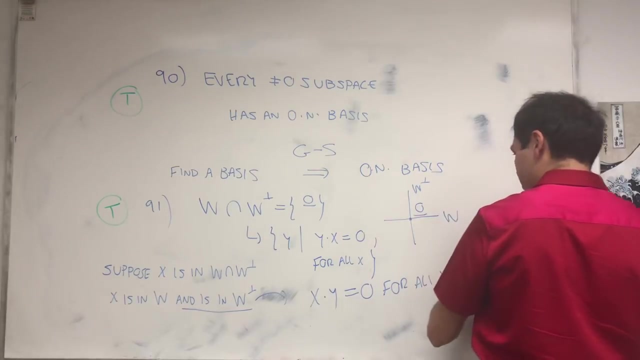 Now, Okay, Okay, So x is in W perp. That means x dotted with y. sorry, yeah, maybe I mixed this up, but look, Because x is in W perp, x dotted with y equals to zero for all x. sorry, for all y in W. 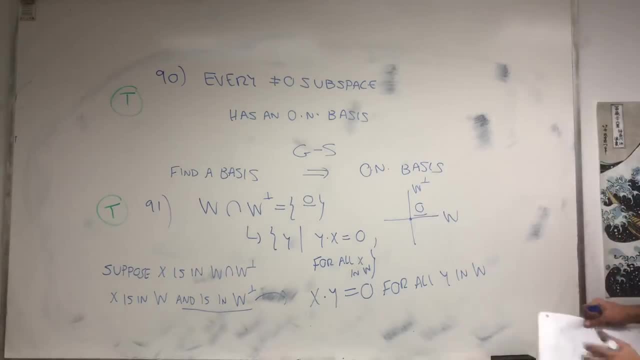 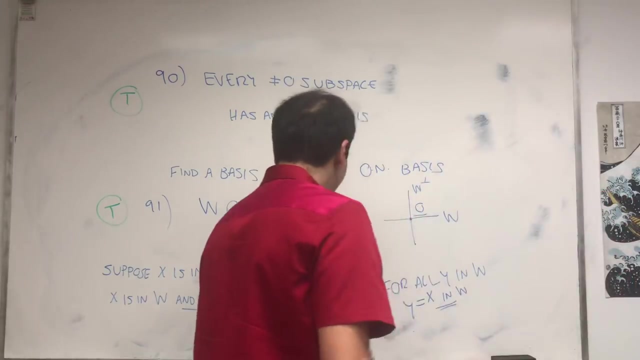 That's of course in W. Okay, So x dotted with y equals zero for all y in W. But now, because x itself is in W, you can take: y equals to x in W And therefore x dotted with itself is zero. 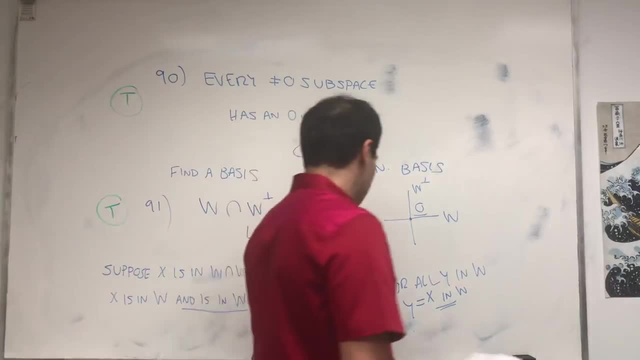 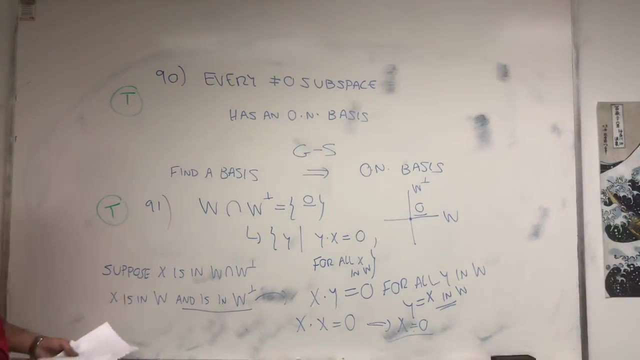 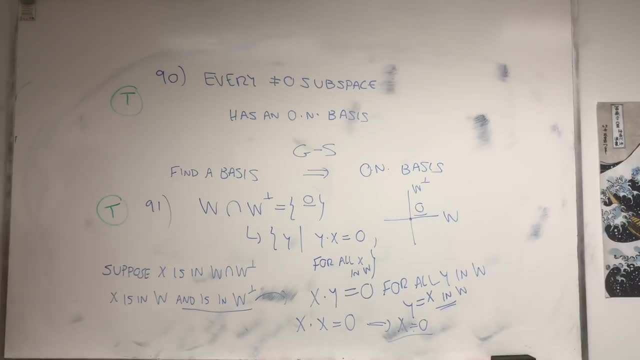 So it is indeed true that if you have an element in the intersection, then the element is zero, And that is because if x is in W perp, it's perpendicular to everything in W. In particular, it's dot perpendicular to itself. 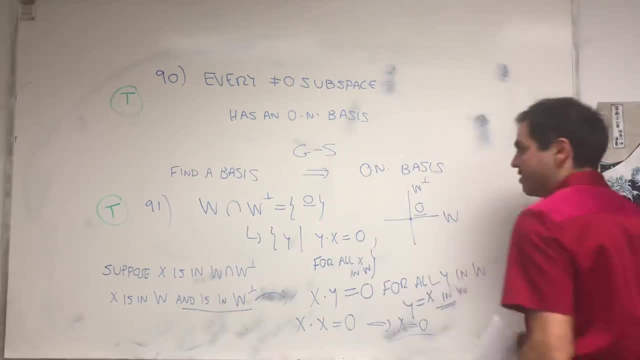 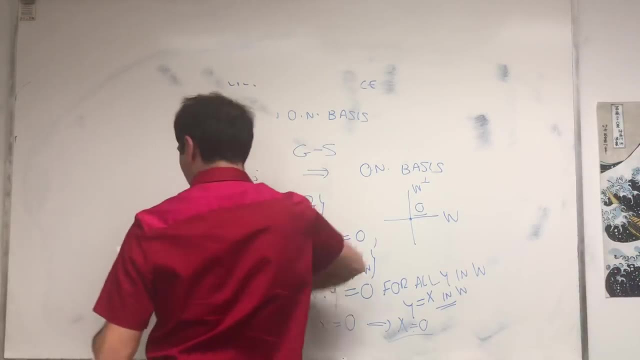 Because itself is in W, and then this just means that the vector itself was the zero vector. Okay, Now let's talk a bit more about orthogonal projections. Okay, Okay, Okay, Okay, Okay. So the next couple ones are more proofy. 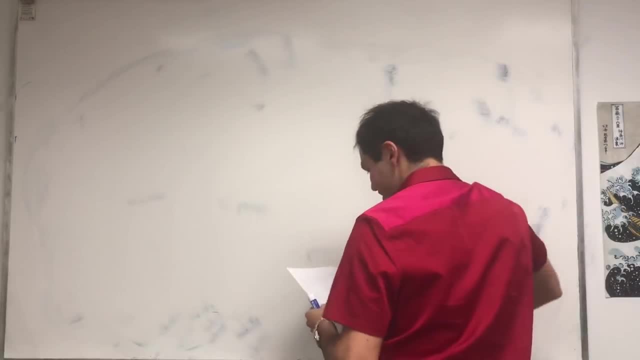 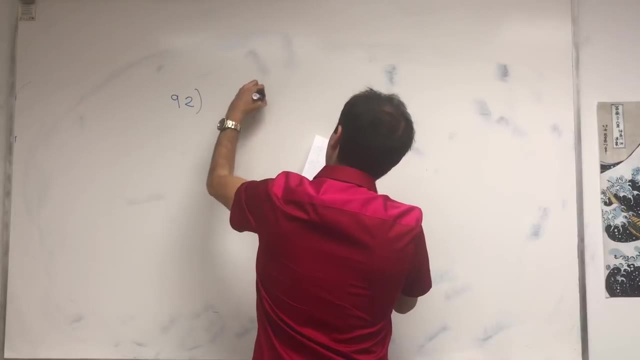 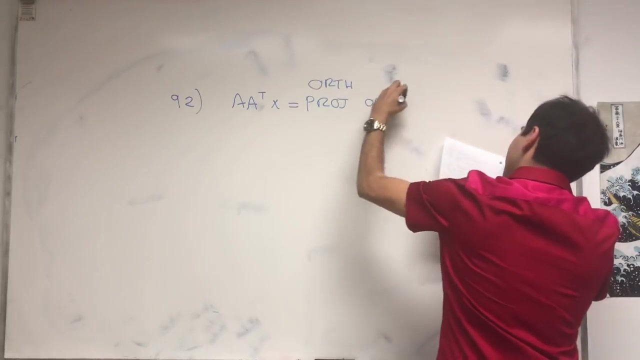 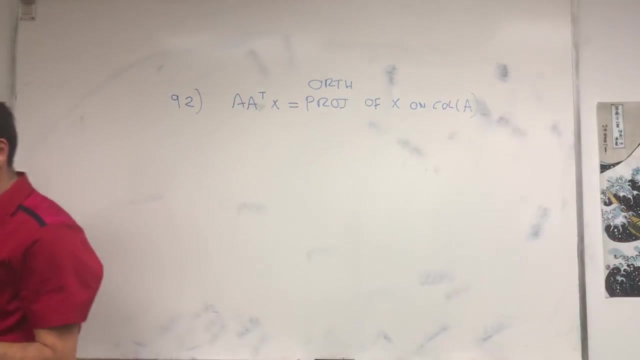 All right, 92. A: A transpose: x is a projection, so the orthogonal projection of x on the column space of A And 92nd language is Pashto, south, I think, And it's Do He Interesting. 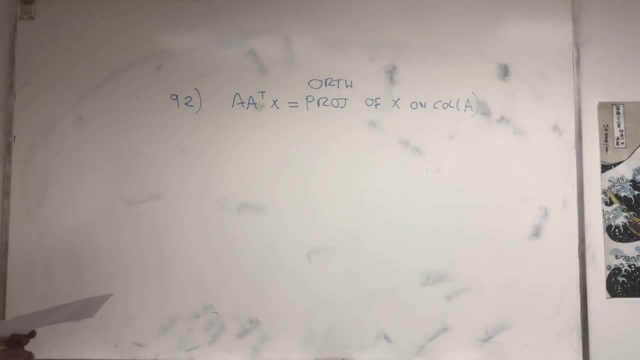 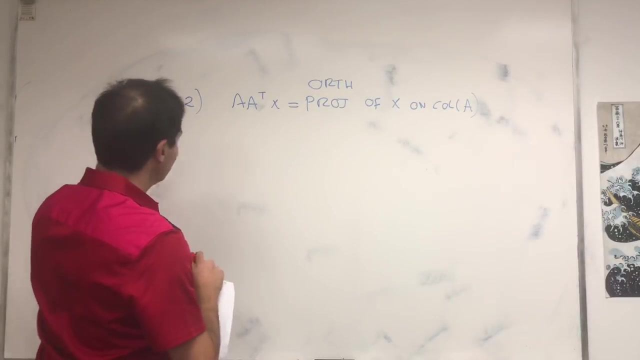 In Farsi it's and here is, So it sounds similar. So, in other words, if you want to calculate the projection of x on a bunch of vectors, you just do A, A transpose of x, And unfortunately the answer is false. 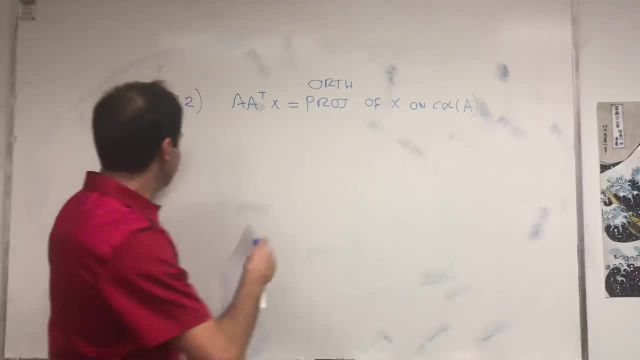 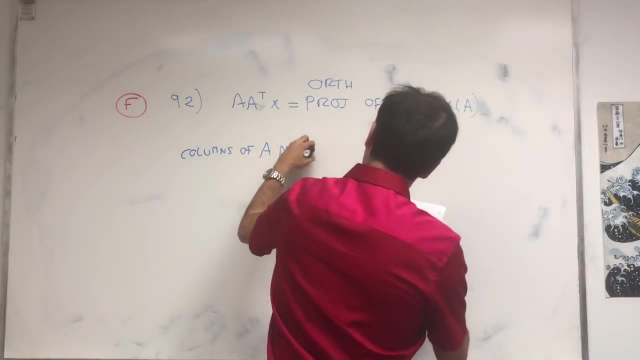 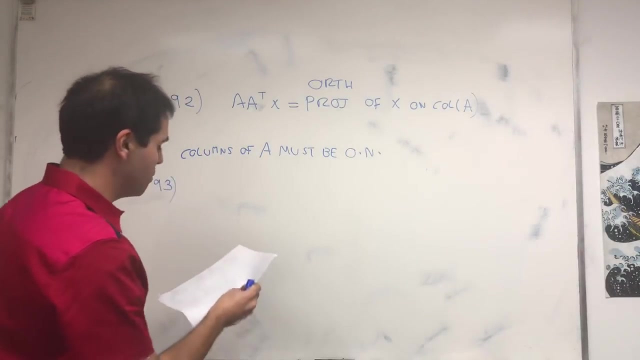 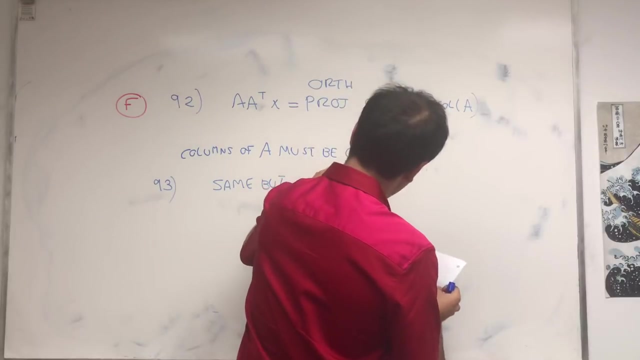 Because it turns out you need the columns to be orthogonal. So columns of A must be orthonormal, And let me explain to you why it's true, so why they have to be orthonormal. So same, but columns of A are orthonormal. 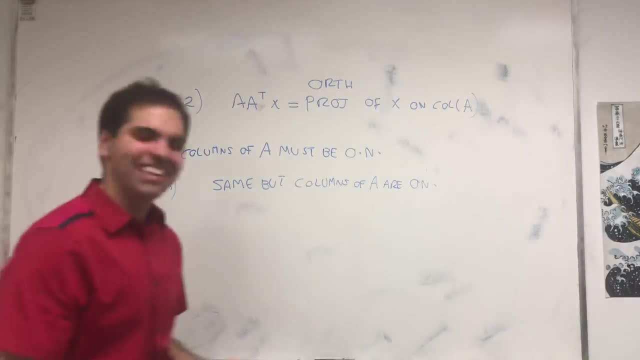 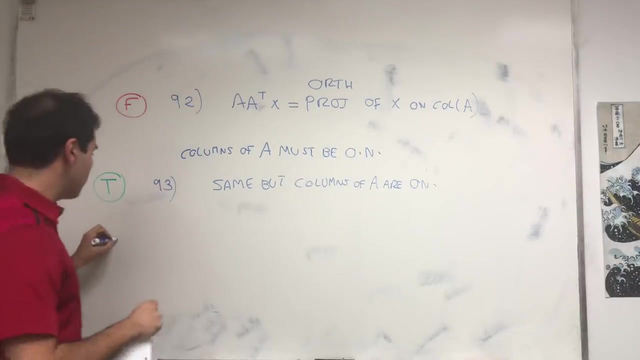 And 93rd language in honor of Borat, is Kazakh and it's Kazakhstan greatest country in the world. And, of course, the way I phrase this question. it is true, And let me show you why. So let's calculate A. A transpose x. 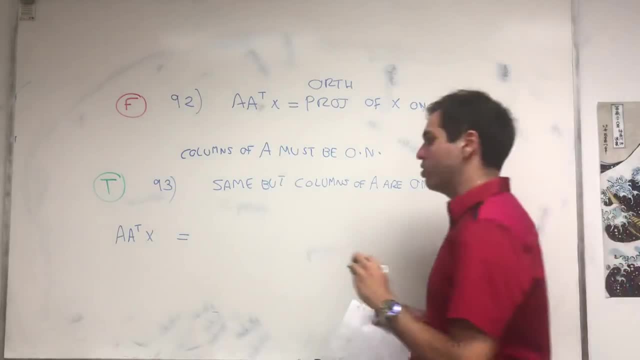 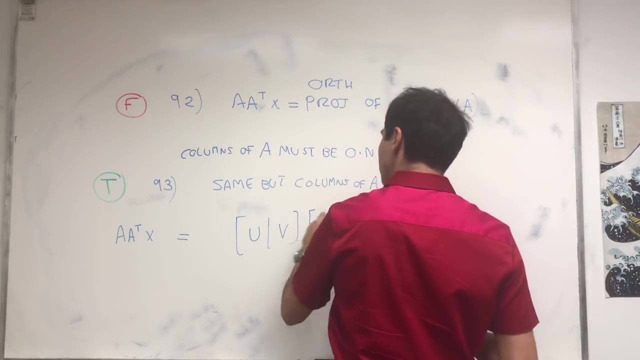 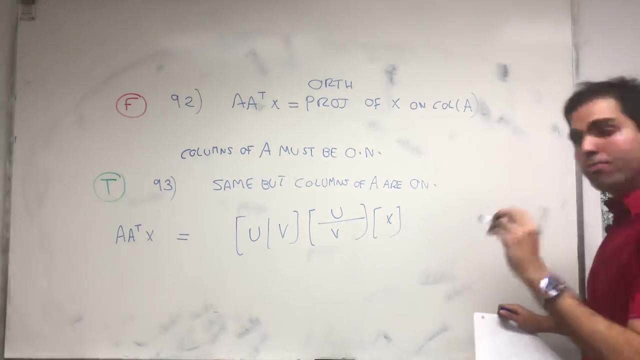 And for simplicity, assume A has two columns, Of course for any number of columns. So A is uv And then A transpose: well, it's uv, but as rows, And then x is x. Now remember, if you multiply a matrix by a vector, it's the same as just taking the dot product. 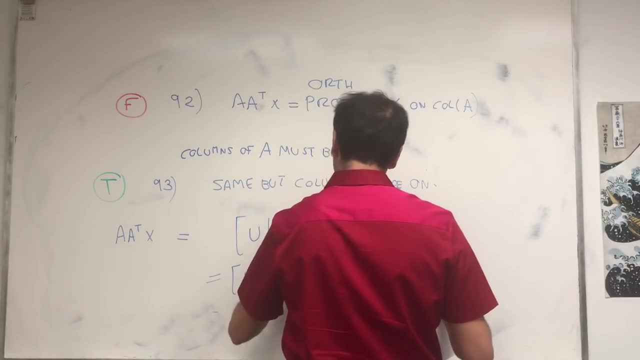 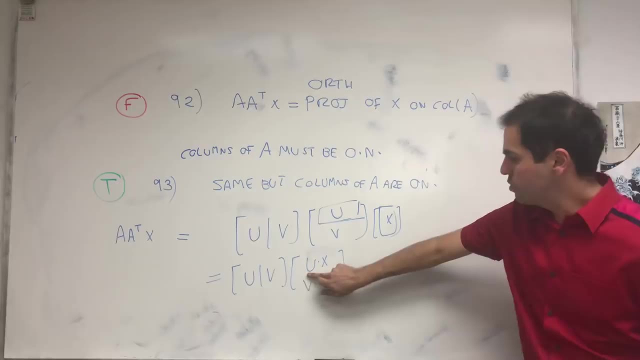 So this becomes uv, and then u dotted with x and v dotted with x. That's one thing. Those are just numbers. so it's just a 2 by 1 vector. And then remember, if you multiply a matrix by a vector, 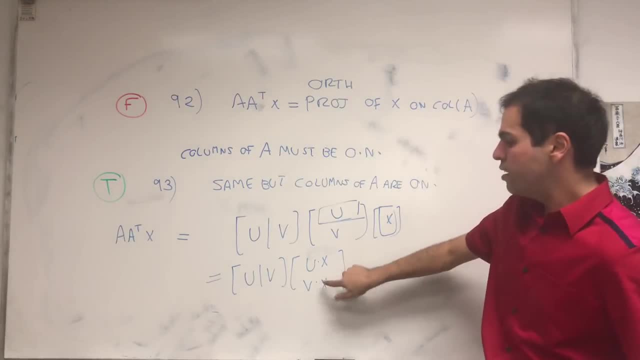 it's just: you take the linear combo of u and v, but with those two values, So it becomes u dot x times u plus v, dot x times v, And you can write this as x dot u of u plus x, dot v, dot v. 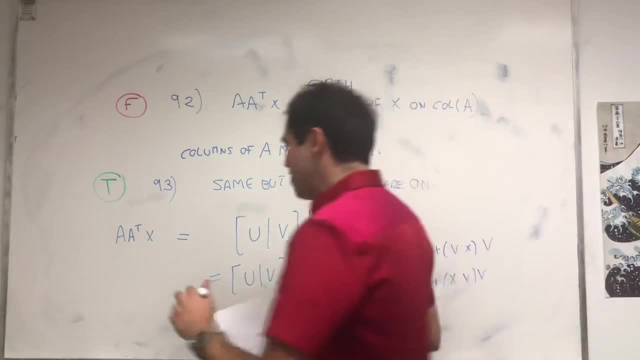 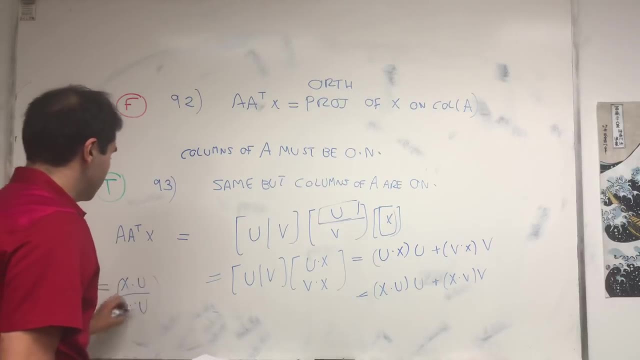 All right, This almost looks like x hat. Remember the formula for x hat is a hugging formula, So you just hug x with u and u hugs itself u, And x dot v over v, dot v, v. First of all, this hugging formula only works if u and v are perpendicular. 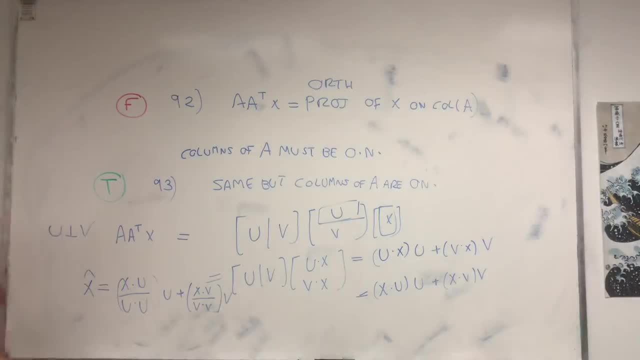 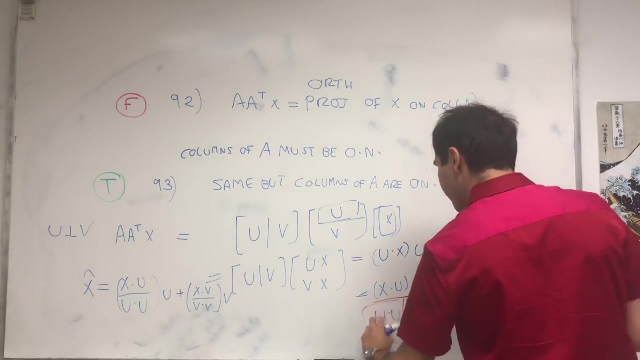 So one thing is you already need that the columns are orthogonal. That's one thing. Also, look at those two formulas. Well, they're almost similar, Except you need a u dotted with u, In particular, if this is 1 and this is 1,, then we do get the same thing. 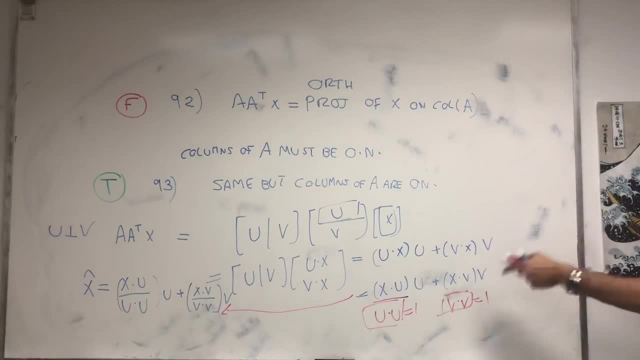 We do get that. it's x hat And therefore we also need the columns to have length 1.. So not only do we need u perpendicular to v, but we also need the length of u to be the length of v to be 1.. 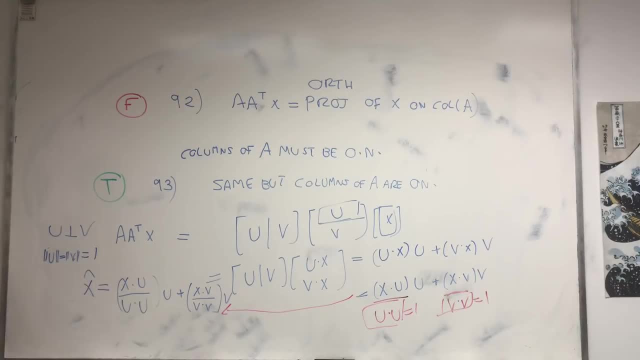 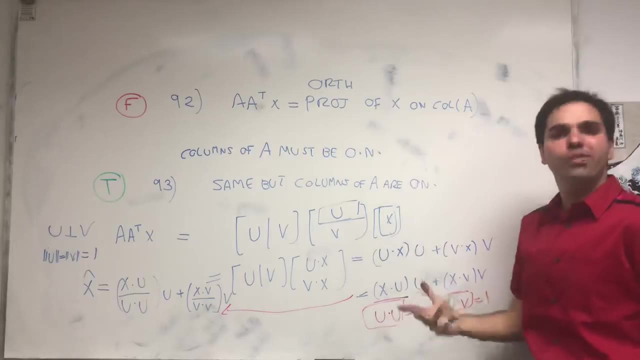 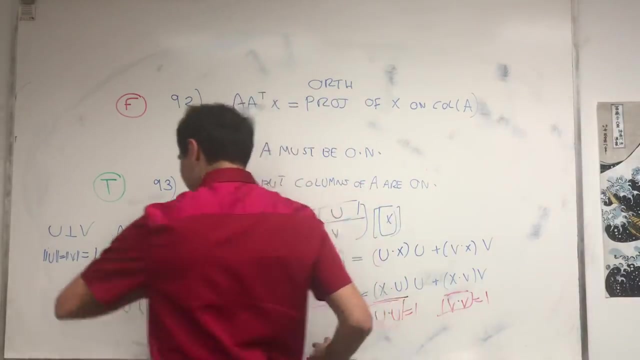 So in particular, the columns of a must be orthonormal for a, a transpose x to be x hat. And that's why we usually write q, q transpose, to make sure that the columns of q are orthonormal. So that's why that's important. 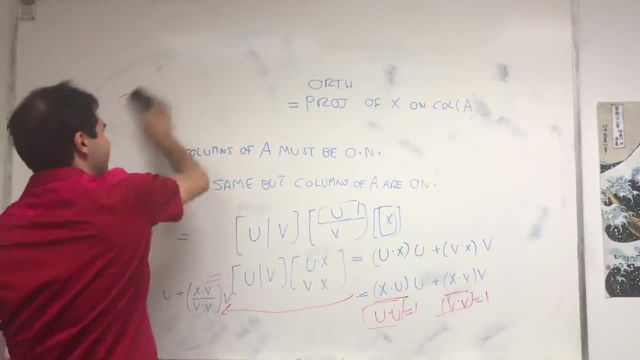 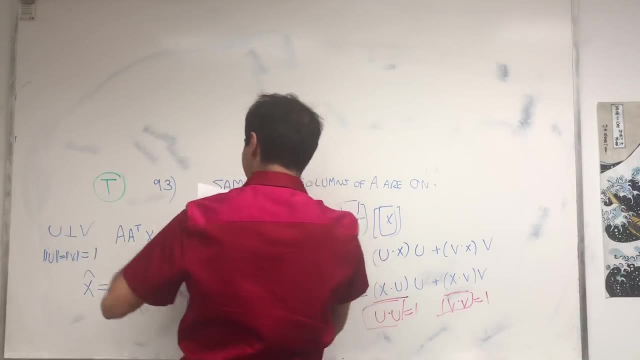 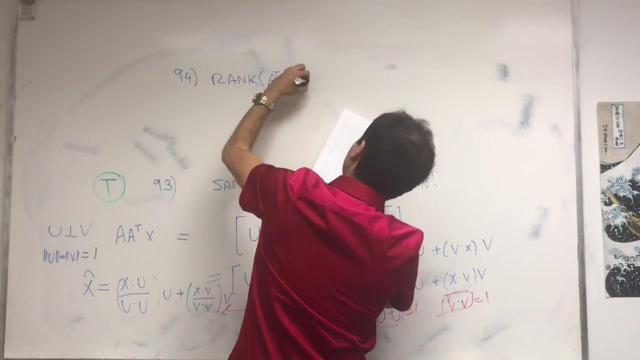 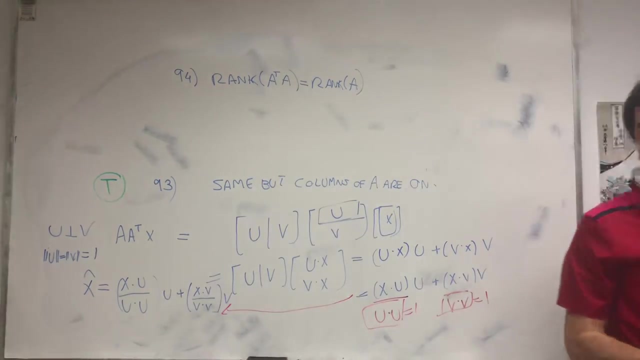 OK, Next one, Thank you. Next Question 84.. 94, actually, Ooh, Is it true that the rank of a transpose a equals to the rank of a, Which might be surprising because, remember, we showed that the rank of a squared is not the same as the rank of a. 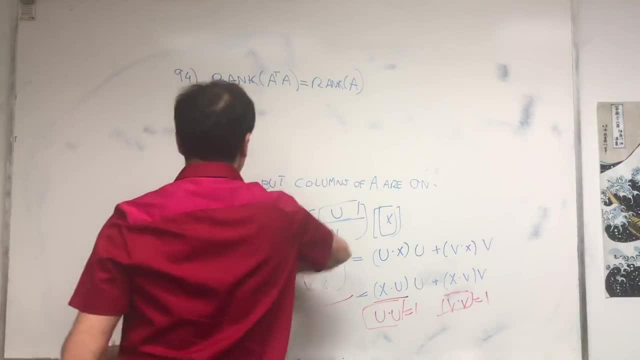 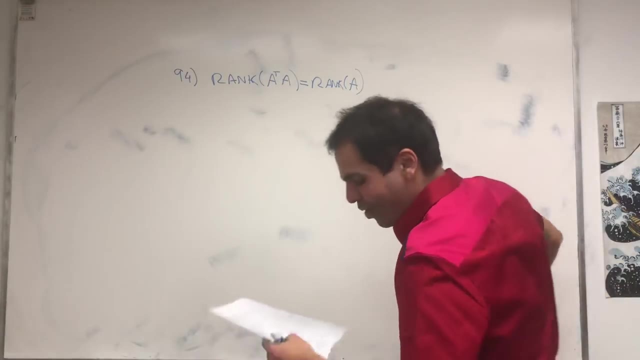 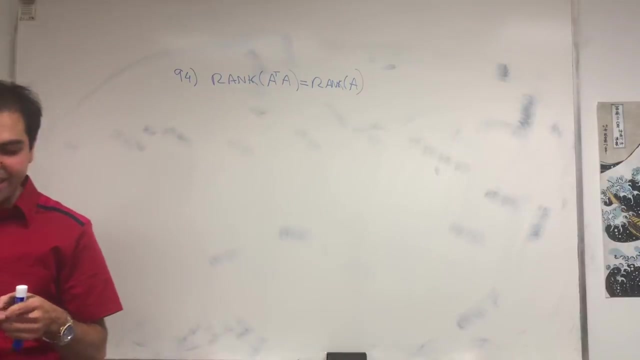 So let's see if it's true for a transpose a And my back OK. 94th question: So it's ilogano. So 94th number is ilogano. Sorry, And it's siam apulo ket upat. 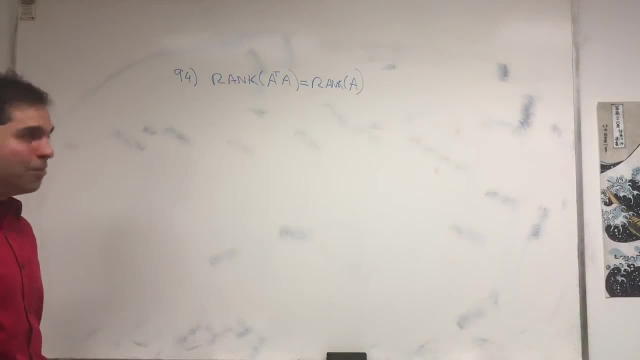 OK, Now, even though the rank of a squared is not the rank of a, turns out, it is true that the rank of a transpose a is the rank of a. That's what makes least squares kind of work. So that's why, if the column of a is a, 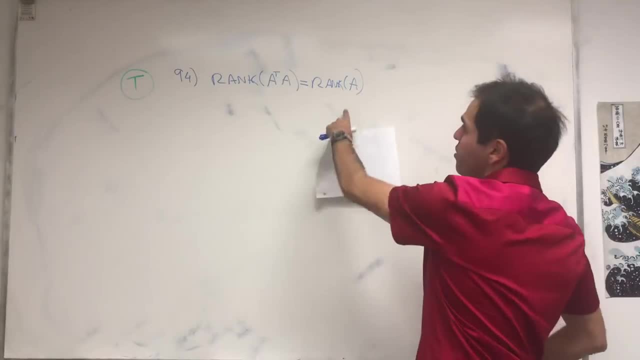 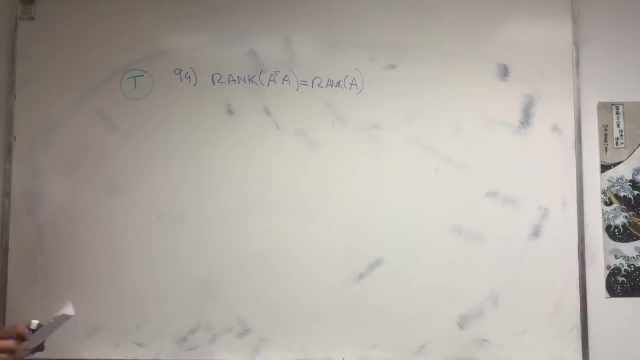 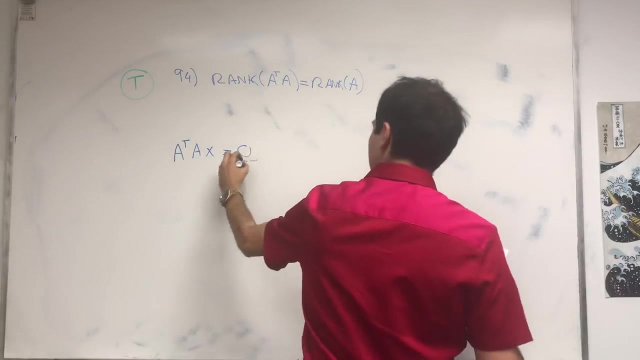 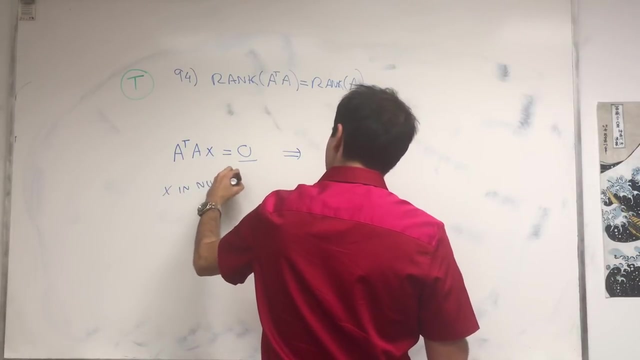 if the columns of a are linearly independent, a transpose a is usually invertible, And here's why Let's talk about null spaces first and you'll see why we do that. So if a transpose a, x equals 0. So if x is in the null space of a transpose a, 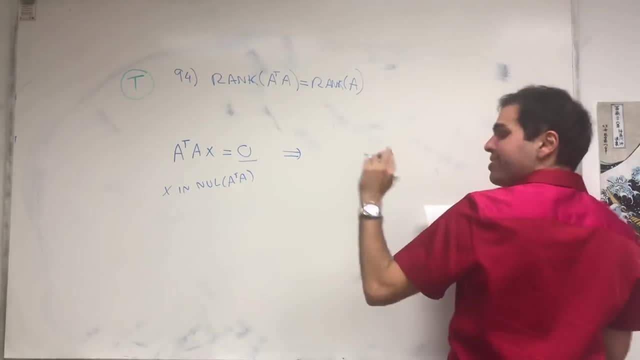 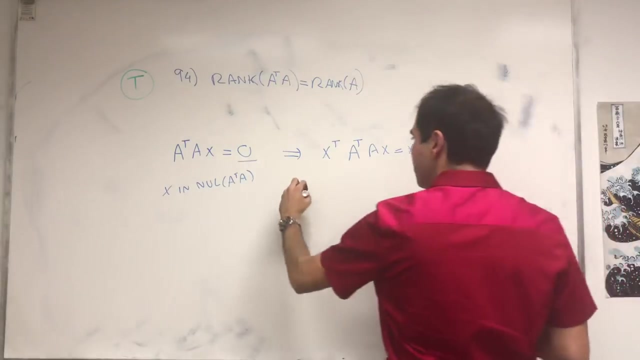 then a transpose a x equals 0.. Now let's just do something fun. Let's pre-multiply this by x transpose, So x transpose a transpose a x is x transpose 0. But that's just 0.. Anything times a 0 vector is 0. 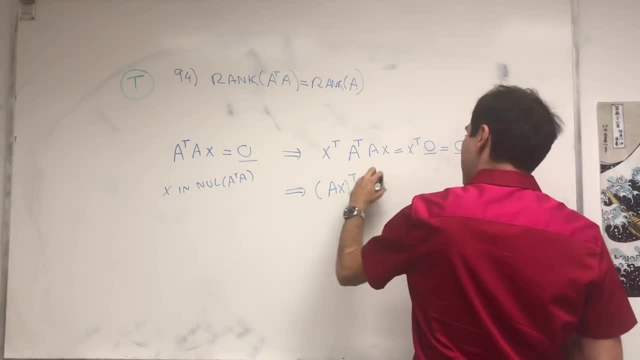 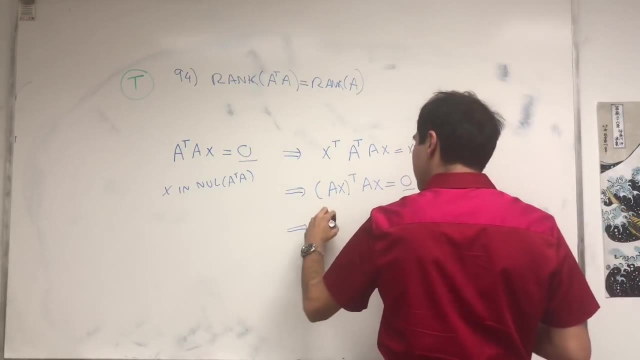 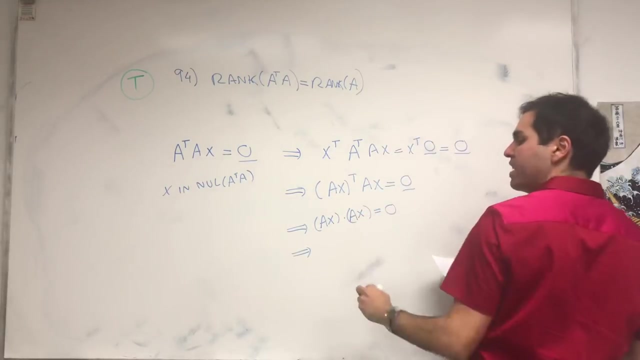 But now we can write this as a x transpose a x equals to the 0 vector, But x transpose y is just x dot y. So a x dotted with a x equals 0.. So and the only way a vector dotted with itself is 0. 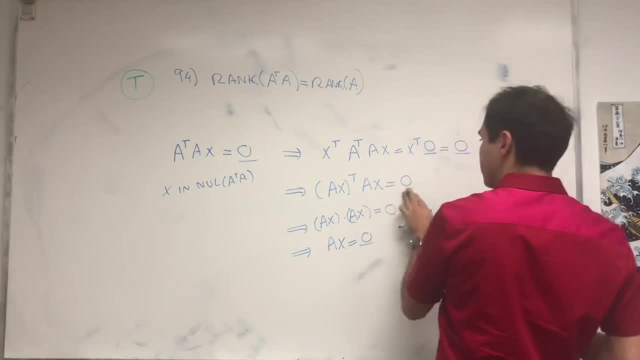 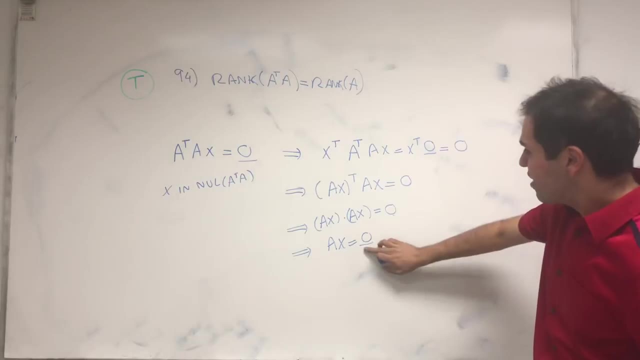 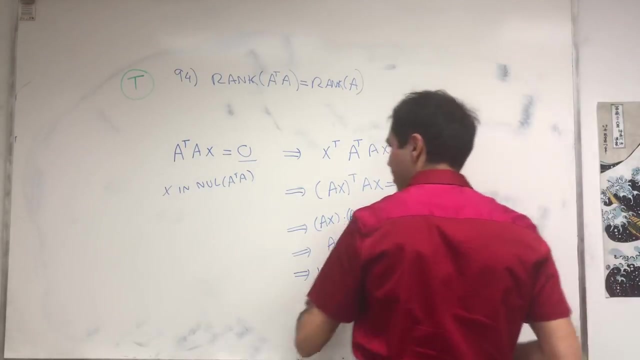 is if a x equals 0.. Oh, maybe that should be. you know something like that. That's me OK. good, And in particular, this means that x is in the null space of a. But here's the thing. 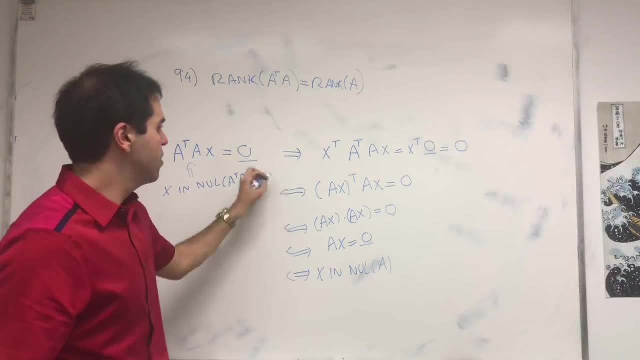 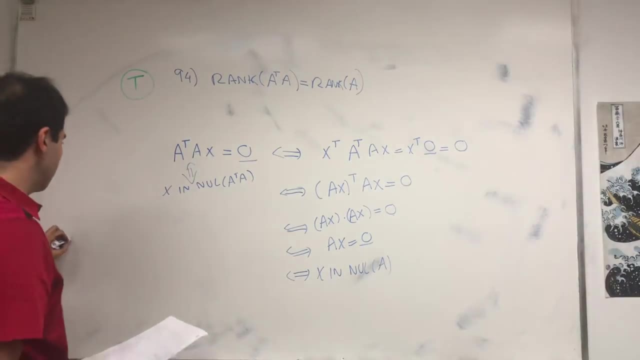 We can just reverse all the steps, So everything is reversible. And in particular, if x is in the null space of a, then x is in the null space of a transpose a, So in fact the null space of a transpose a equals. 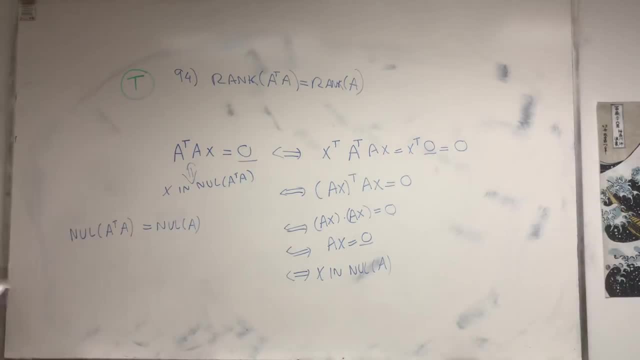 to the null space of a. And why is that important? Because now we can just use the rank nullity theorem. So rank of a again is n minus the dimension of the null space of a, And again a is an m by n matrix. 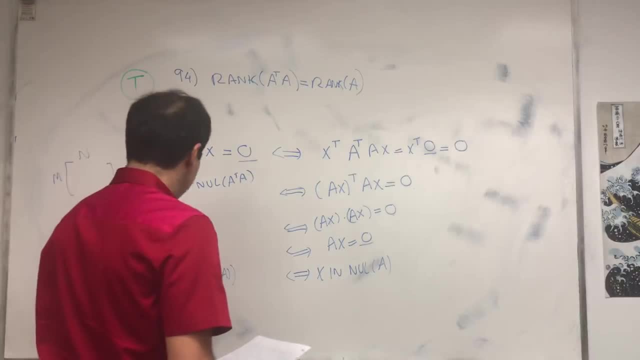 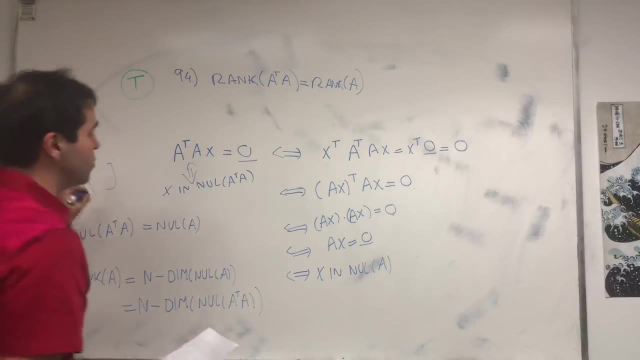 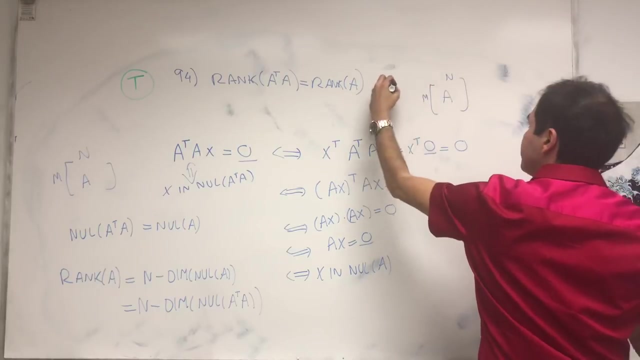 And that's n minus the dimension of the null space of a transpose, a. Now let's look. So let's see if I have space. So a is an m by n matrix And let's see a transpose is. this is m and this is n. 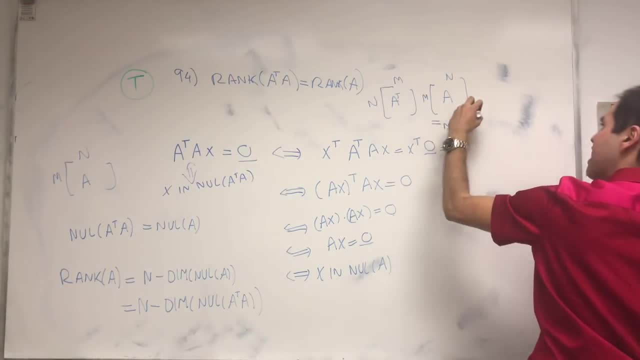 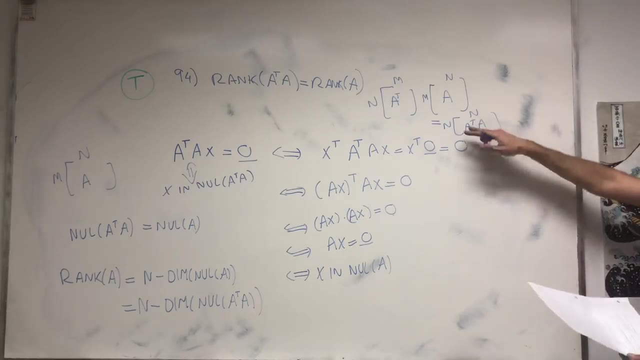 And so if you multiply the dimensions, you actually get an m by n matrix. So a transpose a has columns of size n. Well, of size n it has n columns. So in fact we can now apply the rank nullity theorem. 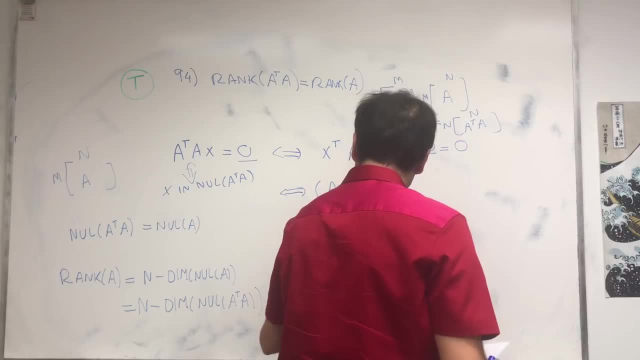 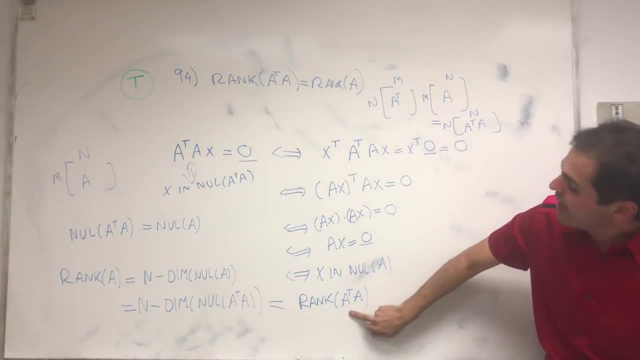 to a transpose a And you get rank of a transpose a, A transpose a. I don't know what that even means, But the rank of a transpose a is then equal to the rank of a. So it is true by a cute, you know, rank nullity theorem thing. 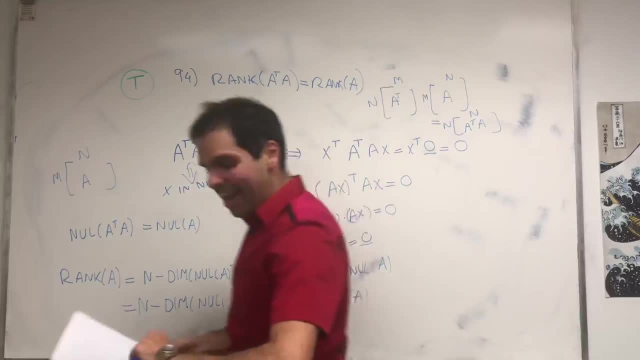 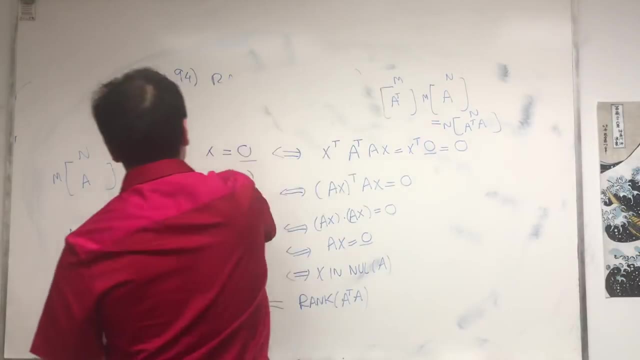 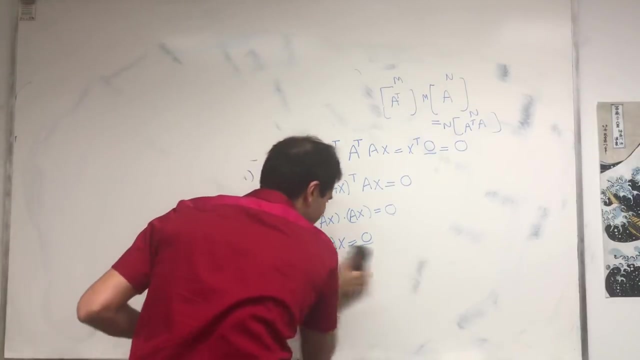 And by this cute calculation: OK, Only two and a half pages to go And then we're done. I can congrats if you've been looking at it so far, But wow, I'm impressed. Well, I hope you took breaks. 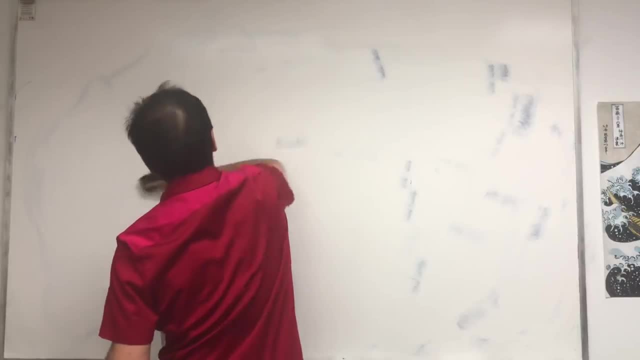 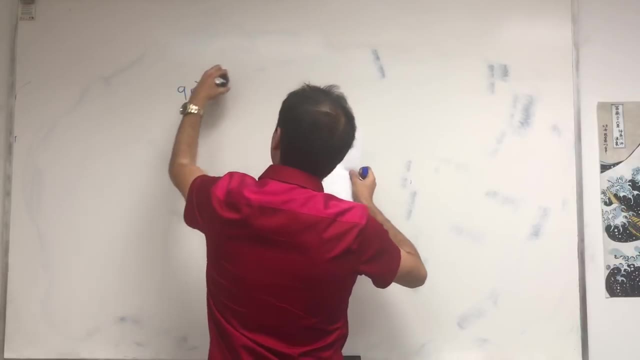 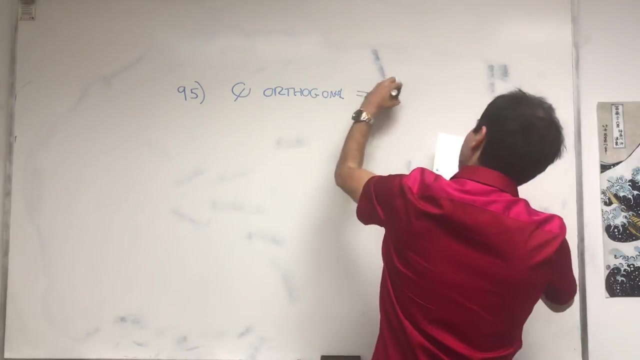 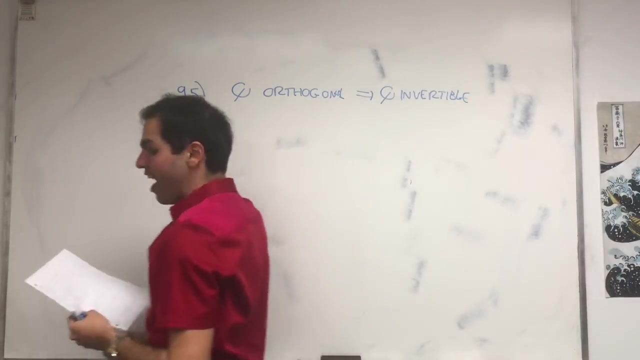 I should have taken a break. OK, Now Let's talk orthogonal matrices a bit. So if q is orthogonal, implies q invertible, And 95th language is Tatar And 95 is Tuxar. I had a professor called Tataru. 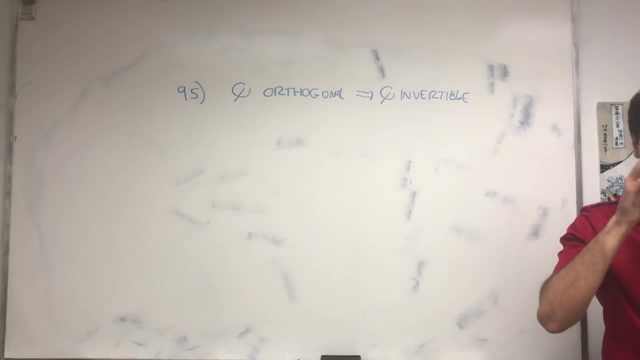 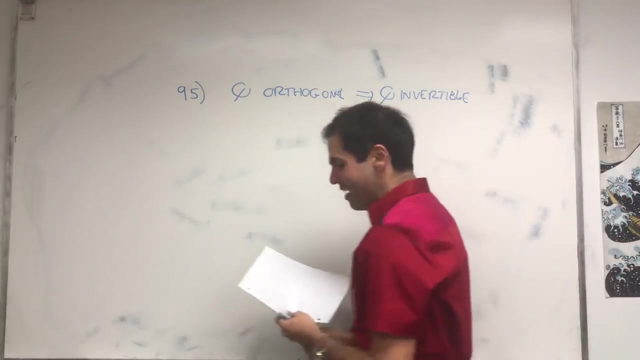 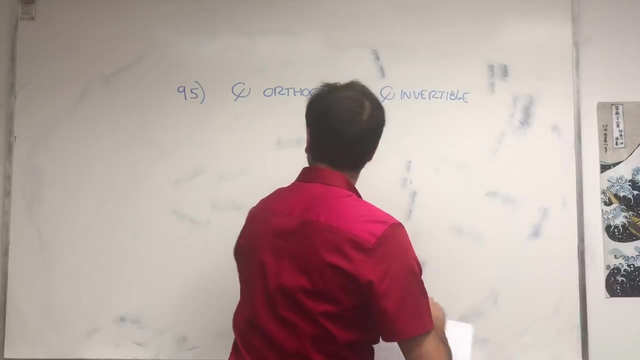 But I don't know if it's the same region or not. All right, I mean, there's also state Tatar, So maybe it's this one, I don't know. Anyway, So it turns out this is true, And it's just an exercise in remembering that orthogonal matrices are square. 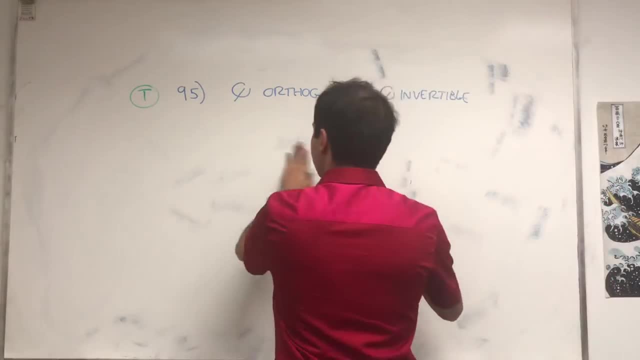 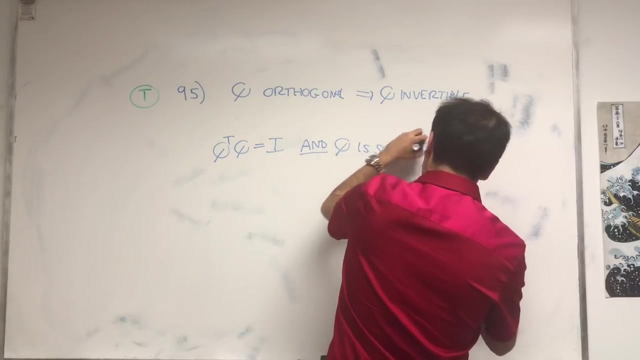 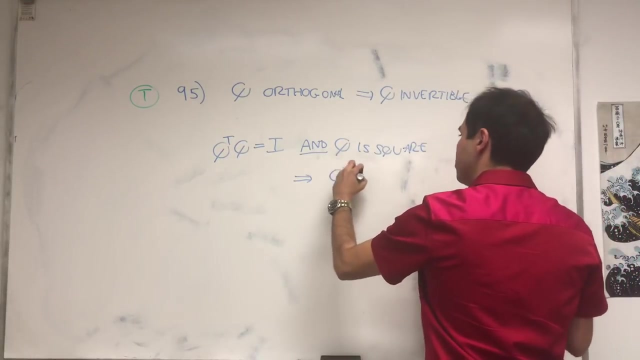 So they're square matrices with orthonormal columns, At least with the convention of lei. So we know q transpose, q equals to the identity And q is square. So in other words q transpose undoes what q does. So q inverse is q transpose. 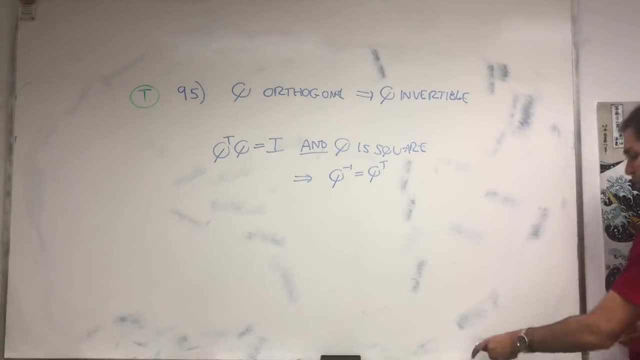 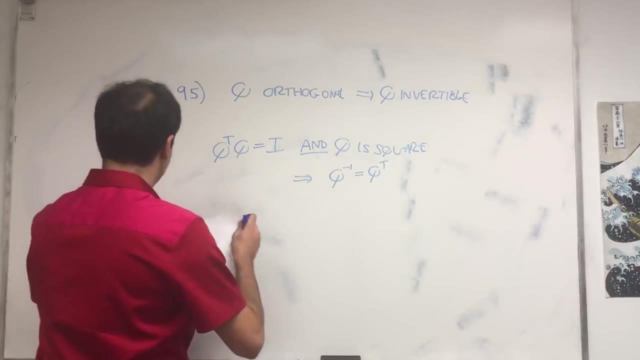 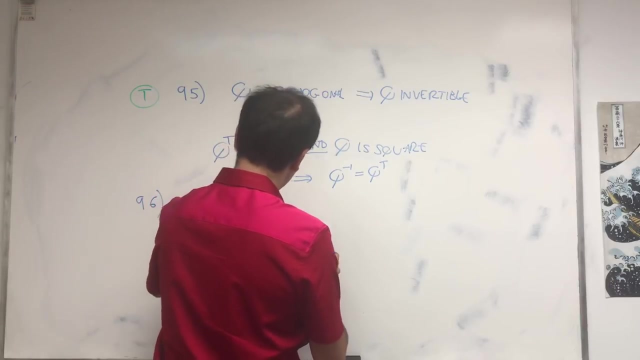 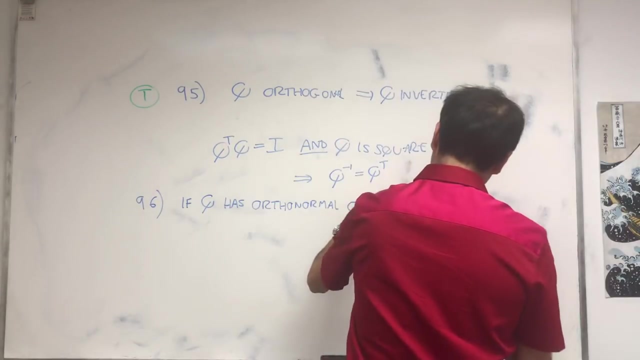 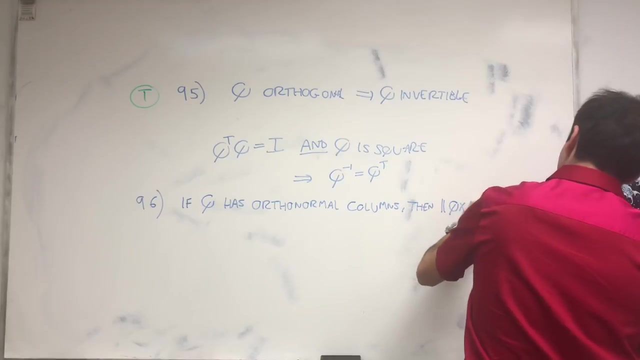 The point is: for orthogonal matrices, the inverse is easy to calculate. You get q inverse is q transpose, All right. Another question: This is also q. Q has orthonormal columns, Then the length of qx equals to the length of x. 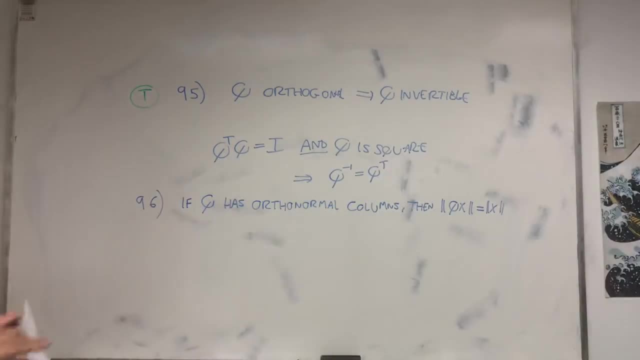 So, in other words, do more or less orthogonal matrices, do they preserve length And 96th language is so cute Fufuilde And oh But cute language. My God, The horrible number. So it's, I'm not sure if it's true. 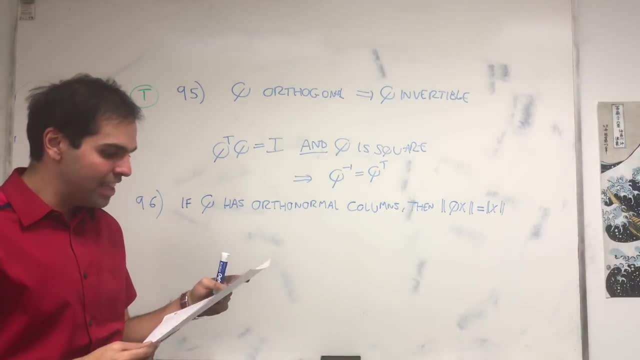 I just put all those numbers together, So 9 and 6 together with ba, And then hopefully it's true. Yeah, It's like 4 times 20 plus 10 plus 6.. That's why it's So it's. 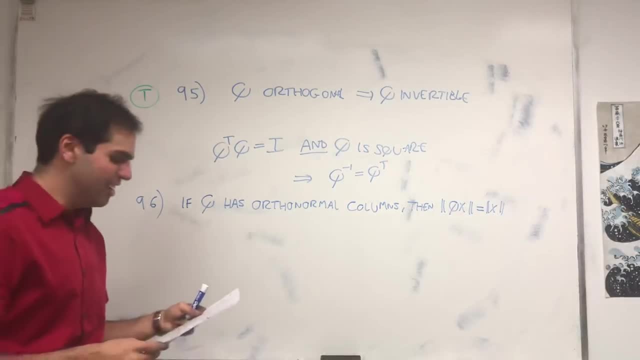 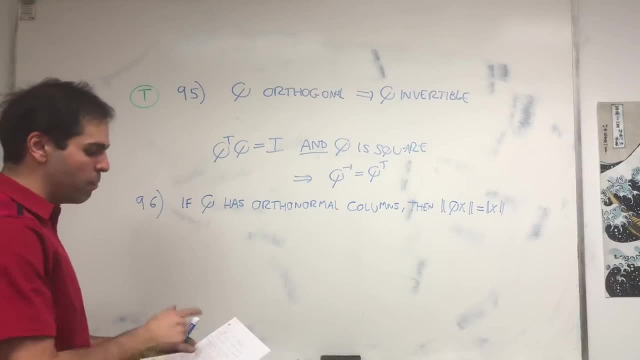 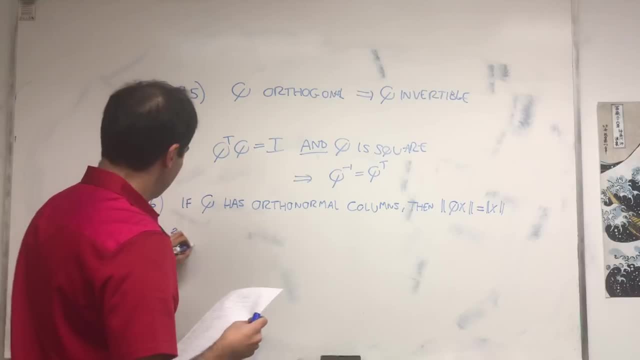 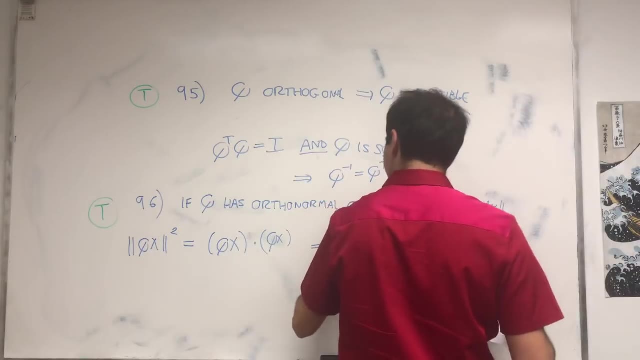 Well, you can write this as a dot product. It's Qx dotted with the Qx. Well, a dot product. you can write it with: transpose Qx, transpose Qx. That's x transpose Q, transpose Qx, But look. 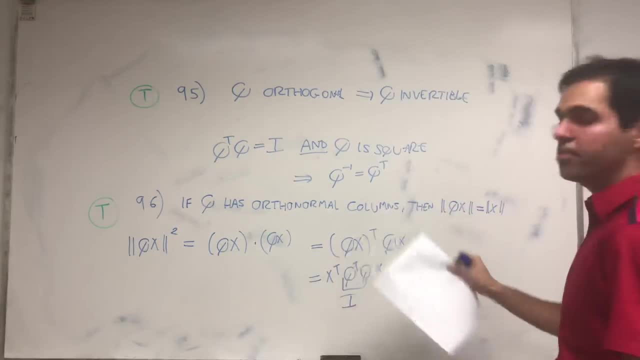 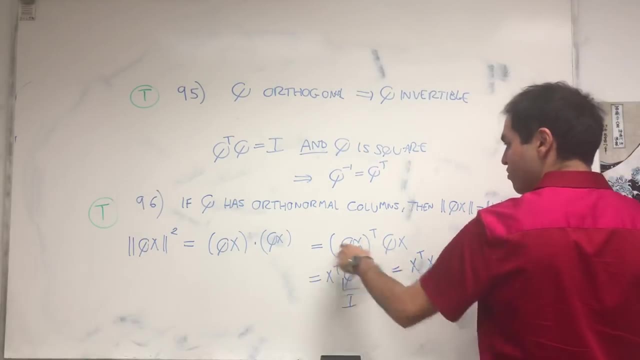 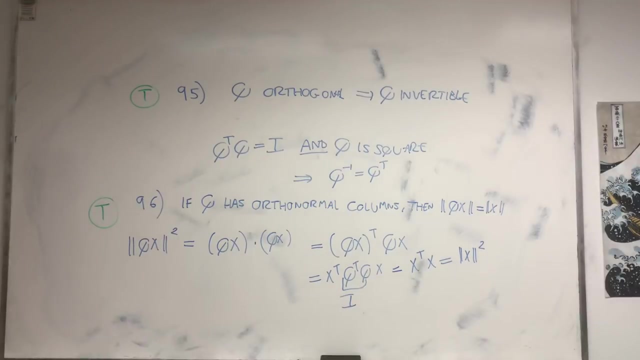 Q transposeóc noodles Q, because it has orthonormal columns. it's the identity, so it's X transpose X. but then by definition of dot products with transpose it's length of X squared. So the length of QX squared equals the length of X squared. then just take: 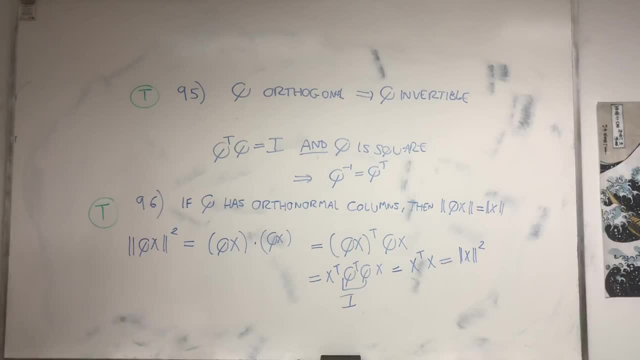 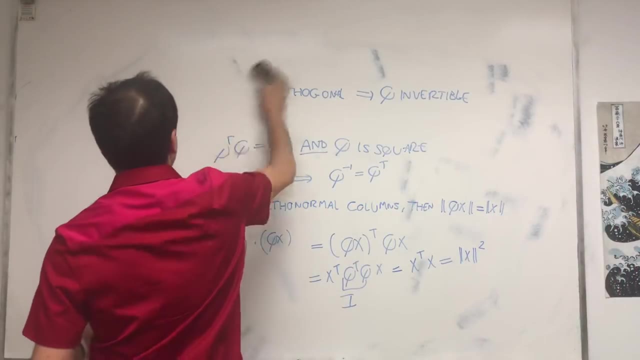 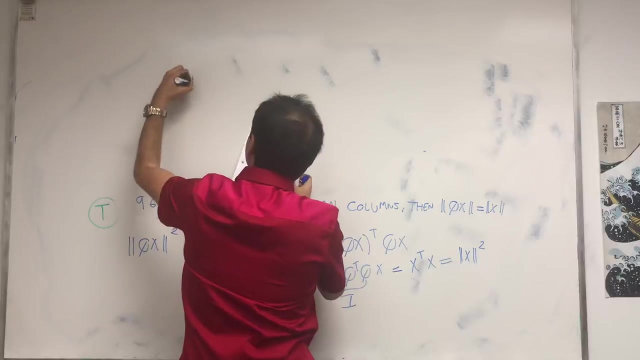 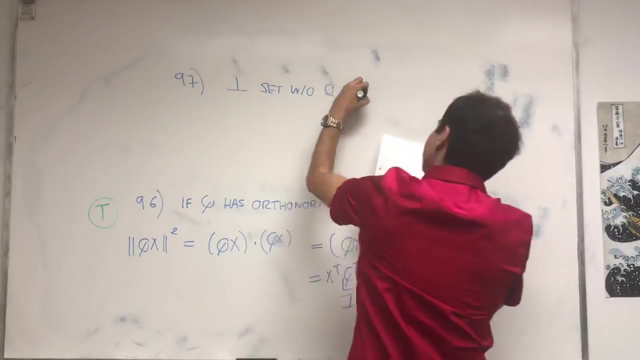 square roots. everything's positive, so good, Non-negative, and therefore we have this result, All right. next question, Also one of my favorite proofs, so 97.. A orthogonal set without the zero vector is linearly independent, And so 97, so. 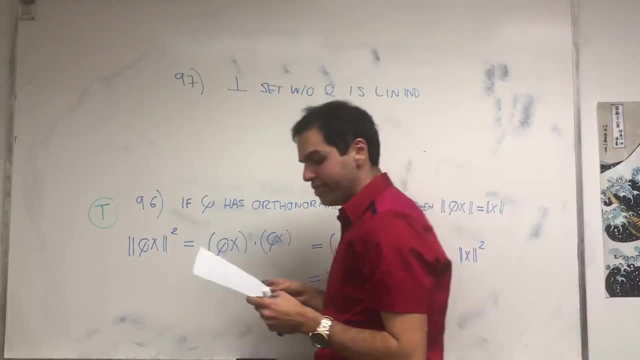 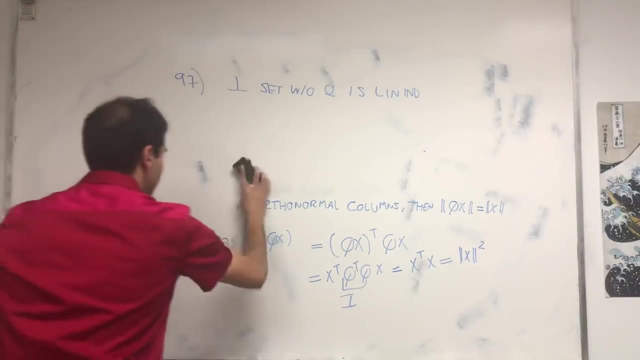 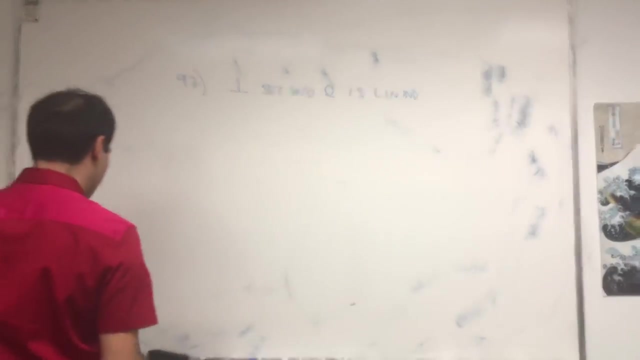 sanani dialect of Arabic. so sapah wa tis'un. Okay, next question. Well, I kind of gave it away. I said it's my favorite proof, so it's probably true. Otherwise I would prove something false, And here's why It just has to do with. 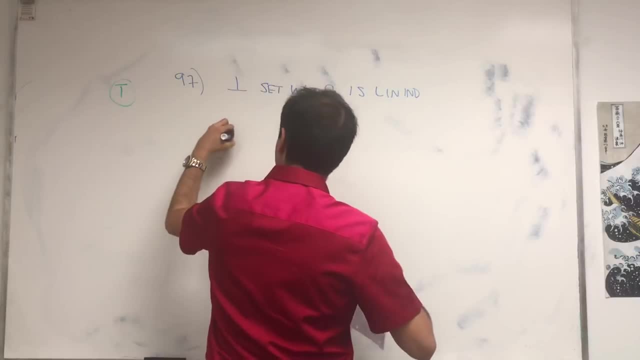 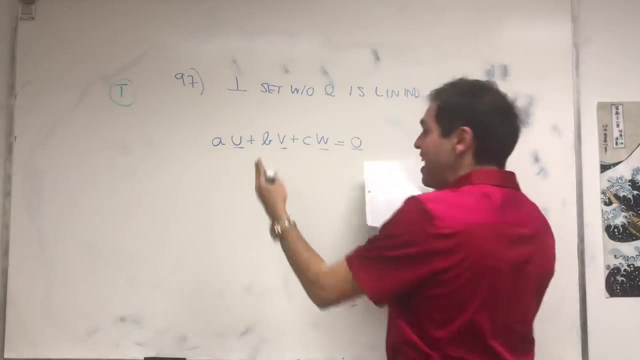 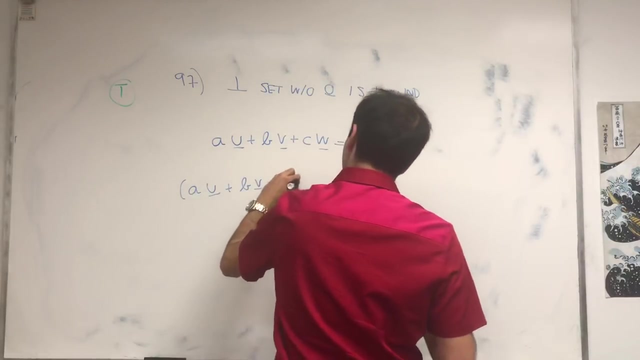 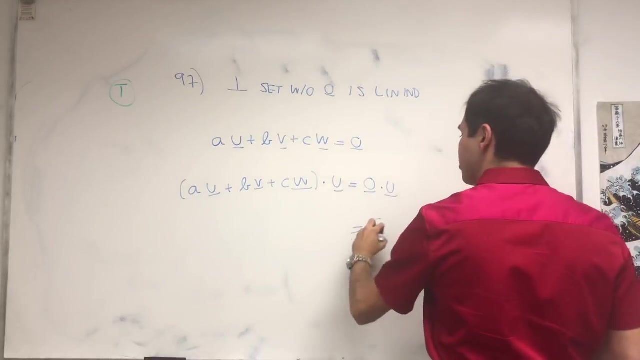 hugging. So suppose let's say for three vectors, AU plus BV plus CW equals zero. Then take this equation, hug it with the first vector. So AU plus BV plus CW dotted with U equals zero dotted with U. but zero dotted with anything is just a zero scalar here. expand it out so AU dotted with U. 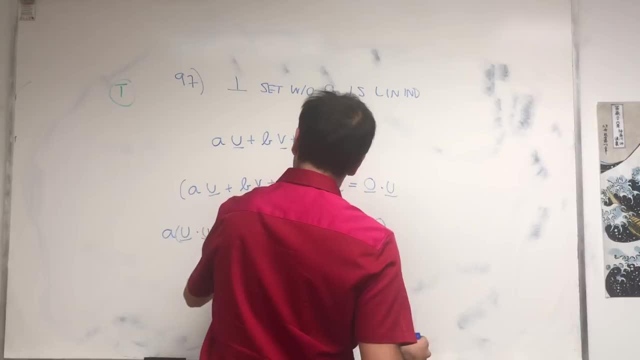 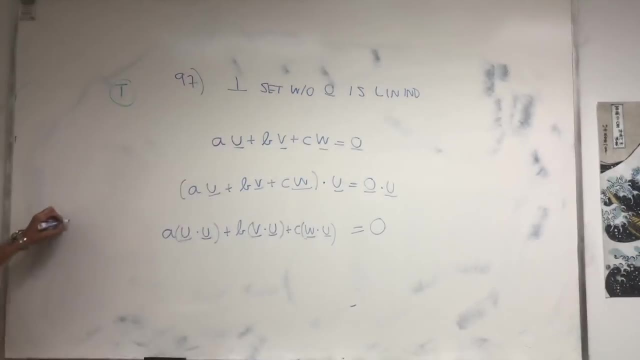 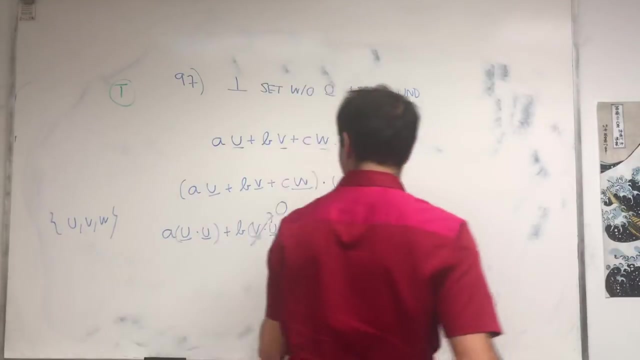 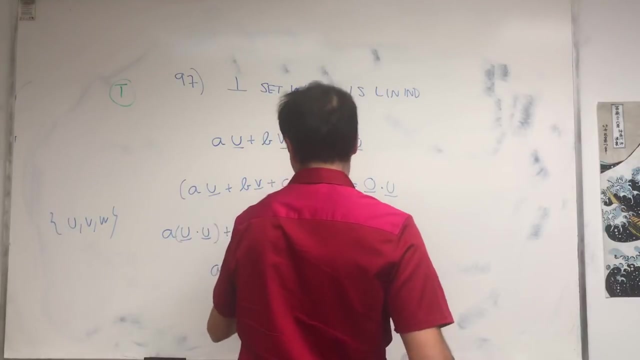 plus BV dotted with U, plus CW dotted with U, but now remember UVW, it's orthogonal. So if you take v dotted with u, that's 0 by perpendicularity. w dotted with u, it's 0.. So au dotted with u, it's 0.. Okay, and 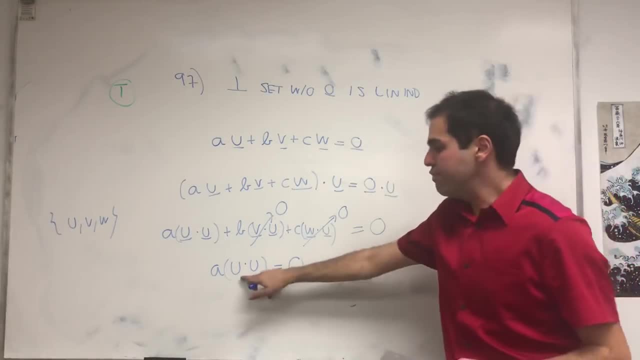 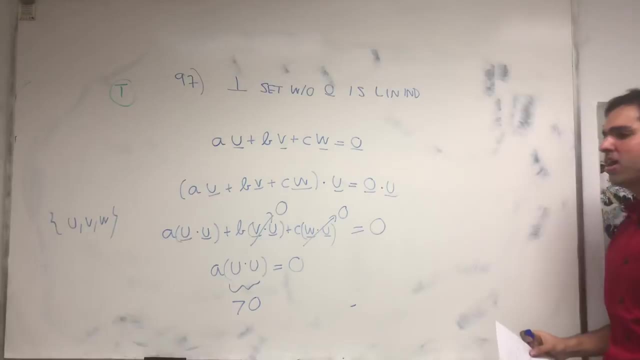 why did we assume that there's not a 0 vector? If u is not 0, this is actually positive. So a vector dotted with itself it's always non-negative, but it's positive if the vector itself is not 0, so we can legitimately divide. 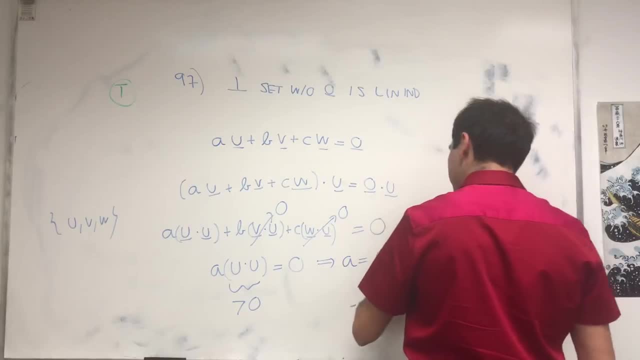 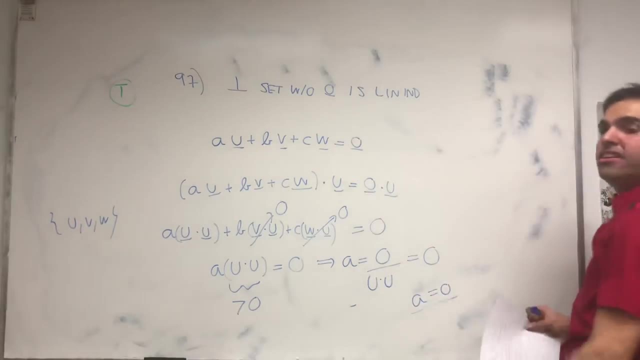 So a is 0 over u dotted with u, and that's 0.. So a is 0.. In particular, technically use induction. but in this equation a is 0, so bv plus cw equals to 0, and then just take this equation and dot it with v and then you get. 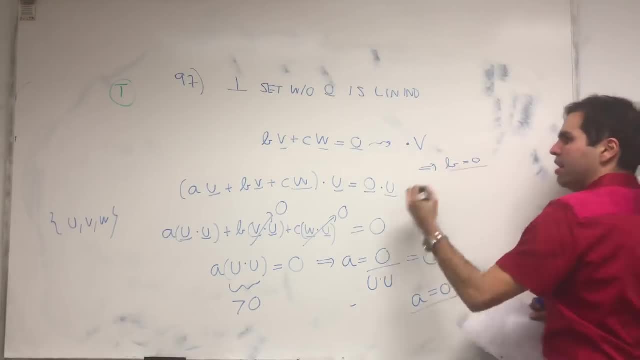 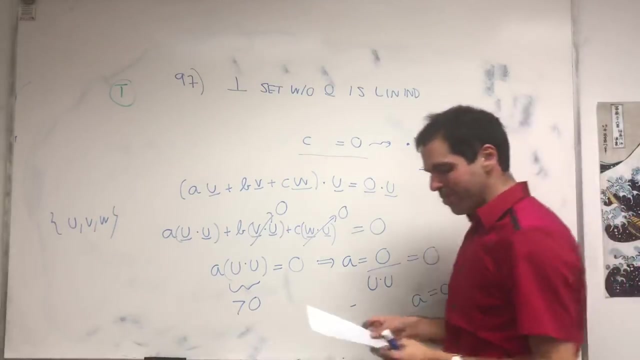 b is equal to 0, and then lastly, so then cw is 0, but w is a non-zero vector, so c is 0,, so c. So a, b and c are 0, and that's all what we wanted to show. so that's good. 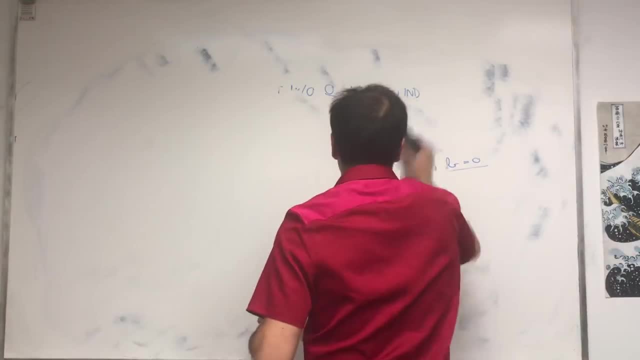 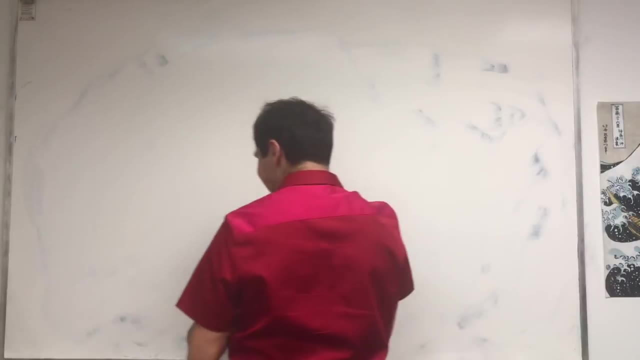 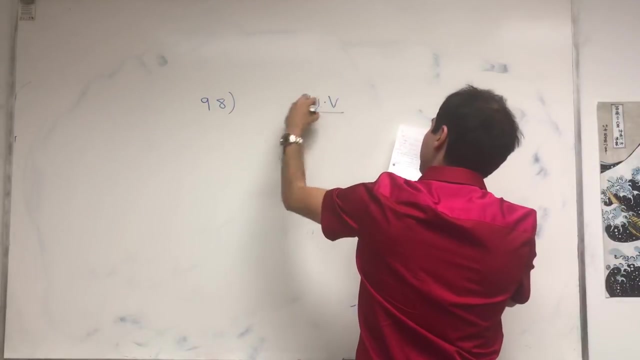 It's true that orthogonal set without the 0 vector is linearly independent. Okay, 98,. oh my god, we're almost close to 100,. so 98,, namely u dotted with v over v dotted with v, v is the orthogonal projection of. 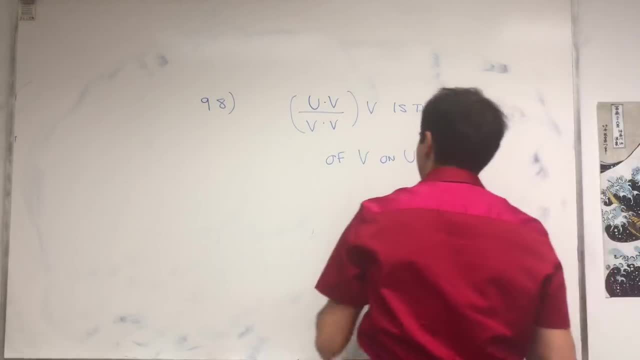 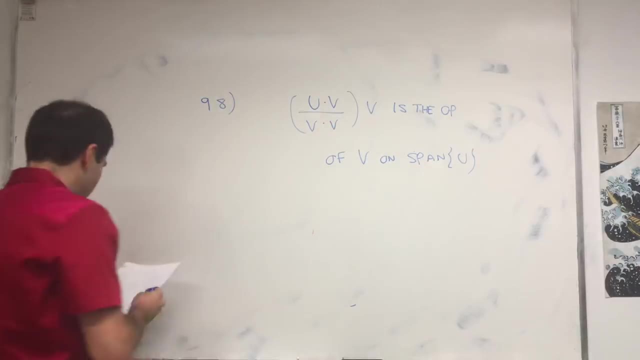 u of v on u like a span of assuming that u is non-zero, Okay, and 98, we would. and then it's tuksan wa sezlik Or no. tuksan wa sekiz Sounds Turkish-ish. 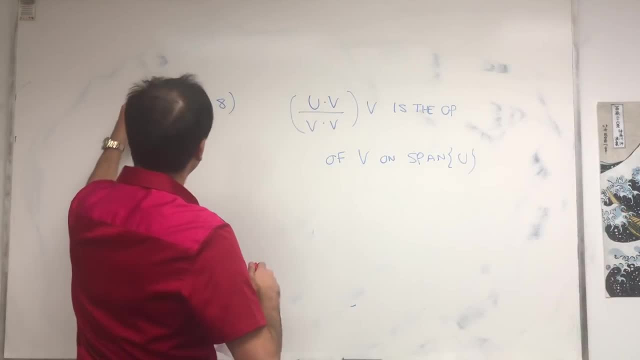 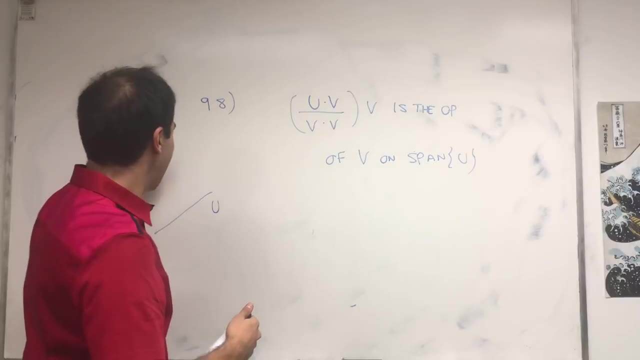 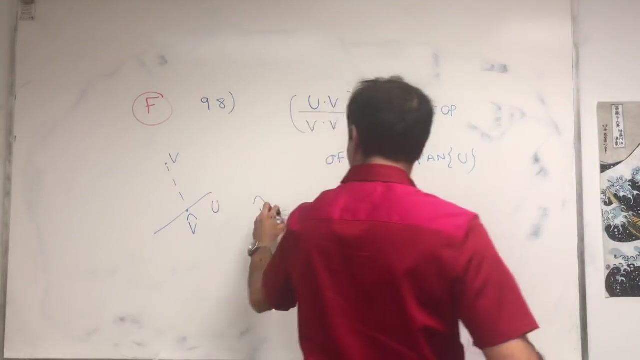 That's it. Even though it is, this is not only false, it's very false, because, look, if you have u and its span and v, then v hat. well, it has to be in the span of u, v hat, it has to be a. 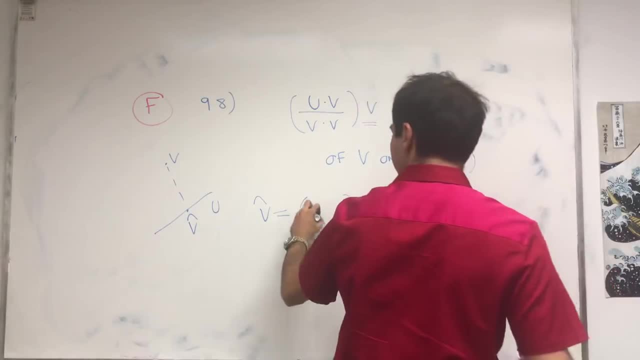 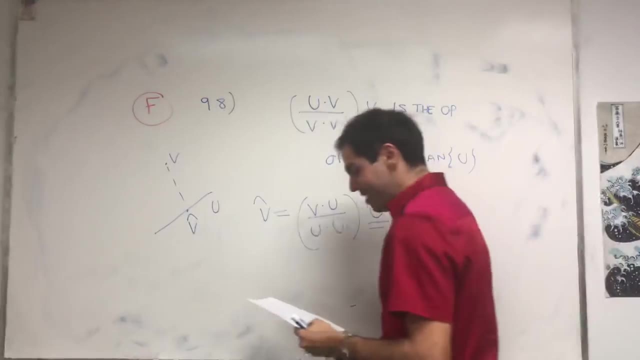 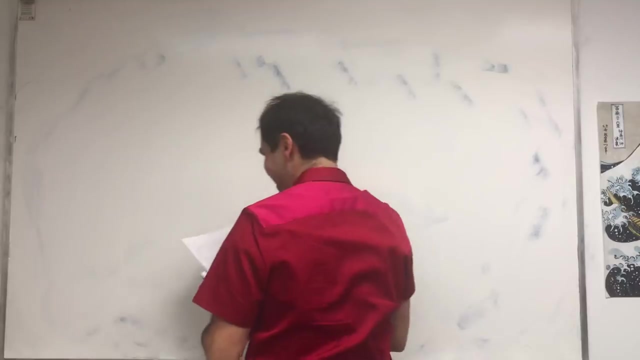 multiple of u, not a multiple of v, and in fact the correct thing is v dotted with u over u dotted with u. u. Just be careful about this. Next one's super interesting, It kind of got me but 99,. not a non-sickness, no fun-ons. dot, dot dot. 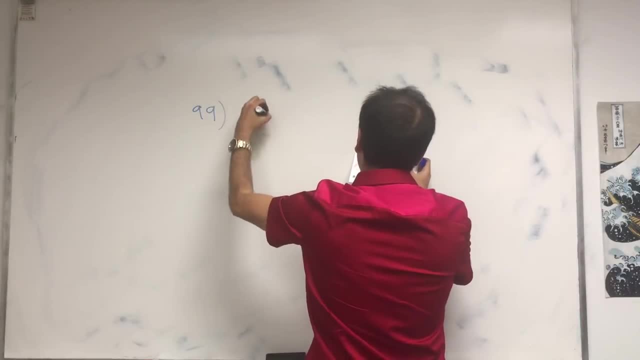 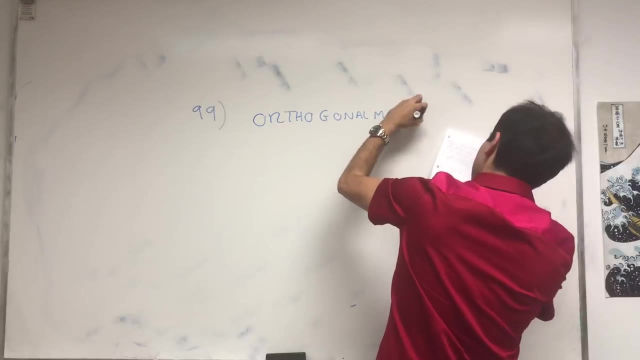 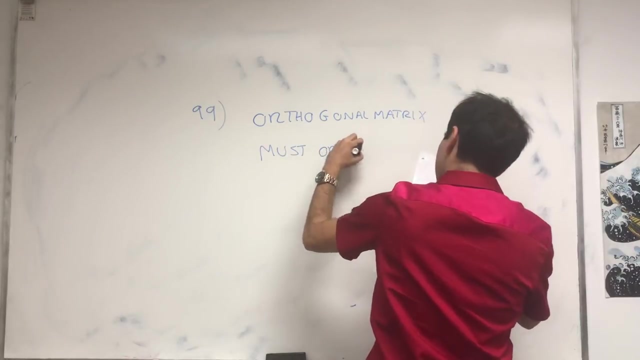 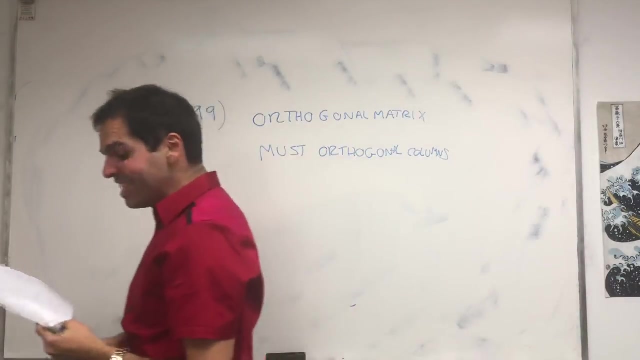 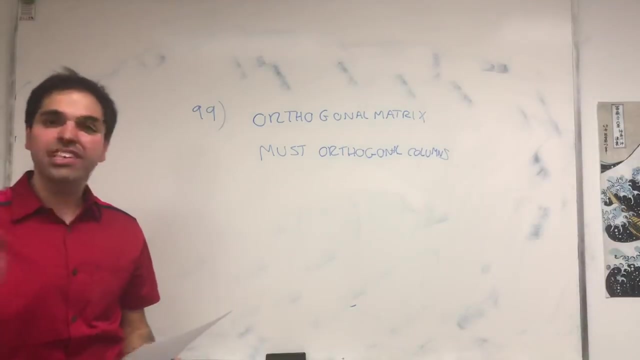 This is what I get after four hours or something. Good question: Does an orthogonal matrix? Does an orthogonal matrix have to have orthogonal columns? Ninety ninth language, so Haitian Creole, the French Creole version of Haitian. it's interesting in French. 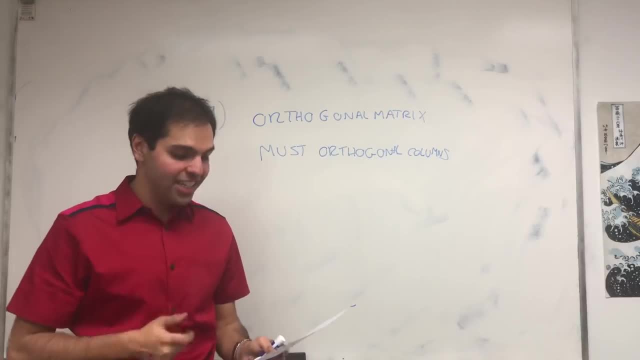 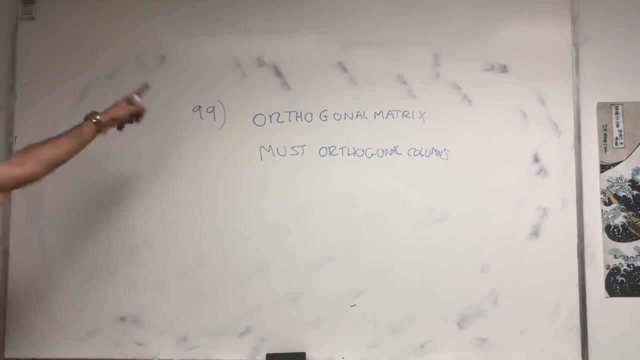 99 is katrandy'sethuf, In Haitian it's katravendidethah Van De Sniff. Interesting dialect, Okay. so let me tell you about this one. I thought: well, it's false, because the orthogonal matrix must have orthonormal columns. but 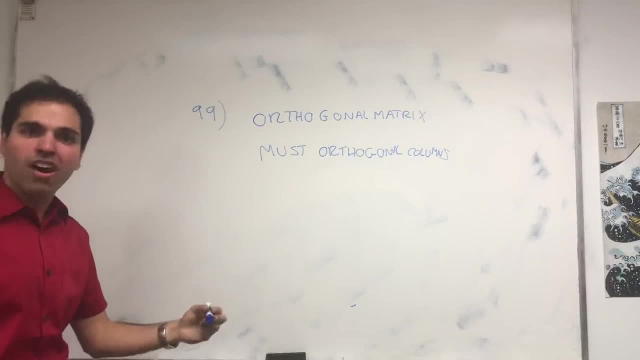 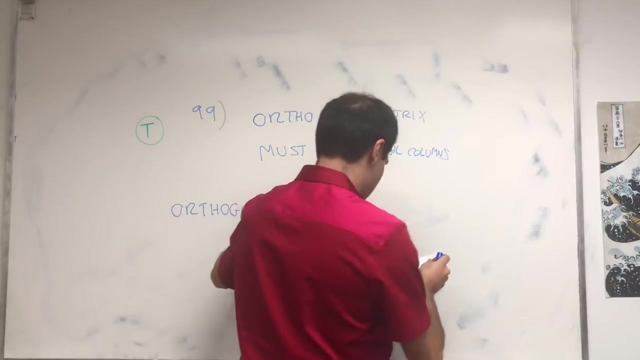 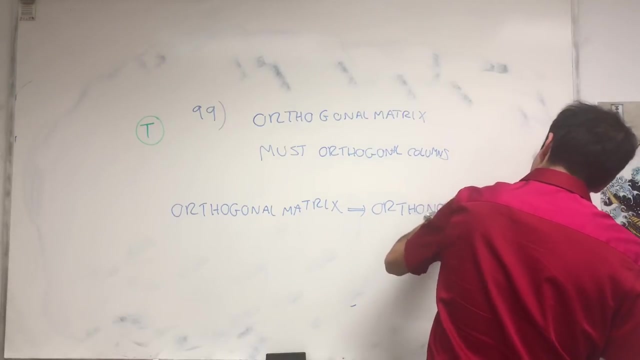 remember, orthonormal also means orthogonal plus the length 1.. So in fact it is true. So an orthogonal matrix is stronger than that. So orthogonal matrix implies orthonormal columns. but you see, if the columns are orthonormal, they're. 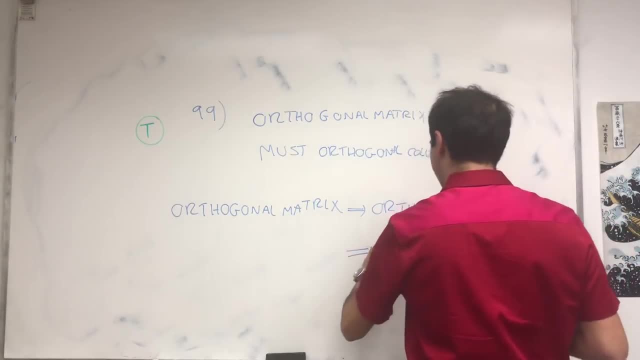 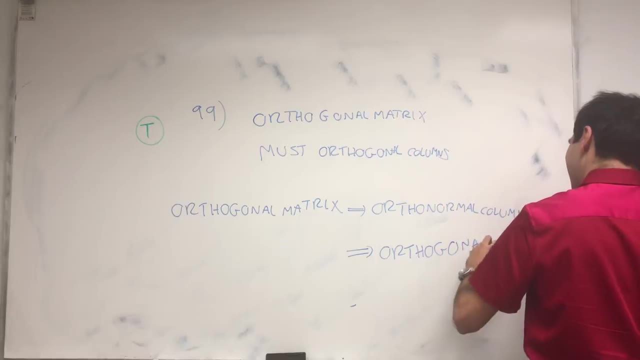 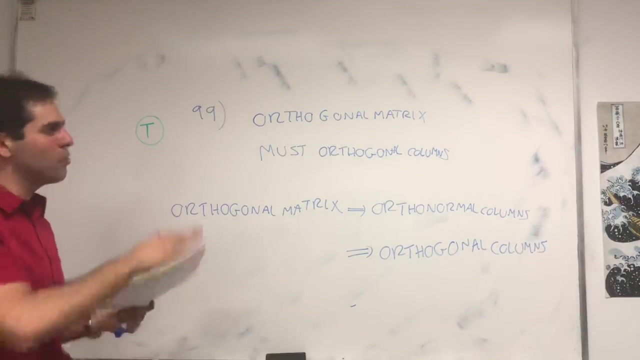 like super orthogonal. so in particular they're orthogonal. This one got me. I wrote this question I was like clearly it's false. but then I was like, wait a moment. Technically true Again, try again, Just to show you. well, it has the orthonormal columns. It's a bit of a. 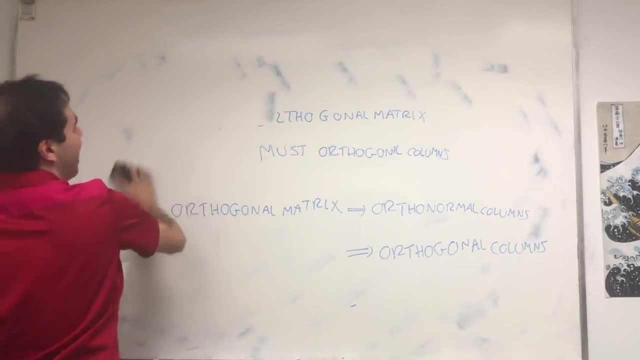 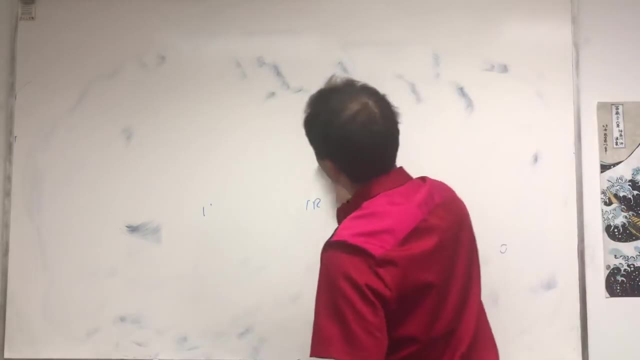 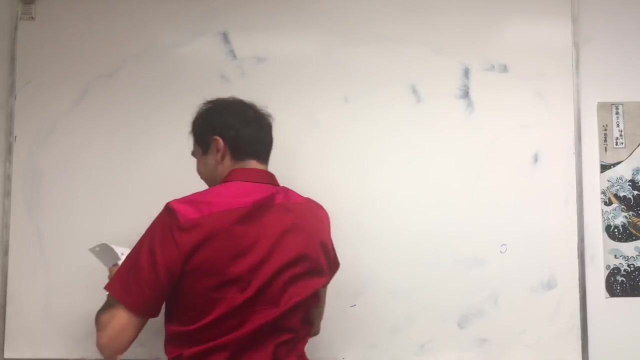 misnomer. Okay, question 100.. Oh my god, I have to say: black men, red men. that was harder than I thought. I thought it would be very quick because it's true-false, but I'm dying. Okay, so it's question 100.. 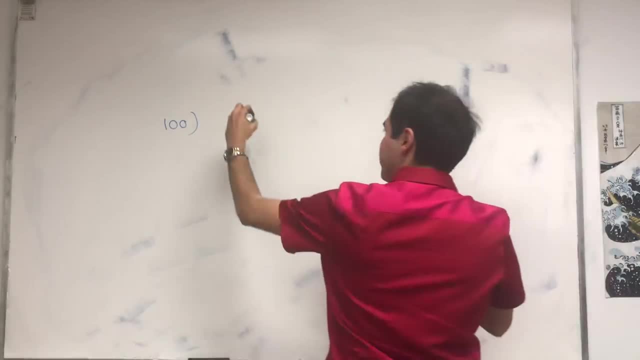 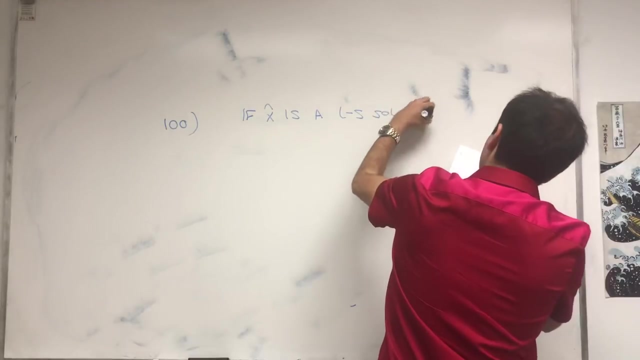 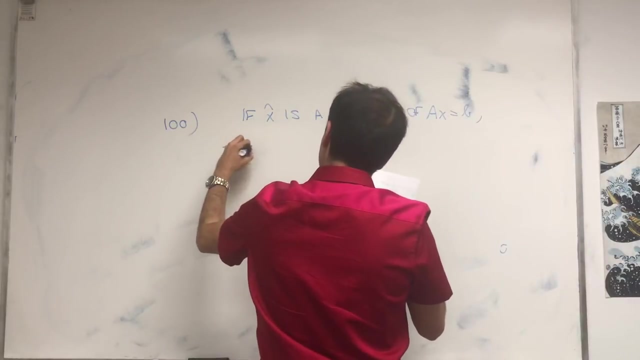 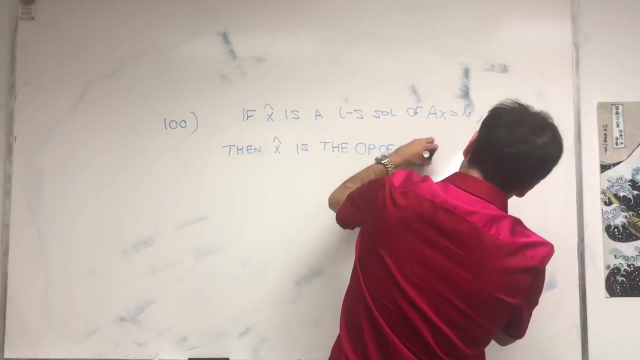 So how many of them are still alive? So let's talk least squares, So the least square solution. so if x hat is the least square solution or a least square solution, a least square solution of ax hat, of ax equals b, then x hat is the orthogonal projection of x on the column space of a. 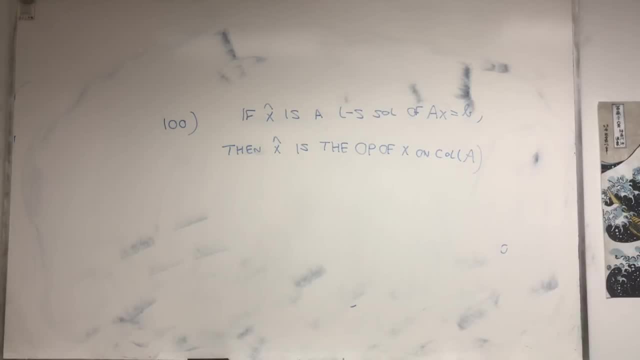 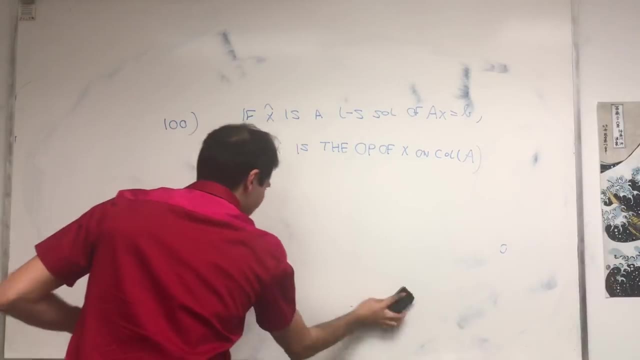 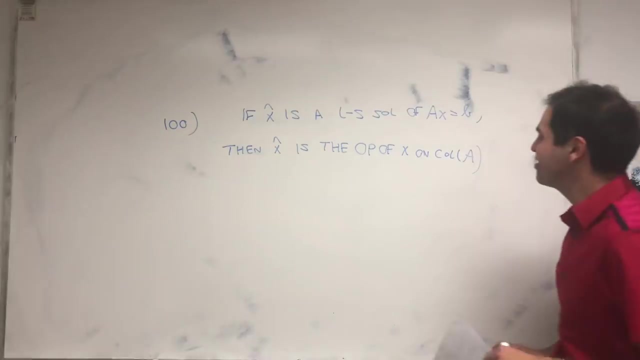 And then the plus square solution is a equals one. So let me check right here, okay? oh, we're almost at the four hour mark. That's so crazy. I would never have guessed that. but cool though I guess, no grocery shopping for me today. Costco is probably closed soon. 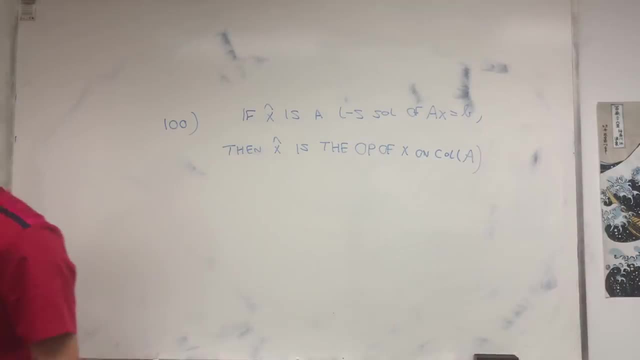 Also 100th languages. so, uh, the northern part of Azerbaijan, So, and language, basically. so 10,000,000,000,000,000,000,000,000,000,000,000,000,000,000,000,000,000,000,000,000,000,000,000,000,000,000,000,000,000,000,000,000,000, and a few more, So 10-100. bad voices are open. 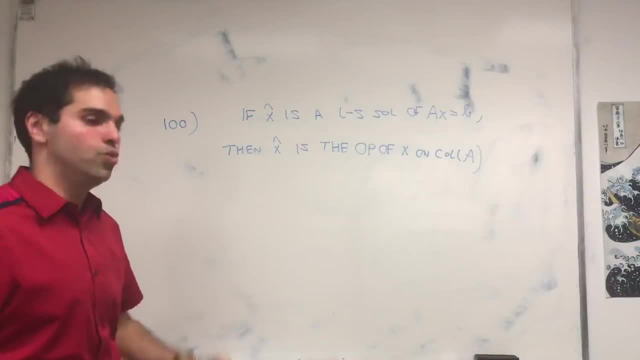 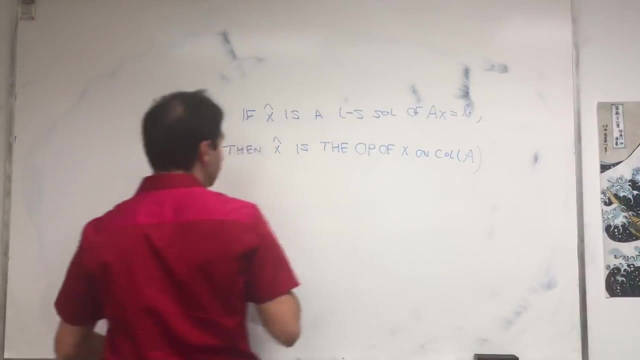 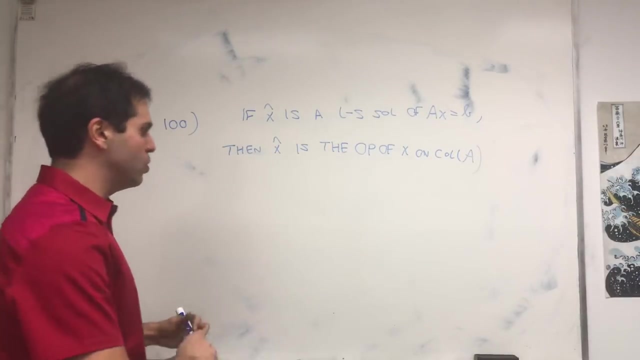 hundred in the other by Johnny is use probably also, I think, in Turkey anyway. so if this is a bit of a misnomer, even though we put a hat here, it's not really an orthogonal projection, because what you really do, you have B and the column. 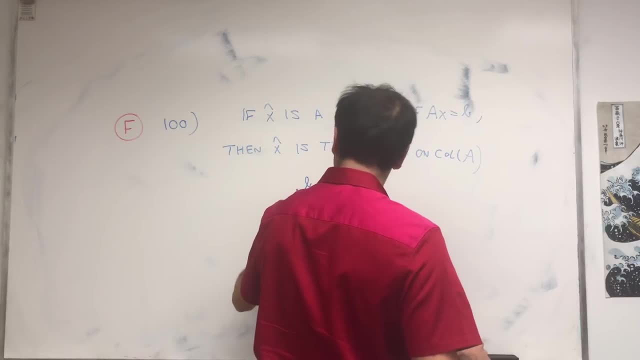 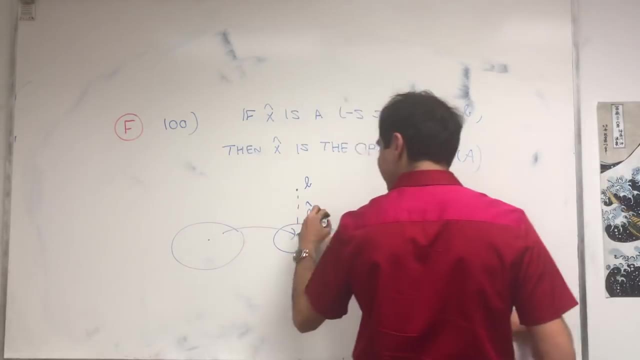 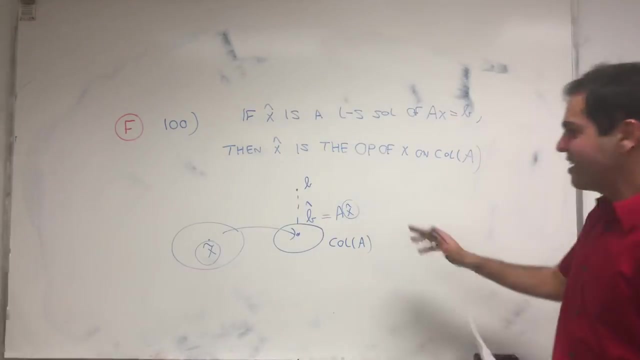 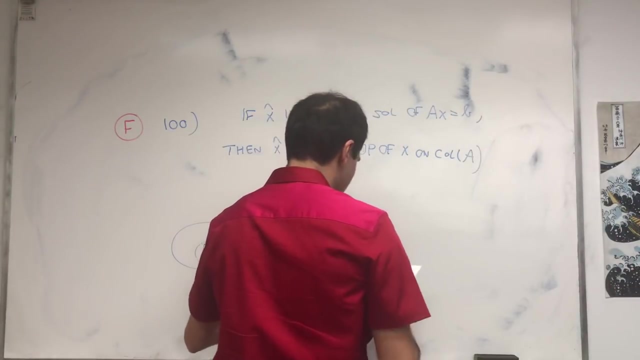 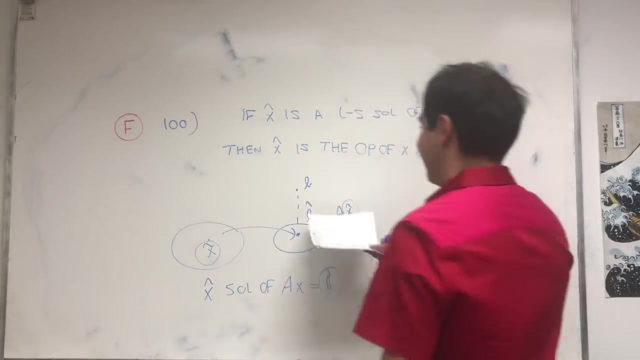 space of a and first you project B on column space of a and then what you do- you saw so because we had- is in the column space of A. it must have a solution: X hat. so you see, X hat has nothing to do with orthogonal projections. X hat is a solution of a, X equal, ax equals to B and B hat is the. 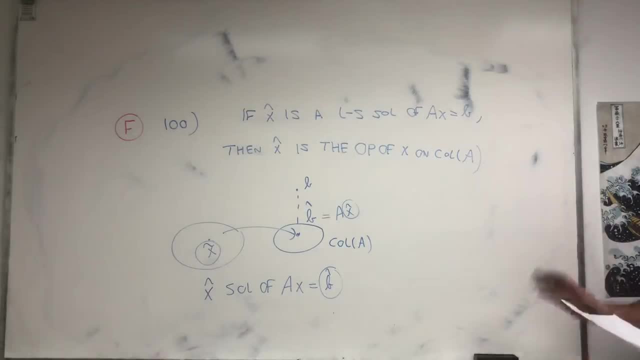 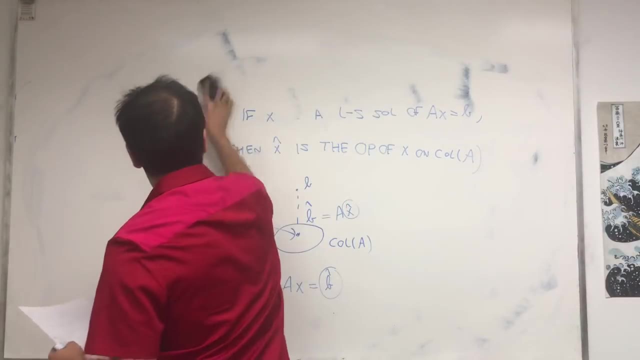 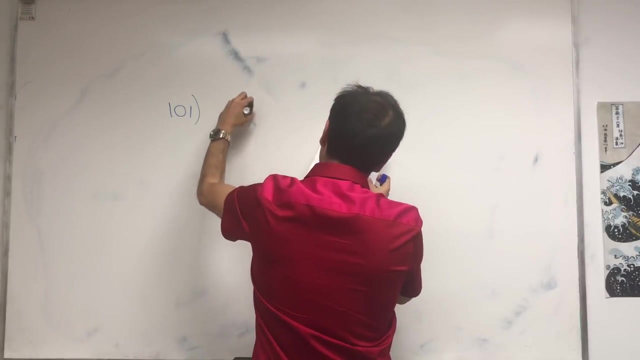 orthogonal projection of B on the column space of A. So again, don't be confused, it's just a misnomer, okay. on the other hand, or maybe maybe on the same hand, i don't know, oh man, i screwed this up- but um 101, so 101 dalmatians, so ax hat is the point. 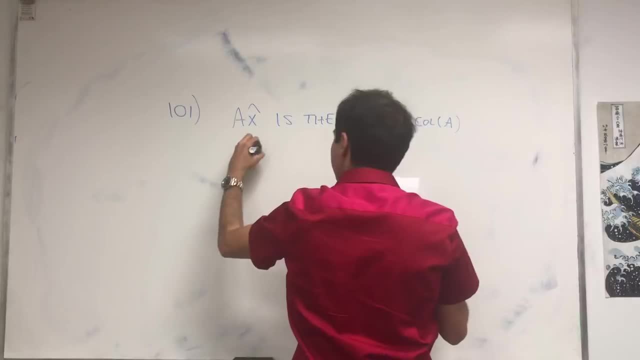 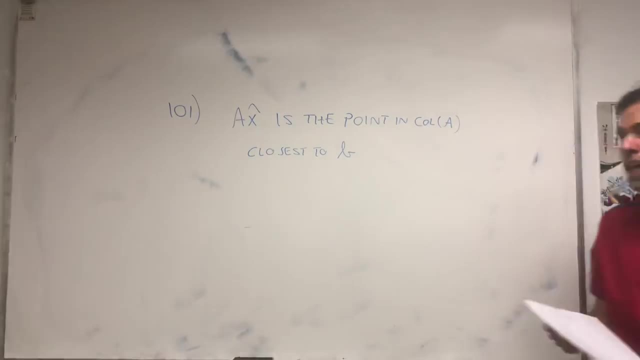 in column space of a closest to b. and again here, x hat is a least square solution of ax equals b. and 101st language, napoletano. i love da michele, it's so my favorite pizza in the world and napoletano, at least in italian, is. 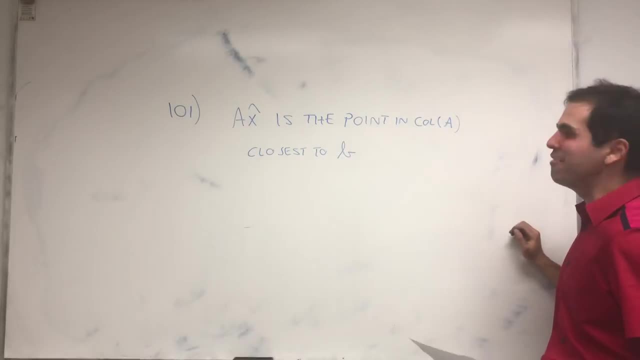 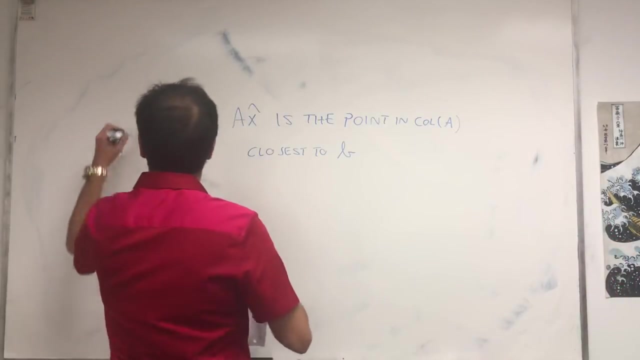 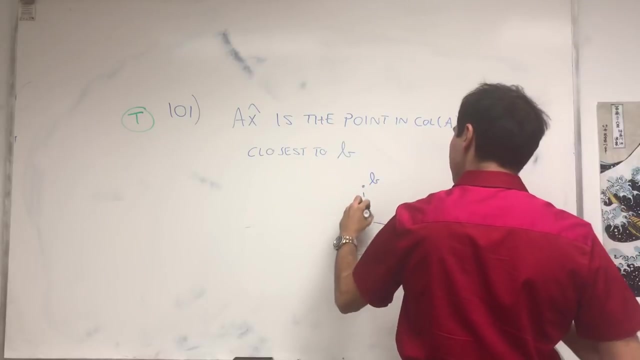 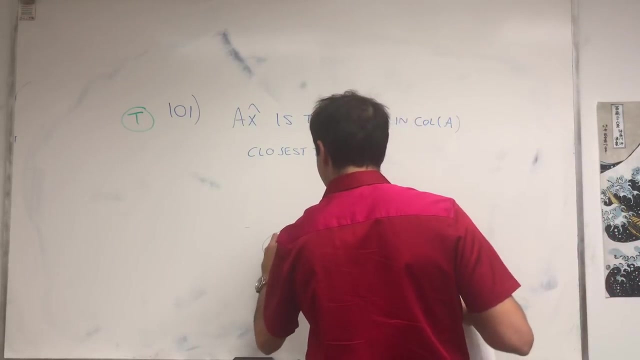 i got 99 problems and what i get, i guess 111 problems, but now it's prussian 101. um, anyway, this is true. so, and again, it's actually the same picture as before. so remember how to find the least square solution. we have b, we have b hat, we project it on the column space of a and then we find a solution: x hat. 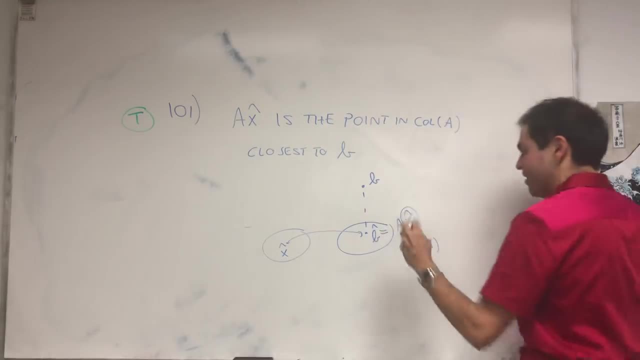 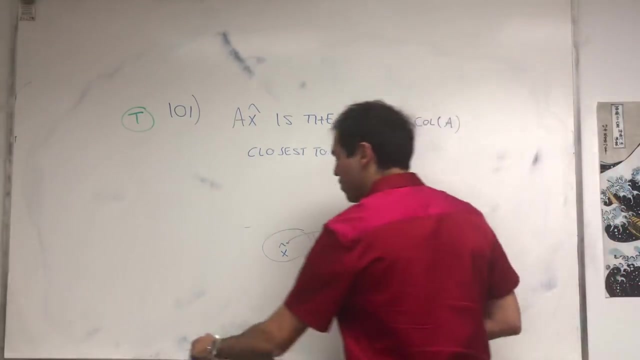 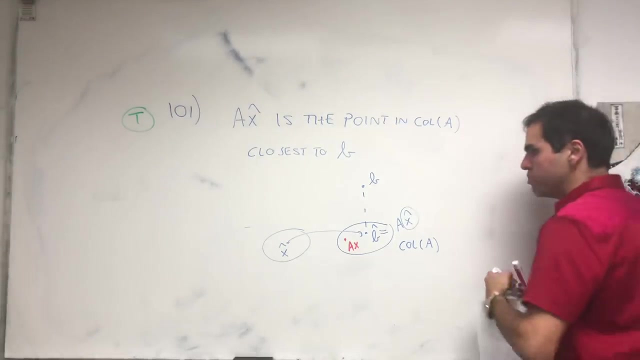 equals. so b hat equals to ax hat, and that is the least square solution. and the point is, what is the least square solution? it's the set of all outputs of a, so any other x must be in here, so ax, and notice in terms of distances: well, b minus b hat, well, that's the small, much smaller than b minus a x. 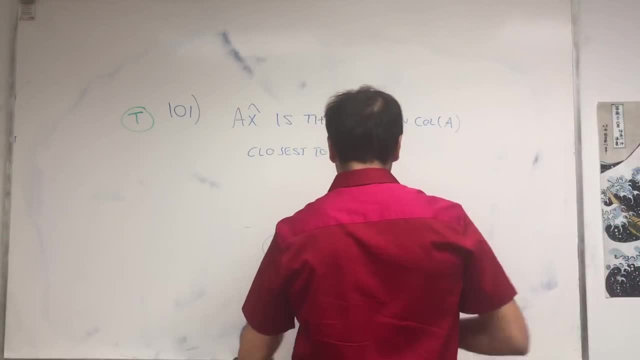 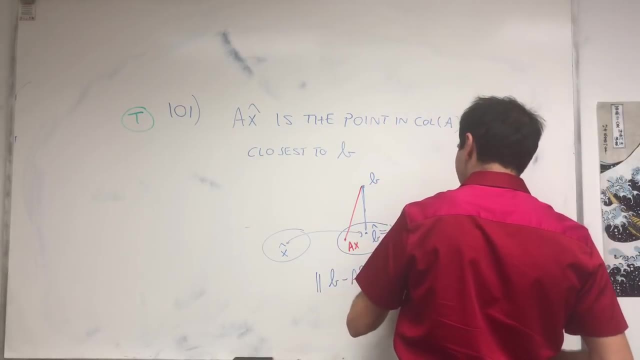 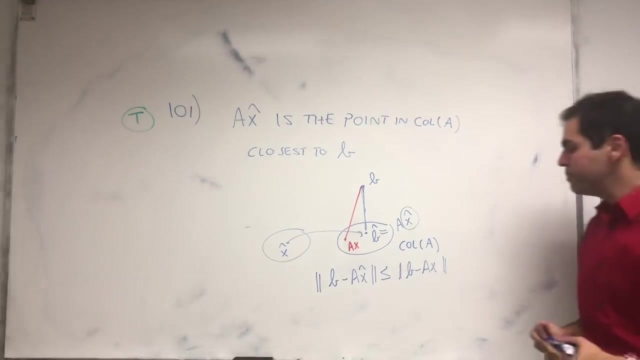 so it is true that the least square solution, x hat, satisfies that it's the closest you can get to b less than or equal to B minus AX, Because the length of the blue segment is smaller than the length of the red segment, And that's why these square solutions are so important. 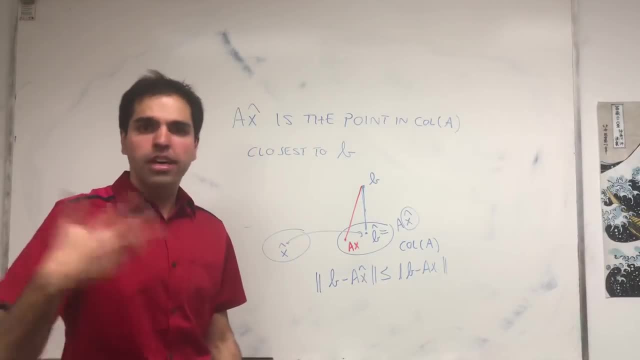 Because suppose you're at the company and your boss tells you let's produce a million dollars. You can say, well, we can't produce exactly a million dollars, but I can show you how to produce $995,000.. It's hopefully good enough. 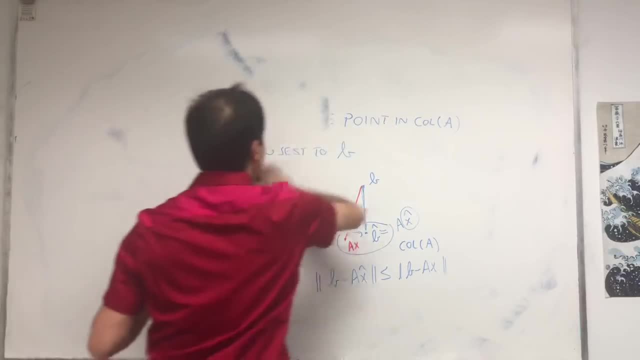 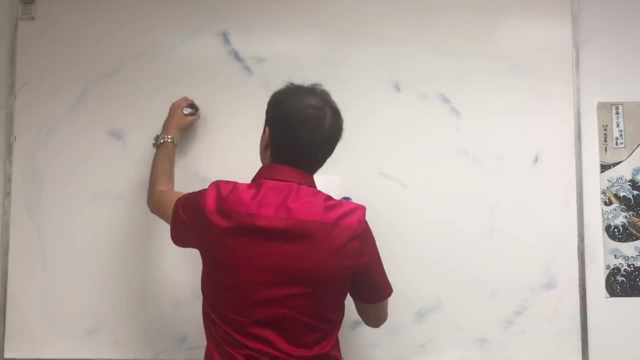 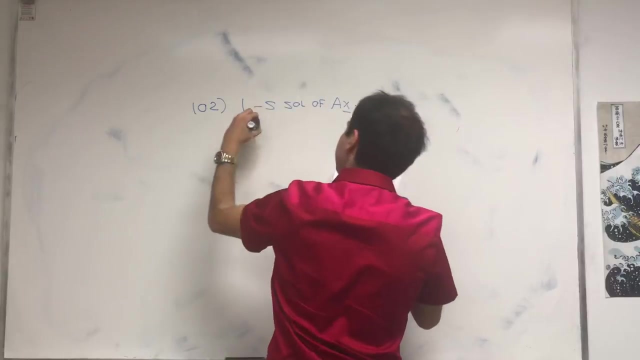 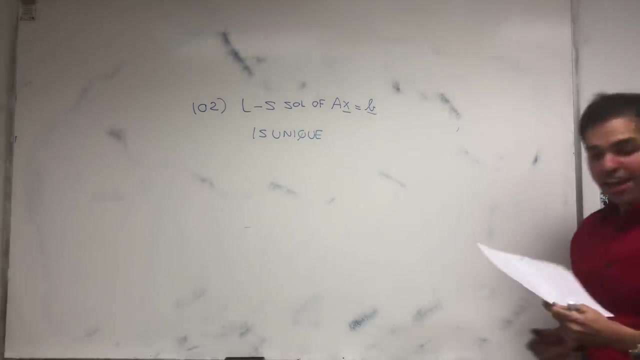 Okay, one and a half pages to go, So question one or two. So the least square solution of AX equals B, is unique, Unique like Monique, One or two, so Khmer, And it's Muoy Roy P Actually pi. 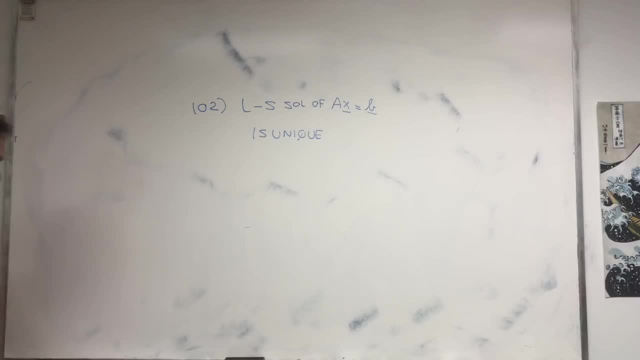 There's pi in it, So Muoy Roy Pi. That says as delicious as this is. Unfortunately, the least square solution is not unique And in fact you can check the following system: I think if you do X plus Y equals 2. 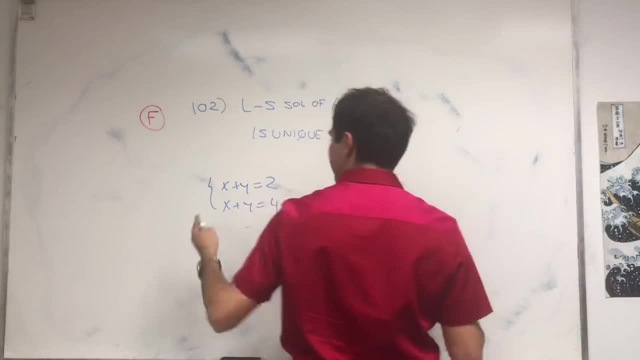 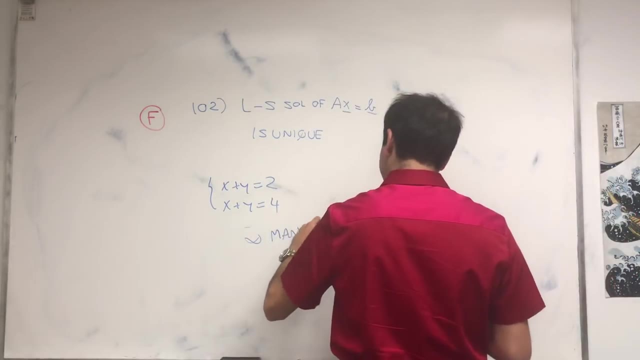 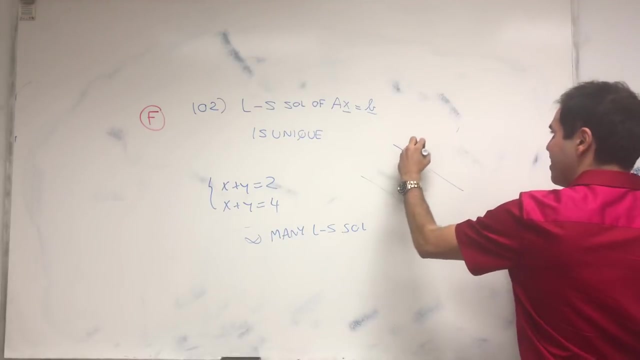 and X plus Y equals 4, it's of course inconsistent, but even for least square solutions, it has infinitely many least square solutions And in fact I didn't do the algebra, but I think if this, X plus Y equals 4, 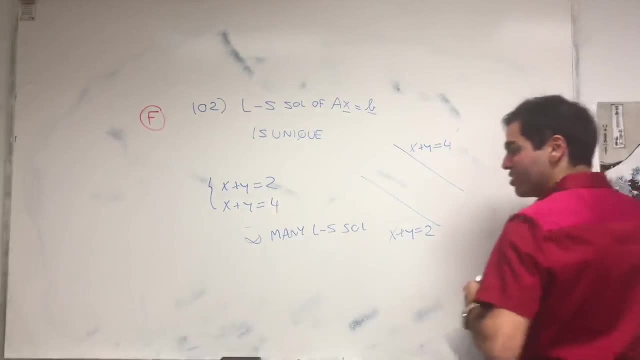 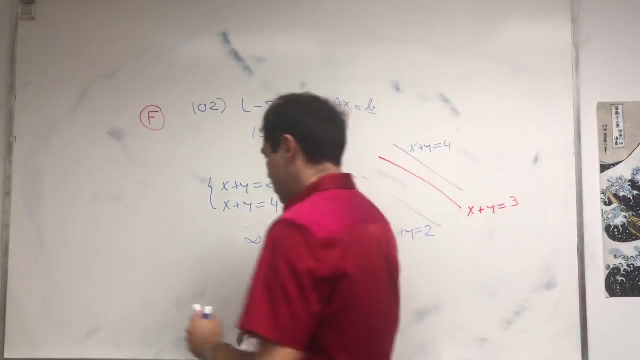 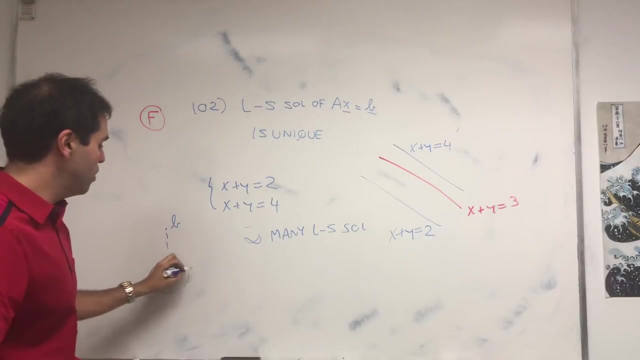 and X plus Y equals 2,. I think the least square solution is any solution on this line: X plus Y equals 3.. And you may say what went wrong. Well, look, it is true that B hat is unique. So if you project B on the column space of A, 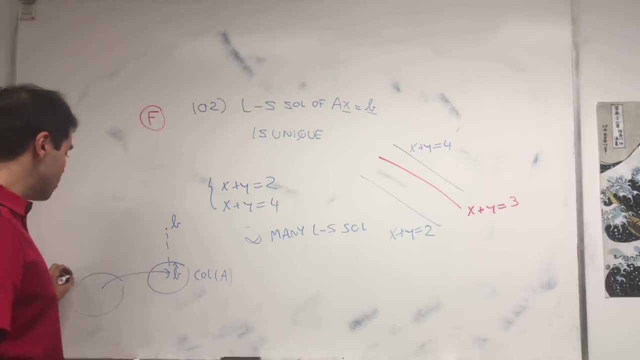 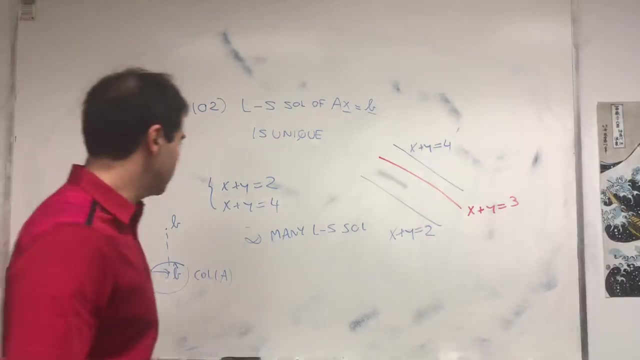 this is unique, But this doesn't mean that the solution AX hat is unique. So, in other words, there could be many solutions of AX equals to B hat, So that's why it's possible that you have infinitely many least square solutions. 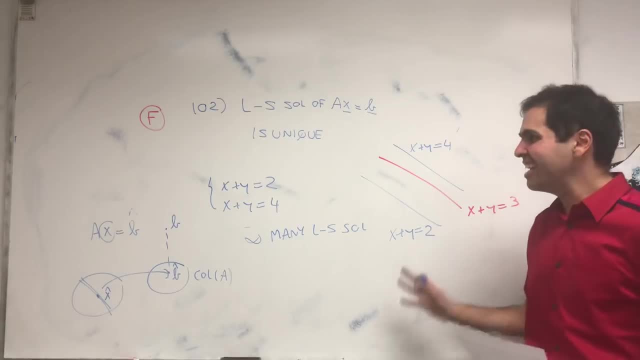 That said, there is an easy condition that guarantees uniqueness: You just need the columns of A to be linearly independent, And it has to do with the fact that the rank of A transpose A is the rank of A. Okay, lastly, 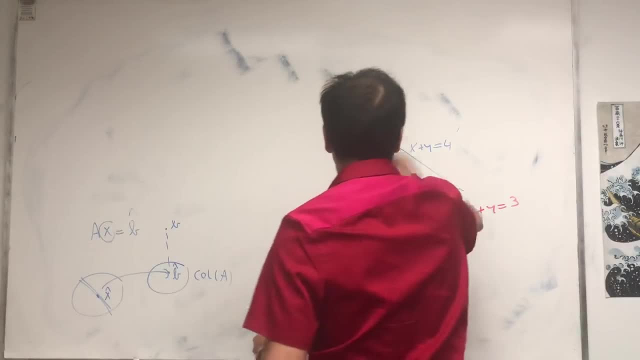 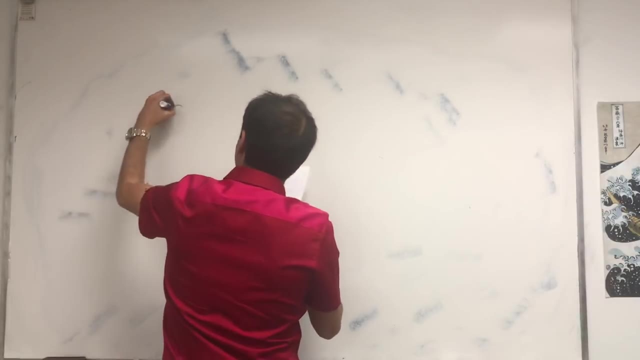 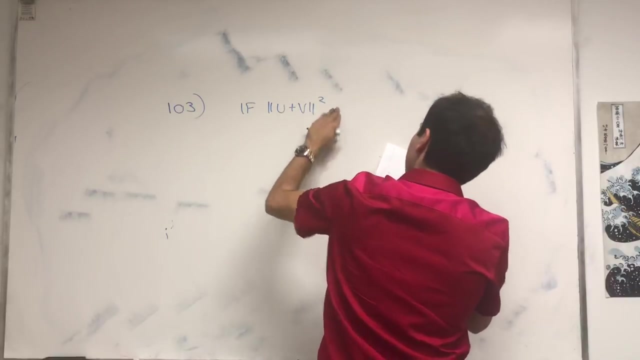 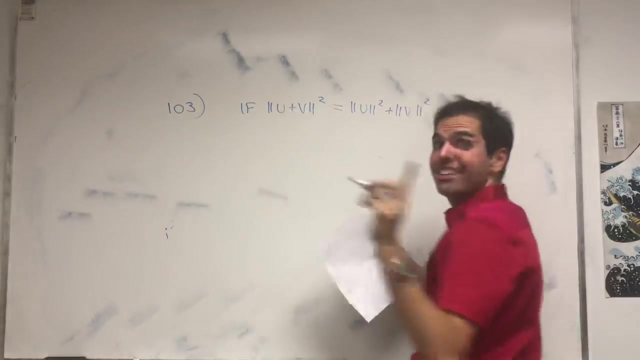 let's do a couple maybe inner product space questions, And it's lastly in this section, So maybe sort of converse of the Pythagorean theorem, So if U plus V squared equals to U squared plus V squared, and then assume it's a real inner product space. 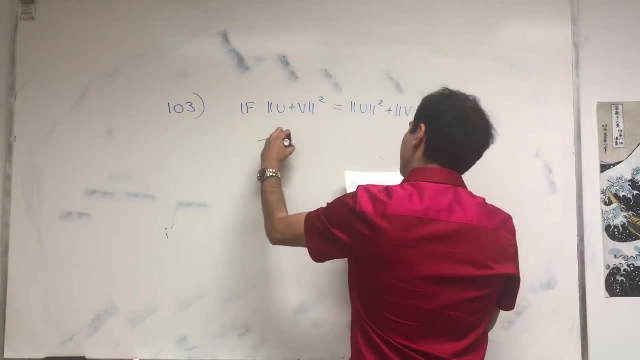 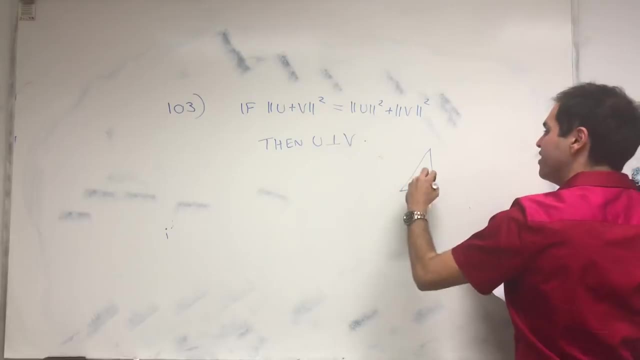 So it's not true for complex ones. then U dot V, So then U is perpendicular to V. In other words, if you have a triangle with the property that U plus V squared is U squared plus V squared, then it's a right triangle. 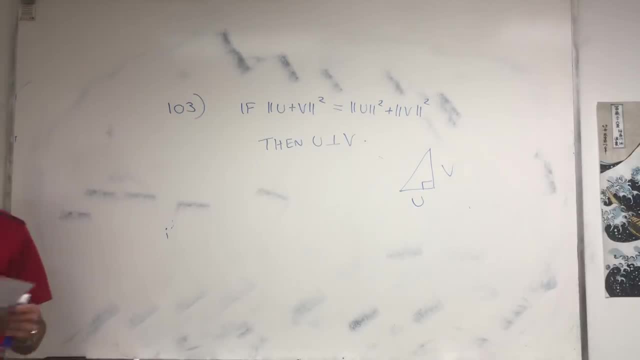 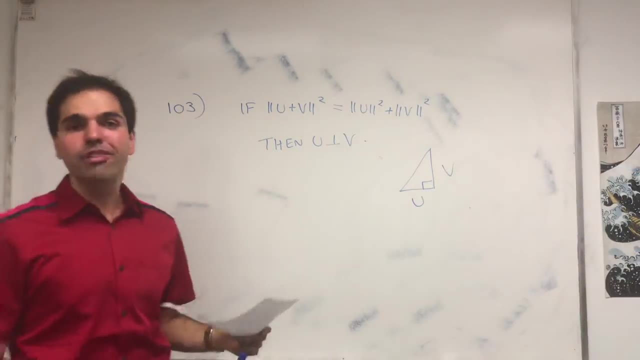 And 103rd language is the eastern version of Farsi, So it turns out the western version is much more popular. And well, 103 in Farsi is Sadose- I don't know what the dialect is. That said, well, this is true. 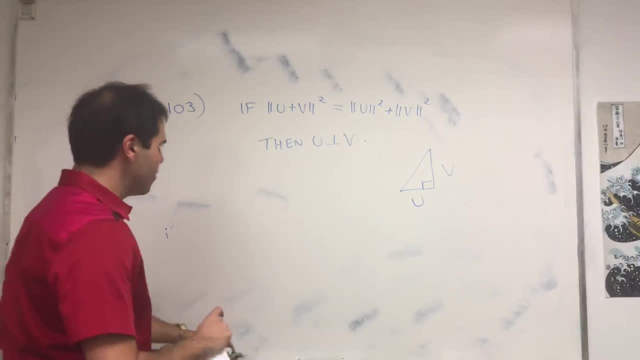 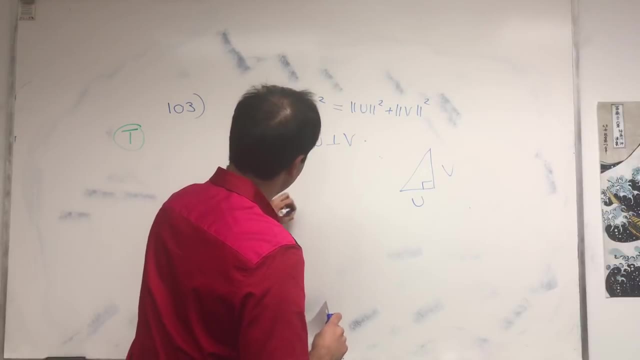 with the reciprocal converse of the Pythagorean theorem. And let me show this. Well, U plus V squared. well, by assumption, it's U squared plus V squared. But if you expand this out, this is U plus V, dotted with U plus V. 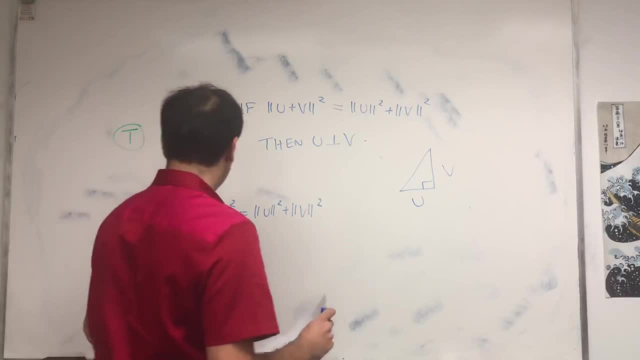 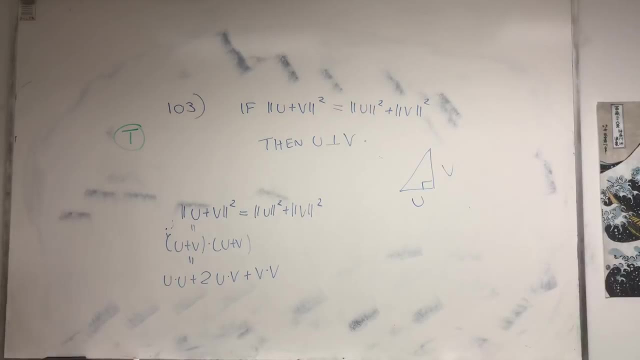 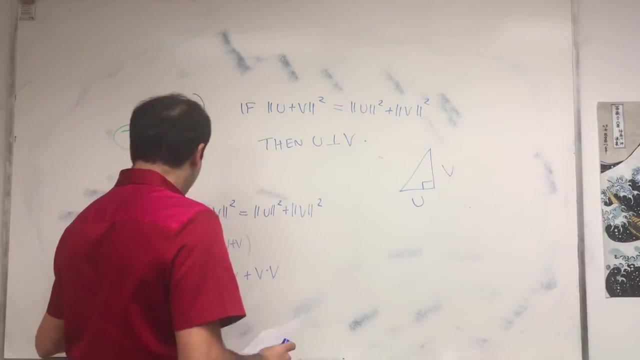 and that's U dot, U plus, basically two U dot V plus V dot V, Which again, by the way, it's not quite true for complex inner products, inner product spaces. you would have sort of u plus v plus u plus v bar and this: 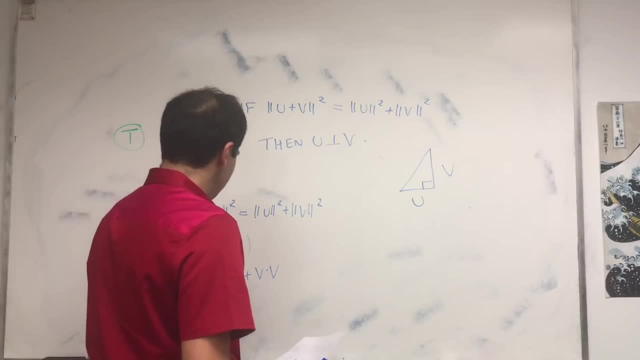 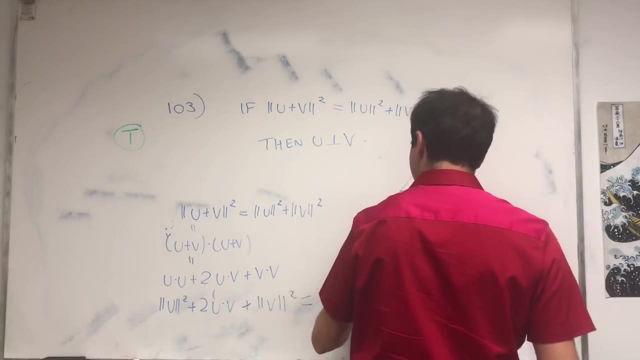 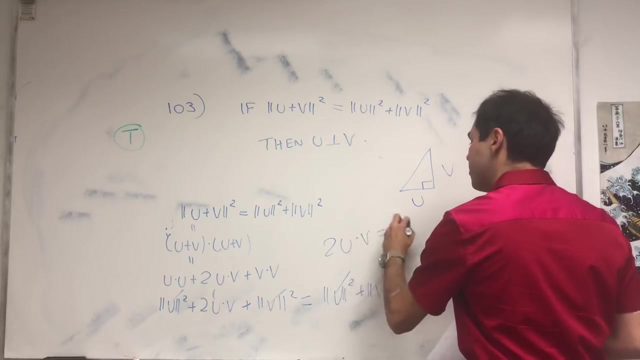 is just length of u squared plus 2 u plus v dot v plus length of v squared. this is equal, and we know this. equals to length of u squared plus length of v squared. everything cancels out and you get 2 u dot v equals 0. this cancels out. 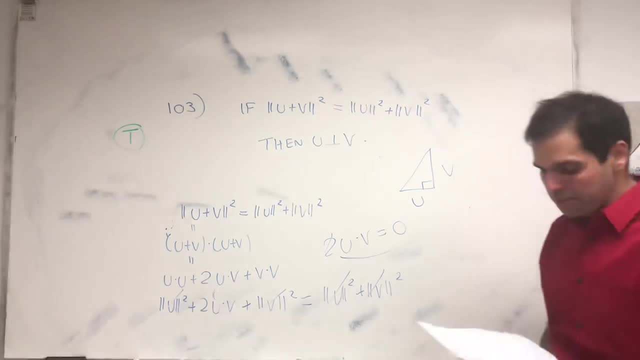 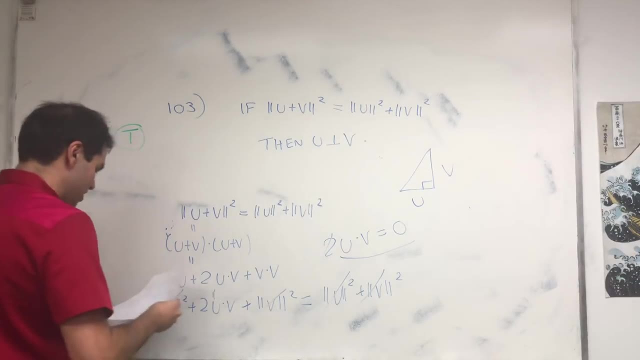 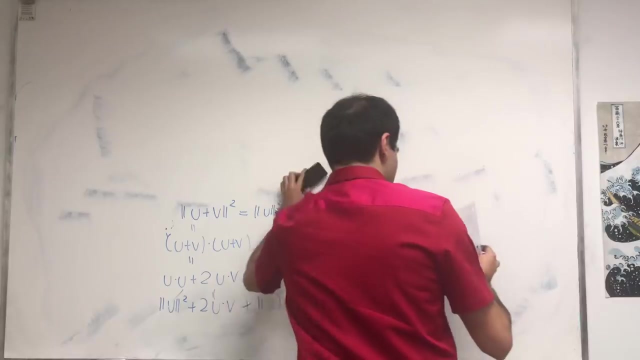 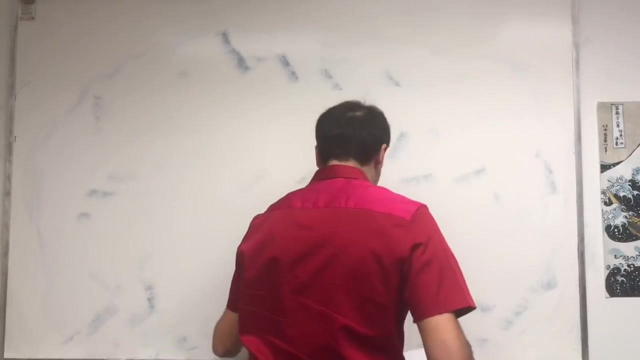 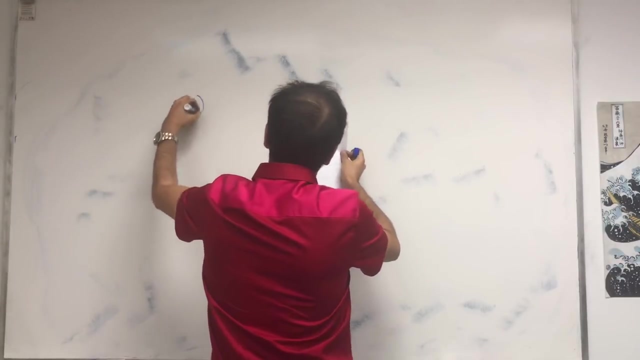 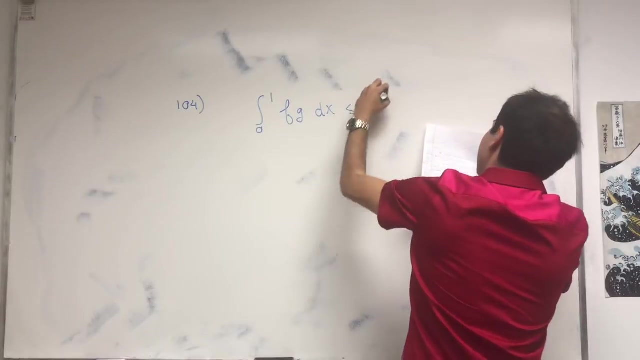 and you get u dot. v is 0, so u is perpendicular to v. okay, three more questions in that section. okay, I wonder if I should. no, let's not switch to black yet. okay, so, okay, so, okay, so 104. the integral from 0 to 1 of F, G, DX is less or equal to the integral from 0. 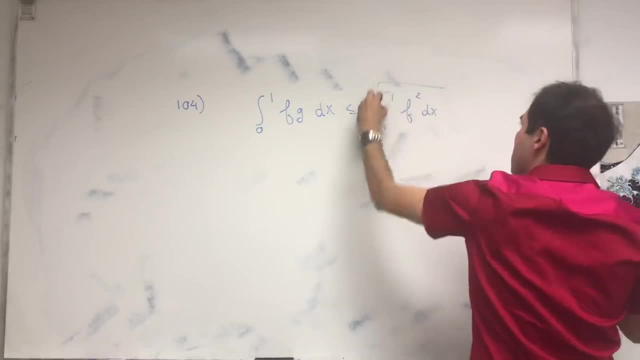 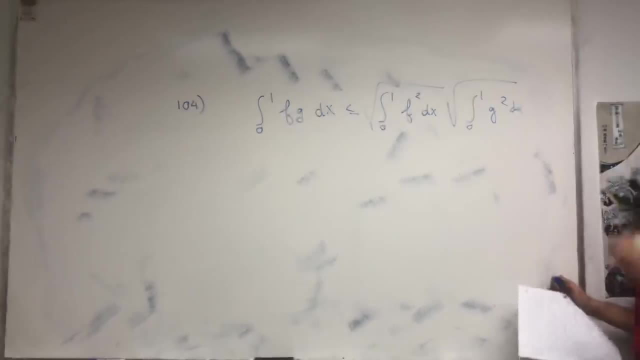 to 1 F squared DX. square root times the integral from 0 to 1 G squared DX. hey, look at that black pen, red pen. I do have some integrals here and you're like, what the hell do integrals have to do with here? probably with some inner products. 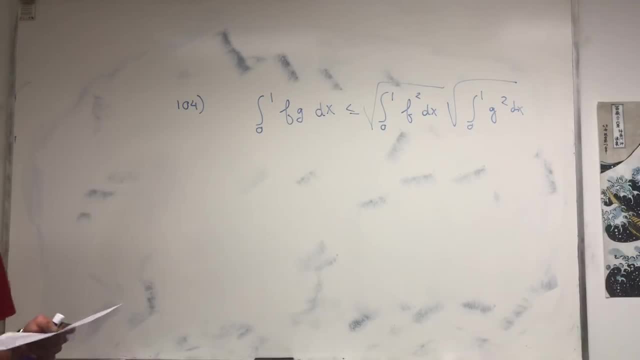 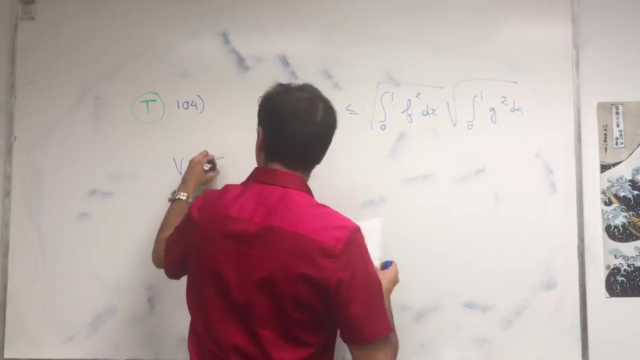 and then 104, so a con. so not a con but a con, and I think it's a char name and turning on, okay, and this weird formula, it is true, and in fact let's write it in terms of inner products. so in this case, let me so our vector space through the space of continuous functions from zero to one, because we integrate from 0 to 1 and F don't have one, because if you take 0 and you integrate derivative from 1 to 1, you get of. okay, I think that's cool, and but then going зам, uh, let's just, let's leave 我是. 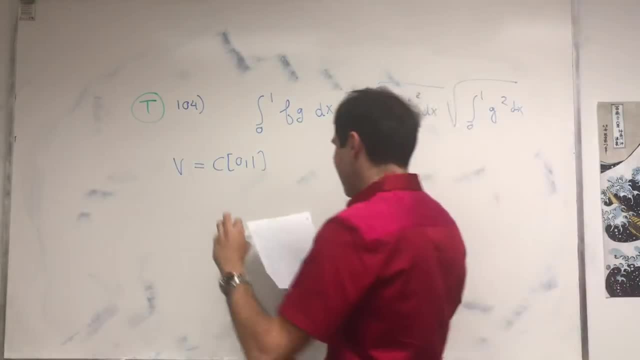 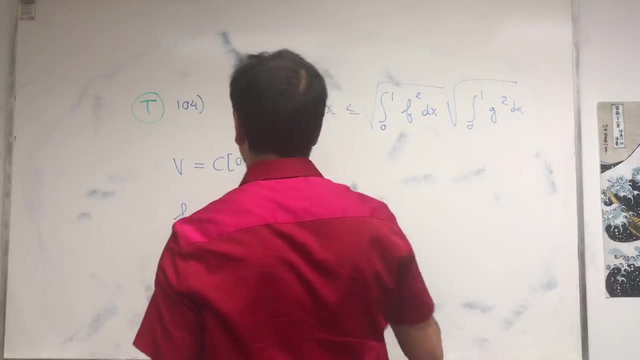 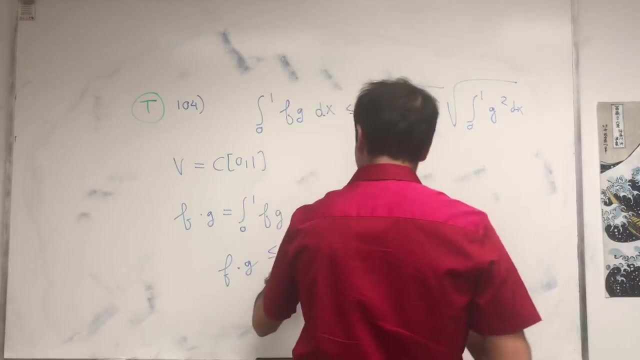 from zero to one, because we integrate from zero to one, and f dot g equals to integral from zero to one of f g. okay, what does that tell us? it's an feg, okay. and it just tells it: f dot g is less than or equal to the square root of f dotted with f, so length of f times length of g and. 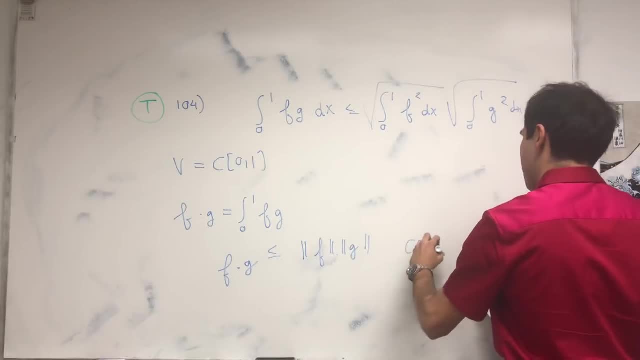 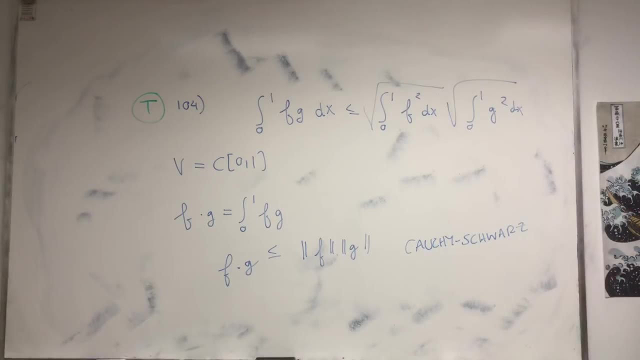 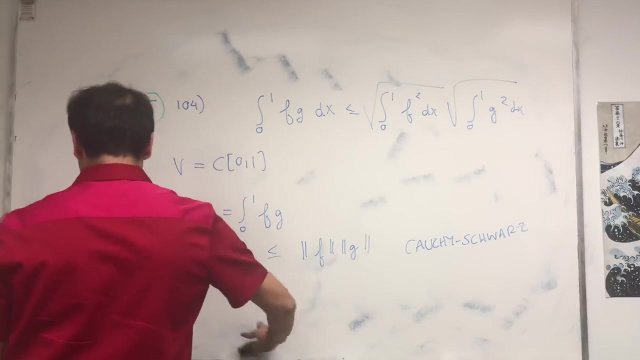 that's just the Cauchy-Schwarz inequality. so that's why abstract math is actually useful. sometimes it allows us to take something very strange and rewrite it in a clean way. in particular, this is true because it's just a Cauchy-Schwarz inequality. okay, next, 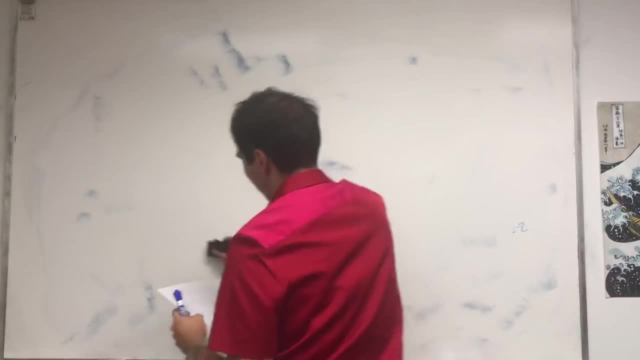 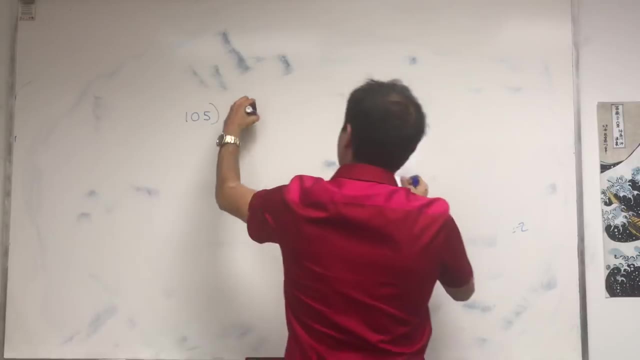 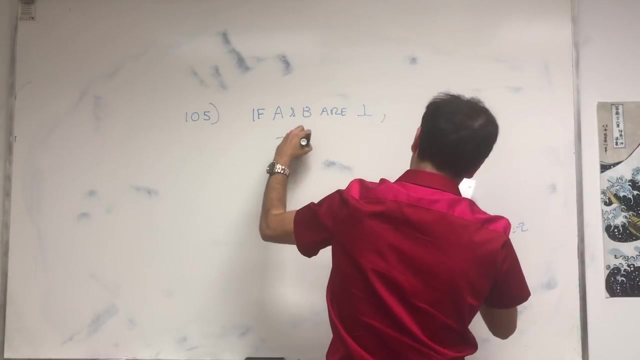 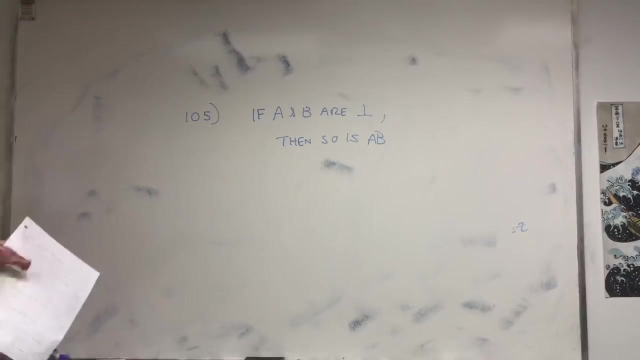 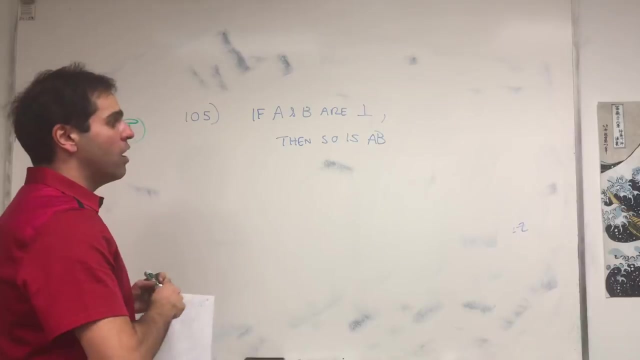 two little questions, questions with like matrices and orthogonality. so 105. so if a and b are orthogonal, then so is a b. the proof is up proof or maybe false. so 105. so Hilli-Gainon and it's Gattuso. Okay, well, I gave it away. It is indeed true because, remember, orthogonal matrices are. 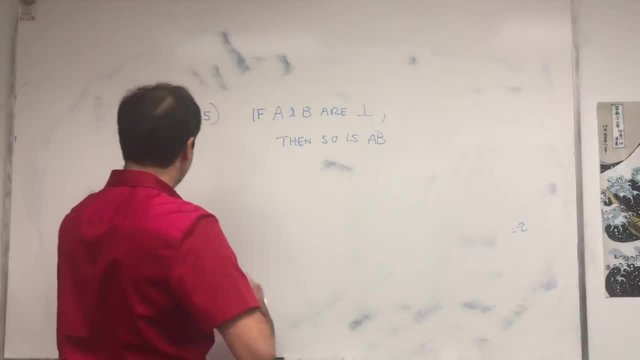 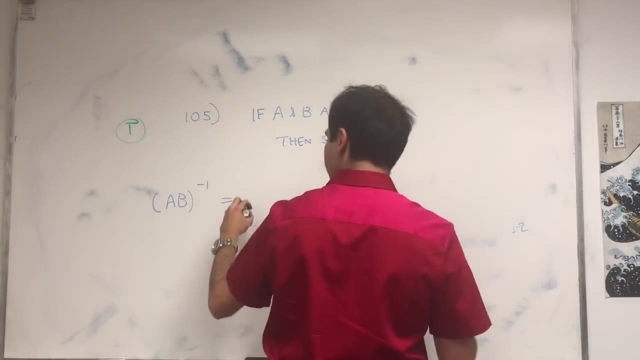 square and okay, I assume that AB is defined. so in particular for square orthogonal matrices we can calculate the inverse. So AB inverse is B inverse, A inverse. but now, because A and B are orthogonal, that B transpose, A transpose and then that's just AB transpose. 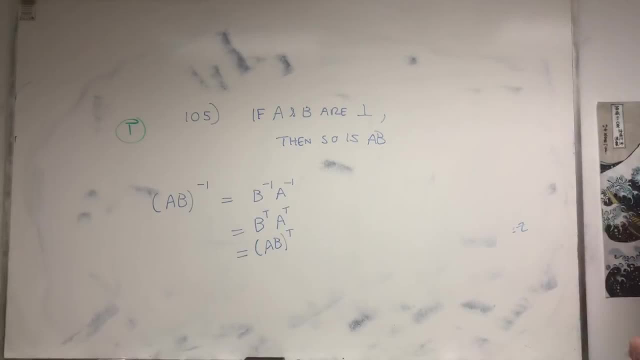 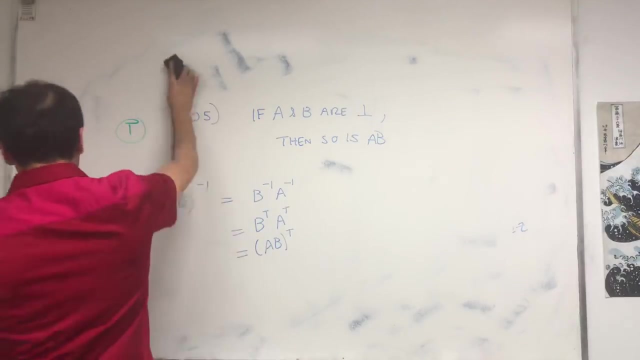 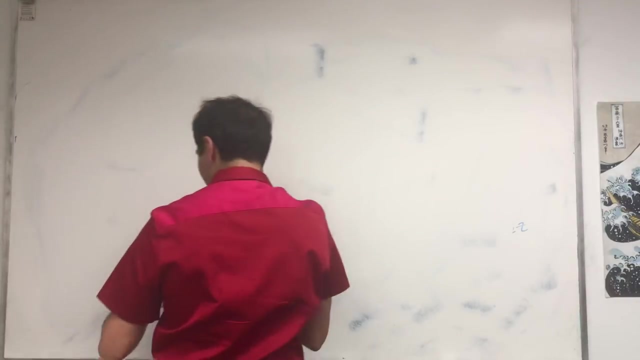 and therefore AB inverse is AB transpose, and both are square. so that's just consequence of orthogonal matrices. So indeed it is true. And last question of this section, and then one more part left, but that one's shorter: 106.. 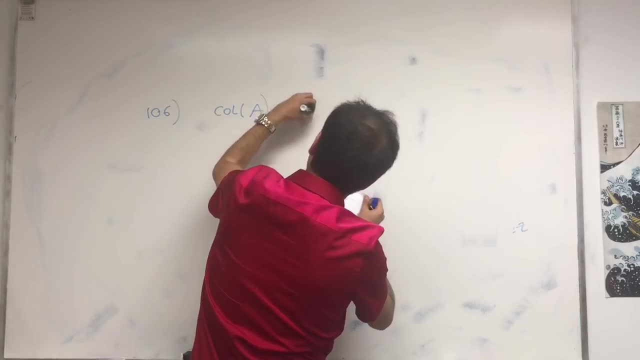 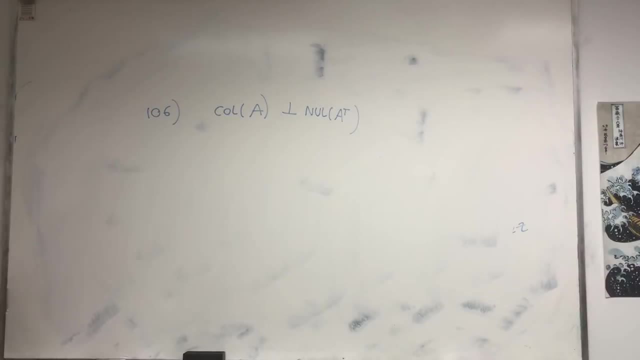 Is it true that the column space of A is perpendicular to the null space of A transpose? So weird. there's two spaces, Are they, or are they not related? And 106 is, I think, Kurdish, so kurmanji. 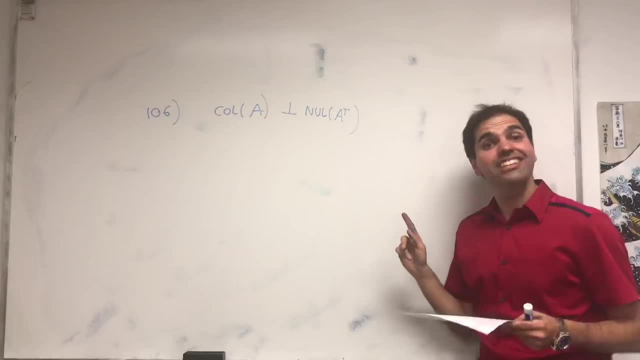 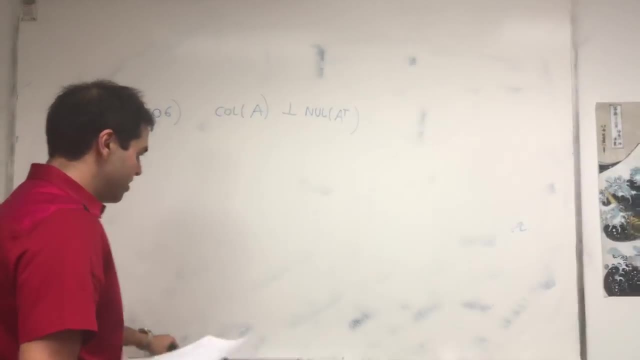 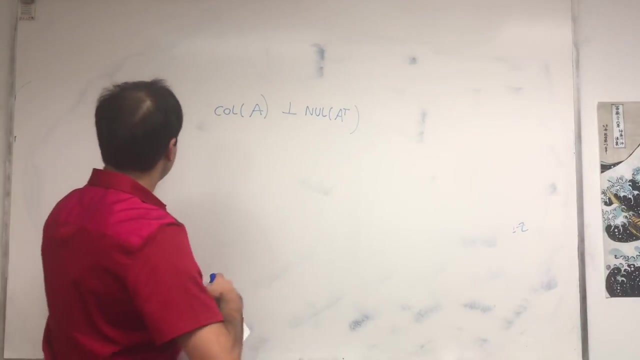 and it's sedoshesh, because it's interesting, in Farsi it's sadoshesh and now it's sedoshesh. Okay, and this is true. Let me show you again with the case of a two-by-two matrix. 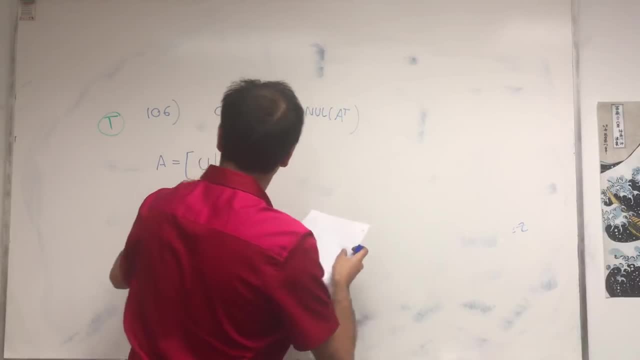 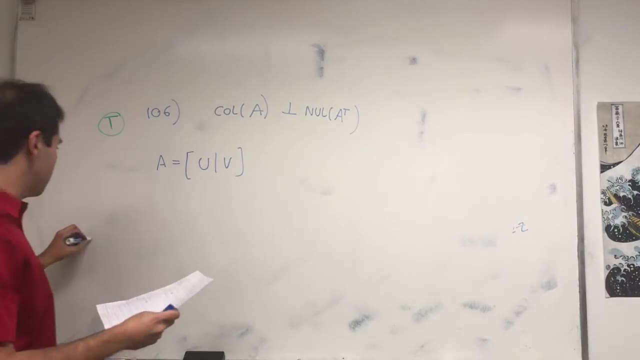 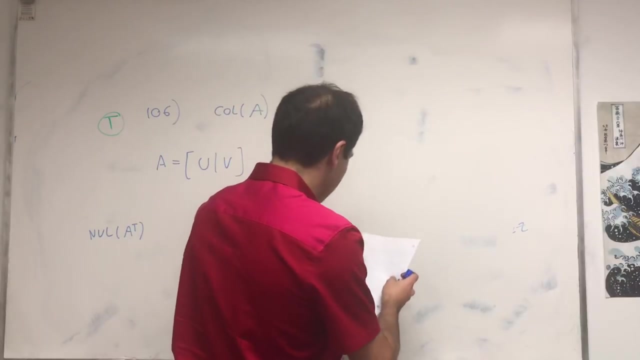 So suppose A is has, let's call it. suppose A has columns u and v, and then what is the null space of A transpose? Well, first of all, A transpose has rows u and v and the null space is just the set of x. 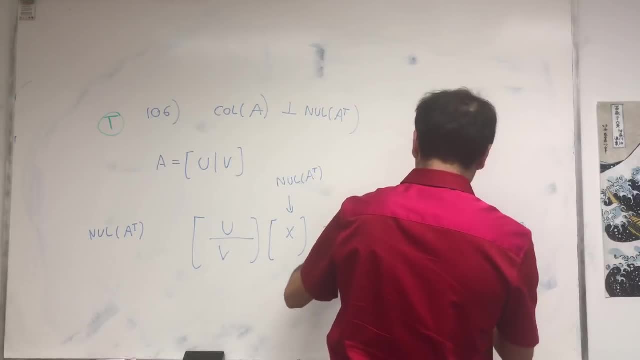 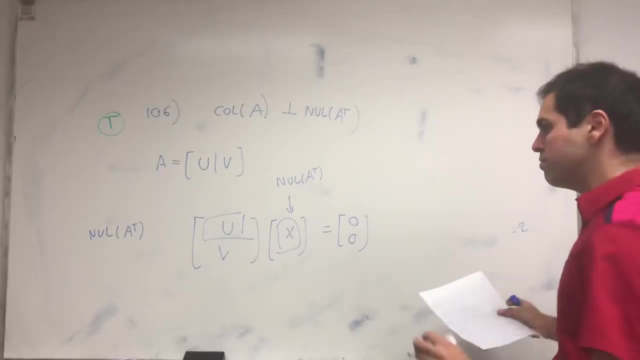 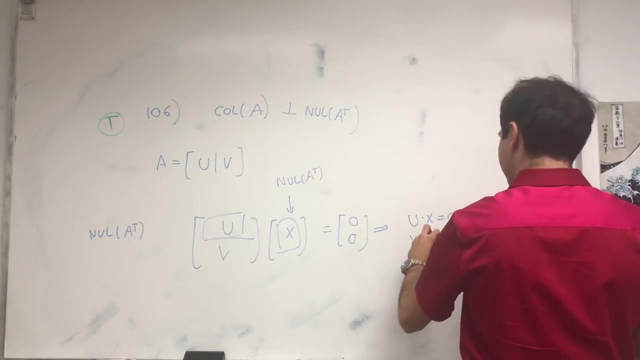 for which this: this is zero. So I think zero is zero. And again, remember the dot product version of multiplying matrices. that just means u dot x equals zero and v dot x equals zero. In other words, x dotted with u equals zero. 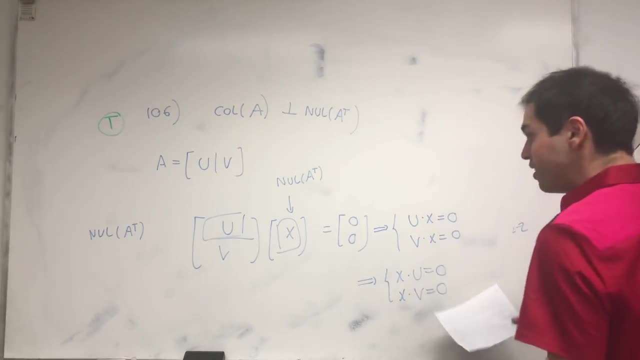 and x dotted with v equals zero. But what does that mean? It means a generic element in the null space of A and it means a generic element in the null space of A. the null space of A transpose is perpendicular to u and v. 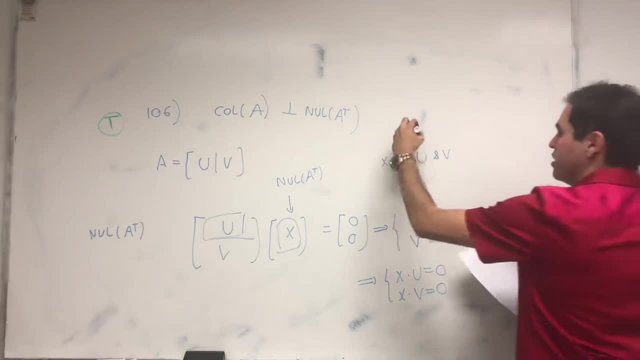 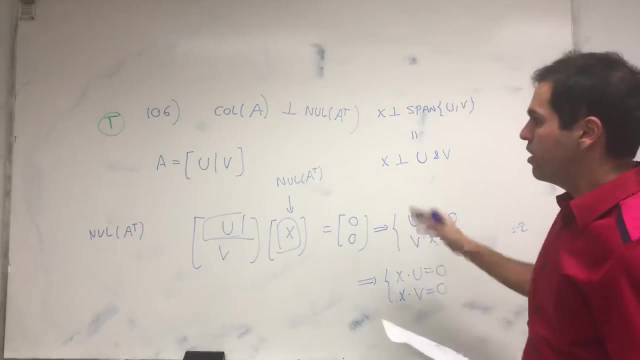 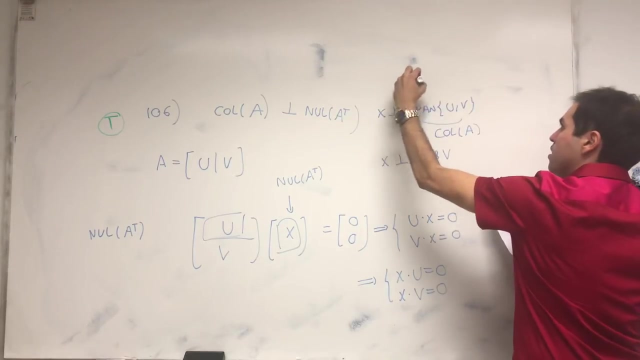 In particular, it's perpendicular to any combination of u and v. So x is perpendicular to the span of u and v. But what is the span of the columns of A? That's just the column space of A. X is perpendicular to the column space of A. 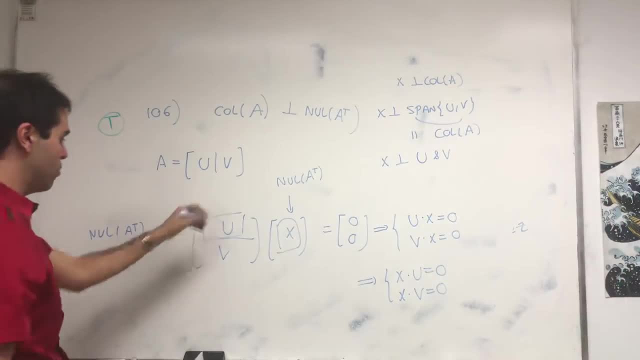 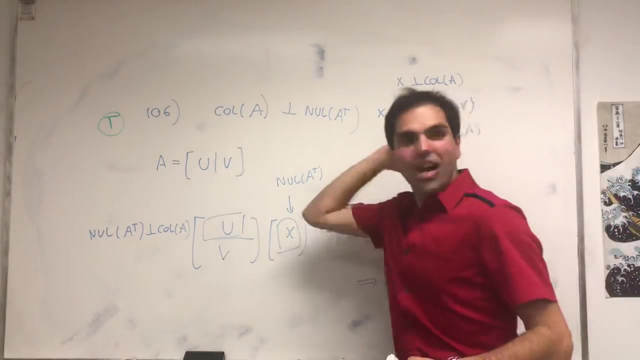 In particular, the null space of A transpose, you know, for any x is just perpendicular to the column space of A. Ta-da, All right, and this ends the section on orthogonality. One more part left, just symmetric matrices. 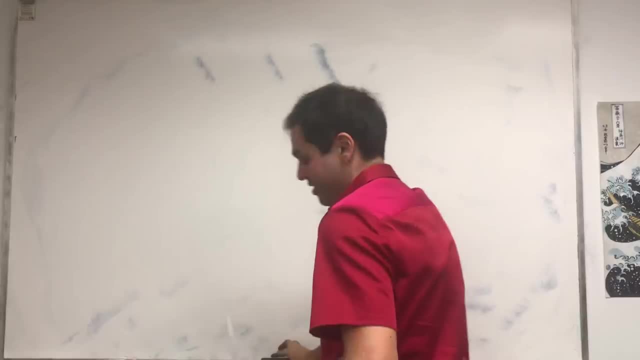 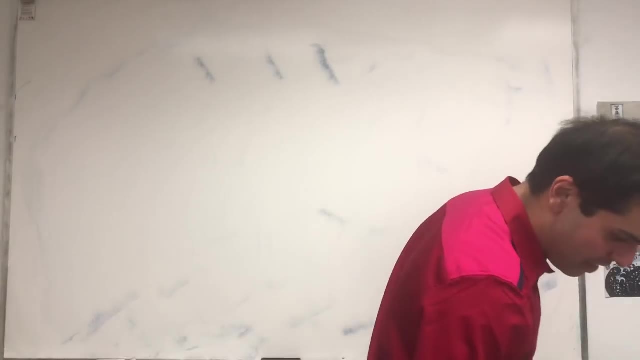 Ta-da And let's see, oh my God, how much time. Okay, four hours, Four hours and 12.. So yeah, just one, two, three, four, five. we have one, two, three, four, five questions left. 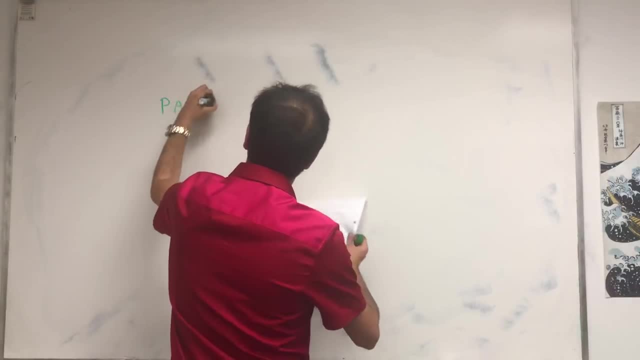 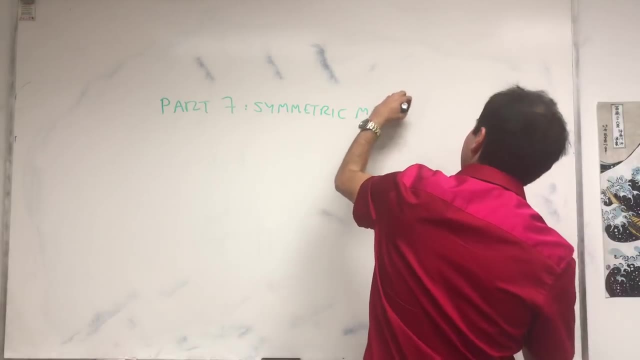 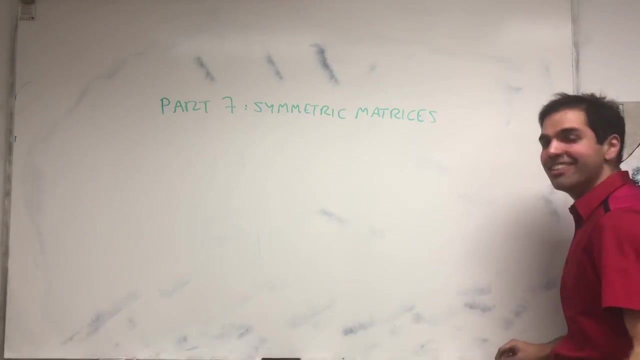 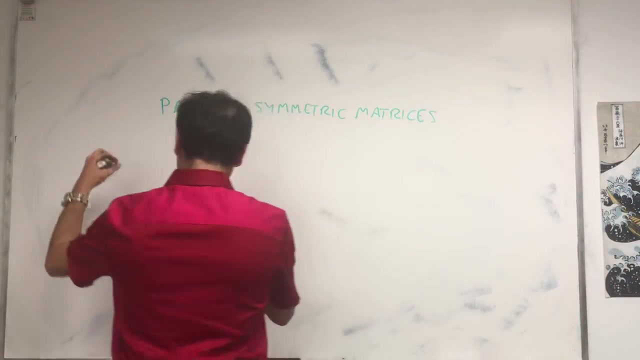 So part seven, the grand finale. By the way, you have to appreciate Blackburn-Redburn. He took like six hours to do his integral, so already here I'm doing just four and a half hours hours and you know it's already dying. so all right, question 107: so ah, one of my. 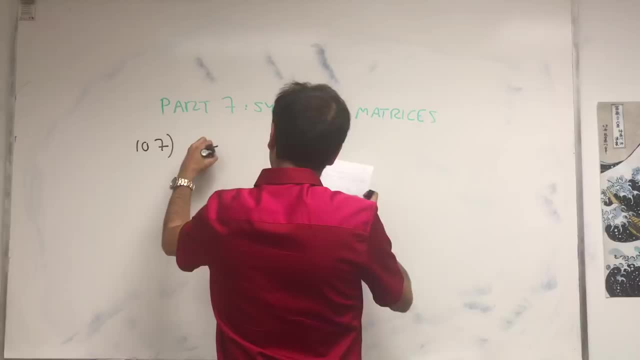 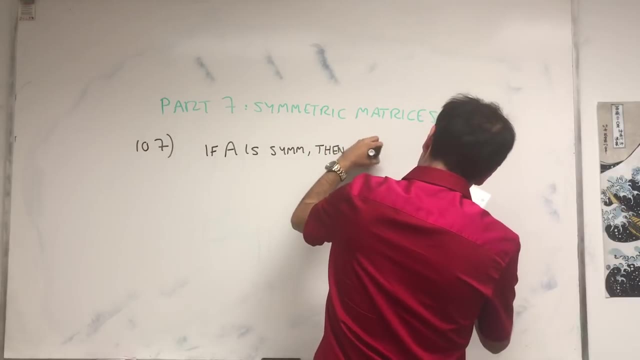 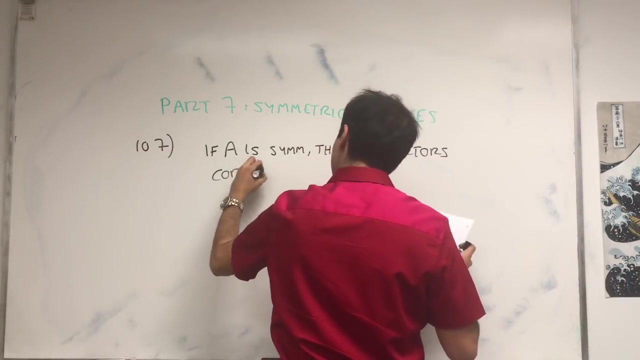 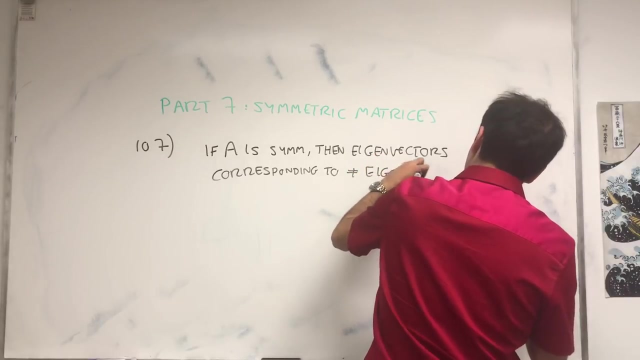 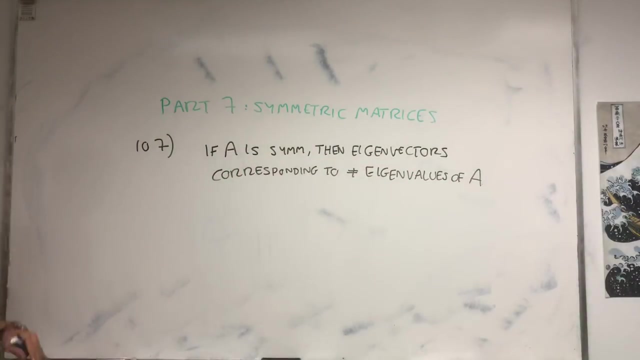 favorite proofs or non proofs. so if a is symmetric, then eigenvectors corresponding to different eigenvalues eigenvalues of a okay one. so in general, if you take and these nonzero eigenvectors corresponding to different eigenvalues, we know they're linearly independent. the question is if your matrix is. 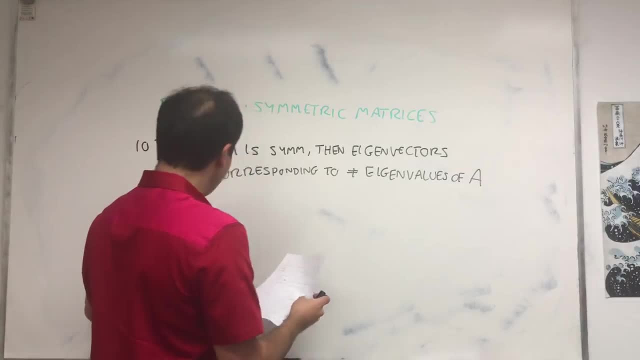 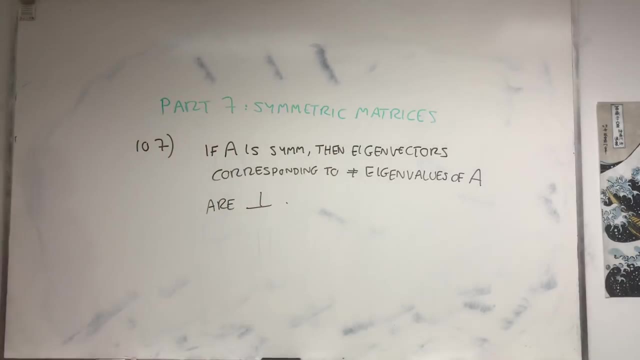 symmetric. and if you take a non-zero eigenvectors corresponding to different eigenvalues, we know they're linearly independent. the question is, if your matrix is symmetric, can we say more about this? in particular, is it true that they're orthogonal or not? obviously, the way I said it, it is true, so maybe it's. 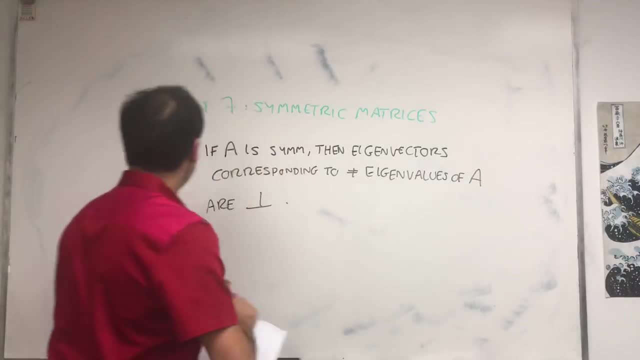 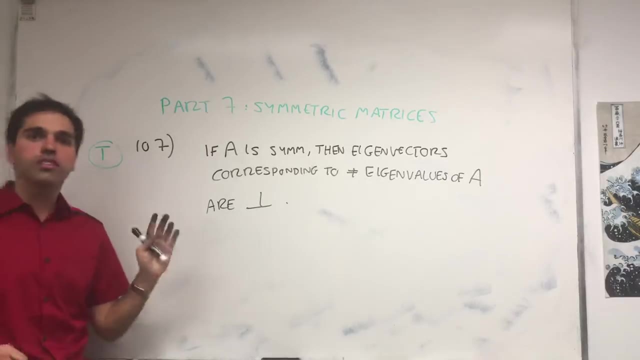 not beat around the bush. so it turns out, if a is symmetric, eigenvectors corresponding to different eigenvalues are not just linearly independent, they are orthogonal, and the language here is Shonazana and it's Nemakumi Manombe. okay, let me show you why. suppose you have two. 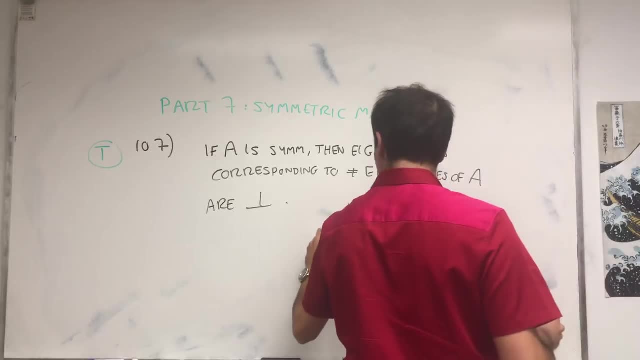 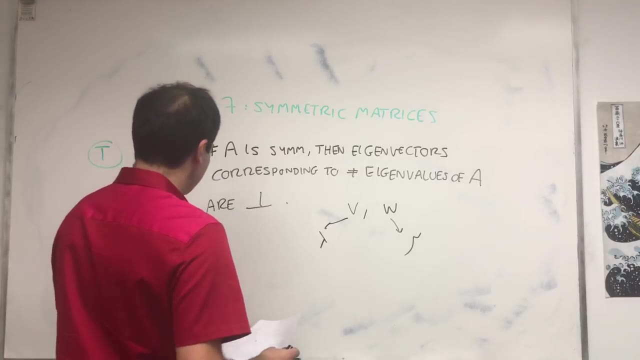 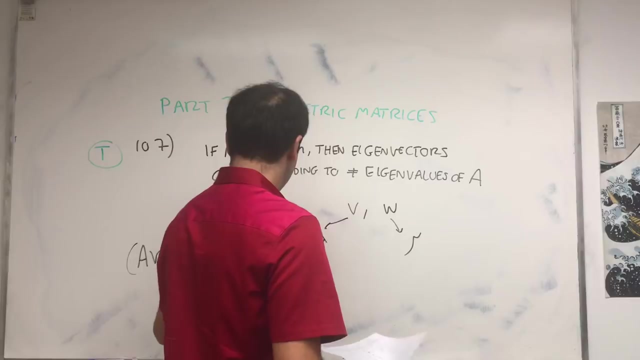 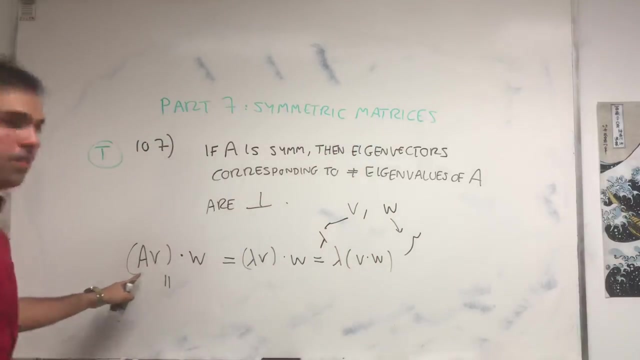 eigenvectors V and W, V corresponding to lambda, W corresponding to mu. consider the following expression: AV dotted with W. well, AV is lambda V, so it's lambda V dotted with W, so it's lambda times V dotted with W. now remember the dot product way of. 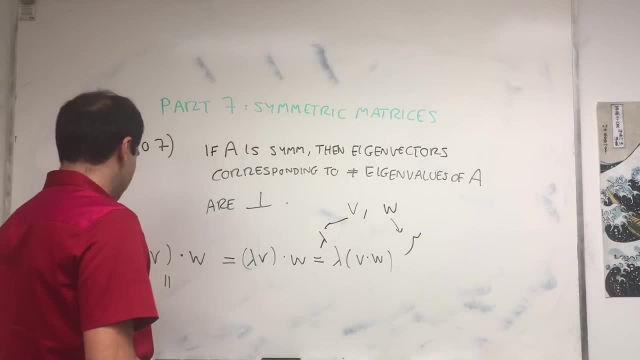 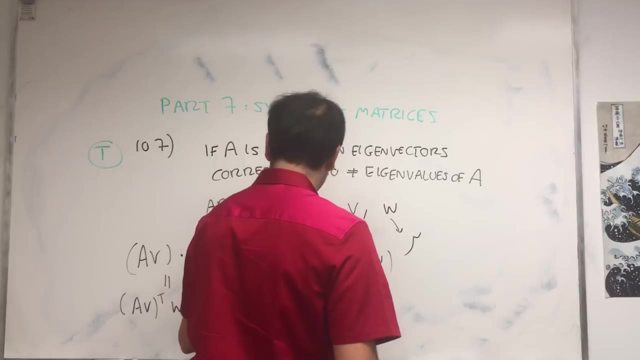 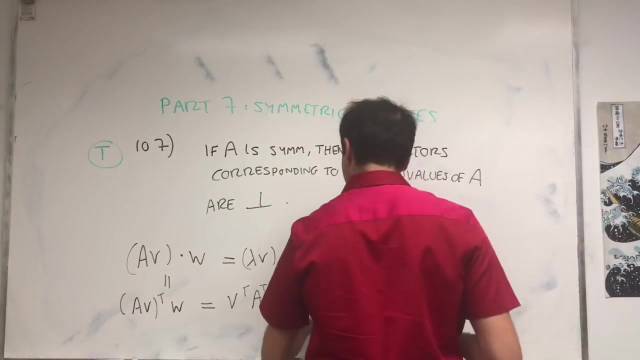 multiplying the transpose way of dotting matrices. so it's AB transpose times W, which is V transpose A transpose W. okay, in general this is gibberish, but A is symmetric, so A transpose is A. so it's V transpose A W, and that's really V transpose times A. 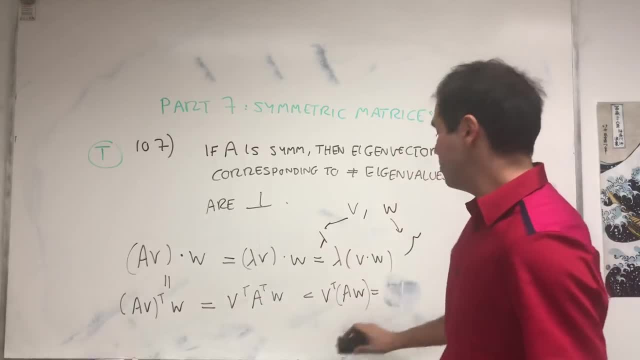 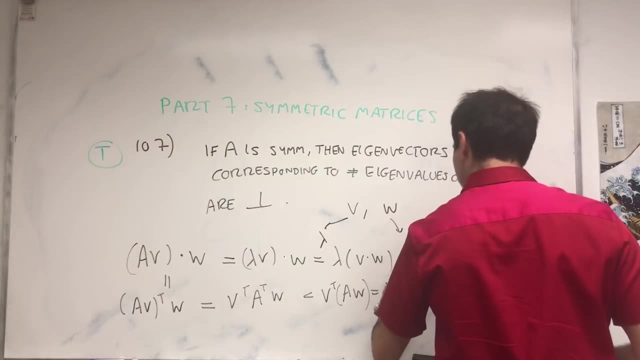 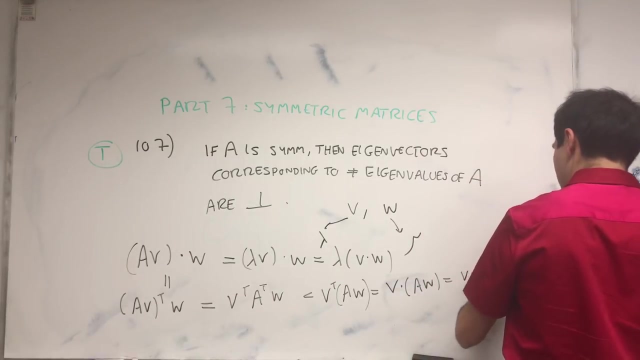 W. and now let's do the opposite of here. let's write transposes in terms of dot products. so it's V dotted with AW, but AW is mu W. so we just get mu times V dotted with W. so, following this whole logic, we get lambda times V dotted with. 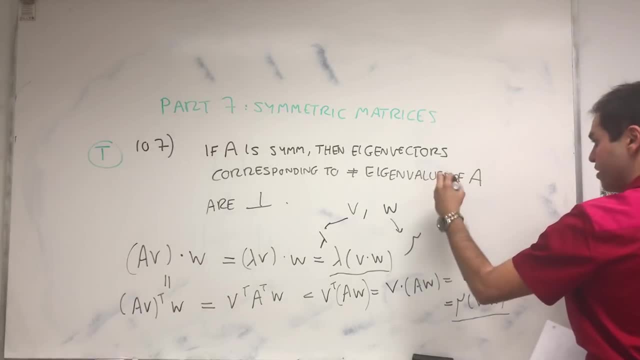 W equals to mu times V dotted with W. so V dotted with W equals to mu V dotted with W. so putting everything on the left-hand side, lambda minus mu, V dotted with W equals to zero. and now very important. in general this doesn't tell us much, but because those 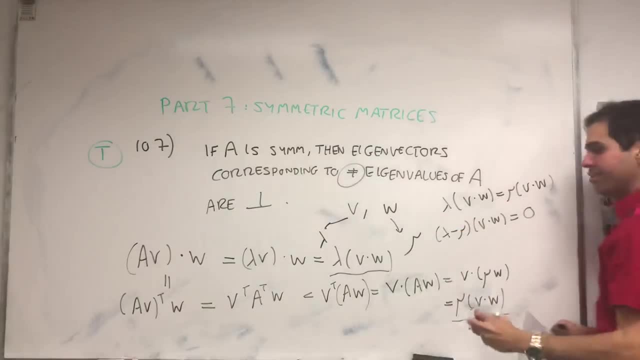 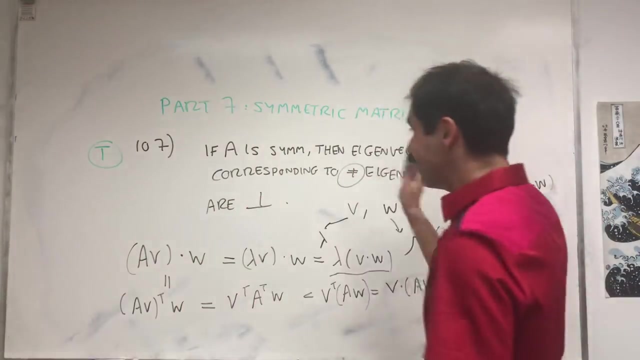 two eigenvalues are different, different eigenvalues. we can cancel this out and you get V dotted with W equals zero. in other words, V and W are perpendicular. so that's why it's nice, okay, and we're done with that. okay, so this is very strong, namely if you take two different 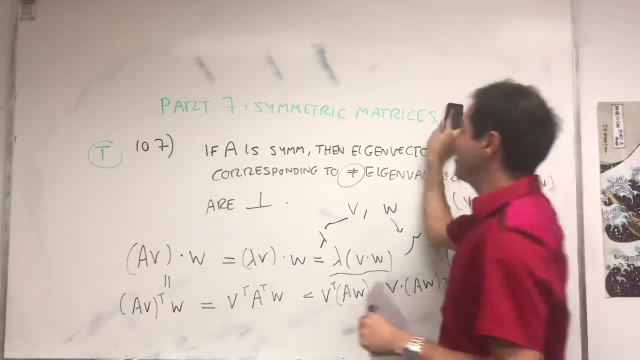 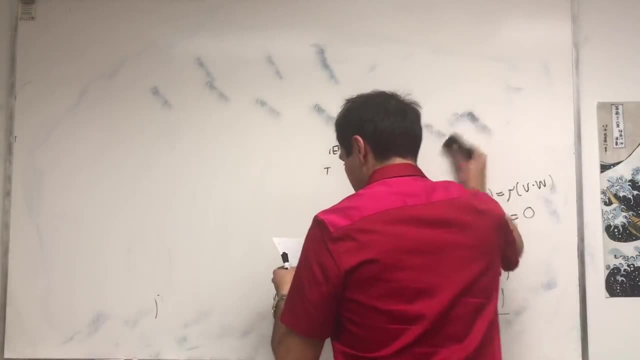 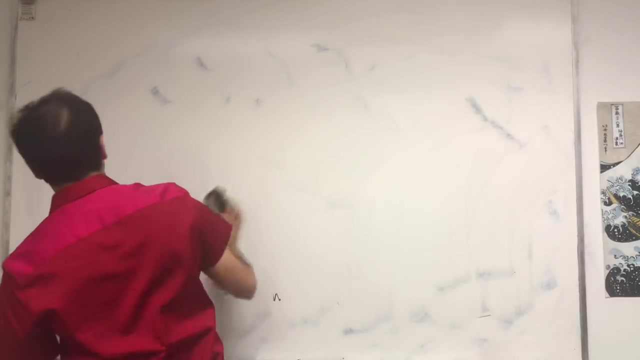 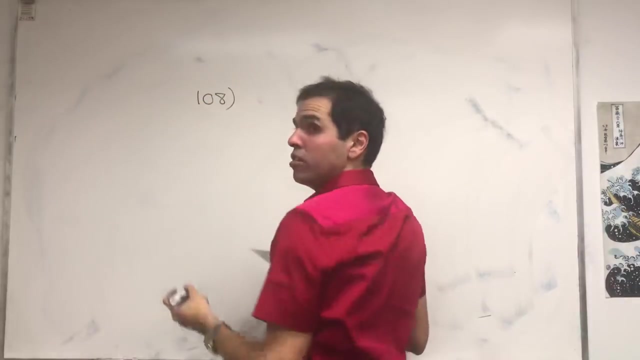 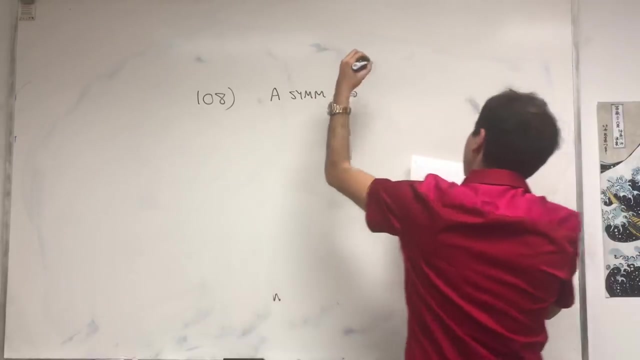 eigenvectors in different eigen spaces. they're perpendicular. okay, then the last sprint. so four more questions. so question 108: is there a matrix with symmetric matrix with complex eigenvalues? or in other words, if A is symmetric, does it imply A has only real eigenvalues? 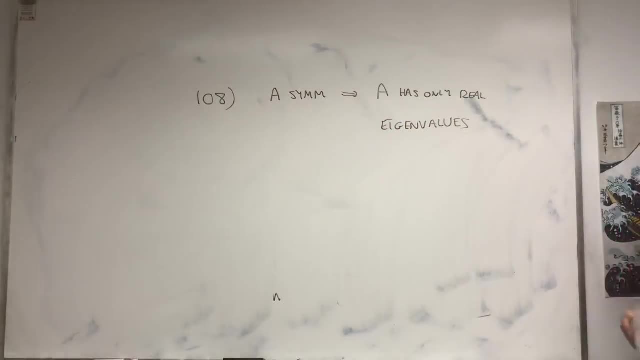 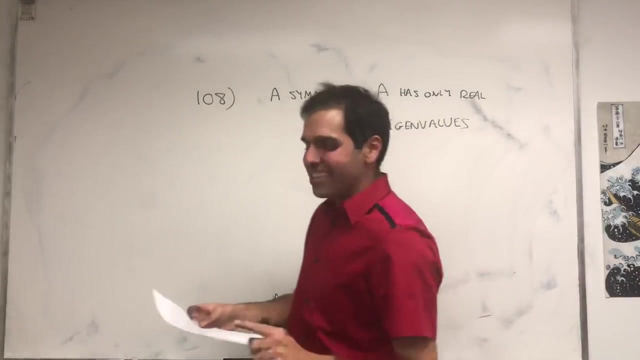 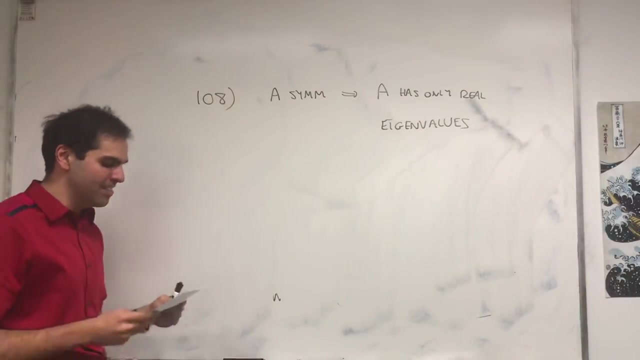 okay, let me also tell you something. okay. so the list. I had only had 107 most popular languages. so the next ones they're not. I don't think they're the most popular languages, but I just had to improvise a bit. so the last question: so 108. so my other office mates from last: 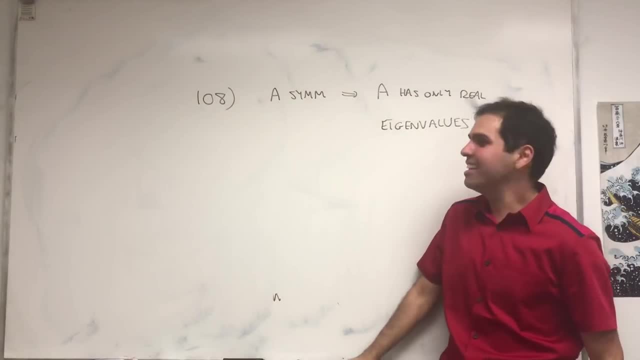 year and he got pissed because it was like why is situanes not in this list? and I was up and saying: why is situanes not in this list? so 108 in situanes isям. So 108 is situanes is not in this list of languages. because you'd get a call and 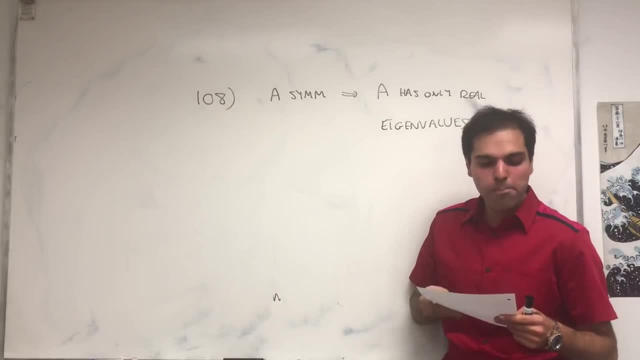 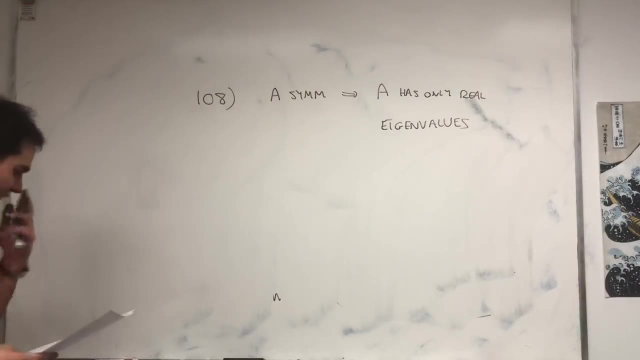 that's why I obedience my other office mates from last year. he got pissed because it was like why I have situanes not in this list? so 108 situanes- there were two categories in Sichuanese- is something. so this is true and in fact my statement was true and this is true. so 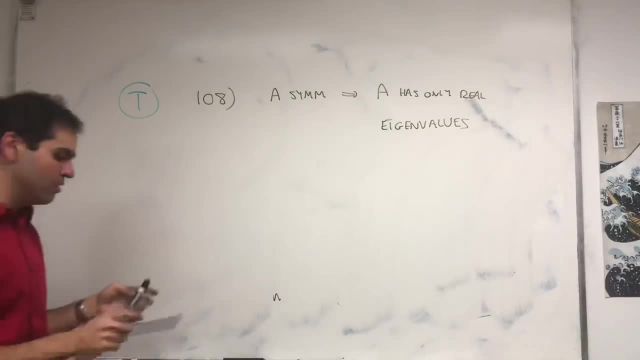 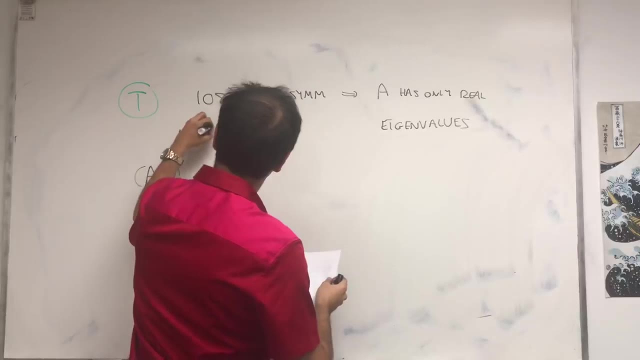 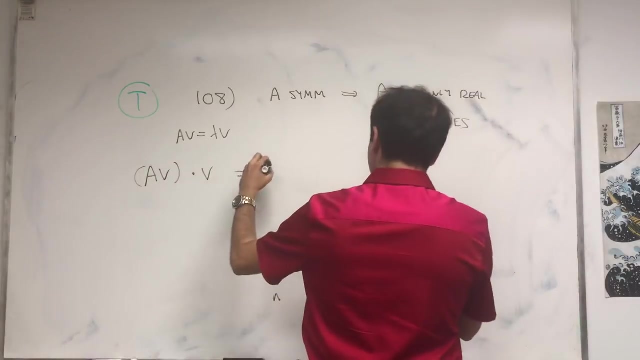 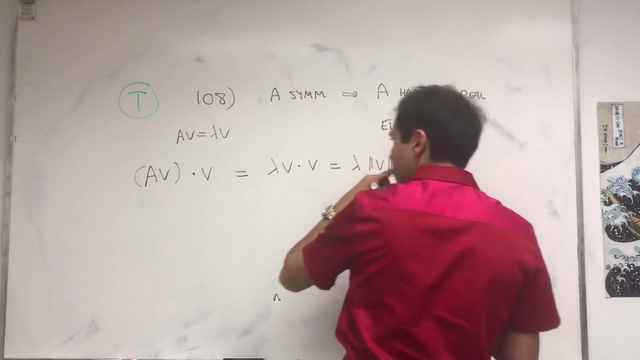 there are no symmetric matrices with complex eigenvalues, and the reason is as follows. so suppose V is an eigenvector corresponding to a eigenvalue lambda, then consider the following: Av dotted with V. on the one hand, it's lambda V dotted with V, so it's lambda times length of V-squared. on the other hand, 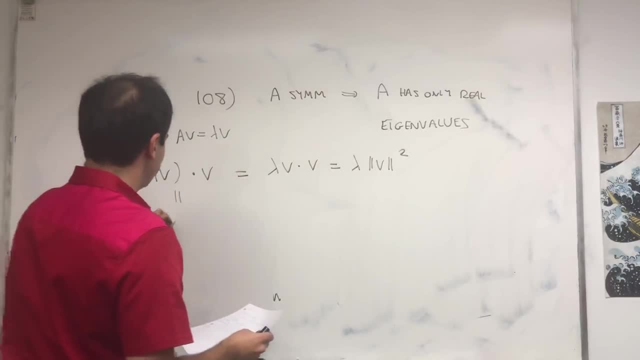 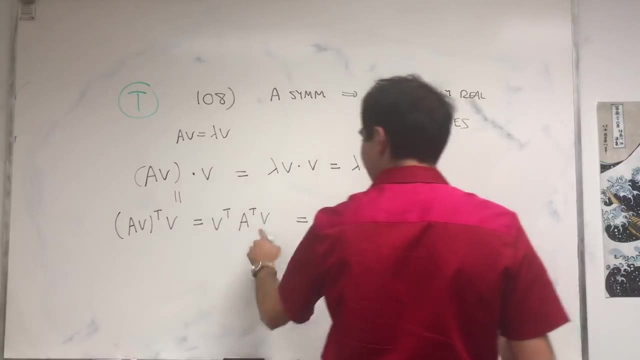 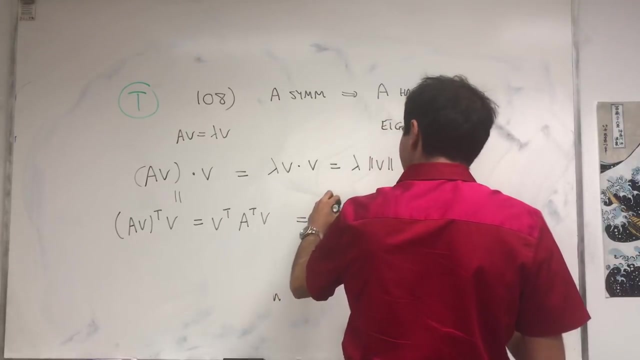 writing this in terms of transpose, so it's Ab transpose V. that's V. transpose A, transpose V, and that's so. A is what do I say? A is similar to a sorry Symmetric, so it's V. transpose times AV, and that's again V. transpose times lambda V. 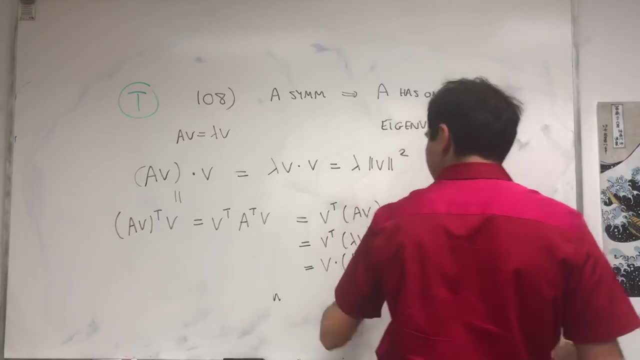 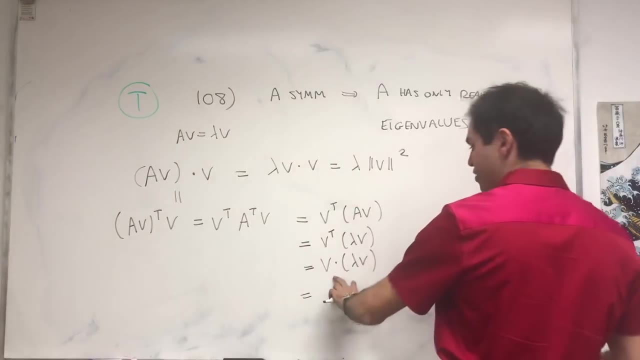 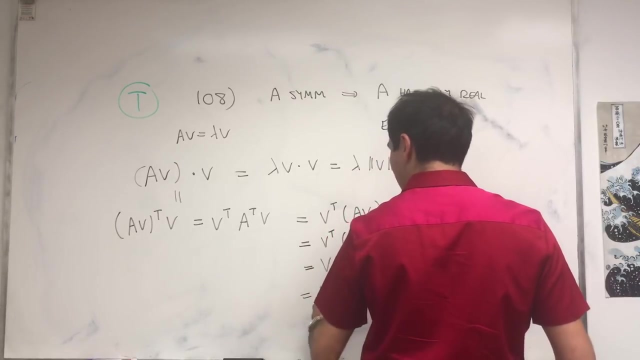 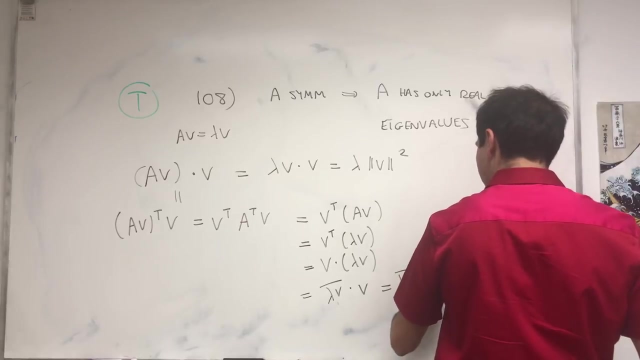 So what this becomes is V dotted with lambda V, and very important. so for What do I want to say? so, if you want to flip the two, then it becomes: You put a bar, so lambda, lambda V, bar times V, hmm, and that's lambda bar V, bar times V, and that's just becomes lambda bar times. length of V squared. 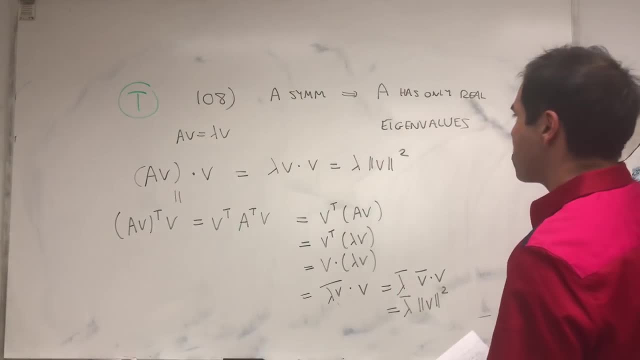 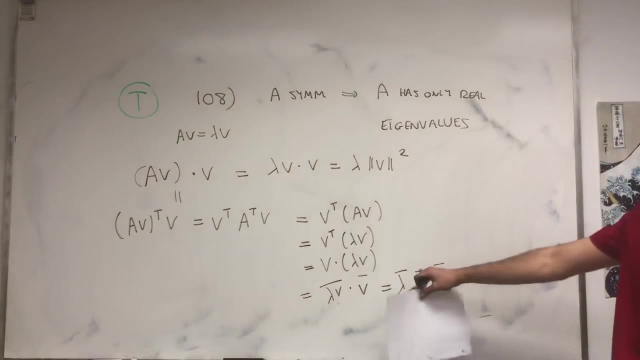 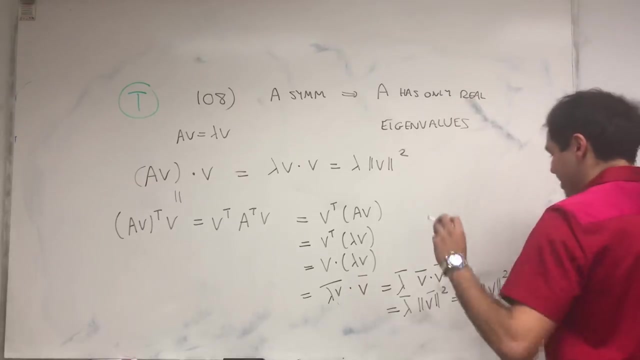 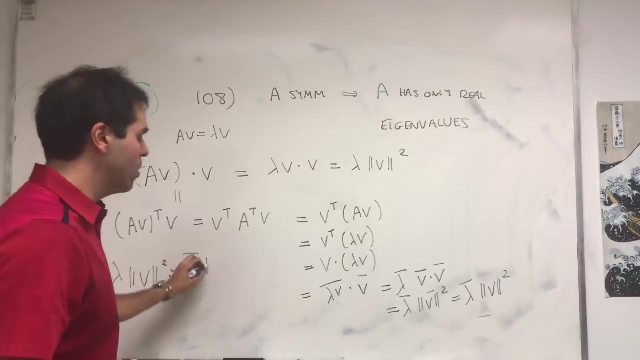 at least complex way, and V bar dotted with V bar. so it's length of V bar squared and that's the same thing as the length of V squared. Okay, there we go. So what do we get? lambda times length of V squared equals to lambda bar times length of V squared. 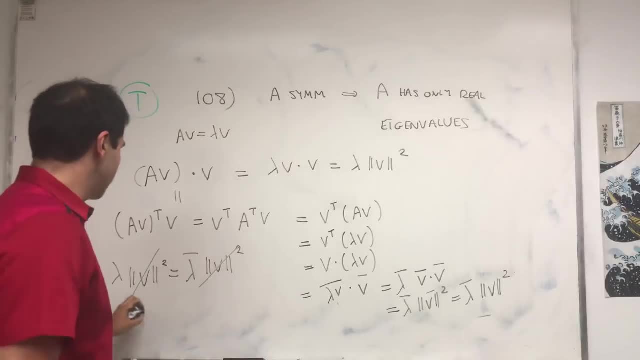 Well, V is a nonzero eigenvector, So this cancels out and we get lambda equals to lambda bar, And so a lambda walks in the bar and you say, hey, it is real. So in fact, that symmetric matrices only have real eigenvalues. It may be easier than that. 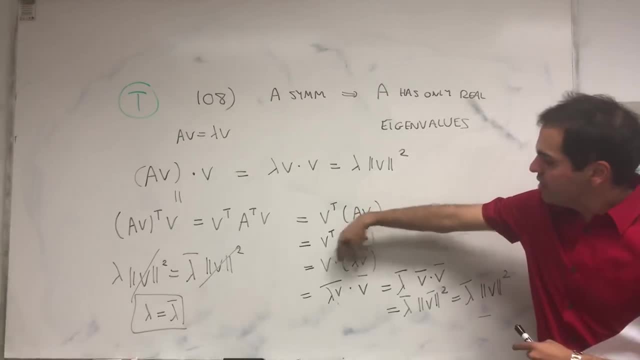 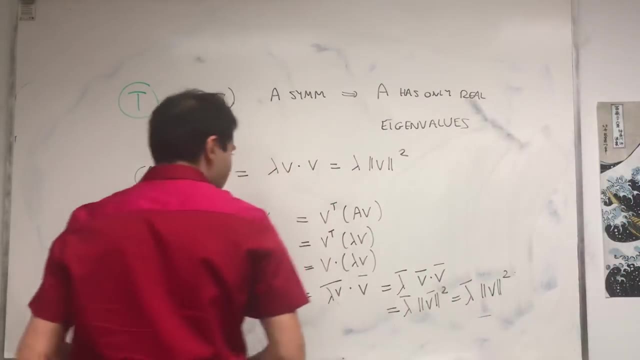 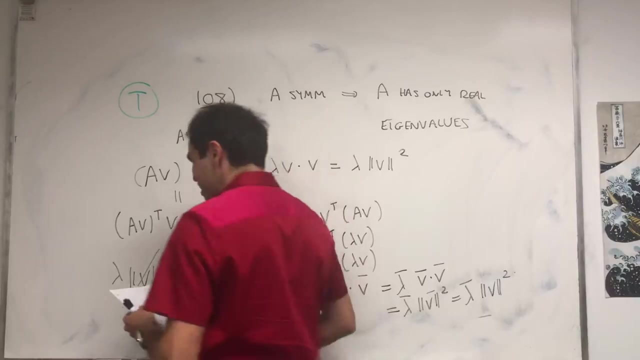 Yeah, Yeah, or maybe you just flip it and then you, if you take this lambda out, you get a lambda bar. That's another way of doing this. Alright, good, anyway, so we have that. so symmetric matrices only have real eigenvalues. now next question: So we saw that. 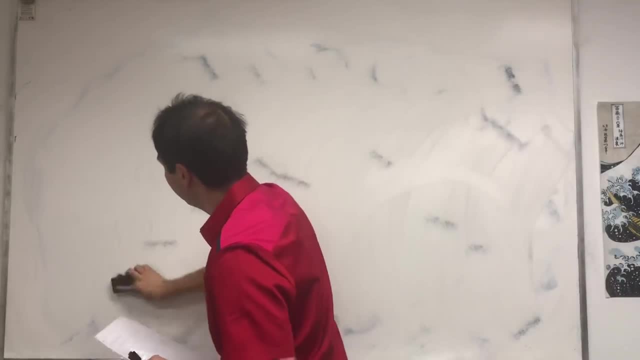 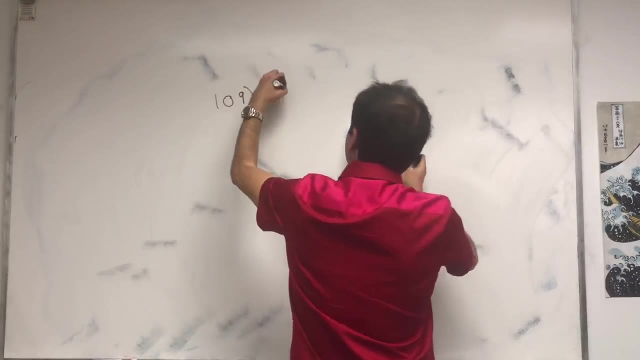 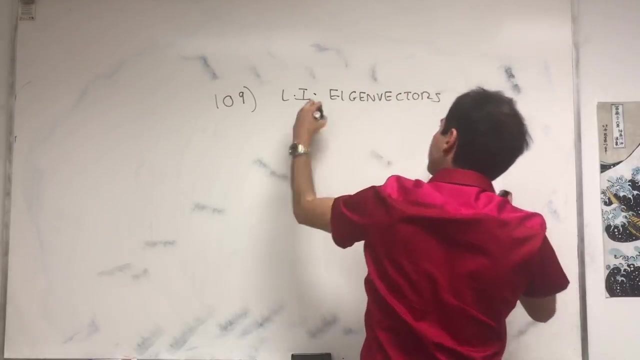 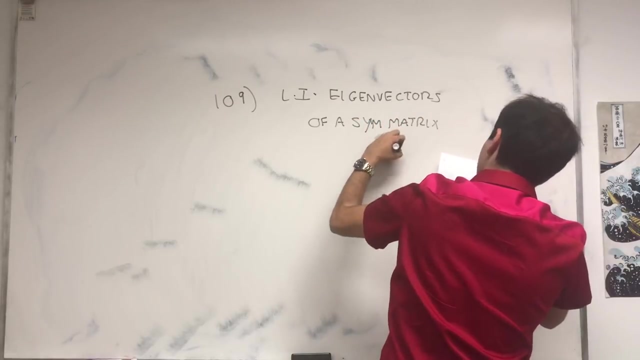 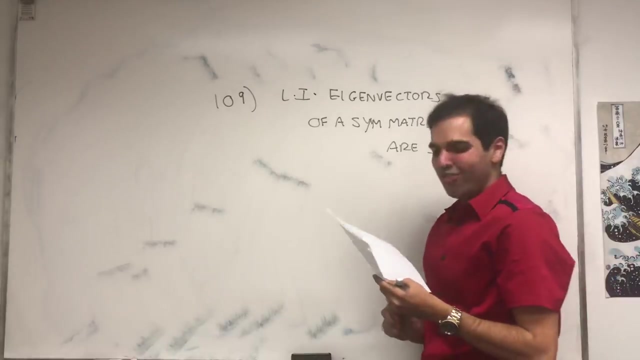 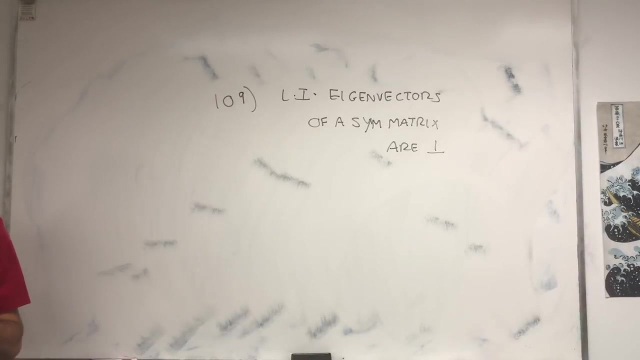 Eigen value. eigenvectors corresponding to different eigenvalues Are orthogonal in the symmetric matrix case. Question is: are linearly independent eigenvectors Of a symmetric matrix Are orthogonal? And 109- because I'm almost finished, Let's do finish. I think it's um, oh, my god, Okay, It's a shot, Ah yeah. 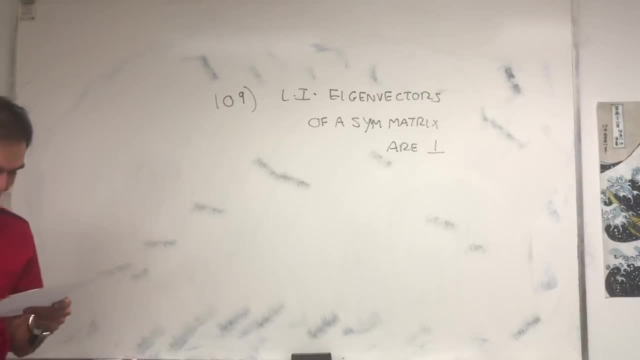 Big John, I think I think so anyway. so So linearly independent eigenvectors of a symmetric matrix, orthogonal, Very important. It's important that they correspond to different eigenvalues. so we showed before that if you have So eigenvectors corresponding to different eigenvalues, if it's symmetric, they're orthogonal in general for the same eigenvalue. 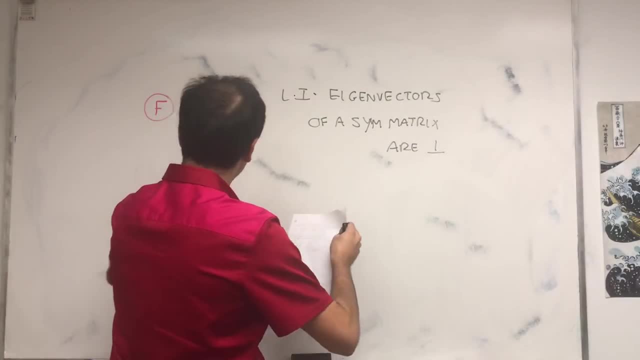 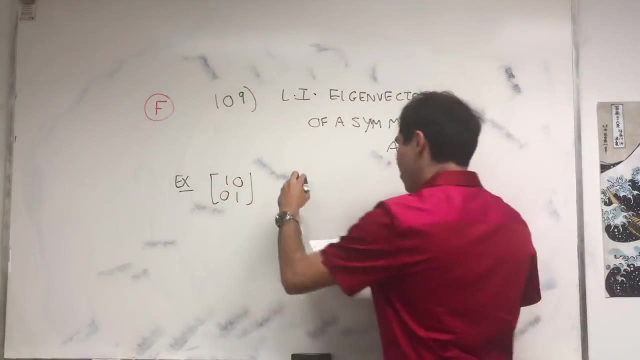 They're not linearly independent. Let me give you an example. take a 1, 0, 0, 1. Well, anything is an eigenvector for this matrix. So if you have, let's say, the set 1: 0 and 1: 1, 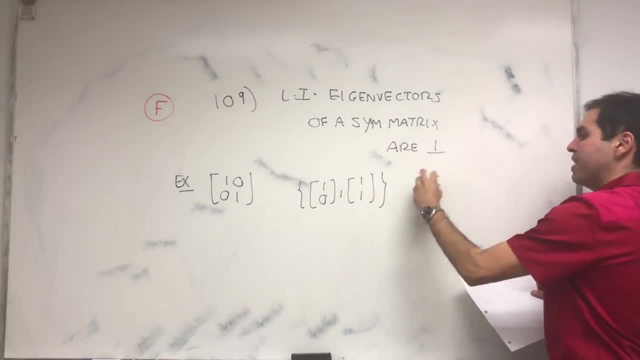 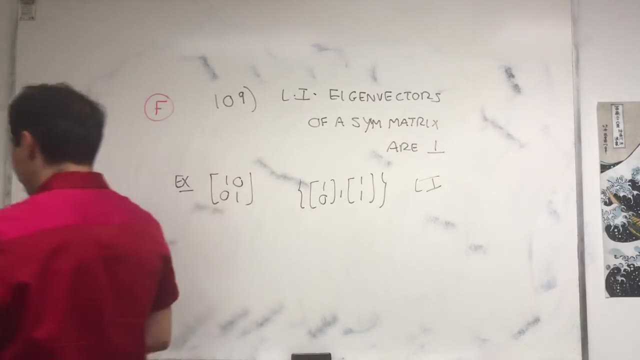 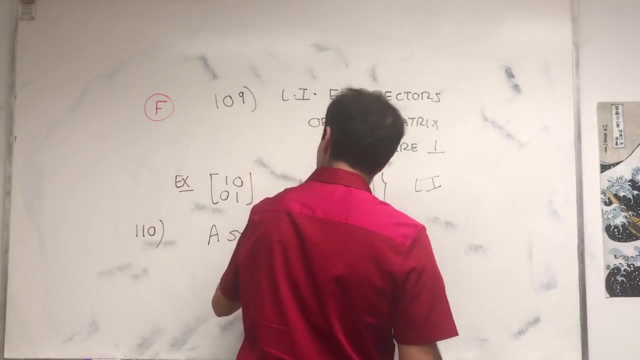 Well, those are linearly. it's a linearly independent set of eigenvectors, But it's not orthogonal, So it's very important that it corresponds to different eigenvalues. Okay, oh my god, almost done. penultimate question: a is symmetric Implies a is orthogonally diagonalizable. 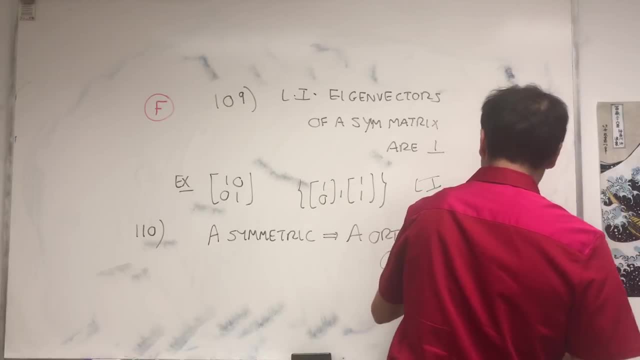 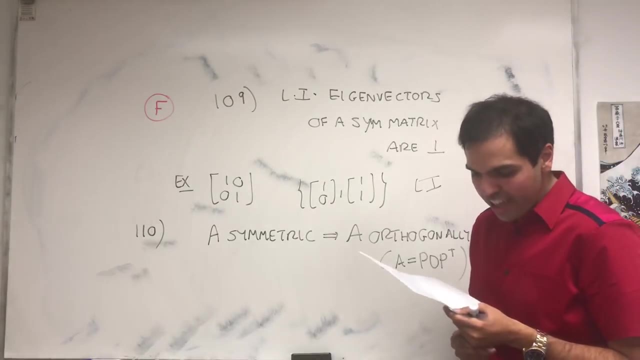 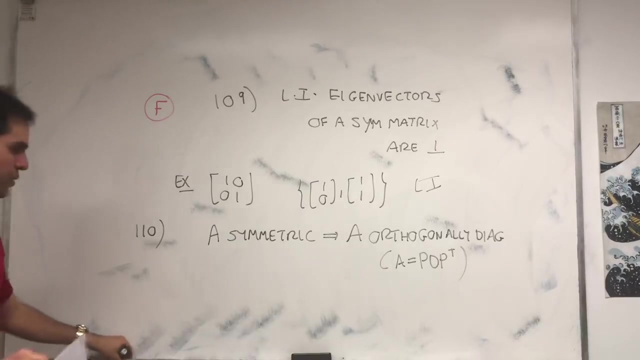 So that means a is PDP-transparent transpose. So 110 Icelandic. I like their yogurt, So I think, Indeed, this is true. That's one of the fundamental things about symmetric matrices. And the question is: how can you find P transpose? Well, first of all, diagonalize a. 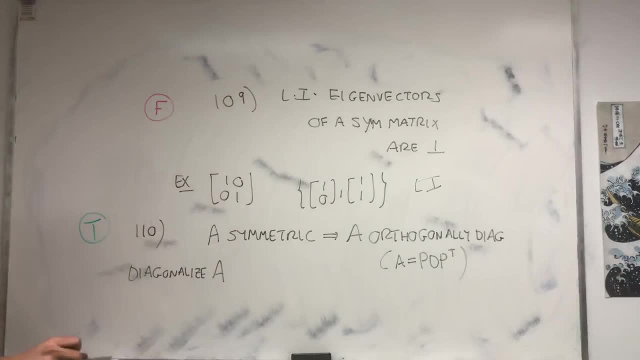 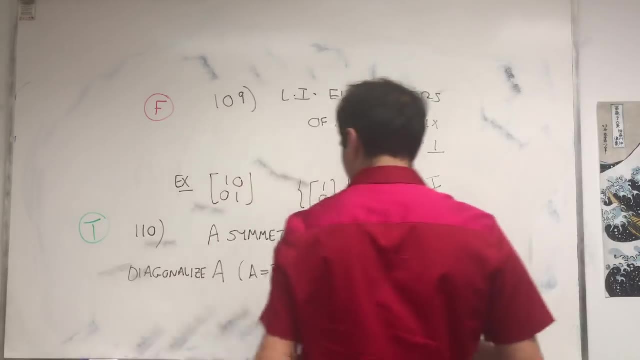 and those give us, you know, a linearly independent eigenvectors, So we get a equals to PD pin right. so you get, you know something, maybe your eigen space, andar yaAN, and then Eigen space of Lambda 2, and Again, by one of the questions, we know that if you're different, you're perpendicular and 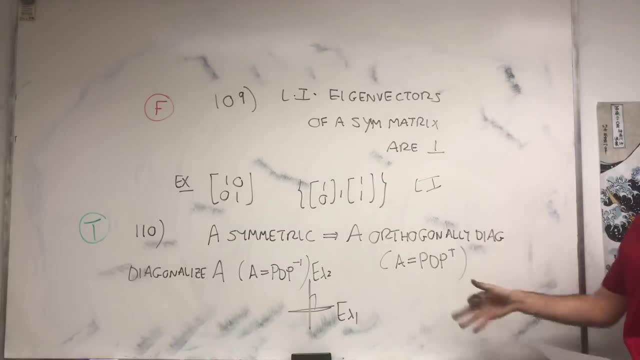 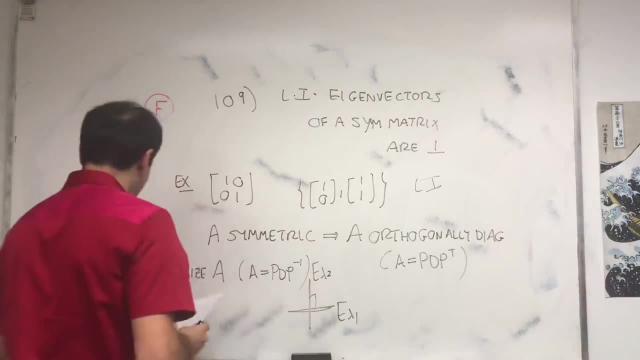 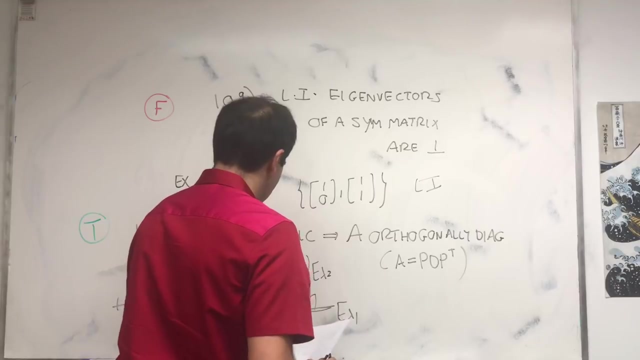 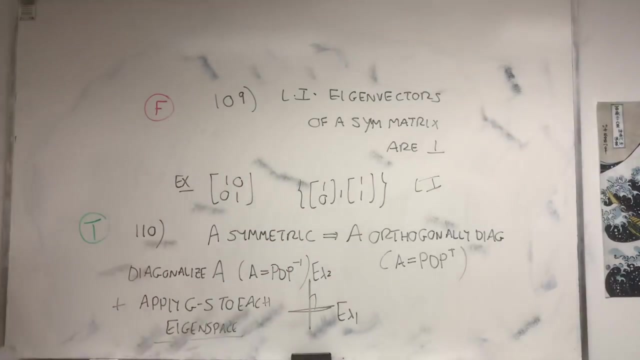 so really, to make sure that the columns of P are orthogonal or mirror from normal, are you have do is then apply Gram-Schmidt to each eigenspace. Apply Gram-Schmidt to each eigenspace, Because here's the thing: If you apply, let's say, Gram-Schmidt to E of lambda 1, you get an. 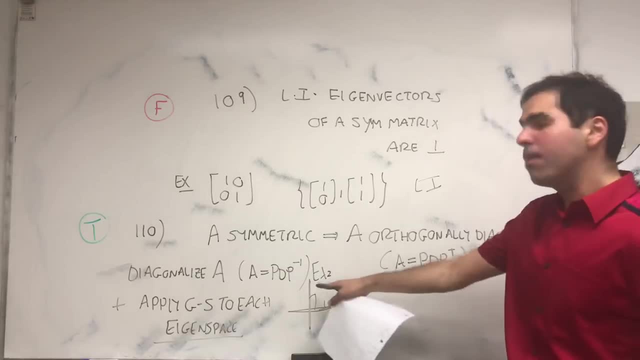 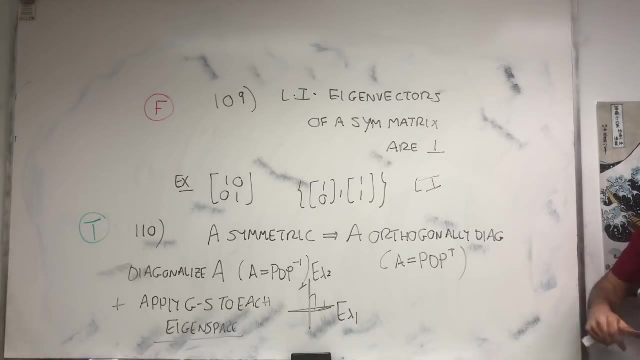 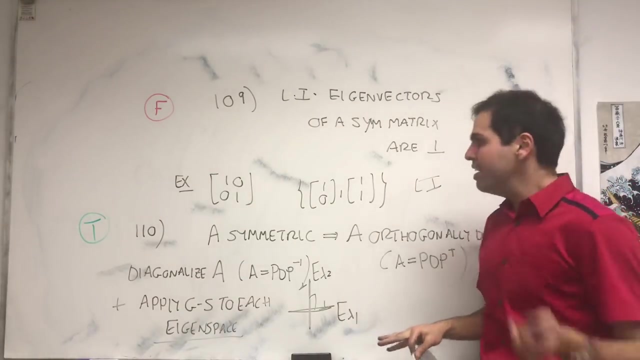 orthonormal basis for E lambda 1. If you apply Gram-Schmidt to the other space, you get an orthonormal basis for the other space. And now it's not clear usually why. if you put them together you get an orthonormal basis of all of Rn. But the beautiful thing is for 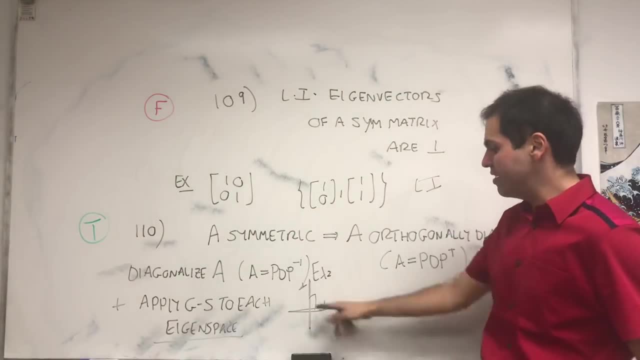 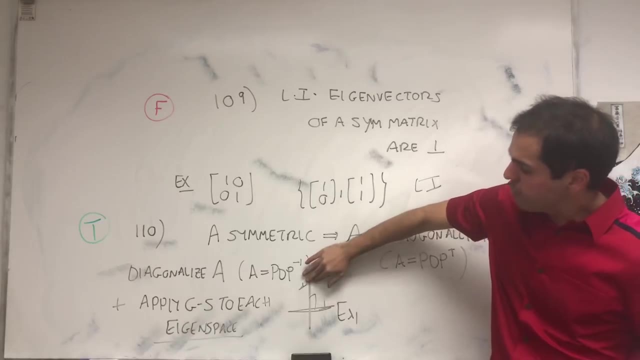 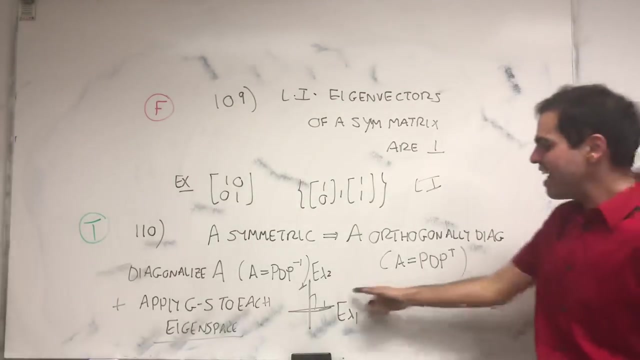 symmetric matrices, you do get an orthonormal basis Because automatically those two spaces are perpendicular. So if you have a perpendicular basis here and a perpendicular basis here and you put them together, you get a perpendicular basis And in fact then your matrix P, because it has orthonormal columns, it's an orthogonal. 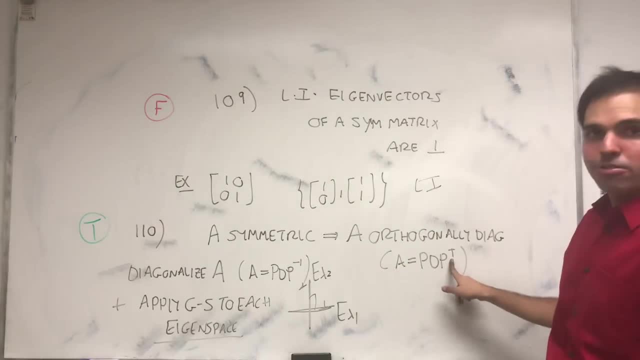 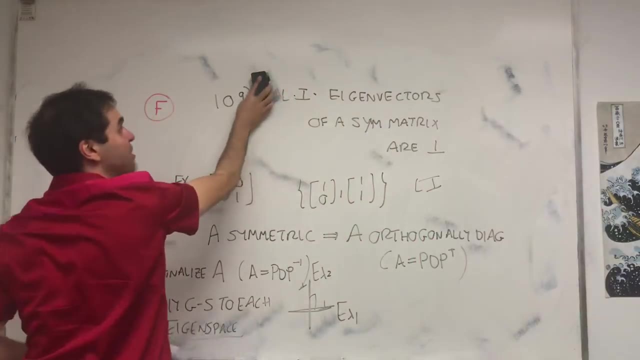 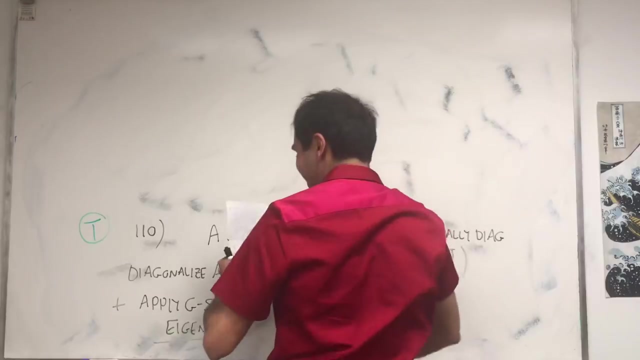 matrix And therefore P inverse is P transpose And that's how you get A equals to PDP transpose. And as a grand finale, I still can't believe this is true. Last question, question 111.. It's the converse. Is it true that A orthonormal 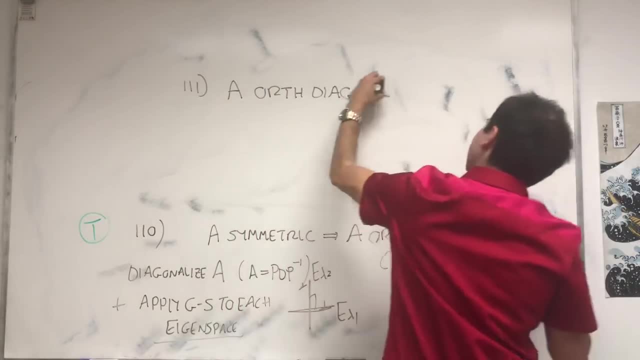 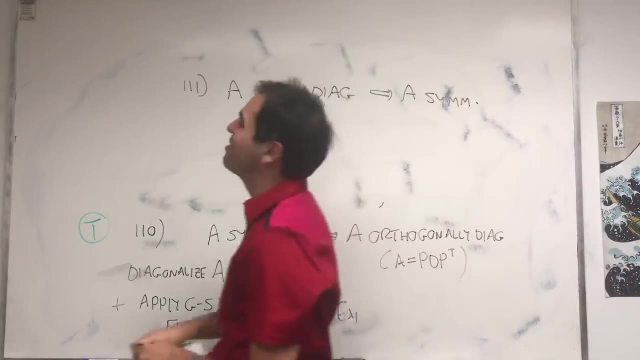 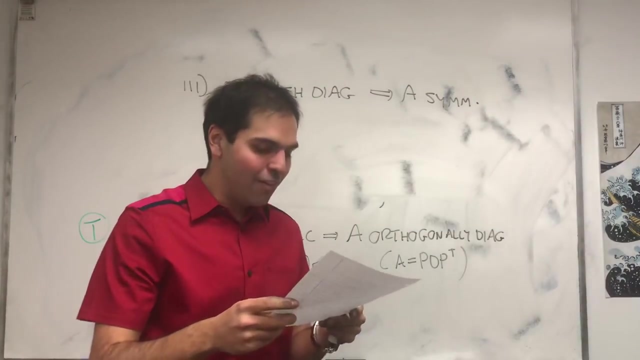 So it's in thing and it is extraordinarily diagonalizable. Does that imply that A is symmetric? And you may wonder what's the last language I used? So drumroll please, Based on the big bang theory. I'll do it in Klingon And it's, I think, wawal, waw maw.